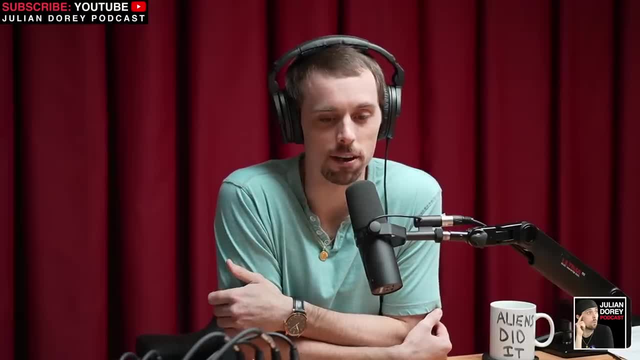 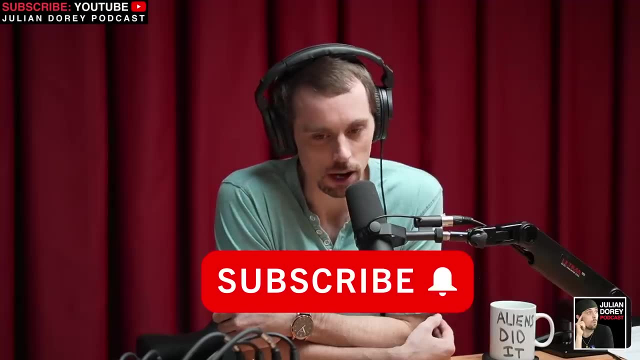 conversations. We had a blast last time. We did, We did. It was a lot of fun. And the night before I had Danny Miranda in town, as I had recorded with him as well, like the day before, And he was pretty blown away at dinner when we were all talking and you were just going through. 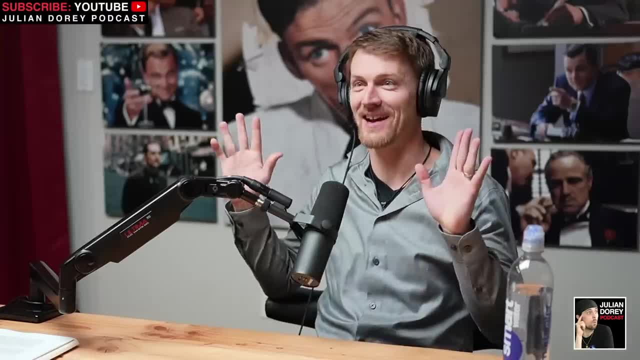 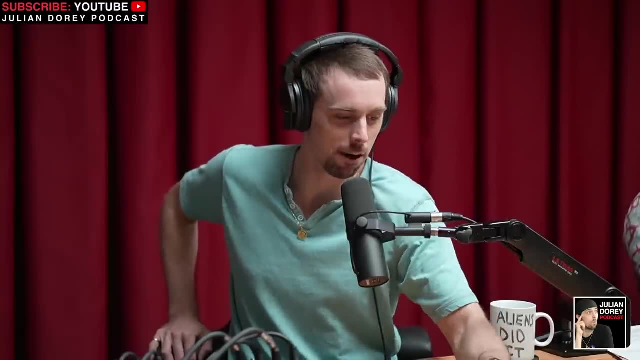 the stuff and just like he's just like sitting back, Yeah, literally, He's like holy. I didn't keep up with this guy, But you have brought some arts and crafts again, as I see. Yeah, Arts and crafts I mean actual, real pictures. of course, There's been a lot that's happened since you and 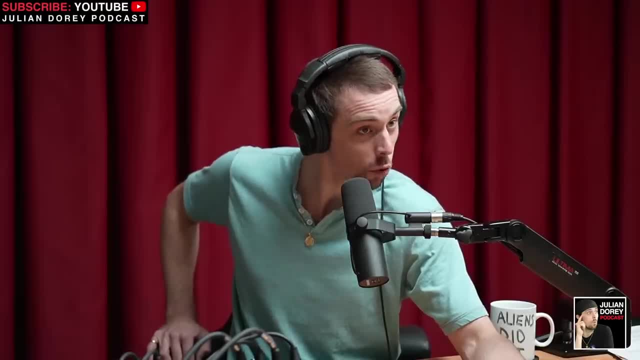 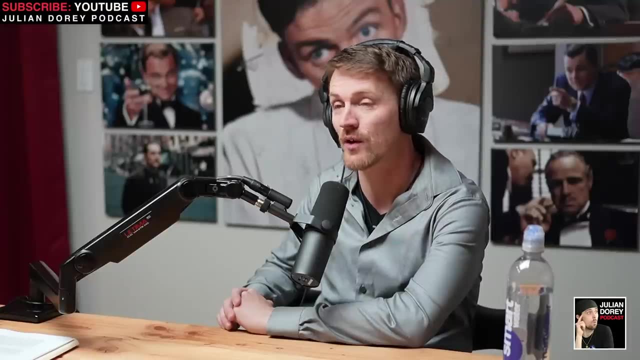 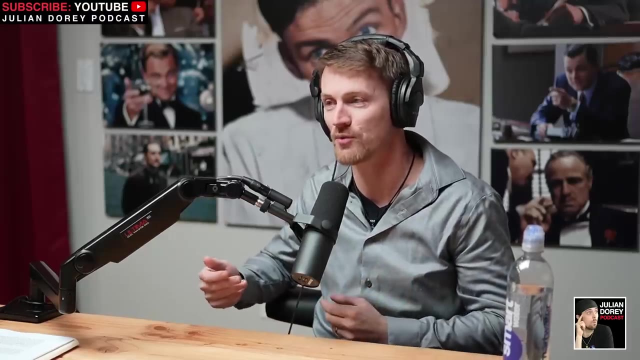 I talked A lot. that's happened, as in. people have found new things. I have found something very, very significant to add on to A lot of our other conversations. So part of, I think, the purpose of this. you could call it, I don't know, part two, part three, depending on how you want to. 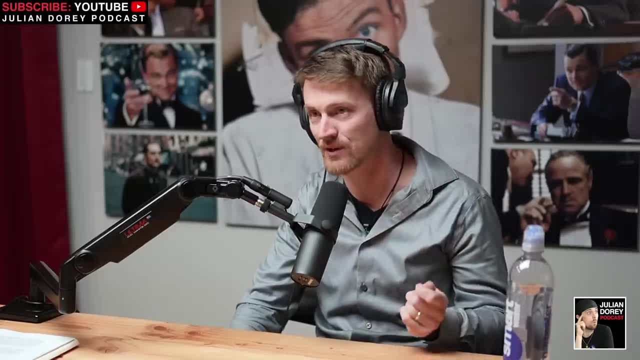 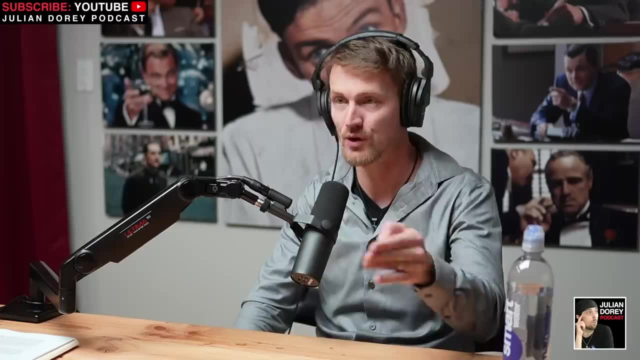 label it is. we're going to be expanding off of a lot of what we talked about, but adding brand new discoveries, things that are even new in the archaeological world, but also new in terms of how they're linked and what they're part of. And I think when I make 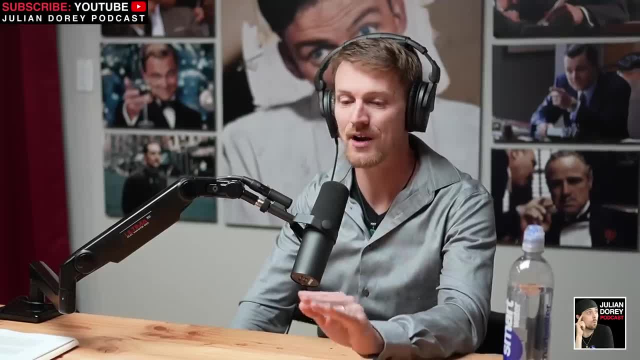 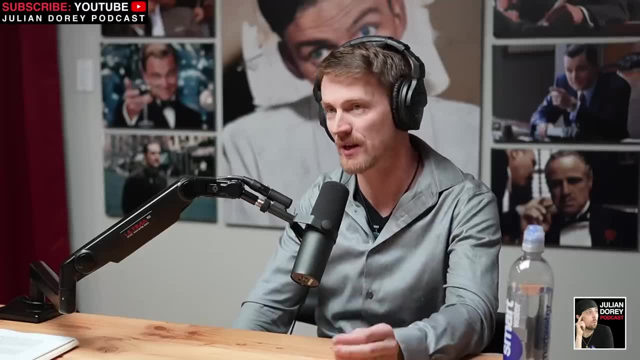 the distinction of saying I made a discovery, I'm not in the field there. I'm not in the field there on site yet, And I say yet with a strong emphasis because that is going to change and we can talk about that. But in the meantime, using every available resource I can, 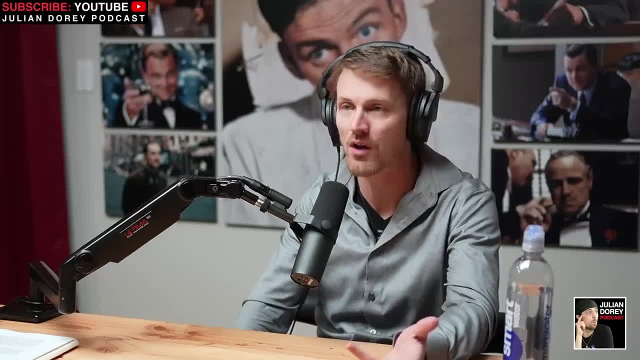 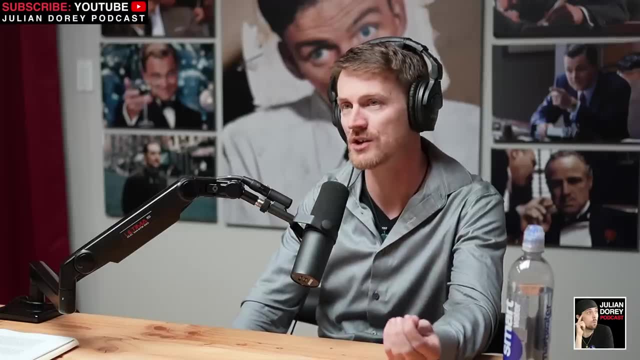 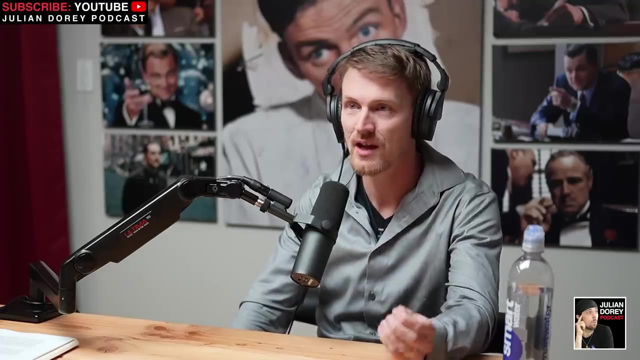 images of people in the field, papers, research papers from archaeologists, satellite images, diagrams- everything possible. with the avenues of technology we have available now, it makes you could call it- being a remote archaeologist more possible than it's ever been. 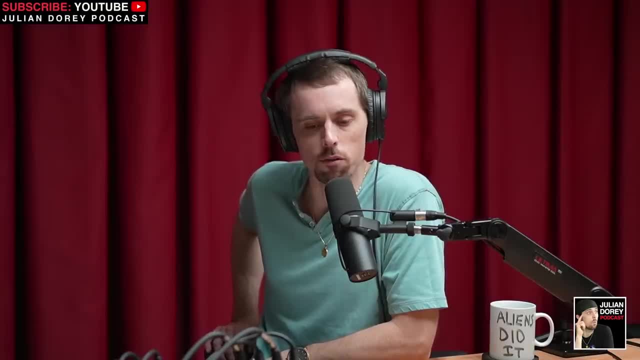 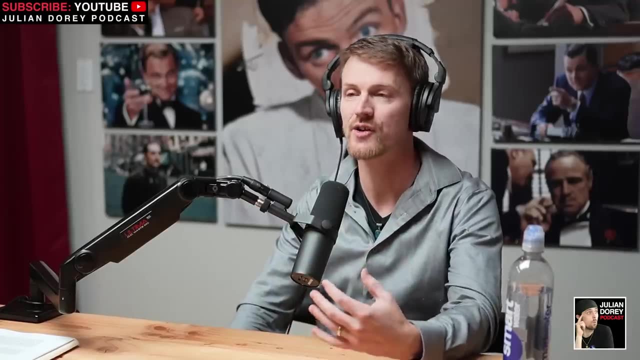 I would agree with that. You can get a lot more information just because of what the interconnectivity we have for sure. So what it means is that it's only going to lead to a greater understanding of what we can- I and others that I can discuss in a second. 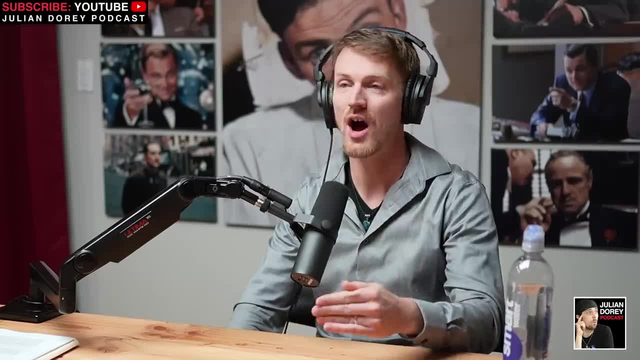 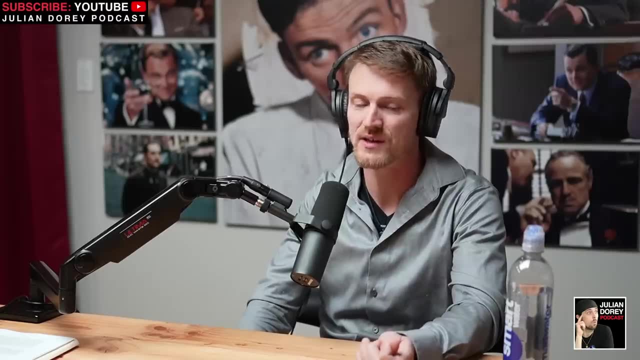 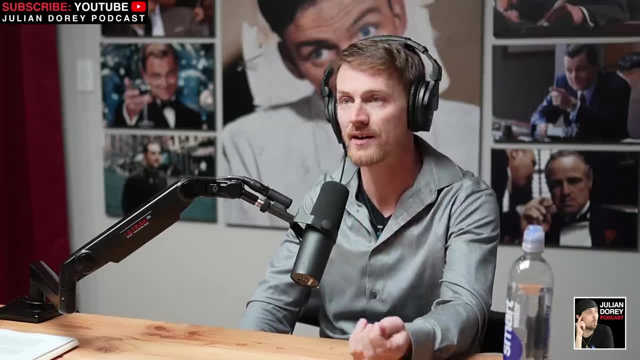 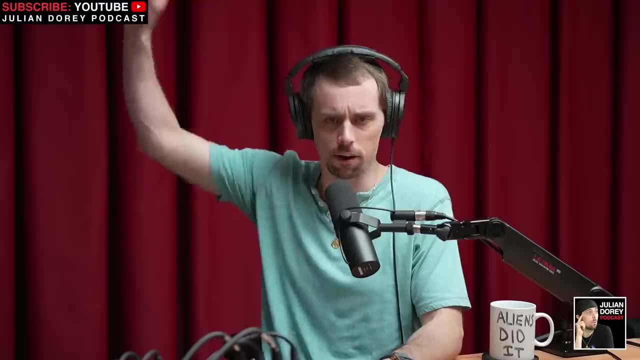 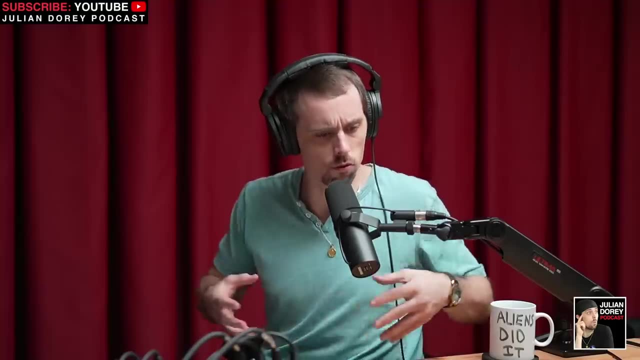 going to do today. we want it to be able to stand alone as well, So people later can go back and watch the old episodes. So I'm going to have to summarize a little bit and sort of bring back some of that, Yeah, And there'll be some things that we'll rehash quickly that we really unpacked. 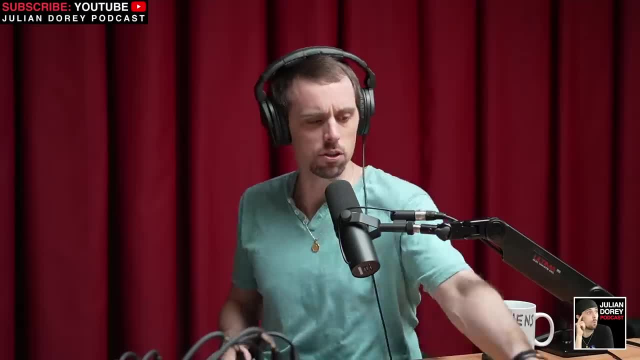 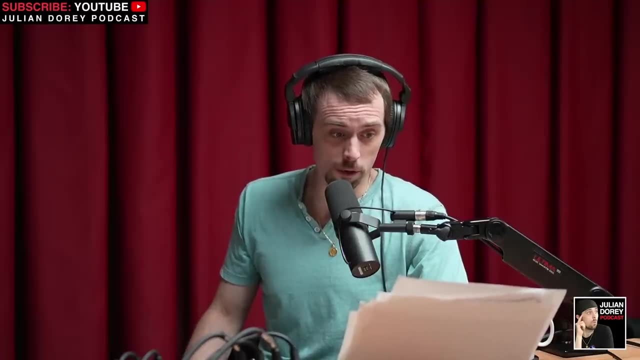 last time we were together over the summer. But I did want to start off with what we were talking about right before the jump here, which is this top picture, This top picture. So we'll put this in the corner of the screen so that people can see this, But 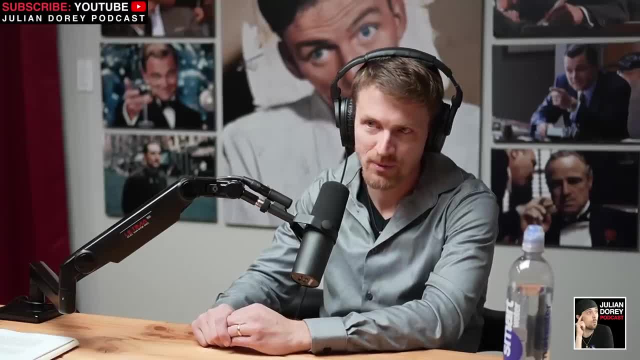 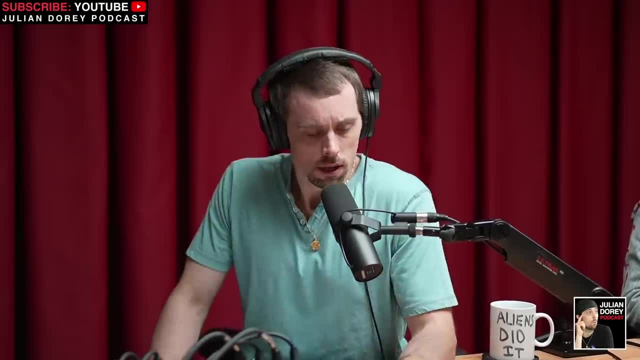 what are we looking at, Matt? So can I give a little background on that first before we jump into that? Yes, Yes Is after you, and I did that last podcast. when was that exactly? It was six months ago, or I think. I put them out in the. I put them out while I was starting to move, So I put one out. right before I moved and then waited three weeks and put the other one out. I think it was end of July. Okay, Summer, Yeah, Right, Yeah. So we talked like early July, I think. Okay, Okay, Okay, Okay. 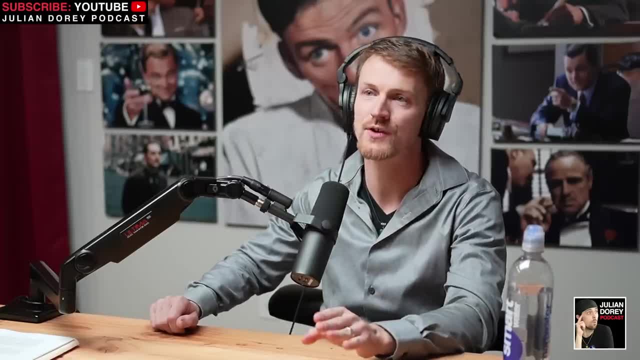 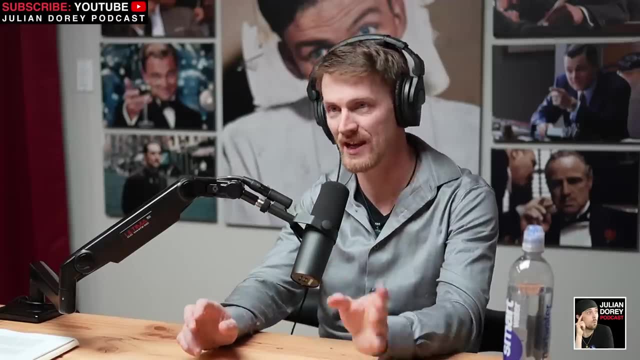 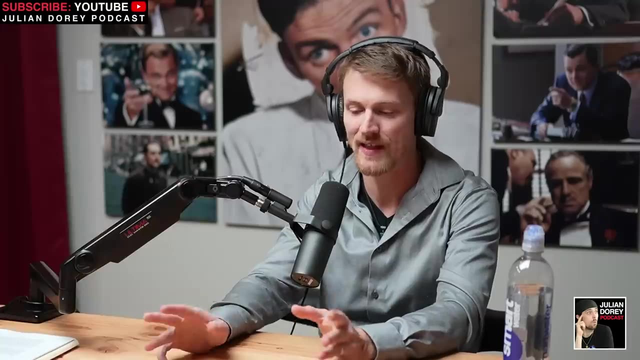 Okay, Okay, Maybe month or two after you and I talked, I was doing some detailed study on one of the ancient sites that I had talked about And we'll give some more background as we go along And as I was doing study on that site called Kef Temple, and we'll talk more about what that means and what. 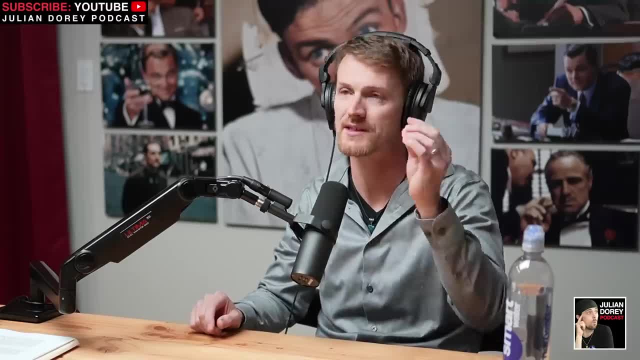 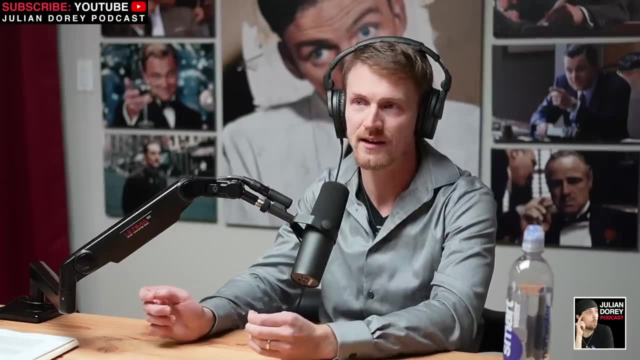 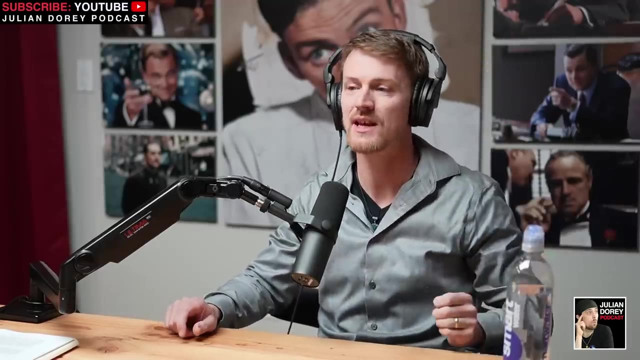 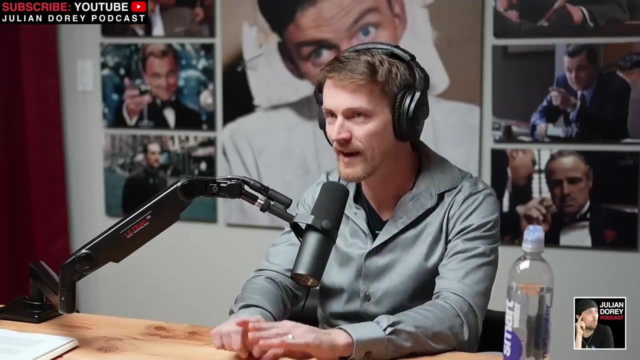 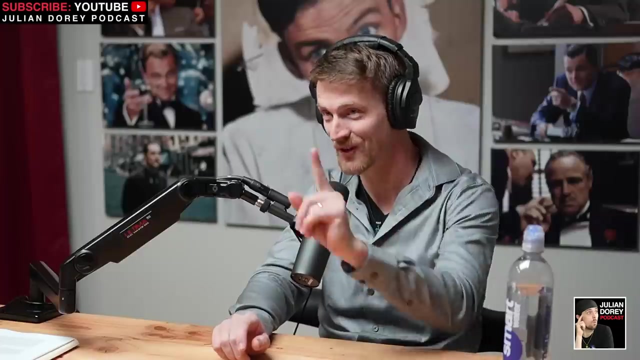 the significance of that. But when I was reading the archaeological papers from the excavations of that site, they had mentioned in it that you know, there was a site called Kef Temple. And I said that there was another site that I had never heard of yet that had even finer stone masonry work, even more advanced than what I was seeing. And I saw the name and I immediately went to search for it. And when I saw this temple I had what I call a George Smith moment. Okay, George Smith for a little background. 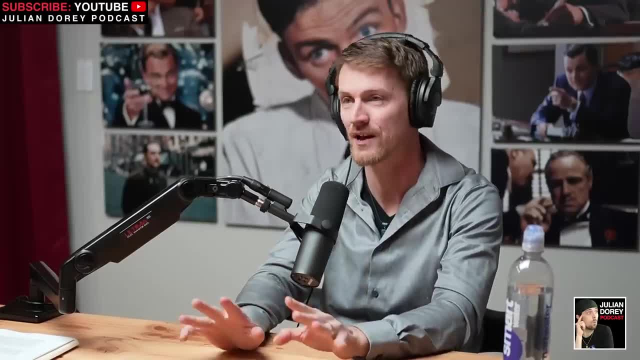 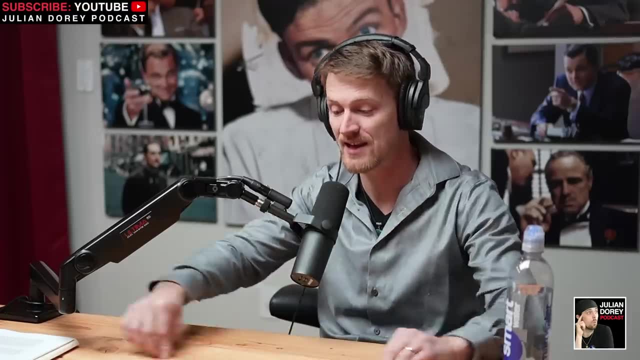 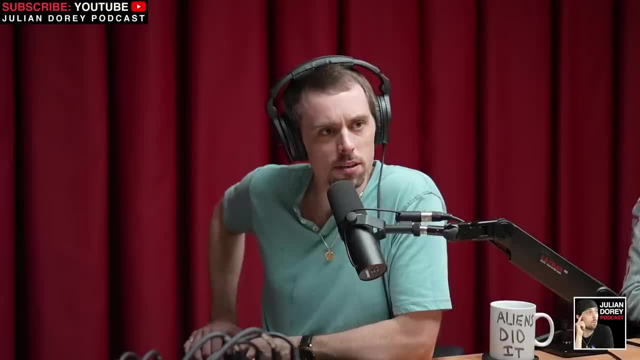 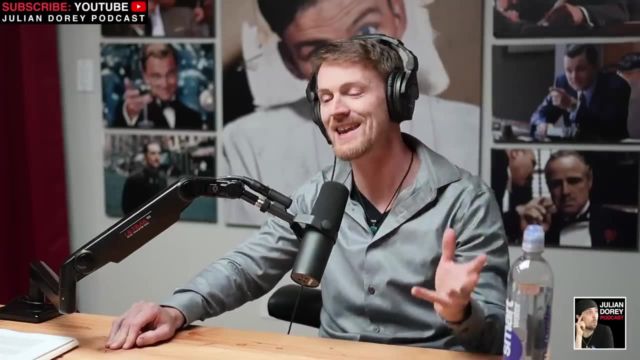 For thousands of years, Right, but he found it mid-1800s. Yeah, so it was found in the Royal Ashurbanipal Library in 1849 by a man named Austin Henry Laird, and he brought all these tablets 30,000. 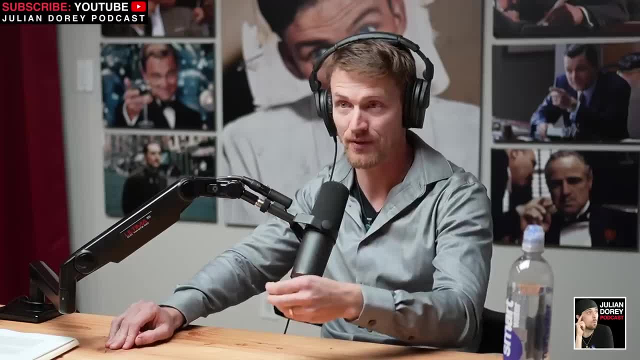 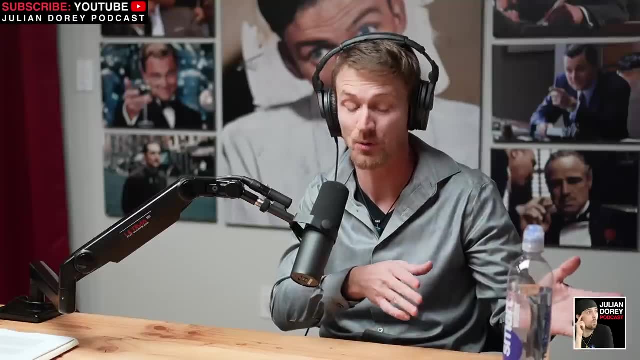 cuneiform tablets to George Smith because he was the expert on translating them. Austin Henry Laird didn't know how to translate them. He just found them in the ancient library of Royal Ashurbanipal Library in what was called Nineveh, Iraq. 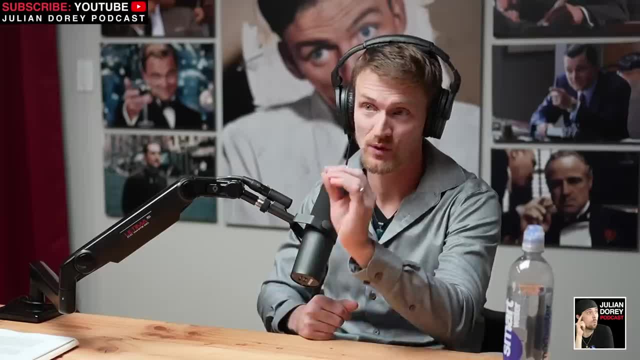 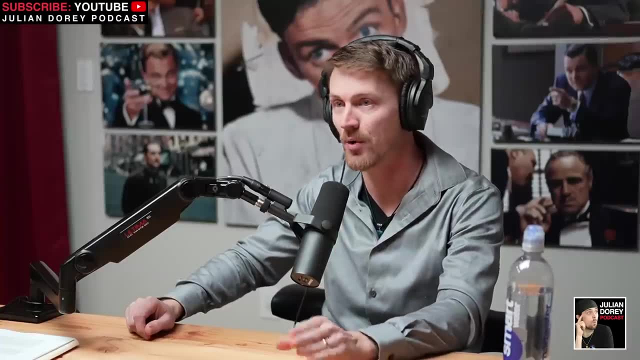 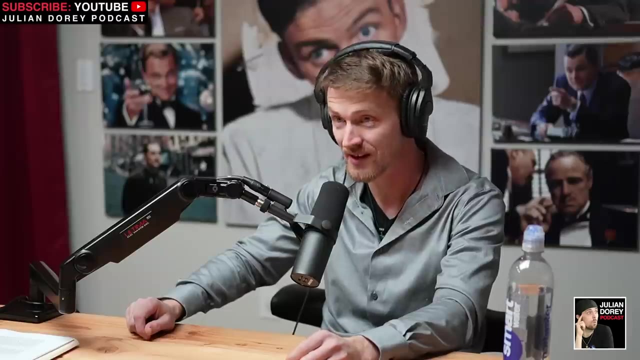 Today that'd be known as Mosul. That was the most. and it's HG Wells, the famous writer. he actually called the Ashurbanipal Library the greatest source of historical information ever in history. Really, Yes, That's his quote. 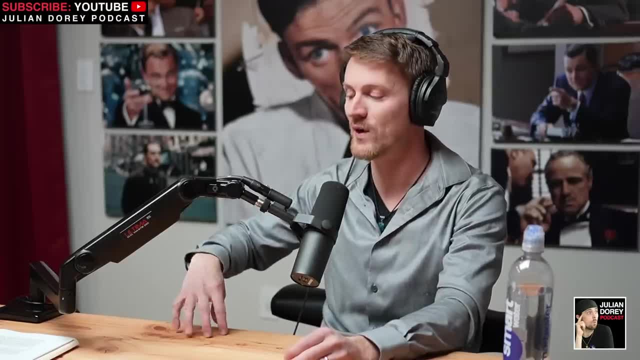 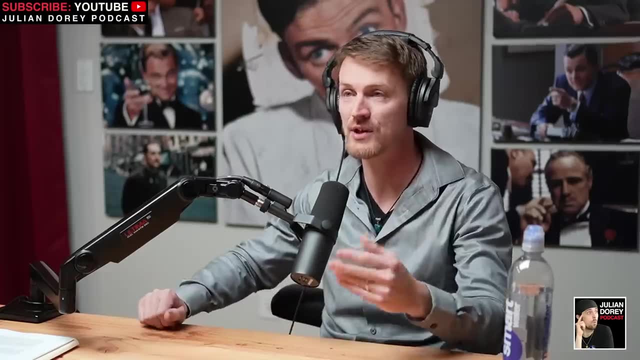 Now, what made him say that? Well, even if we, the general consensus, the general population now hasn't heard of it, There's a number of reasons for that. It's fine, But certain scholars throughout history, certain academics, he was a very smart man. 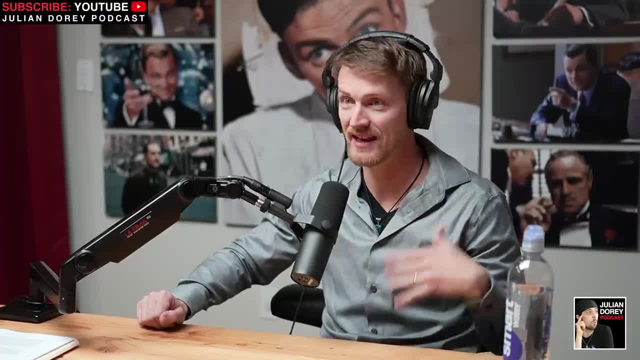 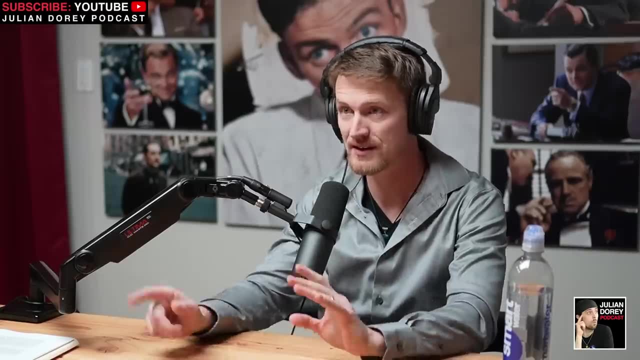 HG Wells was a smart dude, Oh yeah, He was dabbling in some ancient stuff, Okay, And he had found, being a writer, he had found the details of this library and realized what was contained in the library, and because he knew, 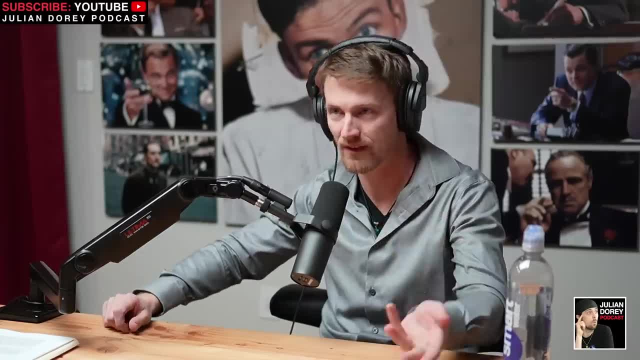 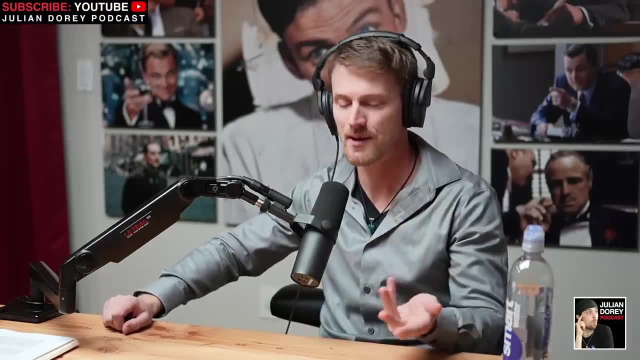 that he then made that statement. So what was in the library? Things like the Epic of Gilgamesh, the Atrahasis, the Myth of Adapa, Eridu, Genesis. Some of those might not seem like anything, or no one's ever. some people. 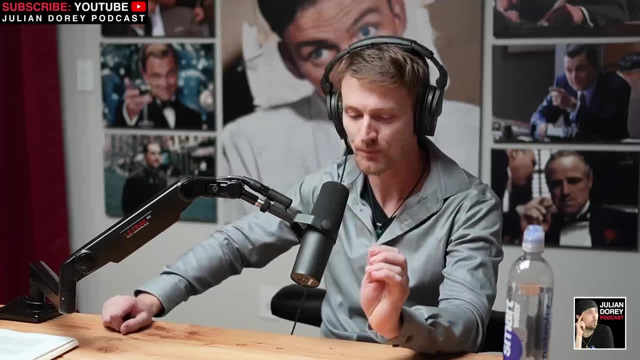 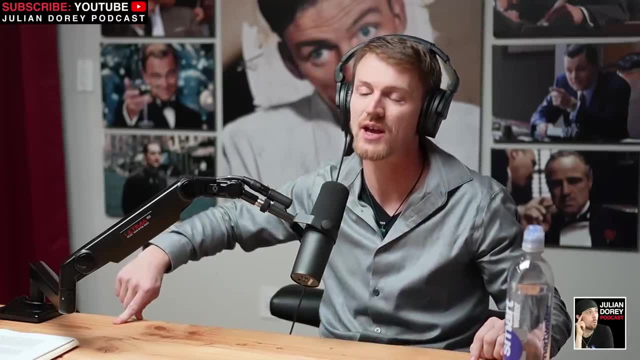 listening to that, might have never even heard of those names, right? But when George Smith cracked how to translate those tablets, the first one was Epic of Gilgamesh. he had broken a code that hadn't been broken in over 2,000 years. 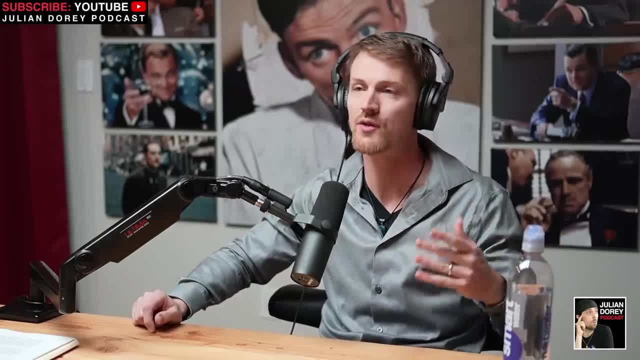 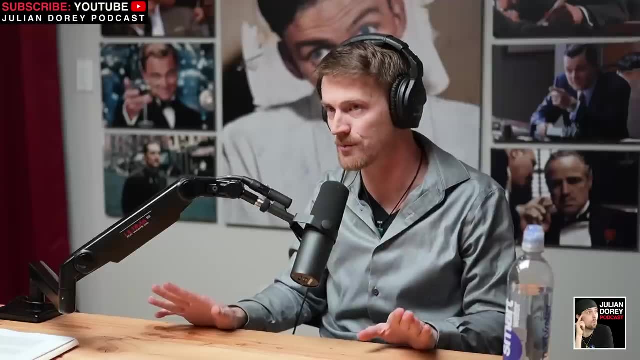 So if you go to Iraq, like, let's say, 500 years ago or 100 years ago, right, And you go up to someone that's been living there for generations in their family, they would have no idea how to reach Sumerian. 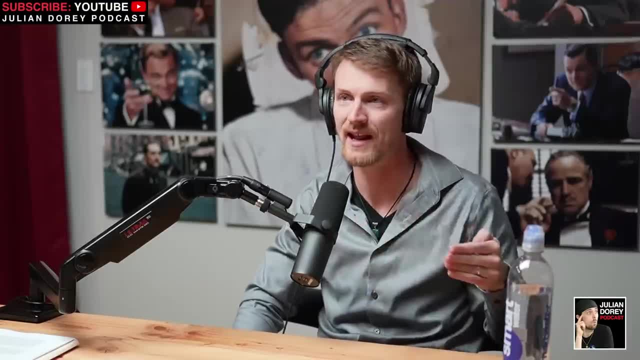 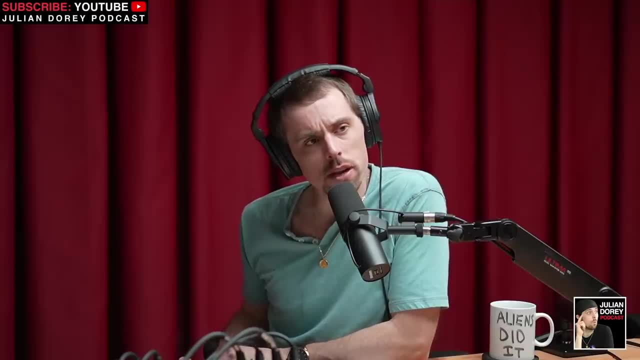 This is not like other languages in the world where there's a common ancestral connection, where they can kind of figure it out. It was literally alien and unknown. Who was 2,000 years before, who was the last person, or the last people, I should say, who were around? 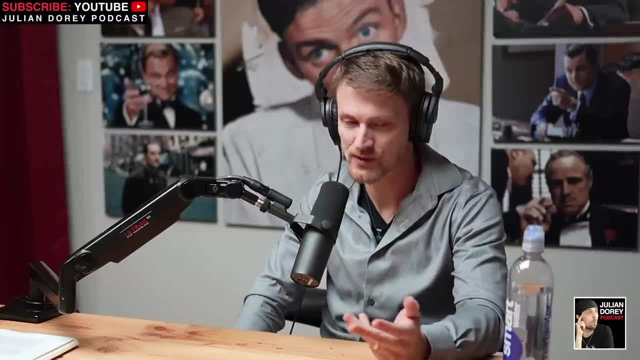 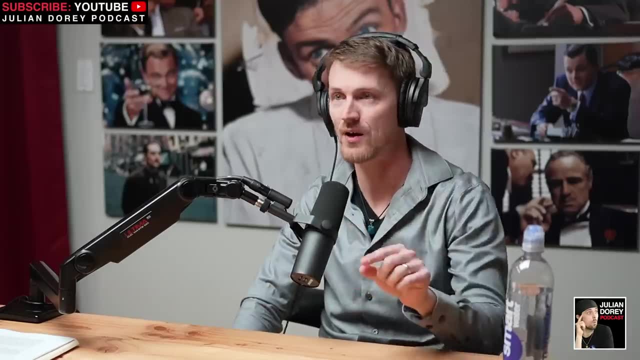 it and could translate it. Well, that's where it gets interesting, because we're often told that the Sumerian civilization existed 6,000 years ago and they put this window on that region. But what I've found in this part of the evidence? 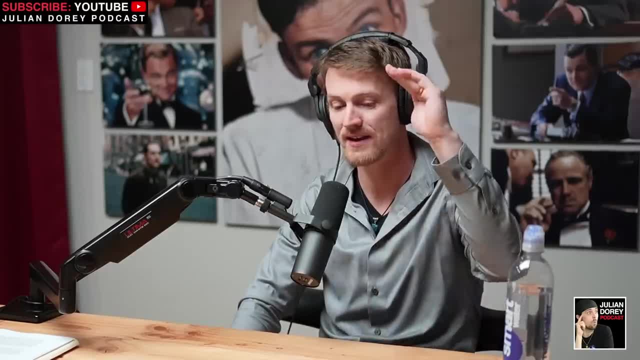 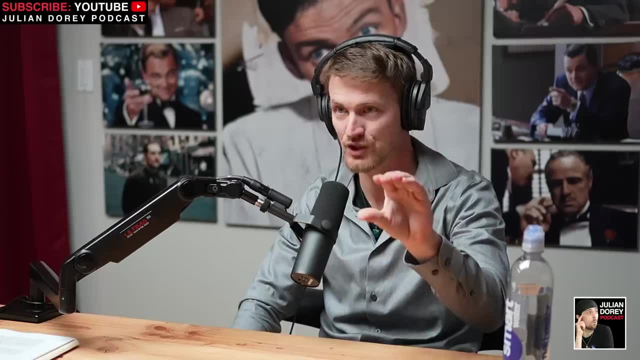 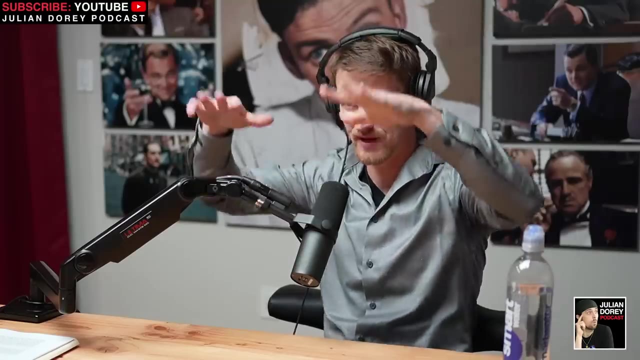 that directly correlates to these discoveries is that there have been three definitive- and I want to make that very clear- three definitive civilizations that have been in that region over the course of thousands of years, who have built on top of things, kind of eroded and been destroyed, and then another culture. came and built on top of them. But the thing that was interesting about when Penn University went into Chirupac, that we'll talk about one of these ancient Sumerian cities to try to figure out where the city, if it was real. if it was a myth they found as they dug down. they had to go 35 to 40 feet down to get to the original base of that first city. And what's the significance of having to go that deep? It shows you how ancient and old it is. 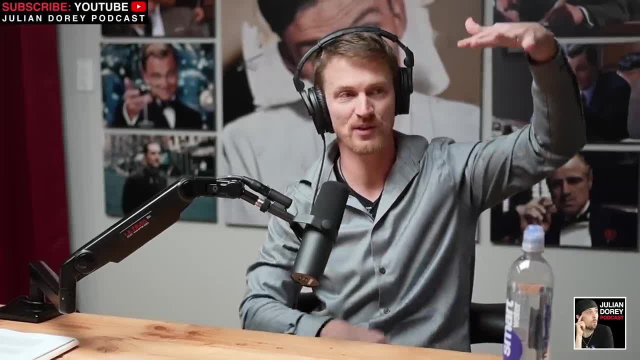 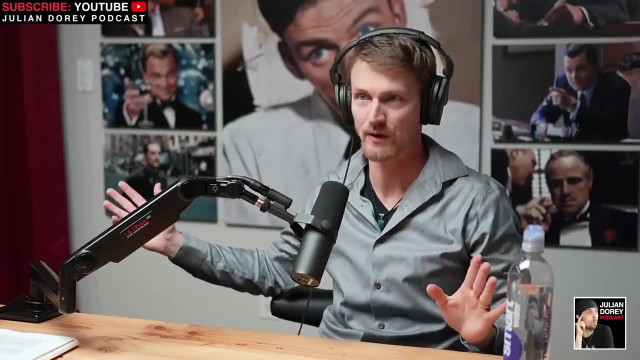 And not only that, but it showed- they discussed in the papers- how there was a 17-foot inundation layer That they found above these ruins, showing that there had been a massive catastrophe flood, that it laid down this huge amount of sediment mud. Now the reason I'm trying to 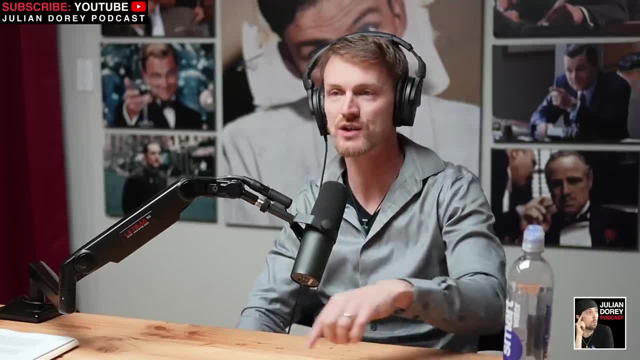 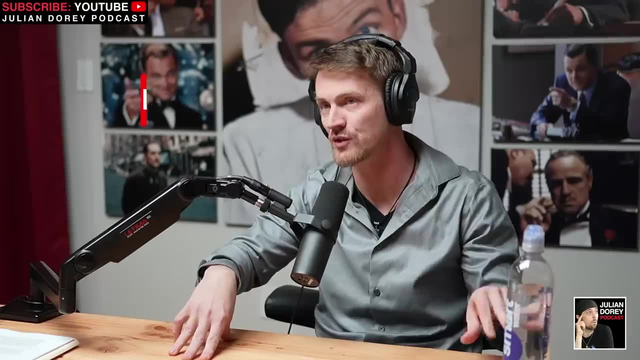 tell you. all that is just to loop back is that George Smith translated the Epic of Gilgamesh, the first set of tablets ever, And the Epic of Gilgamesh has an original Sumerian version. And he, when he read it: 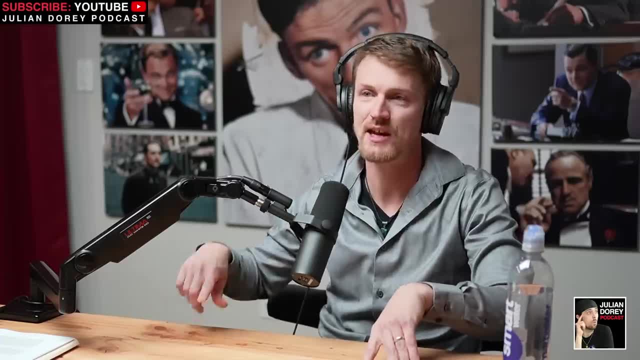 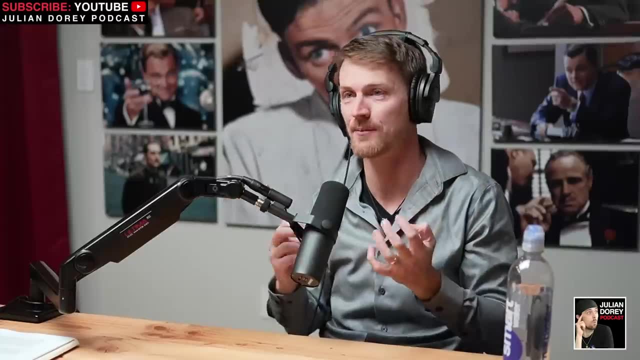 and he realized what was in it. it's described that he ran around the room like multiple times Like ran around the room, okay, Because he had realized he had cracked something huge and significant. Dear heavens, I've got it. 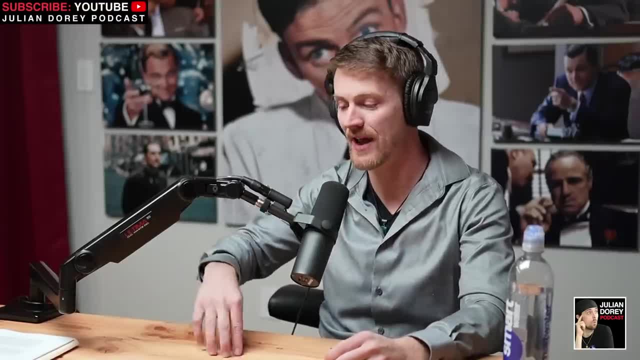 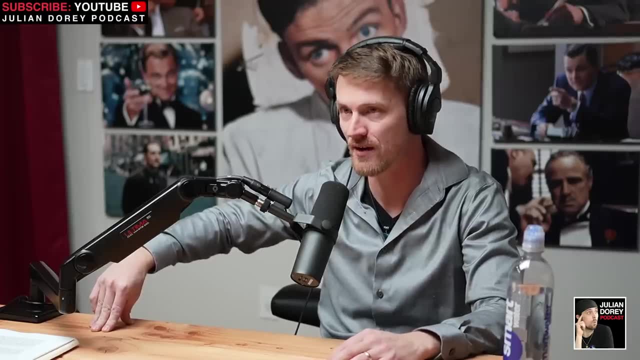 Well, but after that point, he mastered how to translate Sumerian, and then translated all the other sets of tablets, And what he realized is that it was literally the origin of our most ancient stories. What made him think that, though? Well, because he already knew that. Sumerian civilization was the original, oldest civilization on Earth, And I'm not arguing that either. I just think that there have been three iterations of civilizations there and archaeologists have confused the wrong one with dating and time periods, with not understanding that. 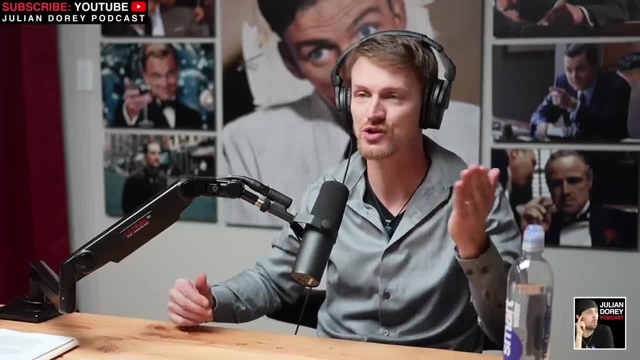 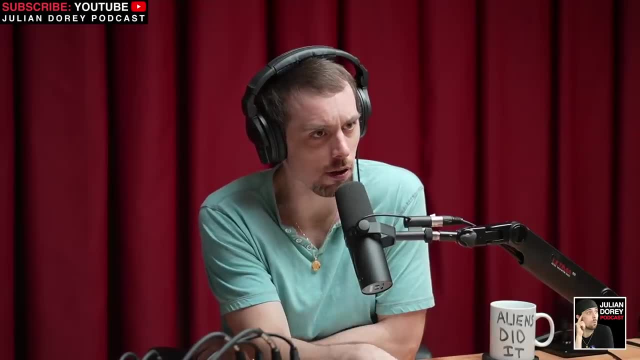 instead of one. there's three that have been there And if you're trying to understand what the original one was, it can be confusing. And how long ago are you saying? you may have said this a couple minutes ago. I just want to follow up. 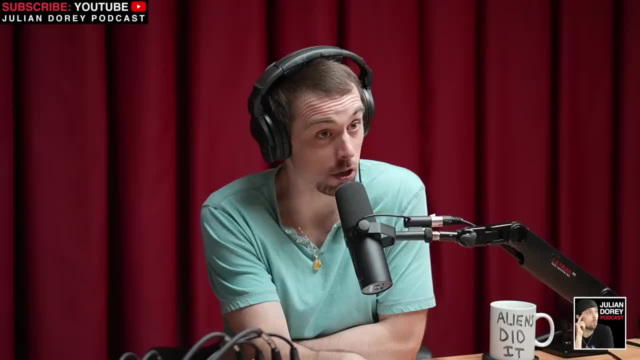 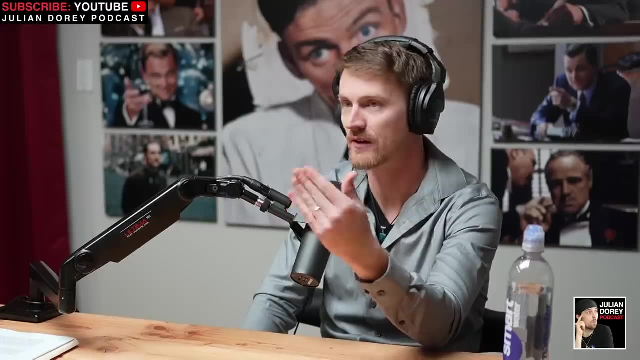 how long ago are you thinking that they are, versus how much history thinks it is 6,000 or something. So right, History thinks that the Sumerian civilization, which is true, they invented nearly everything like mathematics, agriculture, astronomy. I agree. But I just think that dating is completely wrong. So, instead of being 6,000 years old, I think it's over 20.. So what makes you think that? Well, we're going to get into the nature of the stories themselves, what they say. 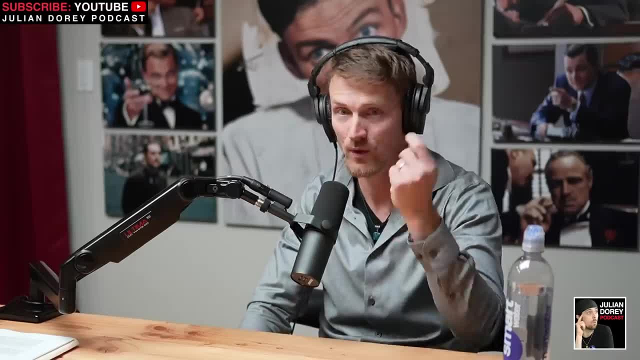 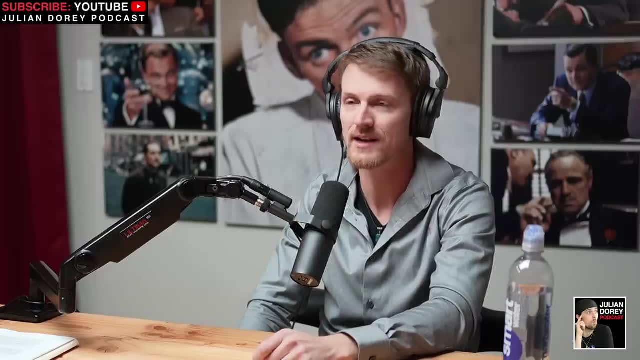 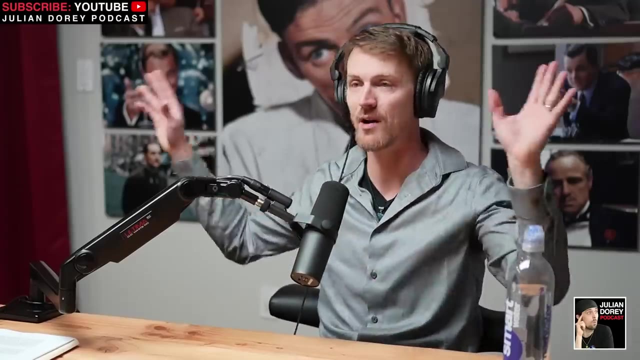 the actual evidence from these new discoveries with bloodlines and these descriptions of what happened and how they seem to be piecing together an origin story from an entire epic that we don't remember anymore ever existed. Imagine for a minute, you know, think about our civilization right now, right? You have that amazing picture of New York City next to us, that huge one. Imagine: 1,000 years goes by, 2,000 years, 5,000 years Long time, 10,000 years Long time. What would be left of New York City? 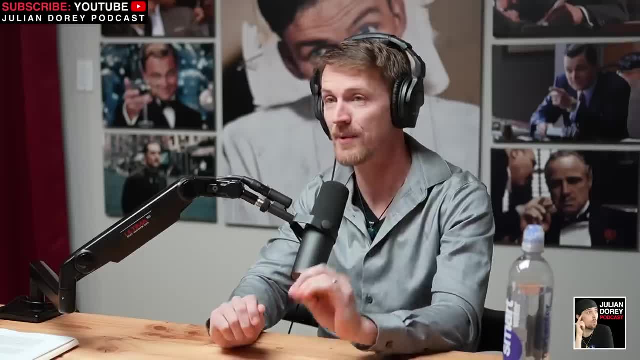 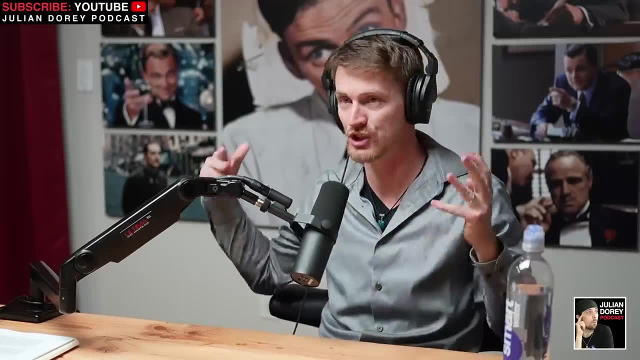 Not much, And we've talked about this a little bit in our other show. But if you imagine glass, metal, things like that, they erode very quickly. Things fall apart, Unless you're building at a giant stone, hard stone like. 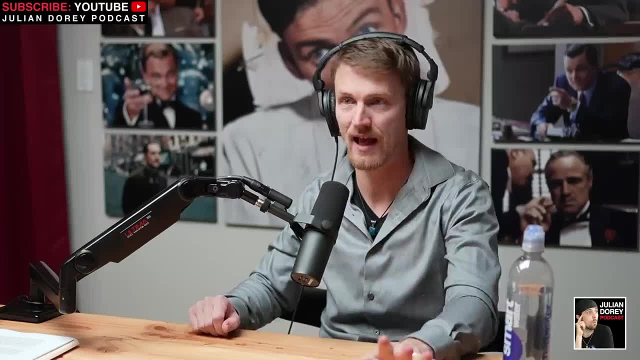 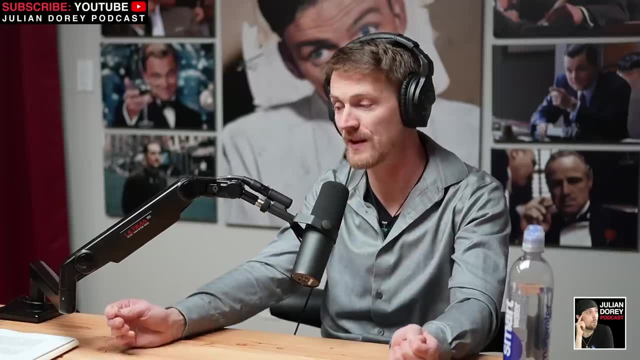 granite or andesite, as we're going to talk about, it simply doesn't last. It won't last the test of time, And what that means is it would actually be a lot easier than maybe the average person thinks for an entire epic or a period. 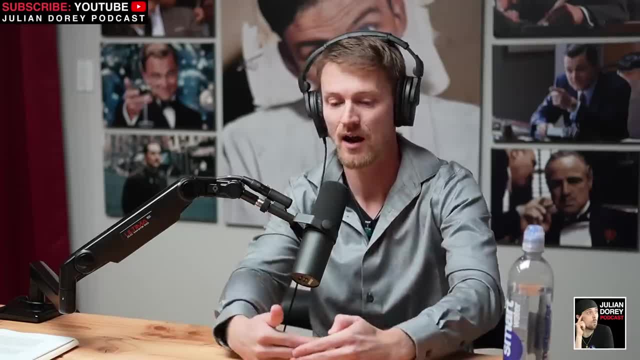 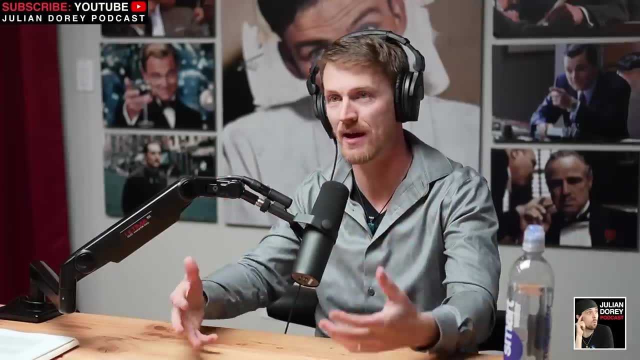 of hundreds and hundreds of years, or thousands of years of us, of a story that we took part in to disappear and then have it be such little amount of evidence left that we almost don't even believe it ever existed. So those writings you said were found in. 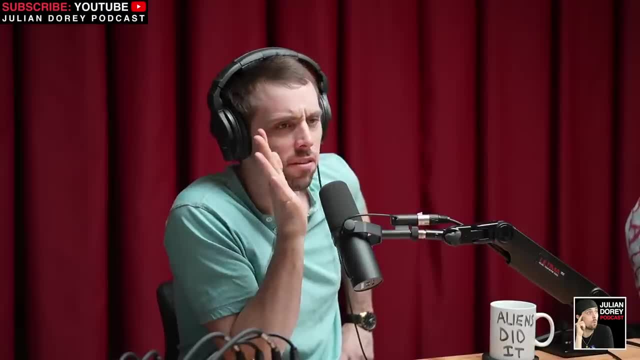 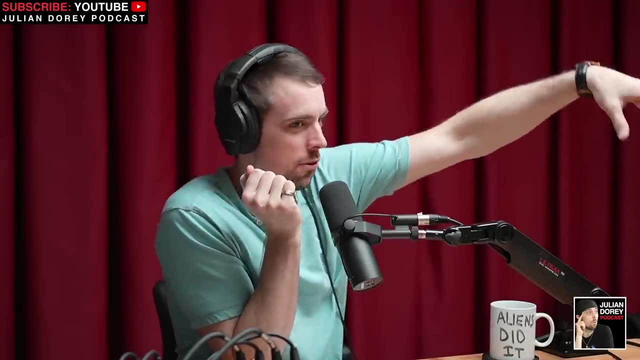 1849, right? Yes, So that is call it 175 years ago: give or take, Right. You ever just stop and think about, even when you're looking, for example, at something like New York now, which is all this big buildings and whatever. 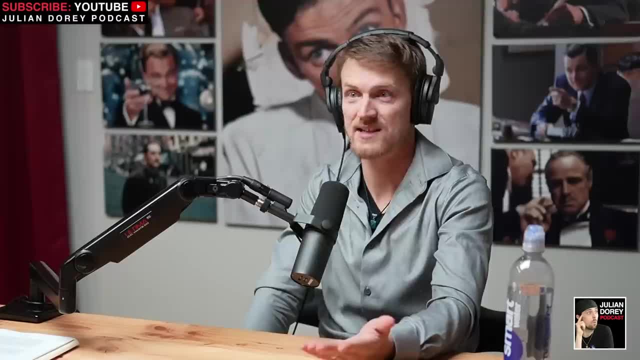 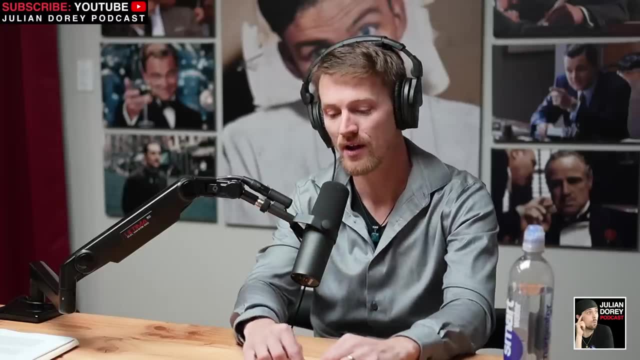 you ever think about how short that is? That seems like a long time ago, But it's literally a flick of the finger, I know, And that's actually a great point to make. Think about how far our society has come in, say, 300 years. 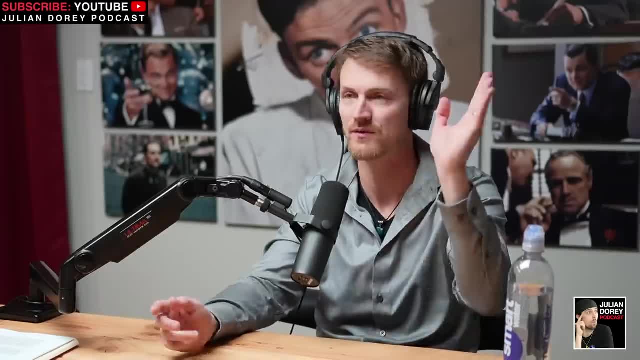 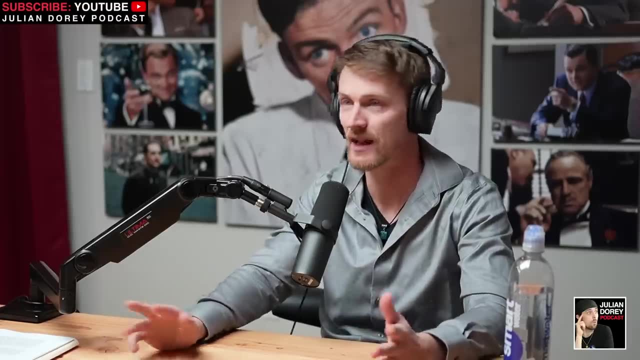 Right, Yeah, Like most of what we know now in terms of technology and all these things that have happened, that have taken us out of our primitive state, have happened in those 300 years. Yes, Right, It's an acceleration, that is just. 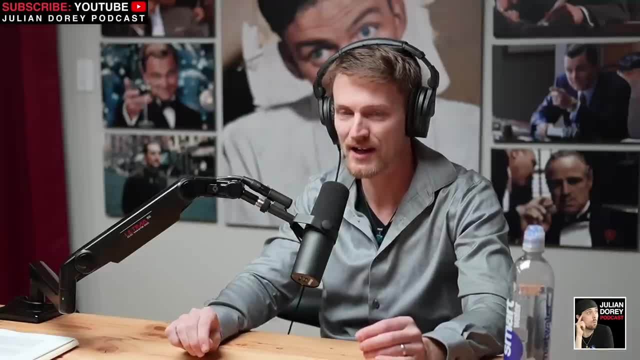 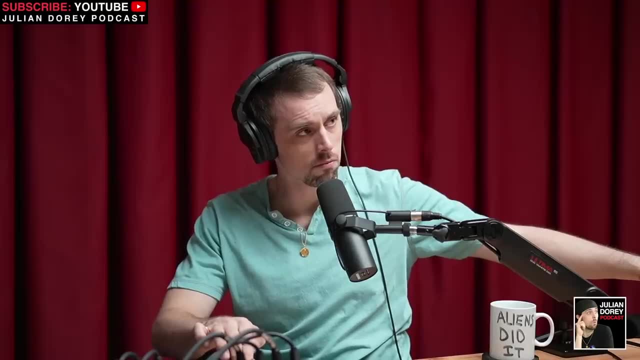 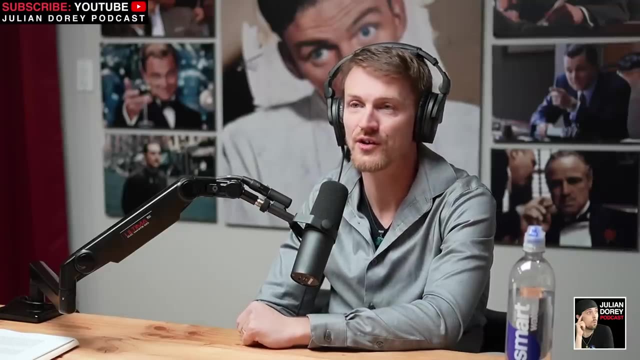 incredible, Yes, Well, but just imagine what they could accomplish in 10 or 20,000 years. A lot of thought, You know, even though we're looking at the fact that we've accomplished all of these things in one, two. 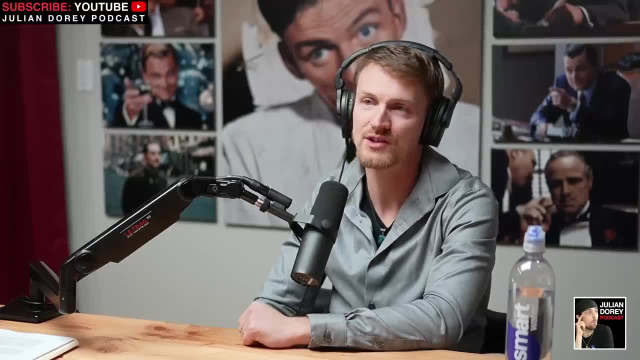 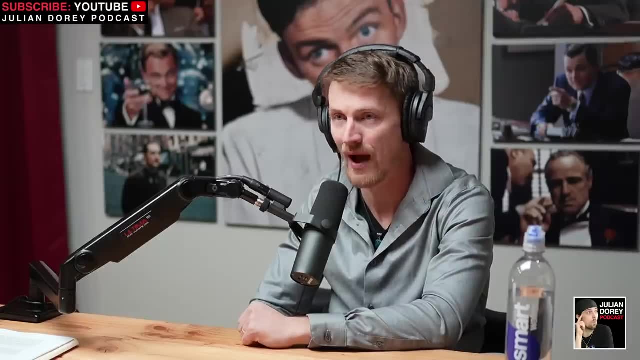 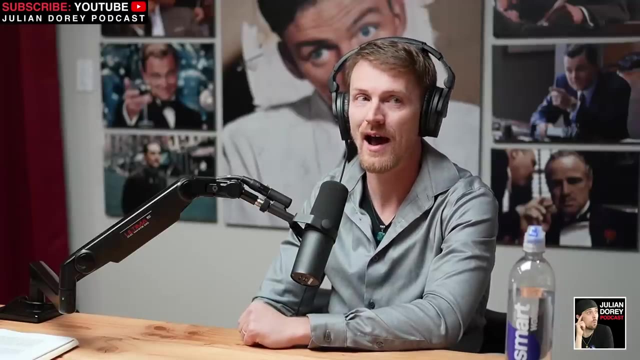 300 years and we're very proud of that. but just imagine what another civilization, in other advancements, in different ways, could achieve in 10 or 20,000 years. And I think that's the point: to look at our own society now and reflect about how. 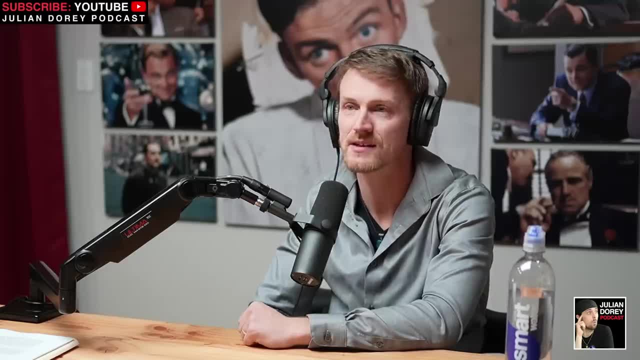 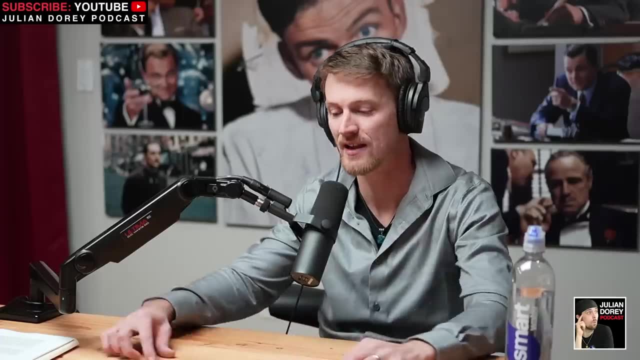 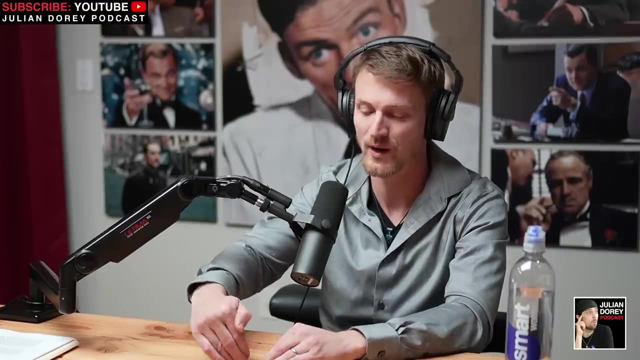 easy it would be to achieve tremendous things but have it disappear and not realize it ever existed in the first place. That's the whole point I'm trying to make, though, is that imagine we have this lost epic of our story that is somewhere, you know, between about 13,000 years ago it ended right. That's when it was the Younger Dry, same as the Ice Age. But imagine that story began 50,, maybe 100,000 years ago And that our entire understanding of history and our origins 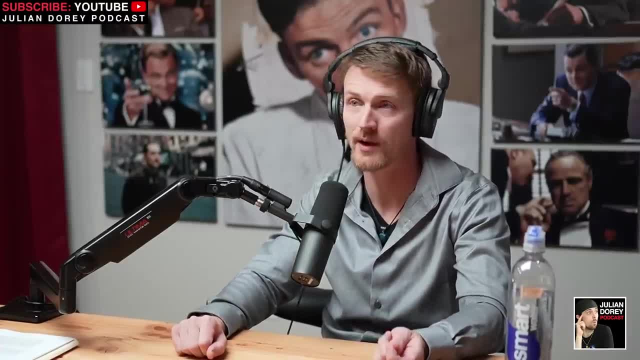 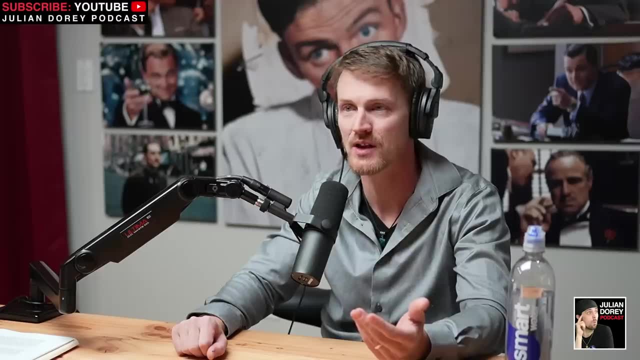 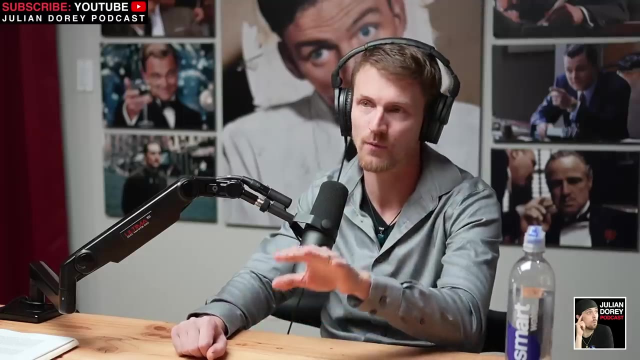 and who we are is extremely skewed, to the point where we actually have very little understanding of what we truly are in the terms of the cosmos and what we are in this microcosm of the macrocosm being something greater, And that's the point of what these 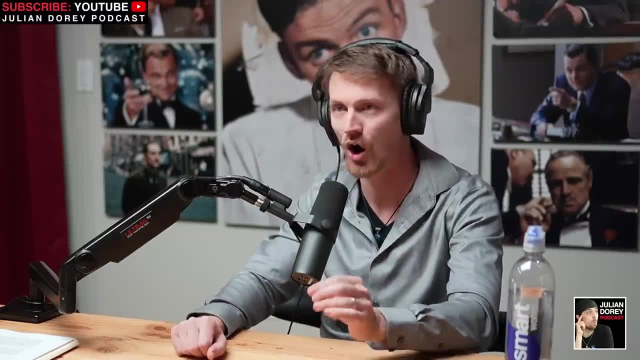 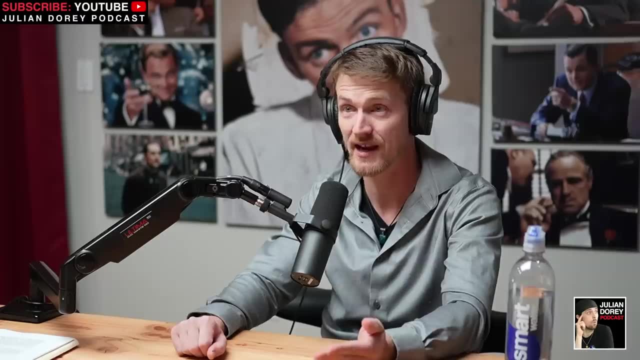 teachings and these discoveries really points towards is our origins and who we really are and what we've forgotten since that point, And that's what makes it exciting. Getting back to George Smith, he ran around the room, like I said, right Because he had cracked. 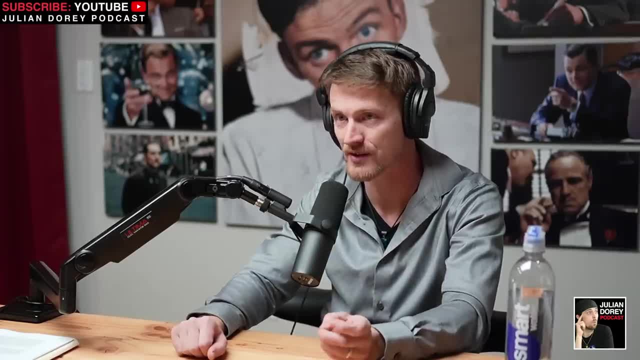 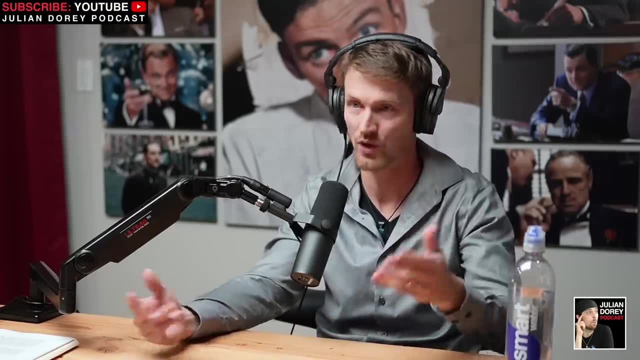 a code that hadn't been cracked in over 2,000 years, This mysterious lost civilization that he felt because of the nature, of how ancient it was in looking around the world and anything else, and knowing that cuneiform, which means the wedge style, 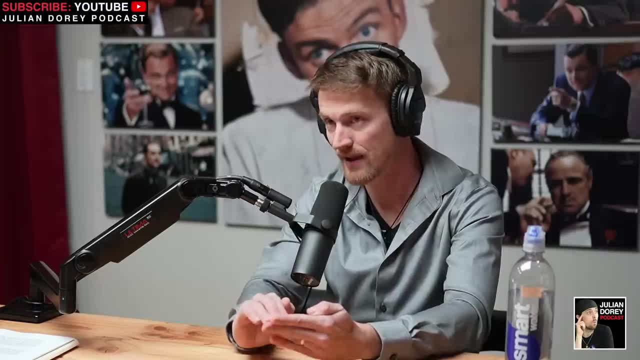 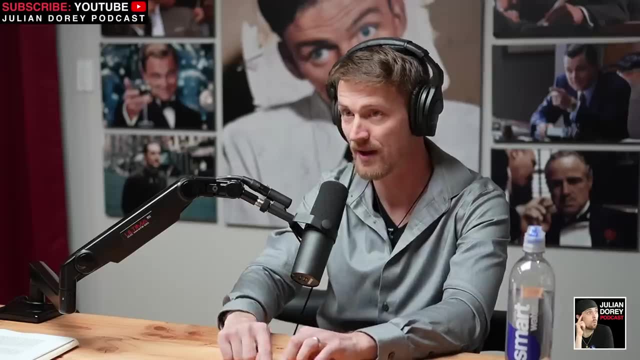 of writing into clay or stone was the only way that anything that can be written down could survive more than 1,000 years. You know we talked about this briefly before, but 500 to 1,000 years is the max that paper can survive. 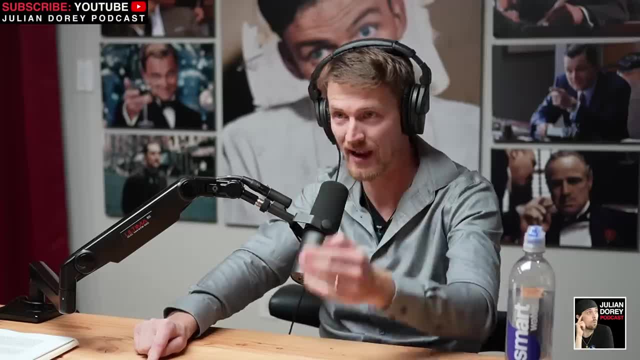 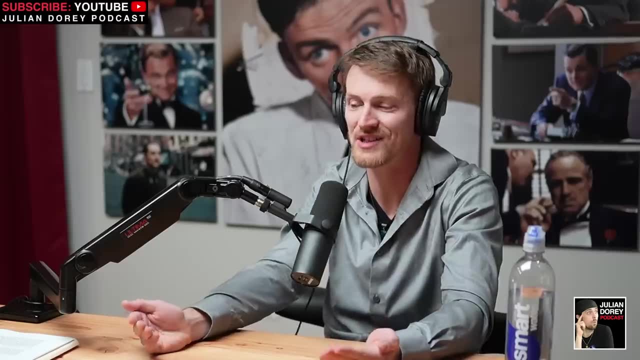 Like that Buddhist, the cave of 1,000 Buddhas, with that ancient set of manuscripts and maps that survived 800 years because it was basically sealed off in a dry environment. But 800 years isn't that long If you're having a written. 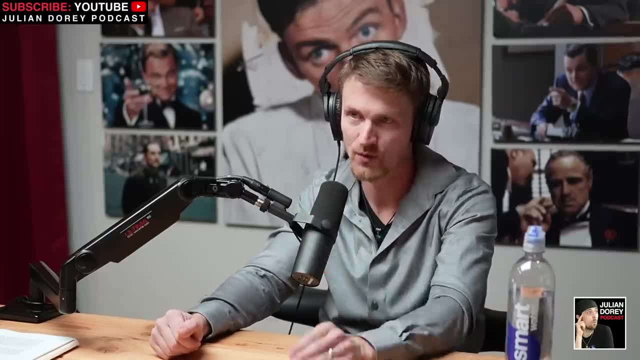 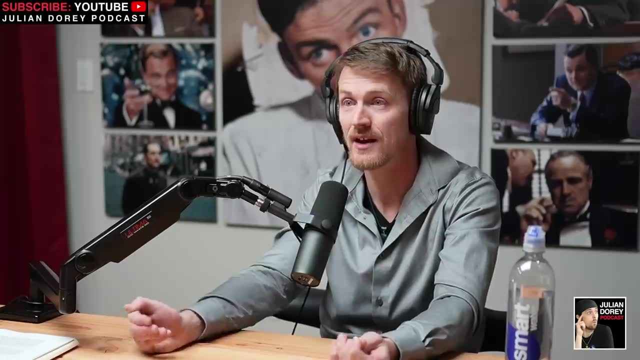 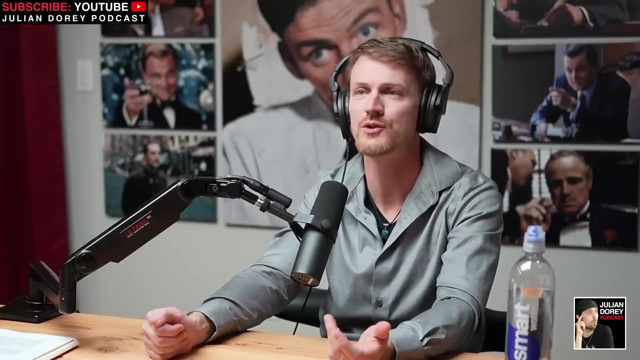 record to try to understand our past. the only way to do that would be cuneiform. It really is the only form of preserving a message that exists that we know of. I mean, if we can somehow infuse somehow information into quartz in the future, or something. 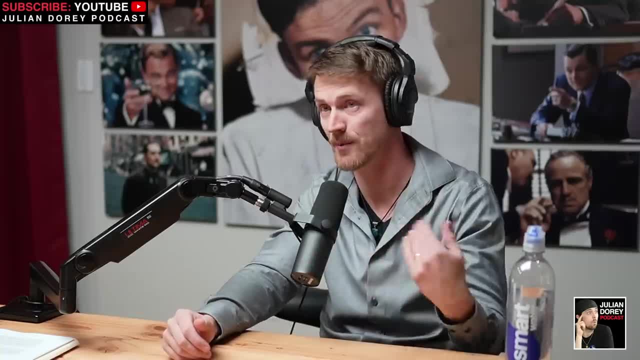 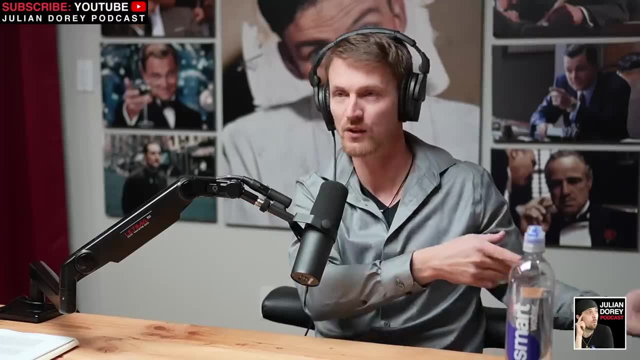 maybe something where it's infused within it, But right now, with our capabilities, the only way we would be able to preserve a message would be not anything we can do now. It would be more or less looking back at what they did and having to. 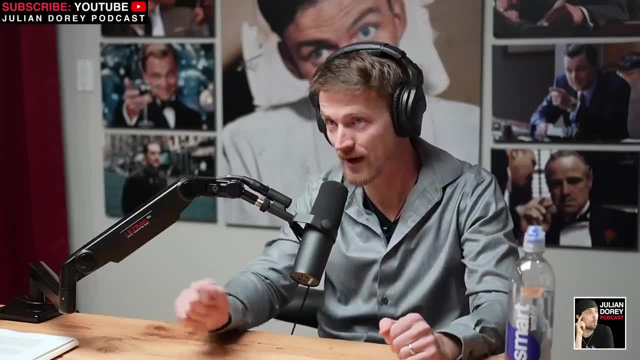 replicate it. So we think about all these things we've done. we probably need to start writing it all down in cuneiform so, if something happens to us, we don't just lose it all and have to start over again, which is exactly what. 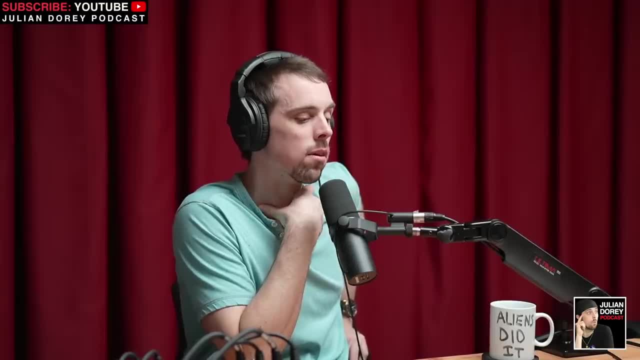 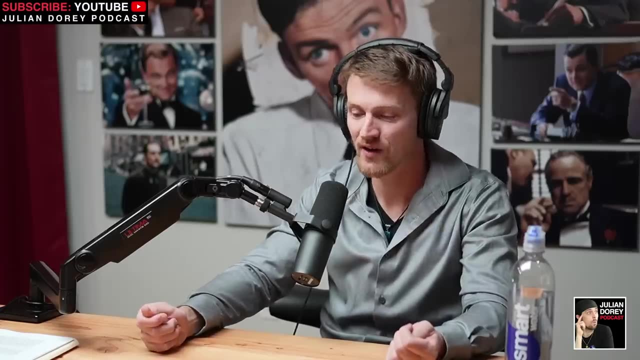 looks like happened. Now. what about Dumb question? probably, but let's go with it. What about digital records? I mean, digital records are only going to survive if you have the technological means, like a computer or something, to be able to read it Also, anything. 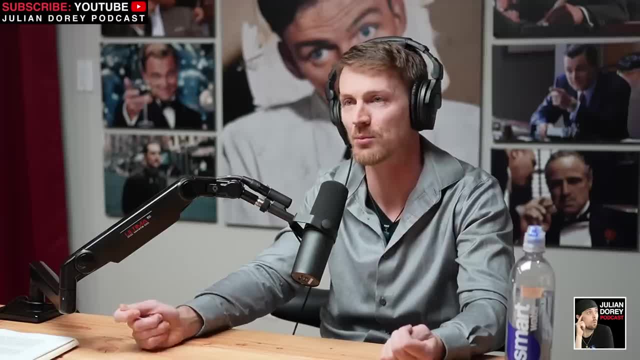 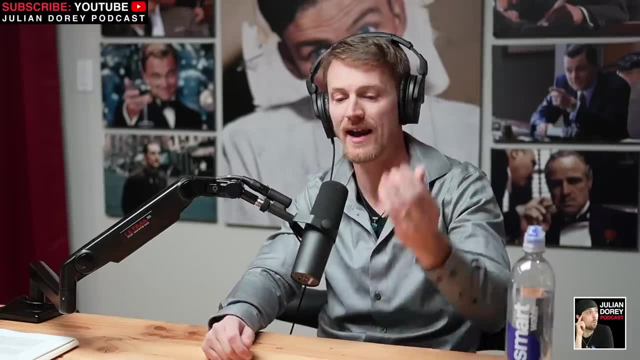 that's based on digital is going to have components like metal components or plastic components or something to make that object right To be able to read something. So you're going to say like I have these digital records that's kept on a USB drive. Well, you have to have. 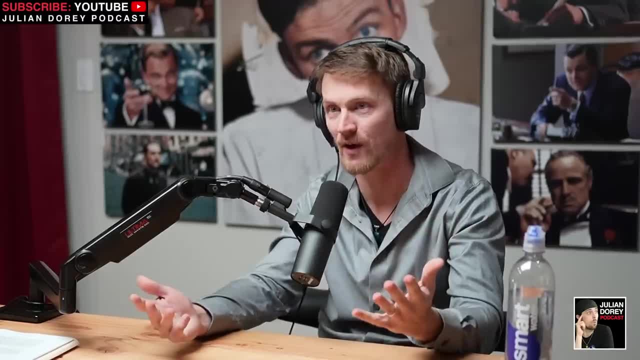 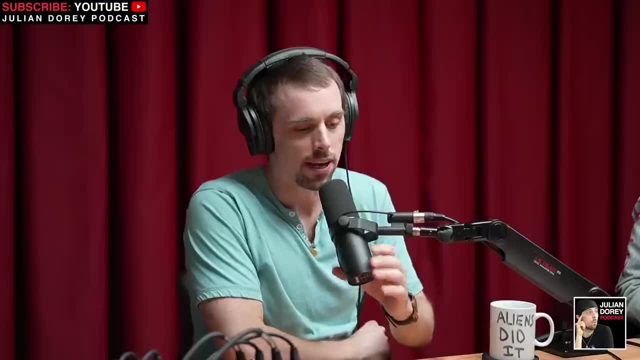 some way of putting that USB, USB drive into something to look at it right. Well, how is any of that going to survive? Any component that's metal actually is a very short. Is there a way to keep rovers- Rovers of some sort? 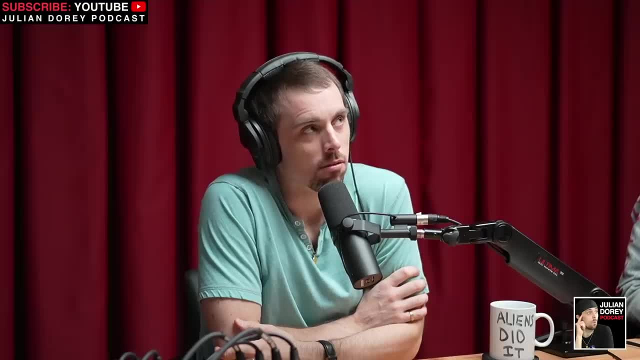 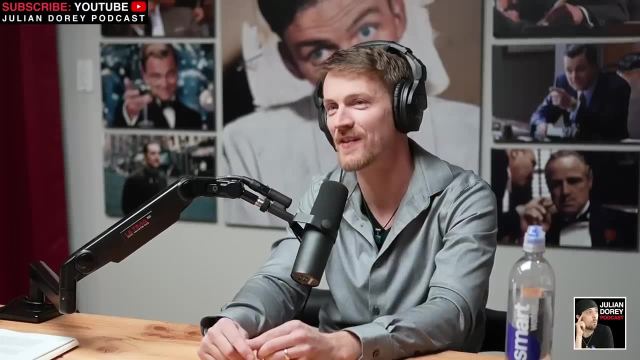 in the not-too-distant space that could be accessed later. I think about all the holes in these all the time, Like downloading data up there and then keeping it away from Earth. so if something happened it'd be Absolutely. I mean, that would be one way to do it. because if you're in space, you don't have the same types of degradation and things that attack metallic objects and others like on Earth. You don't have all of those problems, right? If you had an object just in a rotation around our planet, it could just sit there. for very long amounts of time, as long as it didn't get hit by incoming debris from an object or something. right, Maybe that's what all the aliens are. It's all just like Matthew McConaughey and Interstellar coming back, but they're green. 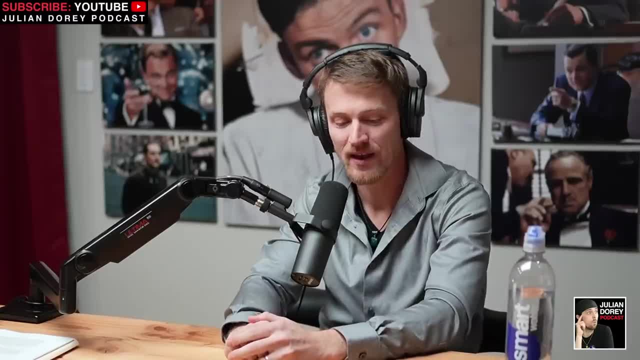 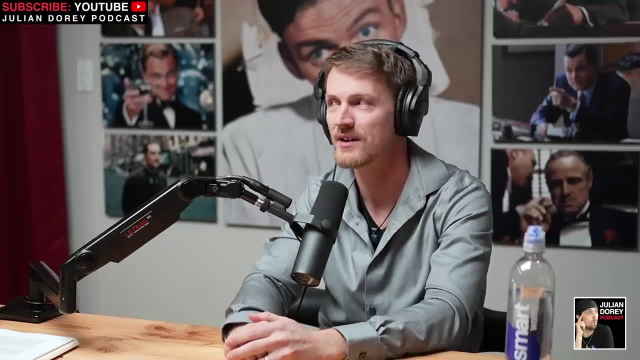 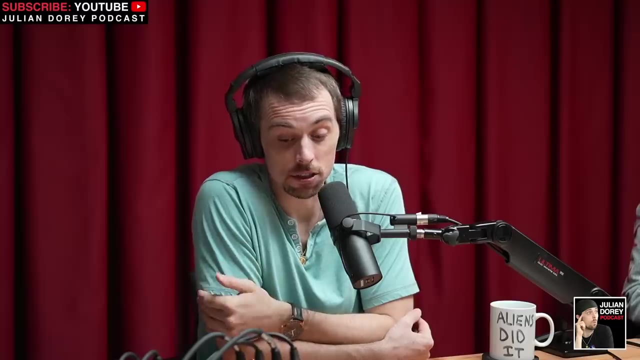 Well, it is interesting in that movie how Matthew McConaughey goes into that black hole, that type of aspect of our understanding of the universe where time becomes non-linear, And I think that's actually very much what it truly is. Well, that's actually been. 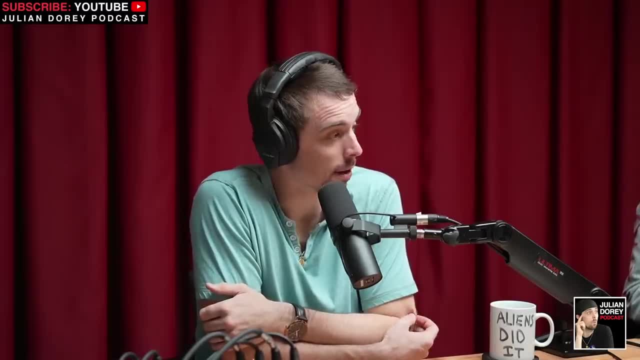 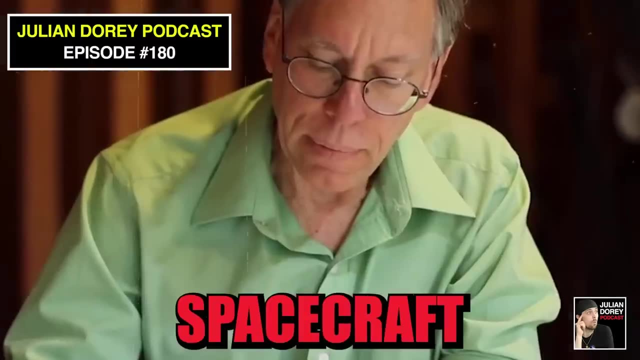 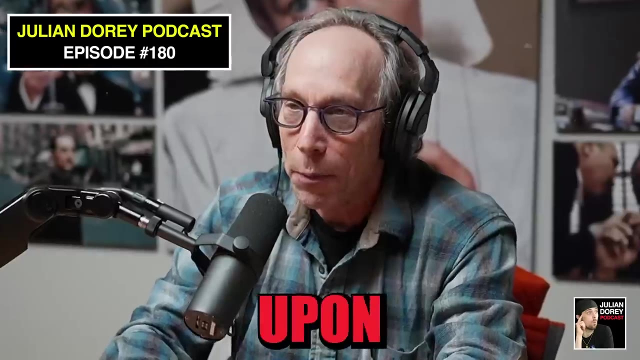 confirmed. There have been experiments on that. It blew my mind. I didn't realize that I hadn't looked into it, But even when we had Lawrence Krauss in here recently By accident, they stumble upon us. They built a spacecraft that spends. 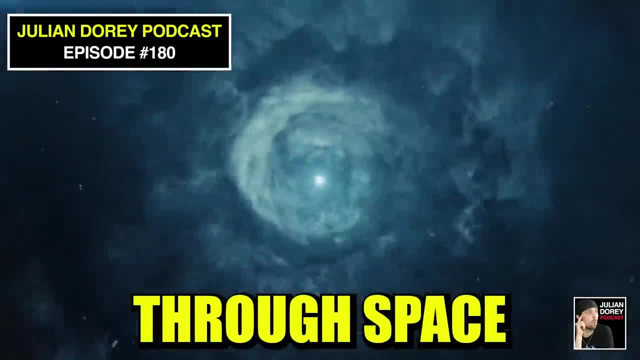 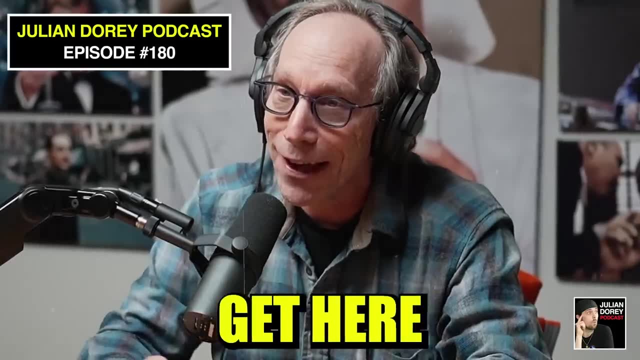 99.9999% of its time traveling through space. But they developed something like a flying saucer, which is meant to be aerodynamic in the atmosphere of the Earth, which they didn't even know was there until they get here. But why would they design? 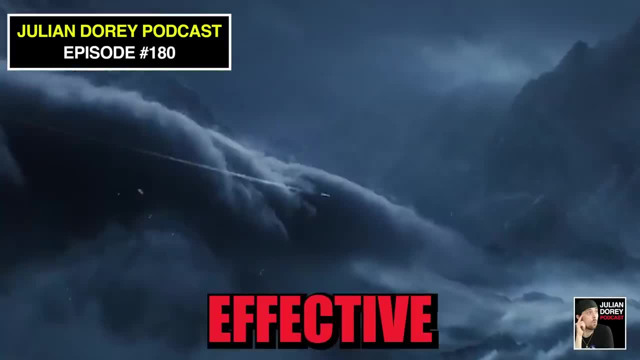 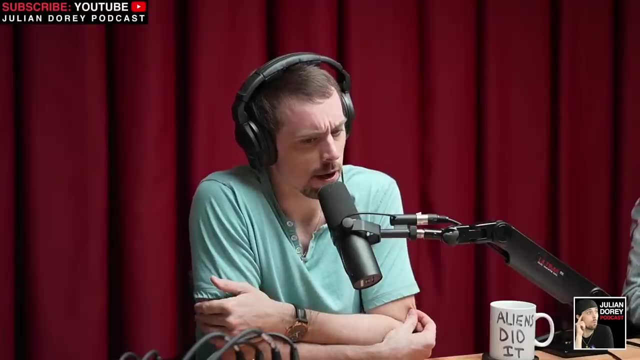 a spacecraft, a flying saucer if you wish, which is not the most effective way of traveling through interstellar space. The laws of physics tell us Here. here's the thing. He was even talking about it because he was ripping that movie. 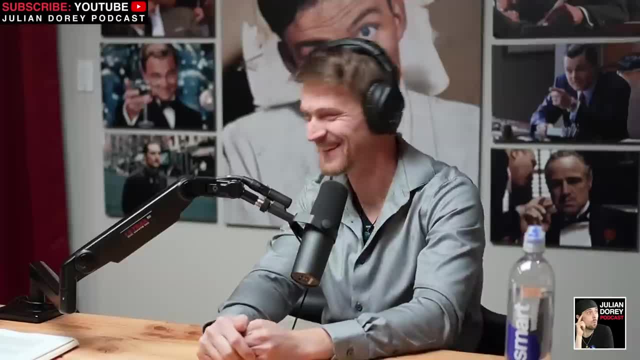 As a physicist, he's like I can't even I can't watch it Because all this shit. He was naming all the stuff, But he was like, well, they got that right, That was real. I was like, ah, look at that. 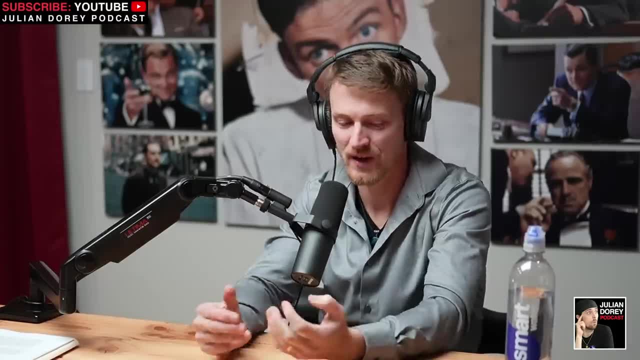 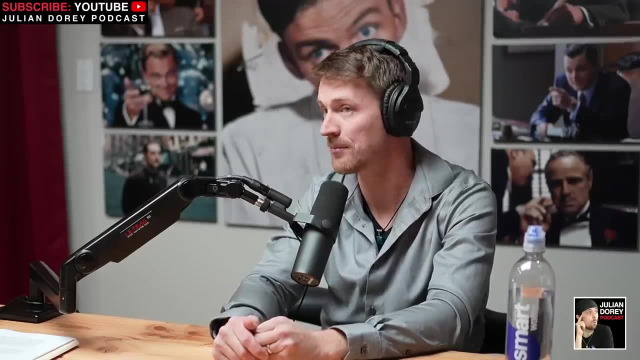 Something I think the consensus of what I'm trying to say is that we should put more emphasis on the ancient past And we need to look at them in a completely different light, And we should stop thinking of them as being primitive and cavemen in this way that 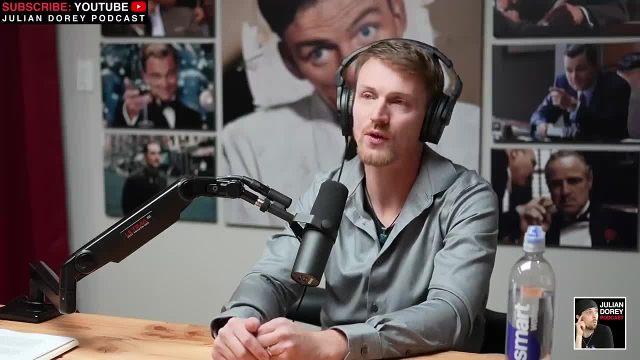 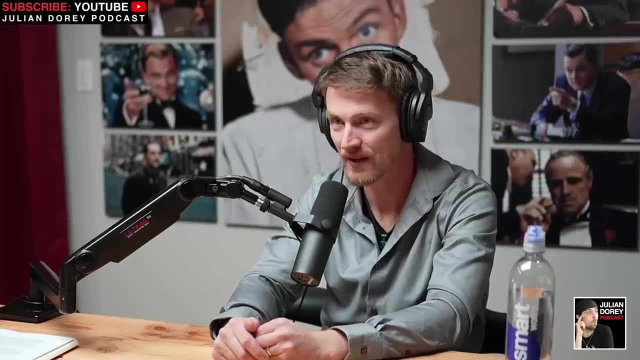 we've been portrayed through media and growing up And rather look at this time when there was exceedingly excellent science, Humans, we'll call them that were here, And I think they were very different than we are now. Very different, Yes. 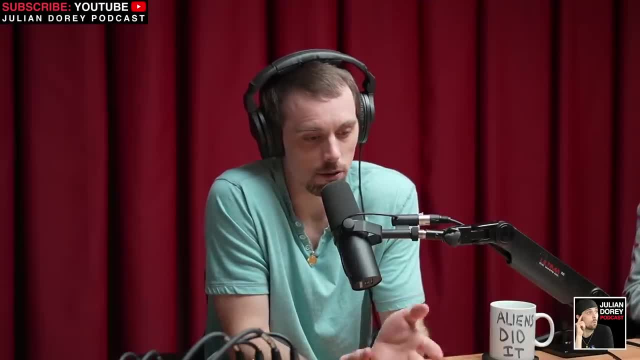 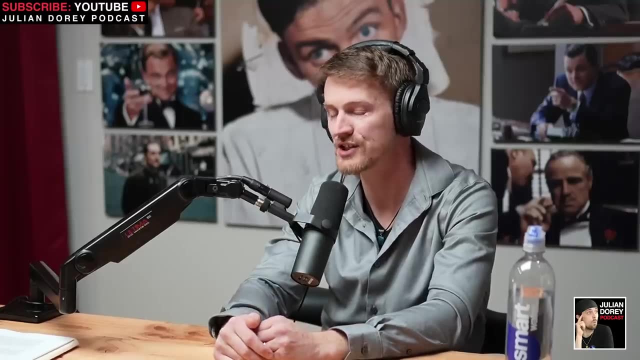 The excellence is measured to your point in all different types of ways. In what they left behind. They could be more advanced in some ways and less advanced in others. Right, And that's the thing that we really should remember. And having said that, 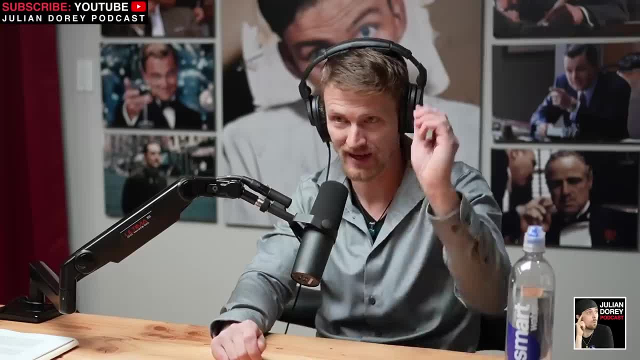 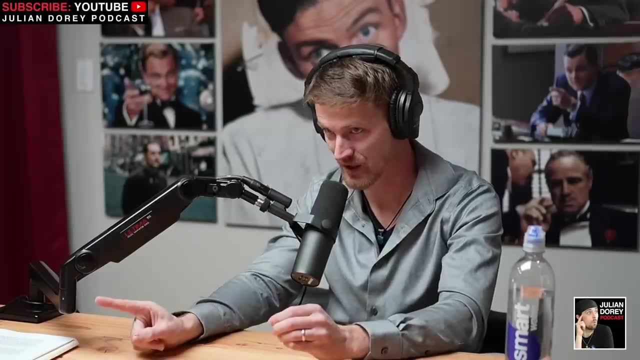 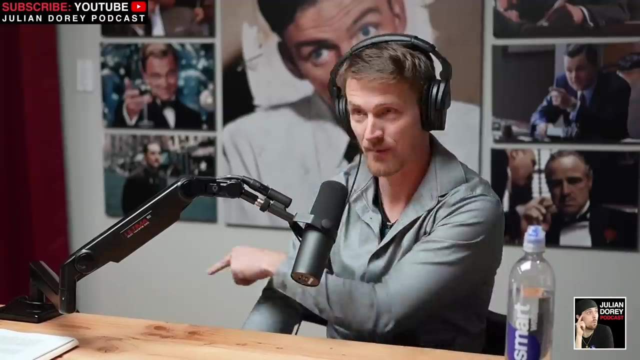 I think there's a lot more that we can learn about the ancient civilizations and what they know than what we can learn now with technology. Can you defend that Absolutely? Let's do it Okay. Imagine right now like someone like Elon Musk. Let's say Elon Musk is. 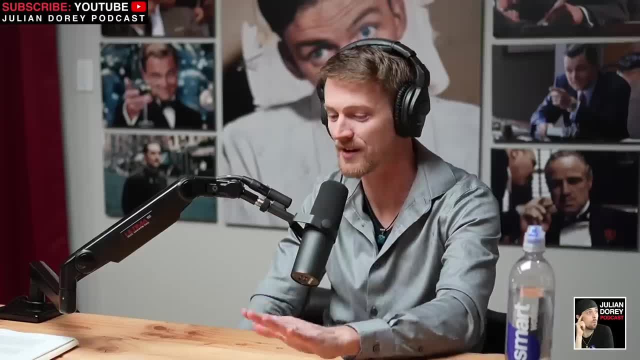 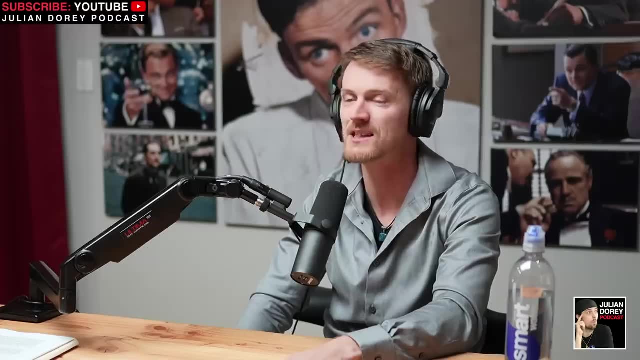 sitting right next to us and we're like having a conversation. Hey Elon, Hey Elon, How's it going? bud, Imagine Elon Musk is trying to understand space travel and aspects of the nature of reality, of the universe, things like that. He's focused. 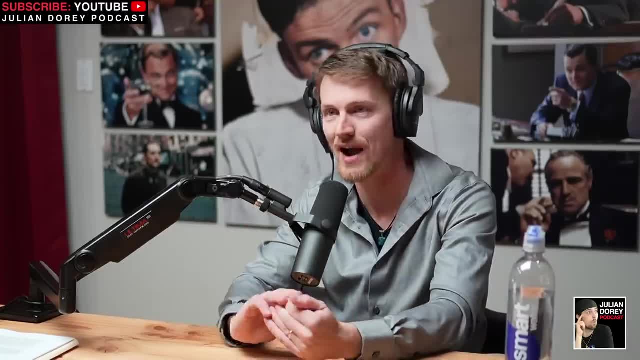 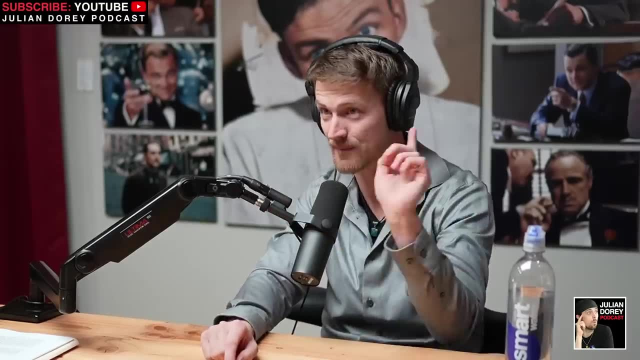 on this idea of creating a technological thing to travel from point A to point B. Yes, Or go colonize a planet or something, And I have a lot of respect for Elon Musk And you and I have talked about a little bit of that in the past. 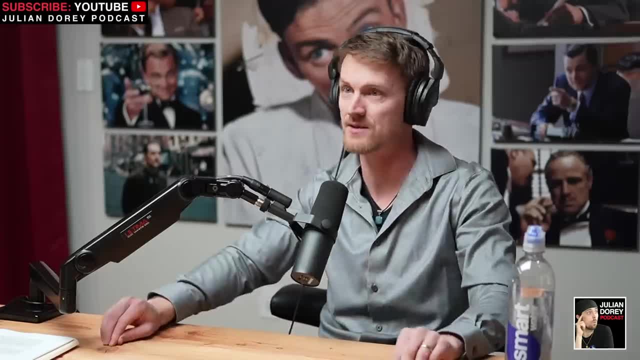 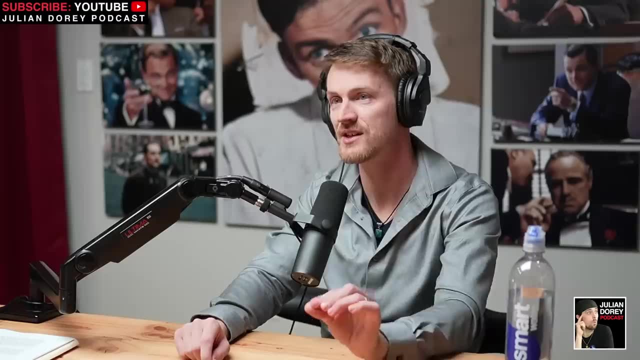 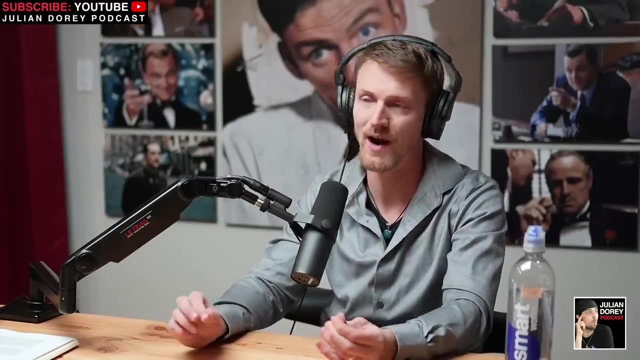 But what I think Elon Musk is missing, that's like a fundamental understanding of everything us the universe, everything is the role that consciousness and energy plays. Okay In the universe, Because if everything is based on this vibrational string theory, quantum mechanics, 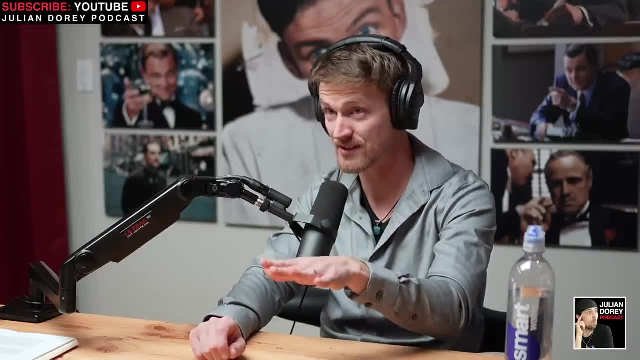 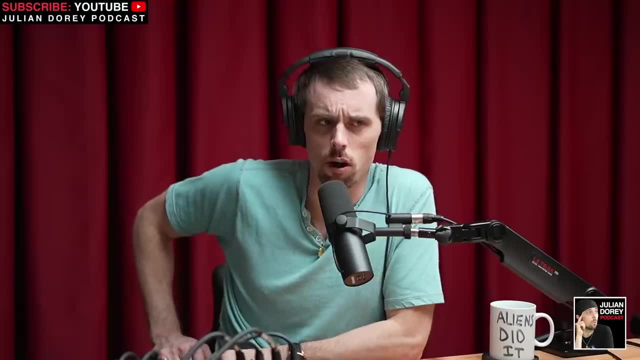 if it's based on energetic vibration, then it means that the physical world and everything we see is actually manifested as a secondary aspect of reality. Ooh, All right, Back up. Secondary aspect of reality. So if you were to think about what the core of reality? 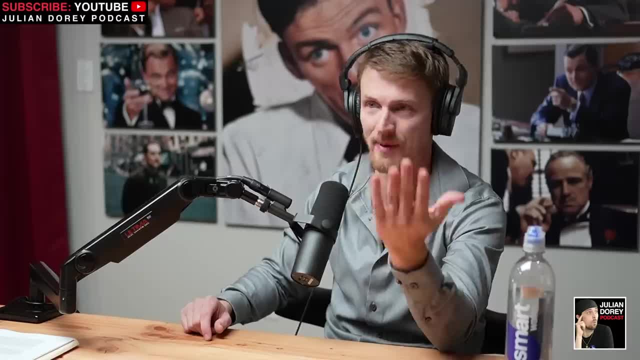 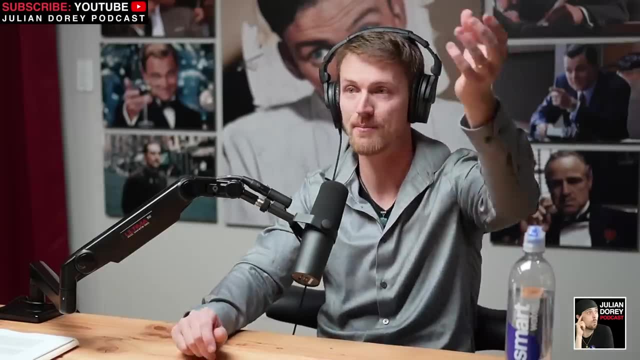 is like, for instance, we can only see the visible light spectrum, like five colors right Or seven colors in the visible light spectrum And that's the same as we see in a rainbow. It makes up a rainbow, The colors you see in a rainbow. 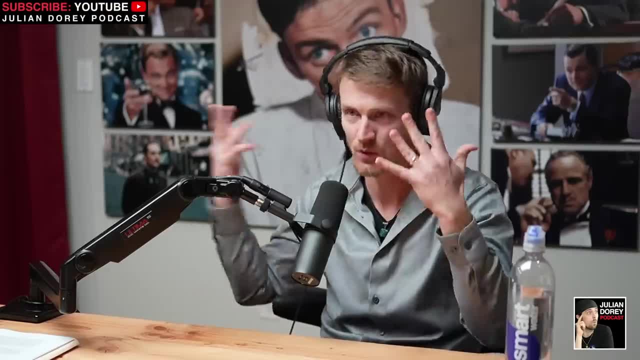 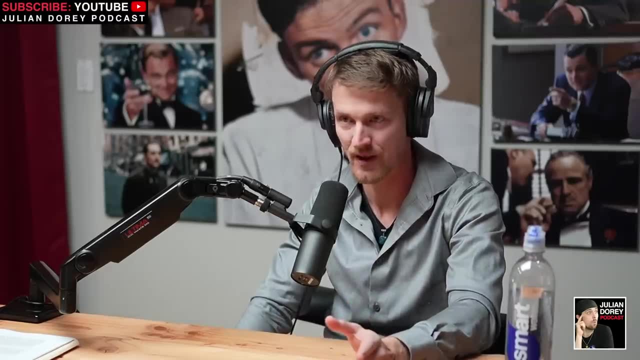 is literally the visible light spectrum being manifested, so we can see it in front of our eyes, Yes. However, reality itself is a lot more complex than just the seven colors of visible light spectrum. There's a lot of other aspects that are going on. 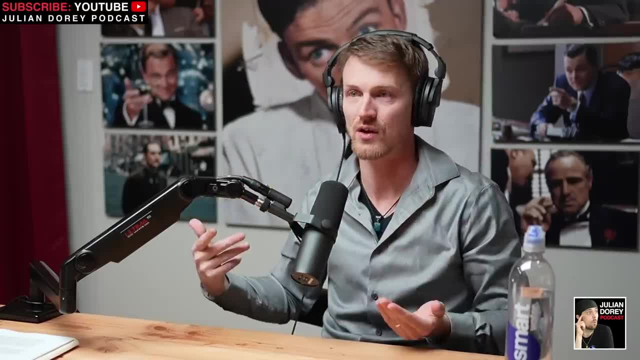 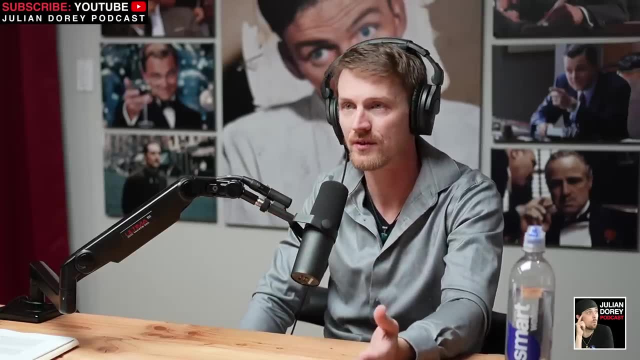 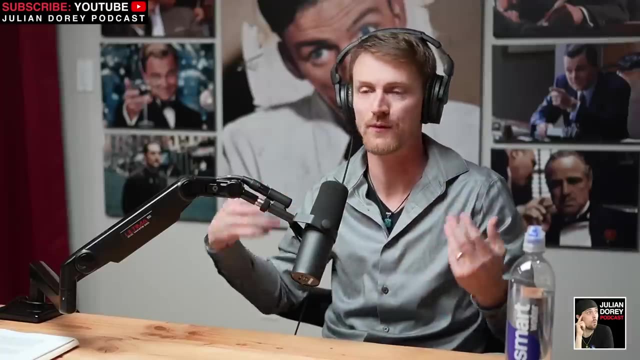 in reality that is not physical. And for instance, how would someone like Elon Musk measure something like love? There's no scientific way to measure something like that. You can't. And how would you measure the ability for someone to go into meditation? I gotta give a huge. 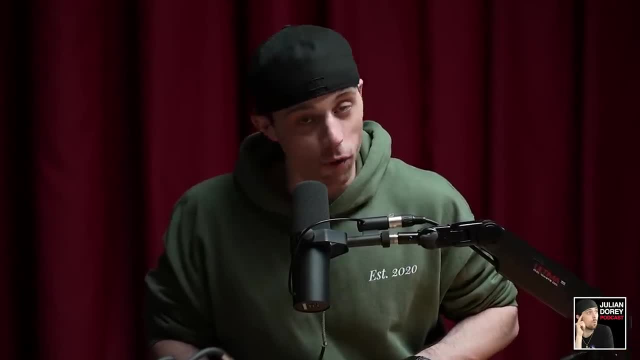 shout-out to my man, Bedros Koulian, for adding a great part to my daily routine every day. And if you don't know what I'm talking about, first of all, Bedros is a guy who has a huge YouTube channel. 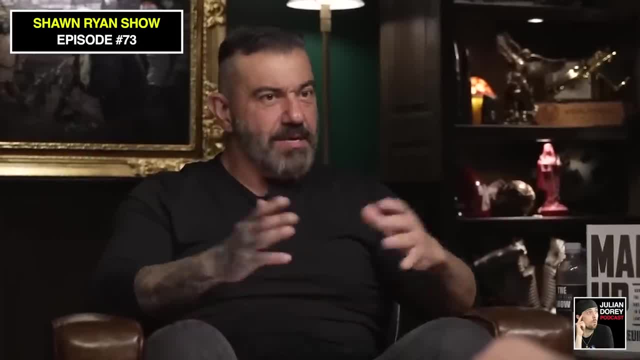 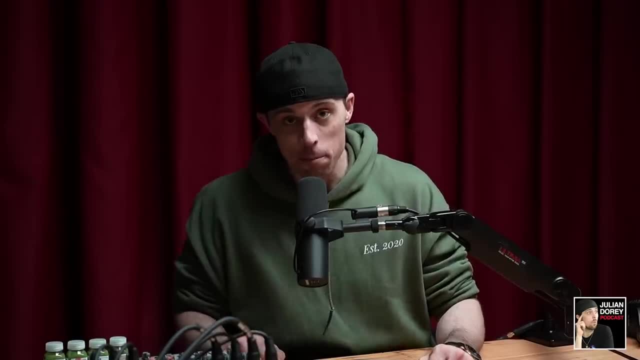 He's got an amazing story. came from a communist country, came to America, built a big business, was very successful, lived the American dream and now inspires many other people to do the same. But one of his latest ventures is called Trulene. 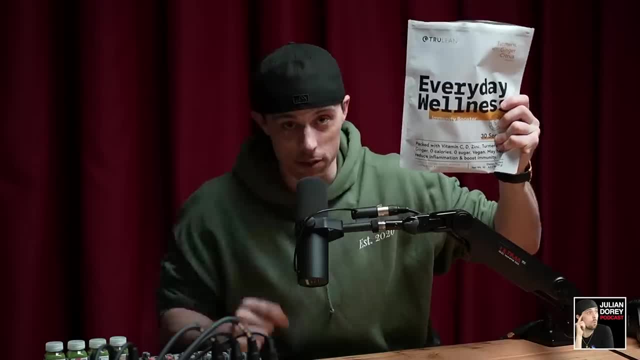 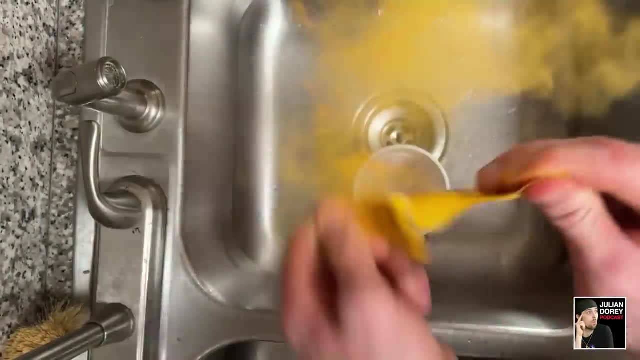 And Bedros turned me on to his product right here called Everyday Wellness. And let me tell you something: this thing is a hack. Essentially, it is a packet just like this. You stick it in a little glass of water, you put it in. 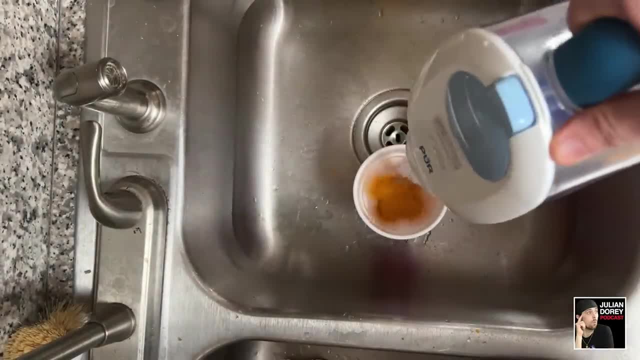 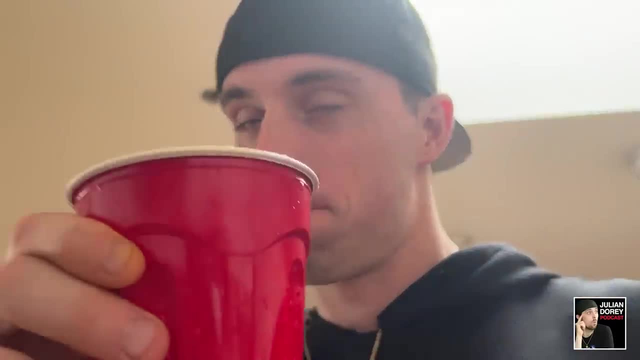 the water, you mix it up, it tastes like orange soda and it's got all the necessary ingredients to not only help your immune system, not only help your digestion, but make you feel better And actually give you a boost to your day, I mean. 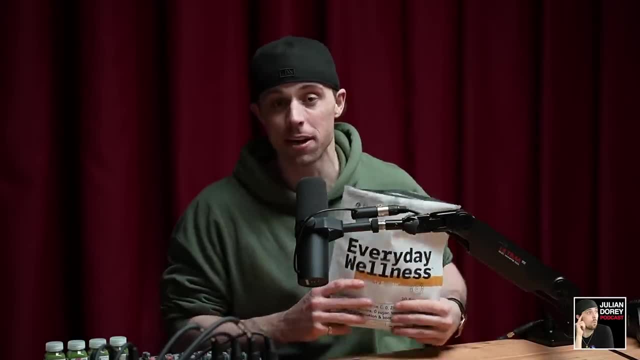 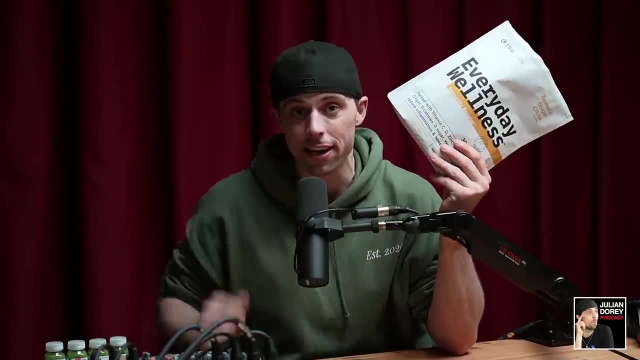 I like taking it at about 3 o'clock in the afternoon, so it's like a nice pick-me-up. But that's because this thing has vitamin C, vitamin D, zinc, turmeric, all these amazing ingredients that you're probably trying to get in supplements, all. 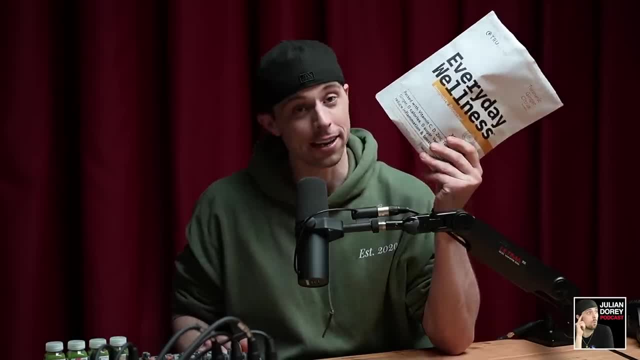 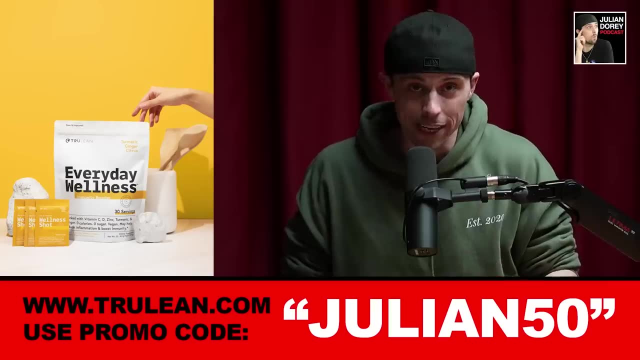 in one shot. I love it. You're going to love it too, And if you don't believe me, go check it out, because these guys have a 30-day money-back guarantee. All you got to do is go to Trulenecom and. 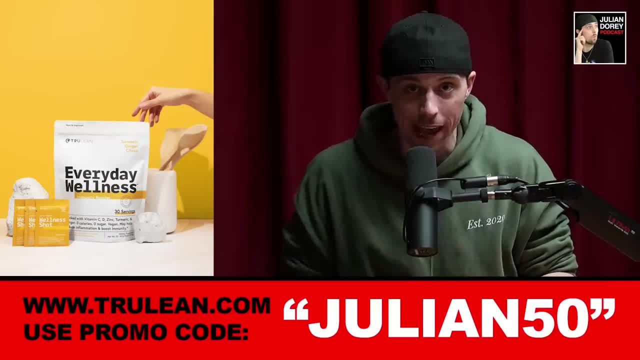 use the code JULIAN50 at checkout. That's all caps: J-U-L-I-A-N. 50 at checkout for 50% off your first order within a subscription and 20% thereafter. You are not going to regret checking out this product. I'm really excited about this one. 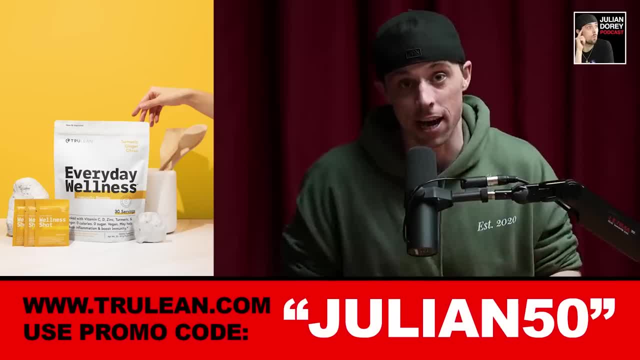 because this is something I now use every day and I'd love to make these guys a part of the show moving forward, because you guys are getting a lot out of it as well. So go to Trulenecom and use the code JULIAN50 at checkout. 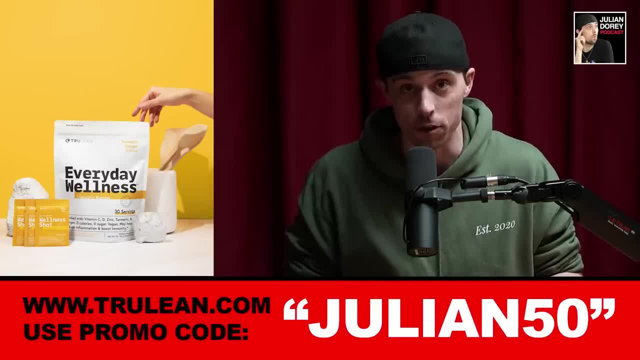 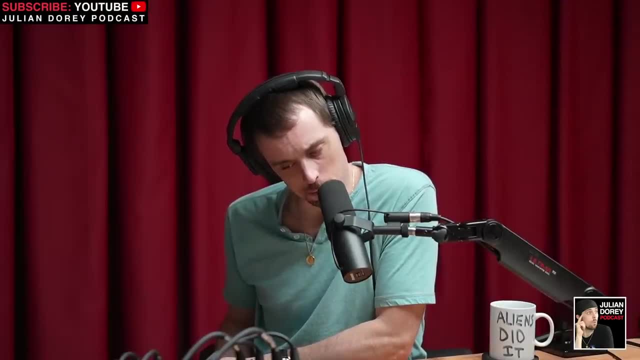 for 50% off your first order on your Trulene subscription right now. Well, can you measure? can you measure? I'm going to make up this is not the official term, but can you measure emotional impulses? It may not be able to say, like that is love. 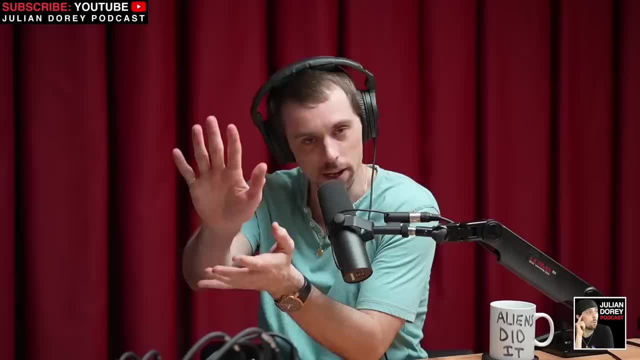 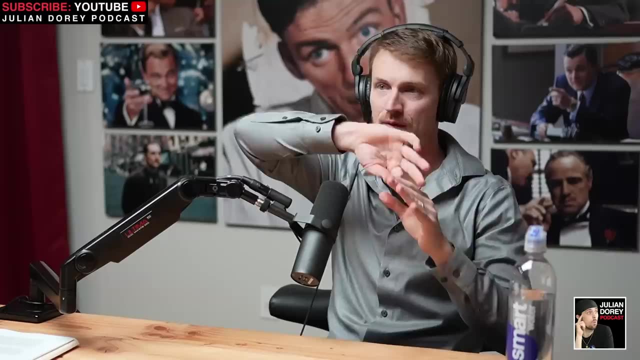 But, like you know, have you ever seen those images where they show like the x-rays of two people who are about to make out and it shows the body change? They can show their color aura. They have the ability to show aura of, like an energetic 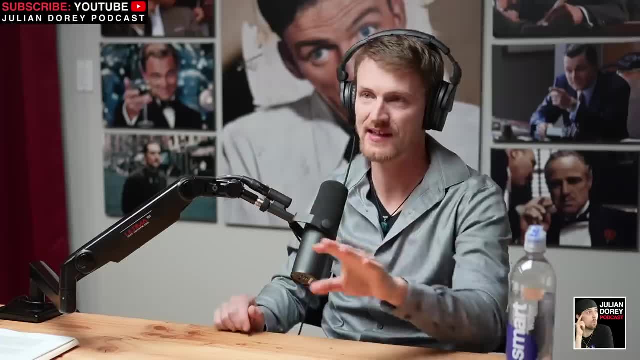 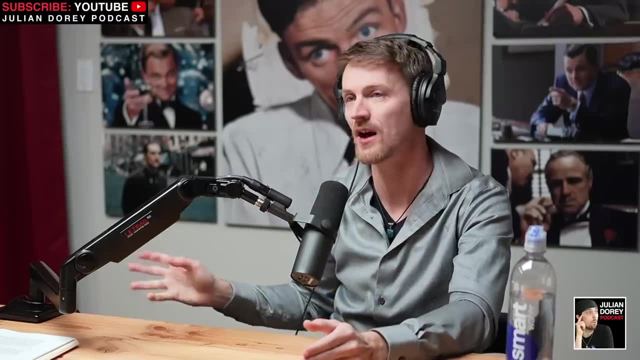 signature of something and they can actually see when it changes And there is that ability to show that. But the problem is the there's no way to measure consciousness in a way scientifically, like Elon Musk wants to. You can't take someone and hook them up to a machine. 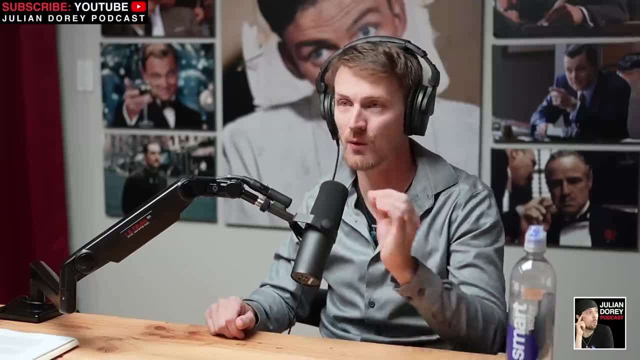 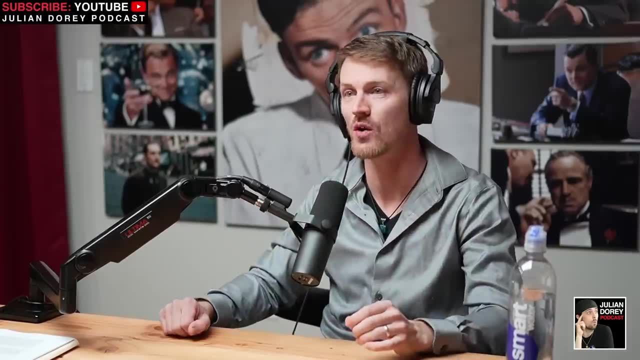 and measure their consciousness, because, fundamentally, we're still taught in school that the brain creates consciousness. That's what we're still taught as a doctrine in school. And if you, Matt LaCroix, were teaching in school, what would you teach people? 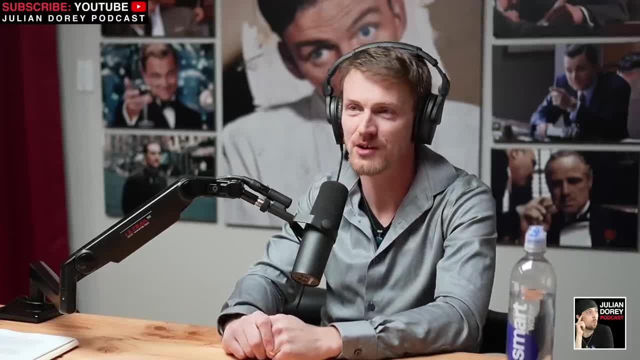 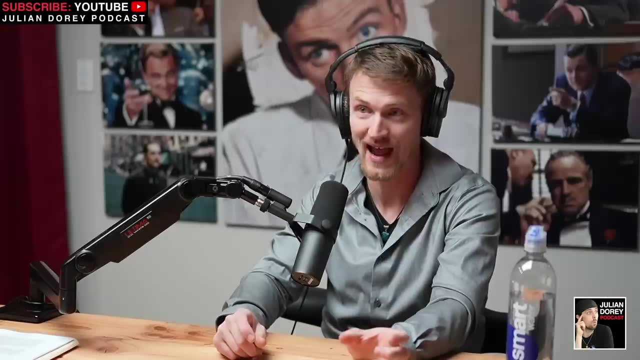 Well, I would teach people that we are eternal energy beings that live forever and we are incarnating in different lifetimes that have a certain time stamp based on our mortality that allows us to only experience this reality for a certain amount of time and then bring back that growth. 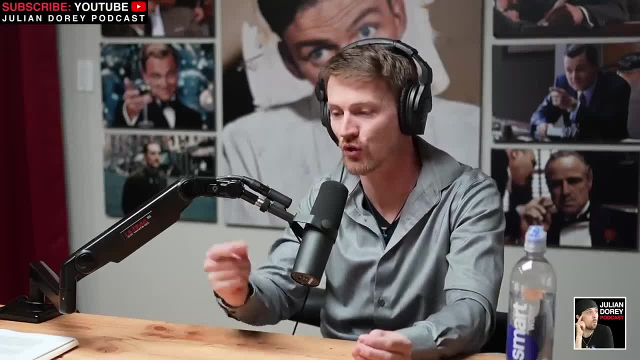 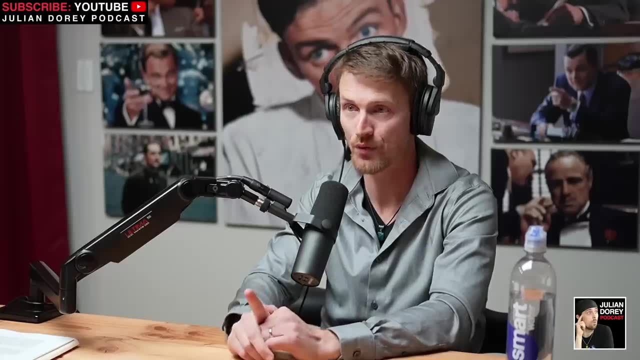 that we learn in different lessons, into different lifetimes, to grow slowly. Are you talking about that on a karmic point, Absolutely, Or on a multiversal point? Both? Both Made up those words, but let's go with it: Karma. 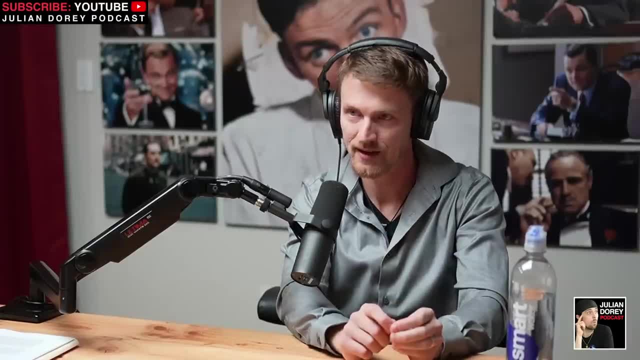 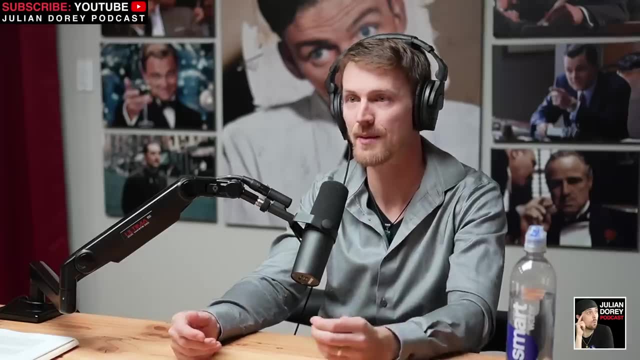 is about the things you've done or not done in a previous lifetime, Right? So if you kill someone in a lifetime, you have to make up for that karma in another lifetime, right? Well, the same thing's true if you do something. 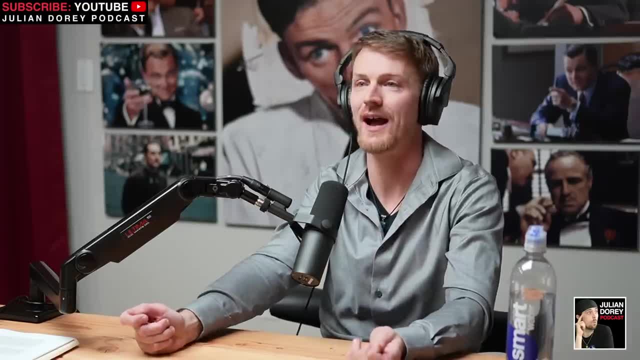 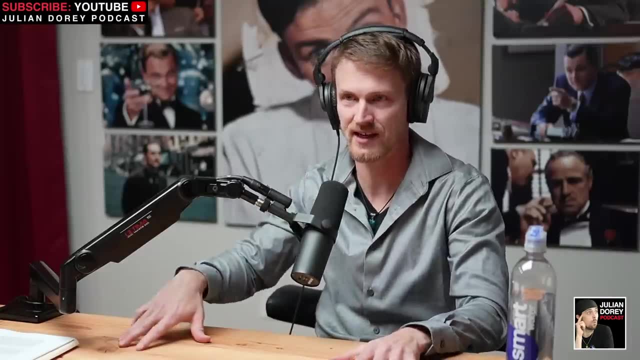 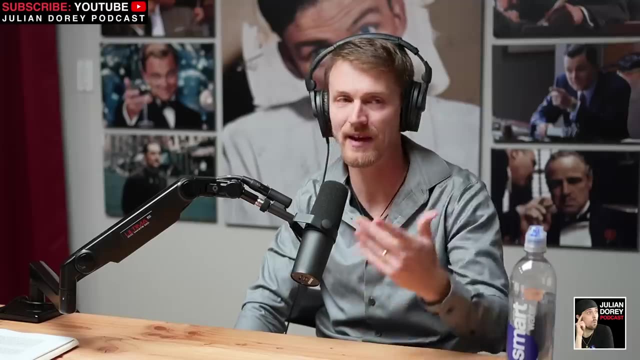 really good If you change the lives of thousands of people right for a positive reason- And I think that's how karma tends to work- is this energetic signature of what we left behind that then allows us to grow from that standpoint, From like, for instance. 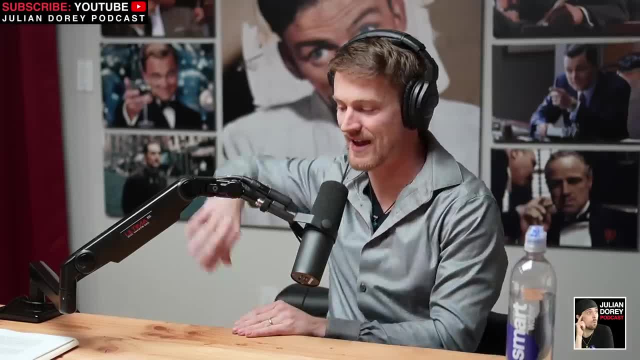 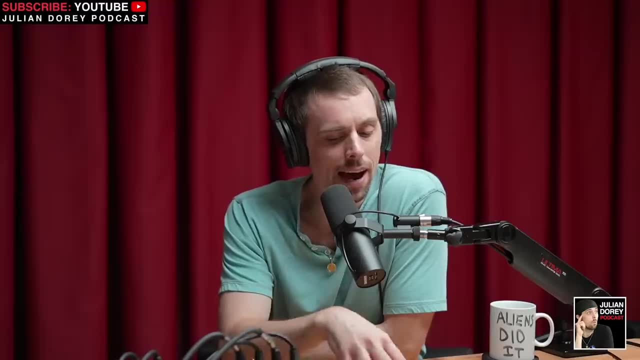 if you lived an angelic life, I think that that next lifetime will be will change based on what you experienced in a previous lifetime. So, Matt, I think I agree with you. I've talked about this topic on different podcasts, not even with people who 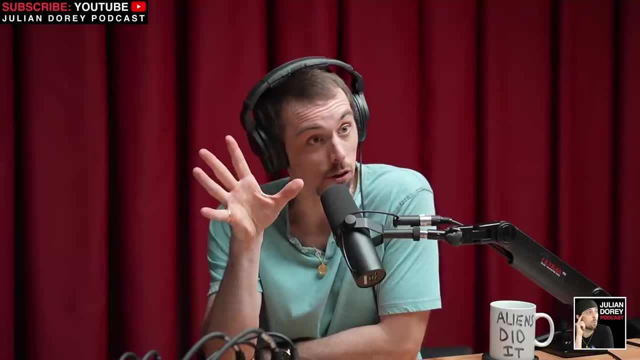 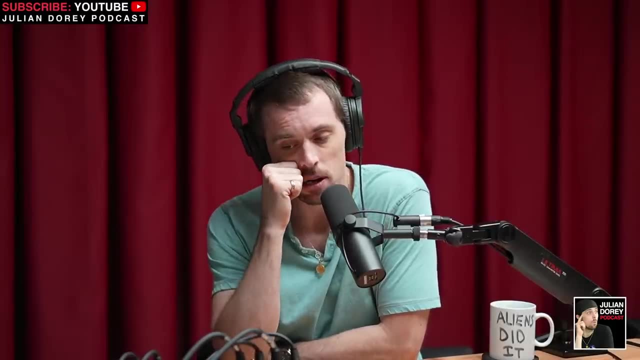 think about it just when we're having conversations about it. I am a believer in karma And it's a part of what you know you want to put in good so that you also get out good as well. But what is the? 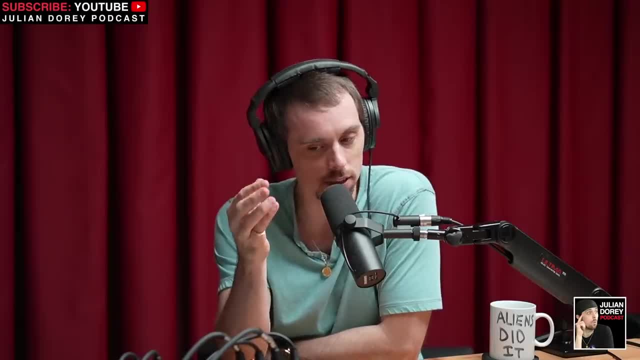 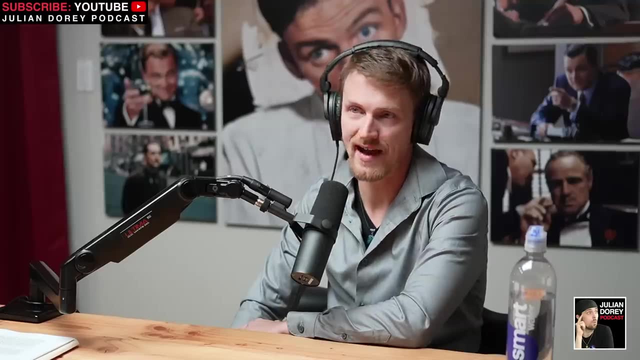 base? are we strictly just talking total, theoretical, technically right now? Like, what's the basis for you thinking that I've never defended it myself either, to be clear, Okay, well, what I'm trying to connect and trying to say is that the ancients seem to know: 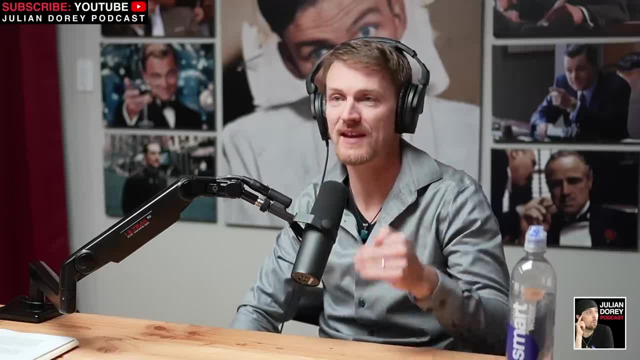 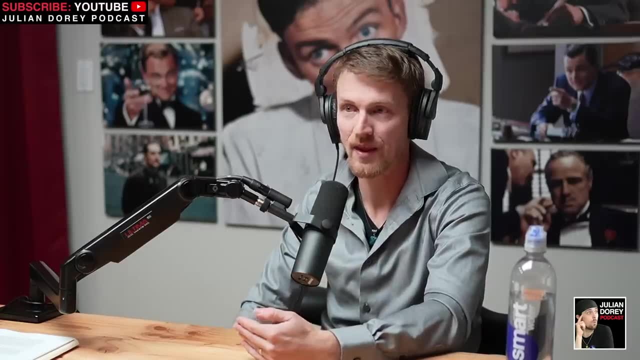 this is what we're. we started off and then got off where we did. Yeah, yeah, yeah. But the ancients seem to understand aspects of our reality that we don't fully acknowledge today. Give you an example: The Hermetic laws. 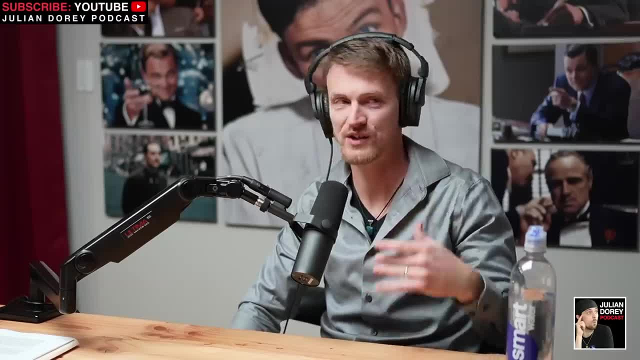 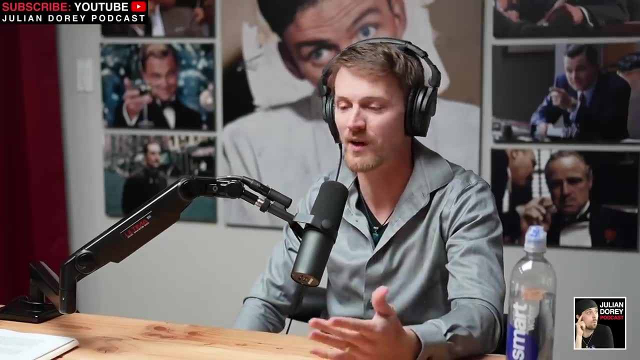 okay, Hermes was Hermes Thrice Great. was this great sage from Greece? okay, He's a Greek sage, And he left behind a number of different books. One of them's called The Emerald Tablet, and there's a number of other ones. 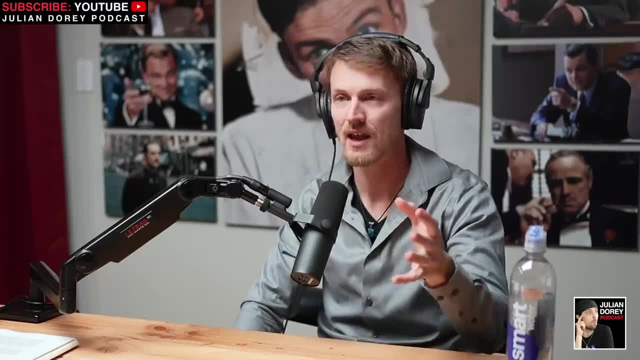 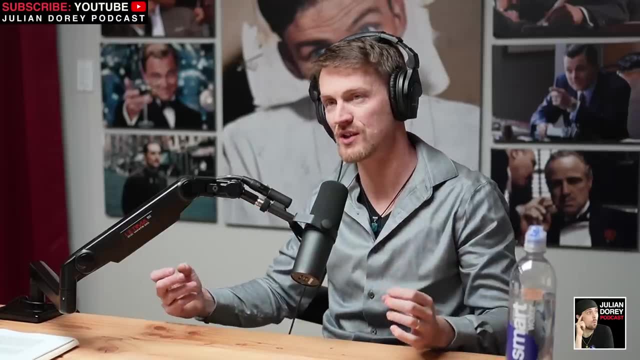 They're called Hermetic Teachings And in those Hermetic Teachings they have the same core as a lot of other teachings with a lot of other ancient civilizations around the world, And what I mean by that is one of the like the Hermetic they call. 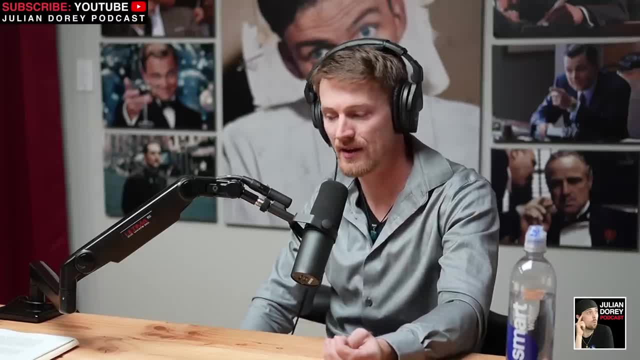 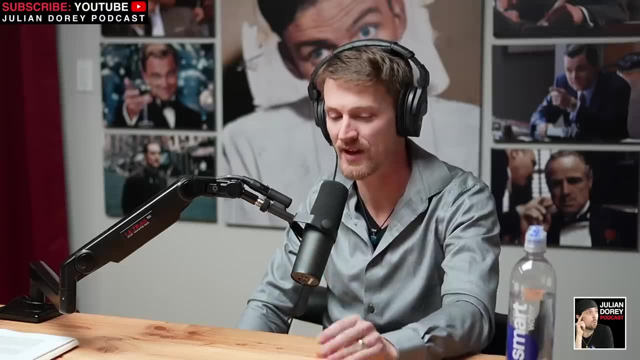 them Hermetic Constants, Because Hermes it's not like a normal person. He seems to be connected to something higher. that was like handing down knowledge, But that's another story. But the point is that they describe that there are cosmic laws that exist, Cosmic. 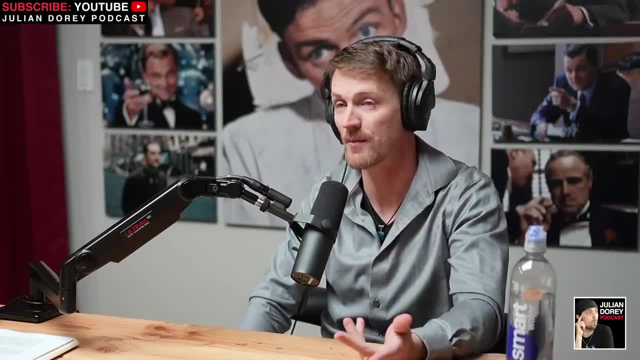 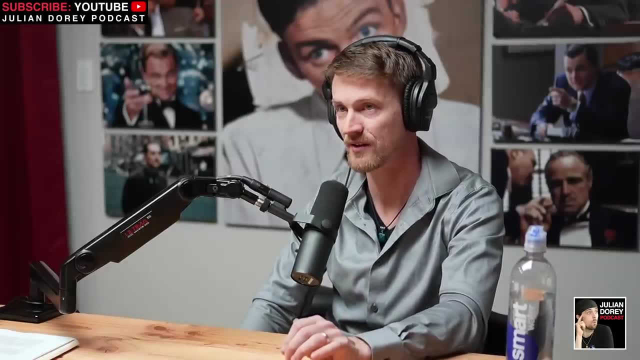 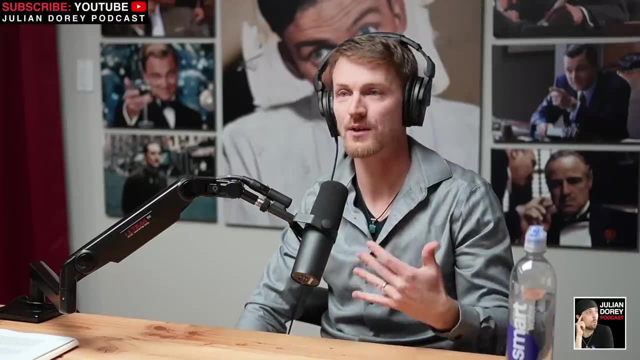 laws which would then emphasize or point towards some kind of intelligent creator. obviously These cosmic laws seem to be fundamental laws in the universe that cannot be broken, Cannot be broken, And again you're saying: Keep going. Yeah, So one of them is as above: 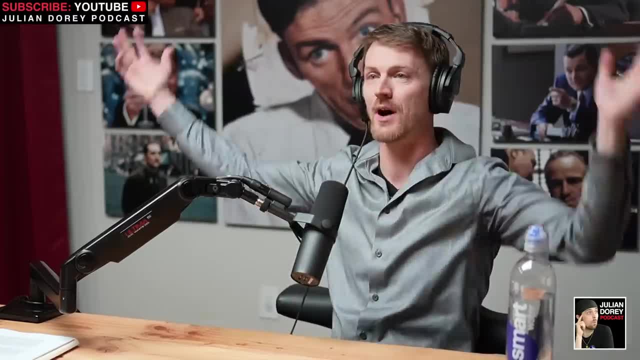 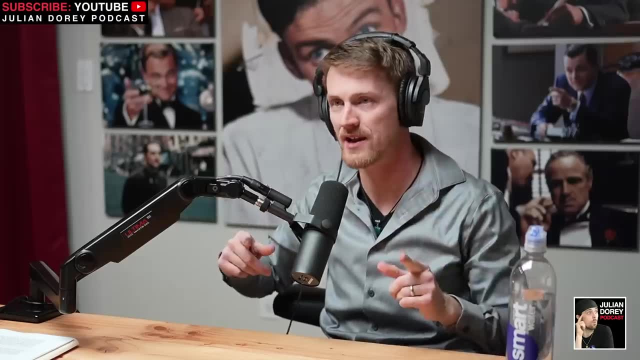 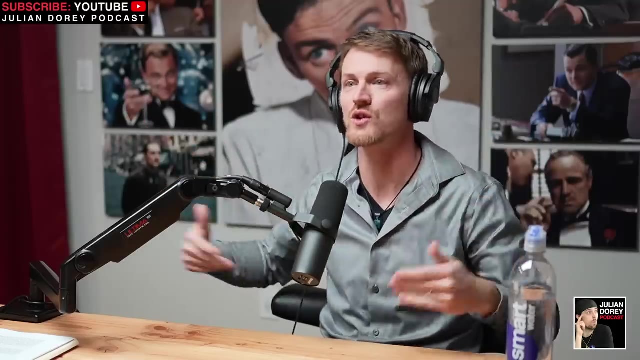 so below Yes, Meaning that everything we see above us, in the night sky, in the universe, is actually represented within our own reality here. So the strive that we have within us developing and reaching higher states of consciousness is like the universe almost becoming self-aware. 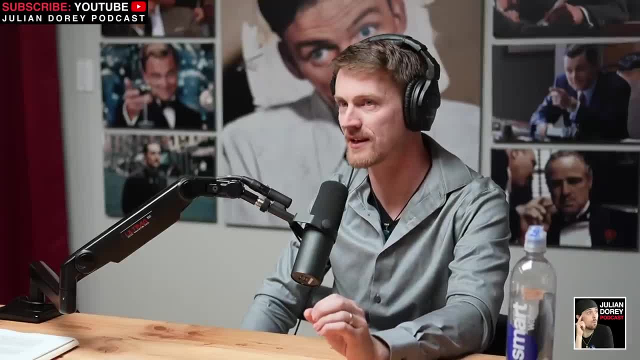 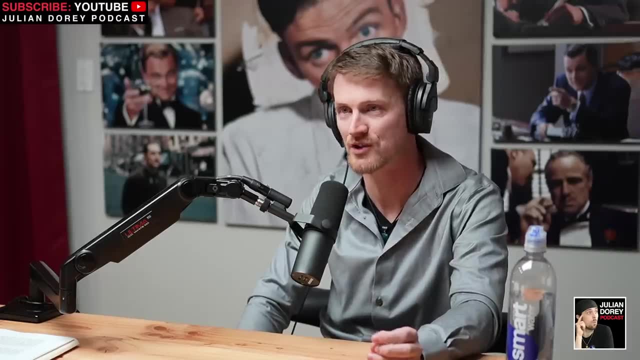 We seem to be much more deeply connected to the outcome than we've been made to believe And, rather than just being this random evolutionary ape that got smart from eating a bunch of mushrooms, is it really seems like we're more something far more powerful and 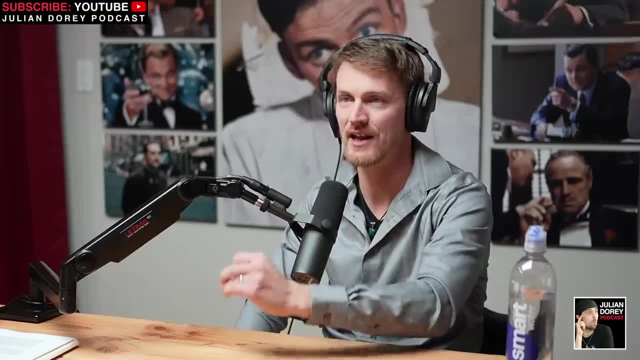 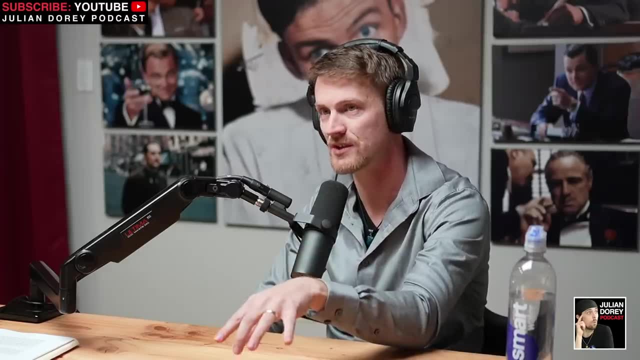 important. But because of that there's been a lot of interest to hide that nature And to prevent us from understanding that, And that's what these civilizations seem to encompass into the core of their teachings And then passed around the world. But when they 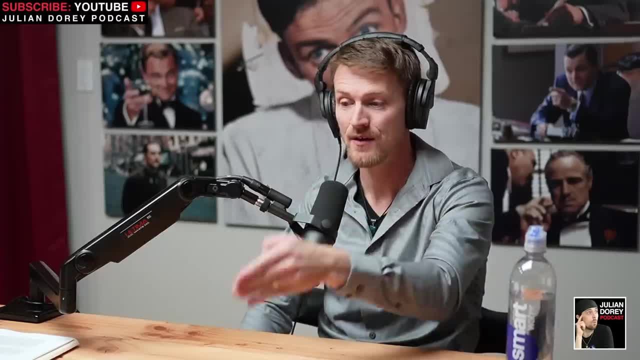 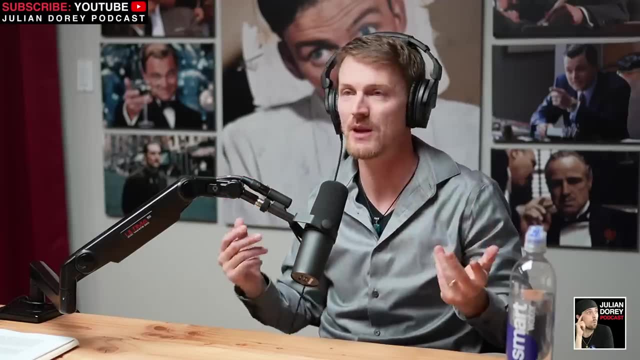 were destroyed from catastrophes, the knowledge of what they knew was greatly lost over time. To where we look back- and there's a few people that seem to understand it a little bit, But the general consensus is they have no idea any of this. 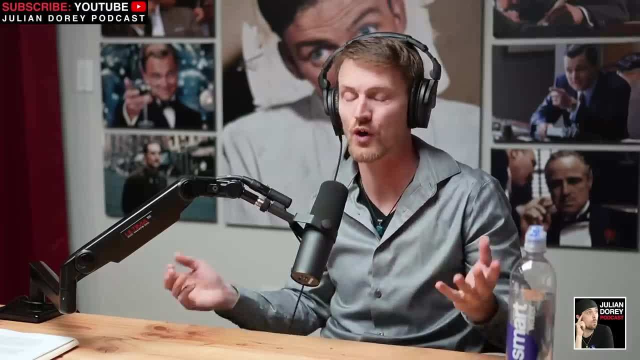 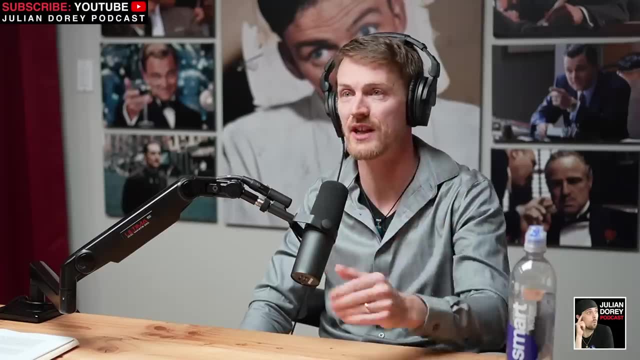 really exists Or what it means. So even though the hermetic laws may be well known within some sects of people that study them, who are like mystics and are interested in that, the majority of the population has no idea they exist. Why is that? 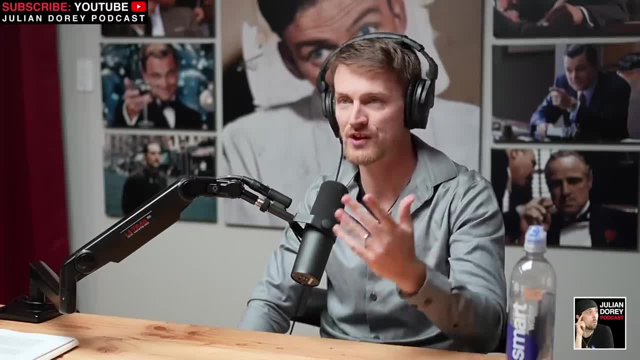 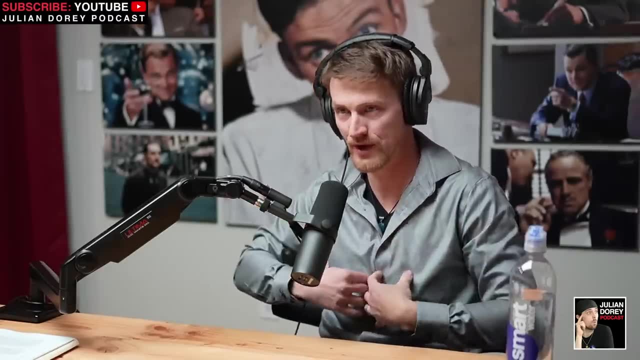 important. Well, the hermetic laws are more than just. as above, so below. It states that as within, so without, And it tries to explain to us that we truly are the microcosm of the macrocosm of the entire universe. 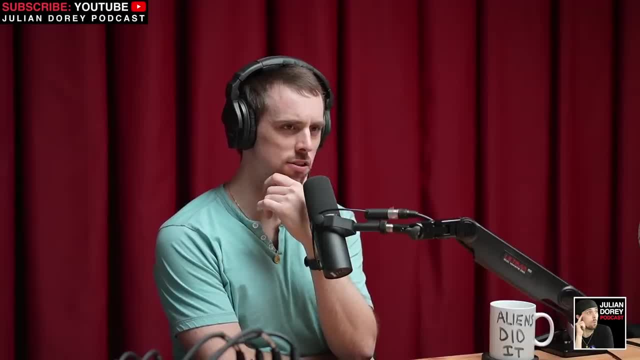 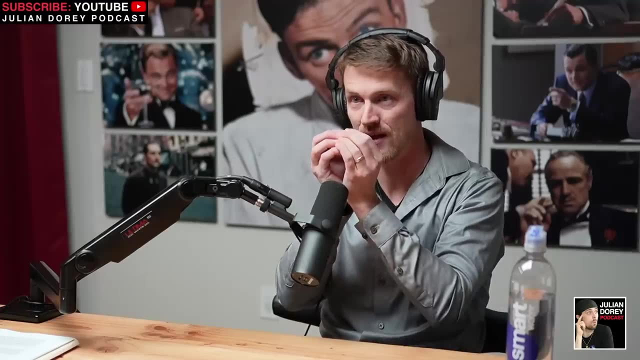 When you look at something like The microcosm of the macrocosm of the entire universe. So it means that we're a small little piece. Micro means tiny. We're the small little representation of the little of the entire universe. When you look at 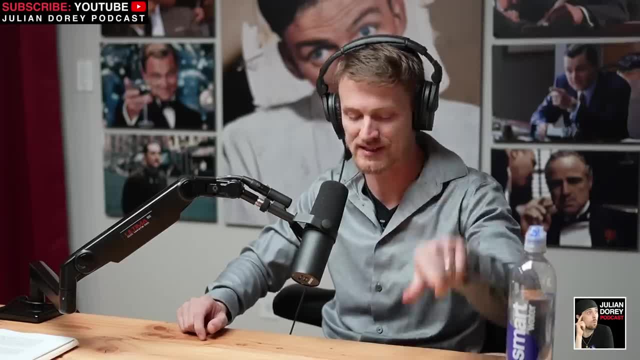 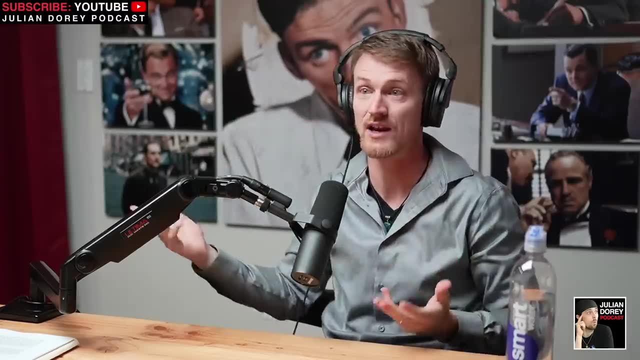 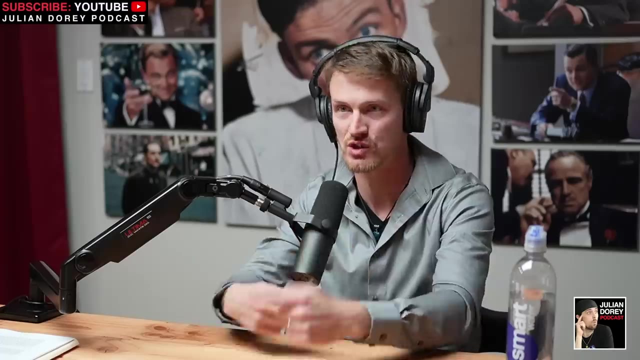 You get into the comparisons of the golden ratio. You look into the designs of the human eye, a cell in the human body, how it explodes and then transforms into creating life. You see the same exact type of explosion design framework in the universe when a 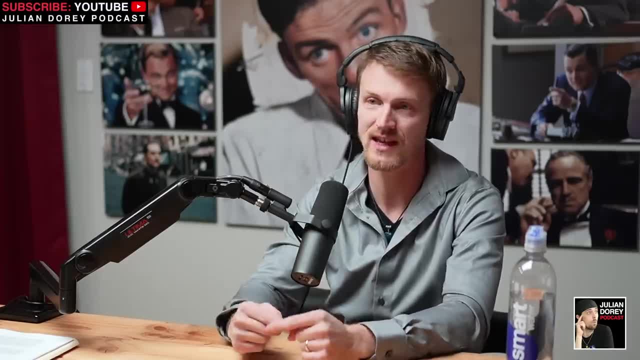 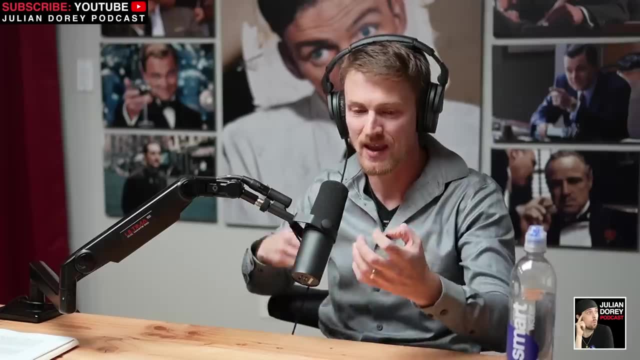 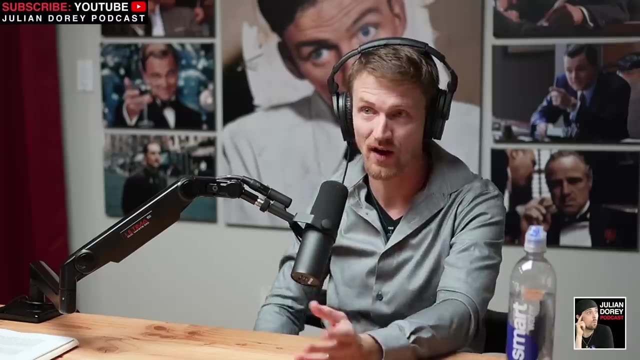 star is born or something is created, It follows the same type of design that's within us, like a cell giving birth and then splitting apart. It seems to be the same, The same type of reflection, as out there, as here, And the hermetic. 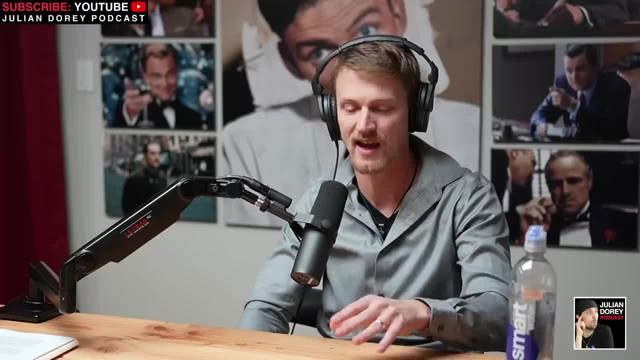 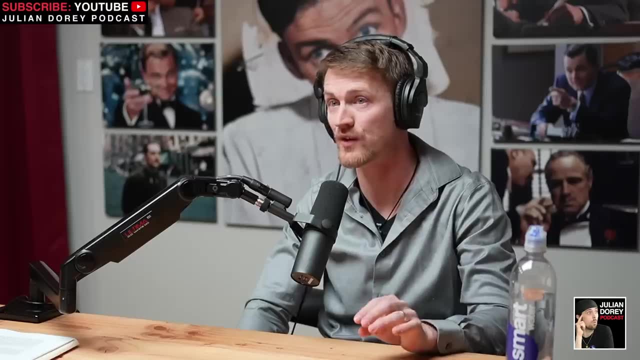 laws which also echo, like the Vedic texts and the Hindu texts, and then getting into the ancient Sumerian and Babylonian texts, and then getting into the ancient Greek, which is hermetic texts, And then a lot of others as well, like, for instance, Gnostic. 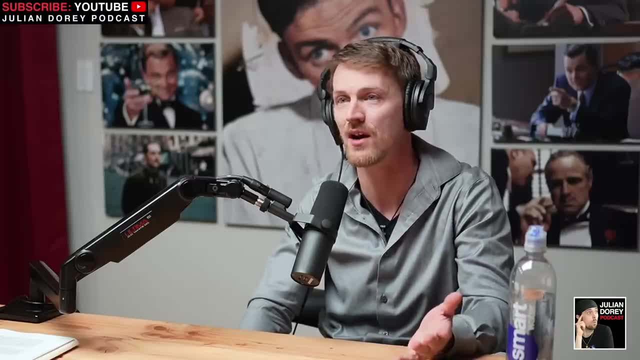 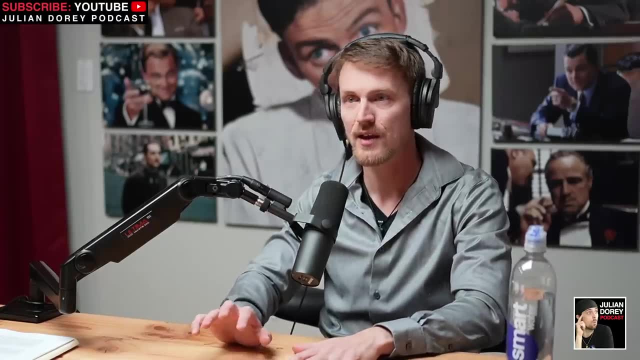 texts. We could get into some ancient Hebrew texts like the Book of Enoch. They discuss a reality that's very different than we understand it today. It's like they viewed reality different, If that makes any sense. Imagine if, for instance, 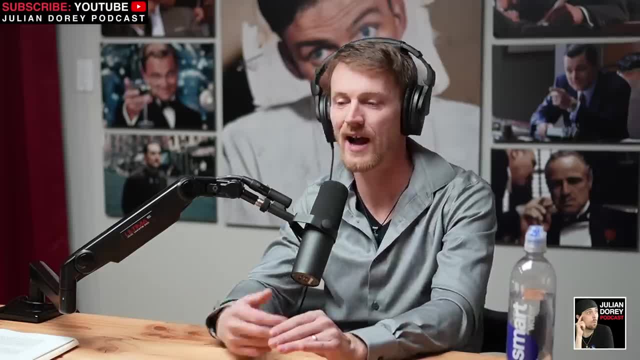 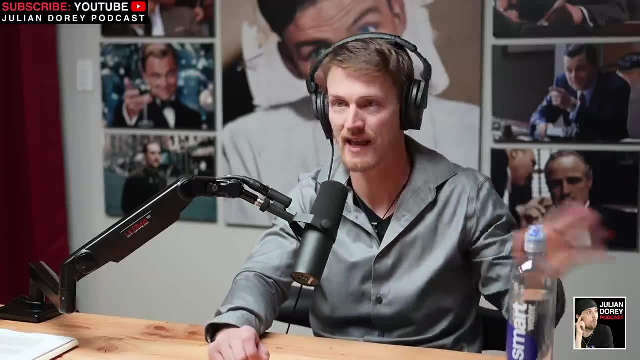 Julian Dory closed his eyes and I was able to describe to him what our reality is like, but he had no memory of what the reality that he thought was ever existed. Like you, almost like you, were born right now. right, But you're an adult. 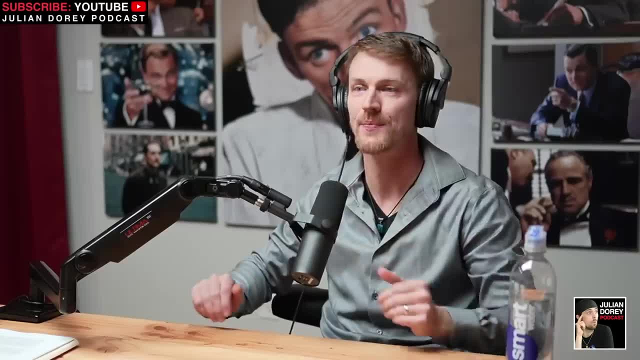 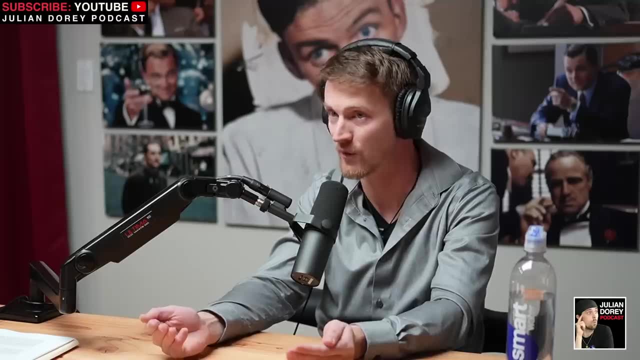 And I was able to describe it all for you. Tell me how the world is Right exactly. You would view reality very different than you did before, But it would also ultimately depend on what I'm teaching you right And what I'm telling you. 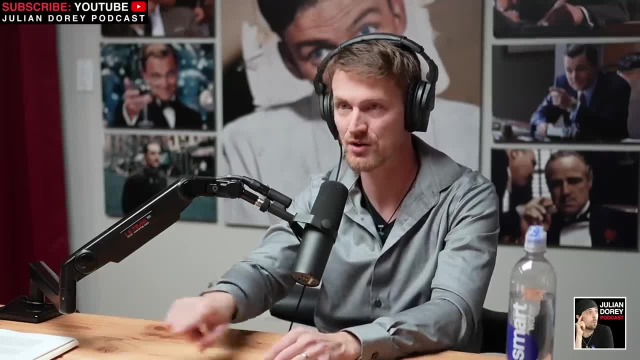 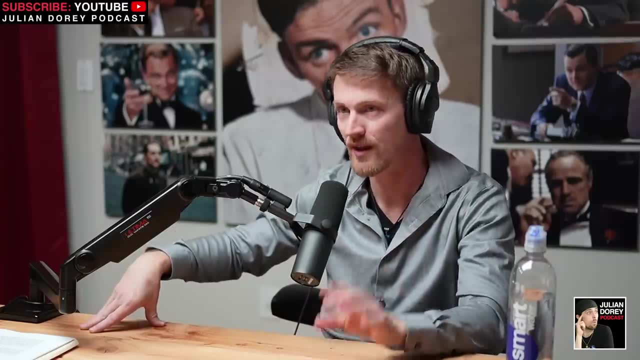 But if I was to try to encompass what the ancient knowledge around the world, of these lost civilizations, not the ones that came in the last 6,000 year window, but the ancient ones, If we were to encompass the teachings of the totality of all of them, 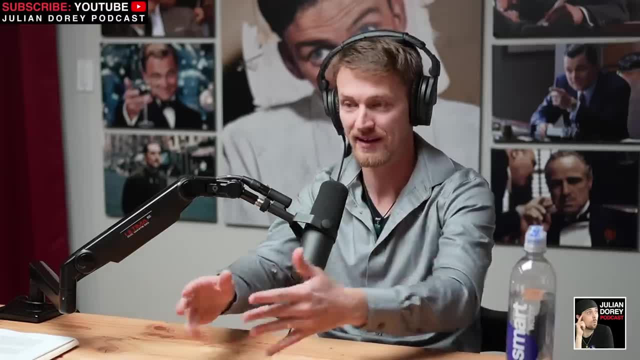 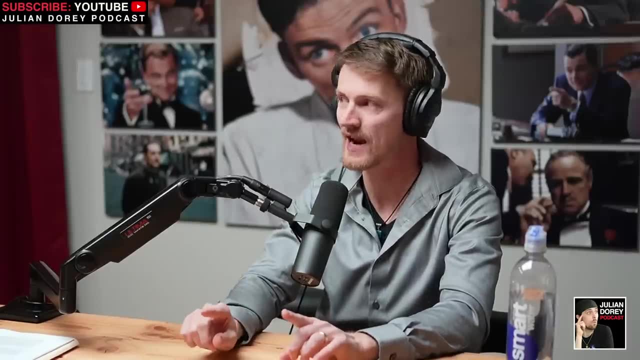 which is part of what we're going to do, and I taught you that and I was as accurate as I could be. let's say right And not biased. if I could, You would view reality so different than people that you would walk out and you'd probably like freak. 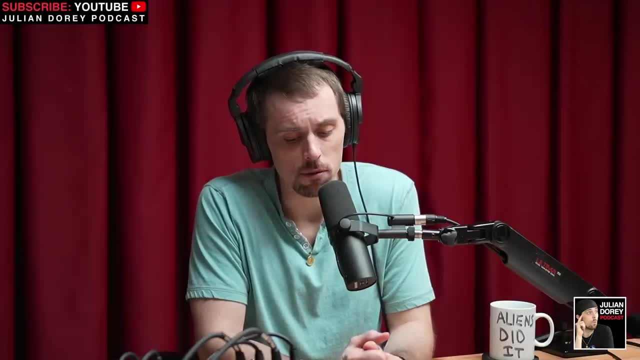 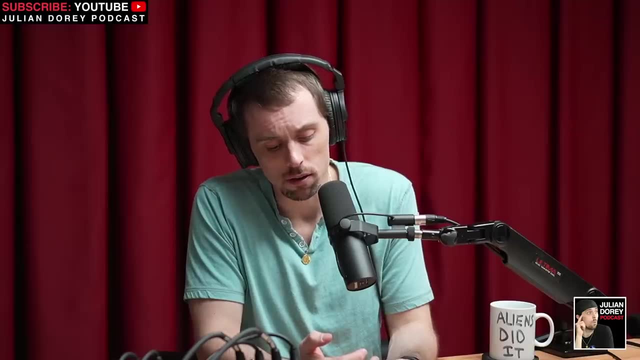 out. Sure, I think there's even a bigger microcosm example as well, Like more down granular. that makes your point. When you look at the phrase, you're a product of your environment, where you grow up. what it's like. 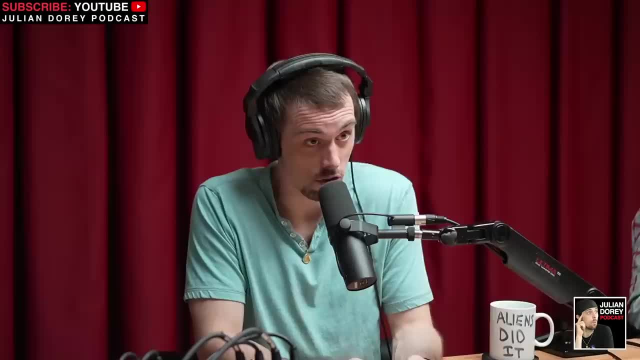 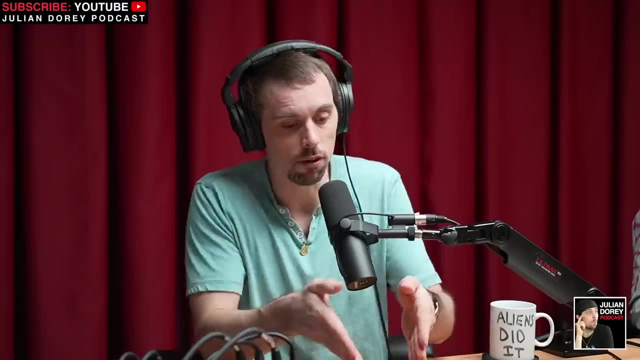 who the closest people to you are, what your parents are like, what they do, where you're growing up within that place. You are like, if you live in America, do you live in Iowa or do you live in New Jersey? If you live in New Jersey, do you live in Gloucester County or do you live in Hudson County? Everything, all the variables, continue and continue as it goes down to go like this and expand, and so your reality- me growing up in Jersey- can be so different than, say, some of the 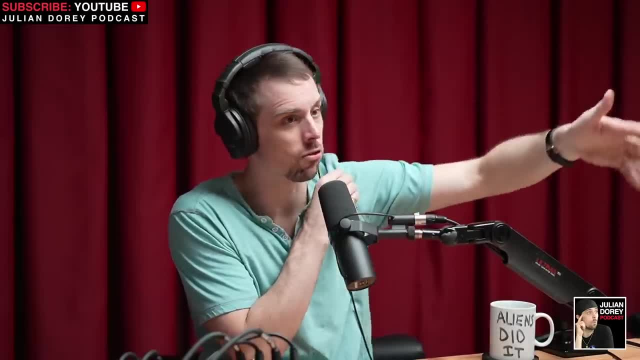 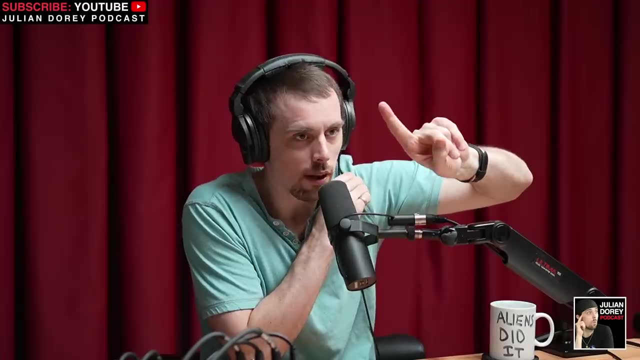 fans of this show, not even to go overseas right now, just in this country, who grew up in Texas or who grew up in Chicago or something like that, that even the stories within one little generation change. how see what I'm saying? So when you're. 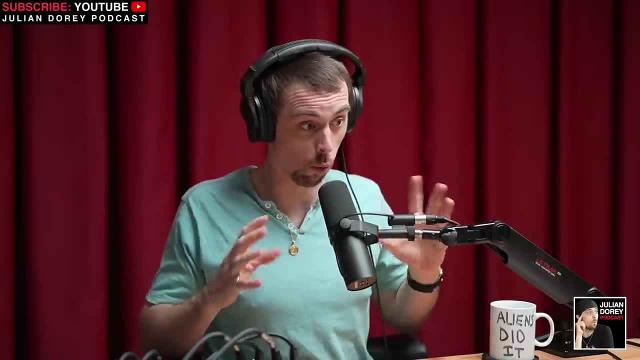 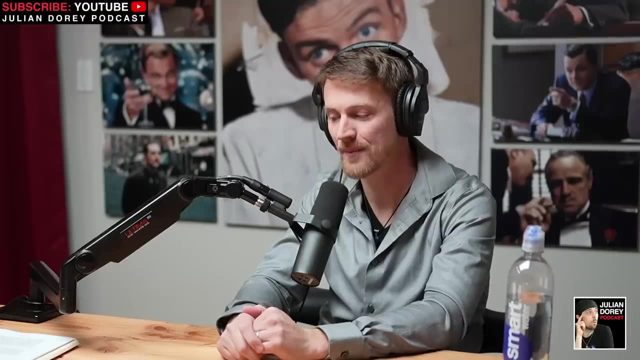 looking at it from the concept of ooh, let's go, the whole history of the world and the ancients and how it was done. the variables are literally infinite. It's incredible, isn't it? And I think that the conditioning, and not always necessarily on. 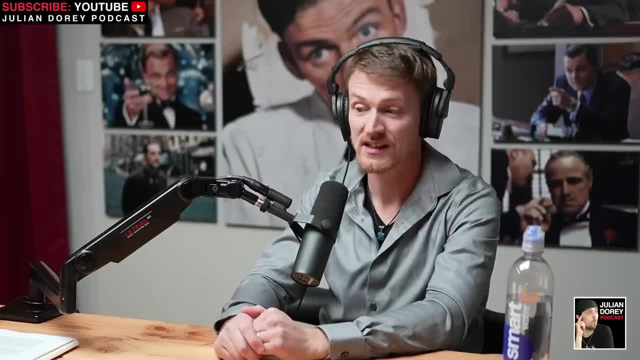 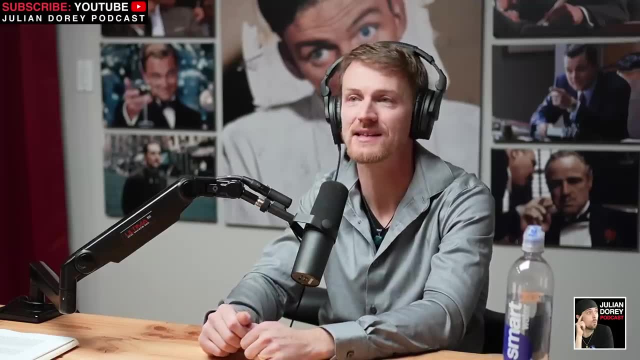 purpose, but the conditioning throughout the last several hundred years- and how many generations fall into that- has led us to a very- we'll call it an- interesting mindset that we exist in. Okay, Guys, if you're still watching this video and you haven't yet hit that, subscribe. 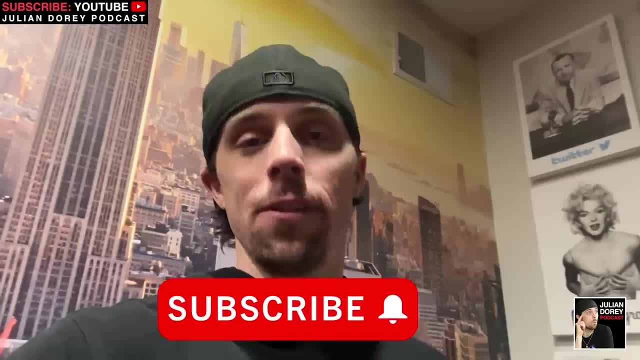 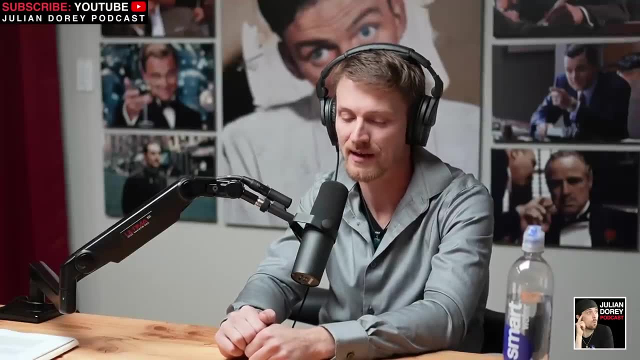 button. please take two seconds and go hit it right now. Thank you, And I find Who's conditioning people? Well, I think that there's a number of different avenues that it's coming down. For instance, if you just want to look at the education system in the United States, 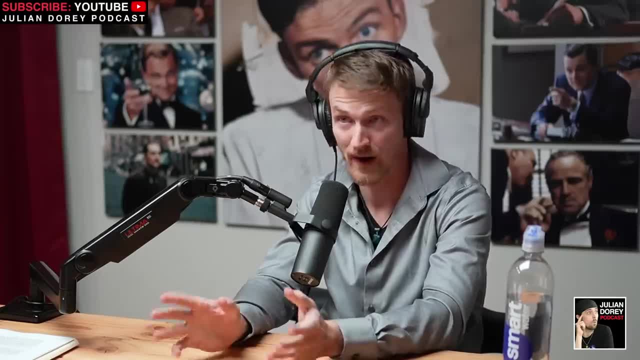 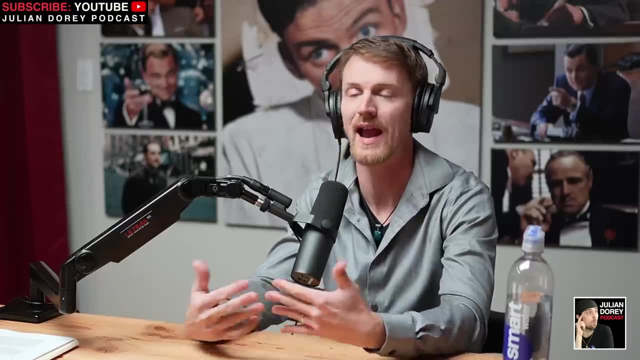 we know that it was designed around World War II by Rockefeller, And it was designed at a time that's very different than it is now, though They created an educational doctrine so that the average person could get an education that would allow them to work in a factory. 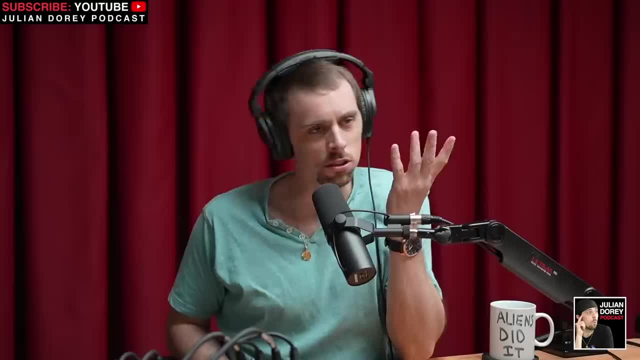 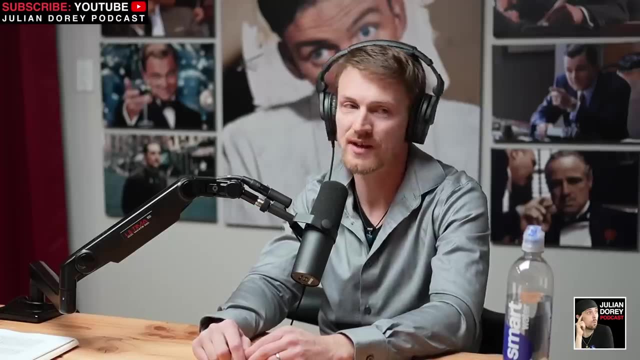 or wherever at the time was a job that was available. But eventually we got to. after World War II, with the GI Bill and everything, we started to push people to college. Well, we did, except that we still taught them the exact same thing in high school that we are now. 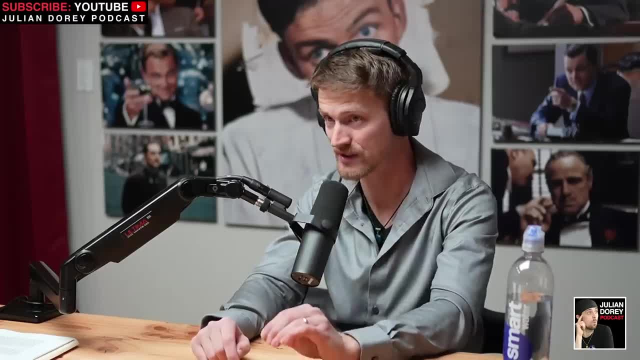 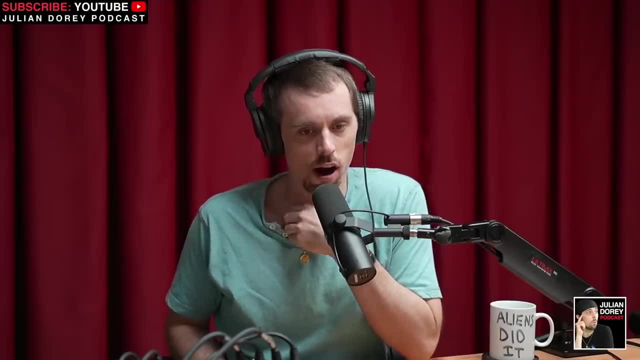 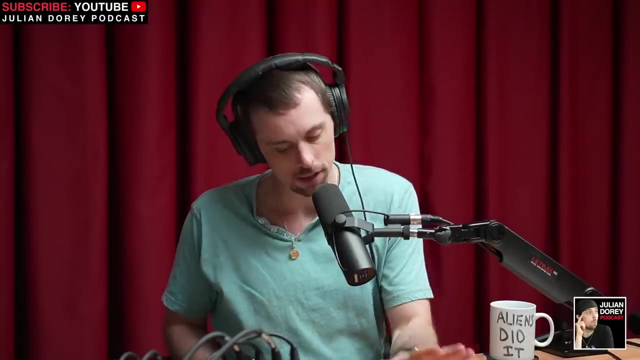 The education doctrine has not changed at all since Rockefeller Right. but doesn't it make a change when you then add in higher education as a more common trait of across society, of kids who are getting their education? So meaning let's say everything stayed the same? and it does change. 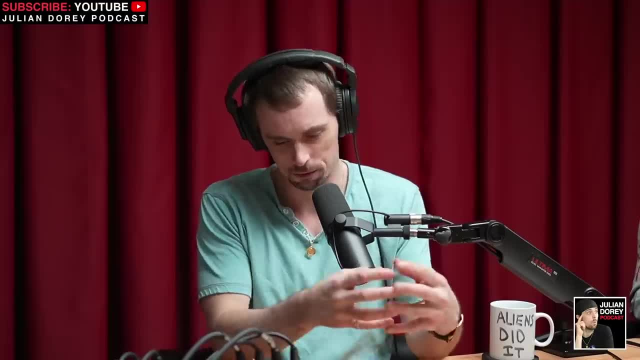 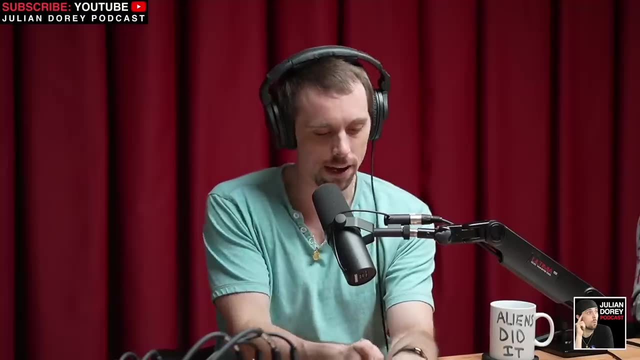 obviously, but you're saying, like some of the base ideas of how classrooms are formed and what subjects are taught, things like that I understand. But once you, then if you keep all that the same, if you add in an entirely new level of education, which certainly has its problems, 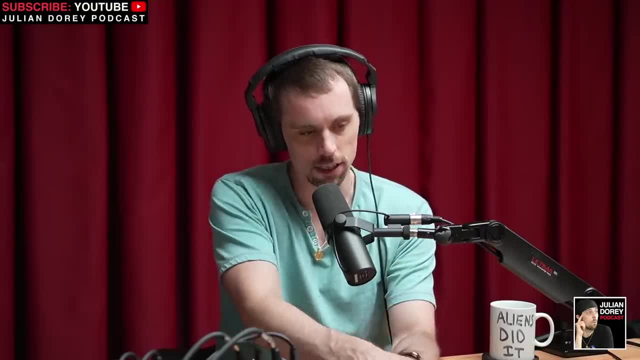 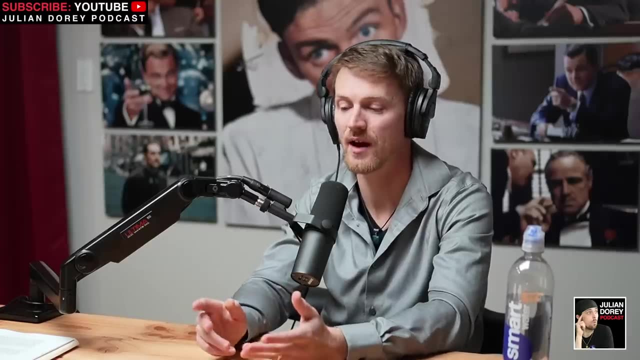 too, as we see these days. but like, once you add that in, aren't you technically changing? Isn't that a huge change? Except that every college still has a curriculum to teach. Yeah, Give me an example: If you go in, if you go into, 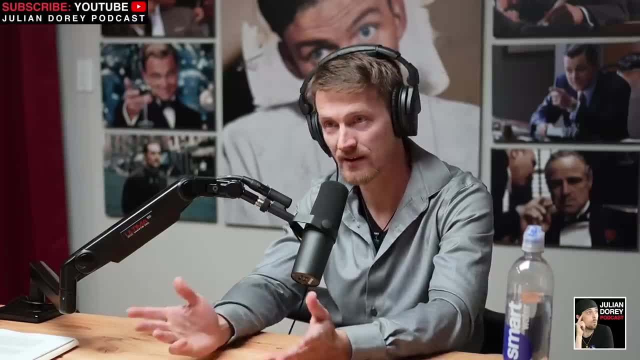 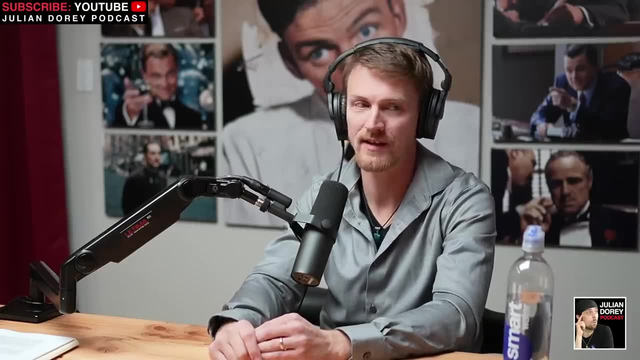 any university and you're like: I want to go to a history class. right, You're not in high school anymore, You're in college. now I did the same thing. You go into a history class and then you go, and then, let's say, you could be in two places. 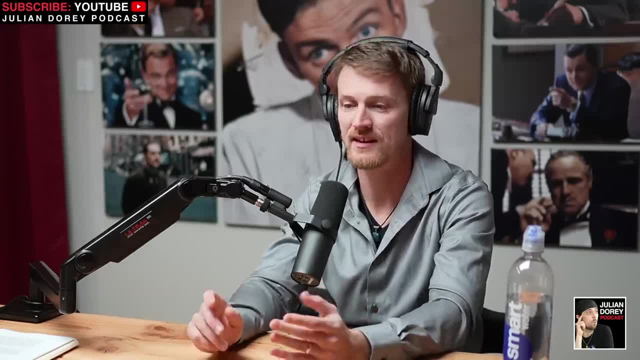 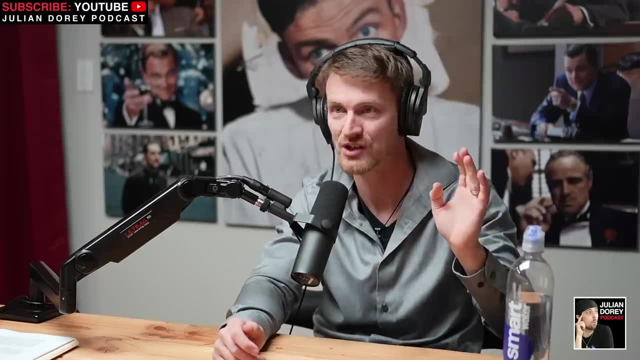 at the same time and you're in another history class, like in another state, They would be teaching the exact same thing, Exactly the same thing. It doesn't matter if you go get that higher education, you're just becoming- and I don't want to say a bad term here- I guess. 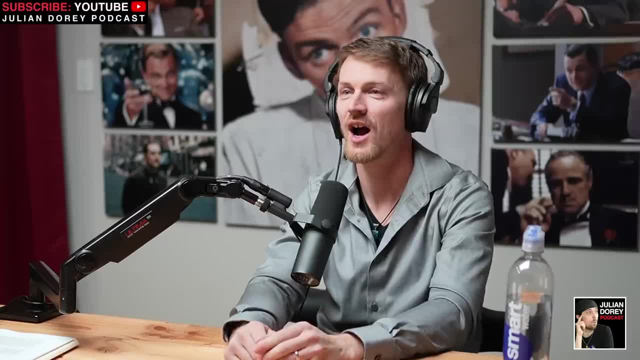 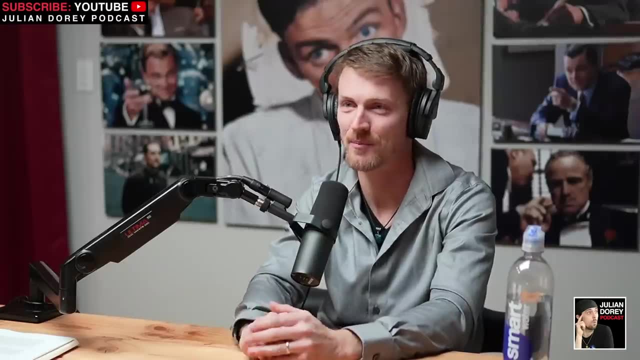 you're just becoming a smarter, a smarter animal, Right? I don't know. I don't want to use a bad term there, but I see what you're saying. I wouldn't say it's the exact same thing. No, it's not the same thing, because 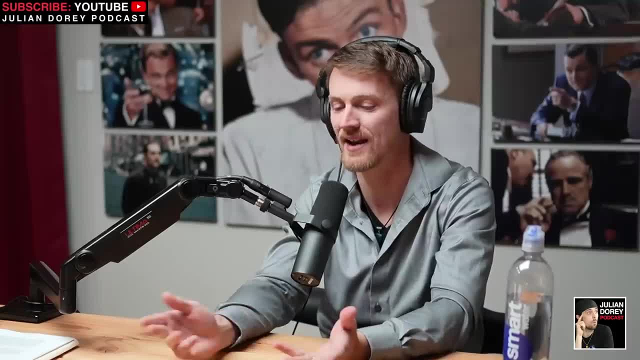 I mean, if you have someone go through a high school, if you have someone in high school and they don't get a college degree, of course they're still going to miss out on a wealth of educational aspects. It's like because, like you have to remember even. 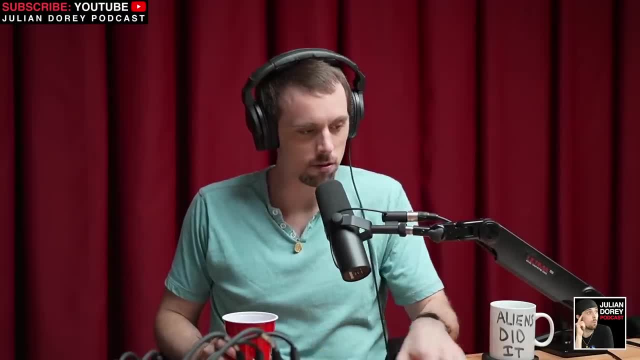 the teachers. human beings have their own take on things, Their own opinions. I mean, I remember a history teacher I had in high school, Mr DeFerdinando. Shout out, DeFerdinando, He was. 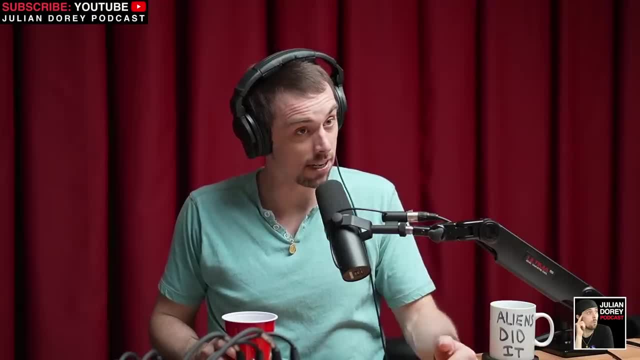 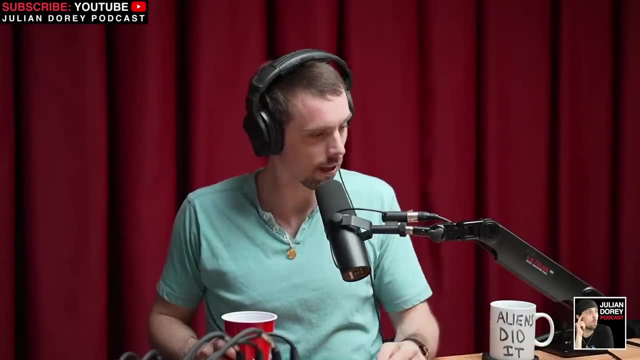 he had all kinds of wild takes on the world and it affected how he taught class. I like that Well. I wish there was more of him out there, Yes, But I know that and again, you know there's some that aren't like that and they're just teaching. 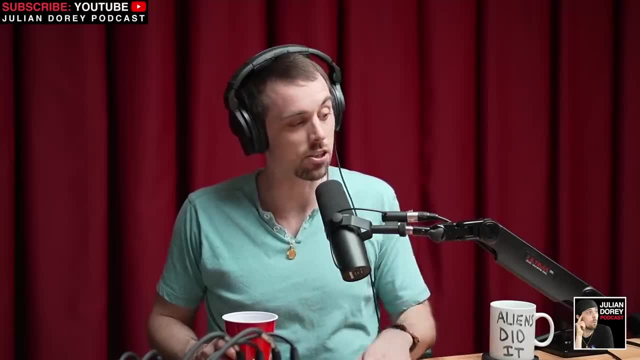 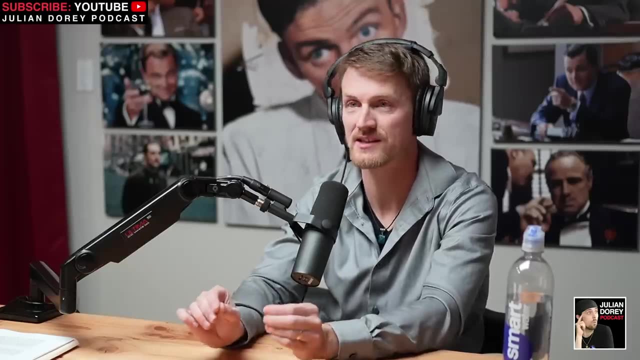 whatever's in the textbook, but that does exist, and I think it exists a lot more in college than it does in high school. Well, let's just say I agree with you, because there's more leniency in college if you're a professor. 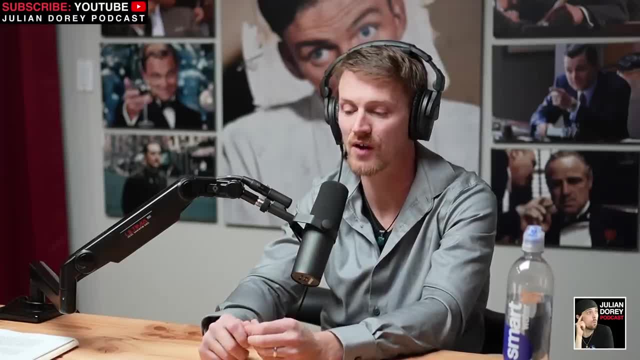 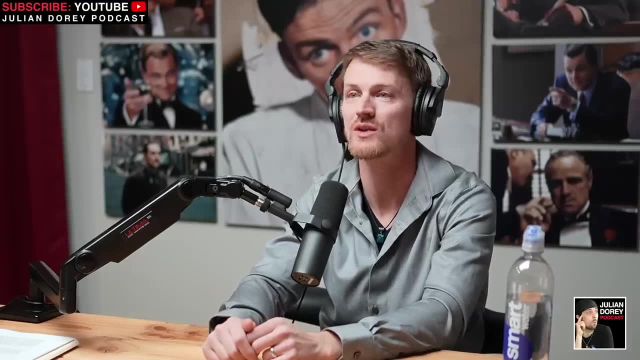 as a high school teacher. However, though, let's say, you're in college and you are a professor of history and you decide: you're like F all, that I'm just going to go teach whatever I believe based on the evidence, and you start talking about: 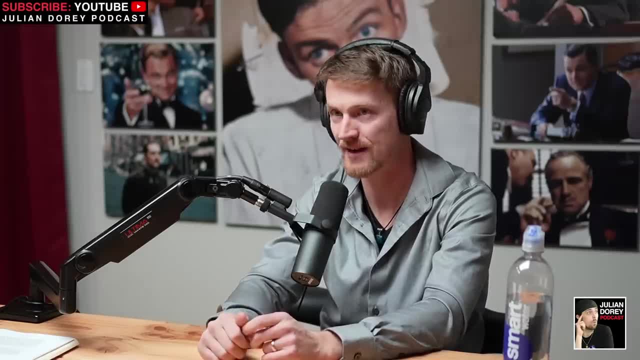 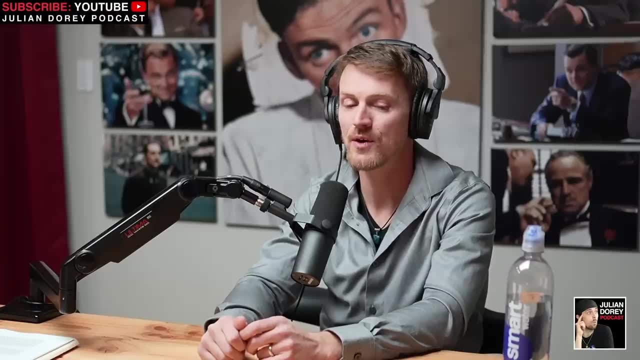 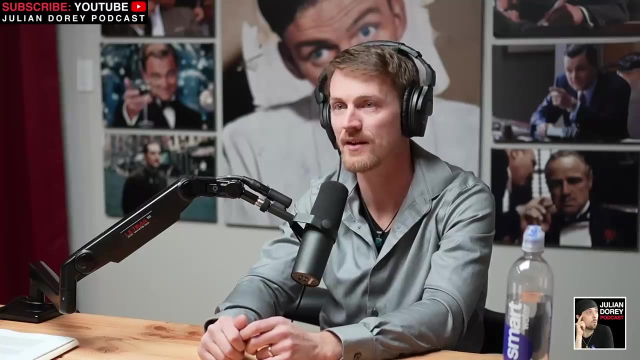 lost civilizations and you start talking about this. How long do you think that professor is going to have his job for Depends where they are? I would caution or I would challenge anyone to tell me if a professor that actually tried to do that. 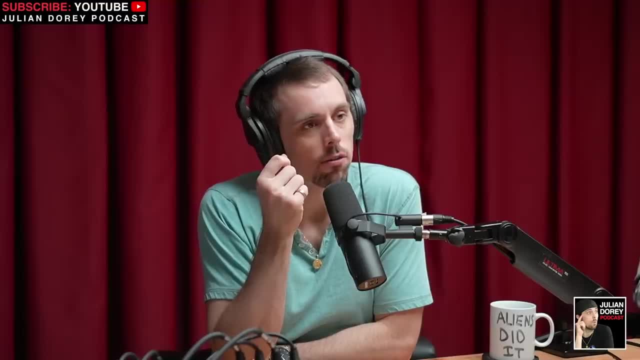 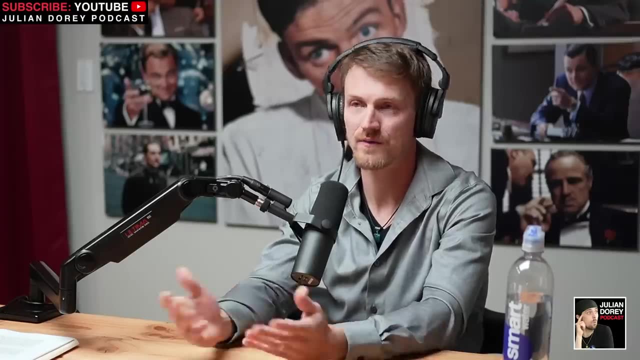 could survive, because I don't believe they could. Today it's a little harder. I think eight years ago it would have been no problem. Today it's a little harder. The point is, though, is that our? the point of this whole thing is that 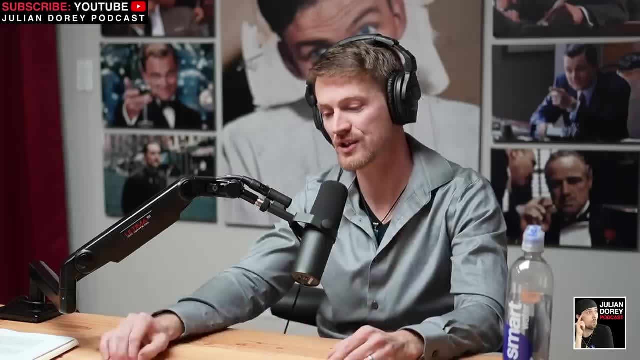 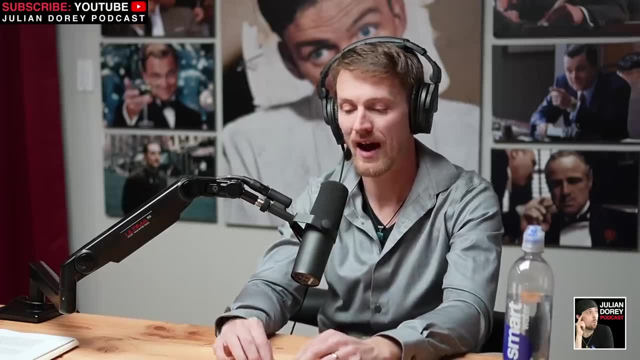 our viewpoints are based on all the conditioning and our parents and the influences we've had: the media, all these things right. And you asked who's doing it. I think that mindset of being a worker, just someone that has enough. 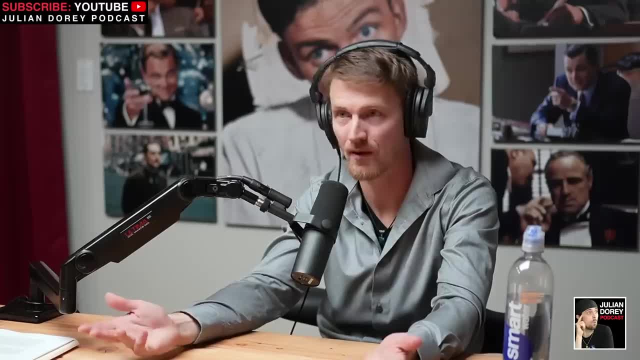 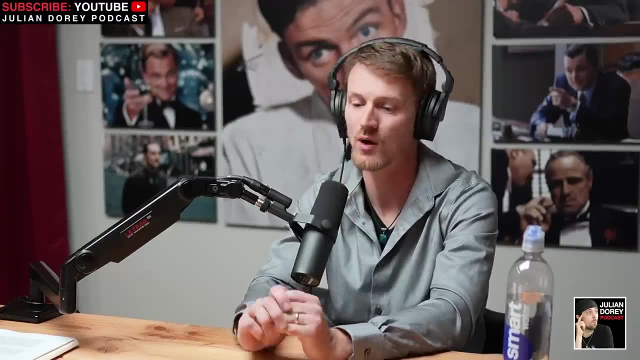 to not be stupid, but to be someone who can be a valuable member of society. I think that's the goal. It's just a good worker, someone who's going to get things done and go home to their family and take care of their family, and that's fine. 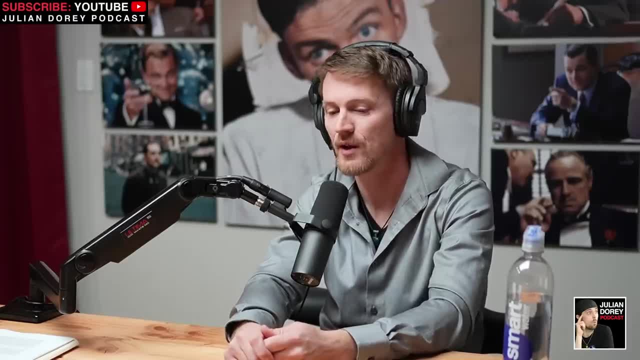 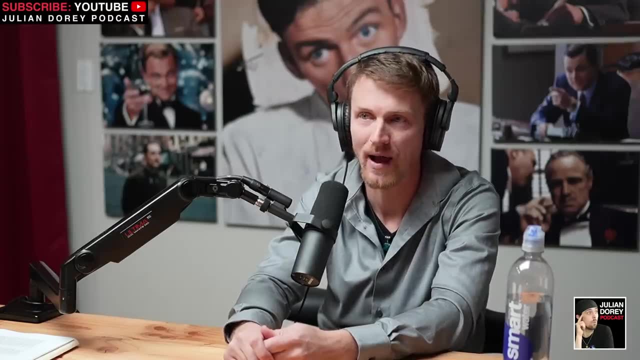 It's a noble thing to do, But what about? what about this whole aspect of what if we knew the truth about our past? What if we knew? what if we knew things that would radically change? What if we knew things that would radically change? 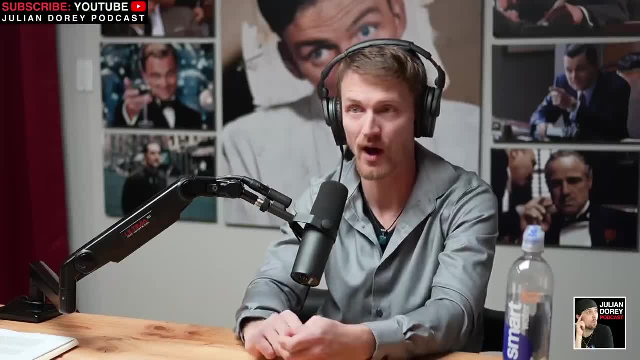 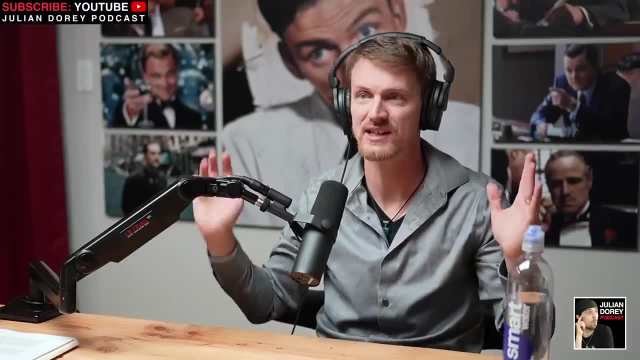 Our entire understanding of who we are now, how far back we've gone, who we really are like our origins, where we come from, how all this ancient knowledge of reaching states that we've forgotten was seamlessly passed to them, and they seem to have built temples. 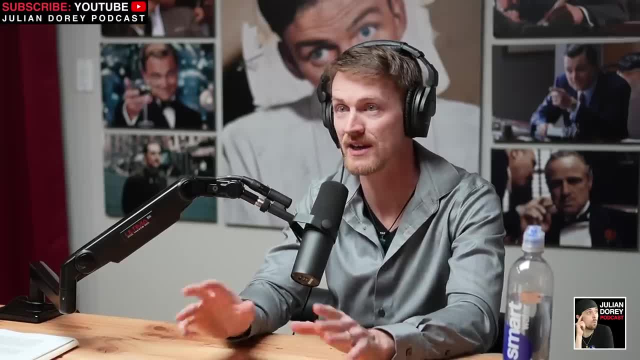 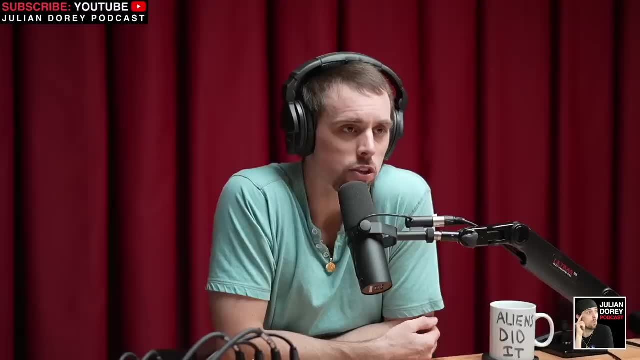 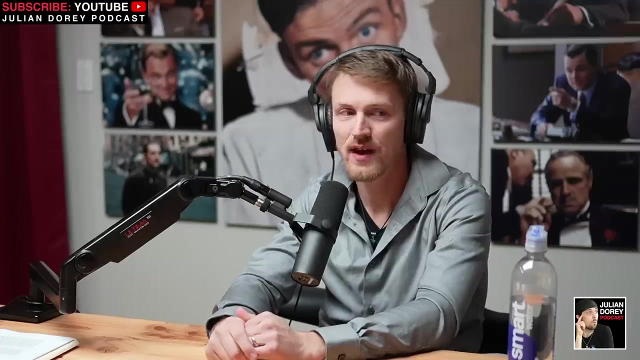 and pyramids and things around the world that we don't even fully know how to do today, but it seems to be for the purpose, largely, of reaching these higher states of consciousness. So question: Do you think that if you had the unlimited ability to have that knowledge and recognize consciousness as it truly is and be enlightened, if you will, do you think we could live in a world where everyone was equal and happy, like socialism tries to make it? 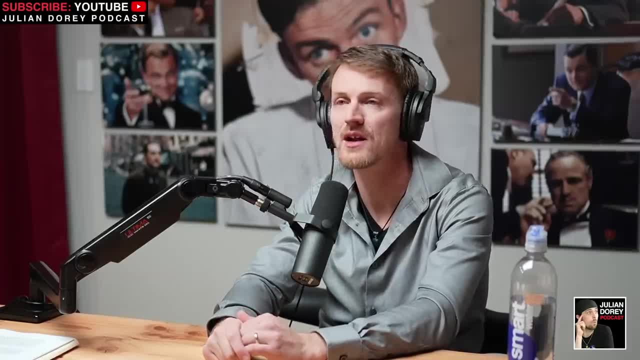 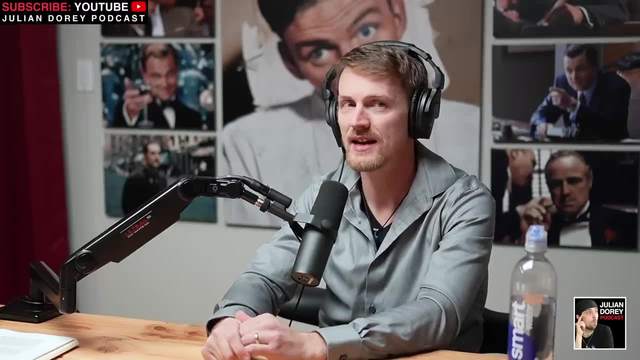 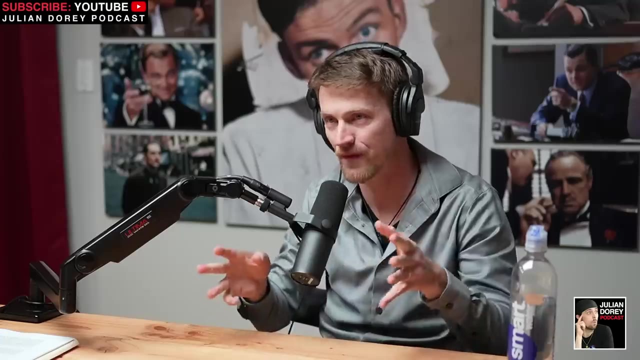 I think that the people that are in charge of those decisions know that humanity is not ready yet, And whether or not that's based on the fact that we've been groomed to not be ready, I still think that it's an interesting thing when you look at the progression of our consciousness and the progression of what's fed to us and what you see. 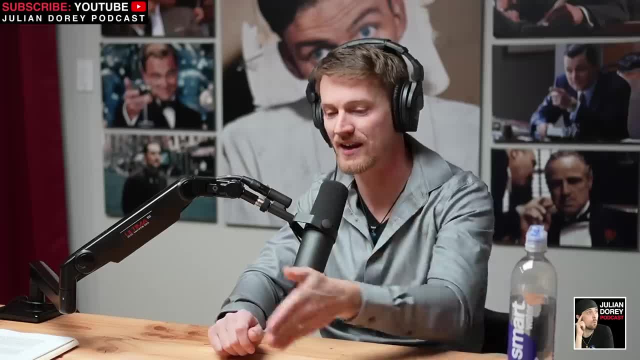 It's very telling. It's like they're dropping –, it's like they're injecting little things to be like: hey, what do you think about this? How does that sit with you? right? Because I mean, I think, when the truth comes, 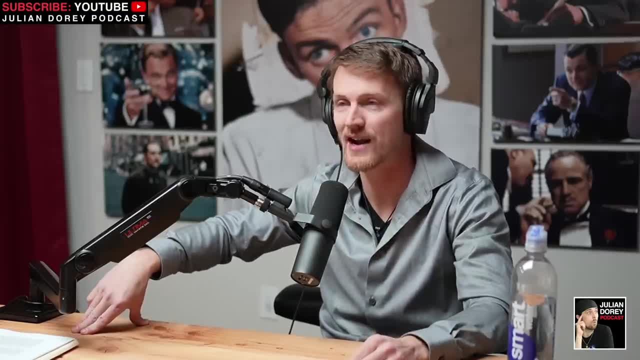 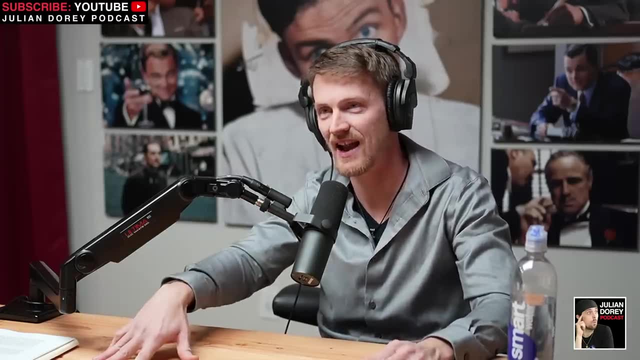 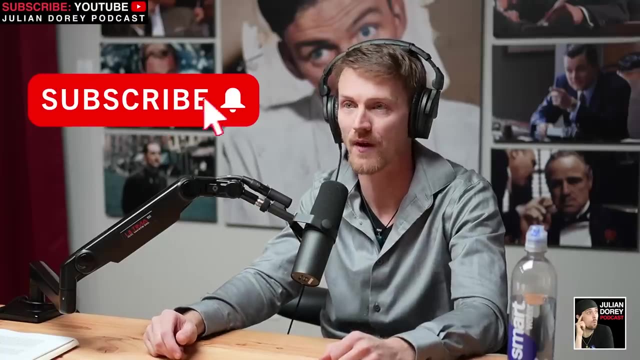 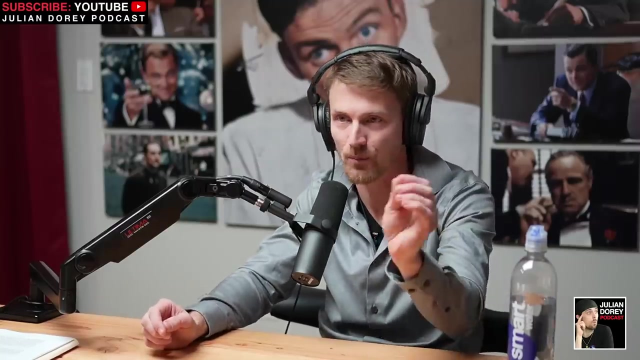 about a lot of things, like even a fraction of what we – like people like me- talk about. I think that by laying those little seeds down, people will not freak out and they'll be a lot more comfortable with the idea. I mean, look at all the UFO stuff, and not that I'm even a big supporter of that angle, but at least it gets people like thinking and talking about something that's beyond just their little periphery of life. 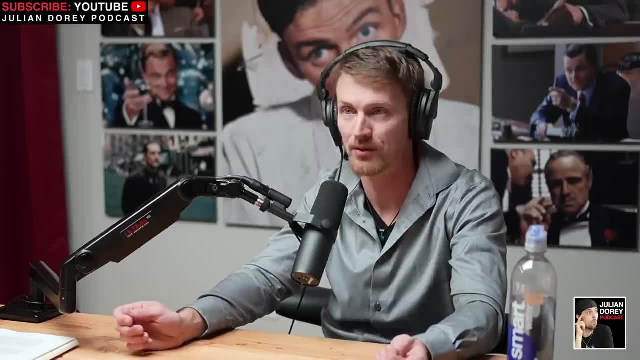 I mean, I wish people would look up and like remember that we're on a planet that's spilling it. It's like spinning 1,000 miles an hour. that's in a vast universe. I feel like too many people forget that. 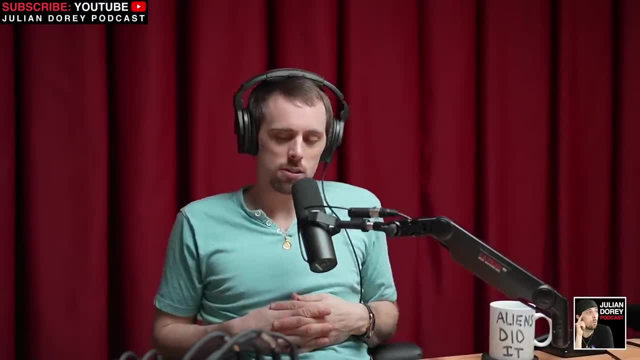 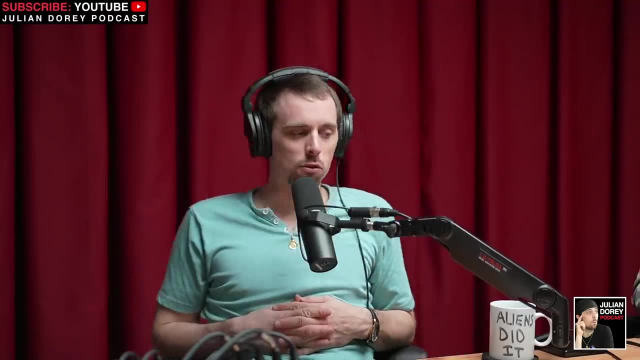 Psychs. at least get that, And you know what's interesting, though, When I start thinking about this stuff too much, my brain plays so many tricks with me because I'm like, okay, well, if some people don't want people seeing things, then why do they push so much of it to us now? 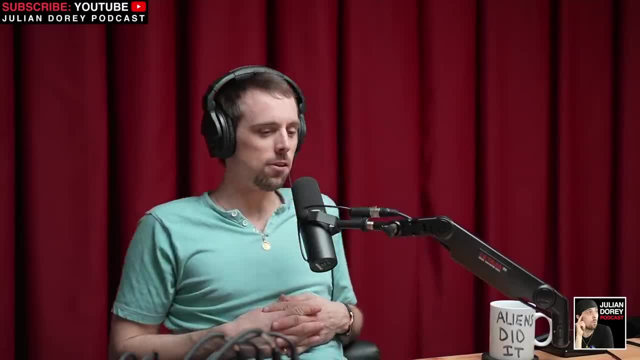 And it's almost like this never-ending cycle where you can't have it both ways, but you want it both ways. Does that make sense? Yeah, You know what I'm saying. It's a little – that's a little complex how I put it. 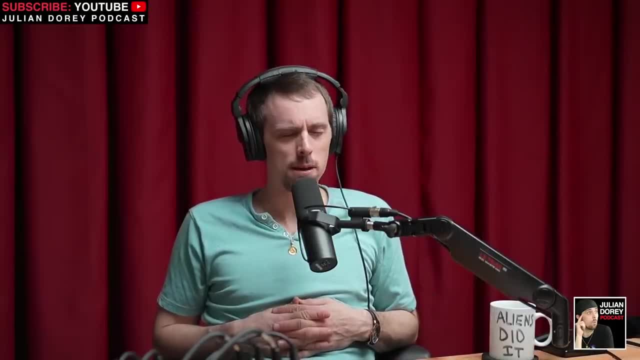 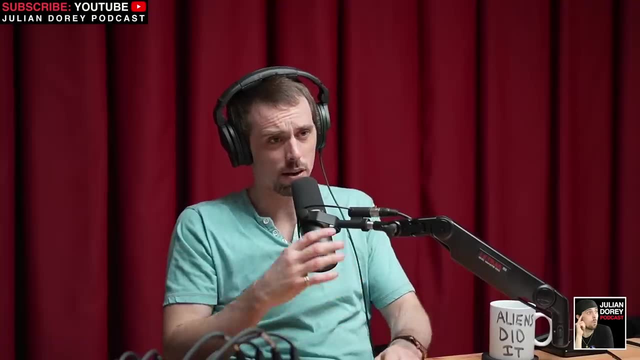 But I do agree The main point that, okay, we have narrative A. Yes, Narrative A is what we teach. Yeah, exactly, We'll teach it over and over. That's bullshit, I agree, Yeah, It's crazy. 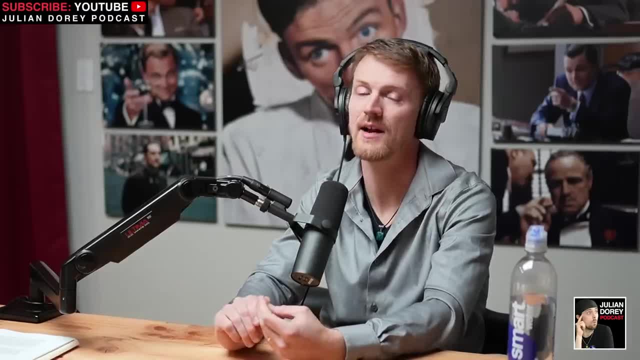 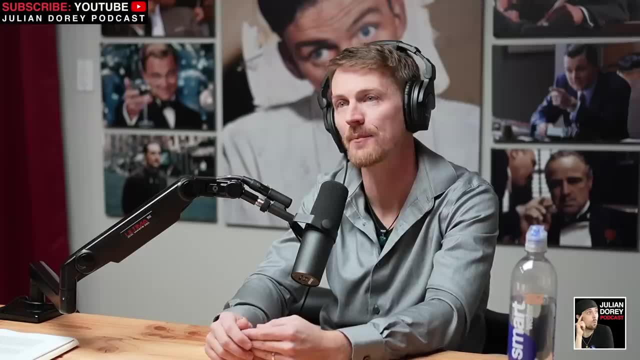 And so at some point that's going to collapse and change, And it's going to be – I think what it's going to come as is a reforming education. I think it will change in the future a lot And it will come – it's going to have to come though, with, like a pretty big movement. 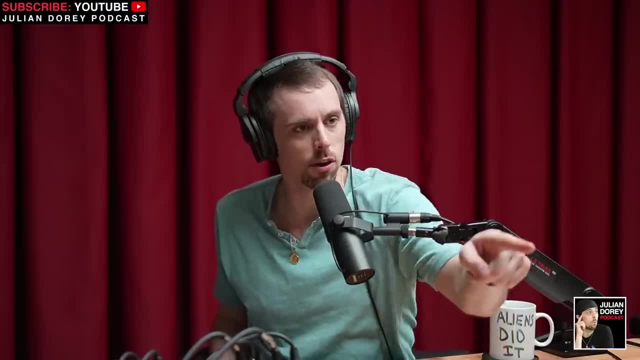 And right now that doesn't exist. Well, can I bring you back to this? Yes, Yes, We'll get down that rabbit hole forever. That's a good conversation, Absolutely, But I want to come back to this picture we were looking at. 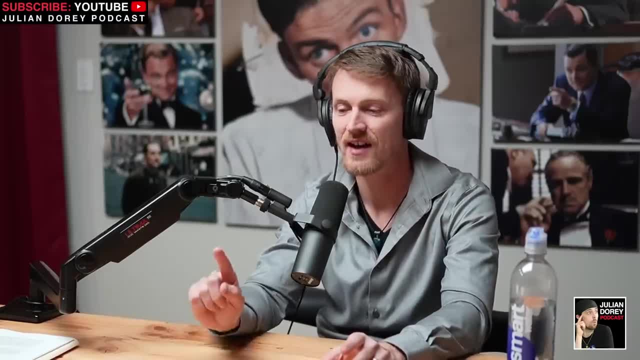 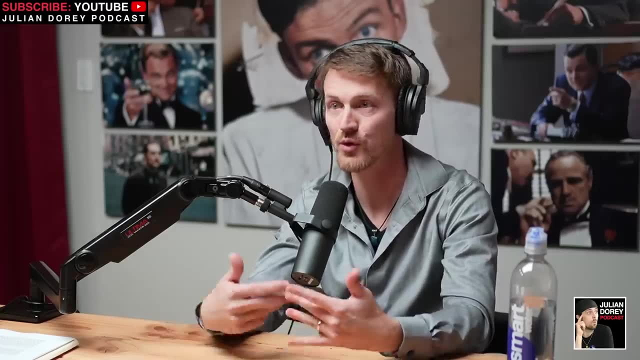 Yes, So getting all the way back, because we definitely got down on a tangent there. But since you and I talked and I found this ancient temple, as I was saying, through images and other archaeologists that have been talking about the stone masonry being some of the 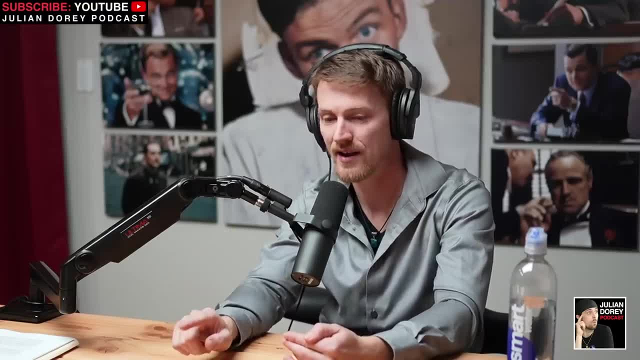 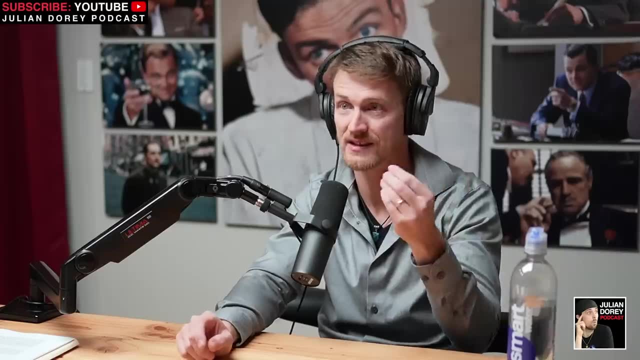 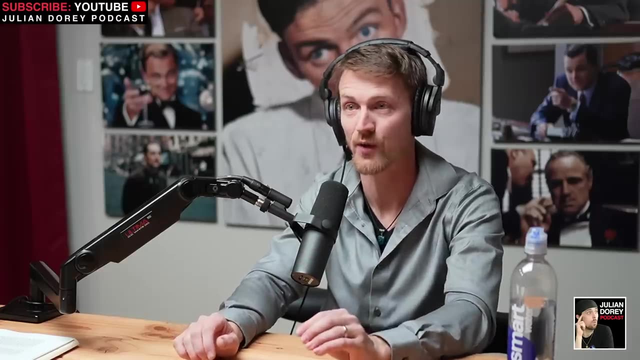 finest they've seen. in all these aspects, when I saw just one photo and I had known already the significance of the symbols and the icons, I had exactly like that moment of George Smith, and not that I'm going to compare to his discovery, but I literally ran around the room three times okay. 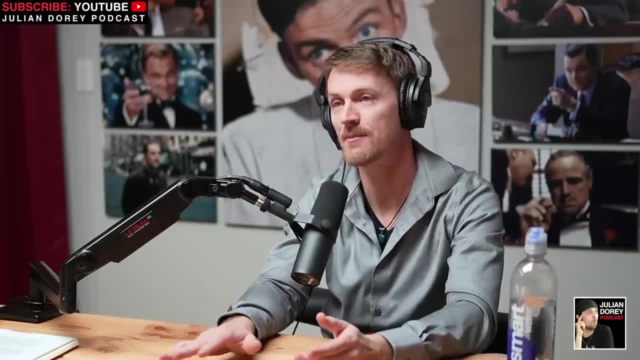 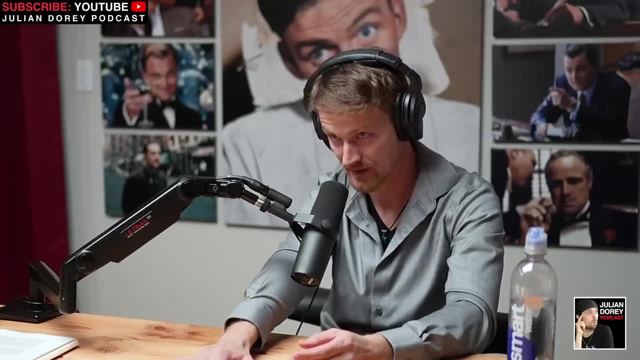 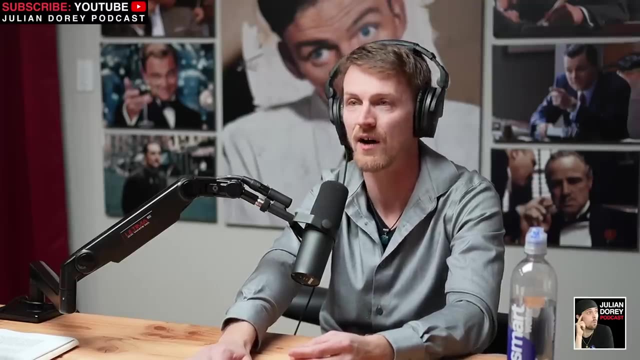 I absolutely did, because I know, at least in my heart, in my expertise and what I've looked at, the significance of this site. Now the site is called Ionis and it's called Haldi Temple And it's part of the new – this mysterious, lost civilization I talked about last time. 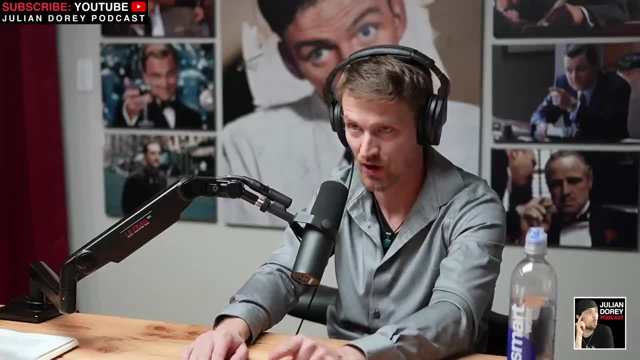 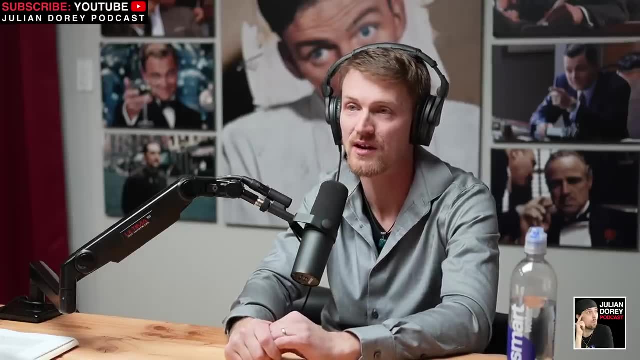 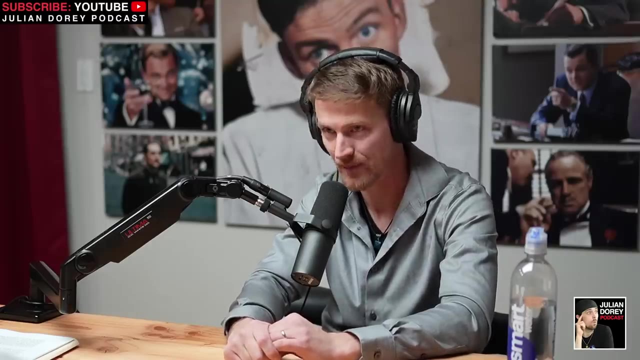 called the Ararat Civilization. That is not what archaeologists are calling it. Archaeologists believe that this entire set of ancient sites around Lake Van in eastern Turkey is built by a civilization that came eight to ten plus thousand years later. They believe that it's built by the Urartian civilization. Urartian, U-R-A-R-T-I-A-N. The Urartian civilization was interesting because the name itself comes from the word Ur, which is an ancient Sumerian city, The city of Ur. Alessi, could you – do you think you could find some? 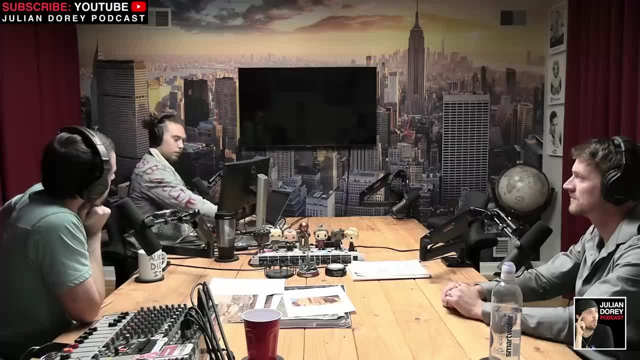 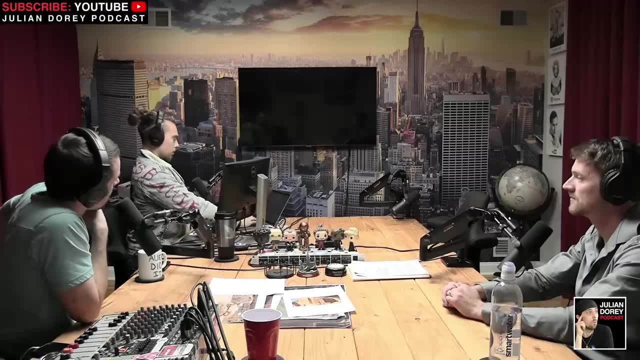 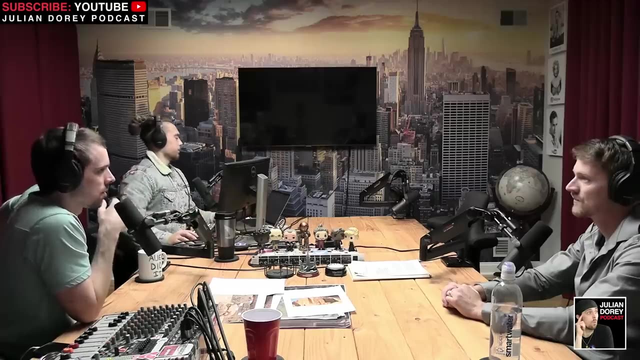 I don't really even know how to search this, but maybe you'll be able to picture what I'm picturing in my head. Could you search like oldest human tribe civilizations? Yeah, just search that. I'd love to see. like what they say, because you hear some of these – like Sumerians. 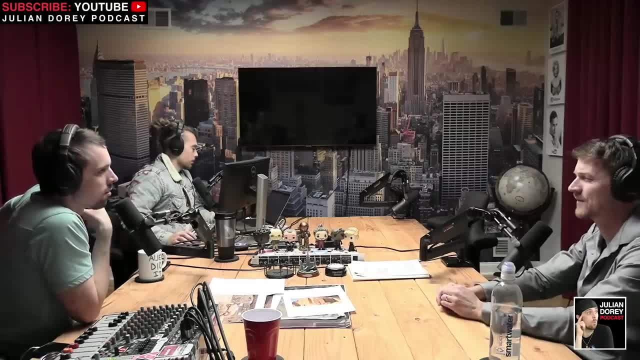 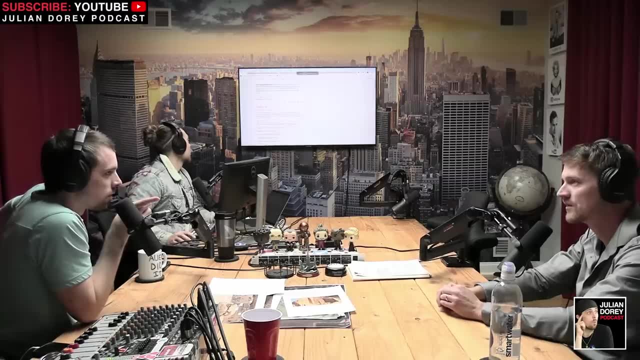 Babylonians. They're always primitive, right? Yeah, they just show something primitive and it's like – the mindset is interesting, Point being what you're – how do you say that again, I-on-us, I-on-us, but the other one that starts with a U? 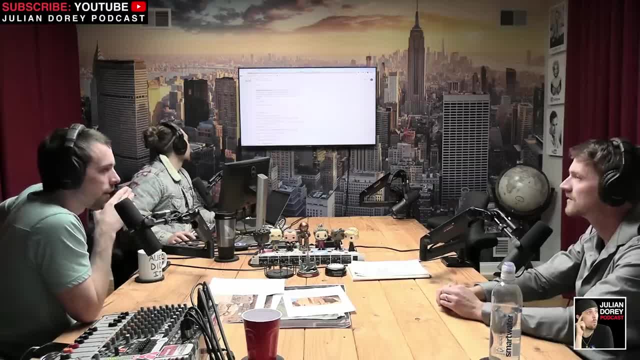 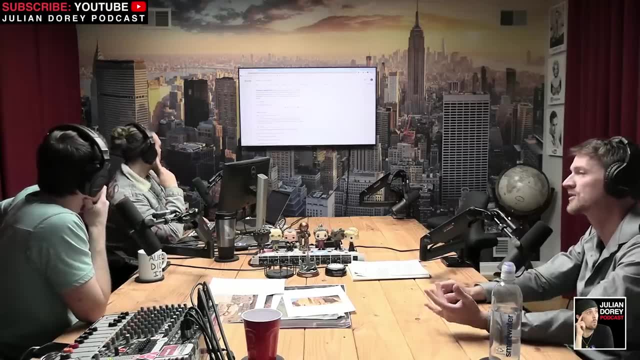 Oh, Urartian, Urartian. So are they like before all this? They came after and they found the ruins and remnants of this civilization. They knew their ancestral connections to it and so they built right on top, just like we see in a lot of other places around the world. 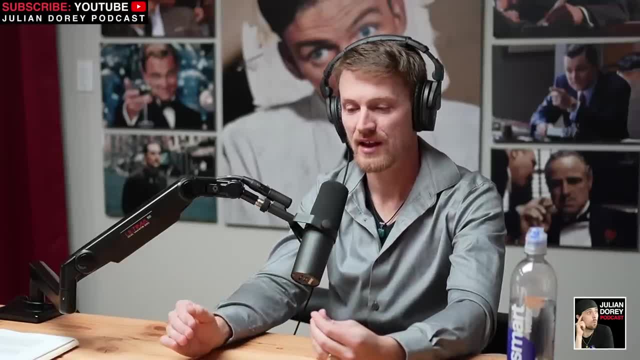 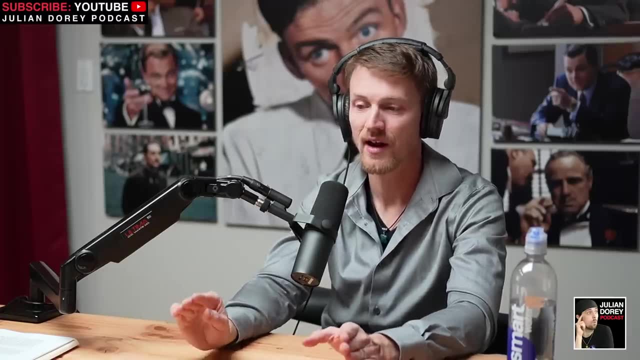 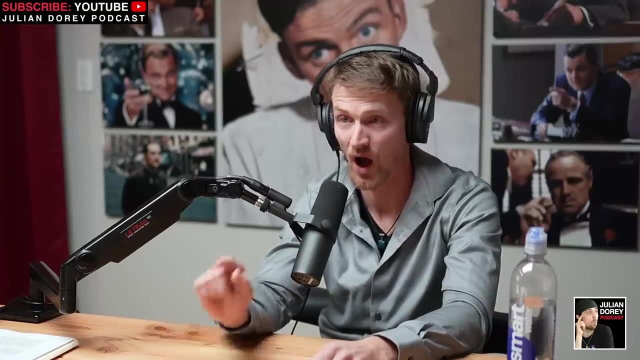 But that – when I found I-on-us, it changed my entire life. just to say that, really frankly, It changed my entire life. It changed my entire life to the point where I realized that what was there was so significant that I was going to focus my entire career and my entire life going forward on uncovering. 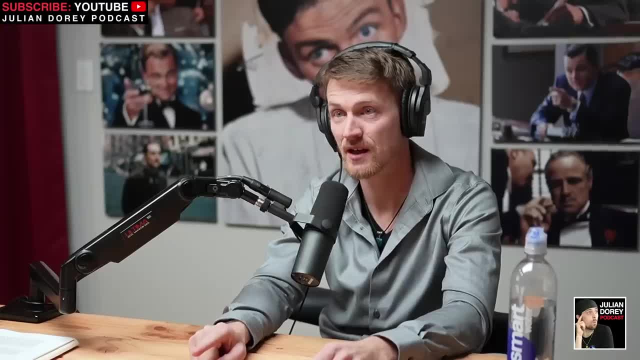 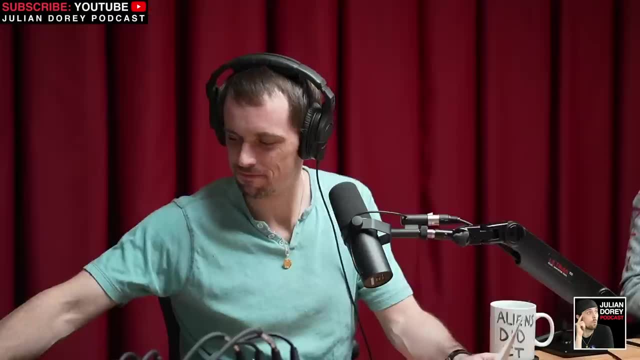 the secrets of this civilization. Yes, Even more than Eridu. It's like if I have a good poker hand, like we were talking about, but I don't know how to hold it back, and I just talk about it, It's a really good poker hand. 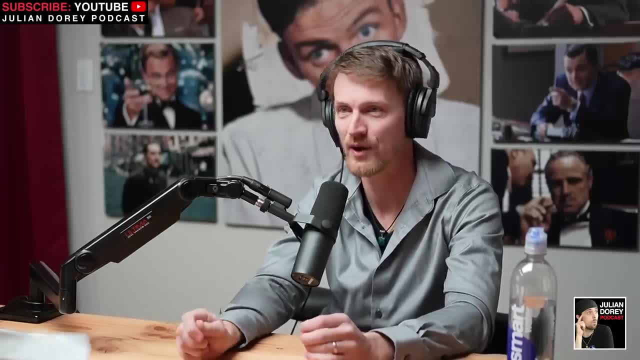 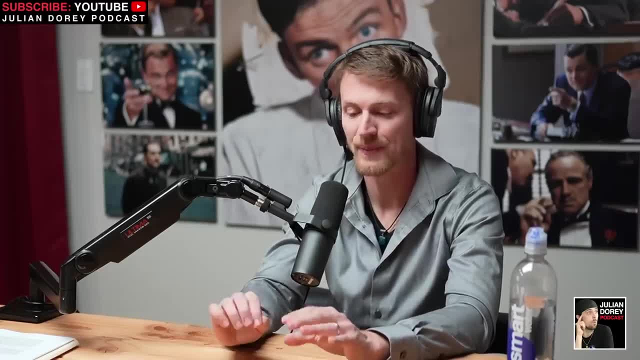 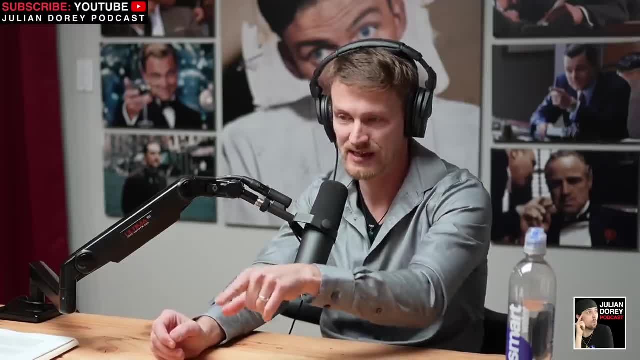 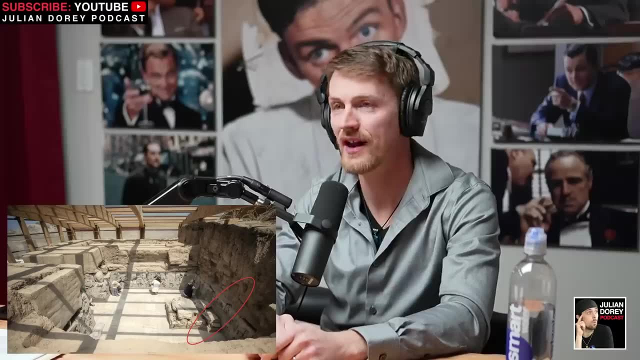 Okay, Now that site called Ionis… And we'll be putting this intermittently in the corner of the screen for people following along as it comes up. We'll put it back up. I realized that those discoveries were so significant that I started my own company. 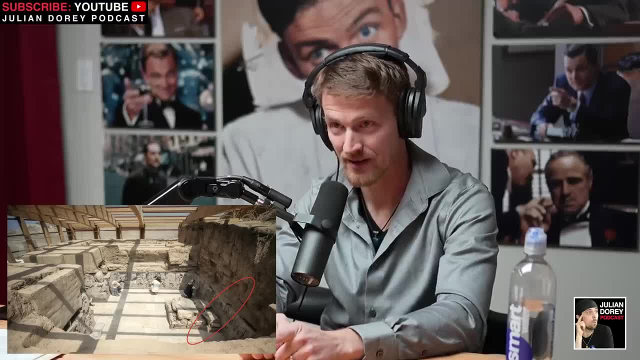 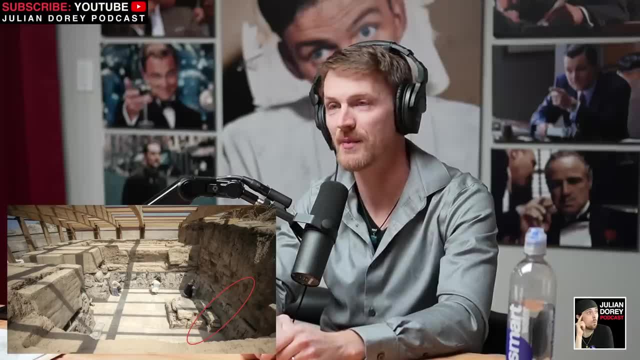 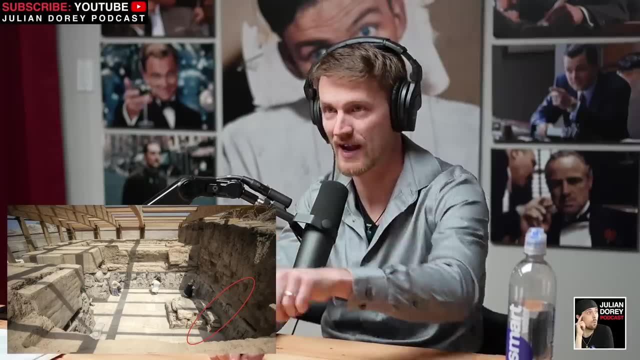 Wow, Wow, Oh, this is like brand new- Okay, Brand new- as my entire focus going forward. Okay, Now, before we talk about that, though, I want to give you what you just were asking me about, a background on the site. 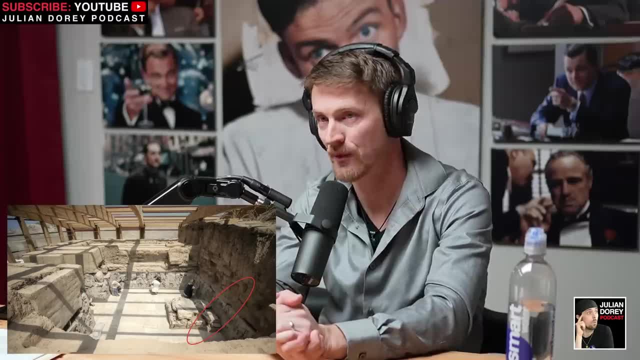 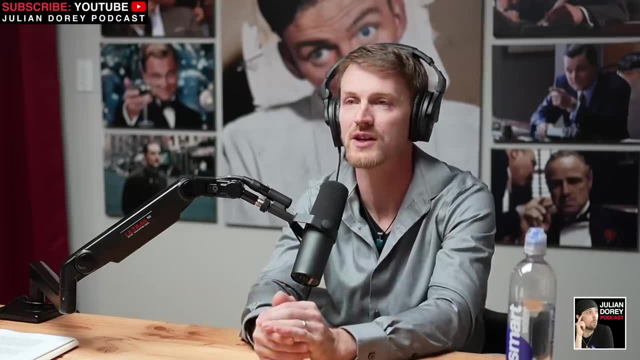 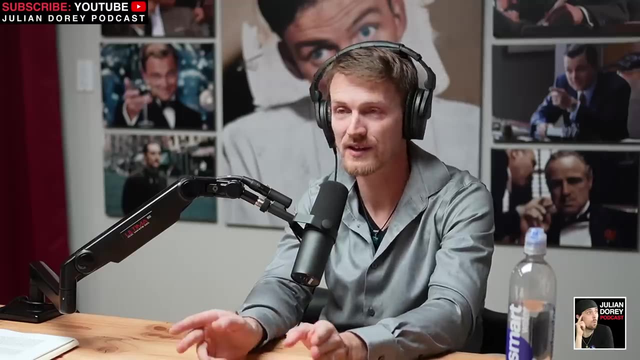 In 1989, there was a professor named Professor Isliki. He's part of the Turkish archaeological- you know profession, professional archaeologist there. He came along and I have to give that man a lot of credit. If he ever listens to that, he is a great man. 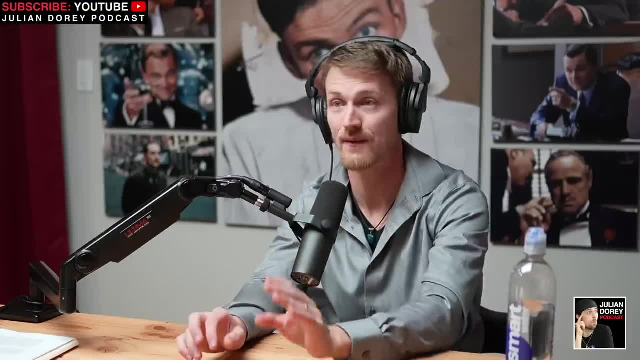 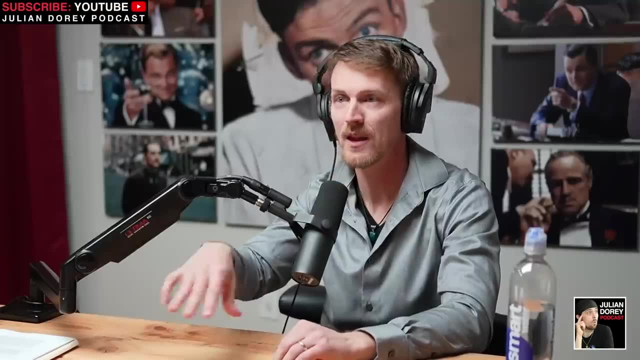 He's not part of the coverup history of the past or any of these things that have happened, because some of these sites were found in 1954, and then nobody ever heard of them again. But in 1989, Professor Isliki comes along and they're studying this place called Ionis. 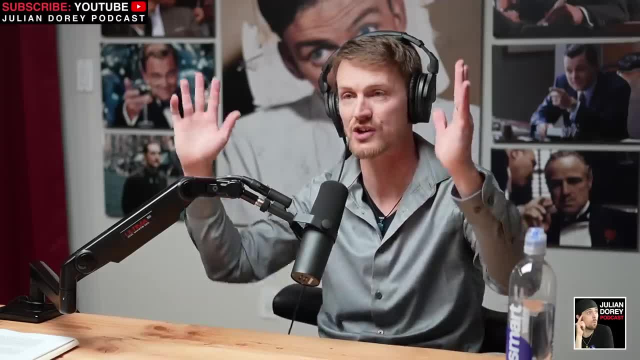 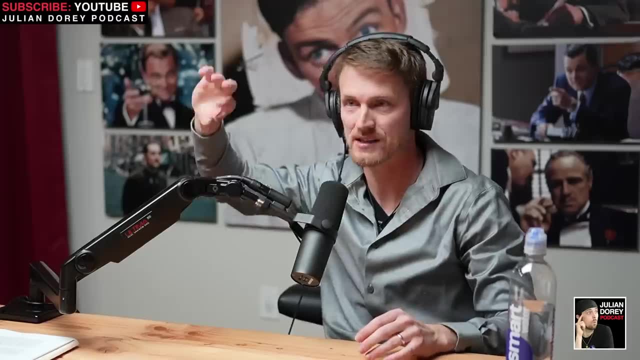 And Ionis is on the east side of Lake Vaughan and it's basically a large hilltop. It's beautiful actually. that looks right over vast Lake Vaughan and it faces directly at this massive 1340.. It's a 15,000-foot mountain called Mount Sufon, an ancient volcano. 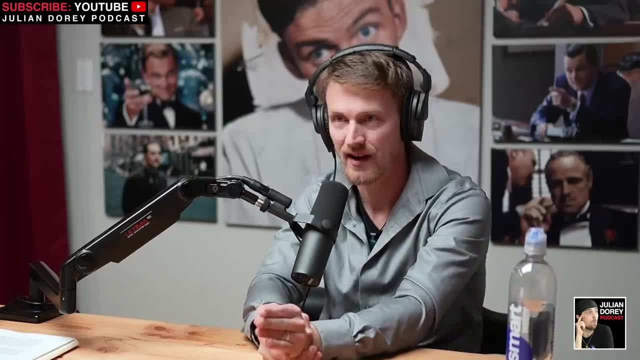 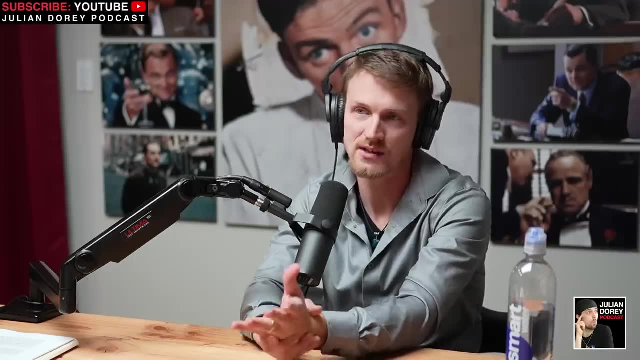 And it faces directly with the setting sun. It's a solar temple. It's based on the. They're basically worshiping the sun. It's a sun temple and their focus is the temple aligns, I believe, to the setting of. 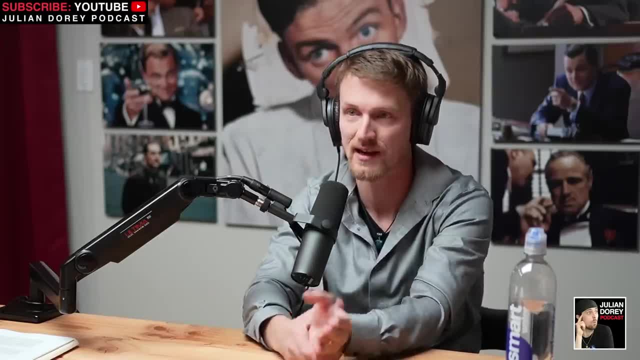 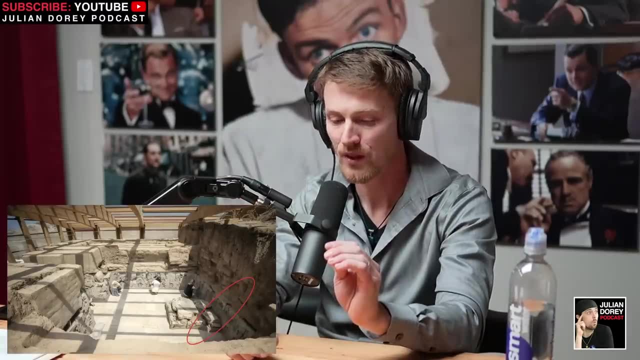 the sun, whereas the Kef temple on the other side of the lake it's facing is facing the east for the rising sun. So they seem to be sun temples And that's That's clear. But what happened was with the story. that's so fascinating is that when they were at the 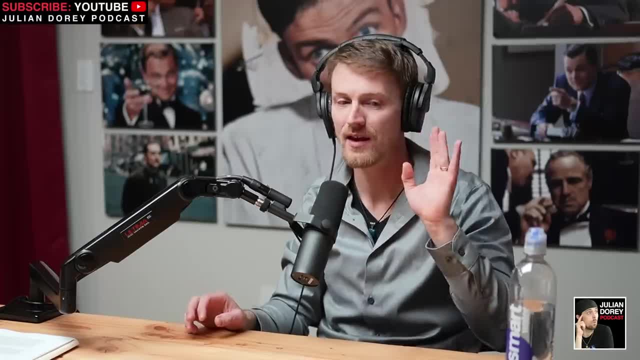 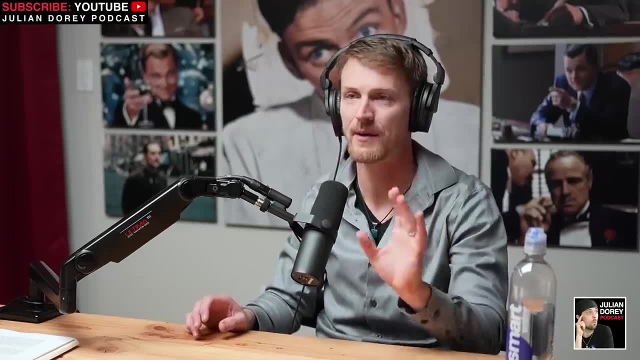 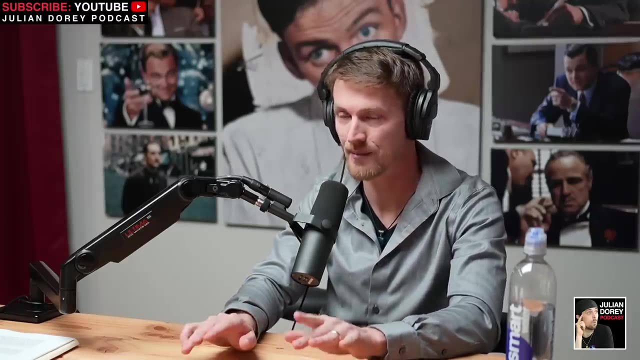 foot of the hill and they were just trying to find. They knew that there was something there, They had history of something being there, and so they had a lot of strong evidence that something was at that location. But it was buried under massive amounts of debris and sediment similar to Chirupac, and 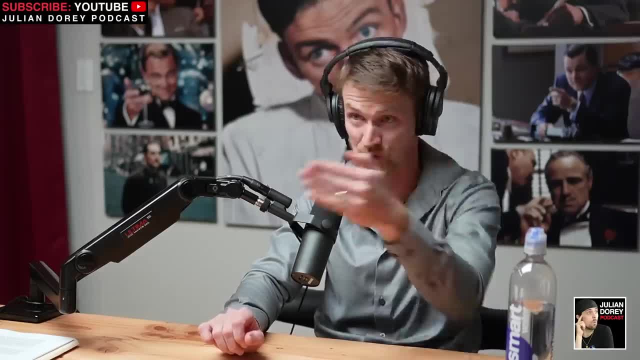 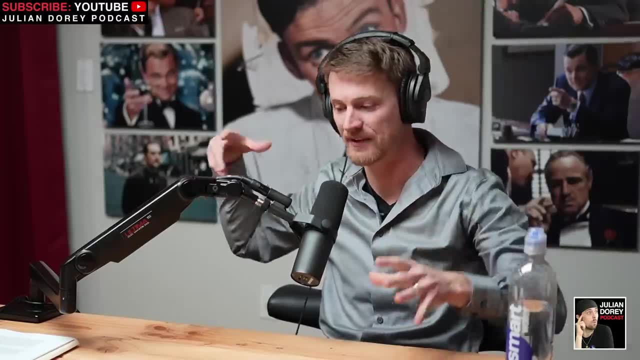 Sumer that we talked about a minute ago, from the ancient Sumerians- Yeah, Sumerian lineage, which is directly related to this. They found a mountaintop that had all this sediment piled on top of it, but they started to find remnants of mysterious walls and things at the lower part. 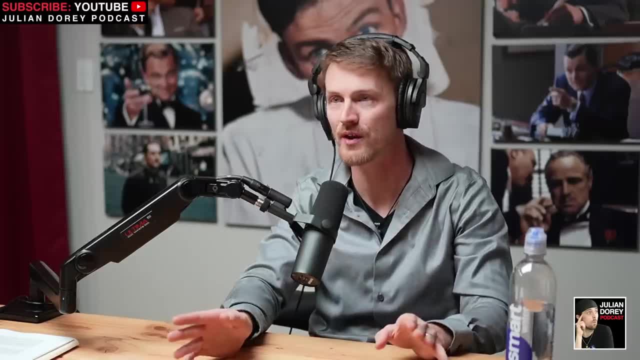 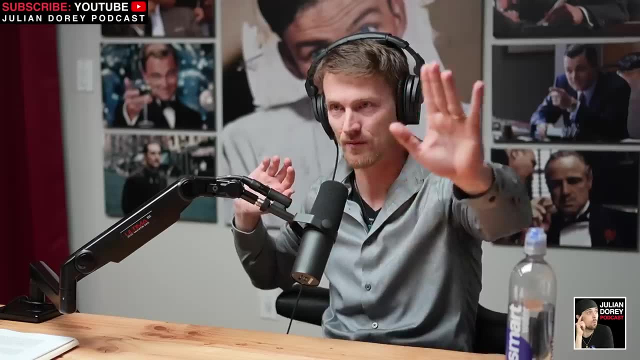 And what they uncovered was, as they came up, they found an ancient road, like a very, very well-made road, And then, when they started excavating, they found these massive basalt megaliths, these walls that were created, that are so precise. 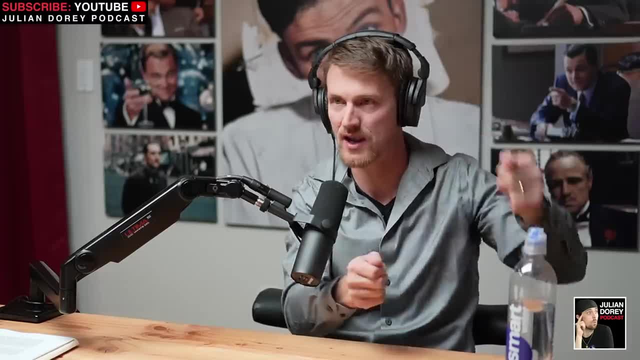 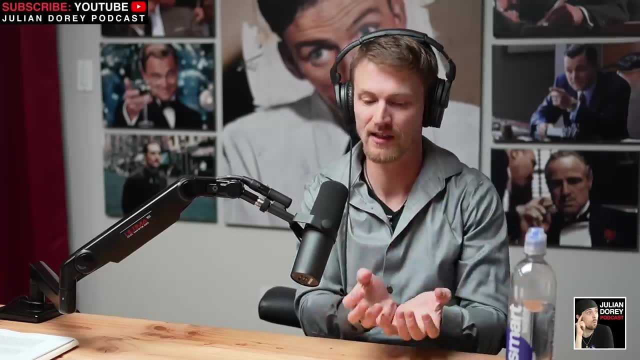 Yeah, That it looks like they were almost cut out of like cookie cutters and just the same. Like if you were at the beach and you had a bucket and you were making a sandcastle and you filled that like a castle-like bucket design, that would make that shape right. 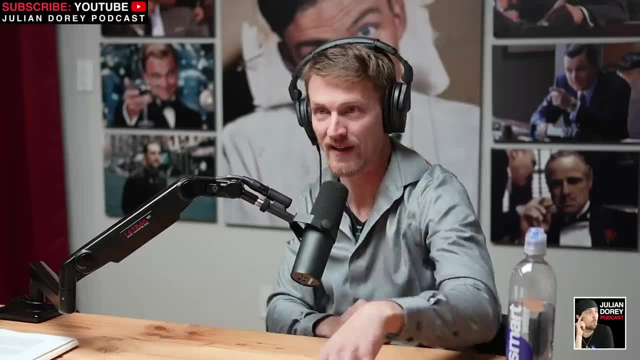 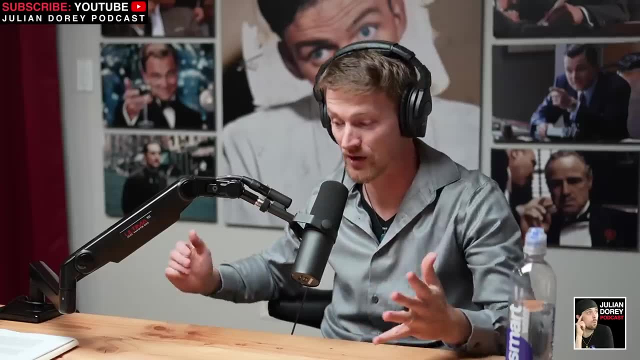 And you filled it with sand and you put it down. you could make the same thing over and over again. that's like identical. That's what it looks like they did When you look at some of the walls that they found as they started going up. Ionis, it's. 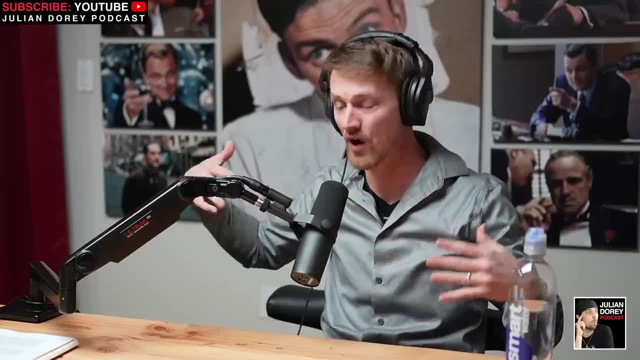 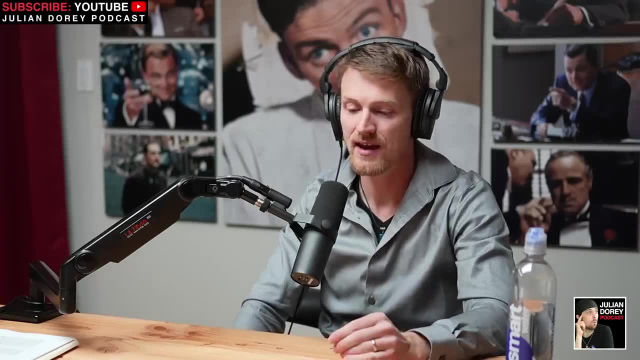 like: how did they build these? like perfect basalt, Very hard stone walls. But what's very obvious- and we'll have an image to show, hopefully, later- is that above it had extremely primitive brickwork- like very, very primitive brickwork, to the point. 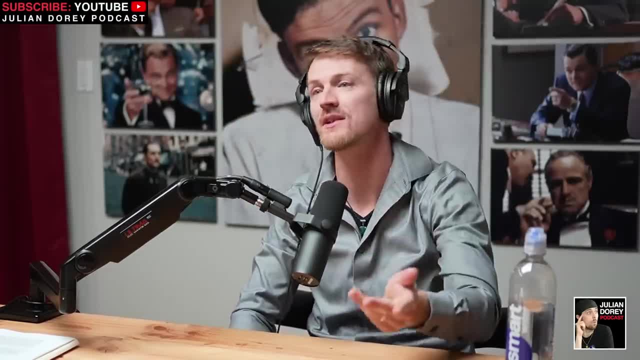 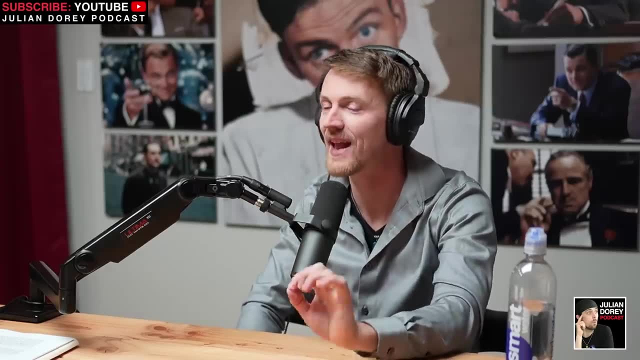 where it had eroded so much that you could almost barely even see the bricks anymore. That's the Urartian civilization. They built exclusively with bricks. They didn't build anything with anything but bricks. How do we know that? Because all of the Urartian civilizations are established based on 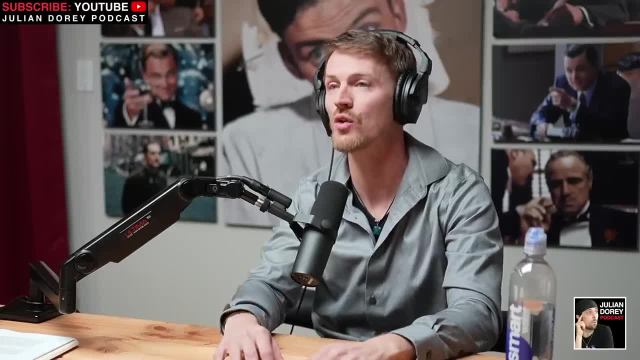 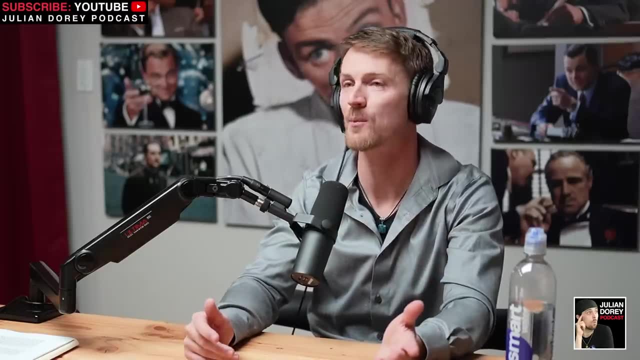 If you have a culture. they have similar mindsets, They have cultural abilities. Like they can only build things to a certain level of sophistication. Artwork is often a way to represent how advanced a culture is, How beautiful the artwork is, the pottery, the things they build is a reflection of how 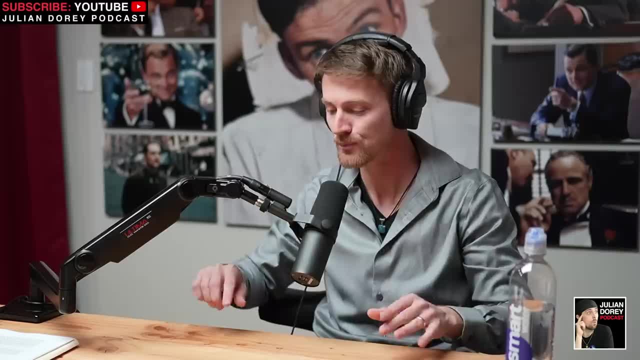 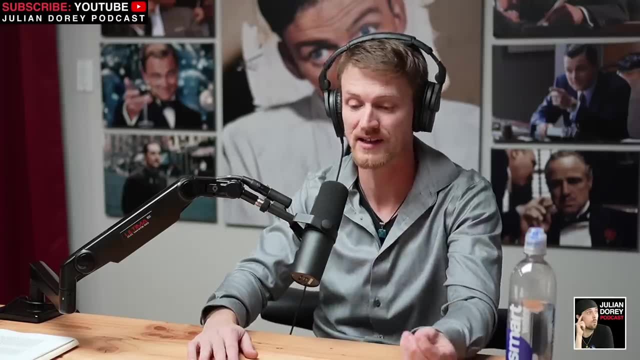 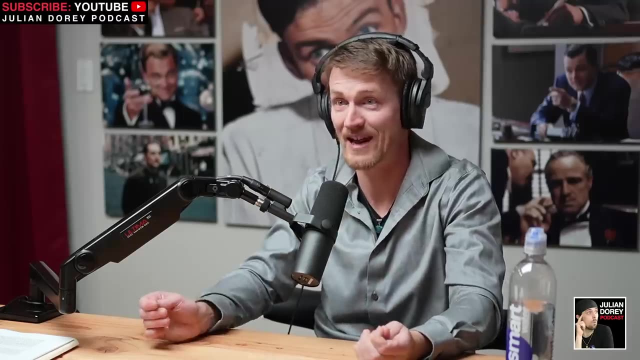 sophisticated that civilization reaches. The Urartian civilization was a warlike civilization that was more of a conquering culture, And a lot of the artifacts and the things they had are not only pretty primitive And compared to what we're talking about, but they literally don't even match in any. 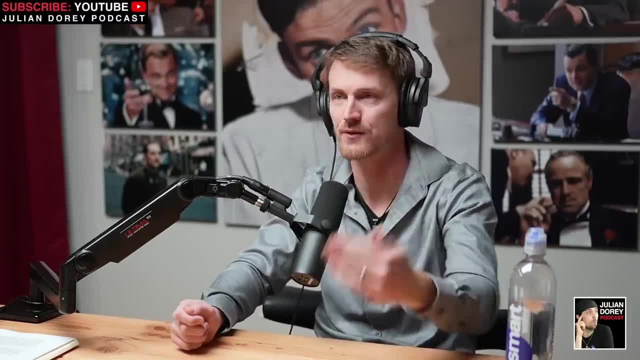 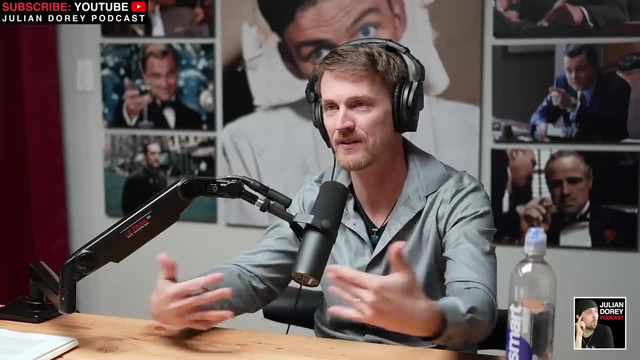 way. It would be like you trying to take artifacts from now and then like matching them up to like the colonial era or something. It doesn't make sense, It's like doesn't come from even the same. it doesn't, it doesn't even relate to each. 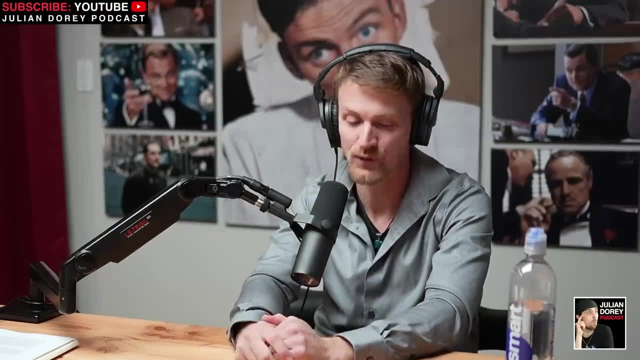 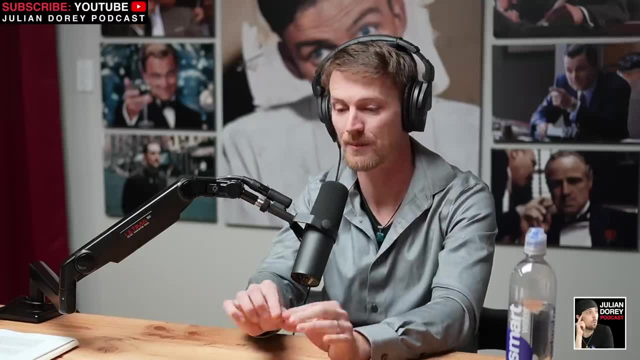 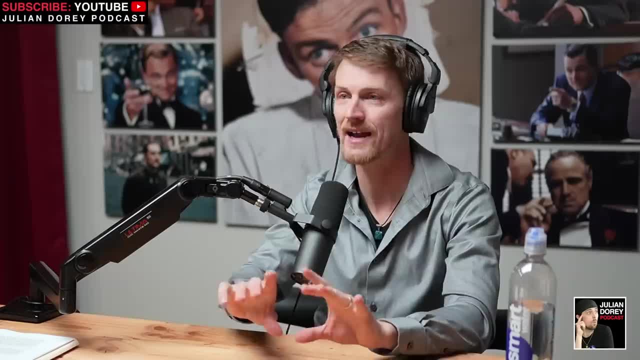 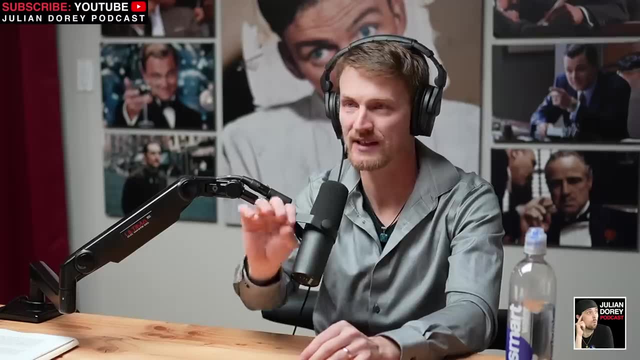 this is a. this is a. these symbols don't realign with the Urartian symbols. This seems highly advanced, seems to emerge at a nowhere. Things like well. previous archeologists that laid the framework believe this symbol means this. 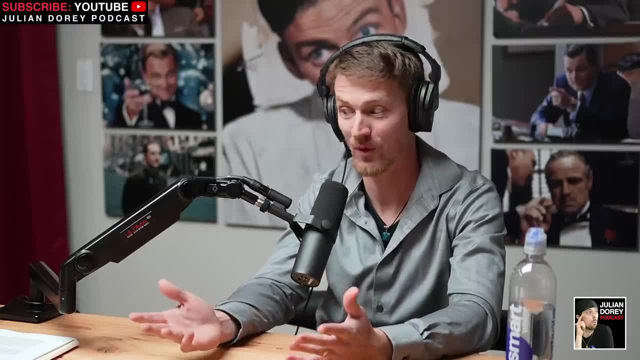 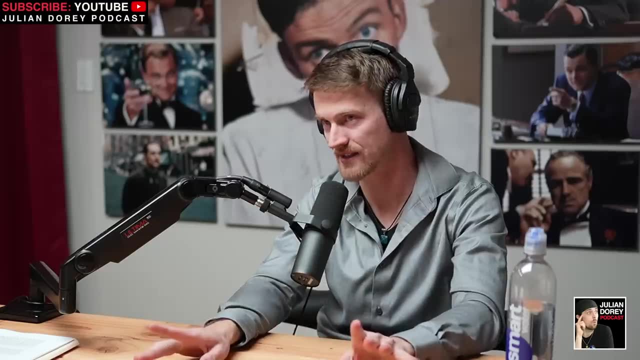 And they- it's so hard for them to say it to- to be like: oh well, I guess it does. They're like: well, it looks just like the tree of life icon. Let me give you an example. This site's called Ionis Khaelesi for the mainstream name. 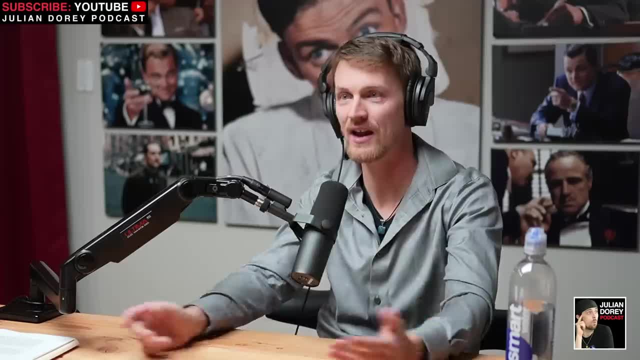 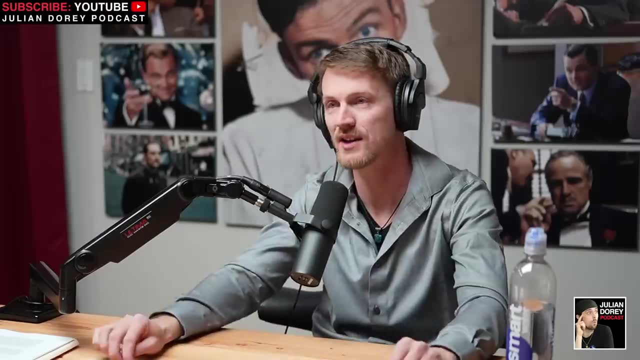 Khaelesi means fortress, just never a fortress. Yeah, That automatically gives the wrong purpose of the site in the first place, because they're looking at it through the lens of the Urartian civilization, which was building castles and was warlike. okay, 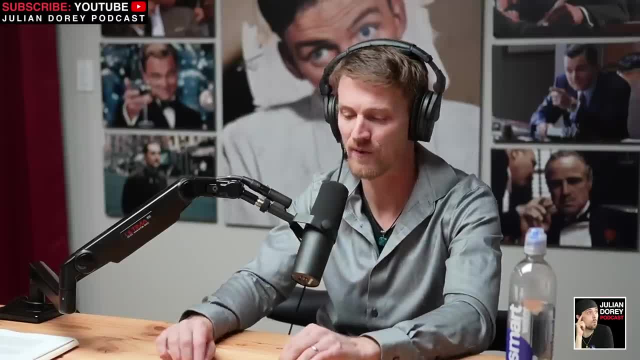 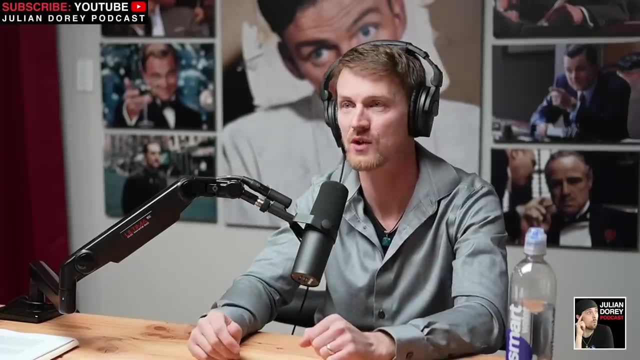 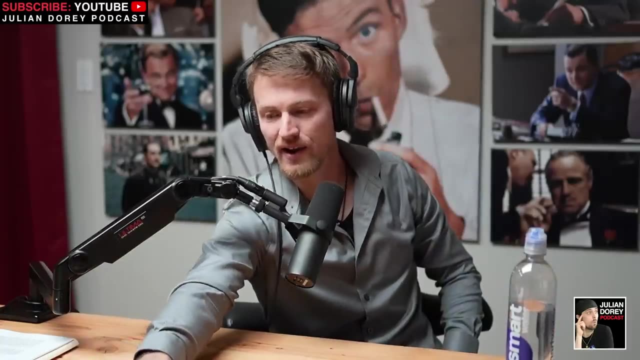 Did. they conquer a lot of people. They conquered the region. They had some wars, But the point is, in one of these depictions it's showing this god Haldi that was part of this: creating the civilization and passing all this knowledge. It's showing him passing a pine cone in his hand. 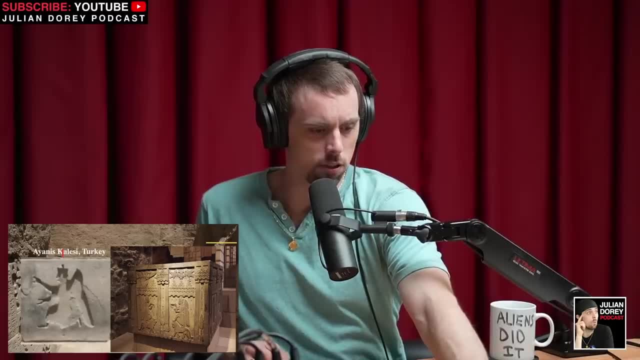 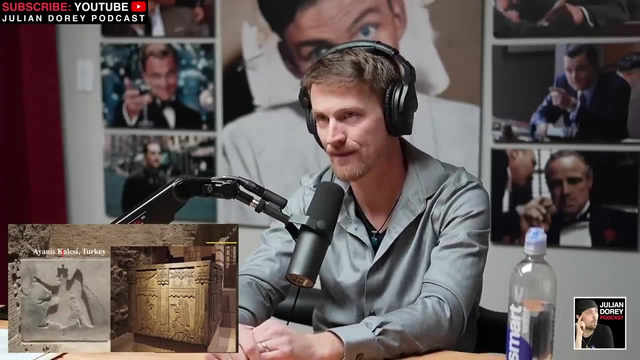 All right. so this is another – Right, This is – what's the term for this thing. This – what I'm describing right now, and we'll put a picture up, is a giant box relief that came from a place called Kef Temple, which is on the opposite side of the lake as Ionis. 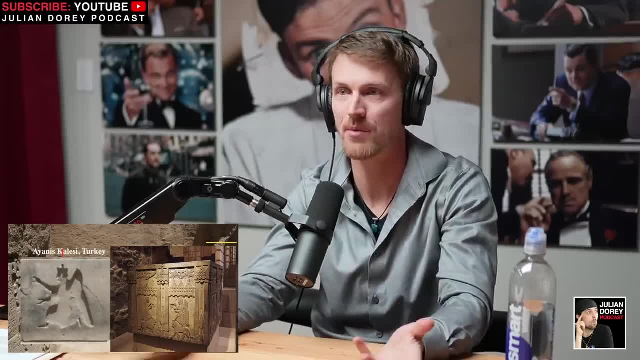 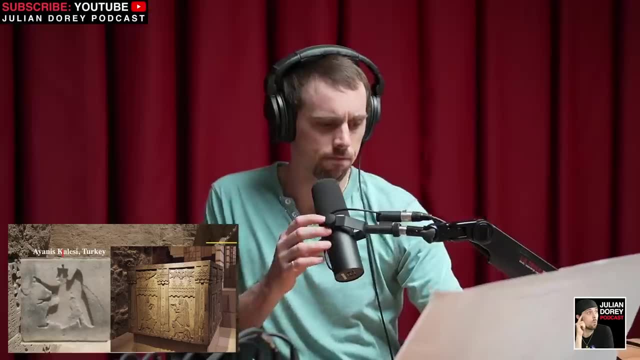 A box relief. Box relief meaning that there's nothing. There's nothing inside. It's symbolic. but it's a gigantic three-by-three-by-three-by-four-foot basalt box that has some of the most finely intricate carvings of like any ancient structure I've ever seen in the world. 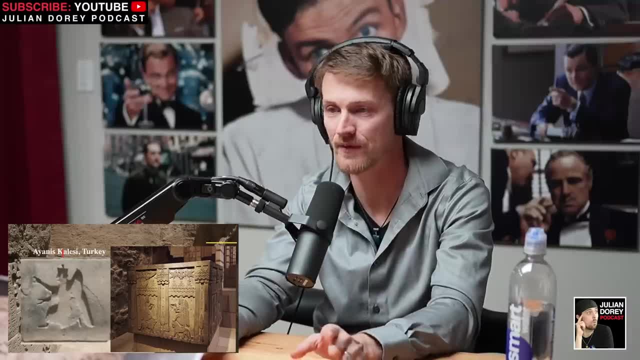 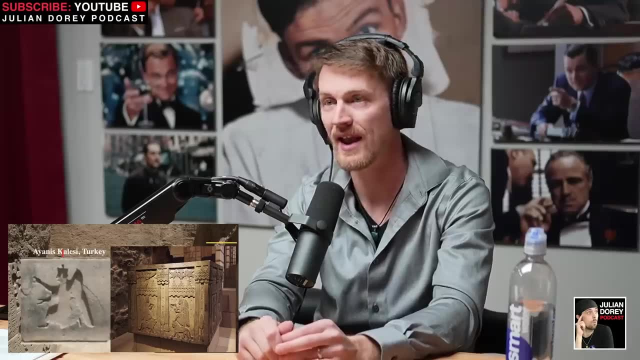 The symbolism on this is insane, Unbelievable, right Yeah, And we could talk about that until the end of the whole show. but the point is, look at what Haldi's holding in his hand: Pine cone. He's passing the pine cone and it's coming out of the cup like the ancient chalice. 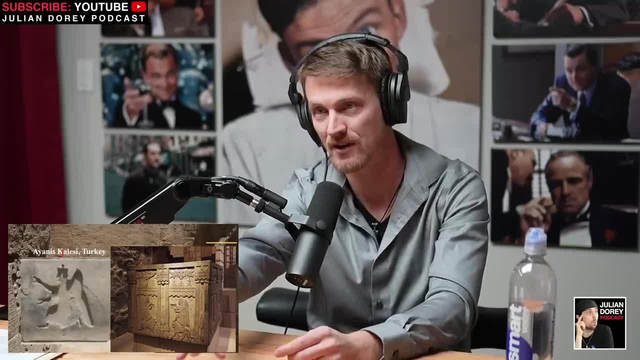 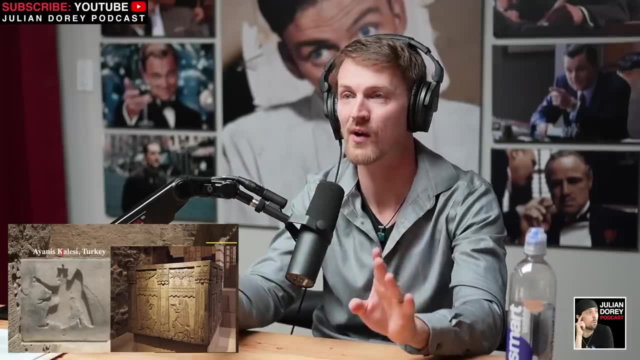 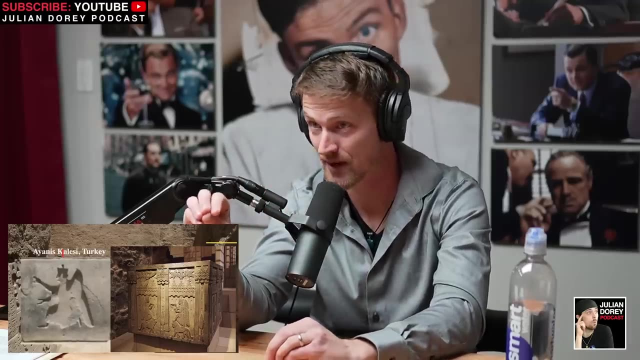 Now that pine cone looks exactly like the Tree of Life in the lower depiction. Now the archaeologists in the actual sites from Kef that found this box relief, they go – and I'm paraphrasing There's something like – the object that he's passing, Haldi, looks extremely similar to the Tree of Life icon on the box relief. 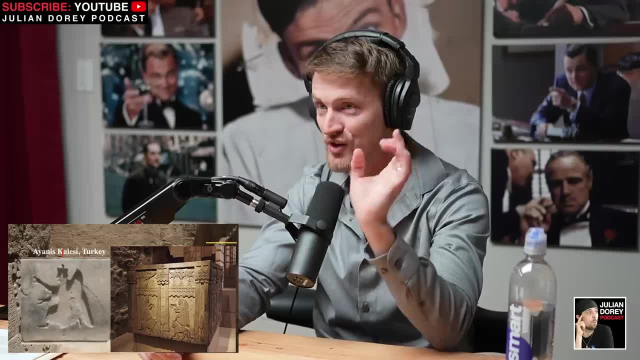 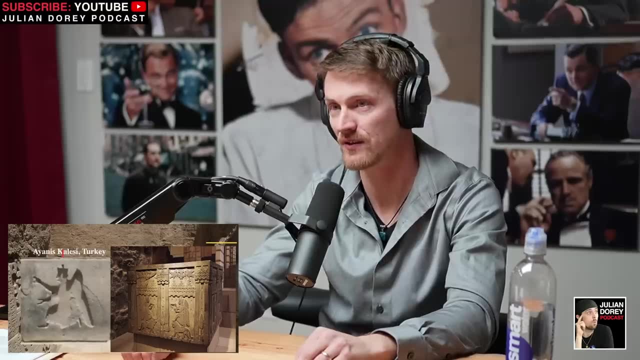 However, other archaeologists have already determined that it is a spear, So they're looking at it through the lens of this warlike Urartian civilization. Right, And that's a tree of passing the seeds of knowledge and showing the Tree of Life icon. 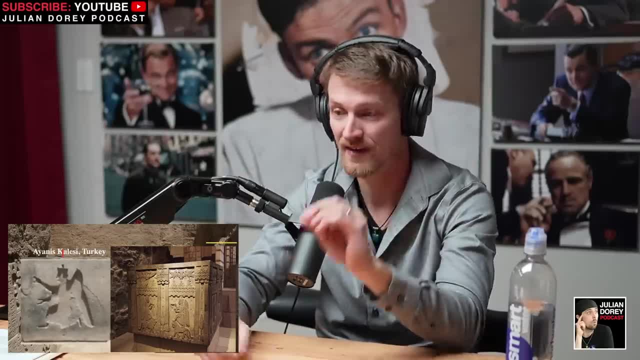 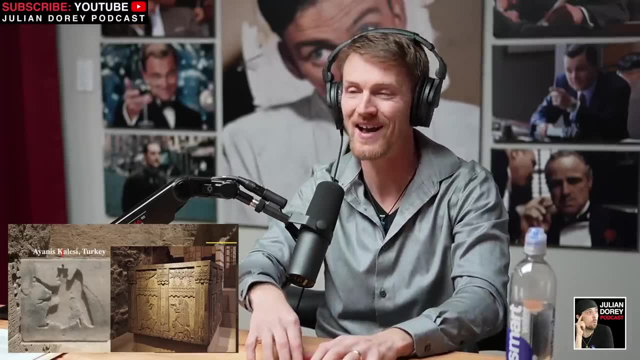 They're looking at it through a warlike empire and they say it's a spear. Does that look like he's holding a spear in his hand, like a warlike spear? No, And that's the thing is. the archaeologists in the papers are like: well, it doesn't really look like that, but it's supposed to be like that. 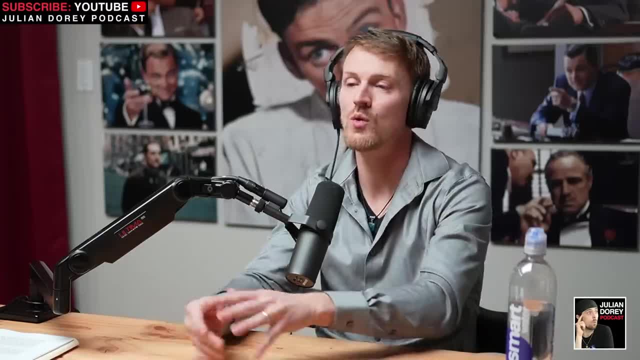 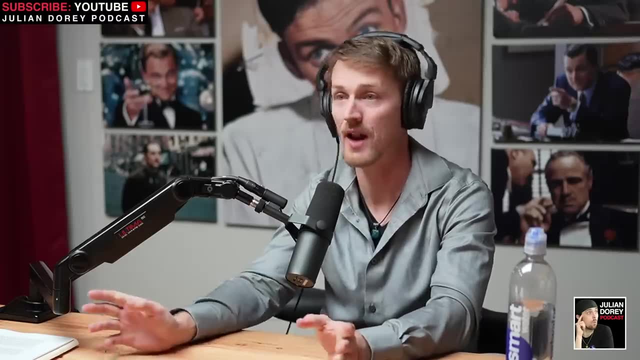 Why would you think that's a spear? Would you want to step on the foot of giants? I mean by giants? Imagine you are an archaeologist And you've spent a lot of money getting your credentials and you go out to study and you're excited. 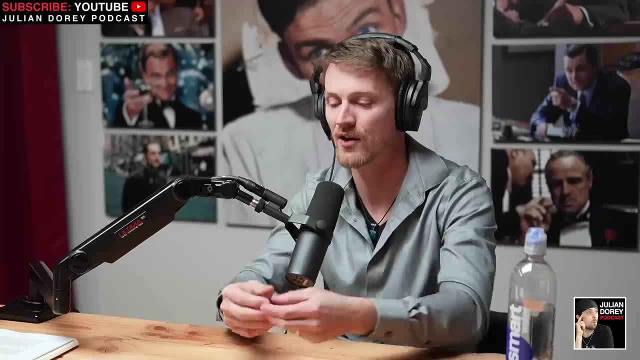 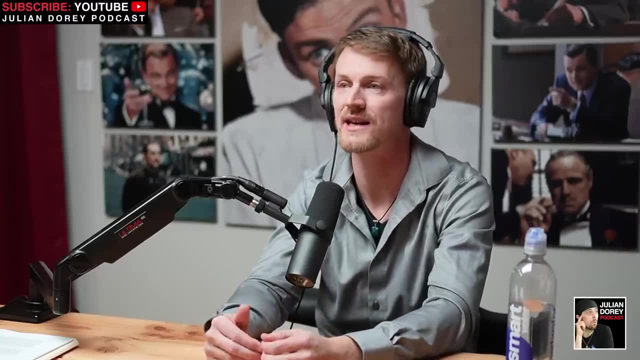 Well, you've spent a lot of your life – typically, an archaeologist, just to back up, is an expert on a certain region. They're not just like an archaeologist for the whole world, right? You'd have an archaeologist that would focus on, say, Turkey, right? 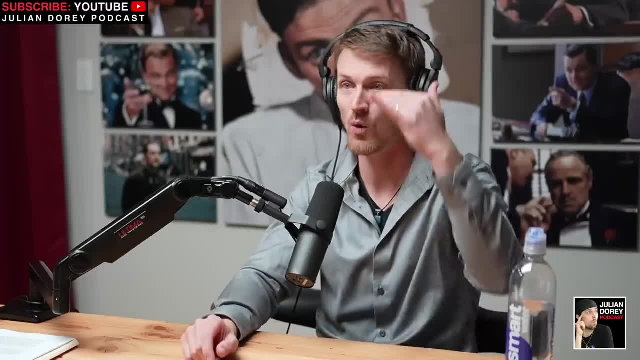 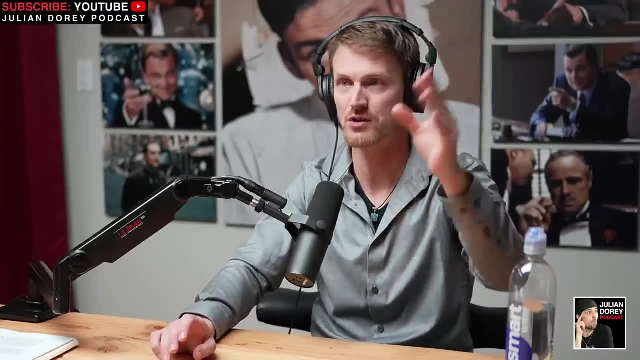 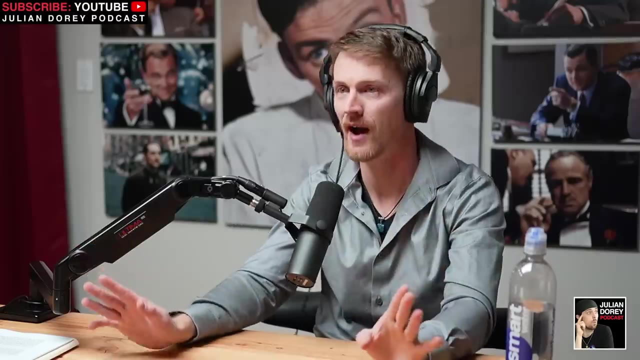 Maybe the Anatolia civilization or something. Well, they would base all of their study on those who came before them. They would be like, well, Mr Schmidt, Or something highly credited ancient Turkish archaeologists who was like the father behind Turkish archaeology. 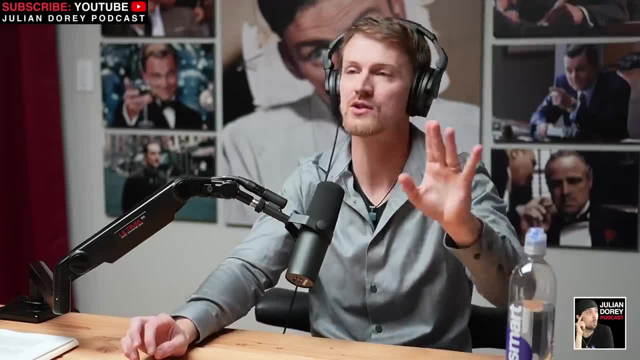 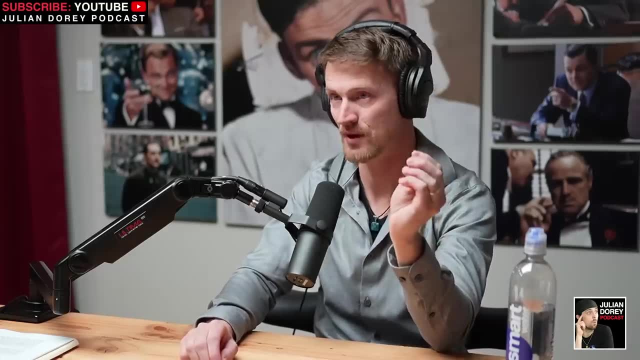 And he – what a great man. Like they laid the foundation, They really discussed the Urartian civilization and they really mapped out all of this right And they have all this praise and they really look up to these key archaeologists that come before them. 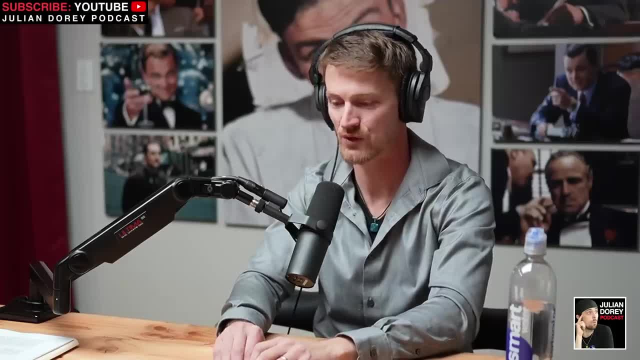 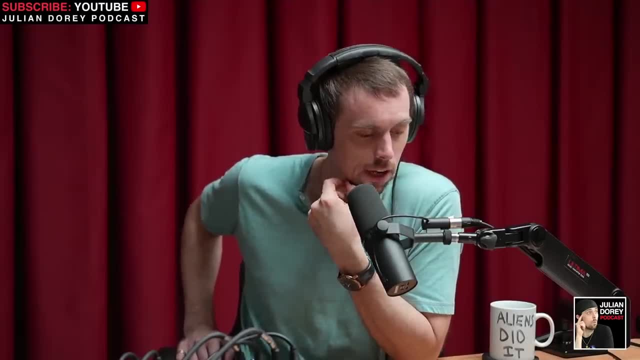 Do you really think that you're going to come along and disregard and change every theory they had? Yeah, but that's the problem. That's what we're looking at here, Because if you're dumb enough to look at that and say that's a spear, I mean I'm not – I'm the farthest thing from an archaeologist. 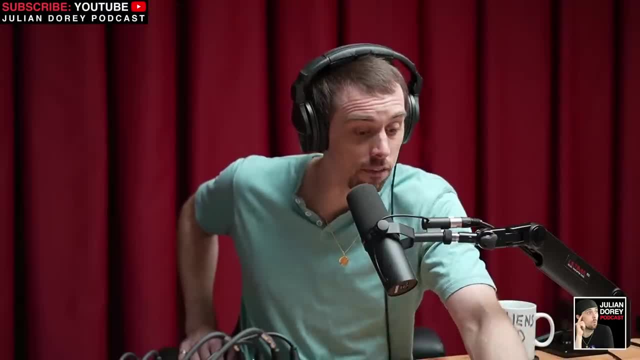 Right, and that's the problem Exactly. Look, I'm not even – maybe it's not a pine cone, That ain't a spear though, But look at this. Look at how similar that is to the cypress tree of life they have in the corner. 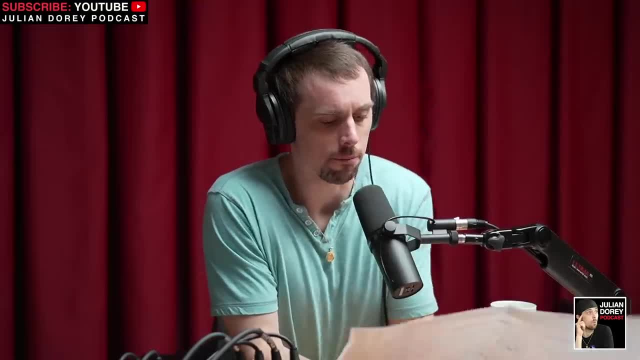 You see that Now actually hold on one sec. Let's play devil's advocate, Okay, okay, Because I – to me that's not what I think when I see this. I don't think spear, Of course not. 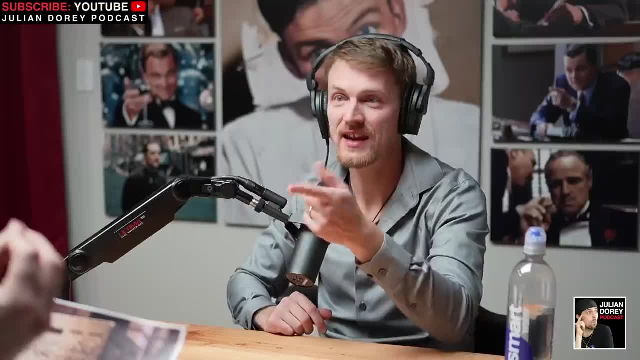 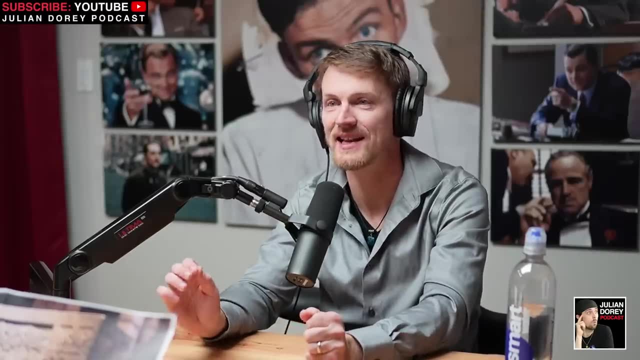 I'm trying to say it is the tip. The tip is the end of an arrow. Yes, Without – Exactly Now, that's possible, But it looks like – but they even mention in the paper that it's identical to the tree of life cypress that's shown in the depiction. 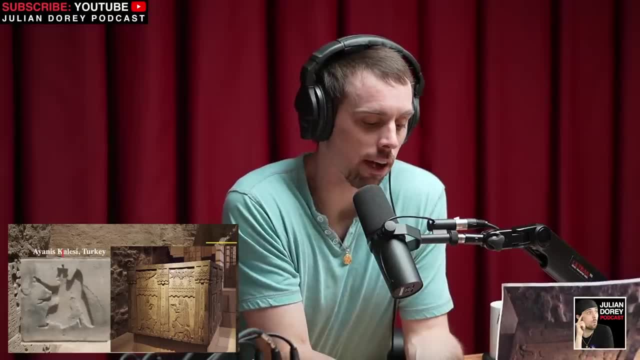 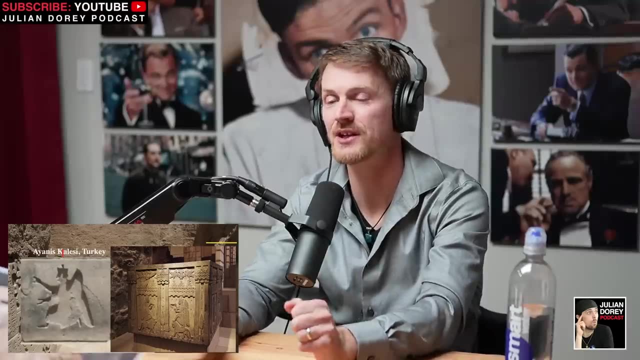 You see that Now, and so are you saying: the archaeologists concede that this is the tree of life. cypress, Yes, yes, So the tree of life – Yeah, that's hard. The depiction of the tree of life changes depending on where you are in the region. They actually pick a tree of life based on some kind of tree that's symbolic for them. Cypress grew in the region, So they used that for their tree of life, whereas, like for ancient Mesopotamia, they didn't use a cedar. 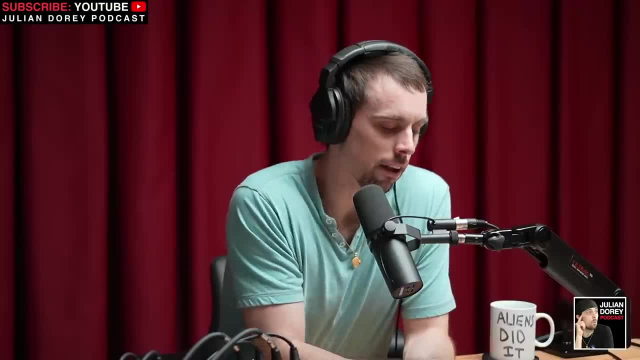 They had, like a willow, I think was their tree of life. So that would be a hell of a coincidence, because even the design would like the lining down the middle. It's identical, It's very – It's exactly the same thing. 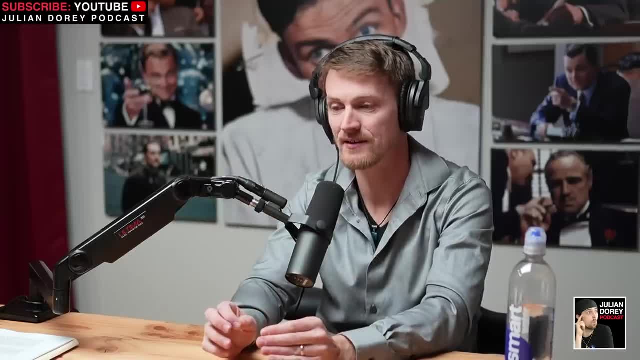 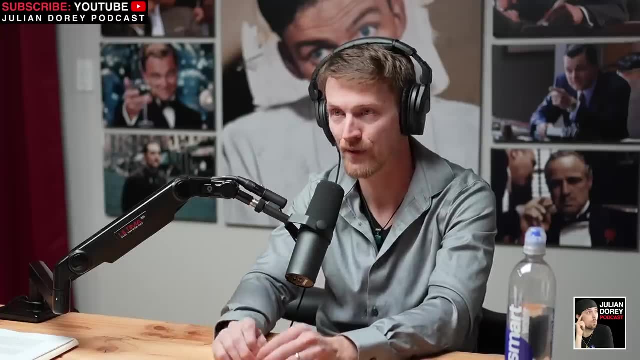 It's damn near identical. But if you for a minute realize that clearly that's not a spearhead, okay, Clearly it's not a spearhead. It shows you that the entire framework for how they're viewing these discoveries is completely – It's completely wrong in my opinion. 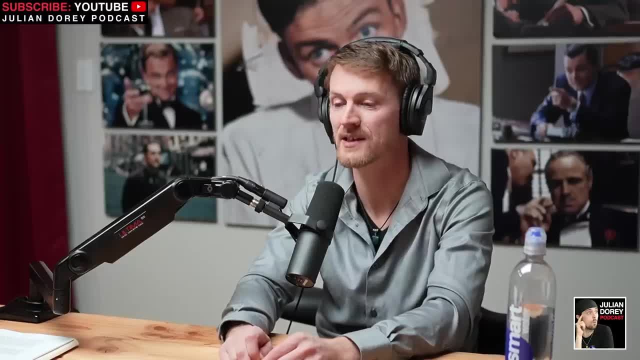 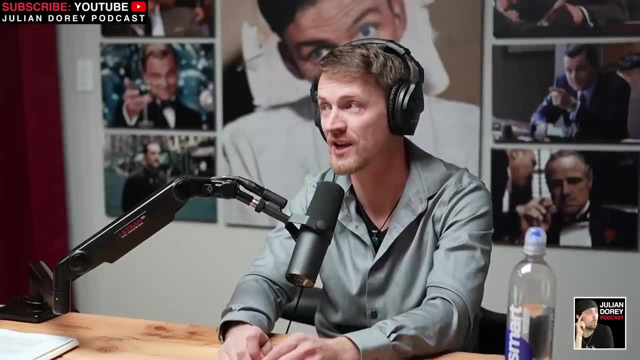 Why do they have wings? Wings signifies someone not being human. Wings signifies something like a divine being Okay. Wings are always shown like on an angel, like in – even in Christianity as like an archangel. It's like some kind of divine, like almost like demi-like human. 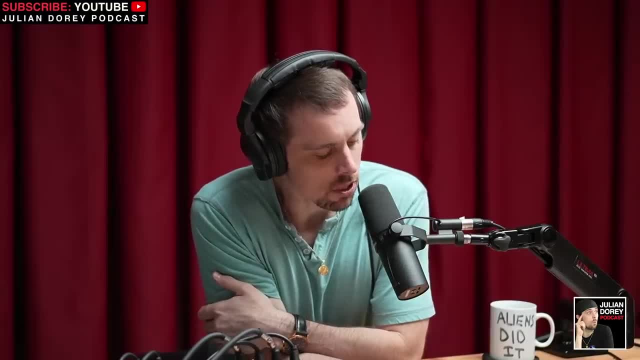 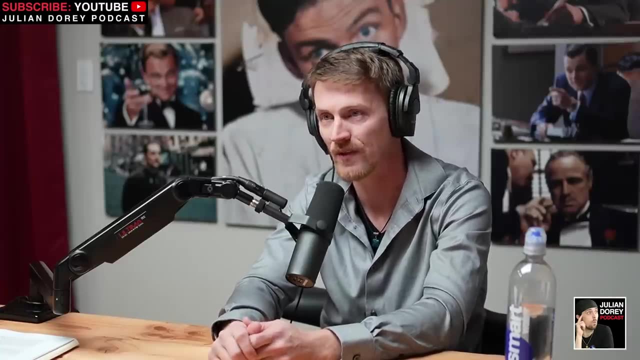 And why are they standing in the same stance? It's not two people, It's one. So most of what we see in these ancient depictions is symbolic. It's not really literal, It's a mirror. Yeah, exactly, And what it's representing is the totality of each side, the totality of all. 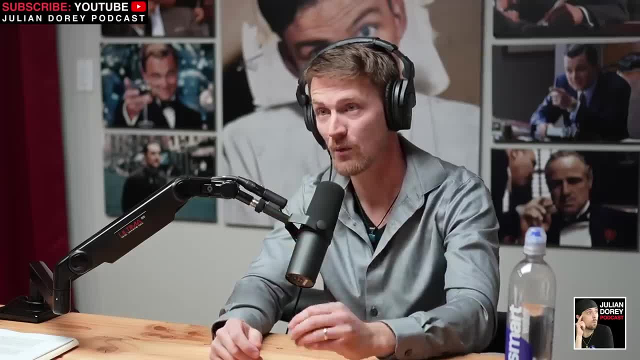 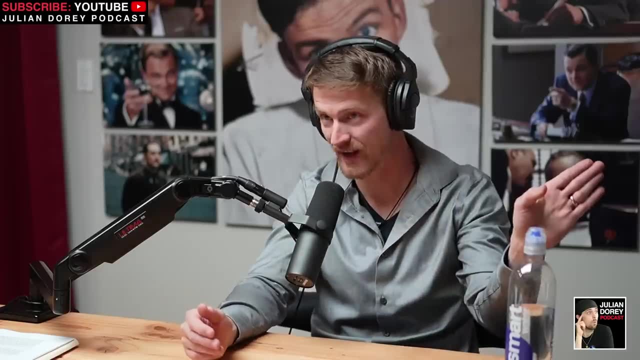 So, if you have – for instance, even the Holy Roman Empire did this. When they converted to the Holy Roman Empire as a war empire, they chose the Byzantine double eagle: an eagle facing the left and an eagle facing the right, showing the totality of knowing all. 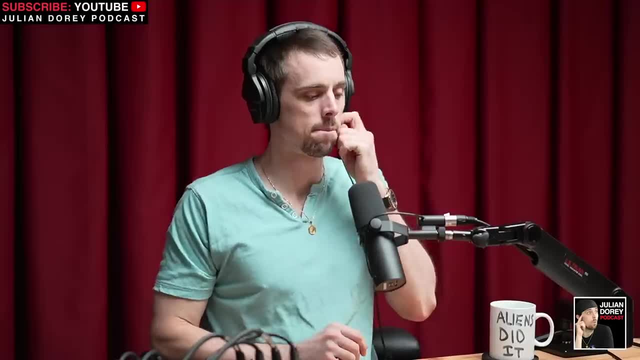 basically being aware of all and commanding and controlling over all, But this isn't about war. This is completely nothing related to war in any of these. This is completely nothing related to war in any of these. This is completely nothing related to war in any of these. Which is why it's so sad that not only is that location where that box was found called Kef Kalesi, but Ionis is called Ionis Kalesi. Remember that means fortress. It's ridiculous Like you're already labeling it with the wrong purpose with the name itself, which is similar to why –. 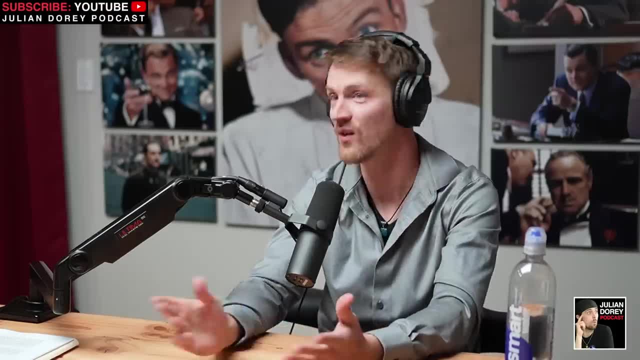 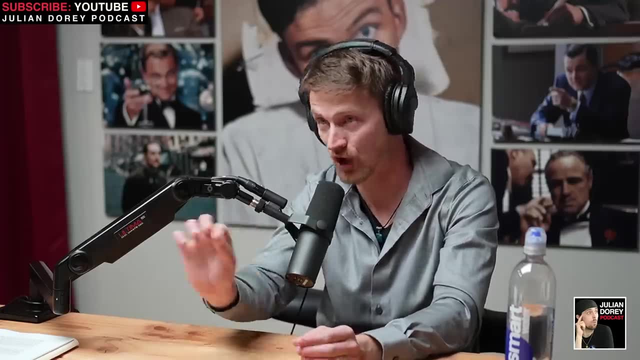 like, for instance, Khufu's pyramid. That's not Khufu. He never had nothing to do with building that pyramid. They never found any evidence that he was buried there. Not only that, but the name, the cartouche name, that was found. 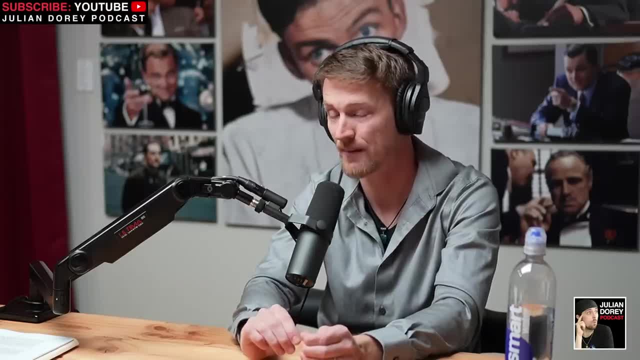 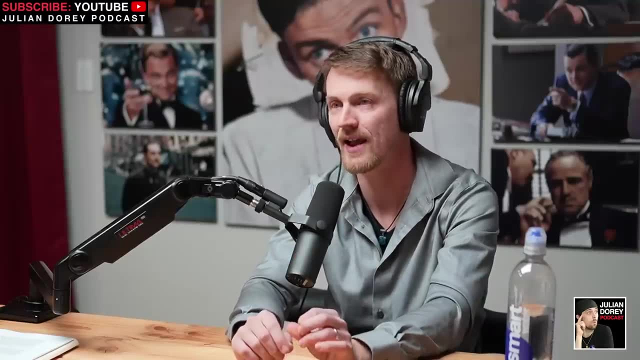 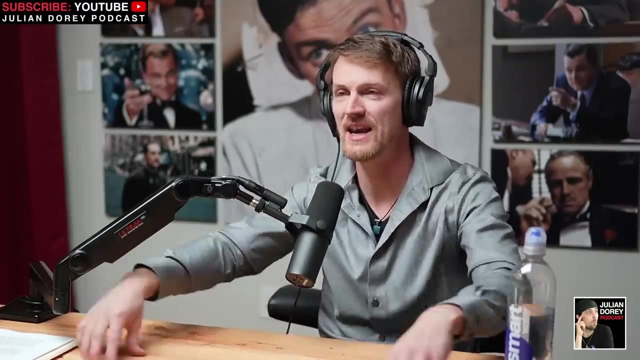 supposedly in the 1800s, was a lot of people have looked into and they believe it's complete fabrication. Why do they believe it's fabrication? Because the individual – and I don't remember the name of the individual off my head, but there was interest in history at that – already at that time being a certain lumped in like a version. 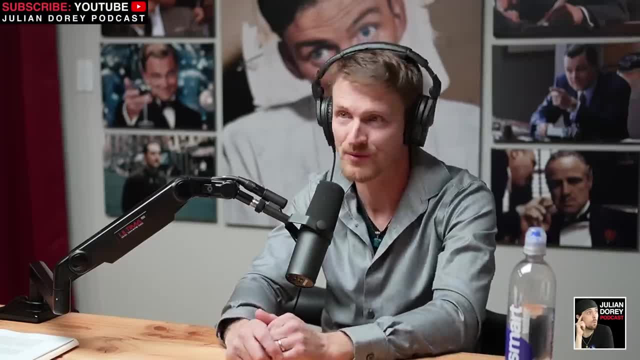 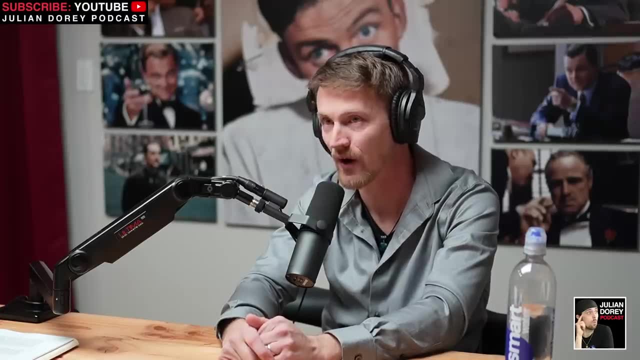 and it was already being established And there was real problems. if it's not Khufu's pyramid, because then why were the pyramids built if they had nothing to do with the dynasties, If they had nothing to do with the dynastic pharaohs, nothing to do with them? 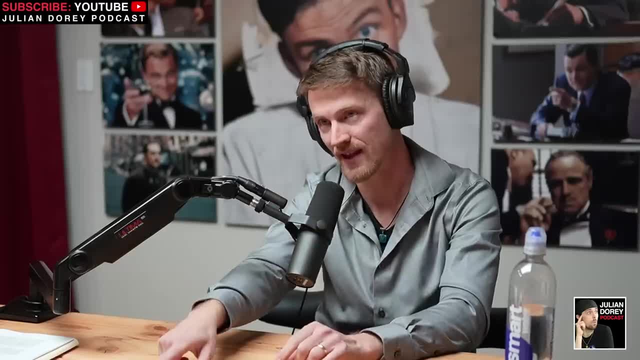 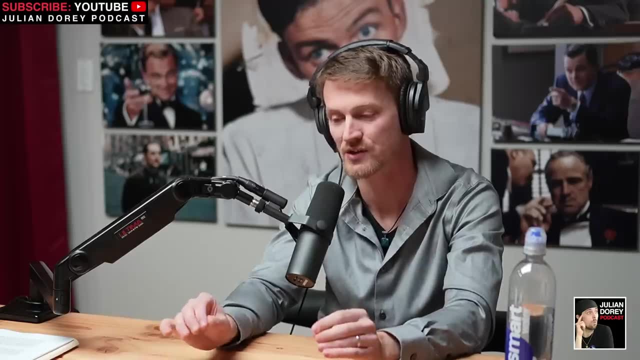 Put a pin in the pyramids. We're going to come back to that, But it's the same thing with this. These weren't – like these weren't – this is why ancient history – this is what history – this isn't ancient history. 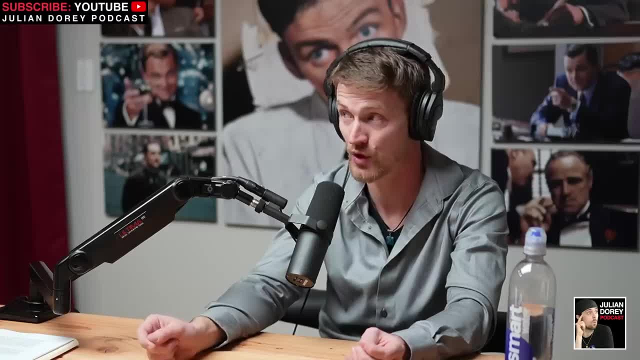 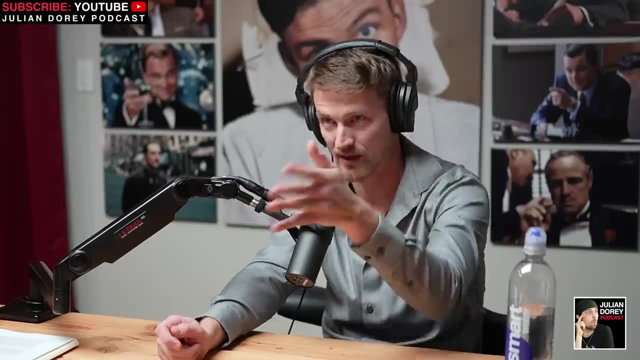 This is what mainstream history tends to do: They'll label something, either a tomb or often a fortress, And it – like giving you an example, Saskia Oman. and we're going to talk more about South America, but Saskia Oman is a perfect example of that. 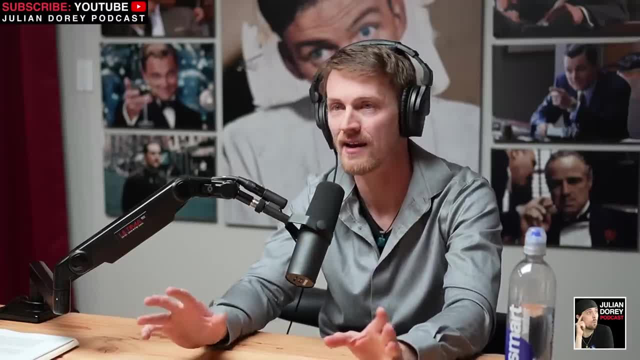 Saskia, Oman, is some of the – It's one of the largest megaliths, some of the most precise design of any ancient temple in the world site, And yet they say it was built for a fortification. Where did you say that was? 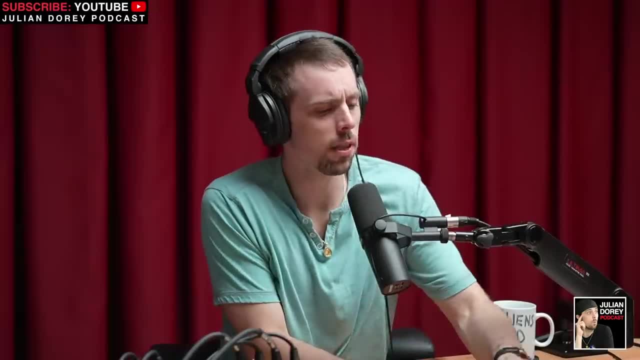 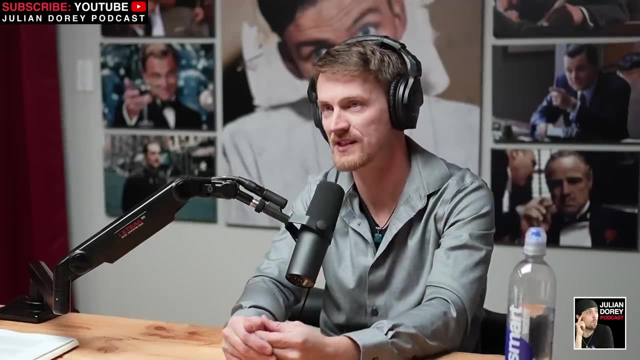 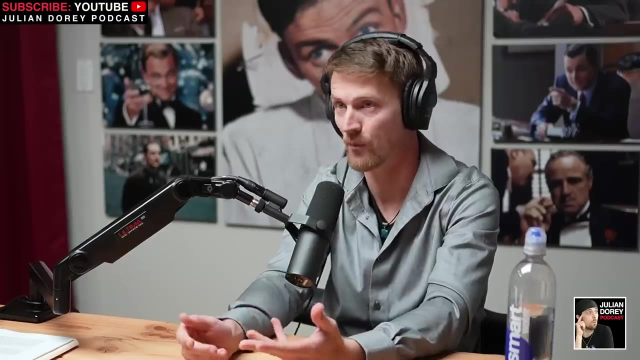 Saskia Oman is in Peru. OK, Oh, were you showing me that picture? That was Oye Tatambo, It's similar. But the point is, when mainstream history labels these things as being the wrong function, the wrong person, who built it, all of these things, it takes away completely from why it was built. 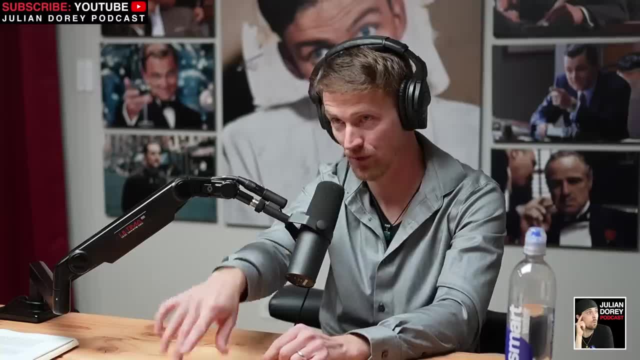 who built it and the purpose of why it was, And that's very much the problem here. And so when I say I've discovered a civilization, yeah, we're going to have boots on the ground soon And I'll talk about that. 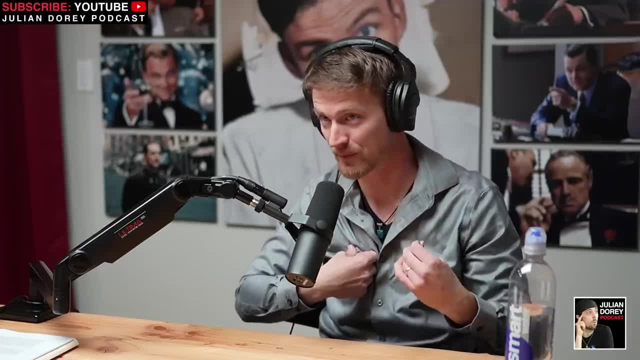 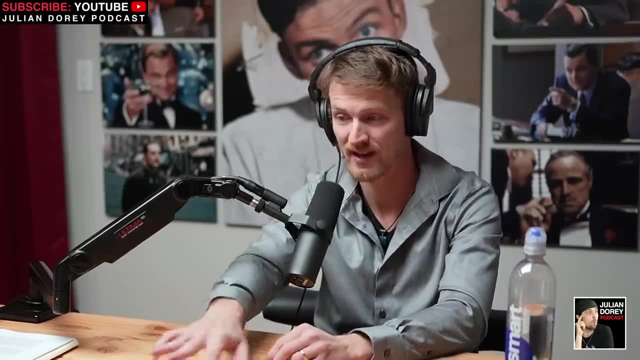 But I've done as much as I can from the computer. Now it's time to get on the ground and actually make real claims based on being there, And we are going to do that. But the point is that – You're putting a team together. 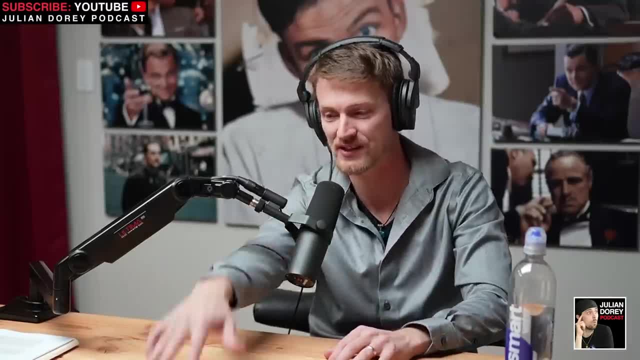 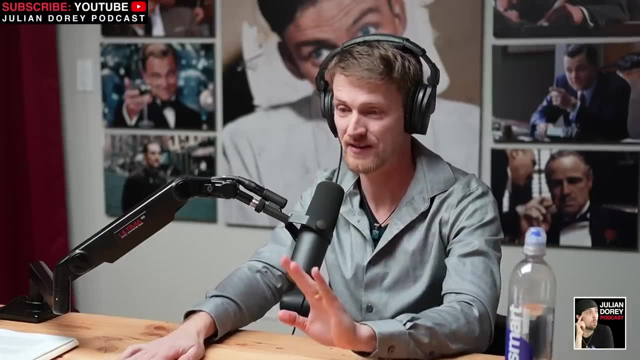 Yeah, So I guess I'll mention that. So this discovery is with Kef, Kavis Tepe and then especially Ionis. And we haven't even talked about Ionis yet, Because I truly believe that that site may change all of history in the future. We look at pilgrimage sites today, like Mecca, right or Jerusalem, and they're considered very, very sacred places to a lot of religions. right, I think in the future, Ionis will be one of the most sacred sites in the world. 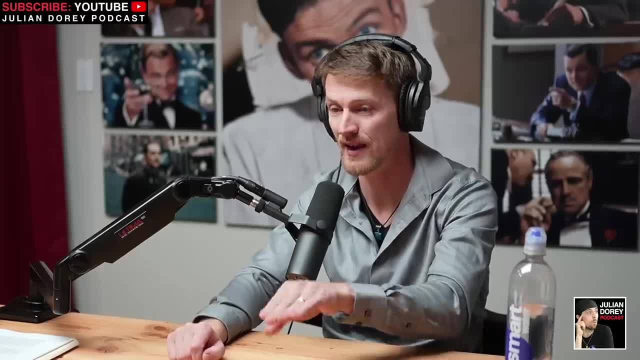 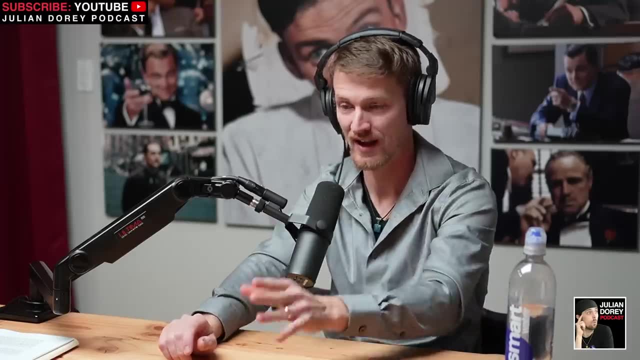 that will be visited by millions of people because of the implications for the symbols and the teachings and what is contained at that site. Imagine, if it is true, And I believe this, that Ionis Temple – and I mean there are places in Sumer like Eridu. 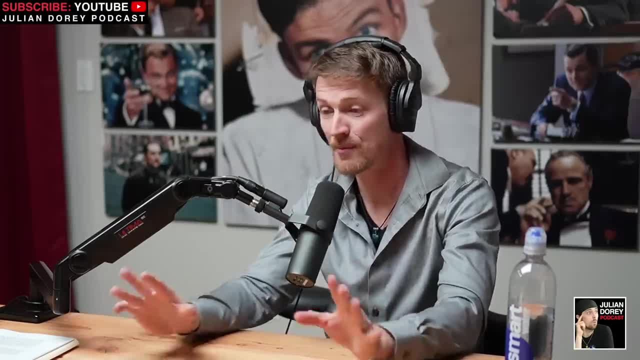 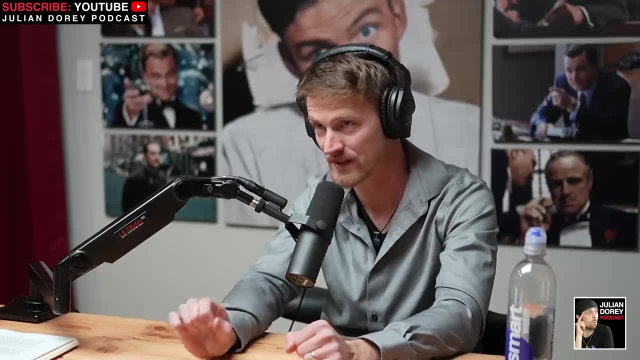 and others that are all disintegrated and there's not much left of them, But in terms of an intact place that still exists, that you can see, I believe that Ionis is the oldest – maybe the oldest temple on earth. Okay, And that is why – 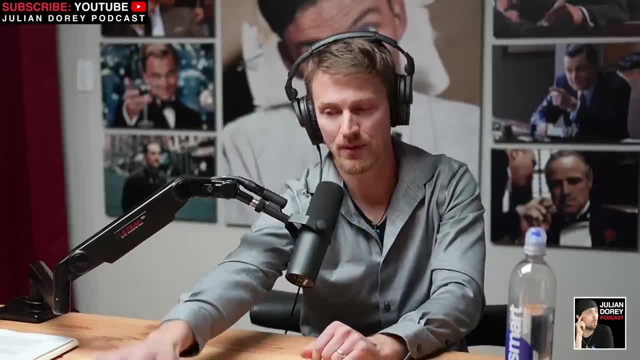 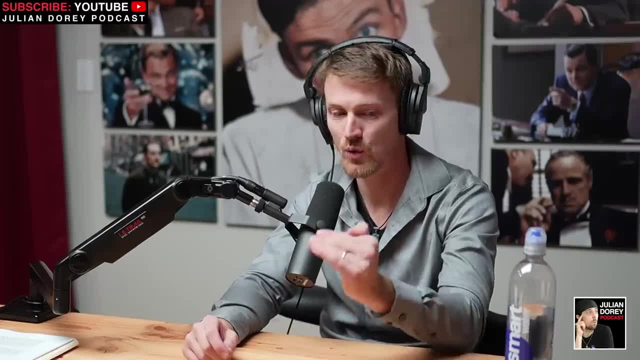 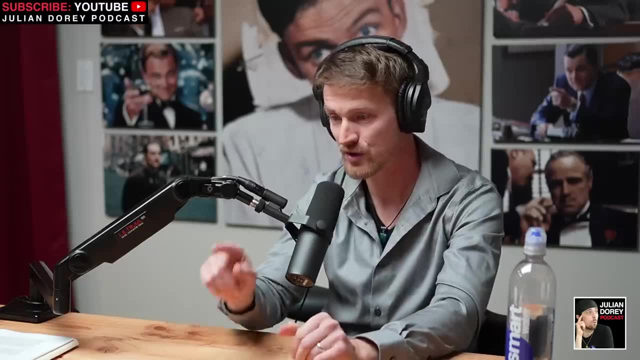 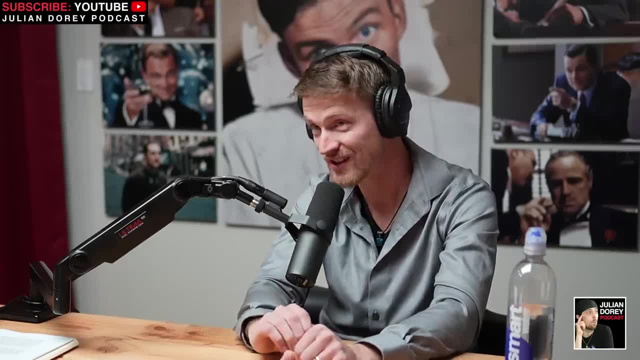 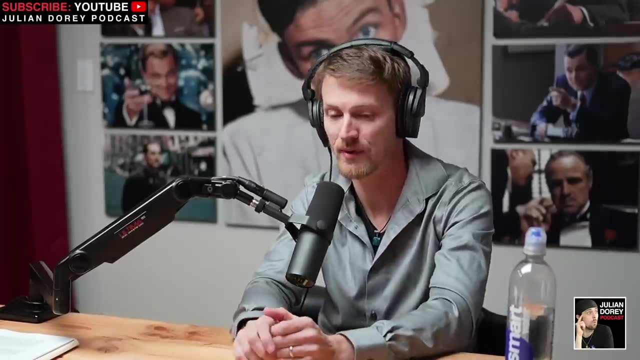 right now that is approaching half a million dollars, Oh wow. To go with experts in their fields in every angle, to be able to come at this from an archaeological adventure standpoint, to take all these theories and then go and make a film. 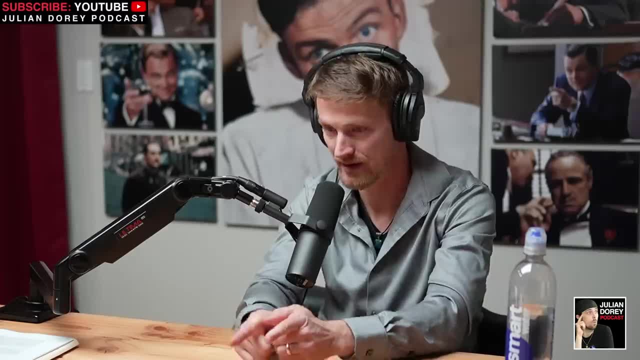 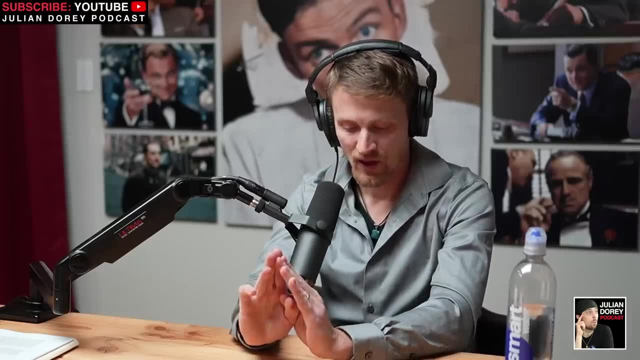 Yeah, To go with experts and then go and make a film and truly show the world what I've found here. Can we walk through this? Yeah, absolutely, Absolutely. Let's do it. So that film is gonna be part of experts like such as I just wanna mention, Paul Wallace. 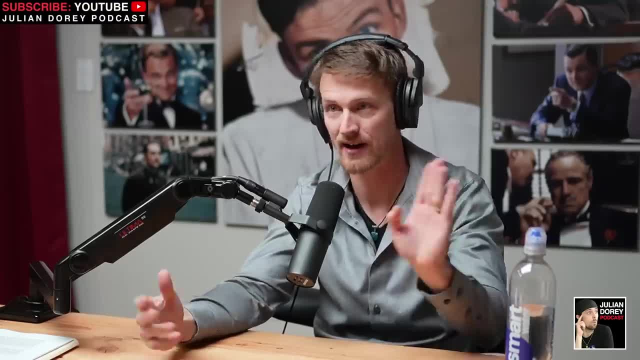 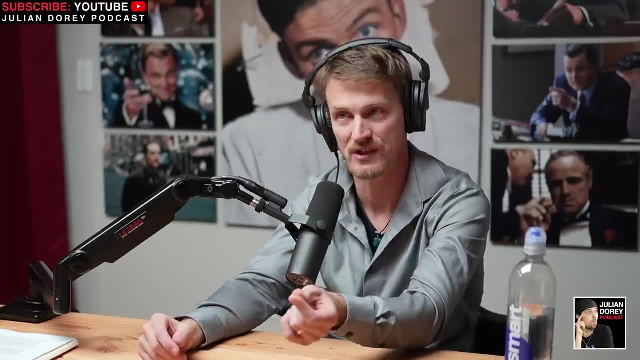 for instance, is a biblical archdeacon in his past, not any longer. He's now an ancient history researcher. But having someone with a biblical background is important here, because we're gonna be talking a lot about religious symbols here And, of course, if you're gonna make statements that are bold, you need to have someone with. 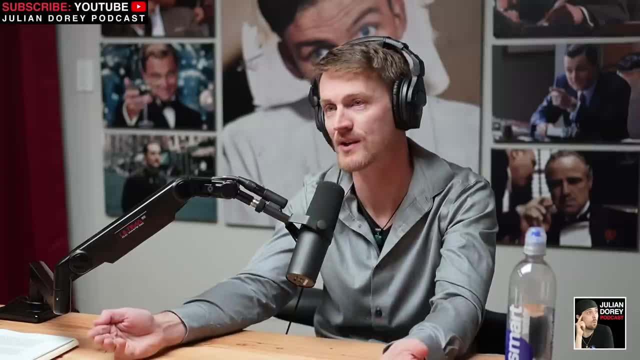 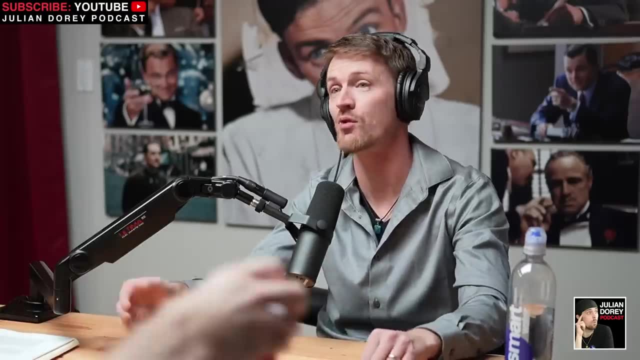 a religious background, have someone with a religious background to be able to back those up. right- And that's the goal with this project- is we want to have someone with expertise in every area. For instance, Brian Forrester is involved, who's a megalithic expert along with me, so we can help use that. 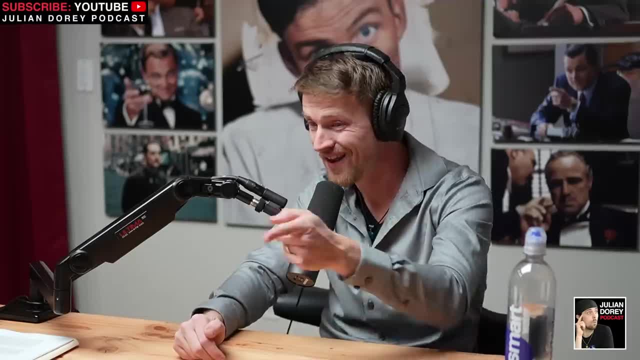 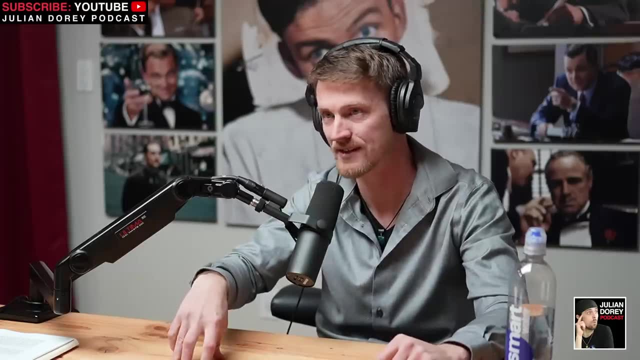 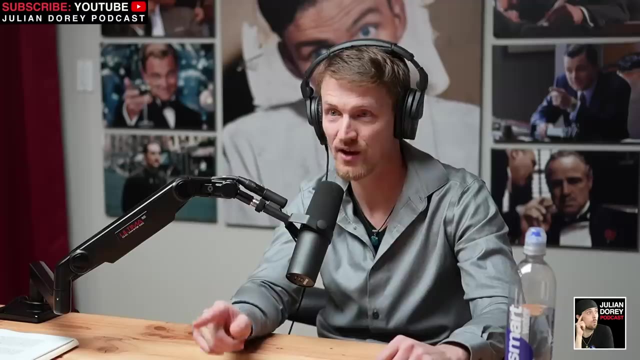 academic understanding. to prove well, you say like. well, ionis is built out of what's called andesite. okay, Well, andesite, on the Mohs hardness scale, 10 being the hardest diamond, is a 7, meaning it's one of the hardest stones on the planet. So how did any culture possibly? 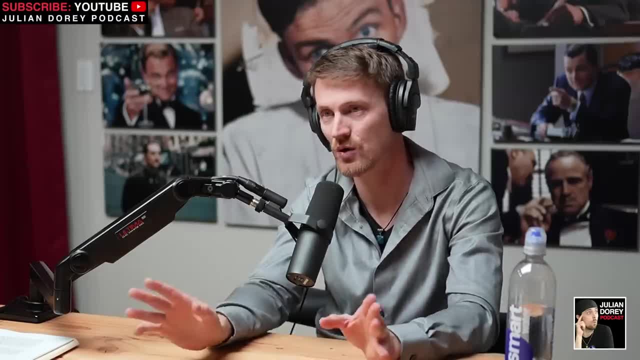 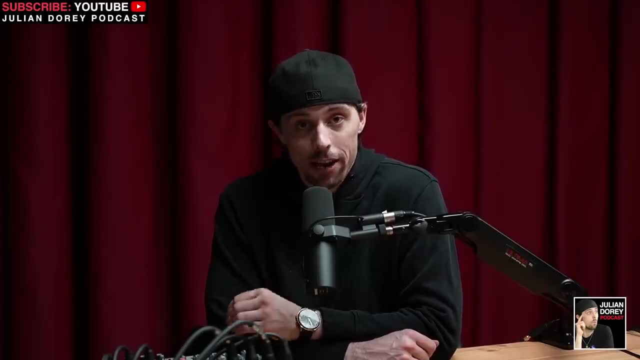 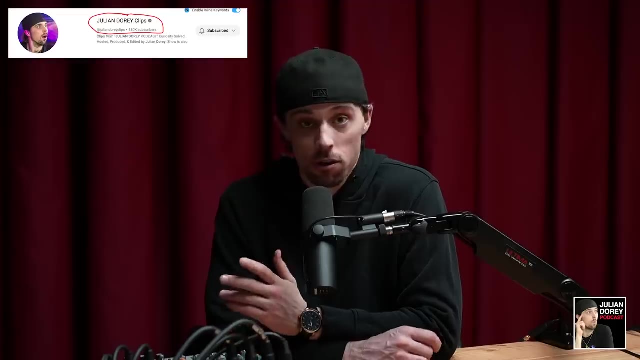 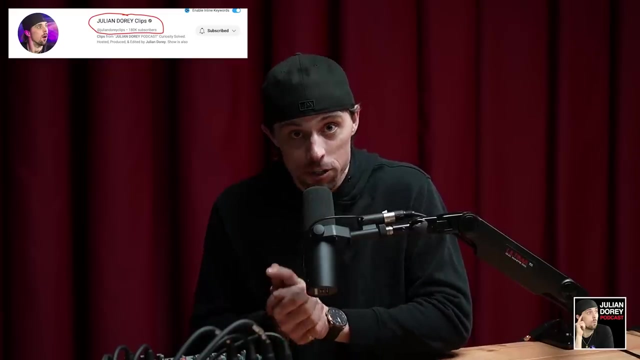 create such intricately created symbols in stone like that. It doesn't make any sense single day and it is huge to help us in the algorithm when those clips do well. So please go over there and subscribe. The link is in the description. The second page is at Julian Dory. 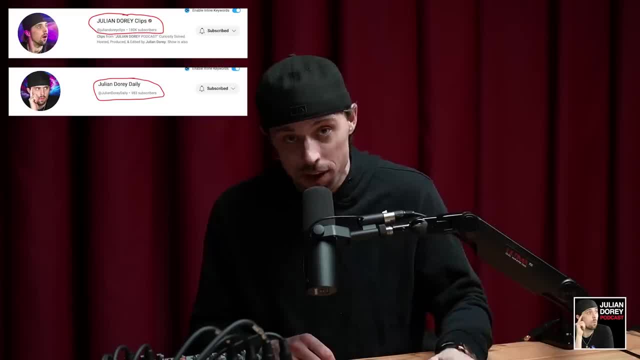 Daily, which is a brand new page with different editors posting exclusive content that is also mid-form and short-form clips. That link is in the description. And finally, we have a page called Best of JDP, which we put on ice for a while but we just hired another editor to bring back It is. 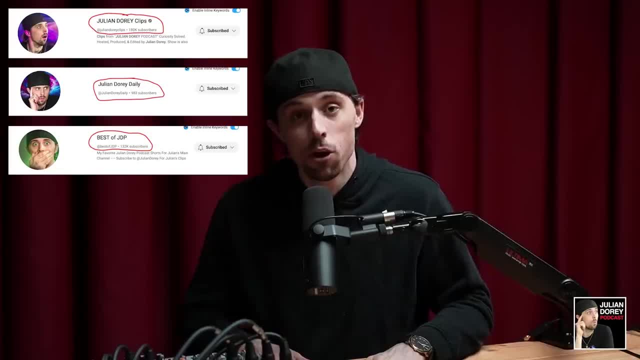 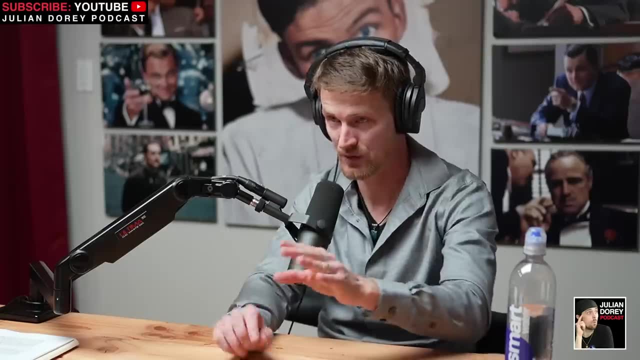 a shorts-only page. He will be making shorts exclusively for that channel. Once again, the link is in the description. You can check out all three down there in the description and I hope to see you guys subscribe, Thank you. So let's expand more on that site and why it's important. 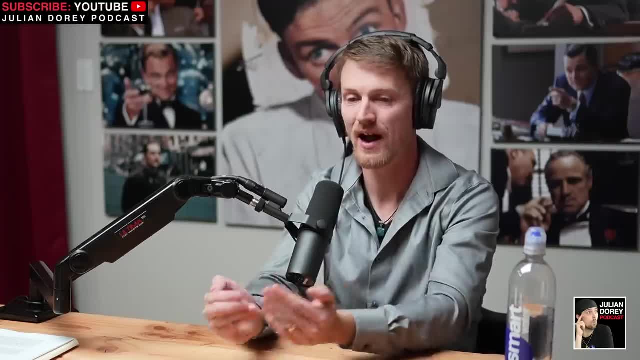 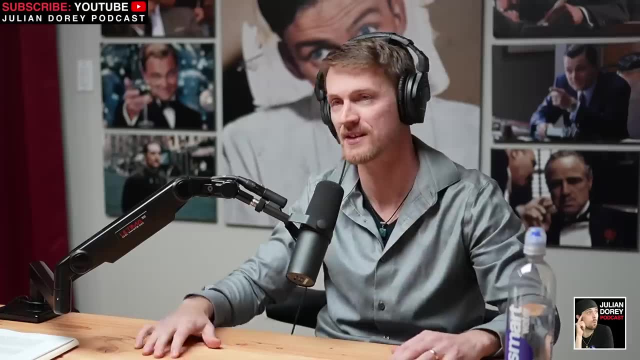 For those who maybe didn't listen to the last show, I study ancient Sumerian connections as almost an obsession: The ancient Sumerian original cities that were lowered in these tablets that discuss, And the last of those cities is called Sharupak, And that's the city. 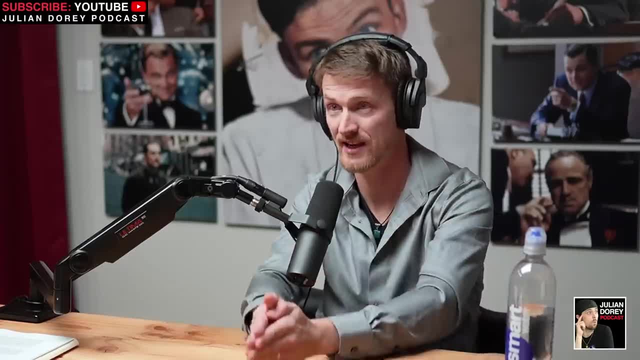 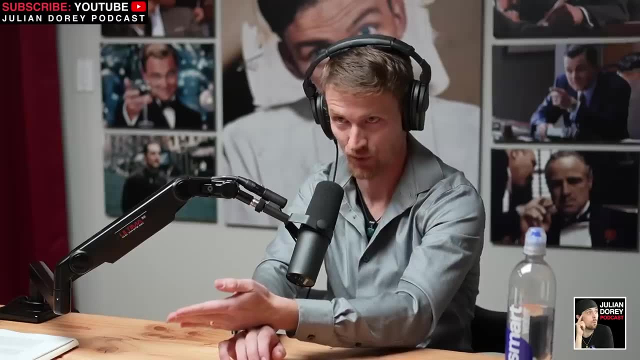 we talked about a little bit before in the beginning. That's the city that's supposed to be the last city that existed in this old world, long ago, before a catastrophe came through and wiped it out, And that's what I believe is the biblical flood. okay, And that. 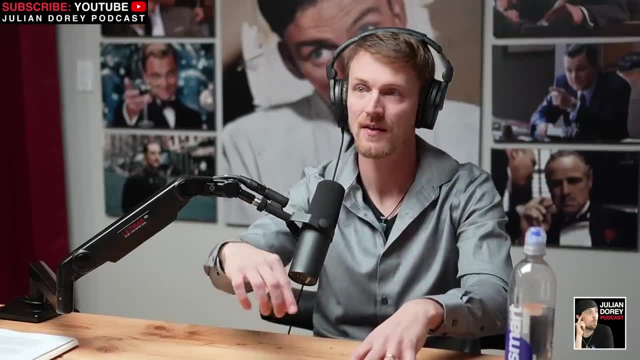 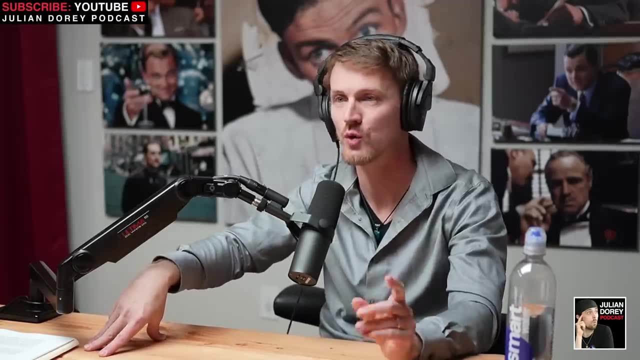 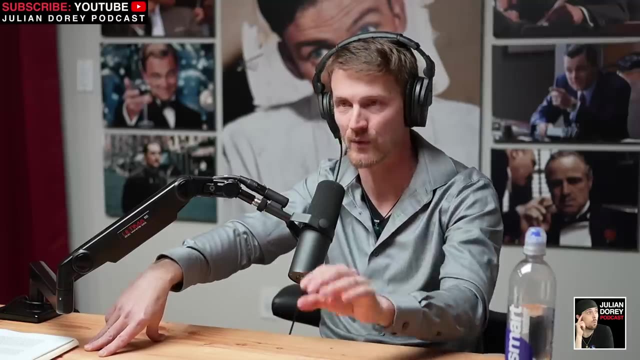 story is what connects this story? because the last Sumerian king was what became the biblical Noah, But he wasn't Noah at all. His original name was Untapishtim or Zayasudra, okay, And he was a priest and a king who was part of an ancient lineage back to the original Sumerians, okay. 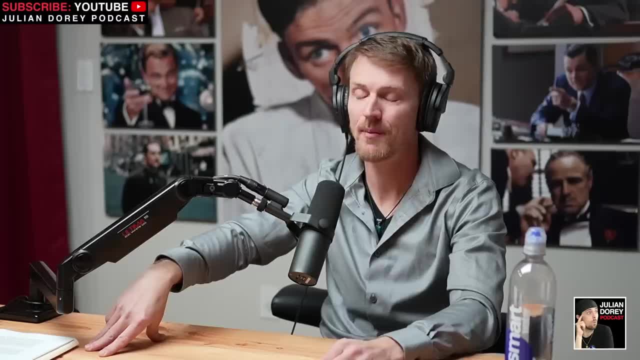 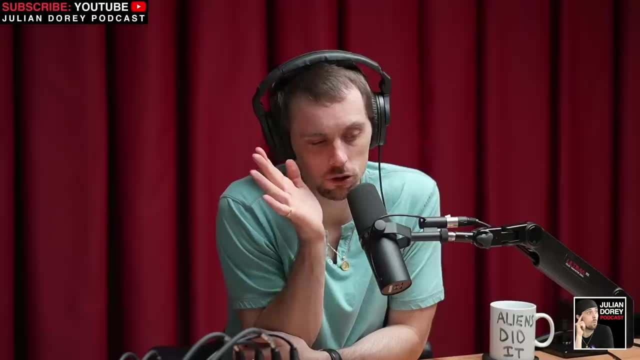 And what kind of year area are we talking about here? We're talking about well over 20,000 years ago. Yeah, We're going way, way, way back. We need to clean the slate and just start over again. Oh, yeah, Way before that. Now imagine just like: 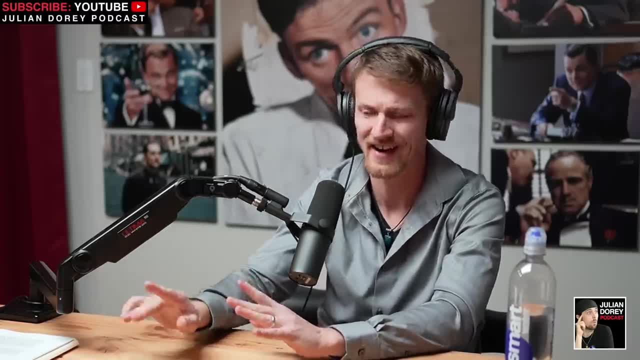 we get the biblical narrative that tells us about Noah and the story that kind of gets silly, which is like not to a very animal of any kind or anything. That's not how it's written. The original story from the flood, which is the story that tells us about Noah, and the story that kind of. 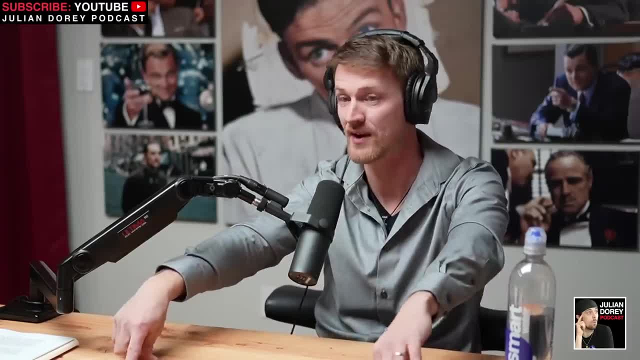 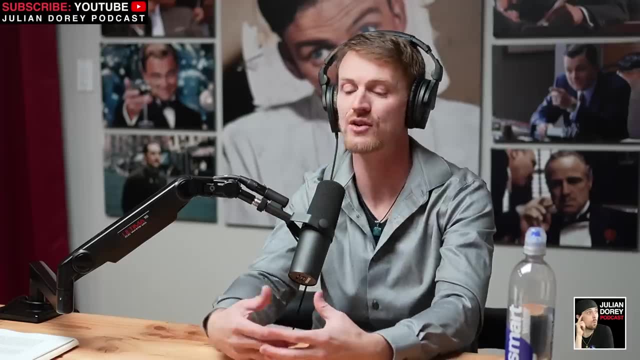 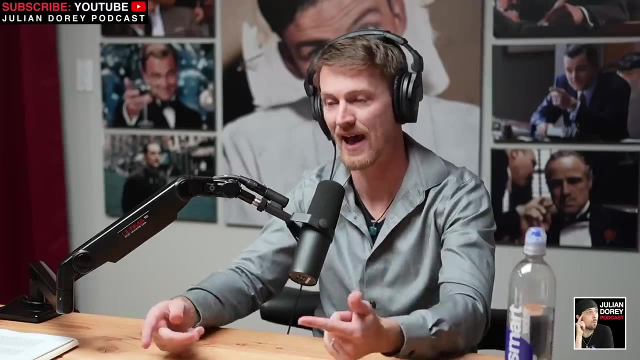 biblical story comes from a set of four different, totally different sets of tablets from the Sumerian, Babylonian and Assyrian civilizations. So imagine a story that was so important. It was like one of our benchmarks that made us who we are, and all these things came out of that. Imagine. 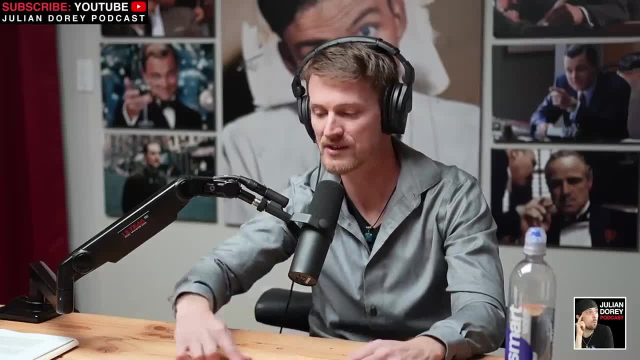 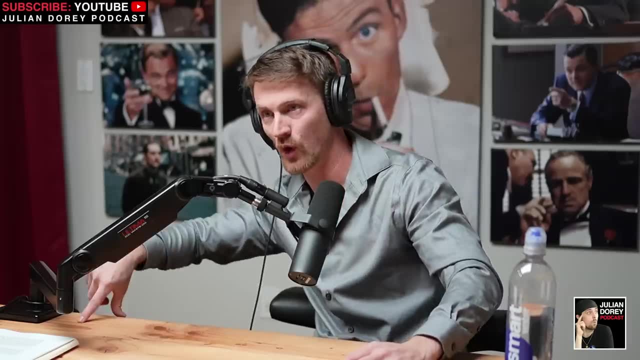 civilizations. that story is so important that even thousands of years later the other civilizations that come along write the same story to carry it on over, and, over and over again. And imagine, you find not only the later versions but the original version. Do we have anything archaeologically that? 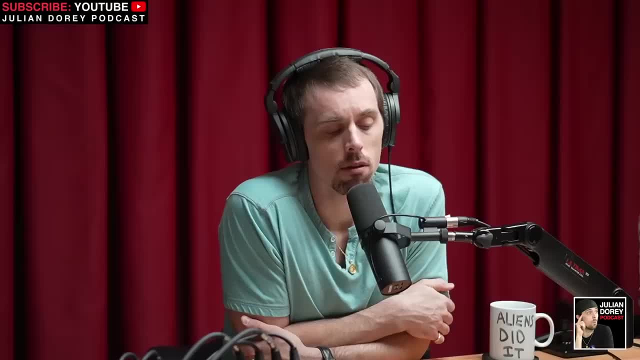 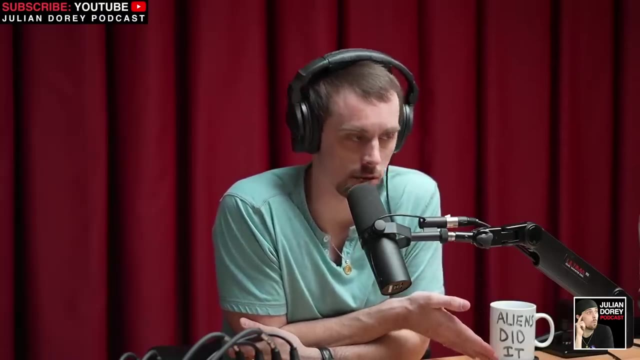 can back that up, though We do now. We do now Because I have to. I mean, before we go to that, though, I have to be fair and give the same criticism I give of all the Bible stuff, And again, there are some things that are absolutely supported by archaeology and stuff like that. 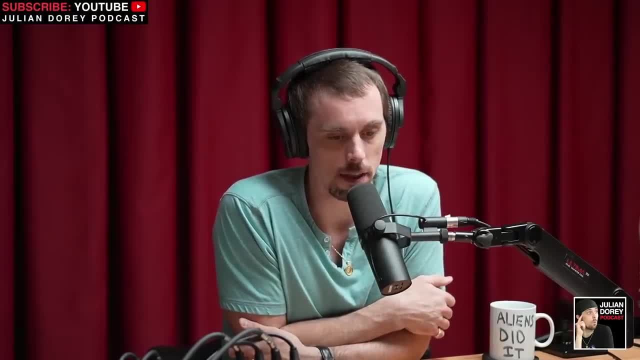 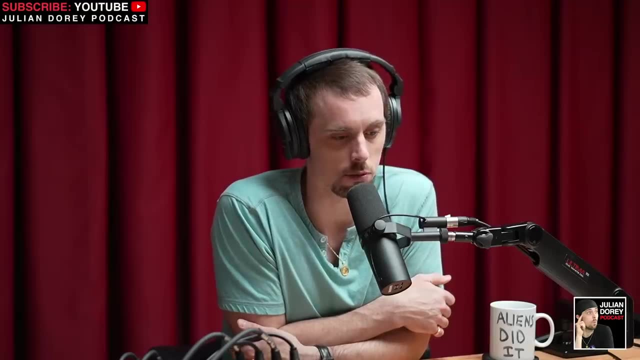 but story. humans change stories, right, And they may change. They may change in small ways, but if you play Whisper Down the Lane with 20 people and tell a story in someone's ear, by the time it gets to the 20th person it's you know 85% what it was at. 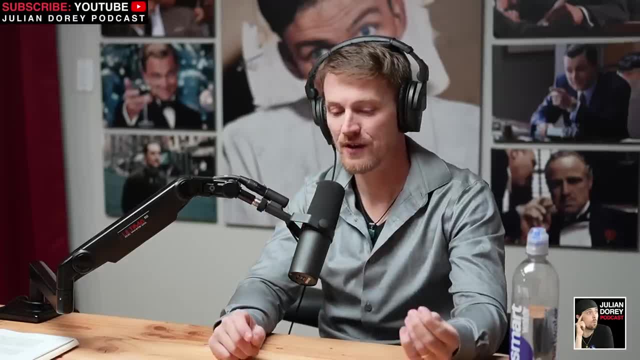 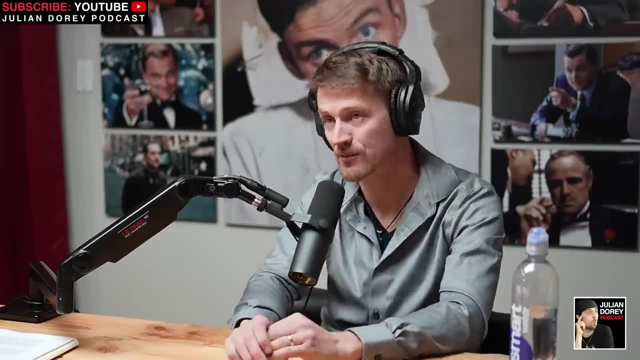 the beginning, Totally understand. But now imagine, though, if you have sets of ancient tablets, cuneiform tablets, from these civilizations, and they were all in the same place because of a man named Ashurbanipal, who's an ancient king and priest, that went out and amassed them into that. 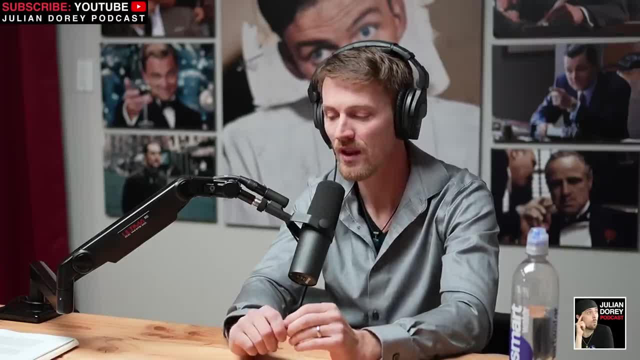 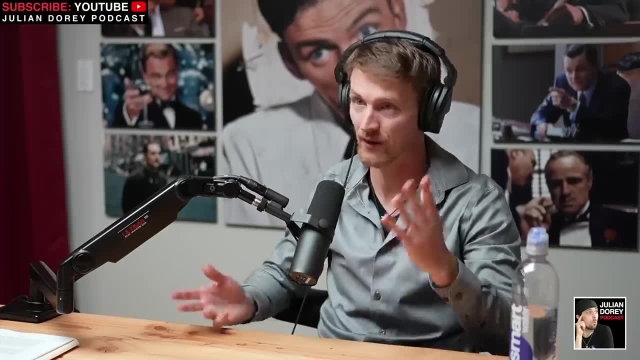 library we discussed right, Brought them all together. That's how we found them. But imagine if all those tablets describe a story And they all have the same parallels to the story. So then you say, okay, so there's some. 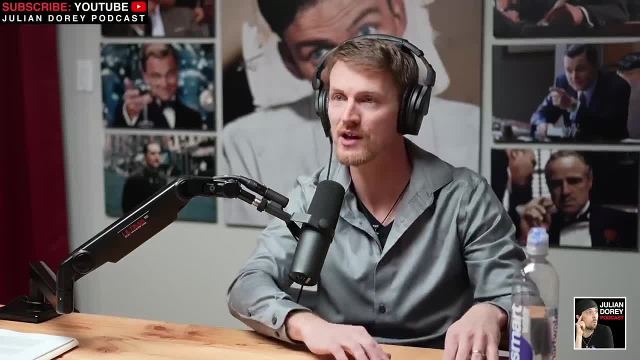 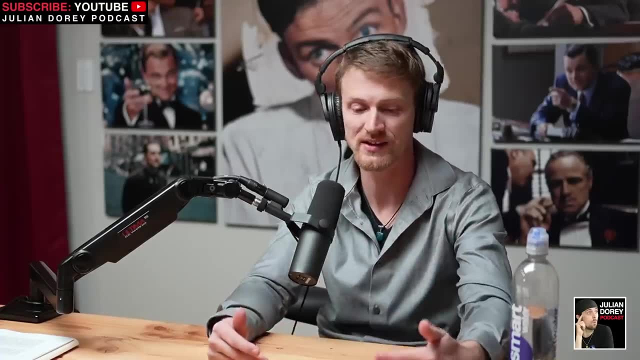 credibility there with that story right. See all the parallels You take and you cross-reference every single parallel and then put it together. There's your story right. You say like well, this is crossing over to this, They align. You take all their multiple avenues, that align too. 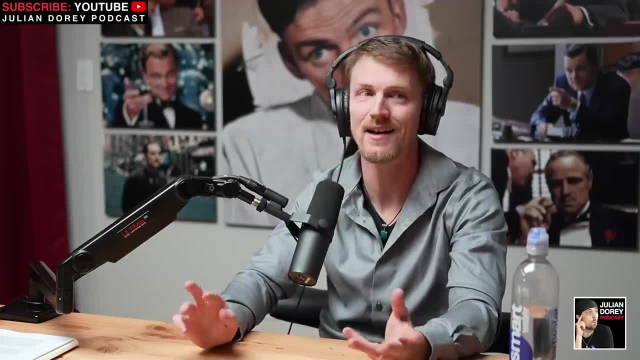 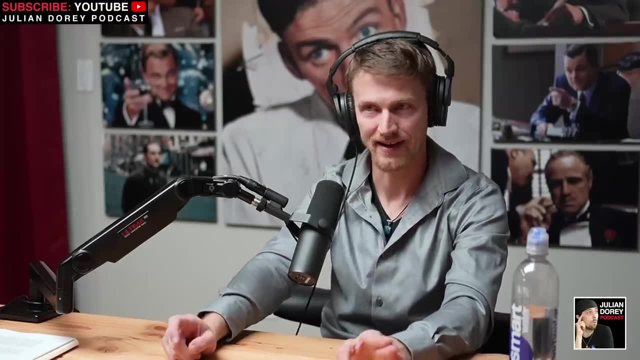 That's how you start formulating what it might be. But, like you said, that's not enough archaeological evidence to prove a timeframe. Take that. Take the kings list that they had: The Sumerian king list, the Uruk list of kings and sages, the Barocius king list. 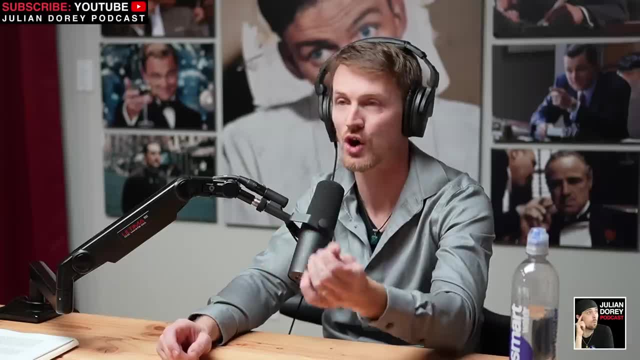 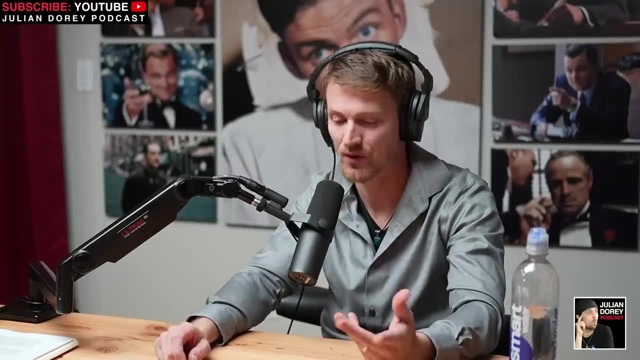 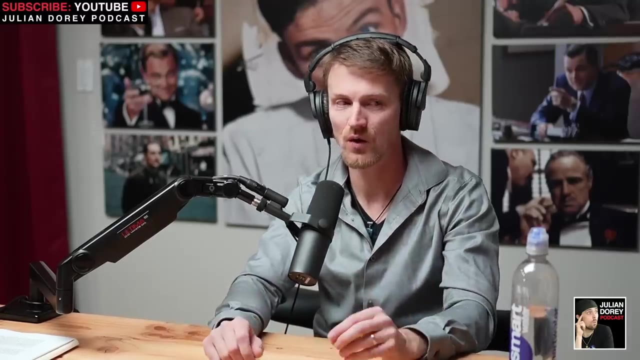 Then you take the Egyptian kings list from the Turin list of kings and kings from Egypt and you go to that as well as some of the ancient biblical texts like the Book of Enoch, and you get these weird correlations They all talk about, like these ancient lineages of kings that ruled for a long time, right, And how long they lived for. 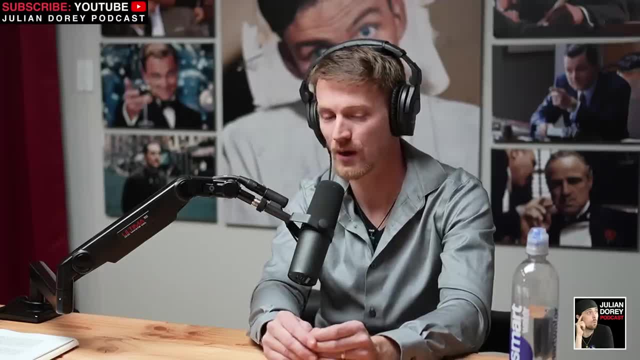 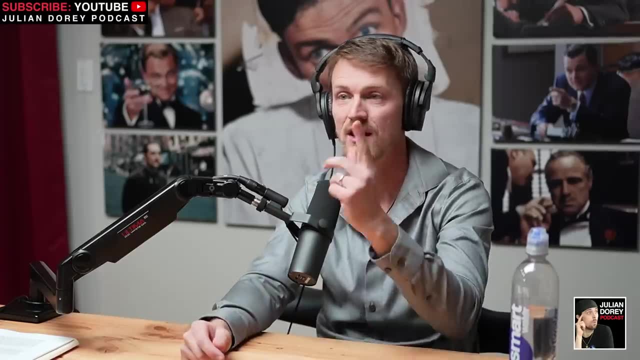 And if you're, if you can take that for a moment in a grain of salt and say, well, I don't know if I trust this one, but what if you take all of them and you combine them together, just like? then you take the ages, you take the reigns, you take the locations and you get a certain time period right. 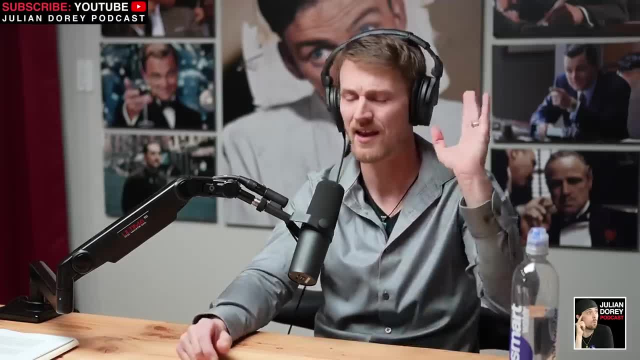 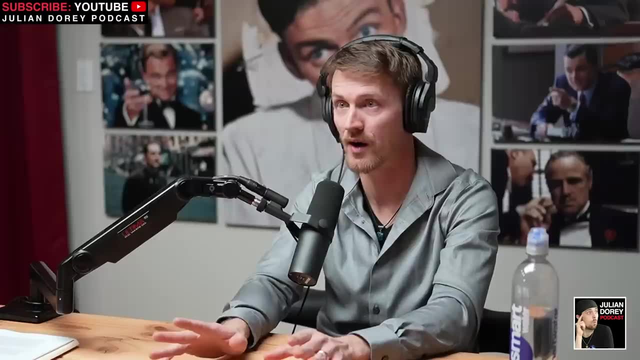 You get something that's like over 50,000 years old And it's like at first you like totally reject, You're like no way, That's. that's gotta be something wrong with that right. That's where we were. 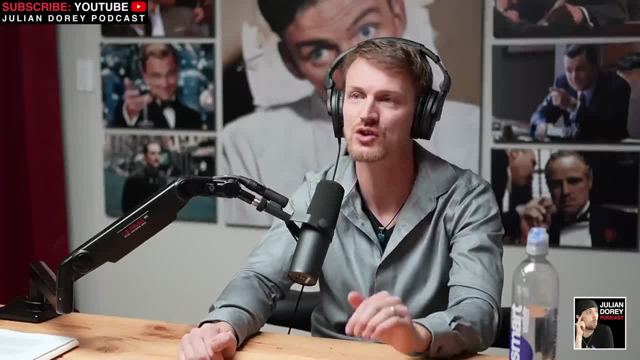 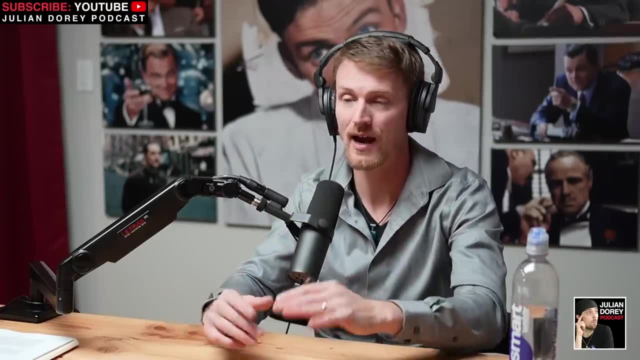 That's where we were before, because the problem is you can't date stone. So you get all these giant megaliths around the world and like people like Graham, Hancock and Randall and others, you know we're coming along, We're like. well, I think. I believe, based on the evidence, that these were built far longer and are a lot older than we're told- right. 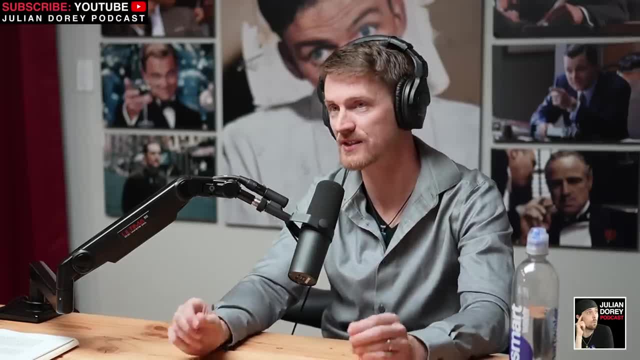 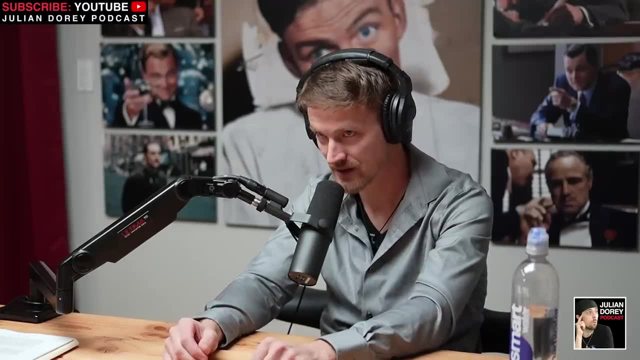 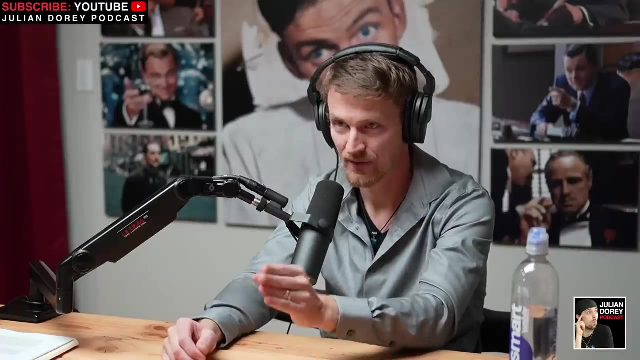 But how long ago. See, that's where it gets challenging, because how do you date if you have no organic matter? You use catastrophes. How does that help you date? You use catastrophes to date Time periods. For instance, you can take ice, you can take ice cores. let me give you an example. 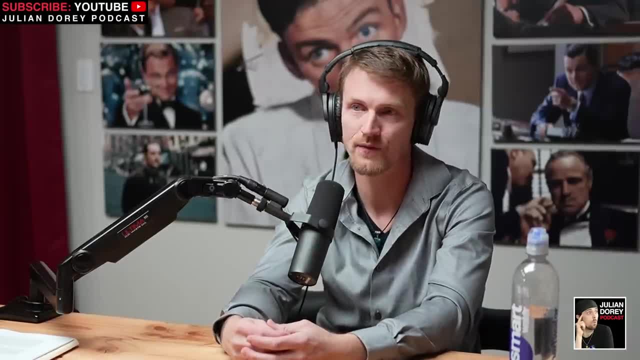 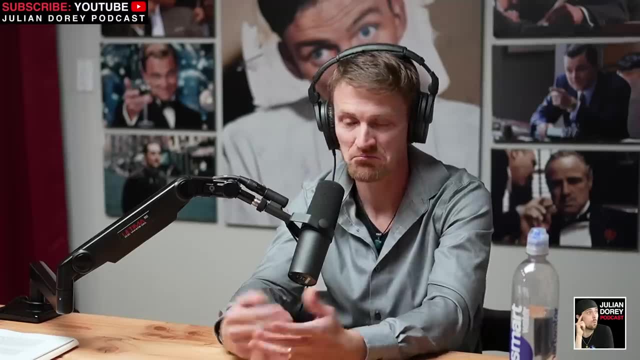 Okay, You can take ice cores, like say from Greenland, and you get a snapshot of 20,000 years max, because the Greenland ice sheet isn't necessarily most of it isn't older than that. So you get about a 20,000 year window, which is pretty awesome, right. 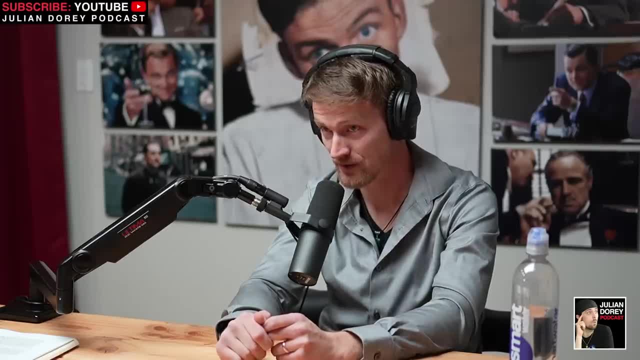 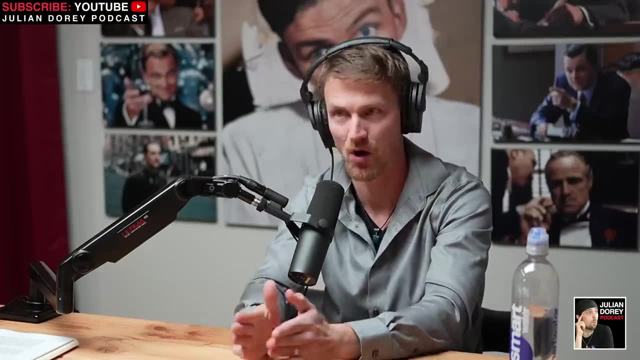 If you go to Antarctica, you can get a 500,000 year window, because the ice there is a lot more ancient. Okay, What do you do with that? Well, let's say you, just, for the purposes of being smart, Smaller. let's not try and get as big as the Antarctic ones. 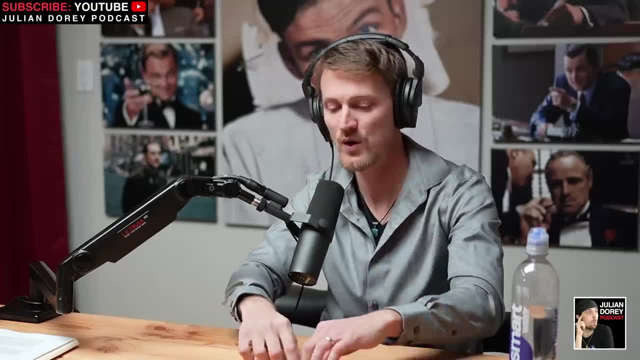 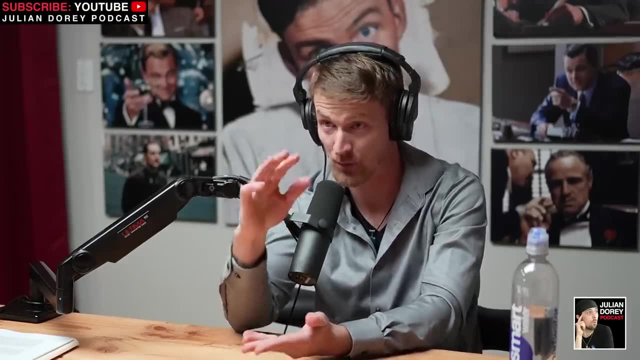 But let's just take the Greenland ice cores for a minute. You can look at that ice core and look at where there are bubbles in areas of like ash and things that have accumulated within that ice and it gives you a snapshot of what happened in the past. 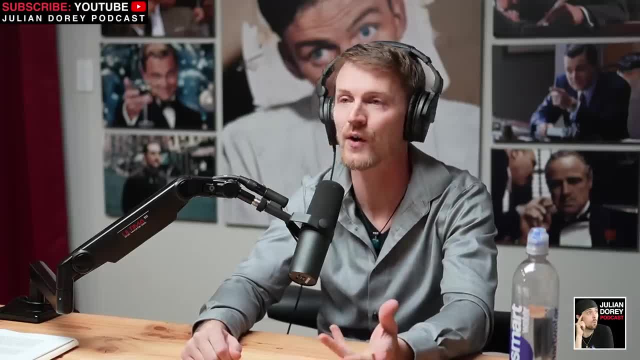 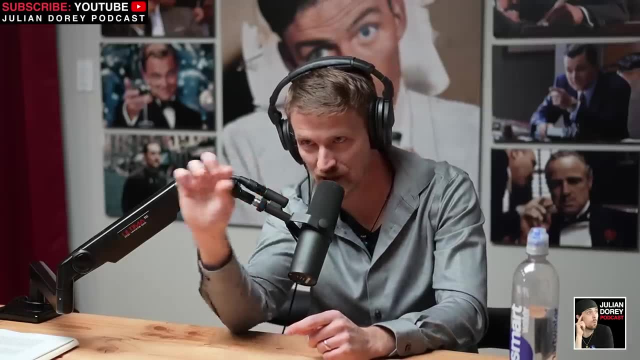 It's like a little. it's a little viewpoint on what happened on the Earth at that time. Some of these ice cores, like I said, you'll have a layer where you might have some microscopic ash that's accumulated All in a certain space. 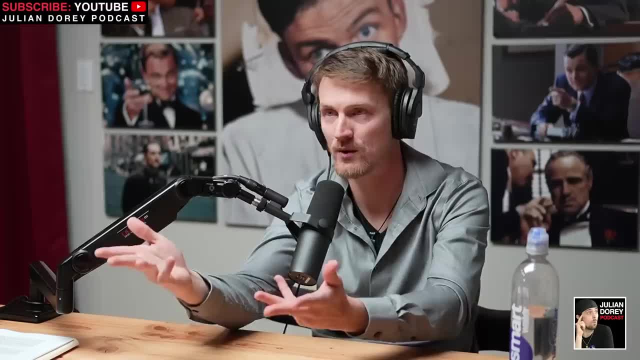 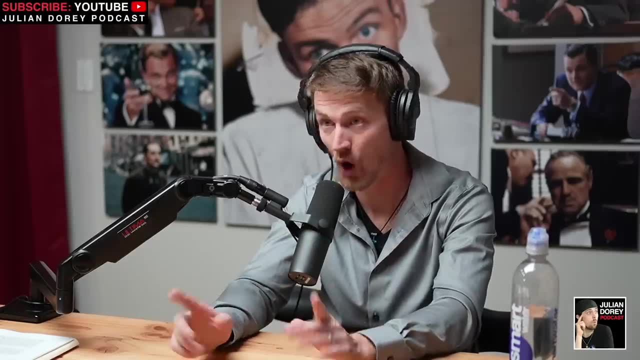 or extreme warming, And the way you would tell that is, you would see bubbles of carbon dioxide, And carbon dioxide is always the precursor to a warming climate. always- That's what you see in ice cores around the world- is that carbon dioxide levels always spike. 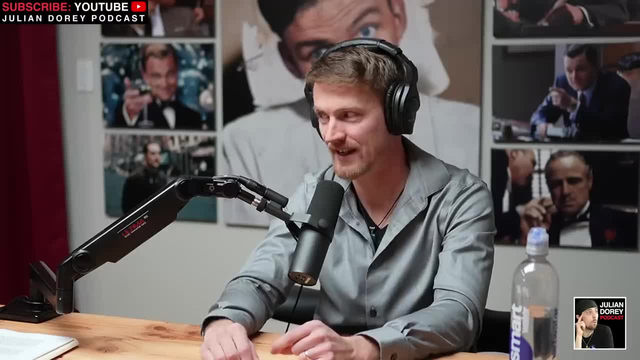 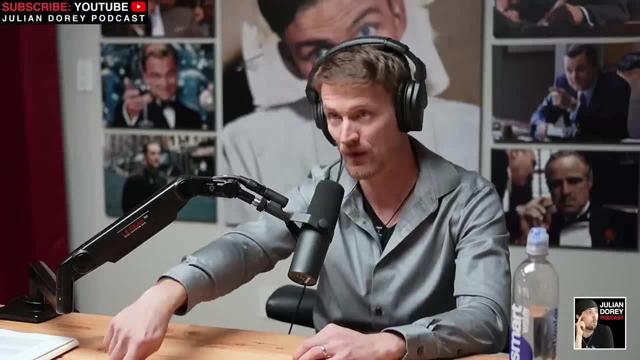 before temperatures do on the planet, showing us that it likely has nothing to do with human activity at all, because if you look at historical time periods, you get massive volcanoes going off, methane melting from permafrost. you already have the means to create catastrophic warming. 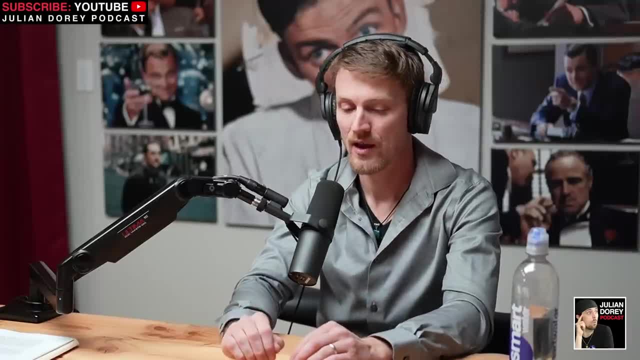 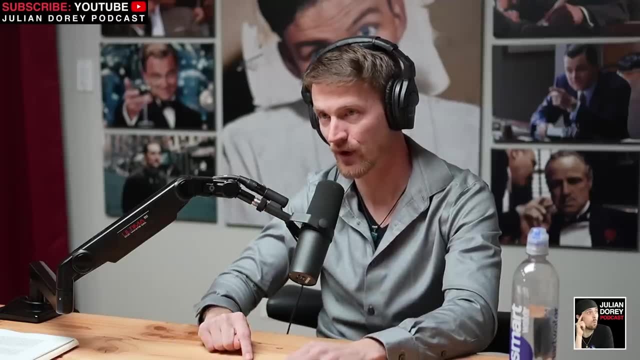 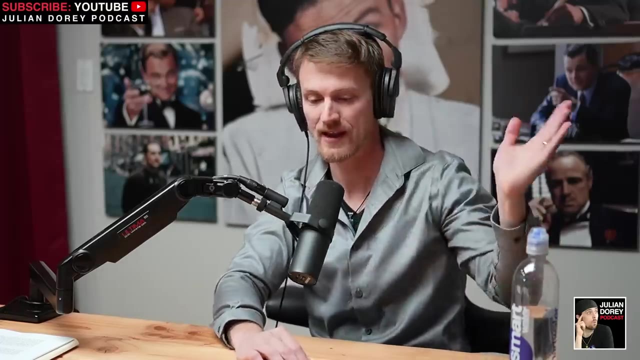 in those types of ways, right? Well, when we look at those ice cores, we find that there is a cyclical nature to the climate of Earth. cyclical: It goes through these very, very defined periods where it goes warm and then it goes really cold for a while. 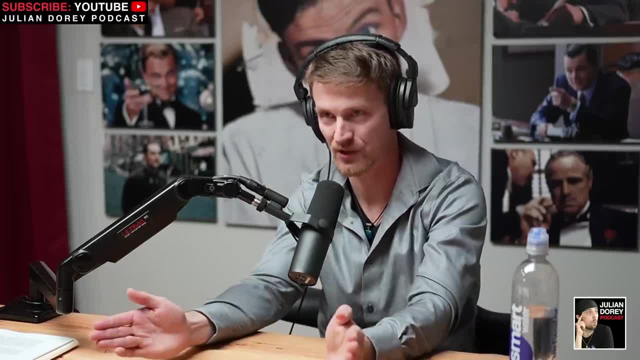 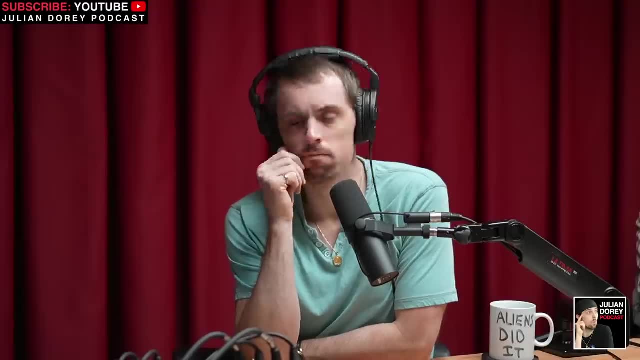 and then you get this interglacial period, which means in between the glacials periods, and you get catastrophes nearly every time. Randall talks about this all the time. Randall Carlson, You look at something, for instance. you look at the megafauna graveyards. 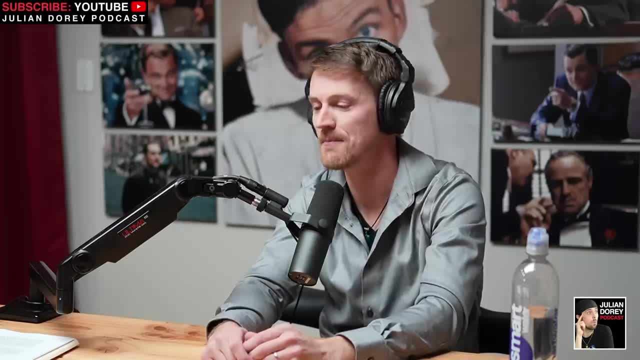 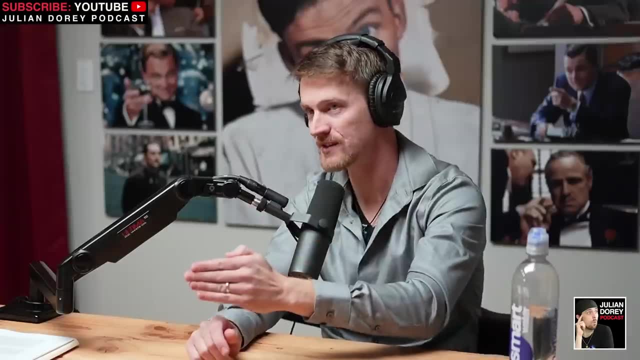 across the Northern Hemisphere, in Alaska and Siberia, and you can see millions of mammoths froze to death and die like instantly out of nowhere, right? So you take those things and then you say something like: well, what are the tablets talking about? 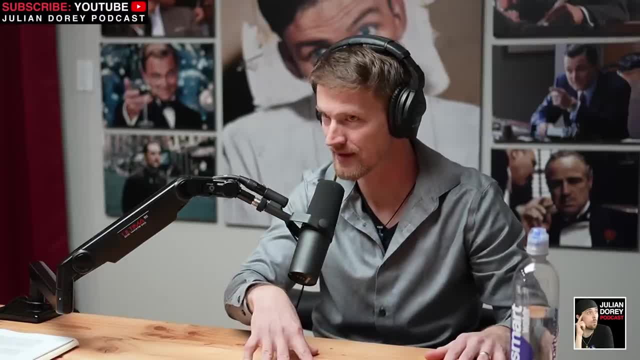 They're talking about some kind of a massive event. massive event- not regionalized though, because also Randall talks about this all the time, Randall talks about this all the time, Randall talks about this all the time. but also, wait, this culture in South America. 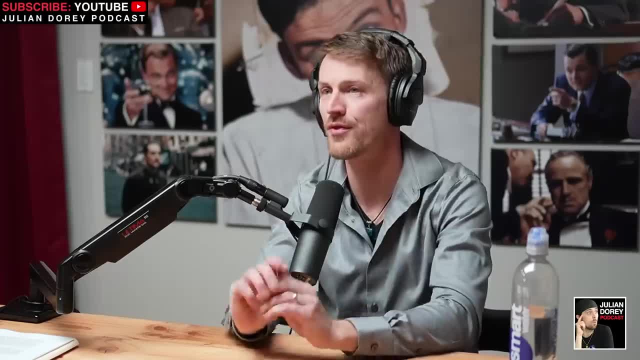 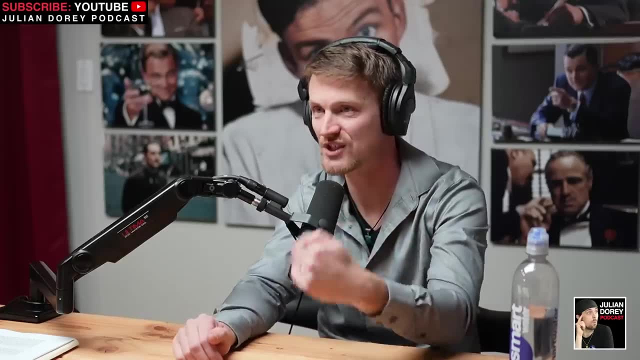 or Mexico is talking about it too. Or how about, like: there's more than a thousand stories in ancient cultures around the world, even indigenous cultures that aren't like advanced, of ancient floods, but not in a nature of like a, it rains a lot and something comes through their area. 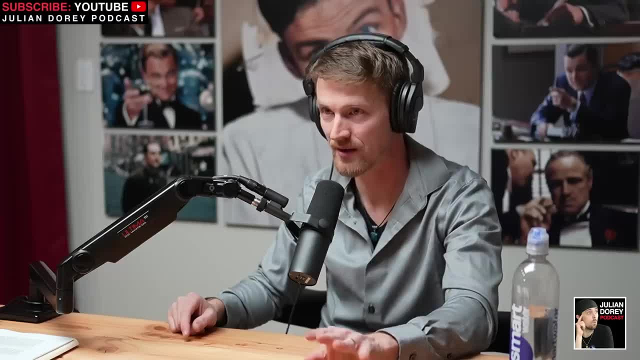 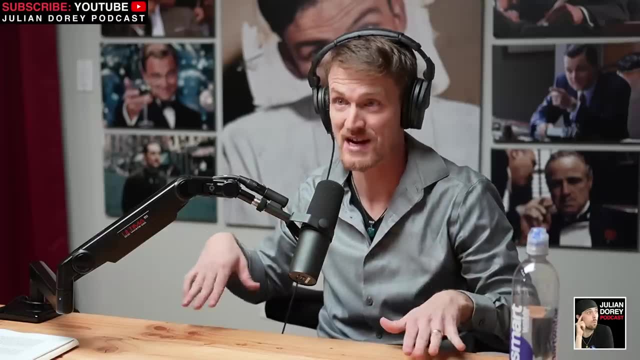 of ancestral stories, not from their memory. ancestral stories from long ago, of events that almost wiped us out so we weren't here anymore. That's the kind of things we're talking about, okay? So for a minute, take out the little stuff. 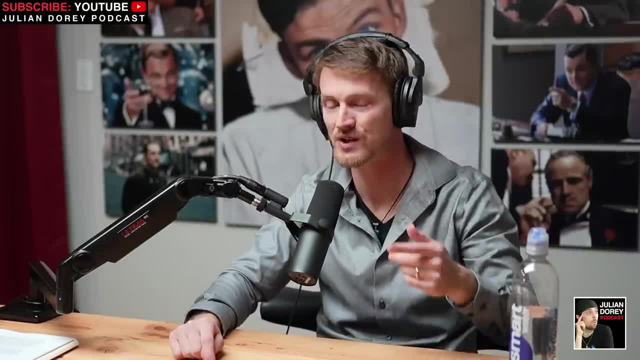 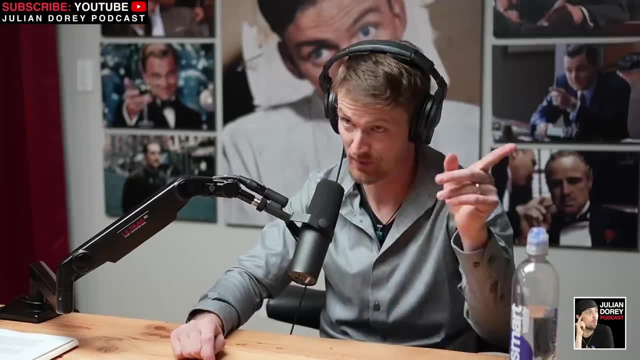 not the little events like the medieval warming. right, If you look at ice cores, you'll see that during medieval periods there was actually a series of years that were warmer than we are now. During medieval times It's called the medieval warming. 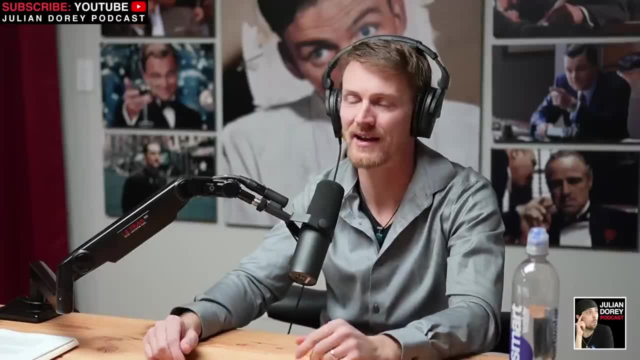 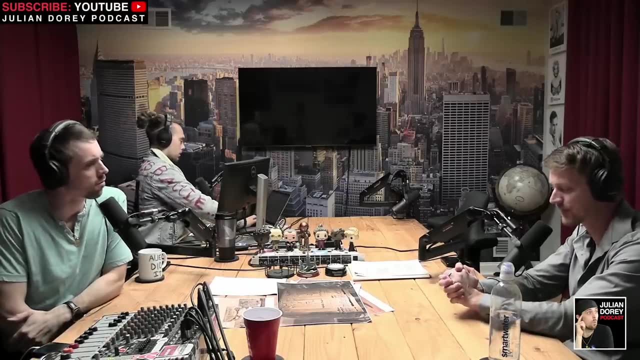 When was that approximately? That was what is that? 400 years ago or something I don't know, right off my head. I'd have to look at that. Yeah, can you look that up, Alessi? Medieval warming. Now, what people don't know is that there is 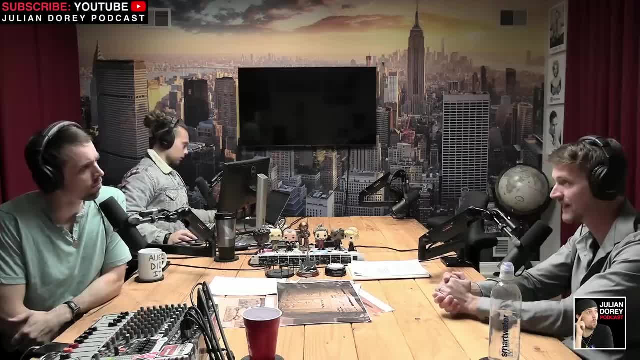 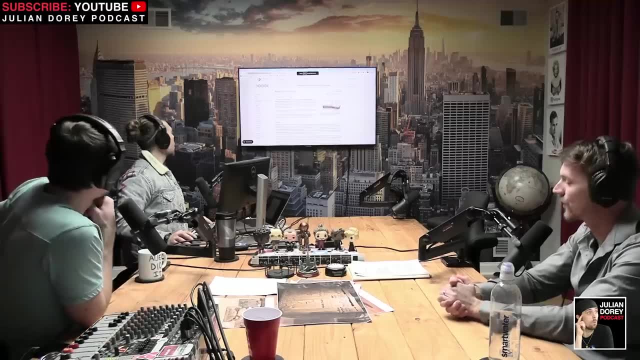 a period called the Younger Dryas, but there's also an Older Dryas and then an Oldest Dryas. Oh, they call them all the same thing, Right, and what it means is that when the Earth went through its interglacial cycle, 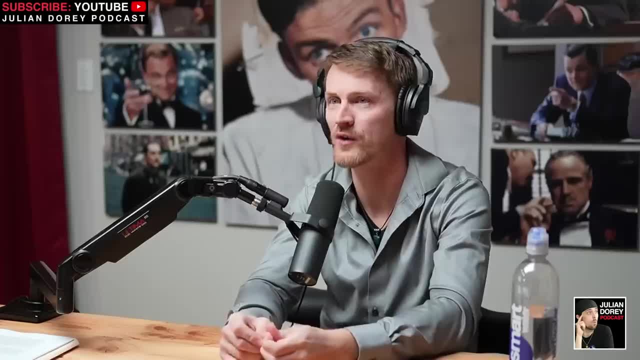 on the last time, By the way: 950 to 1250.. Okay, yeah, a little older than I thought. Okay, a little older than I thought. Now, imagine what was I just saying. I lost my train of thought there. 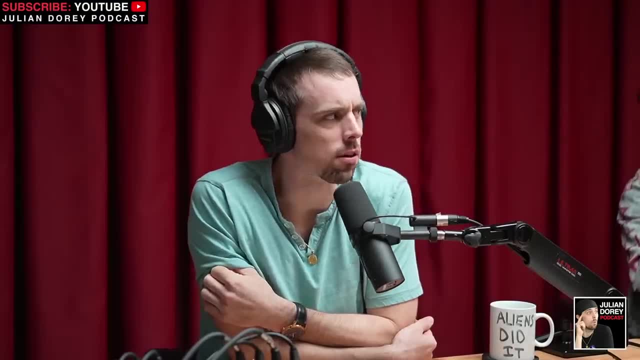 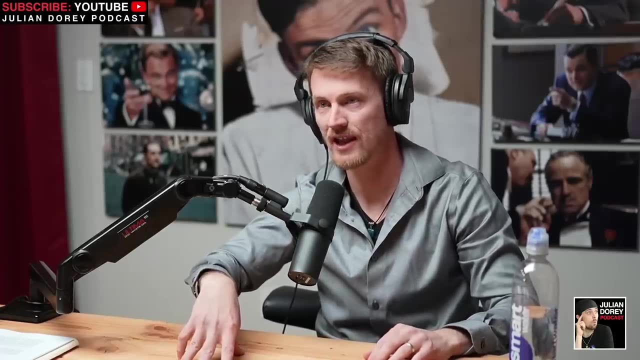 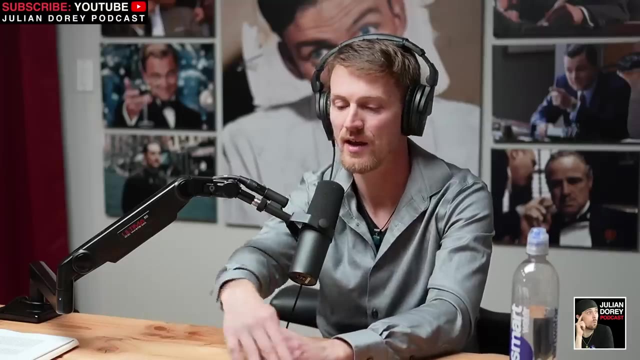 When the Earth was at something. at the same time, I was looking at the screen. Imagine you take these time periods of interglacial and you recognize that interglacial periods come with disasters. right, You're a climate scientist. You look at how, when you 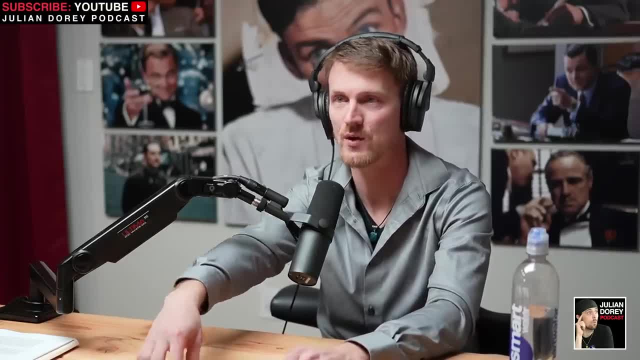 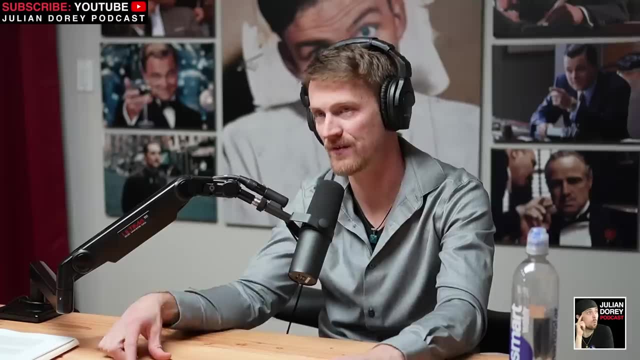 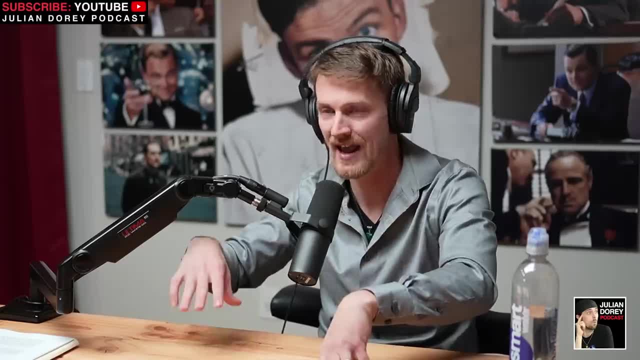 Not for a consistent 1500,, but like 1500 years. Not for a consistent 1500,, but like 1500 years, but like maybe every couple hundred years, or especially like a big one on the front end. 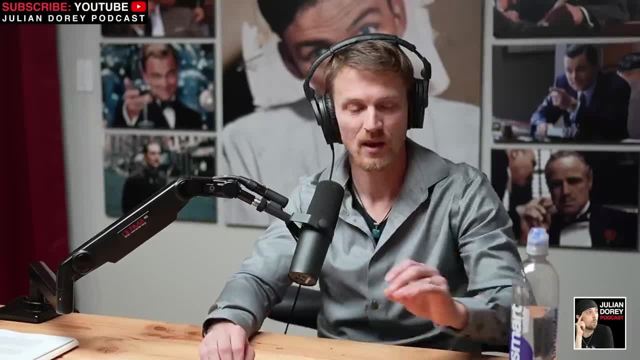 and then a very big one on the back end, right Events. Now imagine that there have been more than one of those though. Now imagine that there have been more than one of those, though, And we know that because when Solon traveled down, 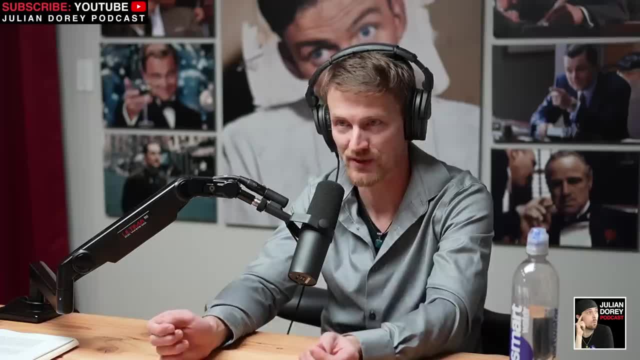 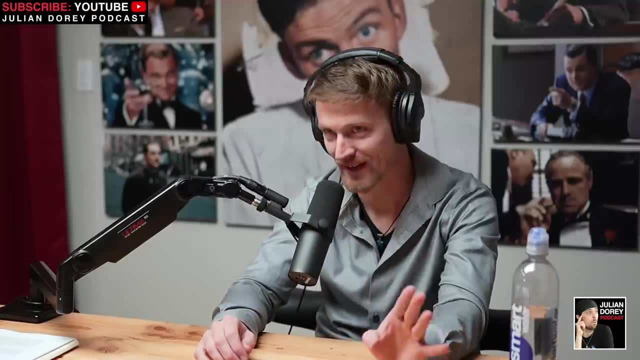 traveled down to talk to the temple priest of Sais that we talked about in Egypt. we talked about the story of Atlantis. Yes, They say, you Greeks remember one deluge only Solon. he's talking, they're talking too, But there have been many prime man of the land. 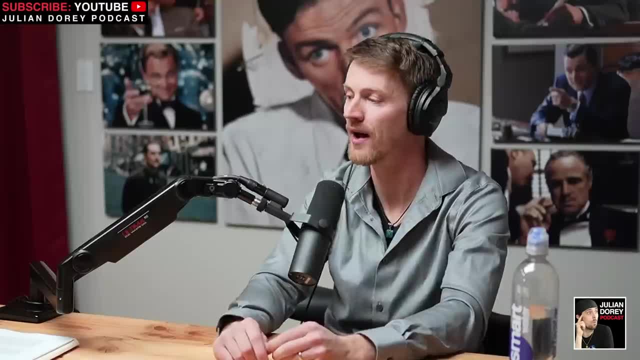 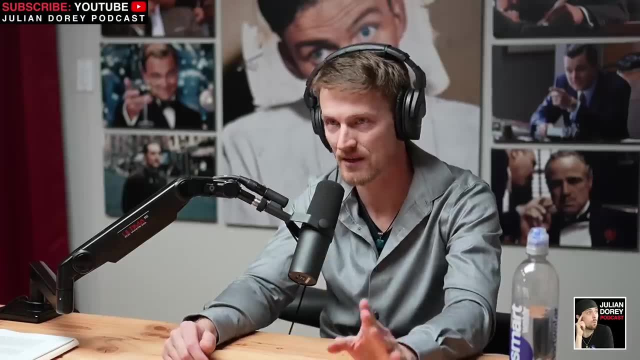 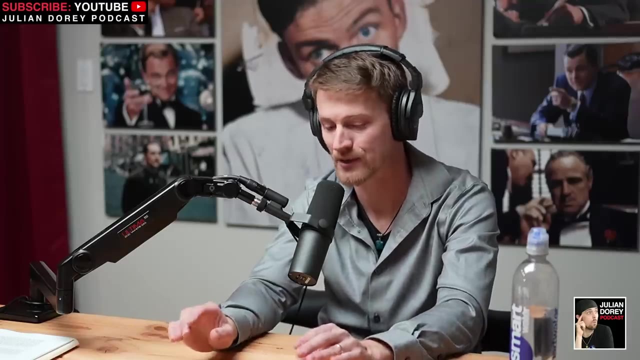 of fire and water. yes, all right. so they're talking about how there have been events with like volcanoes and plate- maybe plates may be moving with all this stuff, and also tsunamis and floods. let's for a minute, just disregard a regional event. i understand scientists and academics. 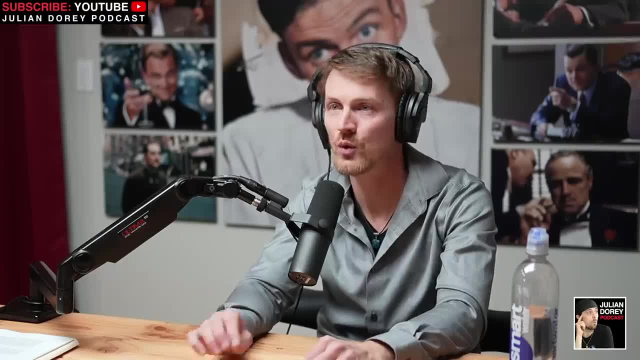 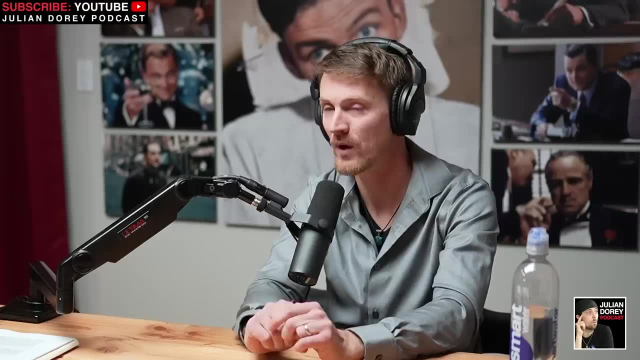 were like well in their world. back then, they only knew a certain area, so for them, if an event occurred, it was worldwide, because their viewpoint was small. right, that's the argument. what if that's not true? what if there have been catastrophes on the earth that have affected the earth in? 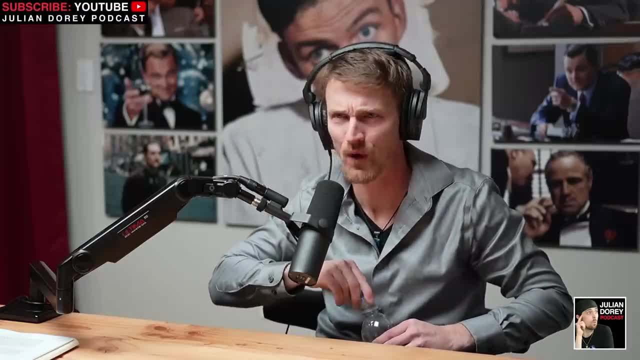 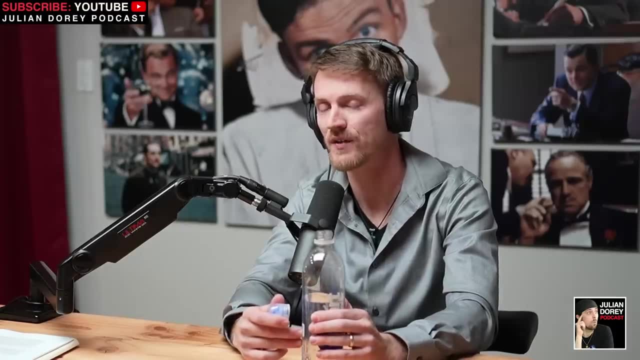 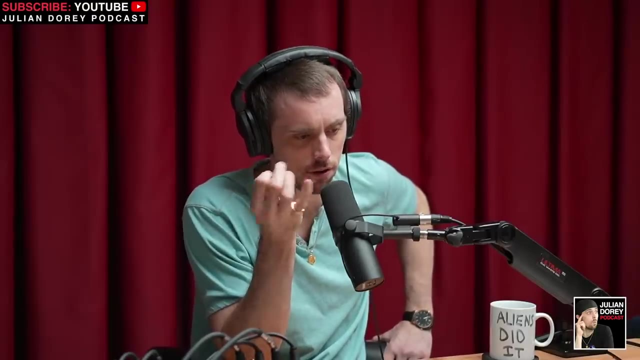 different ways- okay, not like annihilating life all over the planet or anything but affecting the earth in different ways- and some of the areas that got affected extremely significantly were the areas that these lost civilizations were living and are those areas that were significantly affected, very often underwater, now underwater, or they've had massive um tectonic. 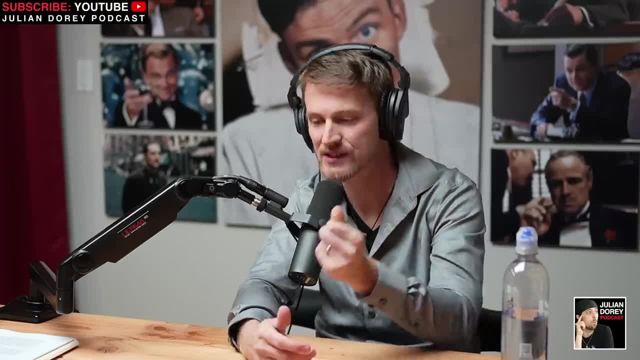 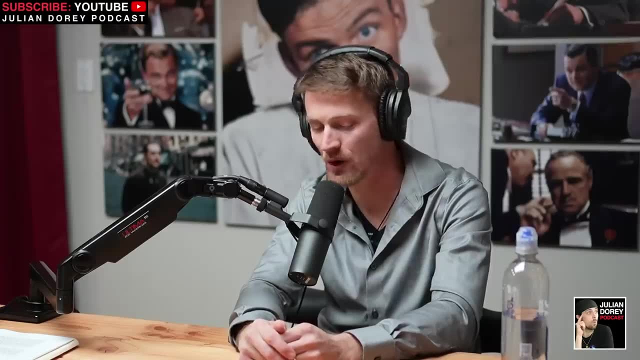 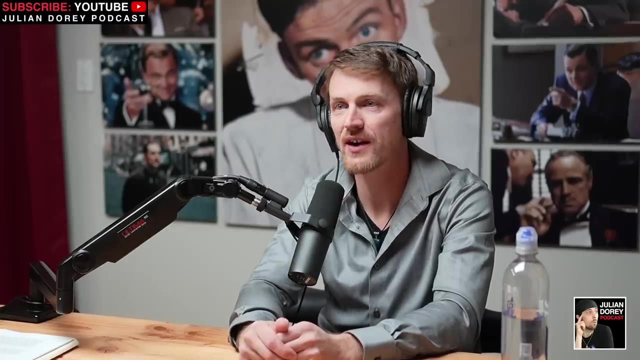 changes. let me give you an example. outside of um, outside of way to tambo and sasuke woman. outside of um, sasuke one oi te tambo. we find these very, very bizarre uh ruins of staircases. it carved into these massive, massive uh rock. watch the camera there. you're massive. 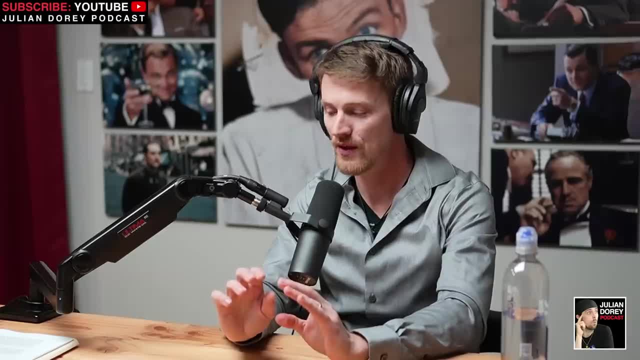 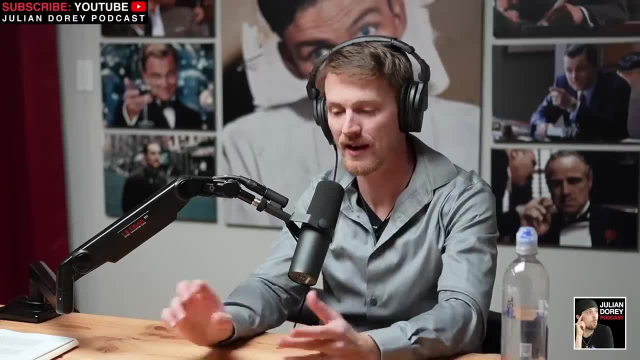 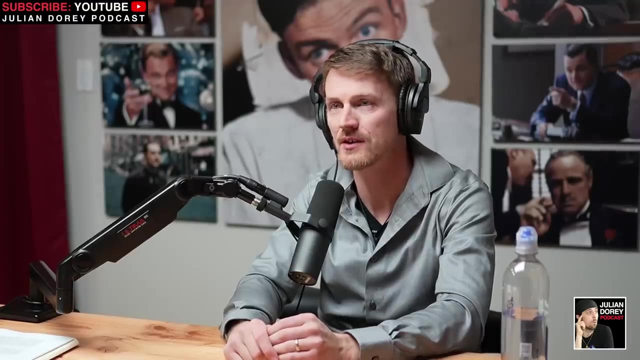 massive amounts of rock, okay, and the stairs are upside down, okay. the rock that they built on in these boulders outside of oi te, tambo and sasuke woman is like hundreds and hundreds and hundreds of tons. okay, and i'm not saying they move the stone. 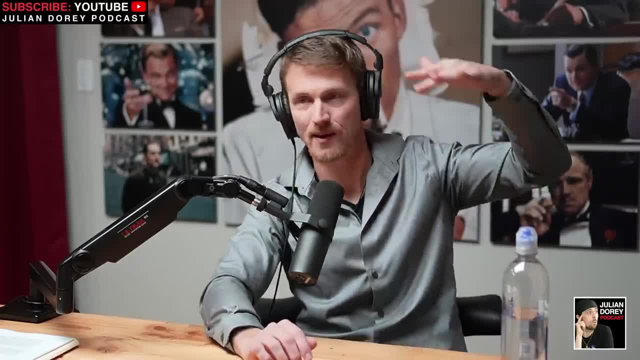 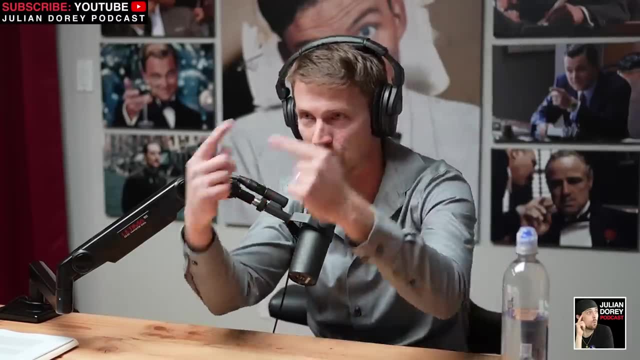 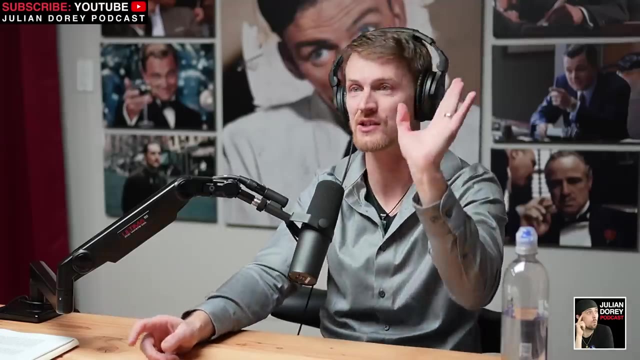 what i'm trying to say is: the staircase is upside down on it. okay, it looks like that massive stone as big as like this building was toppled. okay, if that makes sense, was like literally falling upside down. and now the staircase is staircase is on the wrong side. what kind of 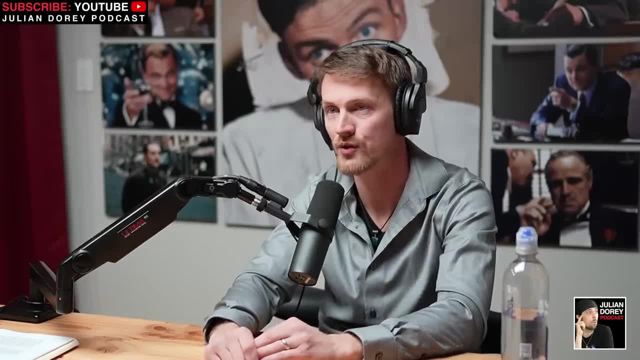 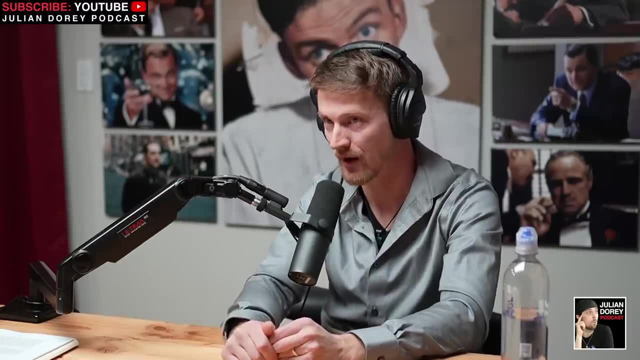 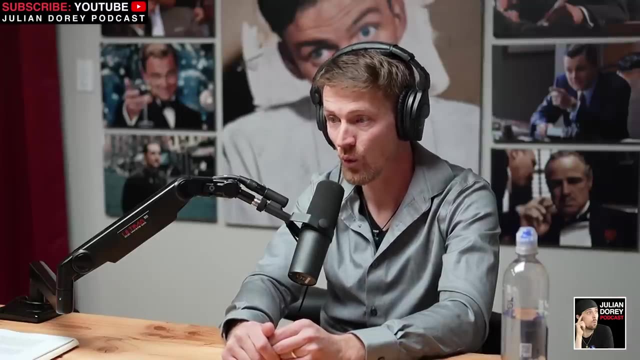 catastrophe or tsunami could move like a 200 ton rock and flip it like a like nothing. that's the kind of catastrophes we're talking about. yeah, something with civilizations like lake titicaca that we're going to talk about, that are over 12 000 feet, had tsunamis high enough, i believe. 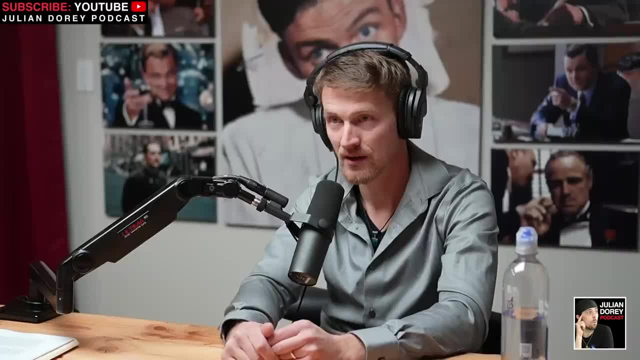 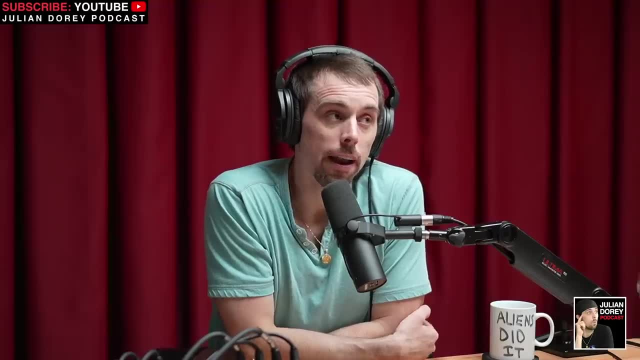 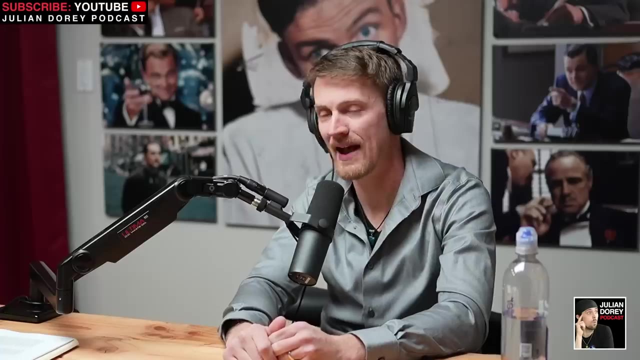 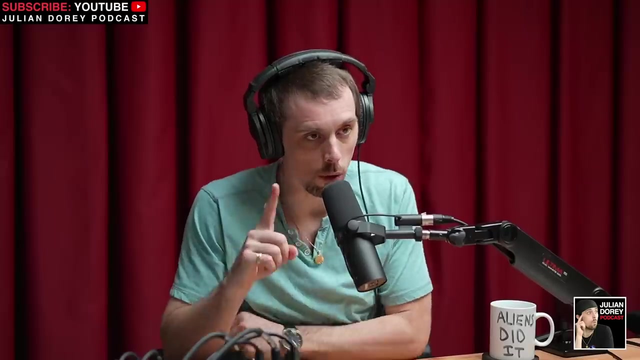 to wipe them all out. okay, so imagine, was that tsunami caused. could it could- and i don't know how far back you're going with these- could it be caused by something like asteroid impact, that? or massive tectonic shifts from like, uh, magnetic disruptions too? okay, all right, real quick, i gotta go to the bathroom. okay, we'll be right back. 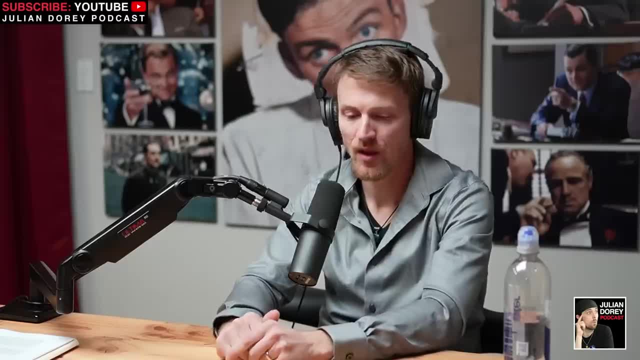 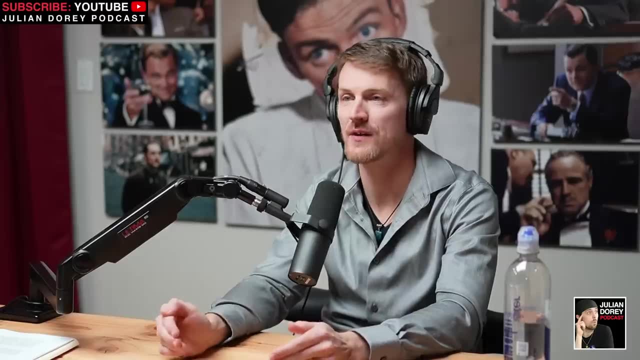 all right, we're back, go ahead matt. so when we when we talk about these massive tectonic shifts or impacts, like we had, we had a lot of people talking about these massive tectonic shifts or impacts, like we had referred to before, there's a number of different catalysts that can create these earth catastrophes. 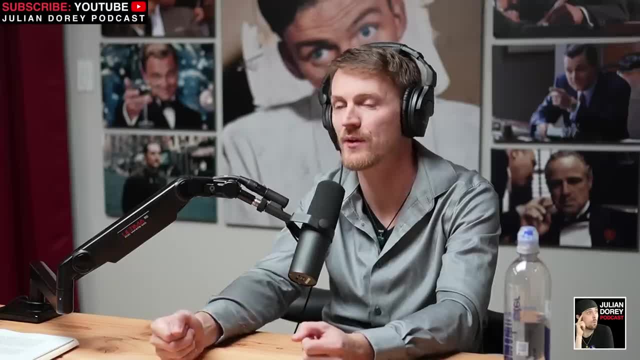 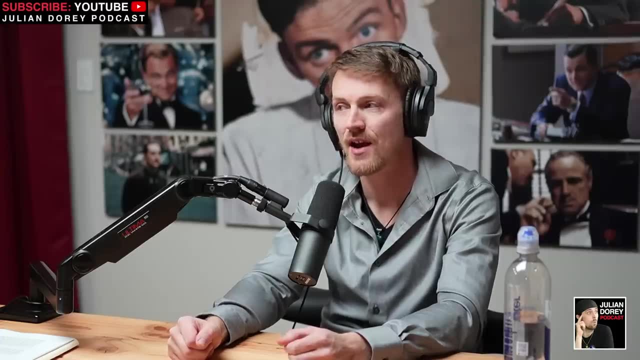 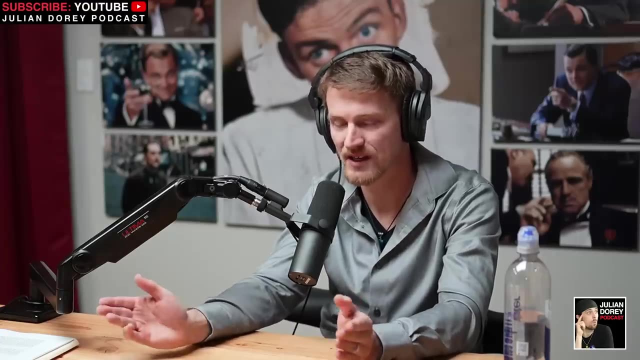 now, the reason why it seems so foreign to us is that we've we've never experienced one in modern history. okay, the events that we've seen over the last 500 to a thousand years are very insignificant compared, even like. i mean some. look, we've had tsunamis in. was that 2001 or i can't remember. 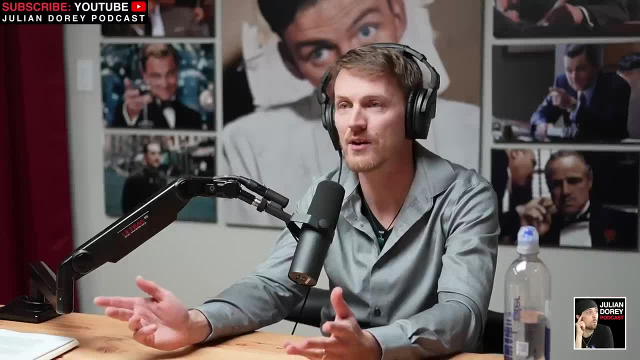 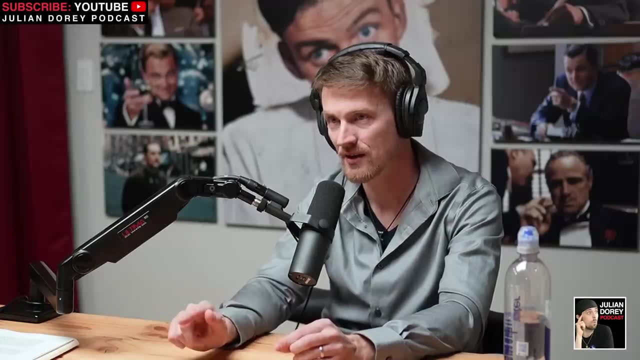 the exact date, or six, were in one spot right in indonesia and parts of that were thousands of people died. that was a horrible tragedy, but that was an isolated situation. imagine if you have tsunamis going across, like entire parts of the world, different regions, not not everything was. 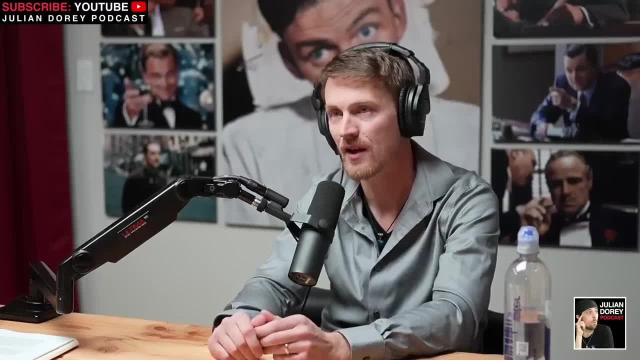 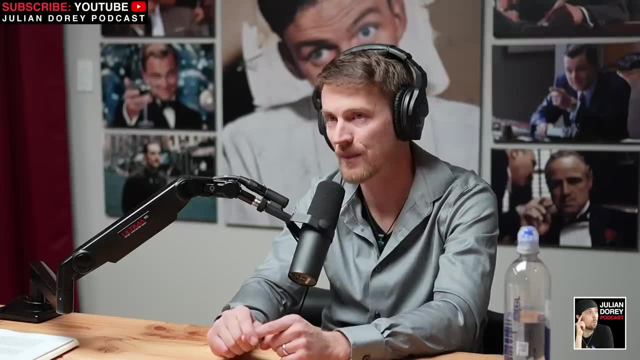 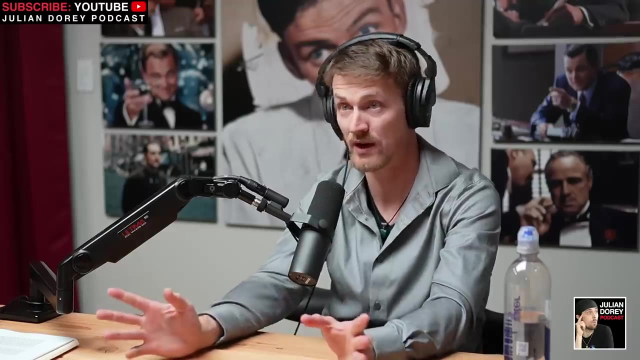 was impacted the same, the same way. obviously life wouldn't be here, but some areas were absolutely devastated and these discoveries in eastern turkey are showing just that. places like kef temple, where that box relief we were discussing were found, and ionis were buried and literally strewn and almost 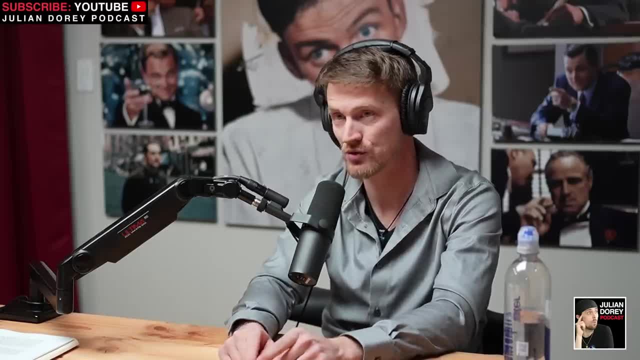 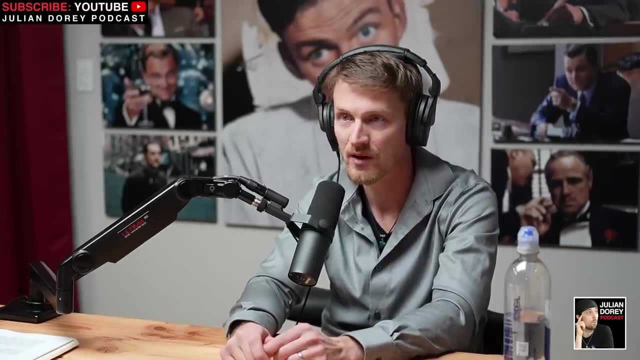 destroyed by something so significantly where they almost destroyed, they were even buried to the point where sometimes the urartian civilization didn't even find them so deep, deep, right and very deep, and some of them they did and other ones they didn't, and they built on top of them. but the point 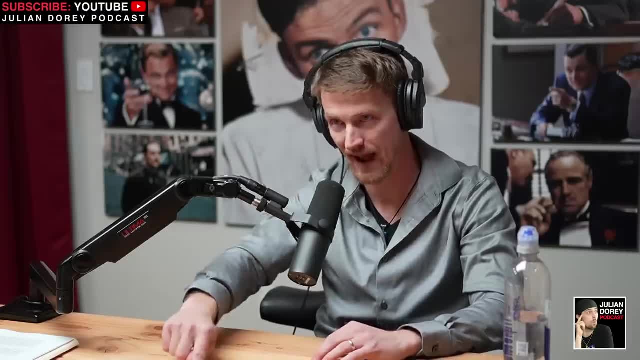 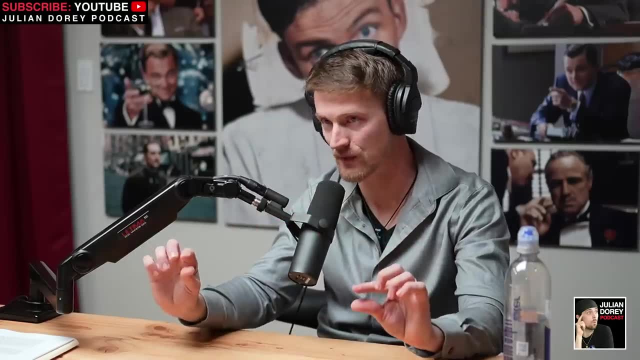 is. what i'm trying to say is, when you map out these catastrophes on according to ice cores and you can find geologic evidence on earth, like the black mat layer that randall carlson talks about, from younger dryas, some kind of a massive forest fire impact layer- you can see literally like a black. 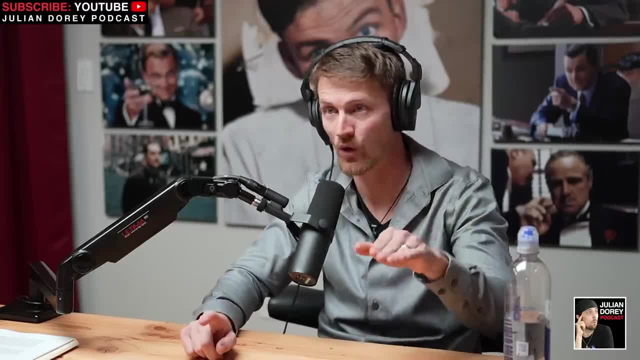 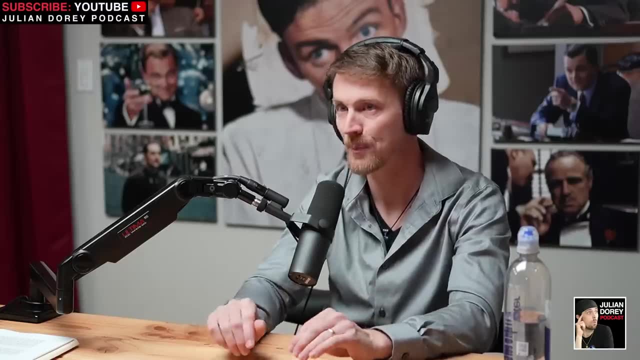 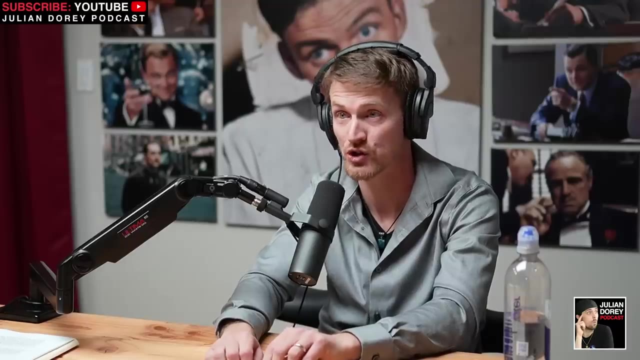 layer in the same spot in a lot of parts of the world from that specific event. so that's how you can sort of correlate and figure out histories. you can actually take those pieces right. in this case we have a set of tablets that talks about a great flood. i mean to the point where it's similar to 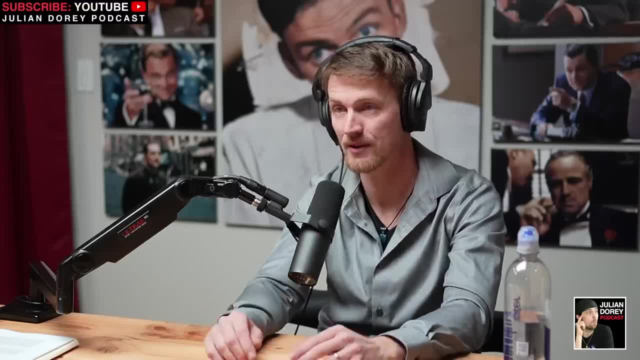 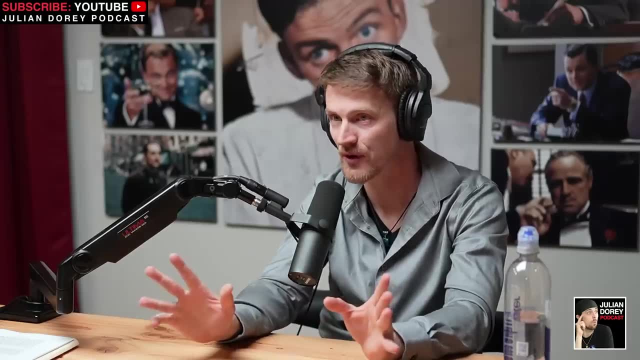 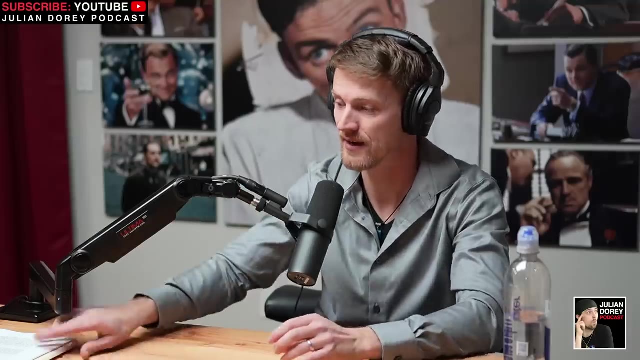 destroying the old world, though like destroying it, and, according to the tablets, the land near mount ararat and the sun's. if the tablets state that the sun's mysteriously disappeared in the world, that we don't know what happened to them, it only talks about the the noah figure as being, and i can i can give you a quote. 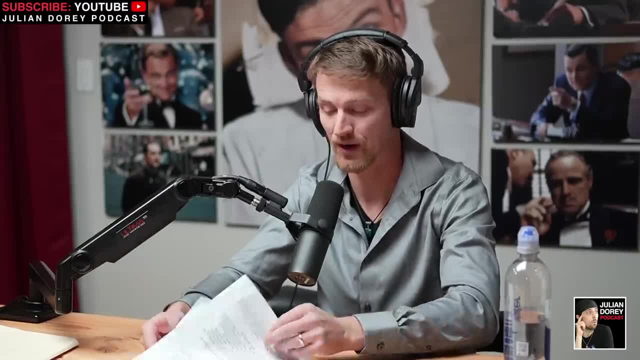 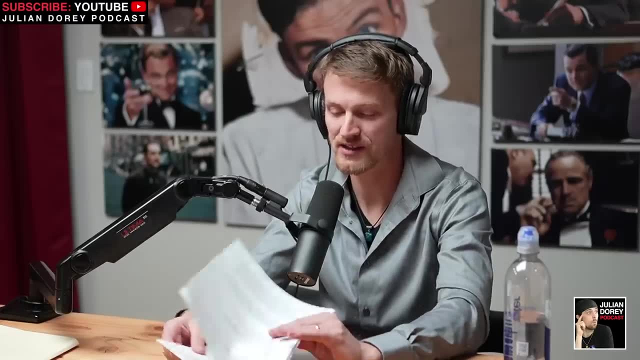 here. let me just, let me just read this. really, i think people are going to love this, but noah is who you were referring to, as i know. yeah, their stories here. here's a quote from a tablet, an ancient set of sumerian tablet called the myth of adapa. okay, is this available online? these are all. 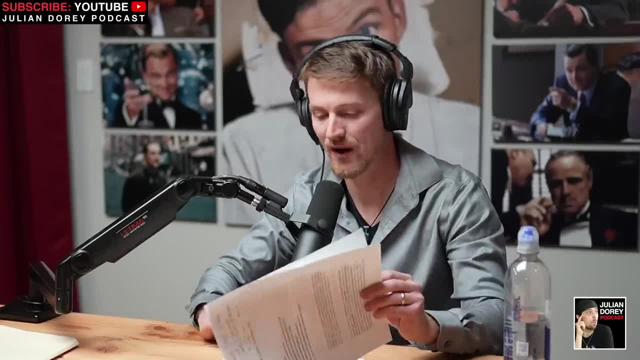 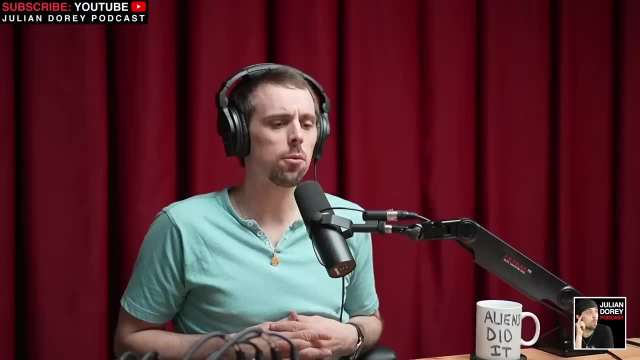 available online. the problem, the problem is the problem is that the sun has disappeared from the earth and the sun is gone, so we're going to have to find the right translation. so we're going to. we can read some myth of adapa, and then also the other tablet is called erudigenesis. okay, how do we that's? 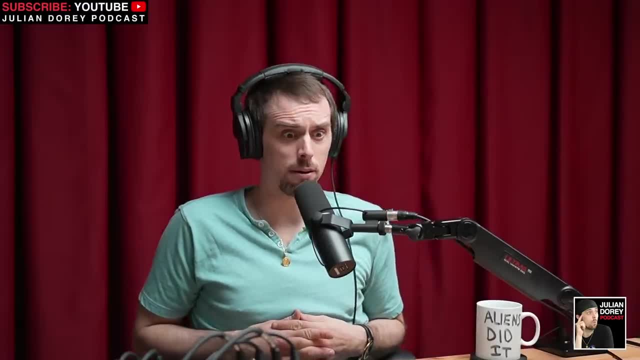 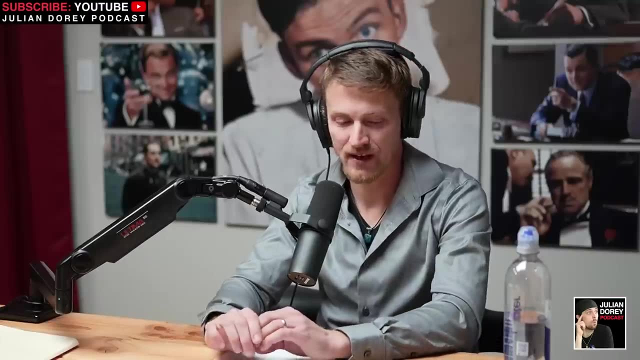 a good question. how do we know that- and i think about this- forget sumerian and stuff. i think about this with regular languages. when we're on social media scrolling these days, how do we know the translations are right? that's one of the things that i've studied very extensively, and i do have 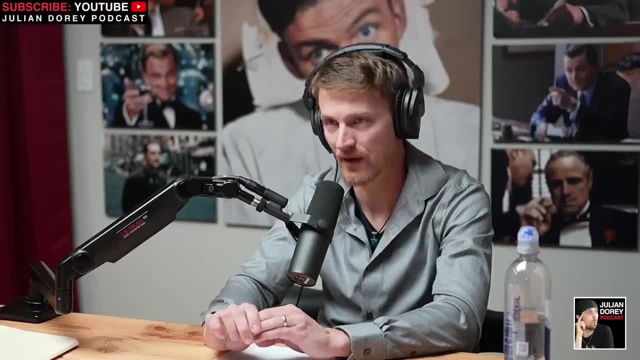 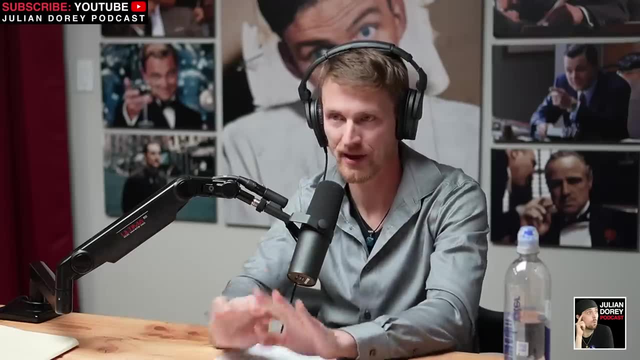 a lot of opinions about certain translators and people that have done that and i don't want to throw out some names because i don't want to alienate anybody. i will just say that the best translators in my mind in the world, cross-referencing and with 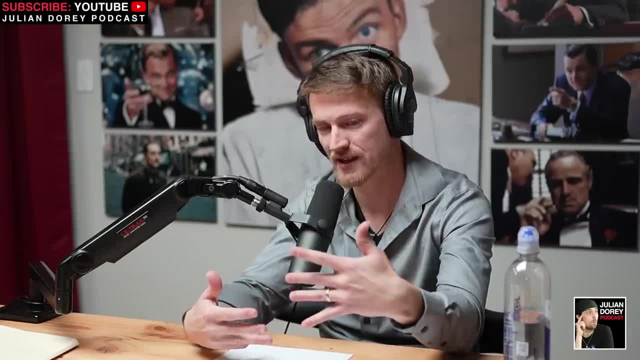 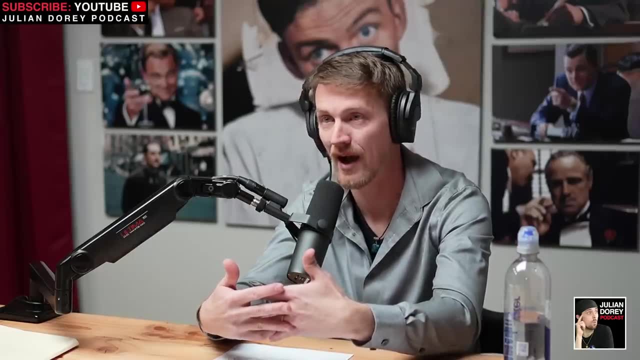 their credentials and then basically like, for instance, if george smith translated something and then someone else comes along 50 years later, do they? do they agree like? do they have the same type of agreement after all that time's gone by? is there disagreements and how something is is? 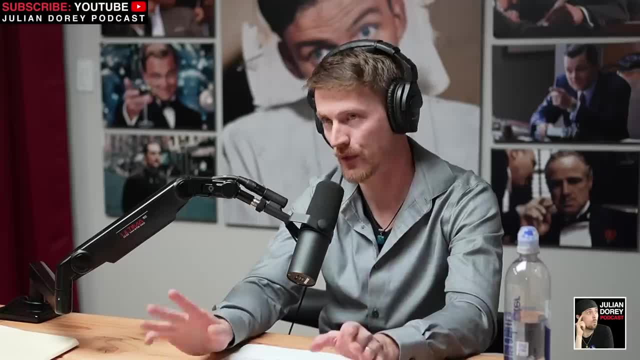 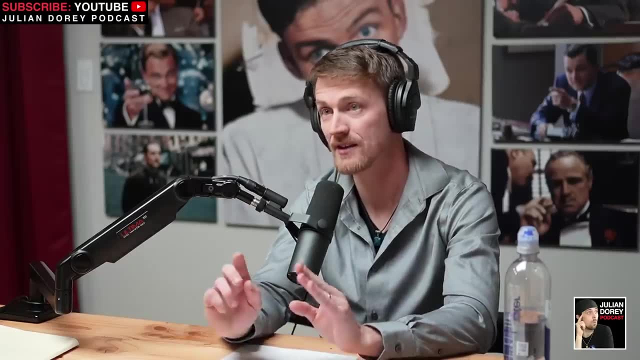 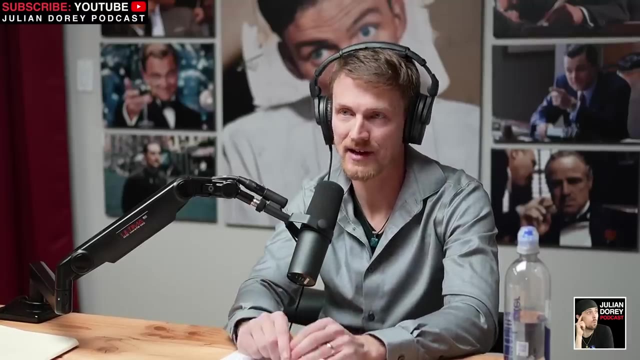 you know what i mean. and those experts, in my opinion, there are three of them, top ones, and that would be george smith, from the 1800s, and then samuel e kramer and then stephanie dally. why are they right? well, they are, in my opinion, the best academics that have studied. 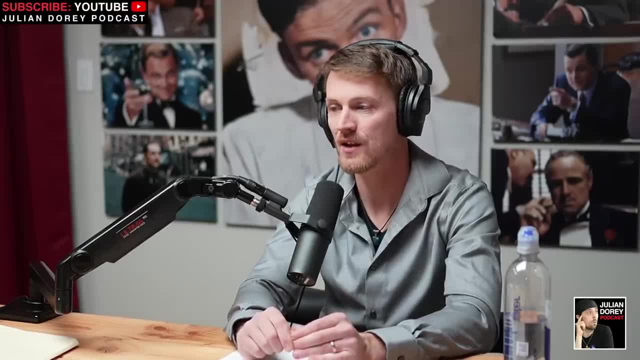 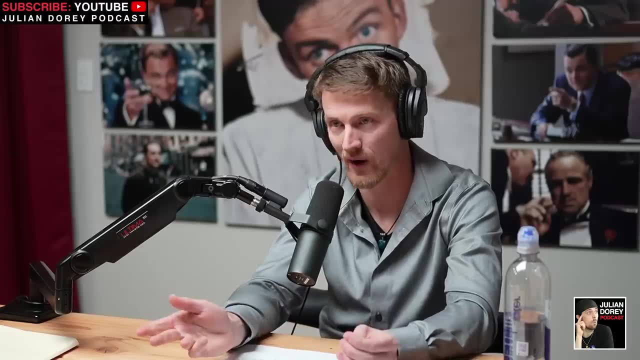 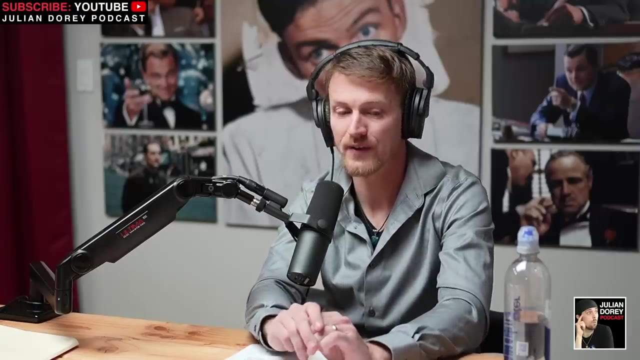 how to translate these texts in the most comprehensive way. they are what's called the seriologists, and the name is misleading because they deal with sumerian as well. it's not just a syrian, but there are other translators that have no experience, that have tried to do it, and i find their translations very inaccurate. it's very hard for me to think about it. 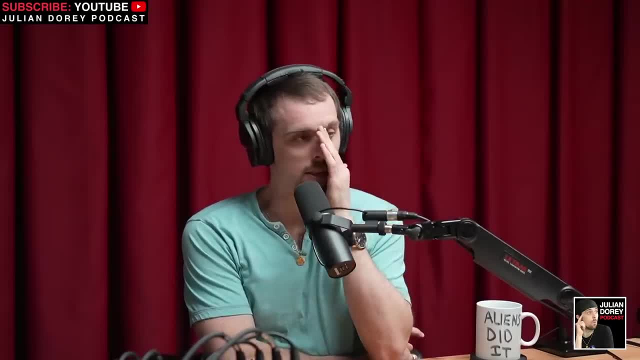 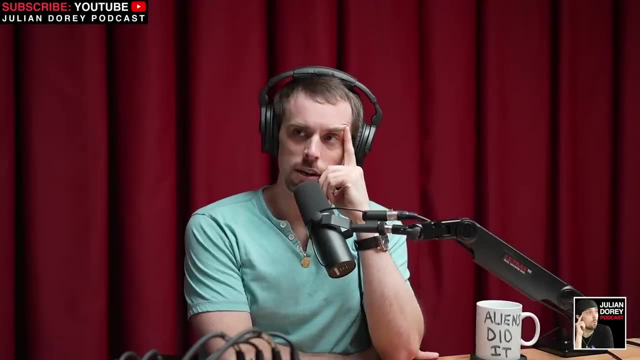 and i can't discredit them, and i can't discredit them, and i can't discredit them, and i can't discredit it or credit anyone in a way, because do we know how many people? well, first of all george smith figured out how to translate it. what was that? again, no one had translated in 2000 years, and 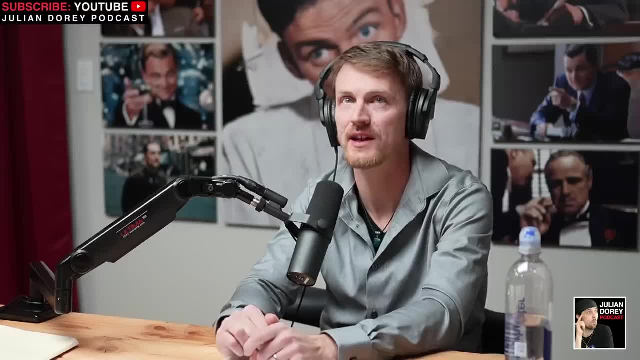 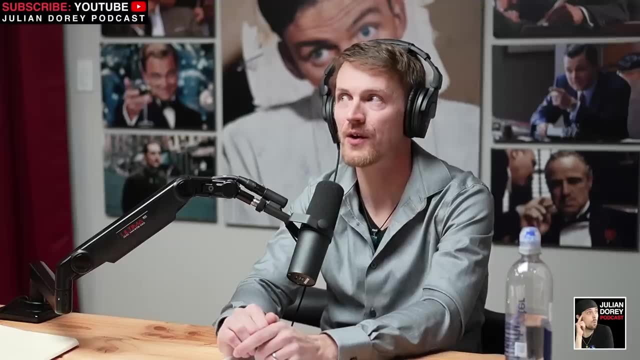 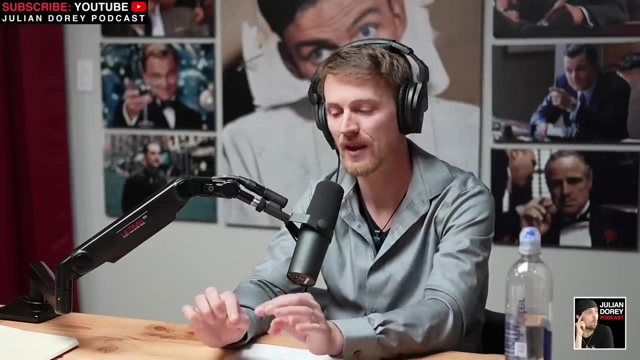 then he crossed the reference. no well, he cross-referenced. what he did, was he um? he was able to take similar meanings in the later iterations of what came out of that region, like: give me an example: a syrian has its own language. they write in cuneiform, but it's not sumerian, it's. it's a, it's an assyrian. 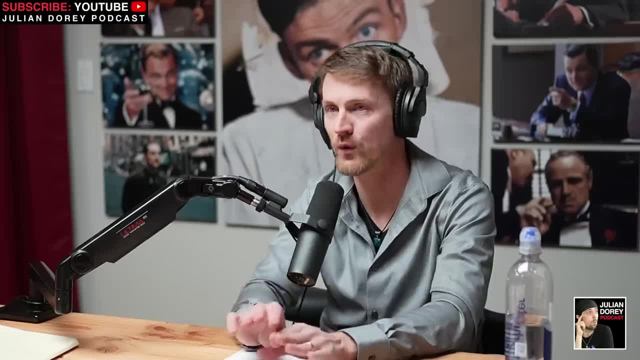 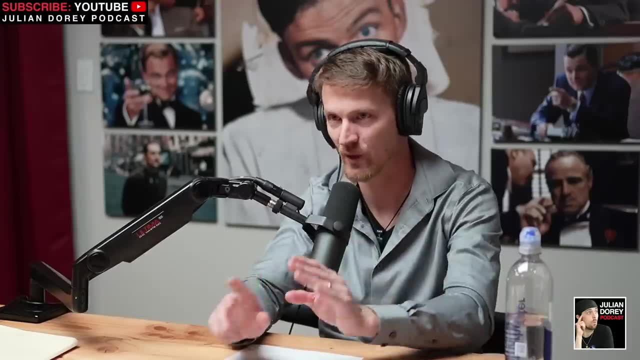 language. it's babylonian, has that too right? they're cuneiform but they're a different language. but they share some similarities in the regional, in regional understandings of what some things are. so if you take, for instance, in the syrian version of a sumerian tablet and you see the crossover, 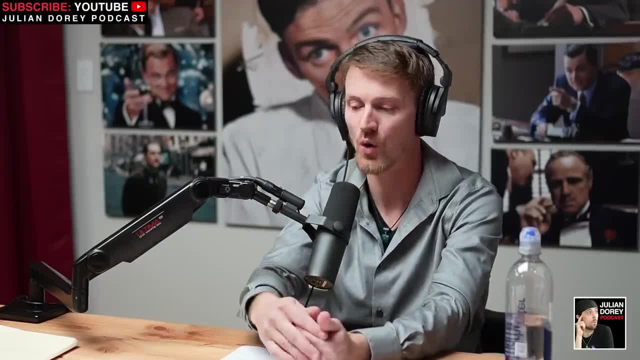 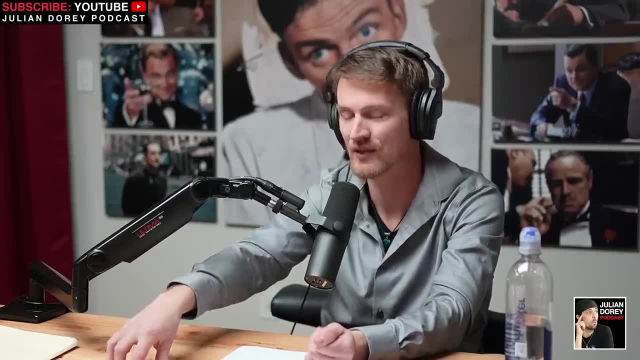 you can start to figure it out, because if you know like, okay, well, this is the um, like, for instance: give me an example: there's a, a syrian version of a sumerian tablet and you see the crossover, an original sumerian enuma elish version. but there's also a babylonian enuma elish. 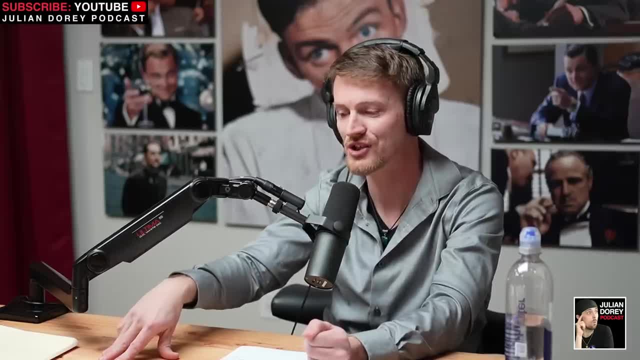 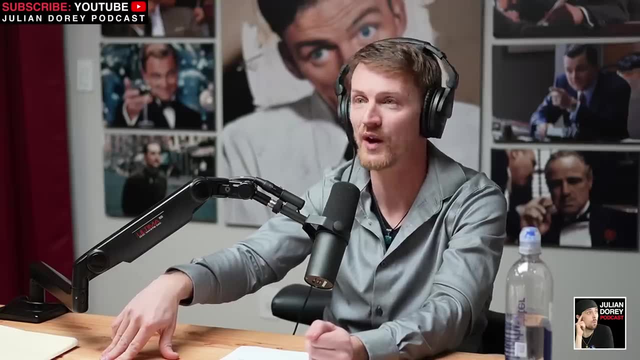 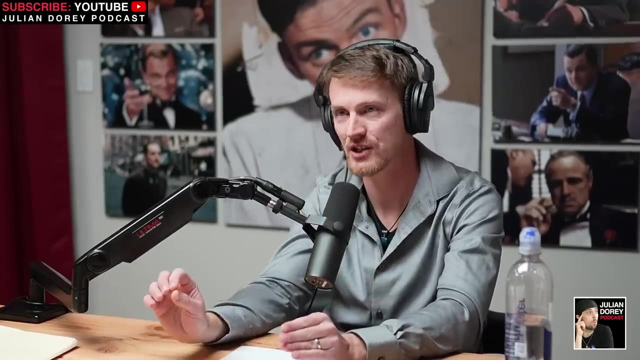 they're a set of tablets. the babylonian enuma elish um has these interesting changes made to it based on who was ruling at that time, making him seem more superior in some ways, and you can see these slight little iterations and changes in some versions, but the core of the of the stories, 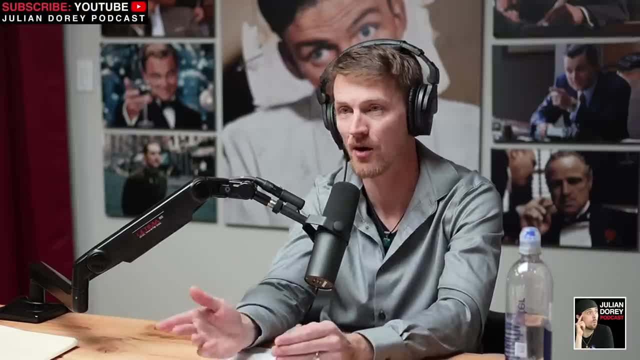 always remained in all of the versions. and he, he's got smartness and he's got a lot of knowledge and he's got a lot of knowledge and he's got a lot of knowledge and he's got a lot of- to realize that he kind of backtracked. that's how he was able to try to associate things that. 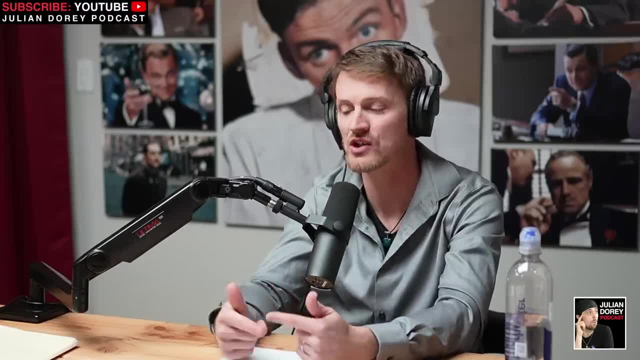 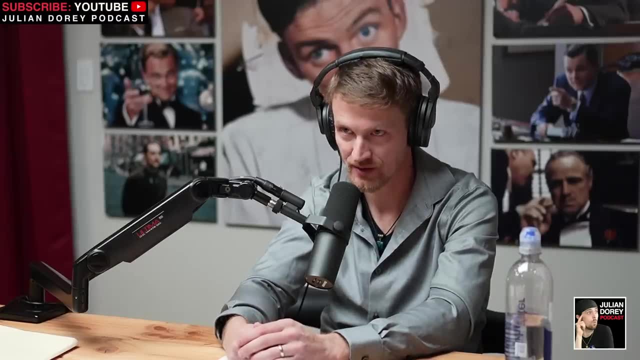 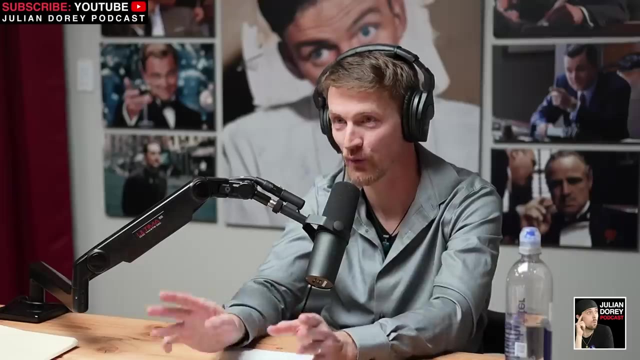 were related but not necessarily the same thing, and he had to. it was a very slow and painful process and it took him 25 years to crack the sumerian code- 25 years. that's why i told you when he was running around the room, after he figured out the epic of gilgamesh he had cracked. 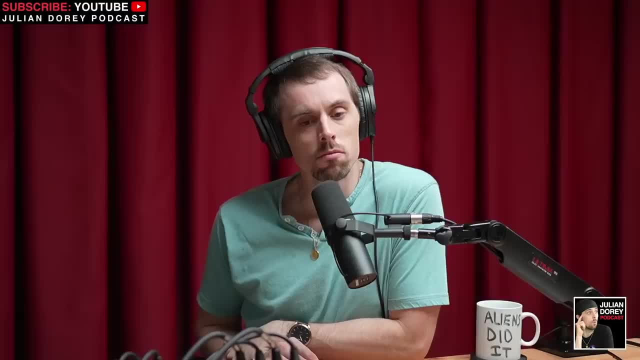 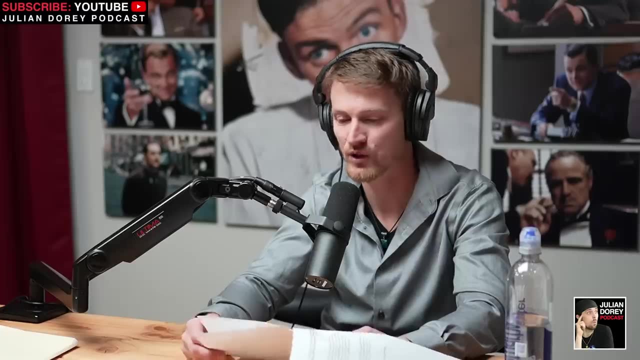 a code, then he was confident that he had figured it out. he was a very smart guy. now in i want to just read a tiny little passage here, very short, just because it relates to what we're talking about, but at the end of what's called eridu genesis- and eridu was the first- 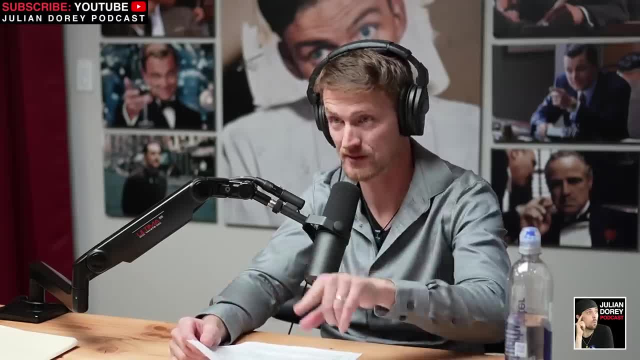 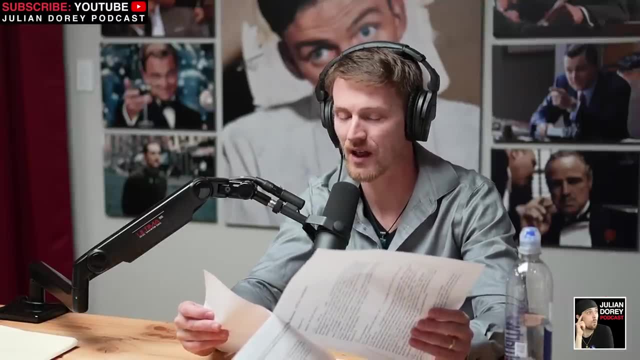 city supposedly ever created and then it was wiped out and then this civilization emerged. yeah, we talked about, and what it says at the end of the tablets is very interesting because it describes the noah figure as a lot more significant than we've been told in this, according to the sumerians, 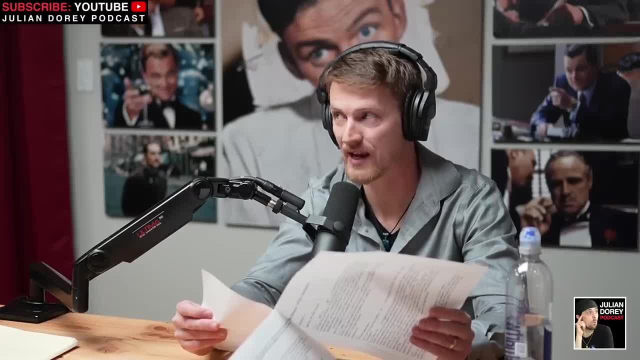 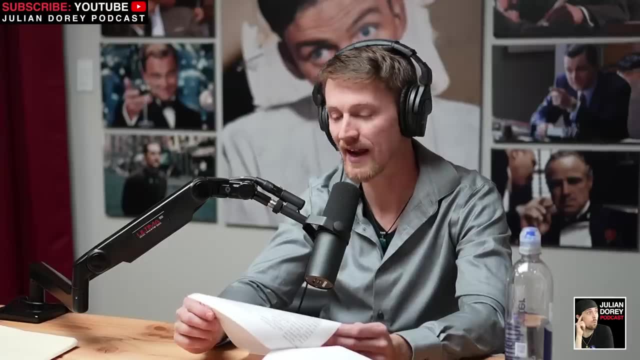 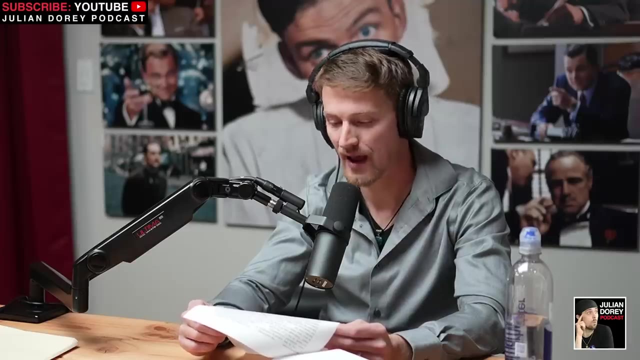 he was, um, like a patron, like a patron of humanity. because it says that right here, what do you mean? a patron of humanity? let me explain. it says zayasudra, the noah figure. it says zayasudra prostrated himself before on an enlil, so he's. 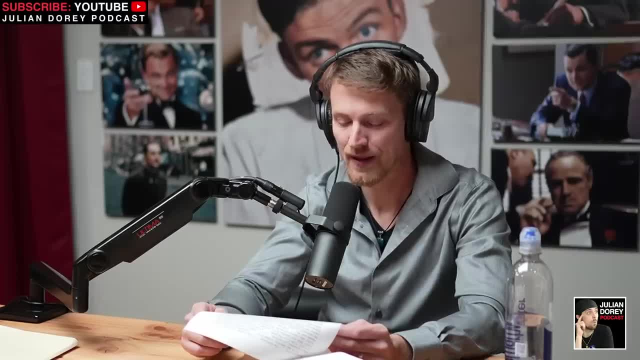 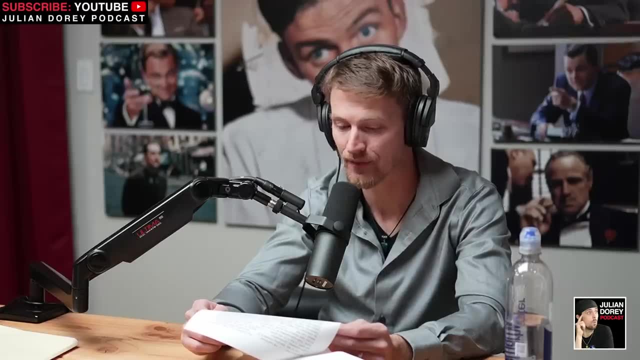 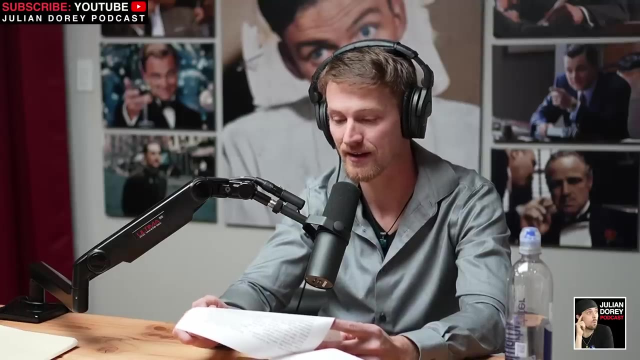 like anuna, gods right and they granted him life like a god. they brought down to him eternal life. at that time, because of preserving the animals and seed of mankind, they settled him overseas, in the land of del moon, where the sun rises, which is like saudi. 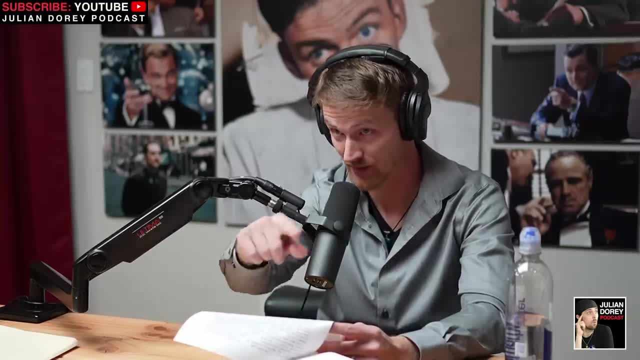 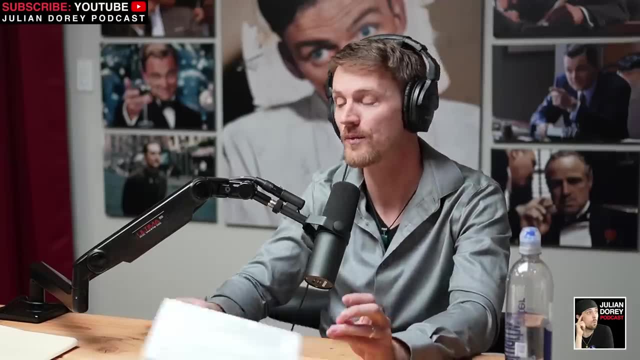 arabia, which is interesting that we have those cross comparisons in saudi arabia. back to this right. the point i'm trying to make is it says he preserved the seed of mankind. he alone preserved an ancient bloodline. it states that it wasn't like there was no other humans on the planet. 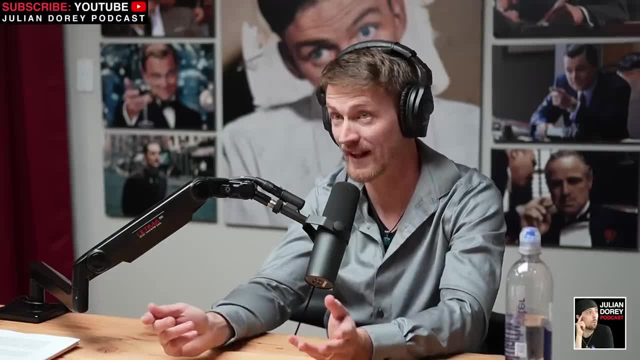 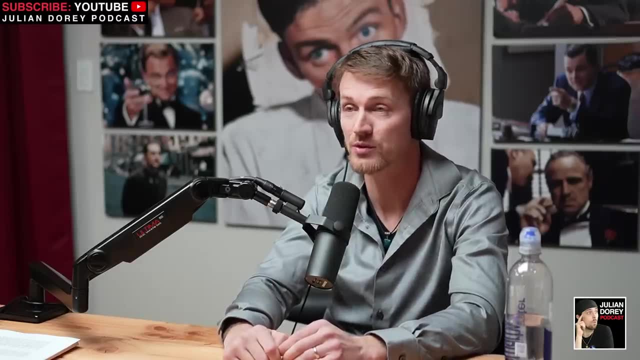 but there was a specific bloodline- which is what maybe relates to why there's a lot of that controversy and, uh, an interest in secret societies and certain groups throughout history- is that there was a certain bloodline that came out of sumer that supposedly had these gifts of the gods. 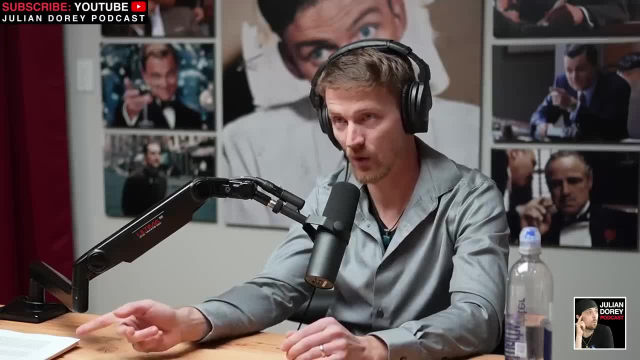 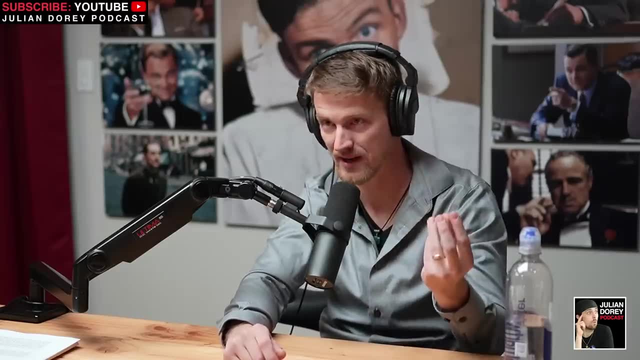 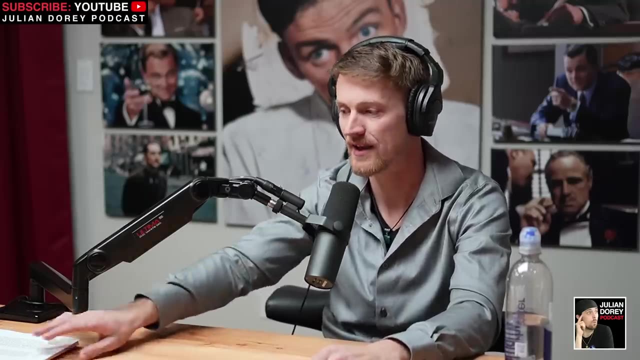 and that noah, the figure of noah that i just read, zayasudra- was the last of this line, this like divine line of these sumerian kings that had this connection to like demigods- almost it's what they basically were- okay, and it's described that in in this. 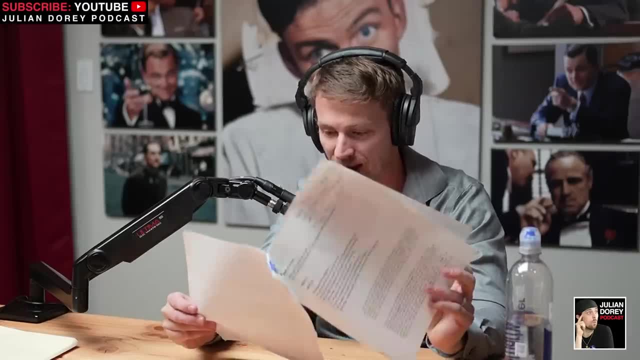 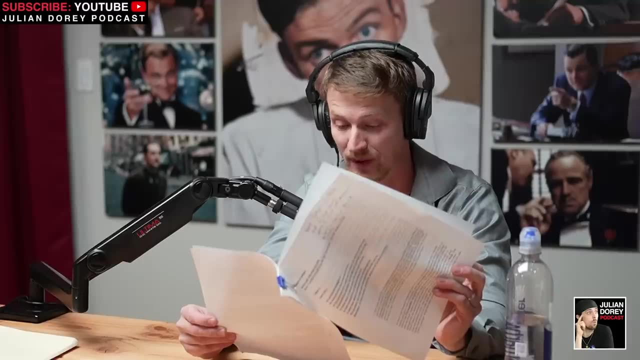 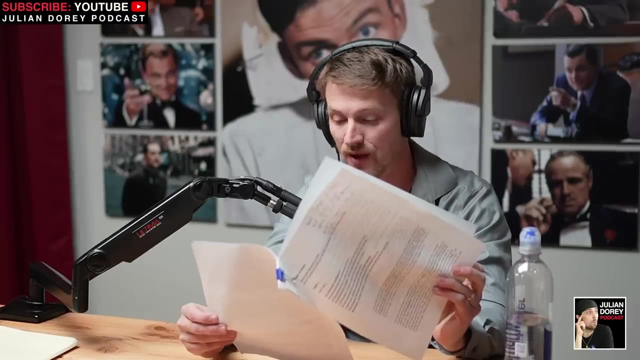 tablet that i just read to you. it says and- and i and i i want to, this is like absolutely, it's mind-blowing to think about. it says that basically, the gods in heaven, gods of heaven, of earth, took an oath to not warn any, any of the humans, and to create a catastrophe, to wipe out the seed of. 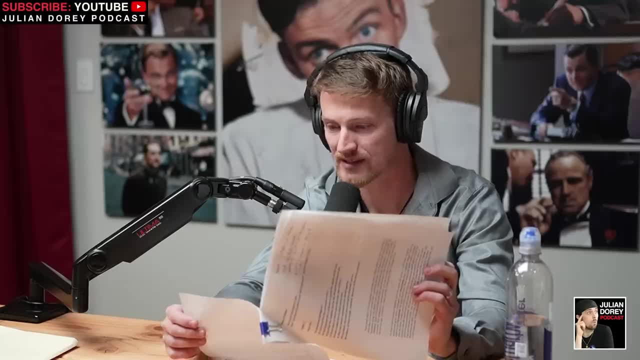 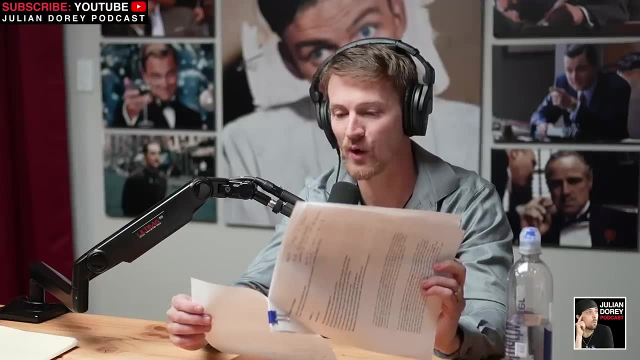 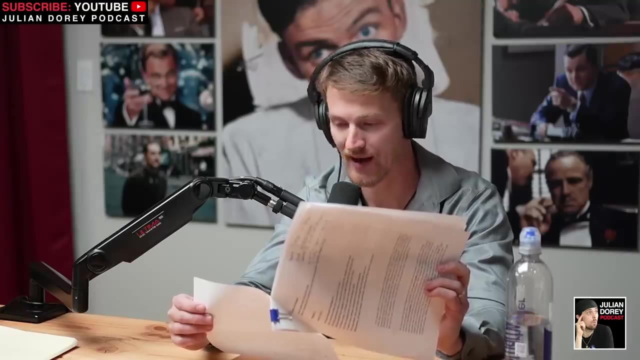 humanity. they really, they literally want to wipe us out. and it says right here, and i quote: right here: it says that a decision that the seed of mankind is to be destroyed had been made. the verdict, the word of the divine assembly cannot be revoked. the order announced by on and enlil cannot be overturned. 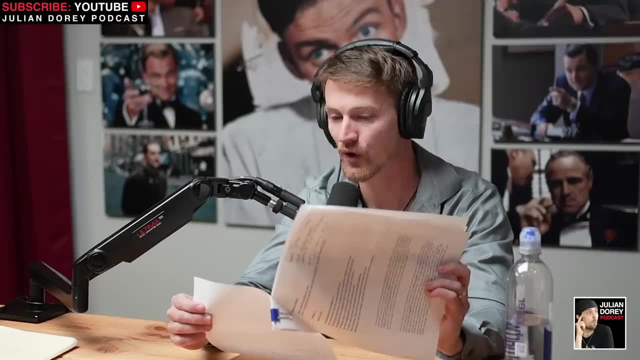 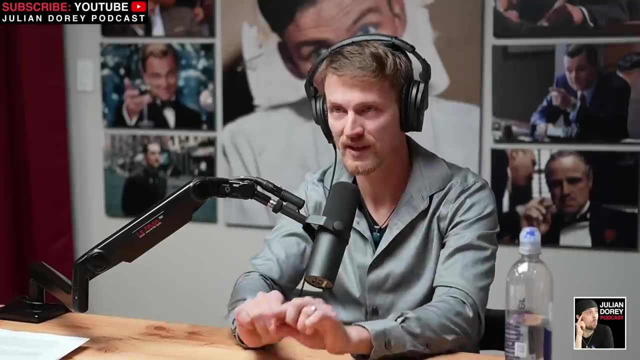 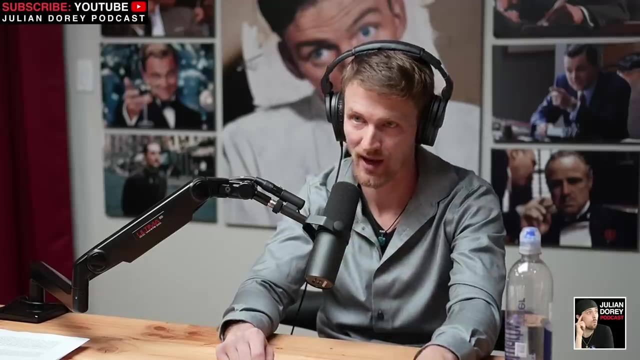 their kingship. their term has been cut off their heart. their heart should be rested now. now, and how old was that? that is one of the oldest tablets in humanity, that is, that was called the erudugenesis asher bonnepal library. that was found in the asher bonnepal library. eighteen, forty-nine, there was part of. 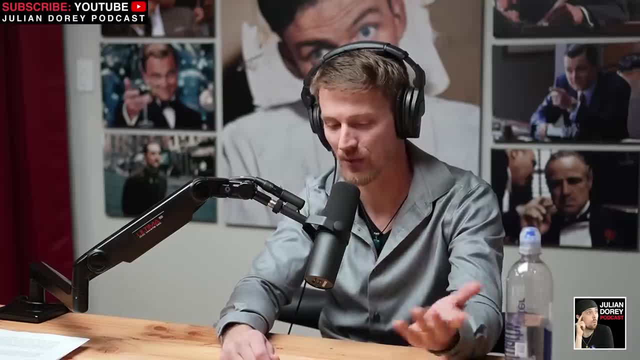 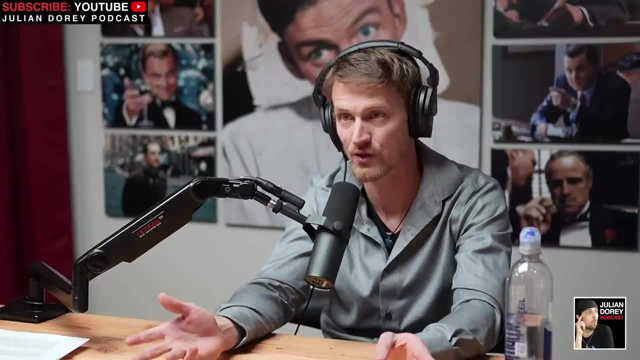 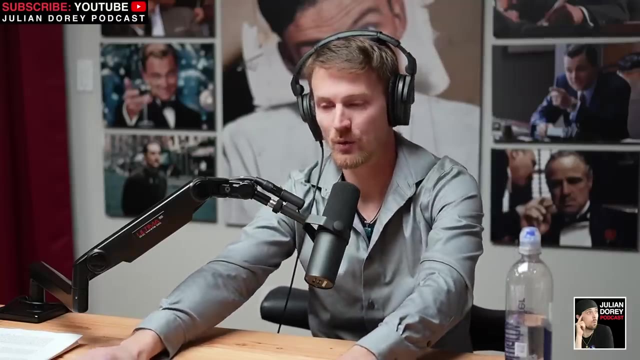 these original core ancient teachings that were handed down, descriptions of what the, this ancient time that we have long since forgotten. uh, what it described as right and how did we date the asher bonnepal library? and well, we can date asher bonnepal because we do know when he lived, so we know asher bonnepal lived somewhere. 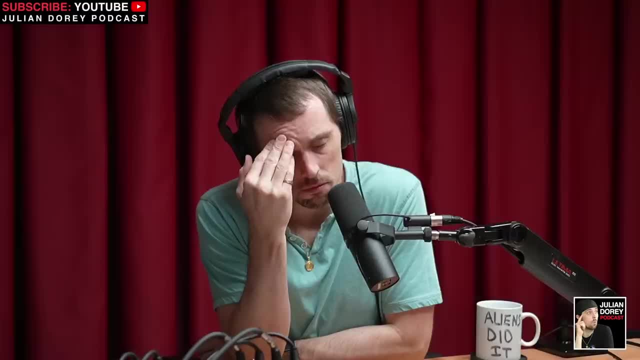 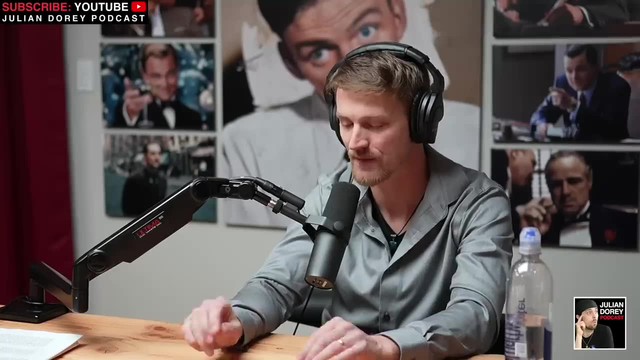 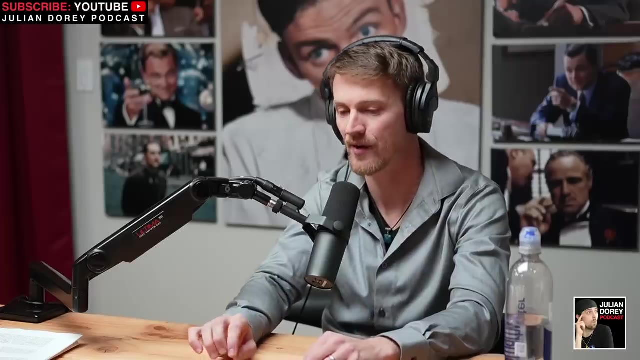 around like two thousand five hundred years ago or so, right somewhere around there, and it depends, cause some of those dates are a little bit off if we want to look at that, but it's that's the time period he was. he was living in um 2,500 to 3,000 years ago Now. he, Ashurbanipal, amassed that library and he describes: 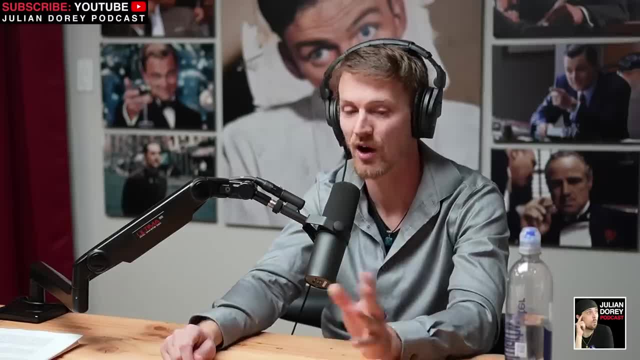 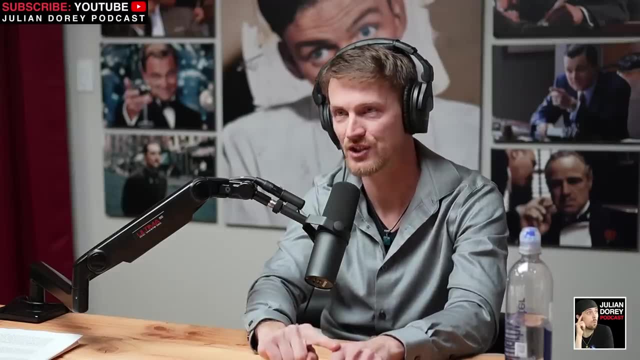 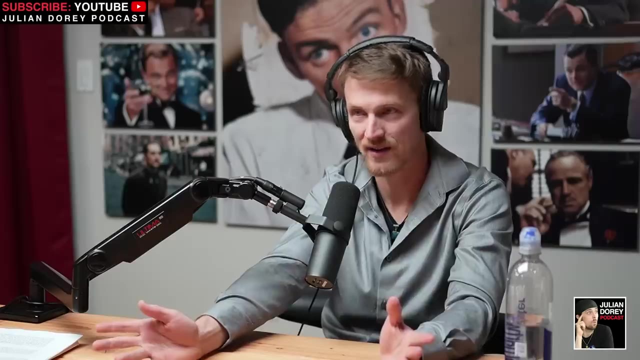 in when he was he, he did. he left some things behind where he talked about his empire and his rule and things that he's done, And he mentions how those tablets were already ancient before they went to seek them out in in Amasa library. So he's like 3,000, right, 3,000, 3,000 plus years. 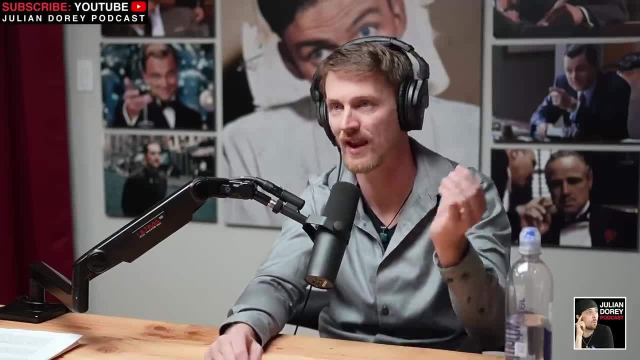 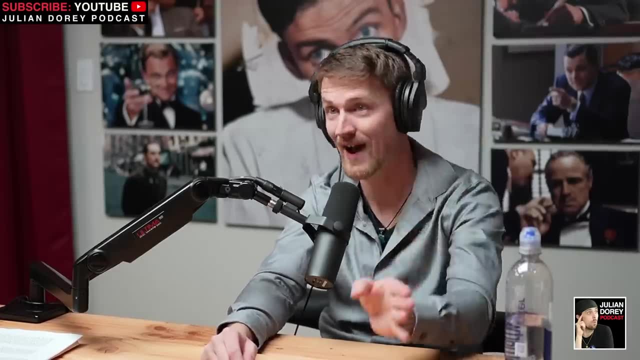 old And he's already mentioning that these tablets are so ancient that he happens to know about them because he's a king and a priest and he's part of that bloodline that survived from those original Sumerians. And they discuss how they're like, divinely chosen to rule and all. 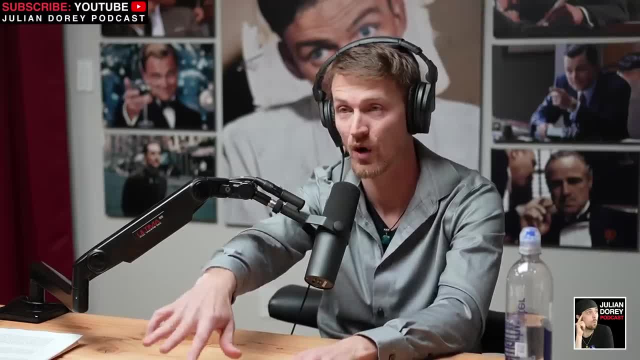 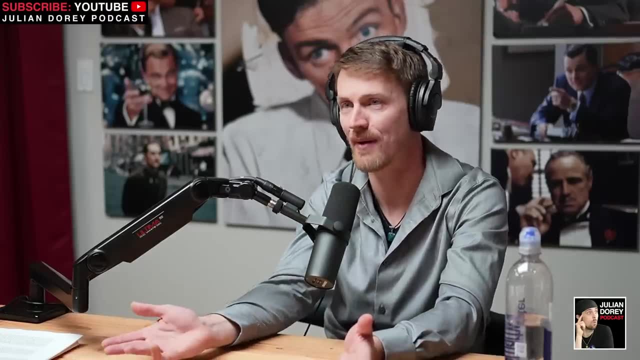 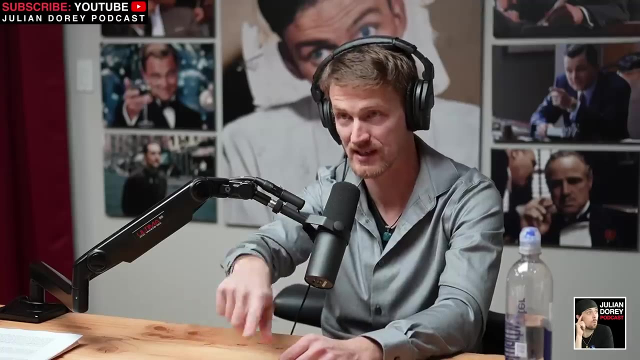 these different things. Okay, The point- what a point is on how it connects to all these discoveries- is that those tablets tell us a story about what happened, but we had no evidence to back any of it up. That's what happened. That's the. that's how this basically unfolded, And when I discovered these, 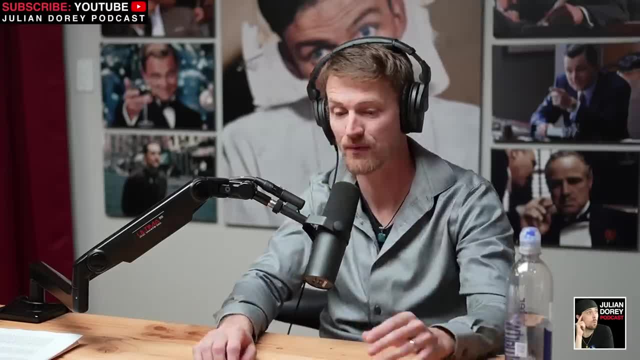 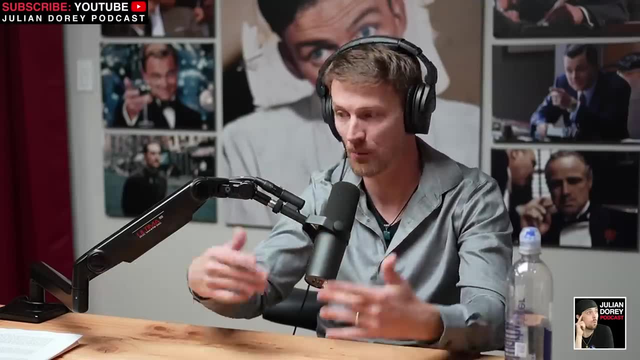 sites around Lake Vaughan and then found, like we mentioned before, like at Kavis, had an ancient king list. that literally says directly: King Haik, a descendant of Japeth, you know, built this incredible temple like right. There's actual translations from that And they actually state: 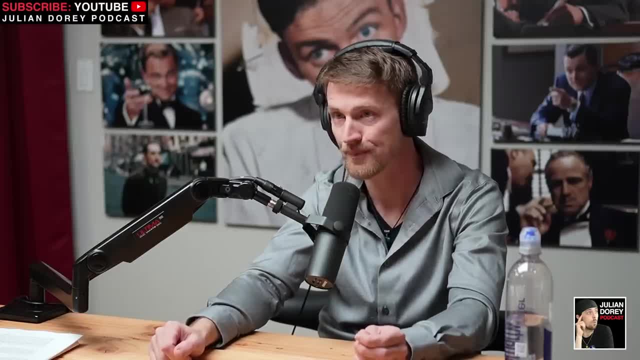 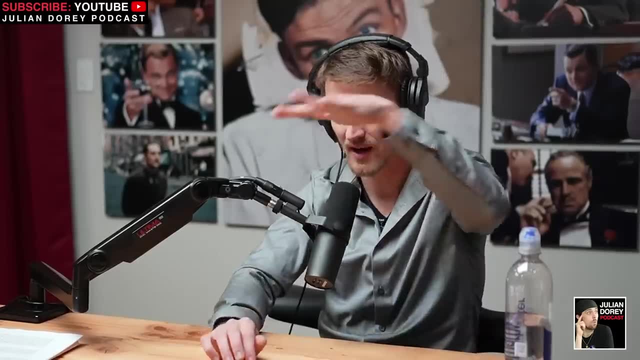 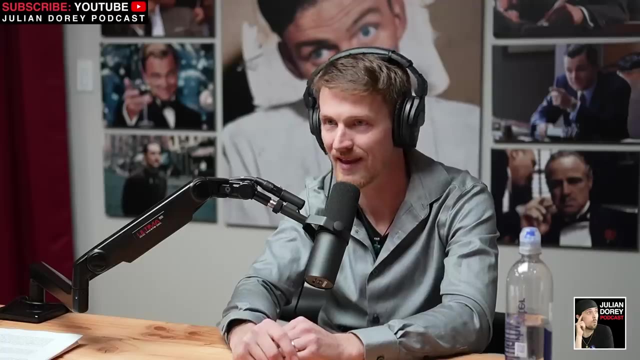 they are direct descendants of Noah. Okay, Hmm, In that, in the translations of these ancient sites, But not only that. the megalithic blocks, the design they have for these temples, should not exist. Why not? There's nothing. there's nothing around it Like it. 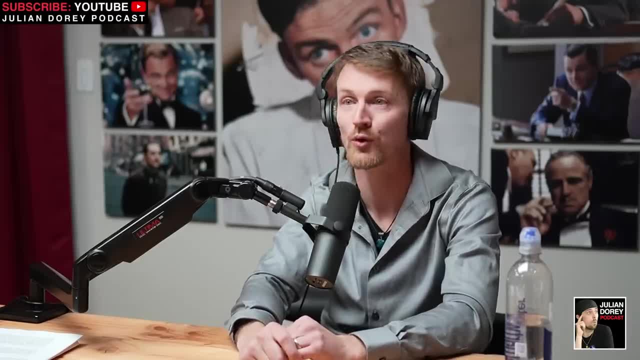 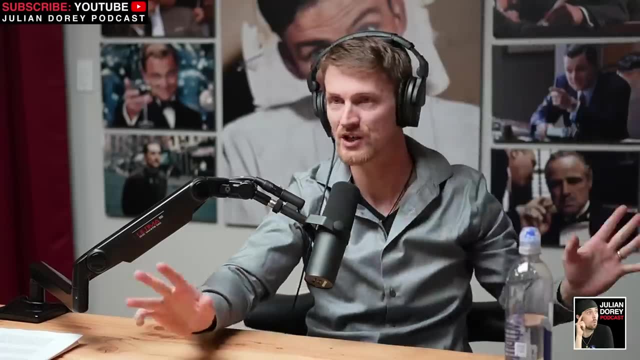 if you have a civilization that builds a bunch of megaliths, like meaning example, like Peru, if you go down to Peru and you go to like Cusco and you go to Saskatchewan and Ollantaytambo- all of those ancient sites are in a region. There's a bunch of them. 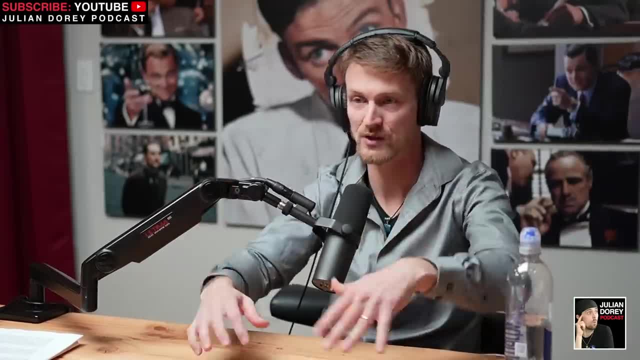 right, They're all in this region, They're all part of the site. They're all part of the site, right. They're all part of the site right, Absolutely of like this emergence of an incredible civilization. but you can't just have that. 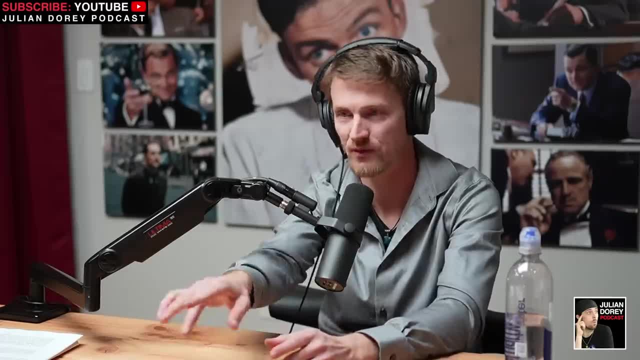 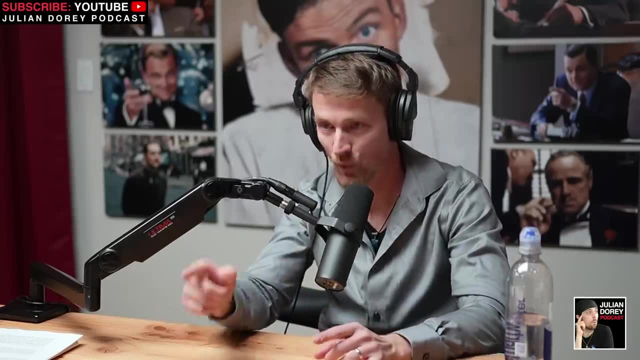 somewhere, with no reason. you can't have a hunter, gatherer civilization build that. they don't know how to do it, they don't have the tools to do it, meaning that that shouldn't have existed where it is based on conventional thinking. it was like it was like an anomaly, and i noticed that. 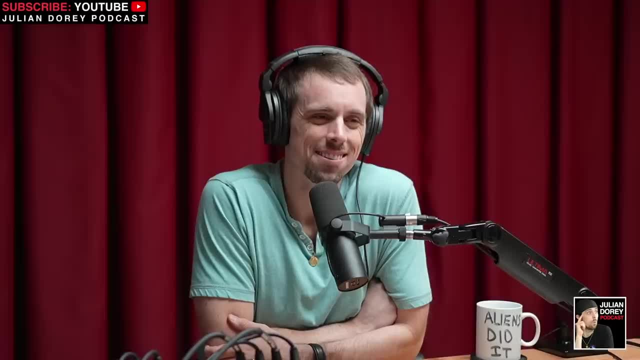 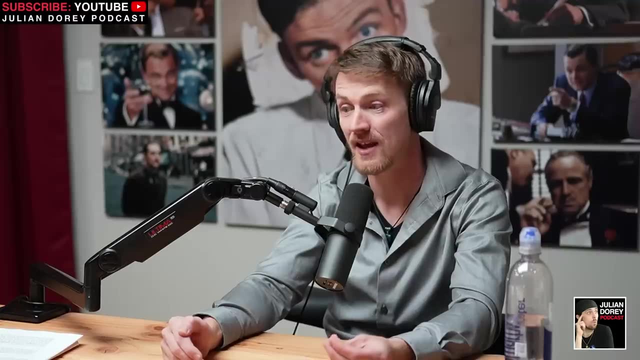 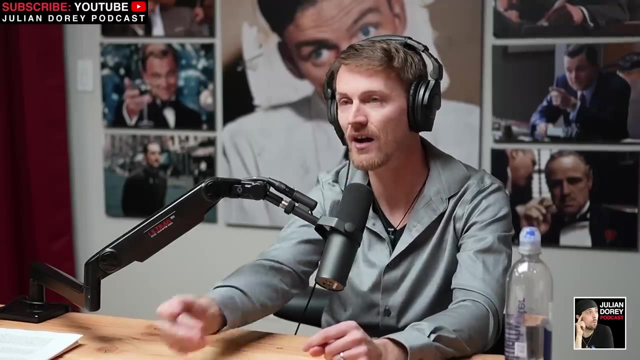 right away. being a megalithic nerd, i'm like i've never seen that those, those walls, those stones before. where is that? and that's how i fell into. this was very much by accident, and i realized the scope of how big it was getting. now. ionis was like the icing on the cake, because ionis 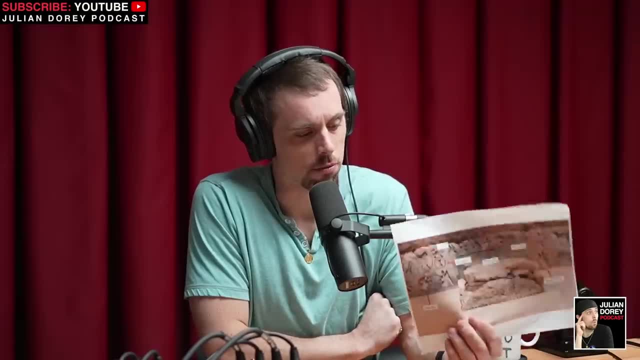 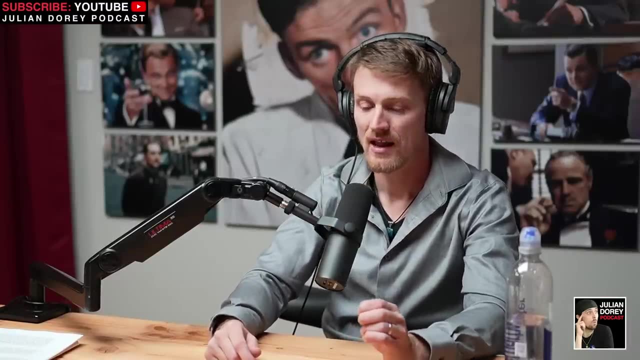 is where that's. just reminders back to this. yeah, yeah, and- and i was telling the story about it- remember i told you about those incredible megalithic walls they built as they were going up. well, that was 1989. it took them 30 years to reach the temple. 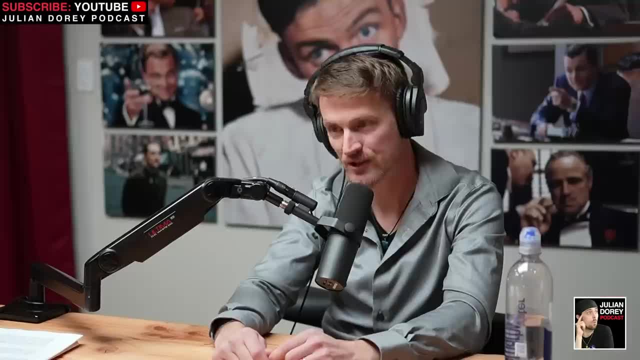 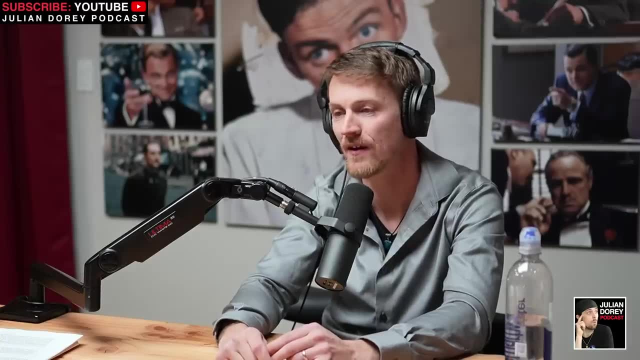 30 years. yeah, this is down there. so imagine that they find these walls that are highly sophisticated, incredible, and they're working their way up and they get to the top of the hill and then they find where they think the temple is, but they have to go down 20 plus feet and then they eventually 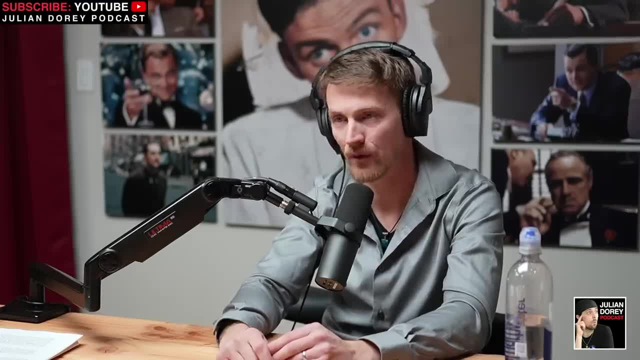 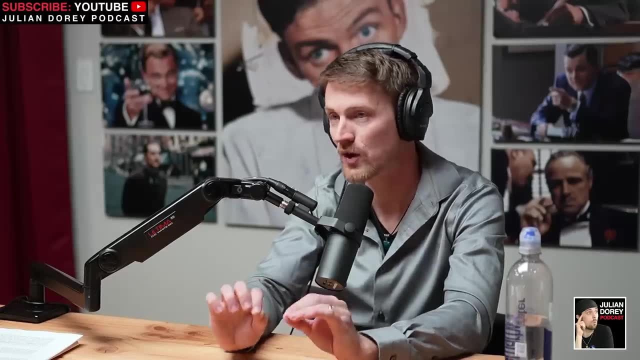 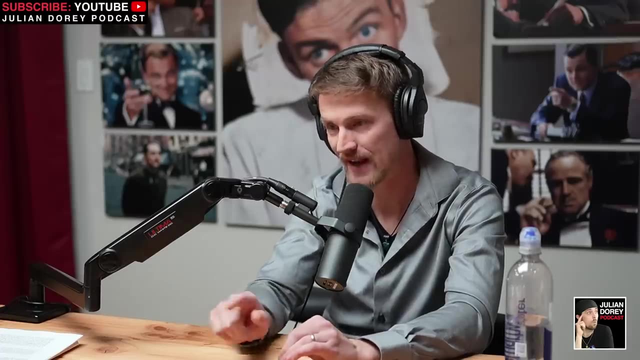 discover the remnants of a destroyed temple, and i've i've seen all the photographs of when they first found it. it was literally in ruins, destroyed, and they intricately pieced it back together over the course of five years. five years it took them to put that temple back together and they did it in a beautiful, beautiful. 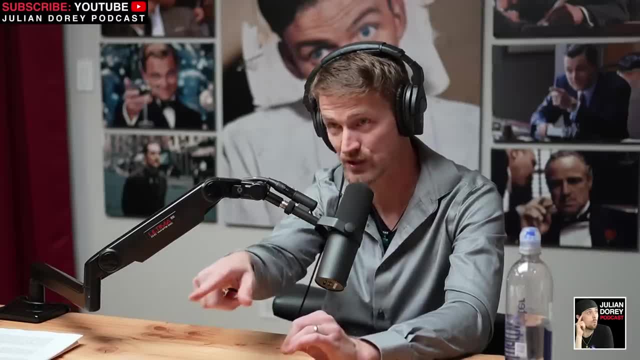 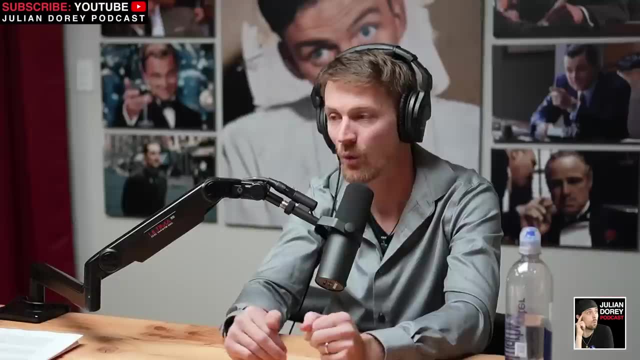 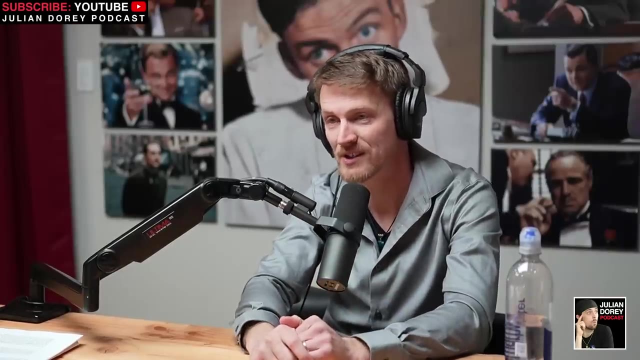 way like. it is stunning, but that stone that you're seeing it at that temple is called again. i said it's andesite- right, why is that a big deal? well, explain that please. andesite is one of the hardest stones on earth. when we look at megalithic structures around the world that are mysterious. 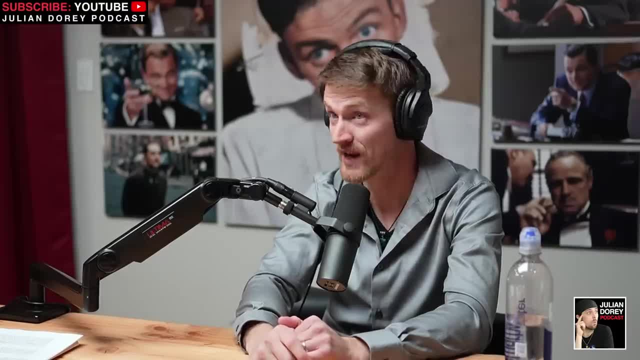 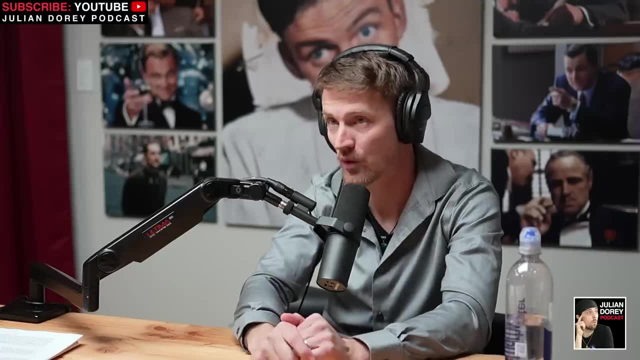 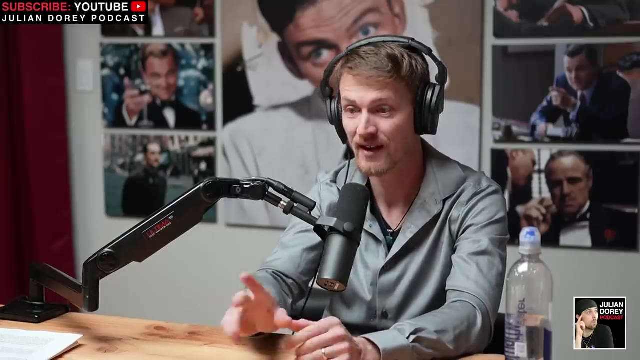 whether or not it's peru or it's uh bolivia or egypt. a lot of the stones that are around the world are the megaliths around the world don't have any symbols carved into them. most of them don't. now there are a few places that do, for instance, pumu punku in tiwanaku in bolivia, does and lake vaughn. 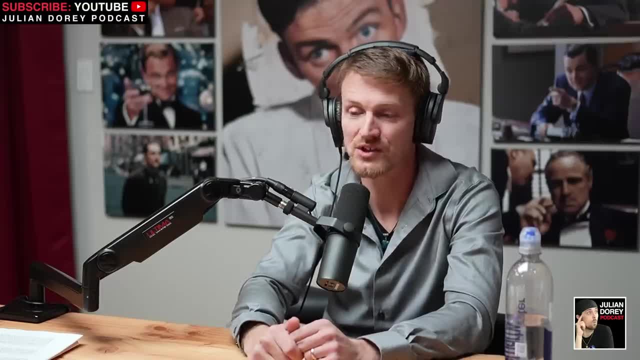 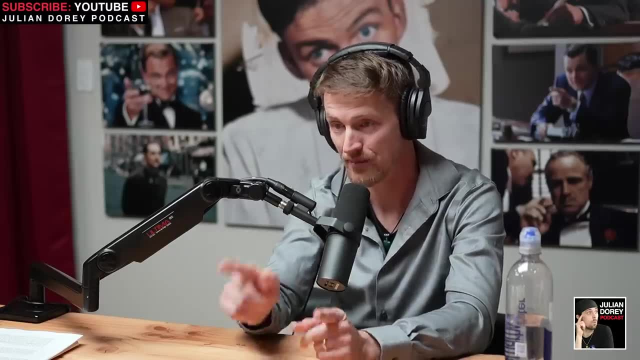 does, and what's unusual about that is they say they share almost the exact same similarities. they both build with andesite. almost no other place around the world built with andesite. both locations seem to be mimicking each other and that's what got my attention as i started to be. 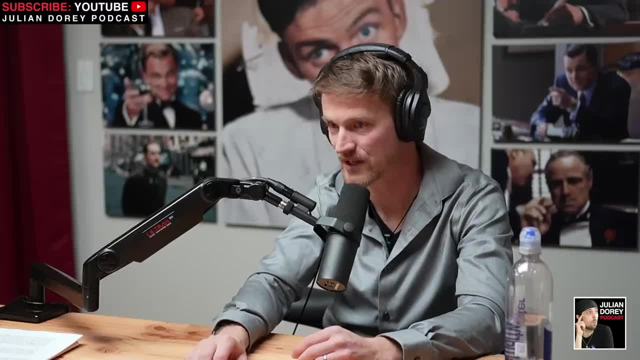 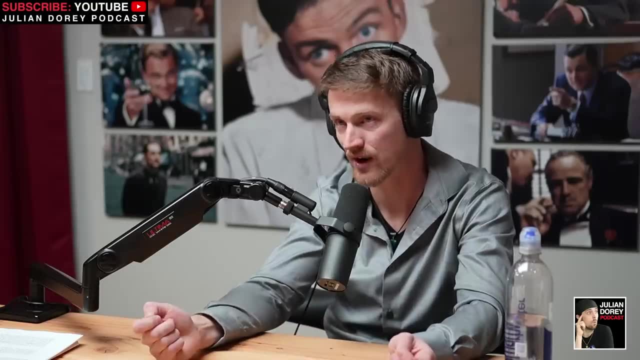 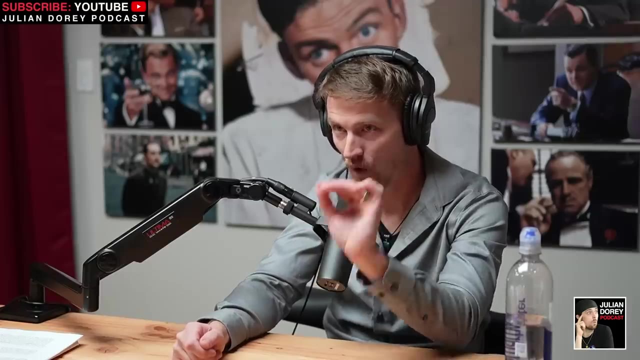 like, wait a minute. what if lake vaughn in the era of civilization is some kind of an origin point? what if it's an origin point for this mysterious lost chapter in our history that we don't really understand? you know what if it's the origin point behind the great pyramids of giza, all the great temples? 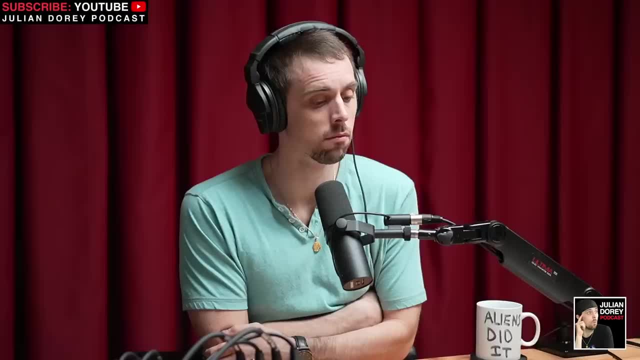 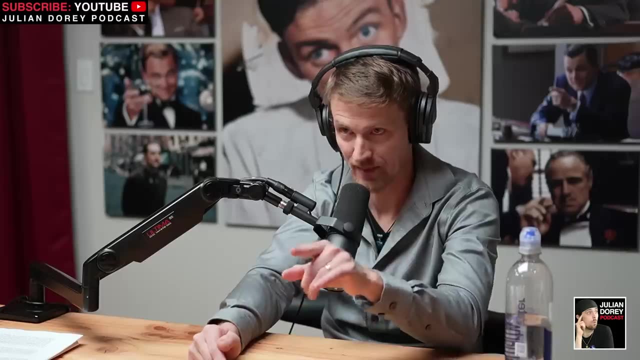 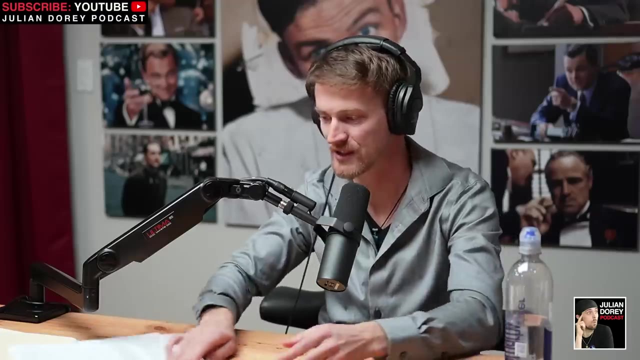 around the world. what if it came from this? imagine if something was lowered that had never been lowered before. and i can say that confidently because when we look at the original sumerian cities, they specified to them and they actually did it on purpose they talks about in the tablets. it actually says laying bricks in pure spots, like all, all throughout. 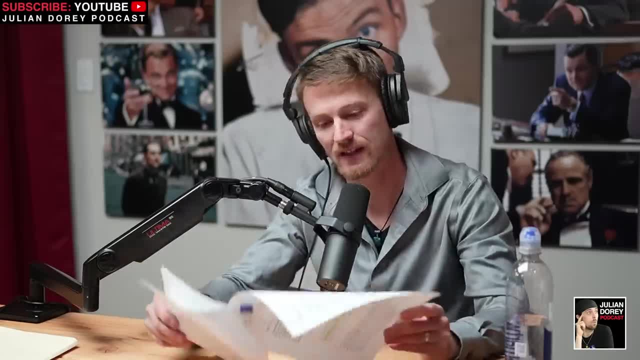 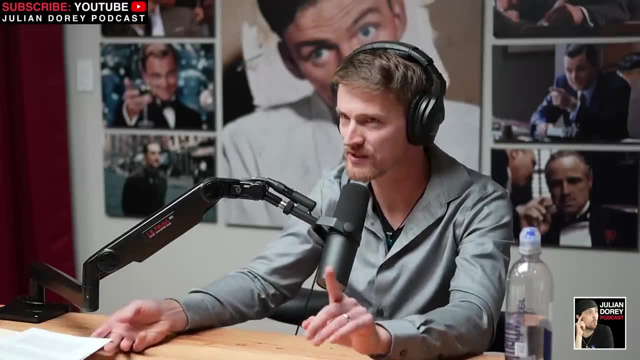 the tablets. so like brick was very much intentional on their part, like, for instance, the legend of says: right here it says: the ajiji founded its brick work in pure spots. the sumerian civilization was only building with brick. that was what they did. okay, the urartian civilization later on. 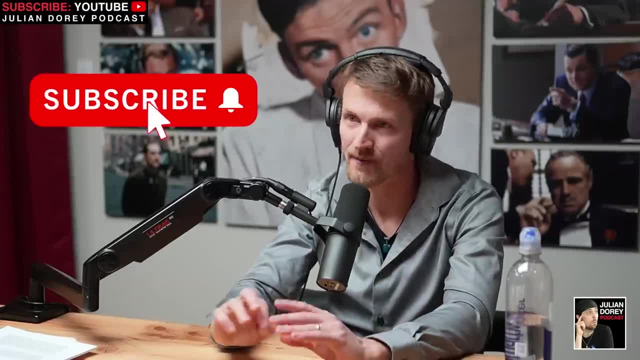 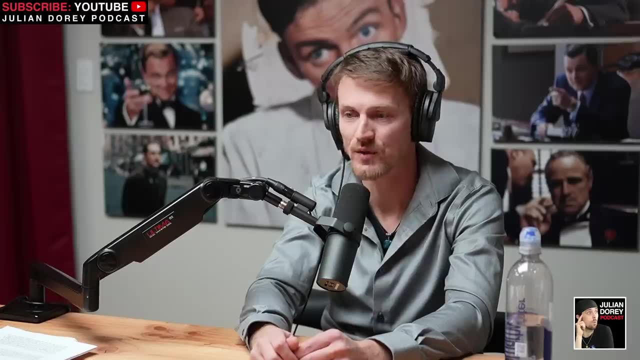 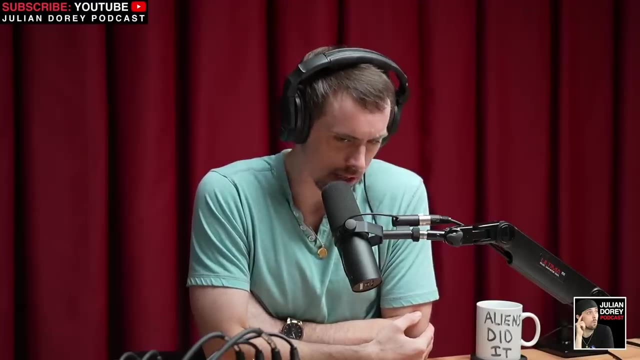 only built with brick. brick in these. it's like a very high-end construction. it's like a very high-end primitive type of building. um, but that civilization didn't? they built with these giant stones. only two types of stone. they built with basalt and andesite. what was the? the stone we discussed last time was: 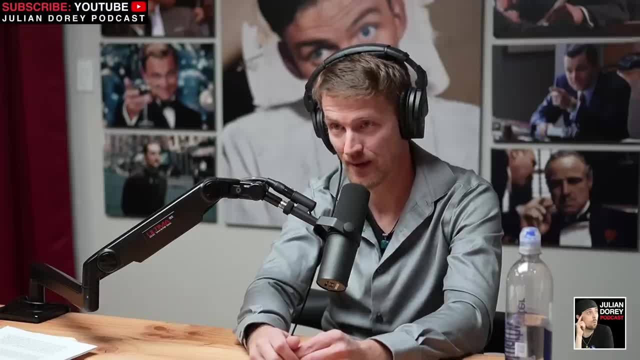 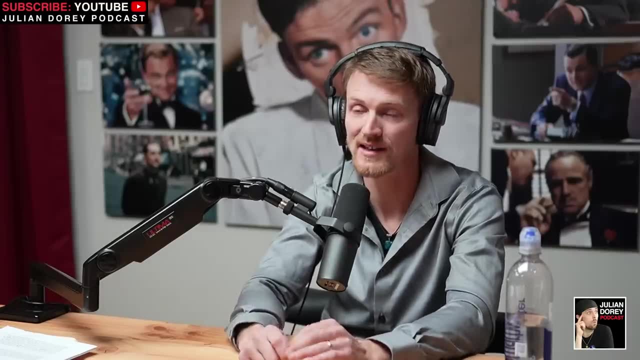 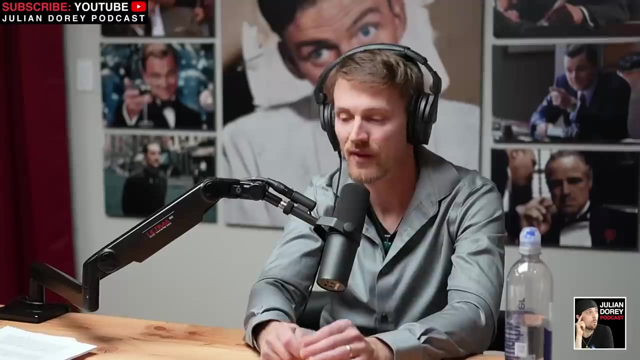 that a cavistepi. that was the basalt, the cavistepi, yes, yeah, very similar, very hard, very, very similar. actually, that site is a combination of the two stones, but the point i'm trying to make is that stone is so hard that it proves the age in itself, because how well it number one, it shows evidence. 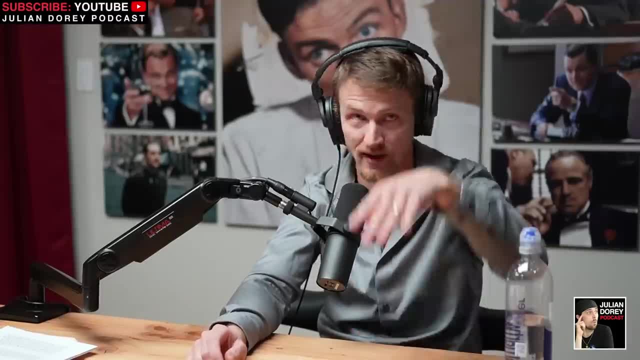 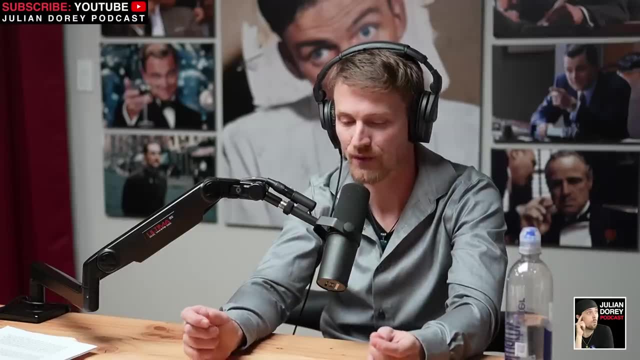 of an absolute catastrophe that was buried in ancient below all these layers, like the erartian civilizations above it. right, so you get that. you get that differential time period, but what you also get is you get the fact that if you had a culture that that was going to carve an andesite. 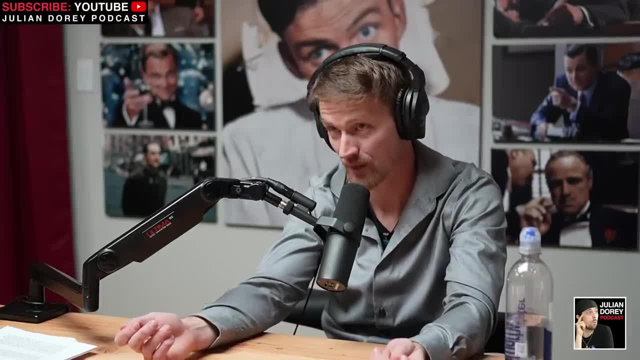 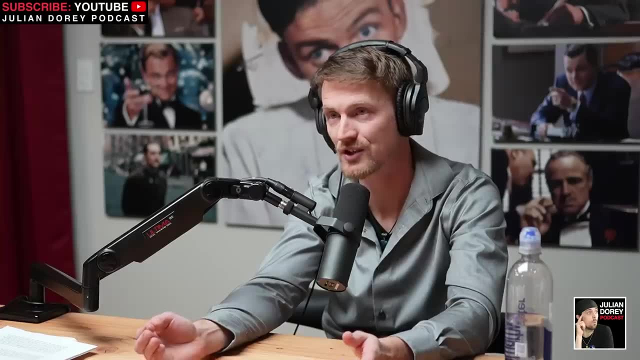 they would have a certain level of technological sophistication to do so. because you can't. you cannot manipulate a stone that is harder than the tool you're working with. it just doesn't work. it doesn't do anything, like if you go take a piece of plastic and go take a piece of granite. you can't do anything. you can. 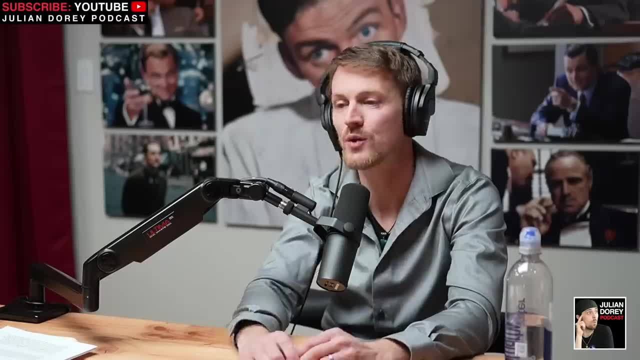 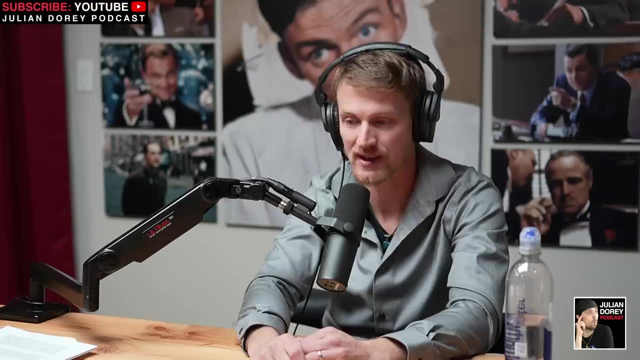 do whatever you want, it's not going to do anything right. so they had to have something. they had to had to have had highly sophisticated advanced tools to be able to create these, and i would go as far to say that something like that basalt box relief that we're looking at right now from 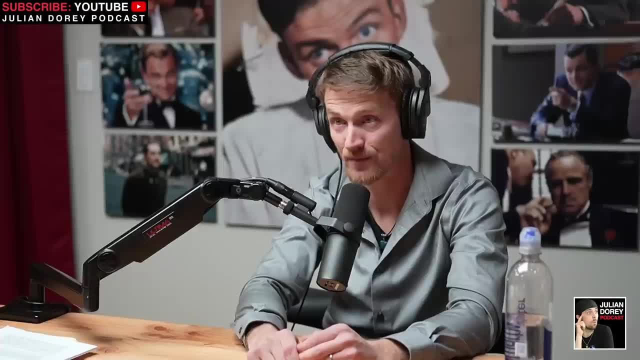 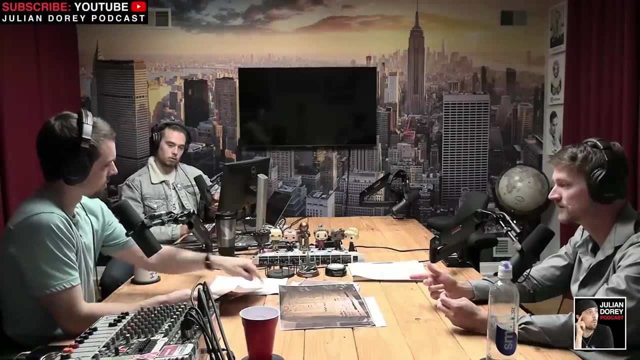 kef temple. and what was this made out of? again basalt, basalt, again. that's. that's a six on the hardness scales right below andesite. yeah, unless you just, i mean, i think you know this, but we're just, we're basically switching between these two right now, just for your own notes here. 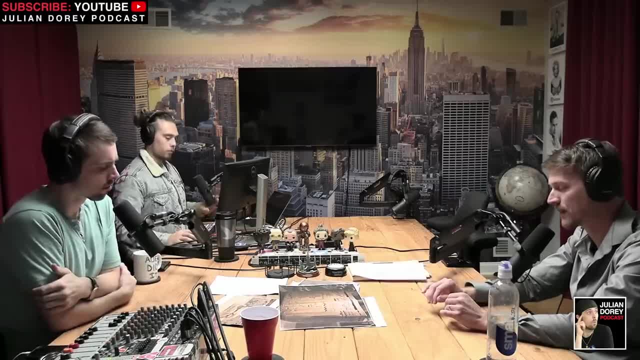 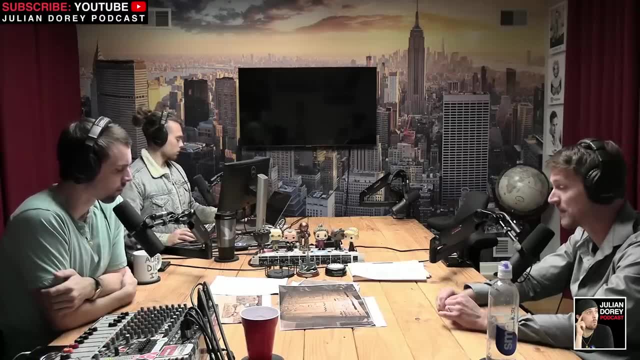 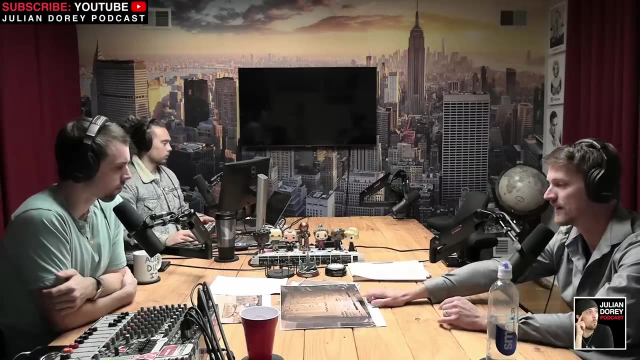 now what i'm, what i'm trying to say is: look at that box relief for a minute. i don't believe, based on what i know about stone masonry and and from the people i've talked to that actually have experience in that- they've told me too is i don't believe that we could create. 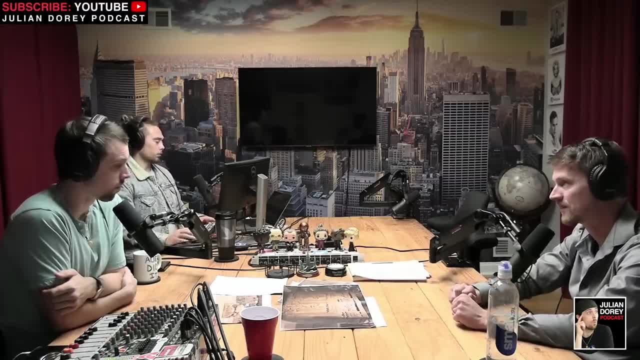 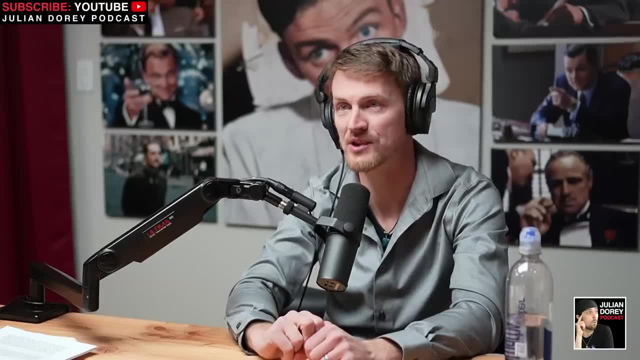 this box relief by hand today? today, you don't think we could do that, not by hand, with it, maybe with, maybe with like one of those types of computers that it's almost like a 3d printer where it goes in and cuts it out. maybe are you saying, i'll bet we could do that well. 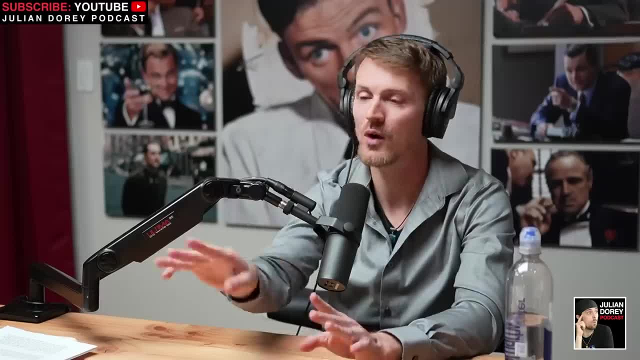 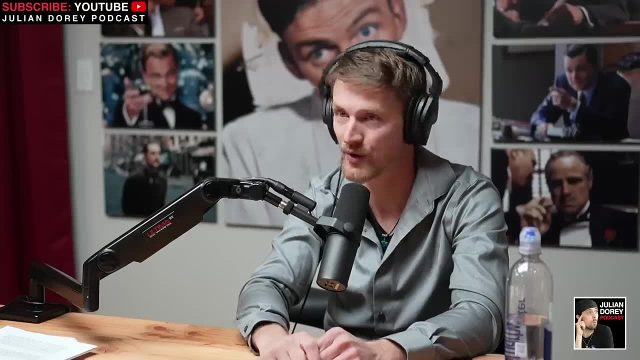 i'll give you an example how i don't think we could with the computer. well, no, no, with by hand right, all right, but are you saying that? maybe i might be way off base here? i'm not saying they created the computers, no, okay, i think that they were using. 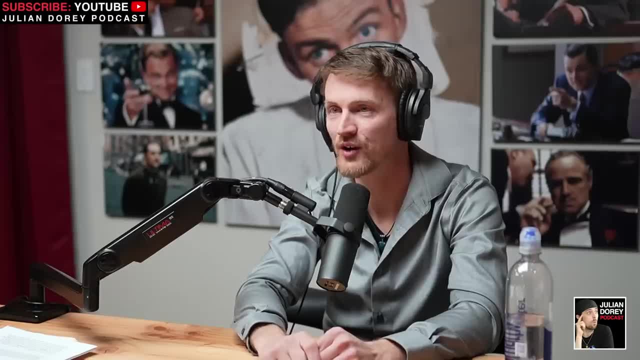 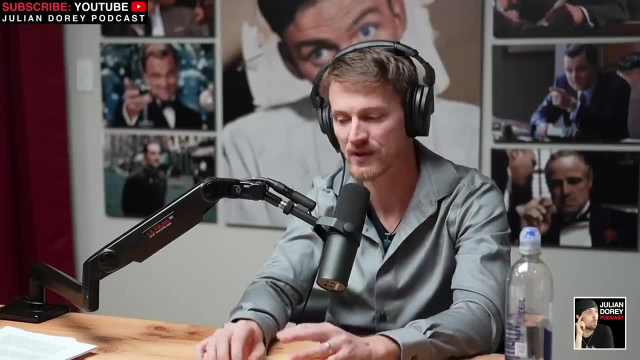 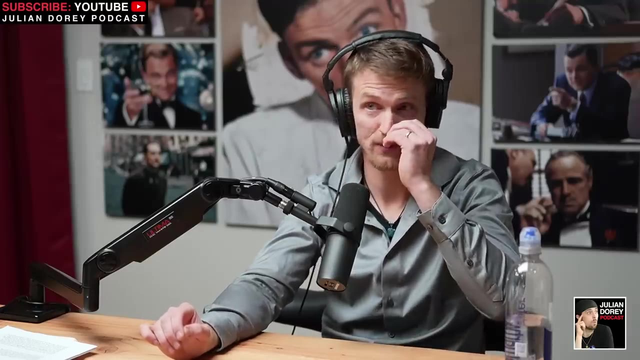 you're about to ascend. you're about to send me. i think they were using technology that we don't understand. it's been discussed often that the evidence that is shown in different parts of peru and bolivia and other places- the stone masonry looks like it was partially melted. now whether or not that was. 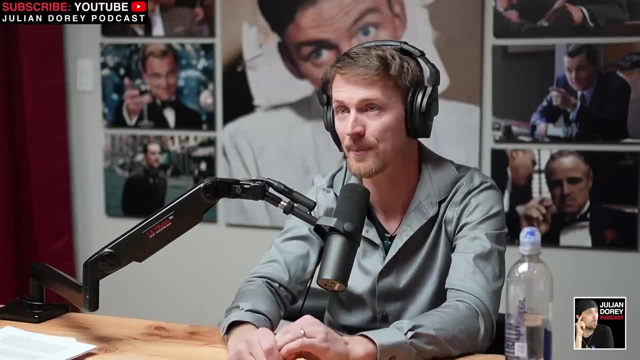 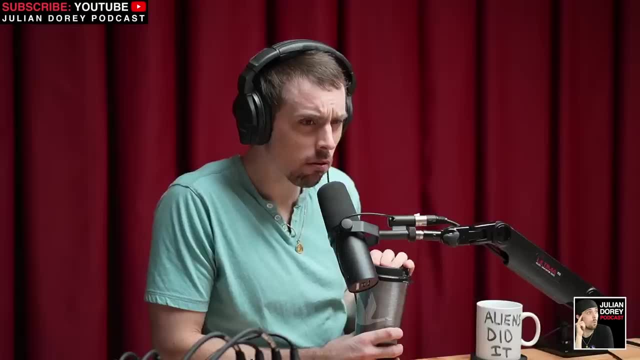 from an event on earth or it's part of their mechanism for creating them. if you were going to put some of those polygonal stones together, like at oyay tatambo or saks kigelman in the way oyay tatambo or saks kigelman, in the way that oyay tatambo or saks kigelman in the way that oyay tatambo or saks kigelman in the way that oyay tatambo or saks kigelman in peru, if you were going to put them together. 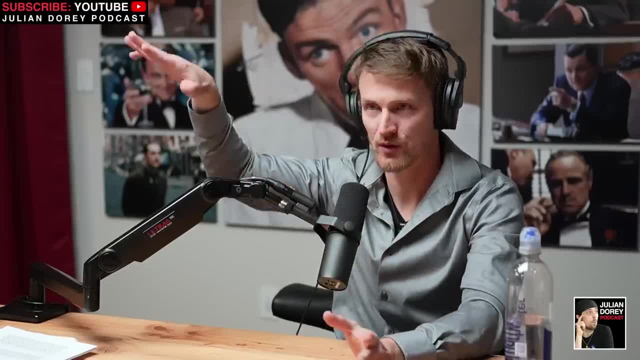 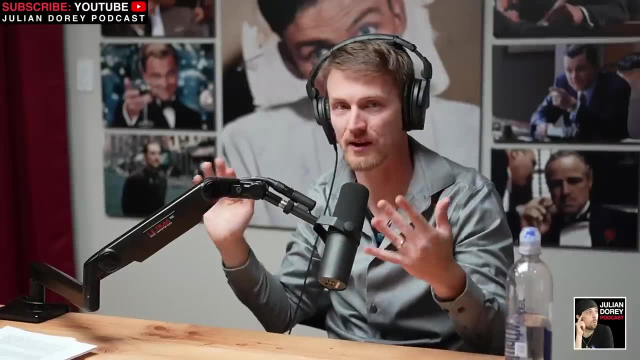 sorry, repeating a couple. no worries, i just got to make sure. but if you look at those stones and how they're put together, you can't even put a razor blade or a piece of paper through them. they're put together in such a way where they're like blocks of like- uh, like legos almost, but they're. 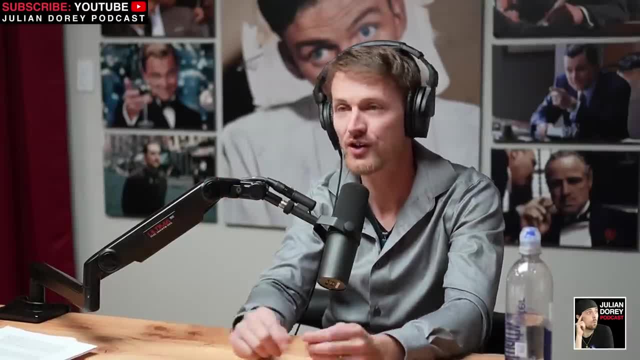 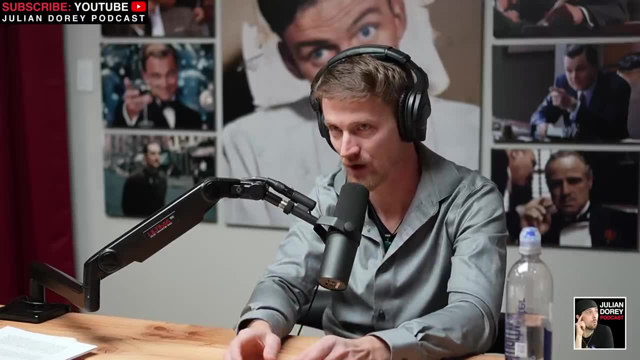 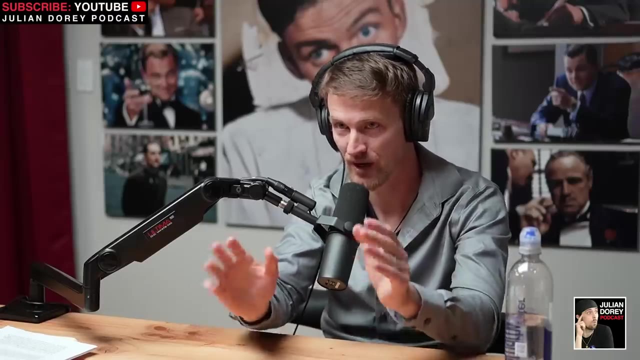 perfect. how would you be able to do that? you couldn't do that by hand carving, because you wouldn't be able to get those, those perfect edges to line up. what if you heated the stone, though, and made it like somewhat loose, moldable, put it into place and then let it harden? that's more like what it's looking like. 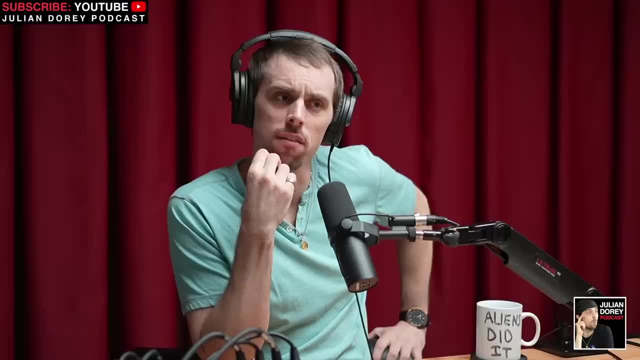 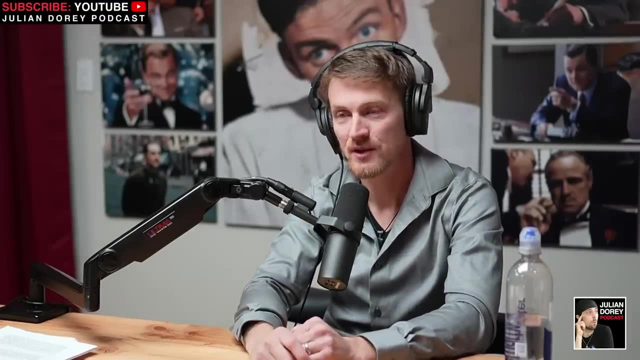 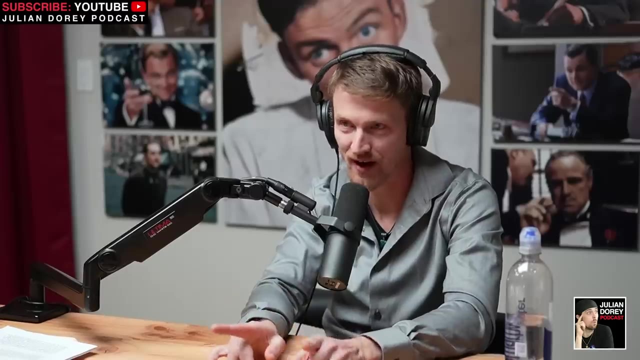 they made it like building these giant walls and these different things. how would they have done that? have you ever played with a magnifying glass? you ever, when i was a kid? yeah, you ever that kid. well, i was proficient enough. well, i was. i was proficient enough, though, that i actually would. 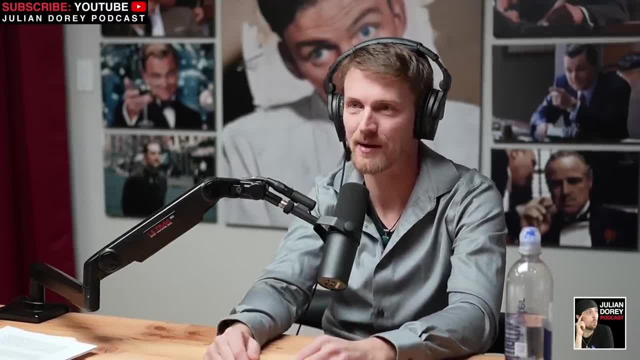 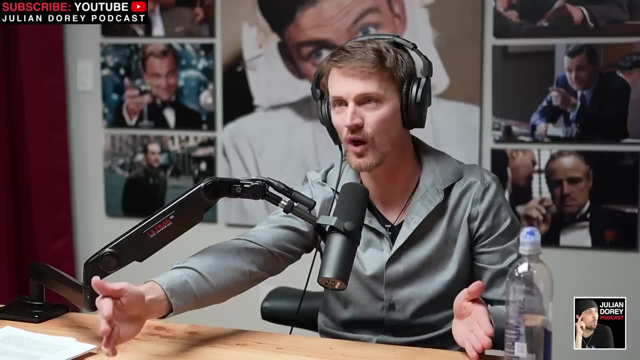 do cool stuff, people. i would had interesting ways of making making money when i was young. but i was like, uh, eight years old and i got really good at that and i realized that you could take like a piece of wood and you could literally like write a name or draw something by burning- burning through the 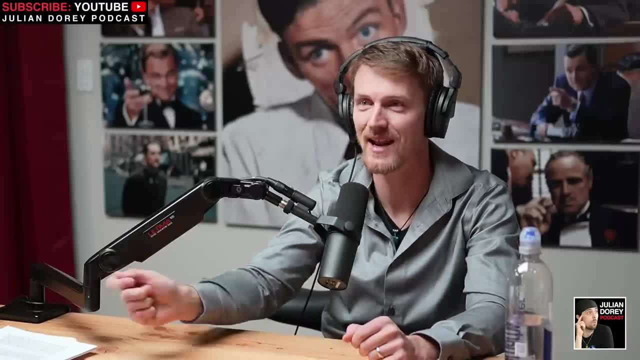 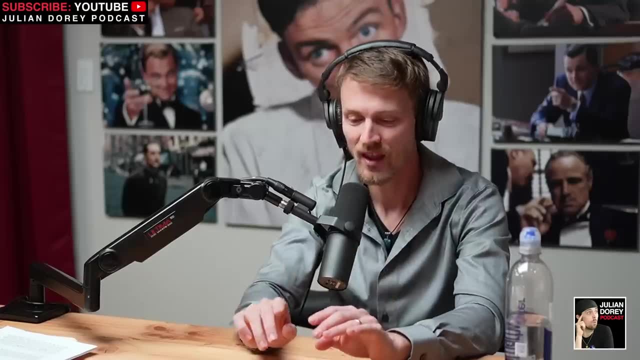 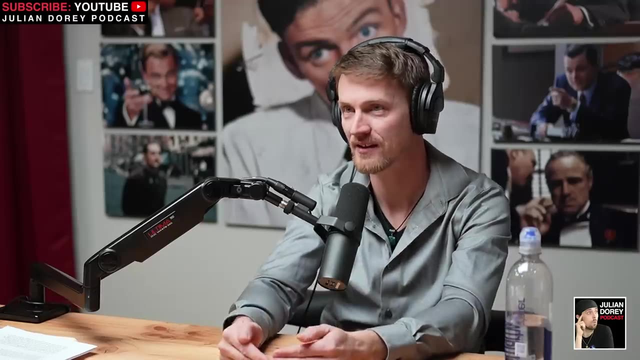 magnifying glass. so i would like sell people, kids, names like burned into, and i like actually started a couple little fires too, because you can literally do that. no, not little ones. but the point is, though, the sun is powerful, and it's especially powerful if you can focus it. some of the theories are that in order to melt them. they somehow put a lens on them and heated them to reach a certain temperature. i've seen theories on, and i've seen even some scientific experiments where people have taken a large lens and focus sunlight and it gets insanely hot. insanely hot, okay now, but it still doesn't make sense for how. 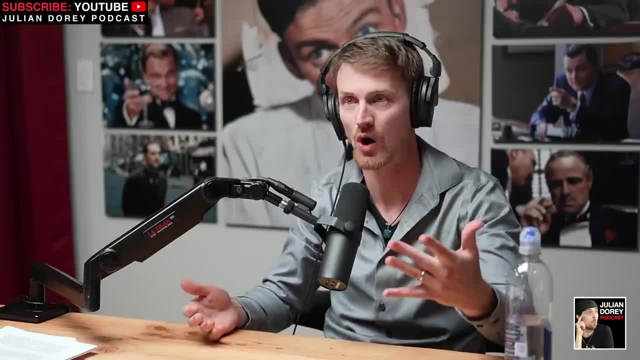 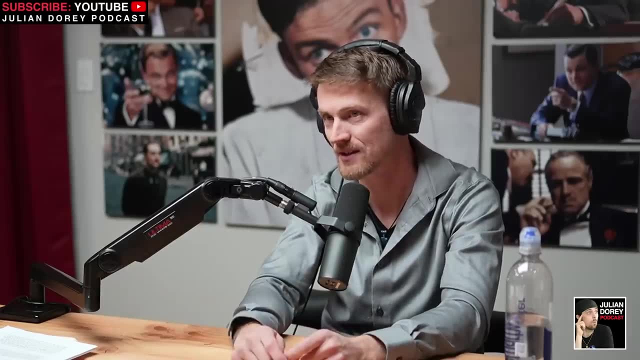 they were able to carve these things, though that only explains how they could maybe mold stones and put them in place. so they're perfect, right, but that doesn't explain how you could carve them, that doesn't. that doesn't really make other than the fact that to do that kind of work with that 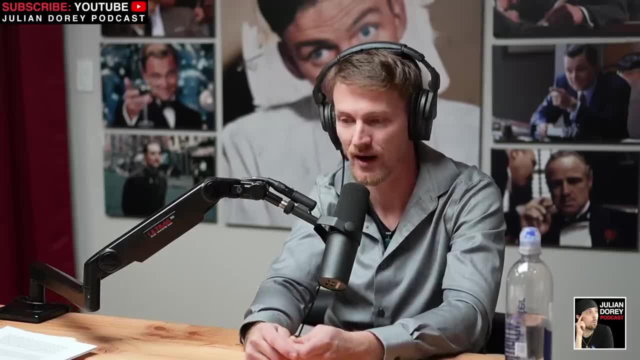 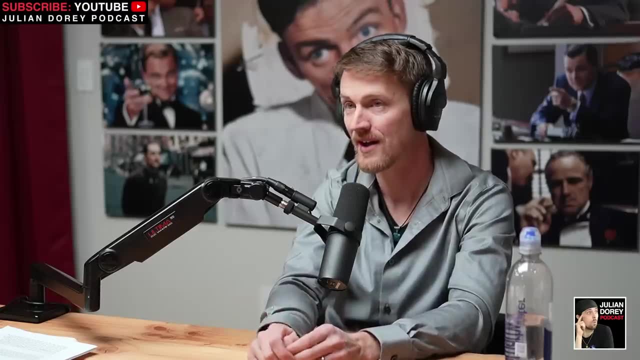 kind of quality. i've talked to a lot of stone masonry, uh experts and they look at sites like this and they look at pumapunku- which is why the comparisons are pretty wild there- and they say they would have to use diamond, diamond tip tools. 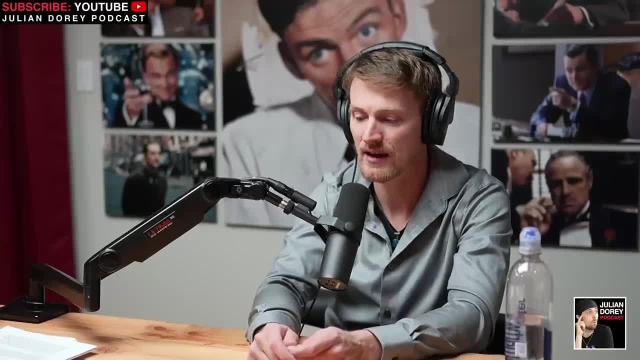 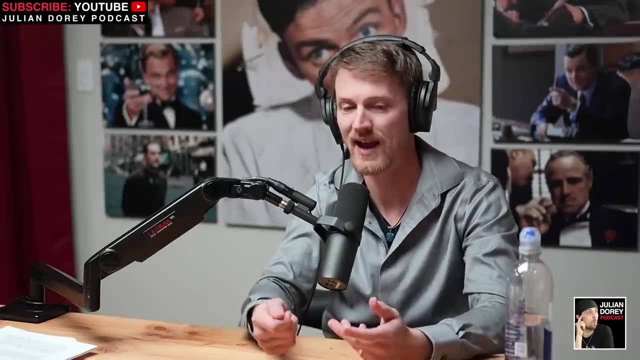 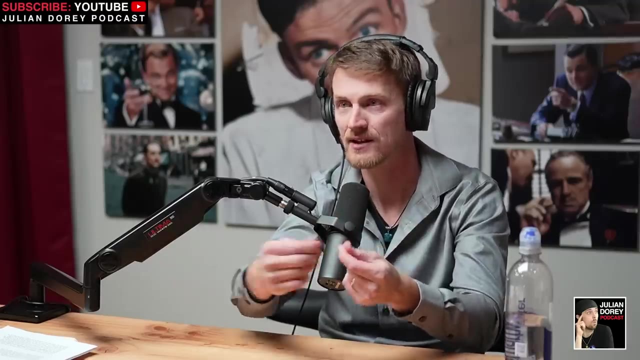 you like laser diamond, tipped diamond, laser diamond tip type of like, for instance, the diamond tip. what does that mean? well, so if you have a saw to cut through- they actually have diamond tip saws- you can cut through solid rock. you use diamond on the edge of the of the, the blade, so it's like: 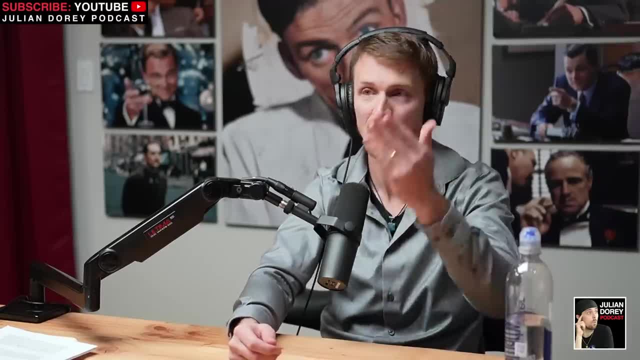 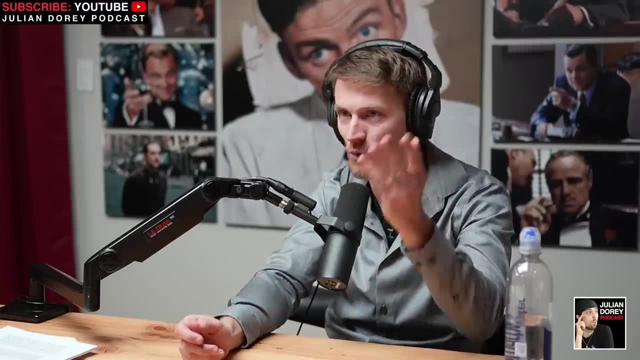 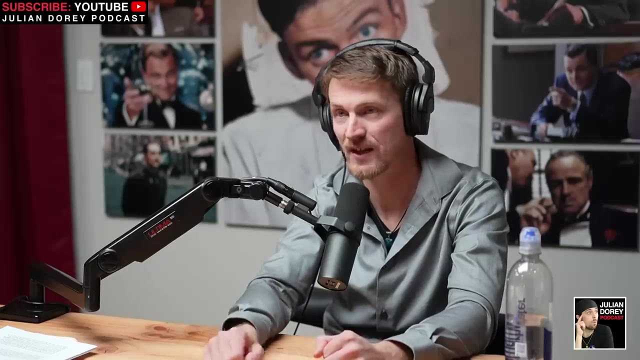 the hardest material possible and you can actually go through something also versus using some kind of a laser. now, interesting, like lasers. i mean, could you create some kind of a laser, like technology with the sun, if you focused it again? that's a good question. i'm not a physicist, but i can tell you that the means for which they created these 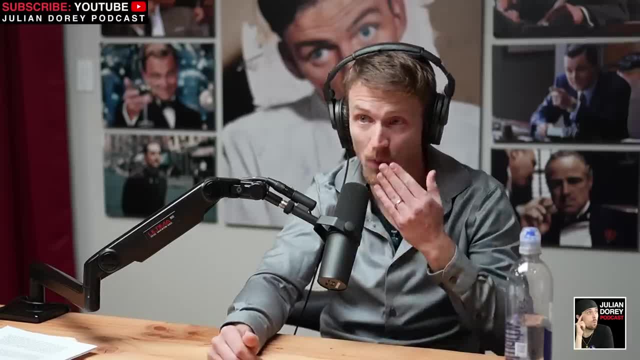 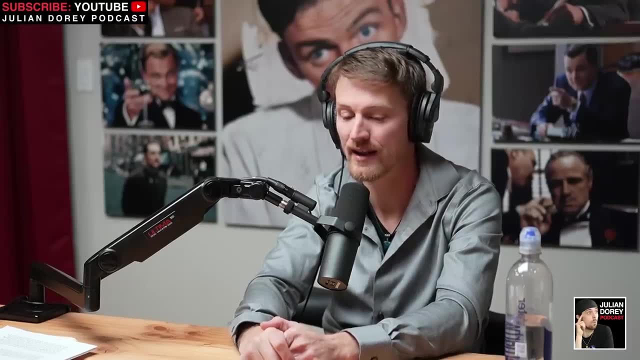 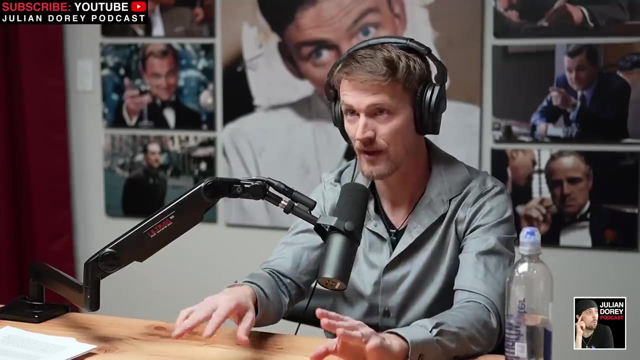 is totally bizarre and unknown, and that's important because my theory is that this location around lake vaughan in relation to the ancient sumerian kings, the last of them landing there in the bloodlines descendants of them, and how the biblical accounts already show them going around the world and being important that something 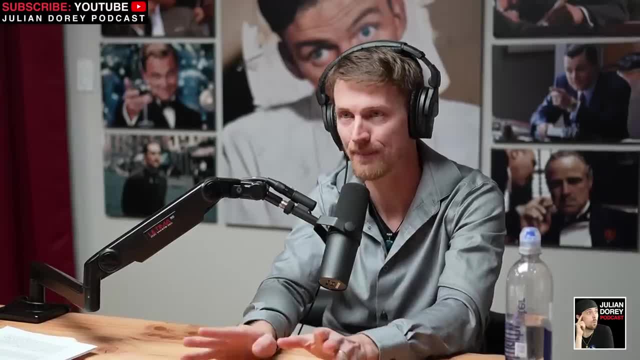 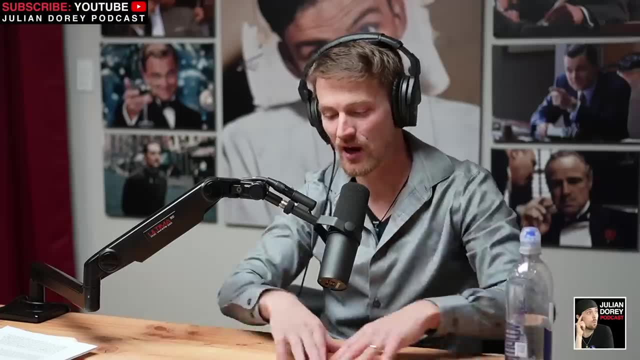 happened at lake vaughan with the ararat civilization. that i don't believe has ever happened, ever happened before in that way. remember i talked about the sumerians. they built these cities and they had a catastrophe that came out. they wiped them out, right, but they didn't understand how to. 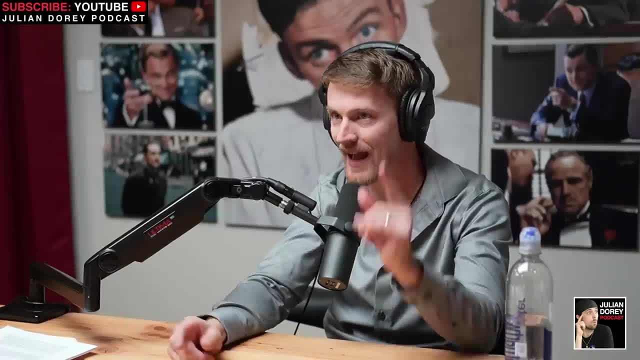 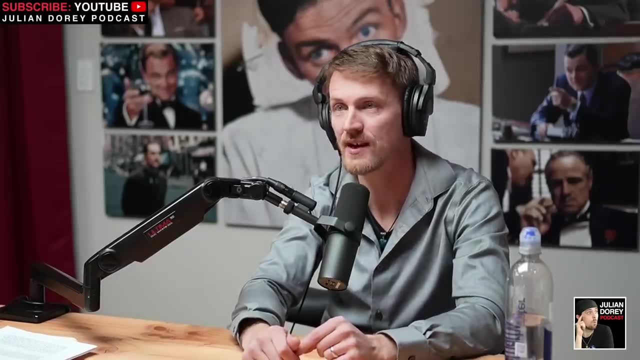 build megaliths. they weren't building any megaliths or anything like that. that knowledge didn't exist yet, which means that if you see like sites like this and they have that connection, all of a sudden you see giant, integrally carved basalt and 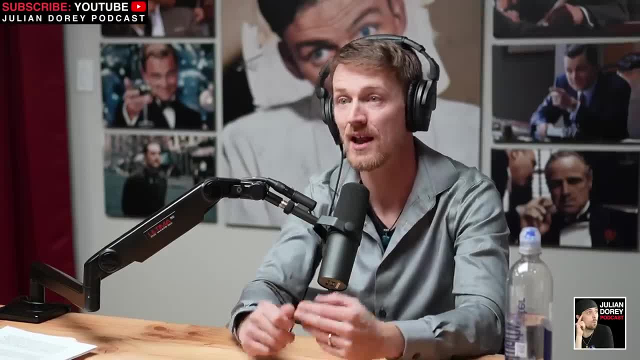 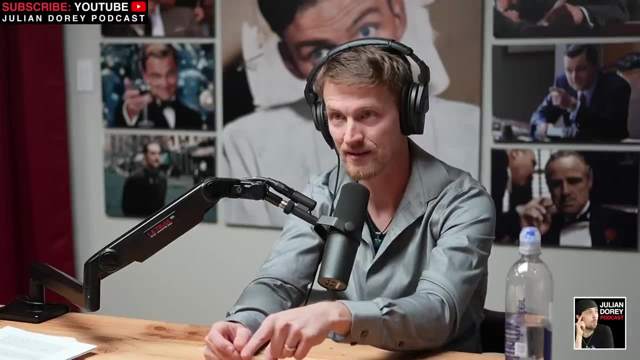 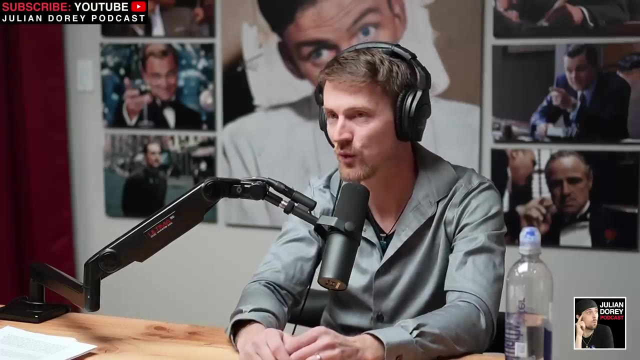 andesite stones and temples that are highly sophisticated like. my theory is that that knowledge was passed down at that site for how to do it, for how to create it and do it in the twin. i think that it was over 20 000 years ago. on what basis? when you're looking at the younger, 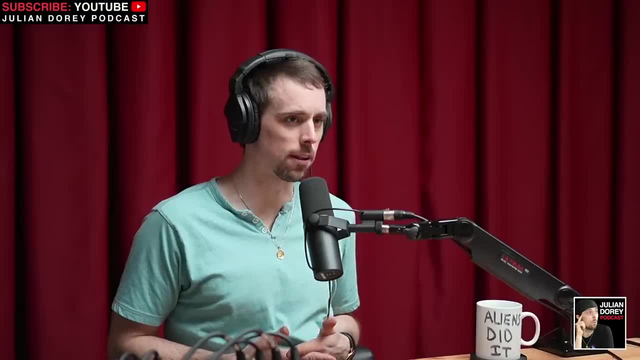 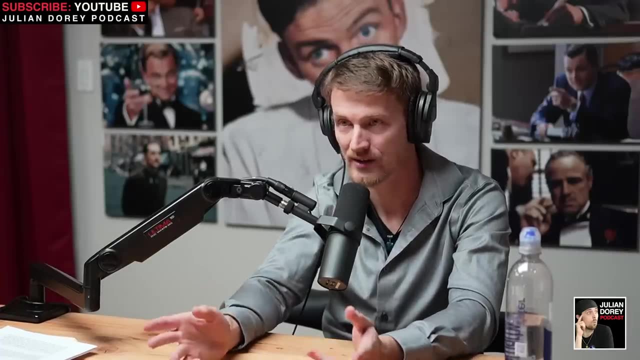 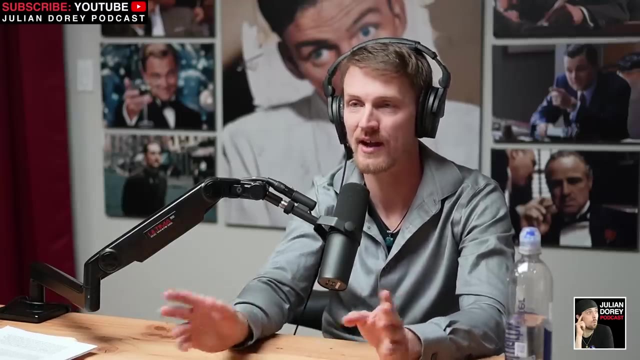 driest disasters. you find younger drives for people, younger drives end of the last ice age 13 000 years ago. the problem is that that site doesn't make sense because it has all the characteristics of the lost civilizations we see around the world: highly sophisticated, amazing stuff they created. we don't know how they did it. 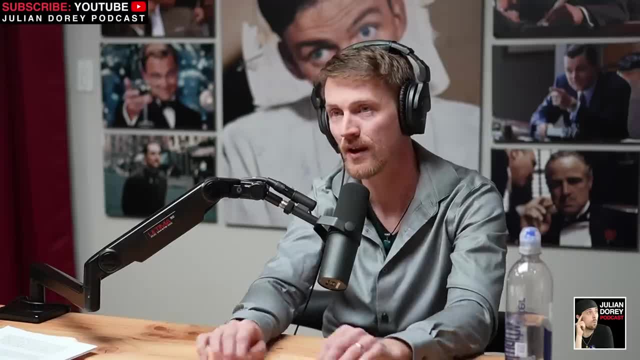 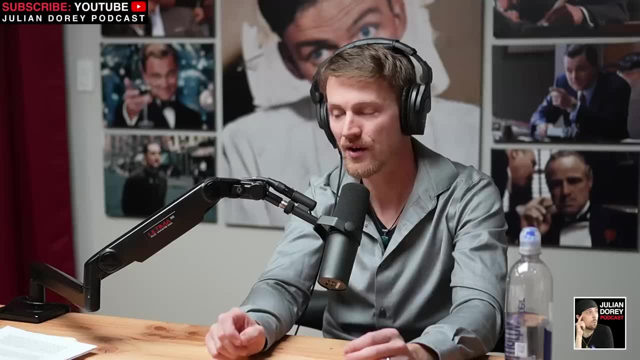 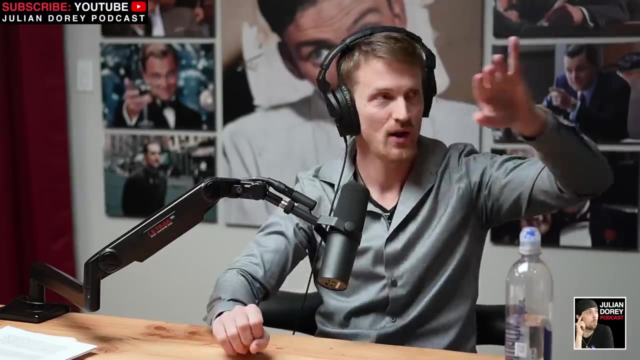 right hard stone, all these things. there's like telltale signs around the world for that type of thing. we know that we call them the lost civilizations, but here here it seems that the designs that they, that they built into the sites, then we could find them everywhere. 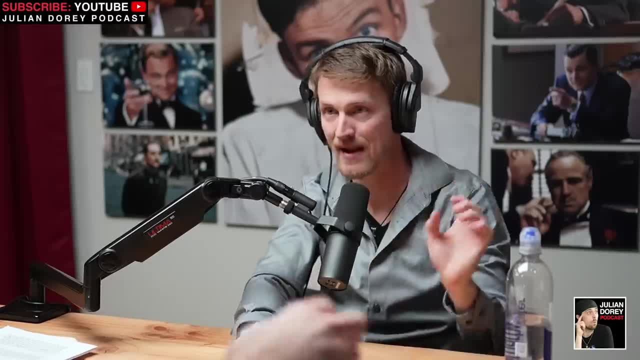 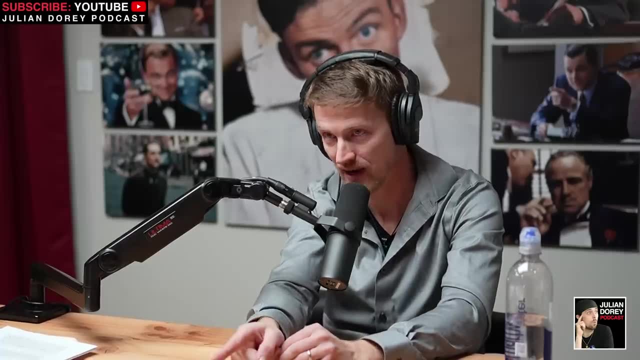 and the symbols that they carved into them then made their way all around the world. okay, but in a way where they're not all together anywhere like they are here. imagine civilizations around the world all having pieces of like how to reach higher states of consciousness and energy, and 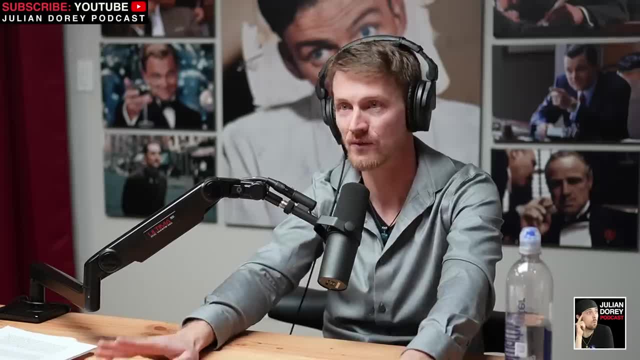 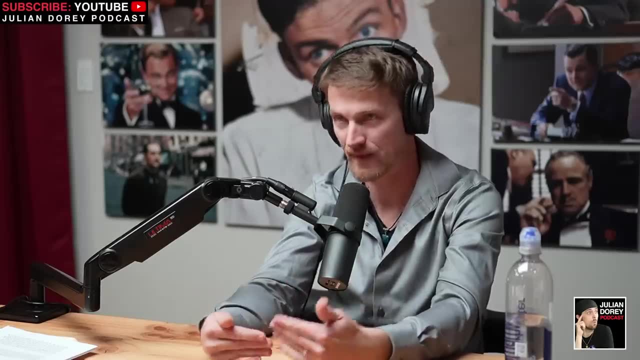 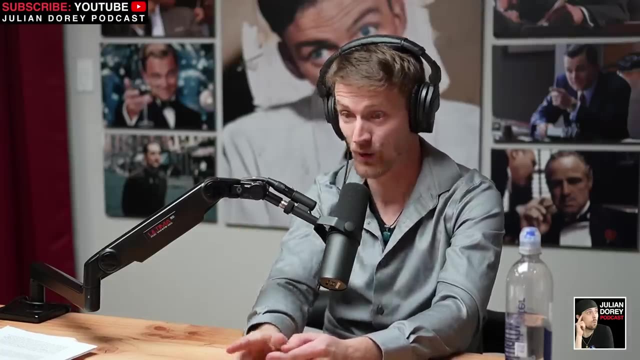 they know all that, but they portray it in like slightly different ways. right, but imagine finding a place where it's all together in in one, in a way, where it's like, it's in its like, pure form, it seems like. and amongst those things, what blew my mind, the reason i ran around the room when i found ionis- is because 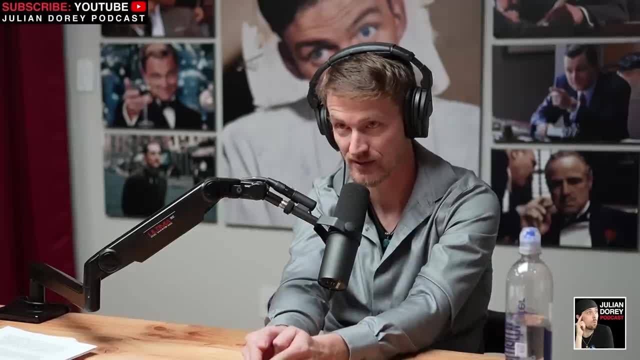 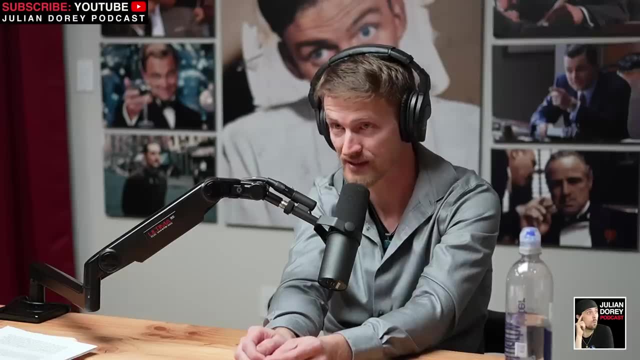 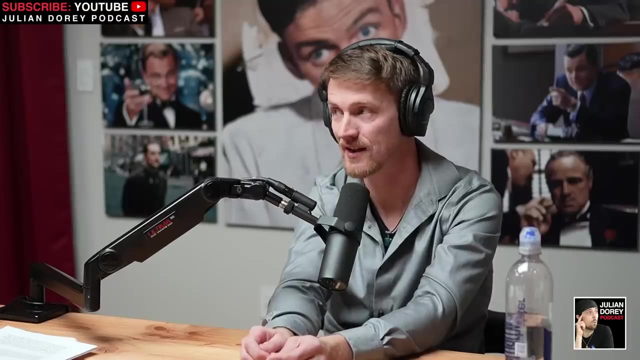 very well displayed in the very center, above an altarpiece carved into andesite, is the depiction that i believe may be the very first cross in all of history. okay, now for those who want to know what that specific type of cross is. that cross is later known as the knight's templar cross, or 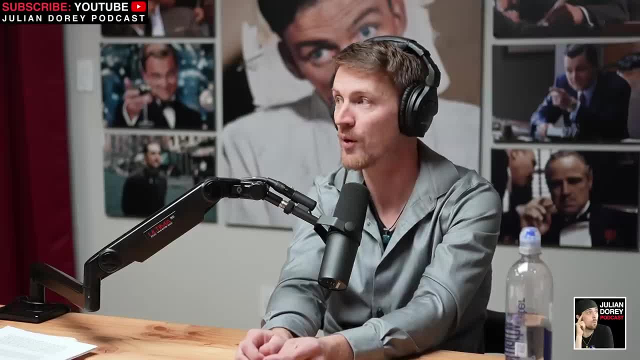 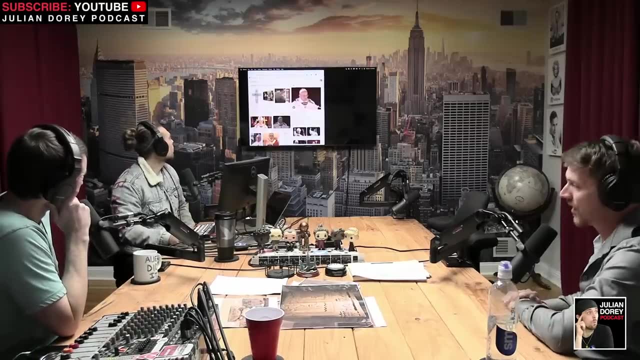 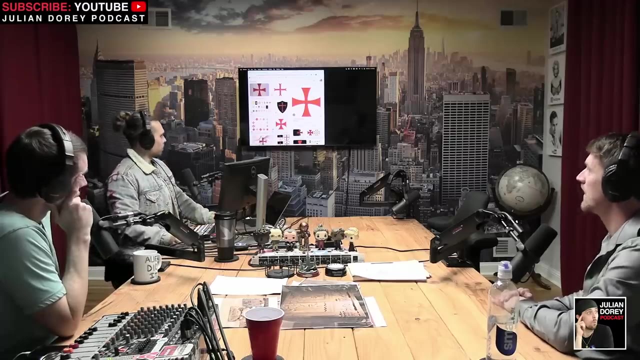 the knight's cross or the red cross. now, can we pull pull up a couple images on there while we're talking? first thing, we i just want to- when we look at um ionis and look at the specific cross that's at ionis. okay, look at how it looks, julian. okay, see how it looks like the edges are all equal. 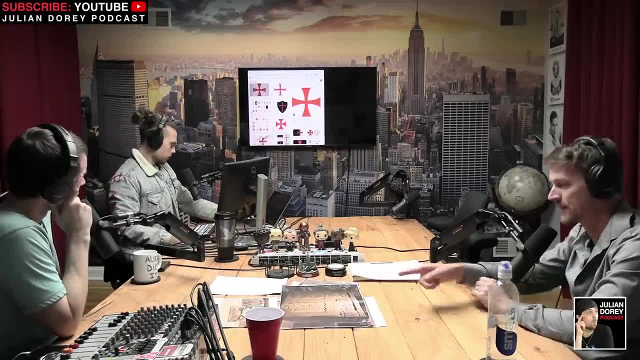 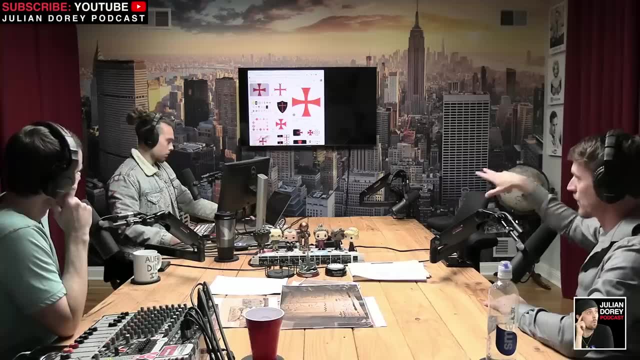 and it almost forms what looks like this: the symbol of the sun there on that, but it's slightly different. those, um, that type of cross is the symbol of the sun there on that, but it's slightly different than the other type of cross that we see that came out of ionis we then find at the core: 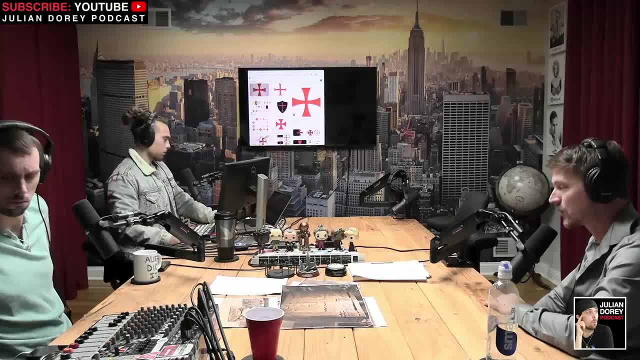 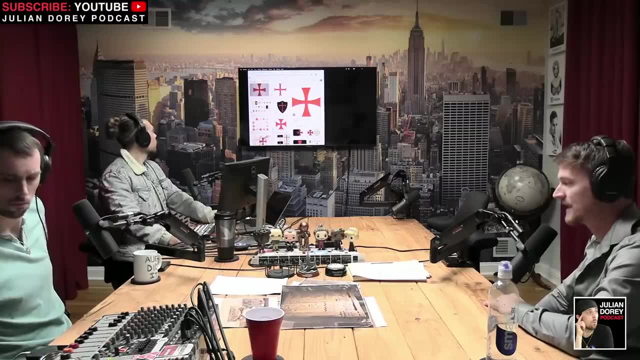 of some of the most highly established and most powerful religious groups in the world. now, what we're looking at right now is what's called the knight's templar cross, which is identical to the cross at ionis, and we also find that same cross in some of the 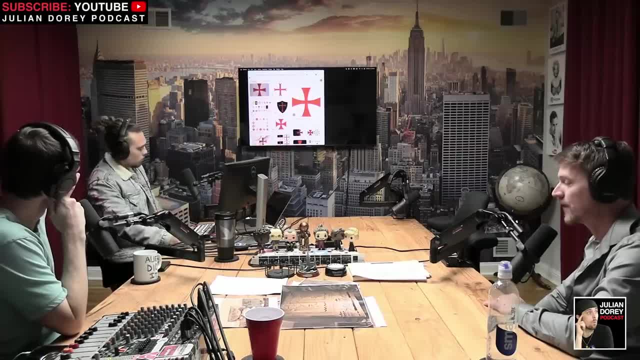 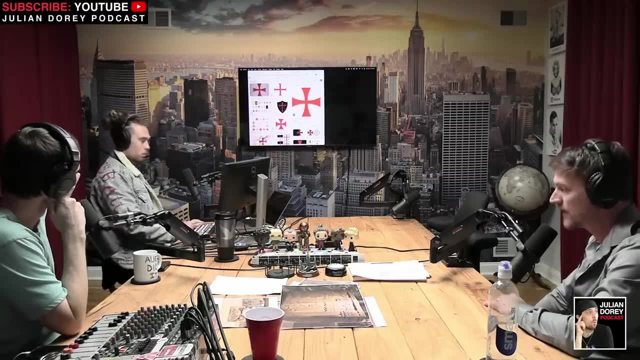 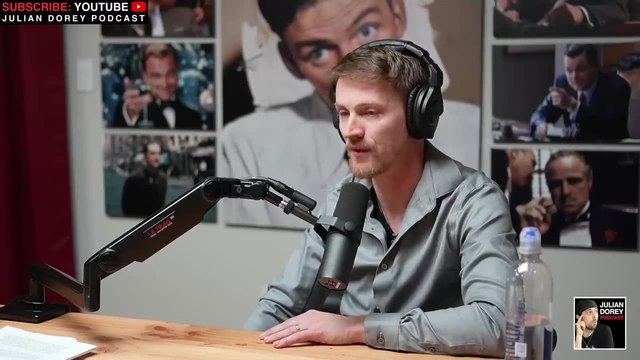 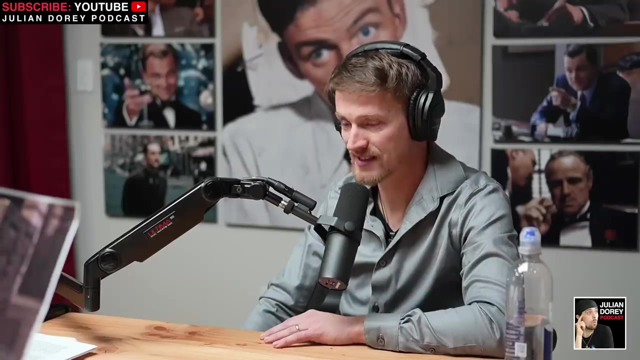 in asher bonaparte's lineages with um, another ancient king that ruled during the time of asher bonaparte called shemshed, and shemshed showed the same exact cross on his person thousands of years later in that region as part of the assyrian civilization. now it gets, it gets deeper. that same cross, that specific. 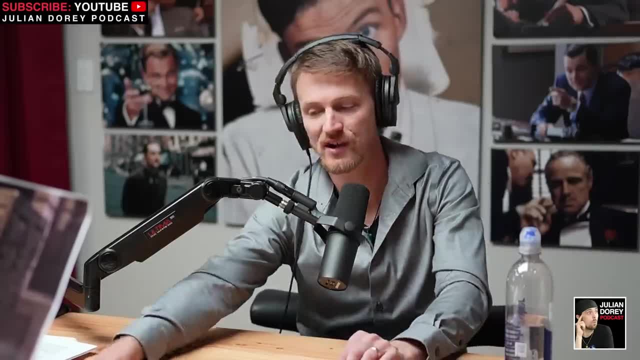 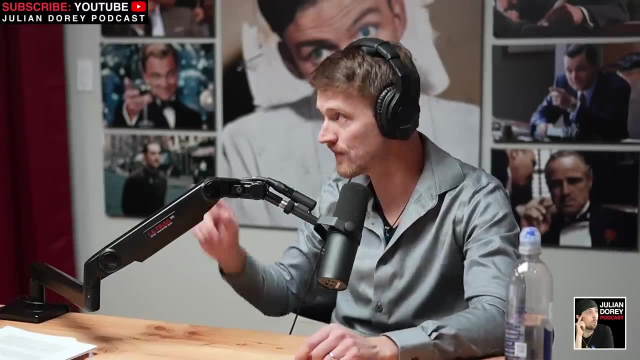 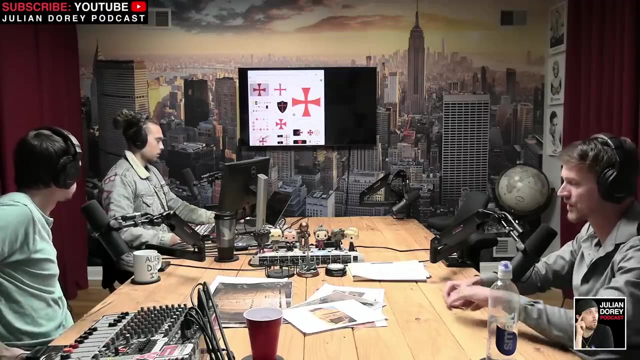 exactly that same cross we then find across the world, in bolivia at lake titicaca. this- i don't have an image in front of me for that, but you, you'll have it in your um, you can pull up over there. yeah, is that the same, the same symbol: the cross symbol at lake titicaca, as well as the chacana symbol from this. 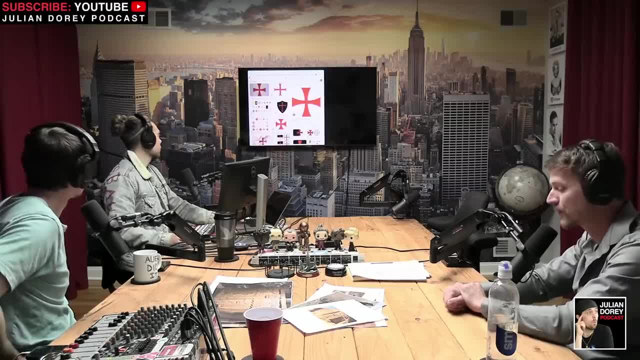 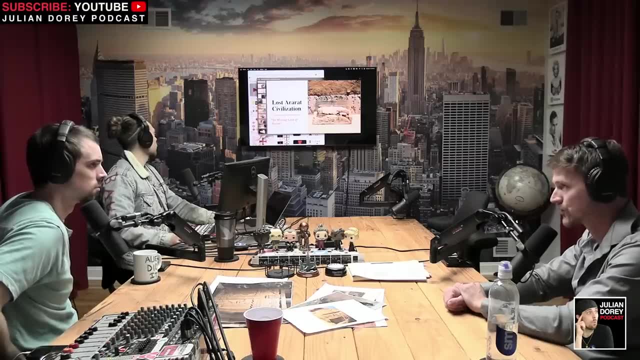 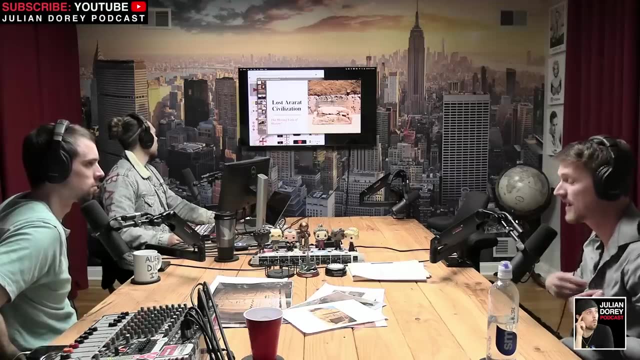 match up identically. and to expand even further, you can look at pope francis or all the popes that have come before him and you look at their wardrobe and the exact same cross is the primary cross shown with with all the popes. okay, different than the christian cross, that's something, yeah. 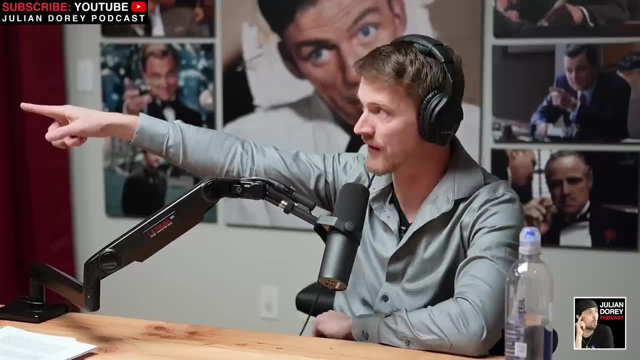 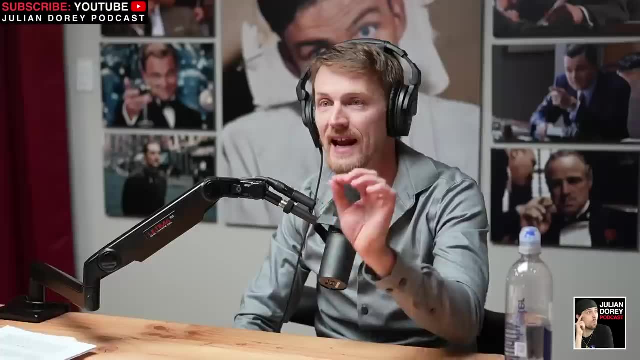 we're going to talk about, but this is, you know, and there, there you go. there's the cross at pumapunku um, at lake titicaca, across the world, and that one's a different look than what we're looking at, slightly different, but it's got the same: three indentations of the, the, the. 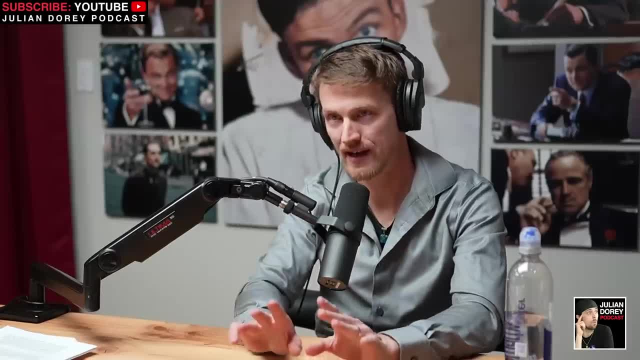 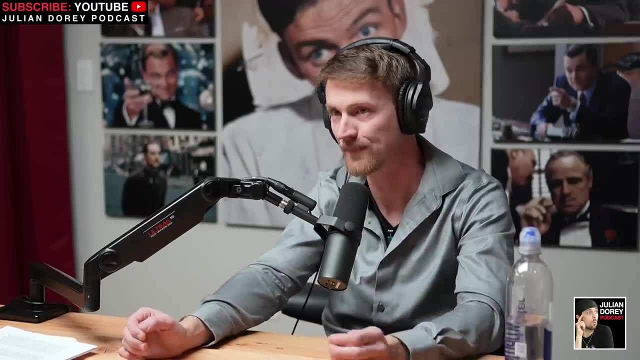 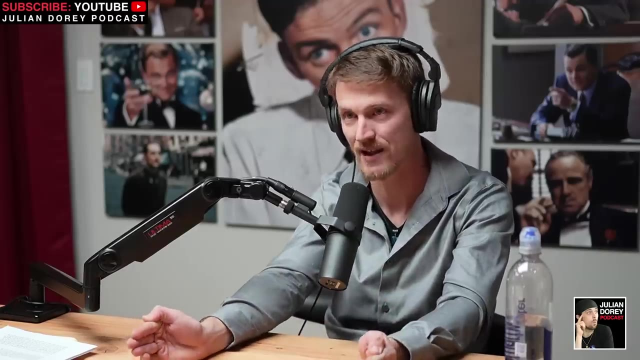 teachings of three, the what we haven't gotten into that yet. there are these core teaching principles that this civilization knew, that then passed its way around the world. okay, and it's this idea of three that we, our totality, what we exist in, is. we exist in a totality of three things. three: 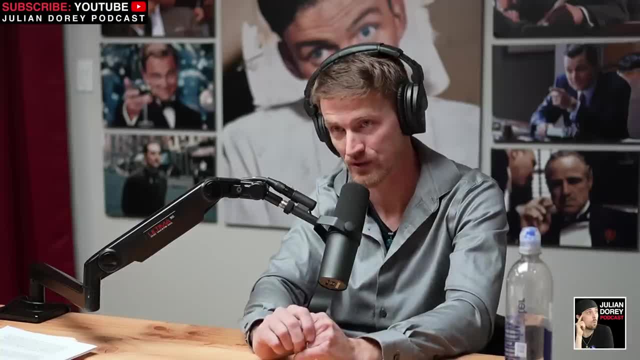 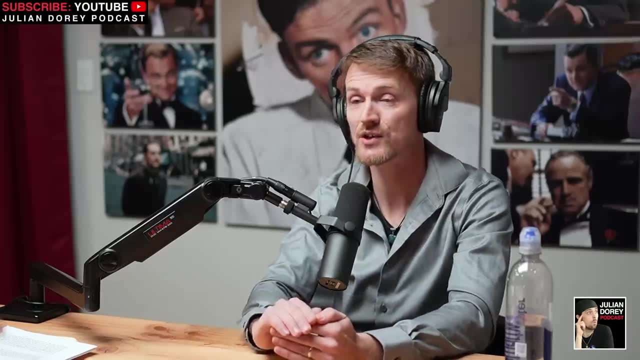 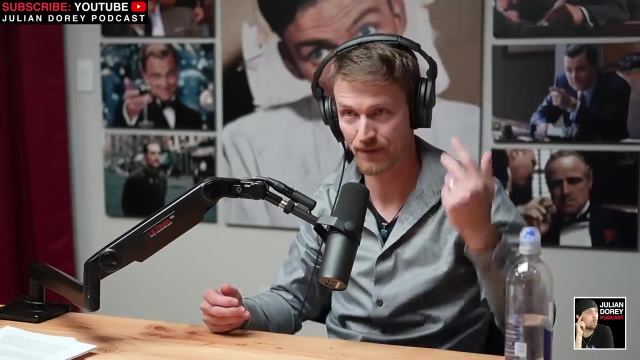 primary things. religion called it the father, the son, the holy ghost. we spirituality, more of like our side. we call it the mind, the body and the soul. okay, but there's all. there's another aspect as well, and it's this aspect of energy, and they believe that because we have a defined masculine and feminine, 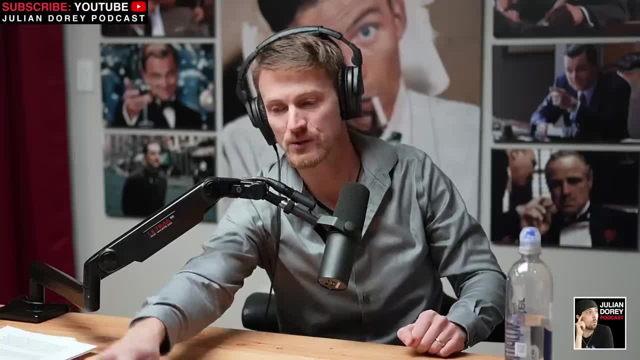 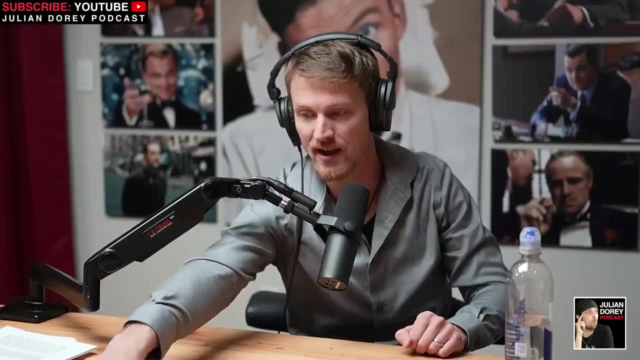 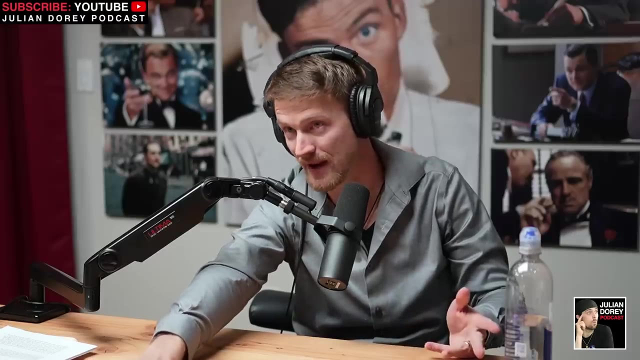 energy. okay- and that's what this is right here, because we have two sides- that if we can balance the two hemispheres of our left and right brain, our masculine and feminine energy, we unlock a key. a key unlocks something that is not hidden. it has become hidden now, but back. 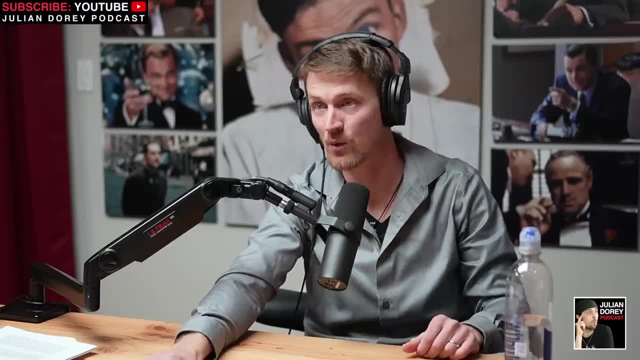 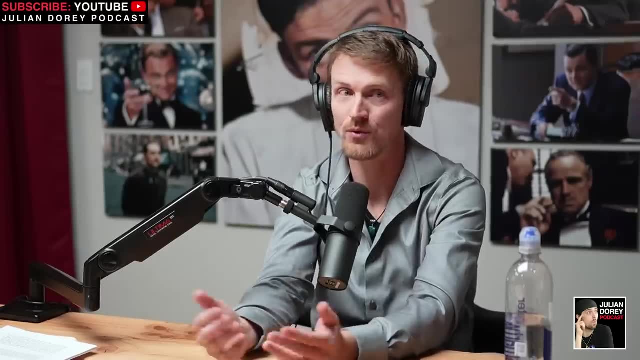 back in this, when this civilization was learning this, they were like teaching us- and this is called the triptych doorway, these three doorways with a central doorway in the middle- on how to basically achieve higher states of consciousness, and what it means is- i just want to add this: go ahead. 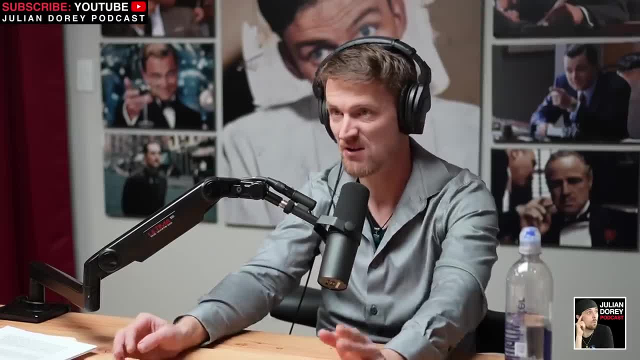 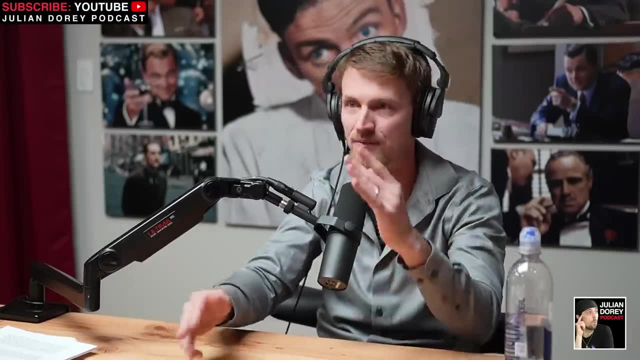 if you balance the left and the right sides, the hemispheres, the energies, it doesn't matter. they're all related right. your left brain is usually masculine, your right brain is feminine. same thing. it's just part of our totality, what we exist in, what they're saying in this and why is. 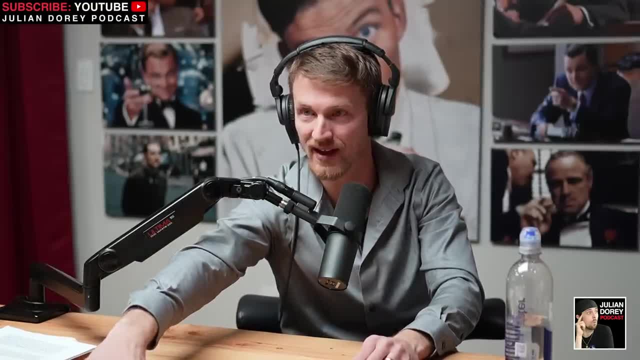 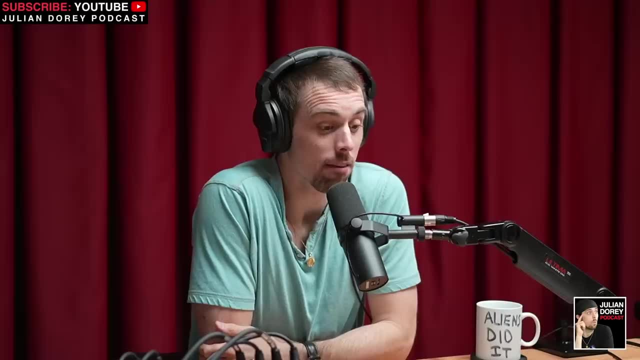 florida lee symbol is pointing to this florida lee's killing me. hearing that? well, i'm telling you that that symbol goes back a lot further than france. yeah, yeah, okay, i, i get the connotation. well, you can see around his helmet and his hat right. i just remember from the movie la confidential. 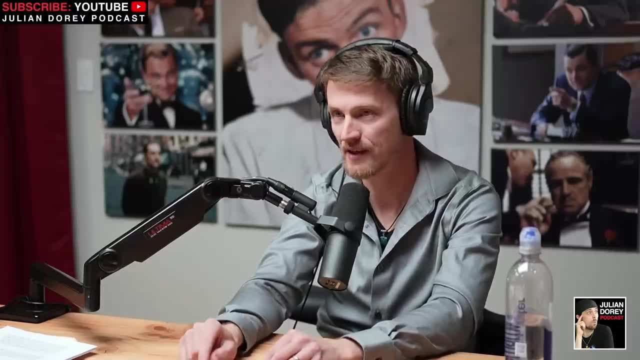 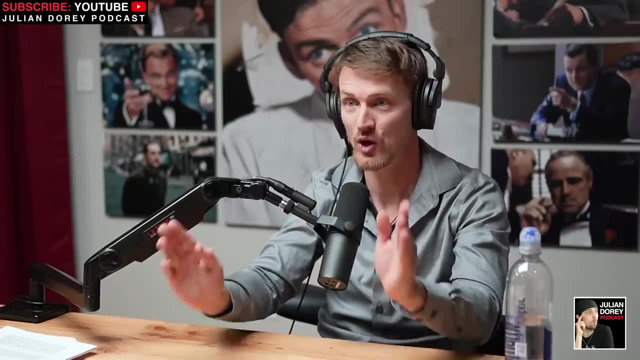 well. so what they're saying is: if you can balance the left and the right sides of your brain, you can balance the left and right sides. these other totalities will be existing, like the mind, the body. right. you can unlock the higher consciousness, or spirit. now, in hindu religions they call it the 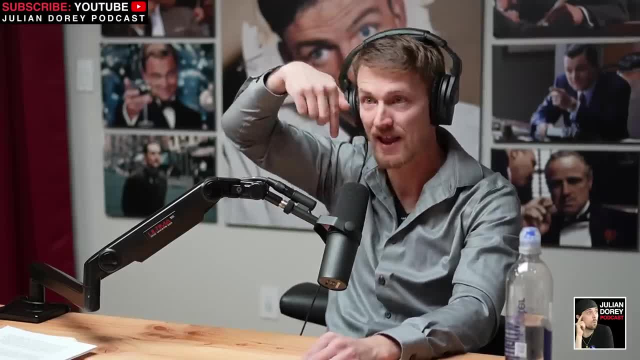 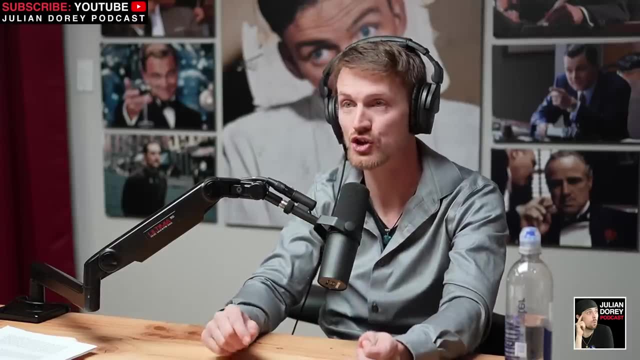 kundalini energy and it has to do with our spine and how energy can unlock to reach, like these, buddha-like states. now the rod of asclepius, or the wings of hermes, shows that, that rod with the energy spiraling up, with wings at the top. 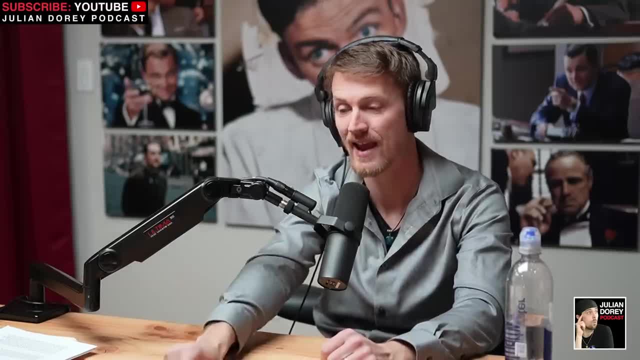 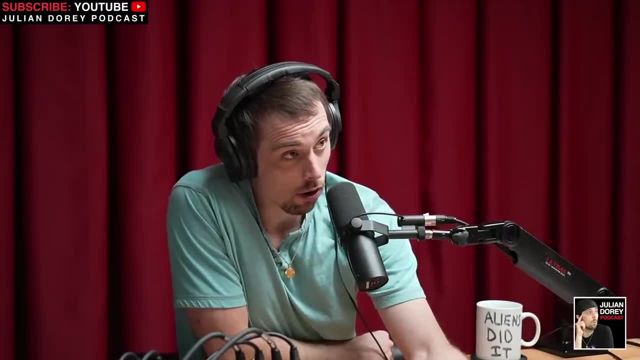 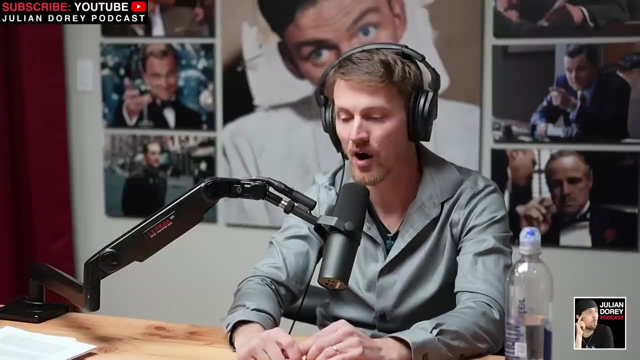 is the same thing as this. that's what they're trying to say in this box. relief from kev temple. is some of what you're saying about the takeaway here, or is all of this your takeaway, building on top of it, or are you also including other experts who have? yeah, so i've brought in a lot of other. 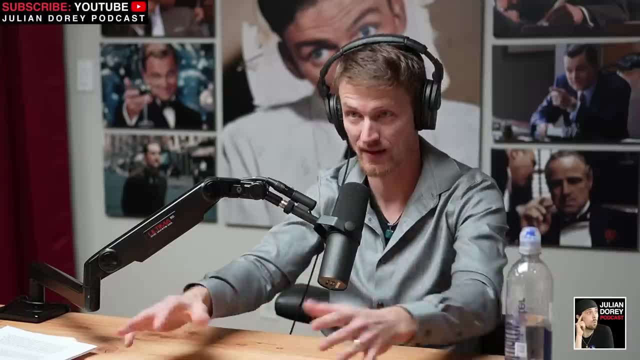 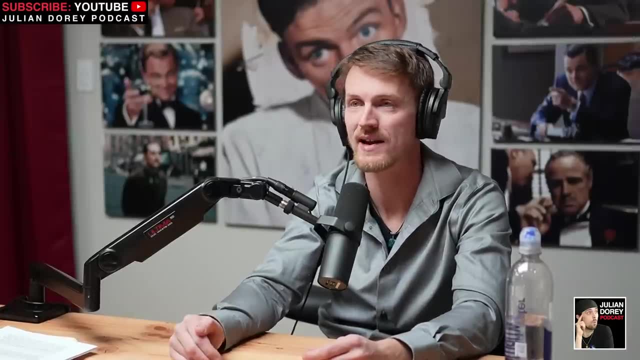 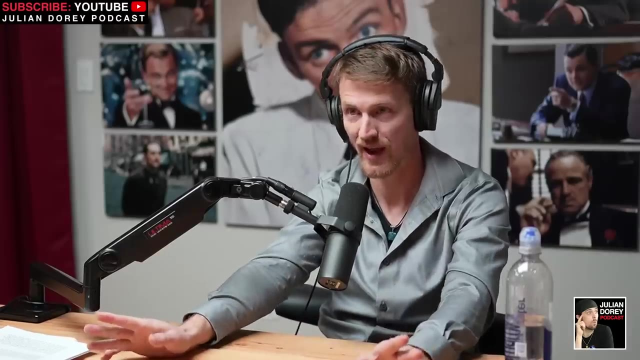 experts, because i was i. i- this was my theory- and and finding these? because a lot of these discoveries are very new. who'd you bring in? i brought in paul wallace to confirm with me. we spent like a whole weekend actually hiking. i came to colorado, um, and who's he? paul wallace is- is an anomaly in our field. okay, paul wallace. 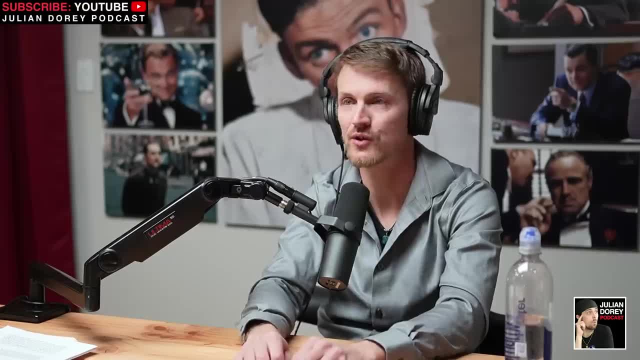 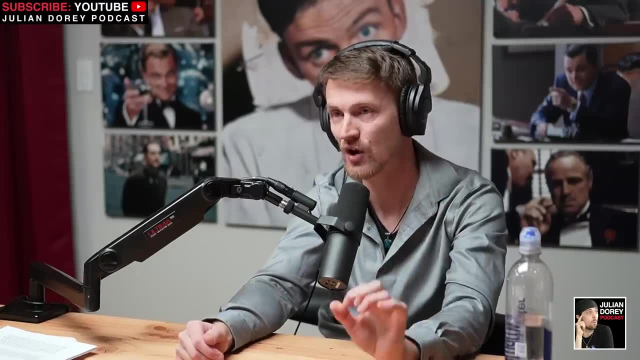 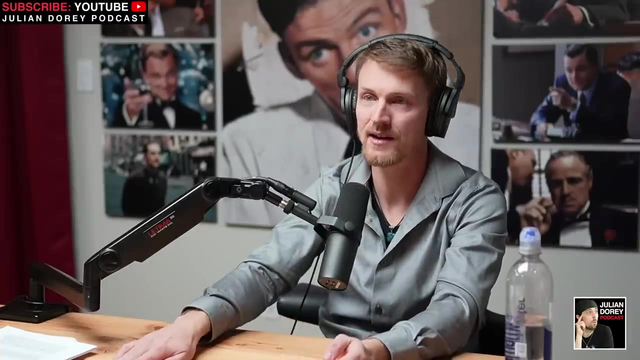 is one of, if not the only, ancient researcher speakers that speaks what we talk about, who actually has a fundamental, significant background in the ministry. he was an archdeacon, which is one of the highest levels in this. you talked about this guy earlier, i'm sorry. so paul wallace i i brought in to confirm. be like, look, paul, i'm. i'm making all these like. 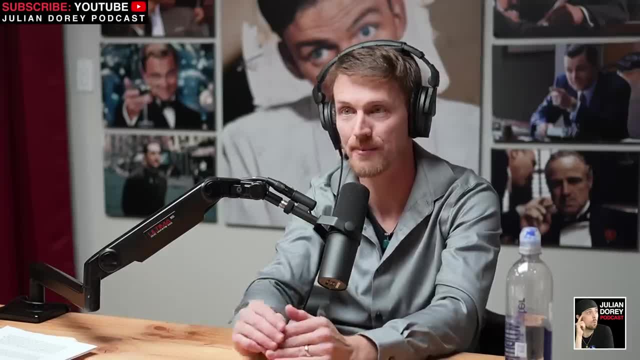 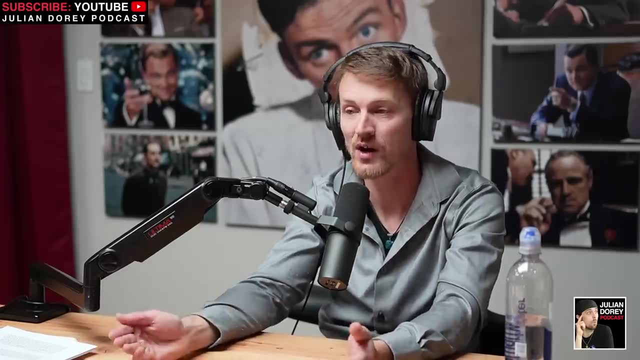 not accusations but, uh, statements right about these symbols being religious, context being the first like i need you to look at this and tell me if i have any holes. tell me if you disagree or if there's something doesn't make sense. and you know what paul said to me. what do you say? he looks at. 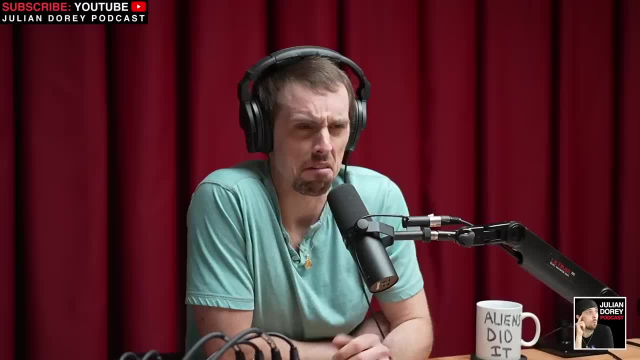 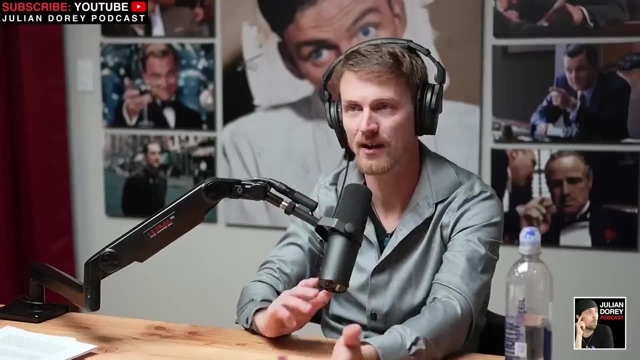 it all takes his time. you know that's what he does. he's careful like a half hour. no, well, i mean well, we had, we. we had actually talked online and then, when he came, we spent a lot of time discussing in person. and what he told me is this: he says i spent a lot of time looking at 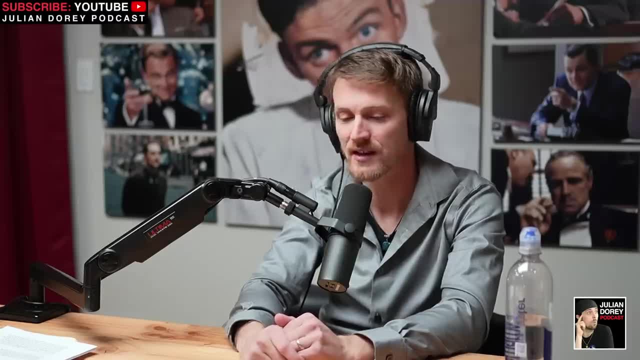 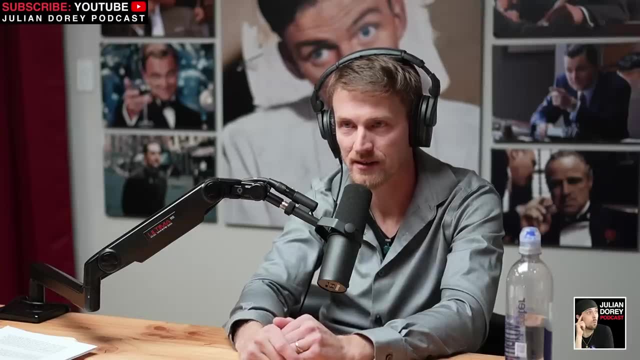 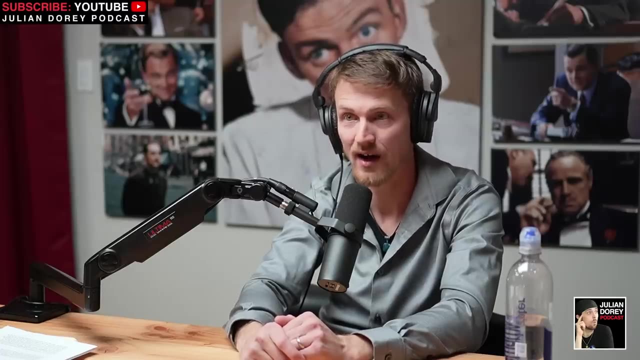 what you sent me and looking over the look at the cross and the history of what i know and he says. he says the thing about it is like just looking at ionis and looking at that cross he's like just purely academically i can't say it's not, but just in terms of what i feel it's. 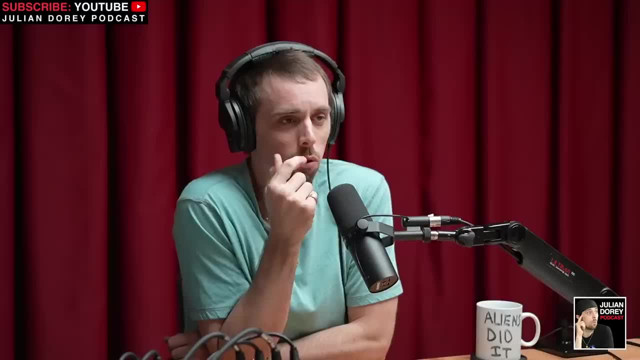 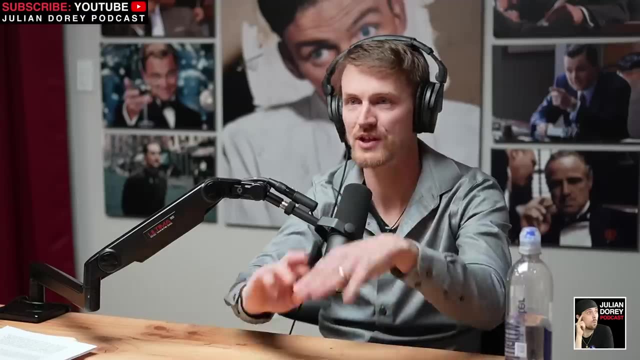 like i know it is. so there's something special about this site, but he's going on feel there. no, he's looked at all of it and he's like i don't know what it is. all the images, all the stuff that depicting it and, seeing it, he's adding another layer to it. 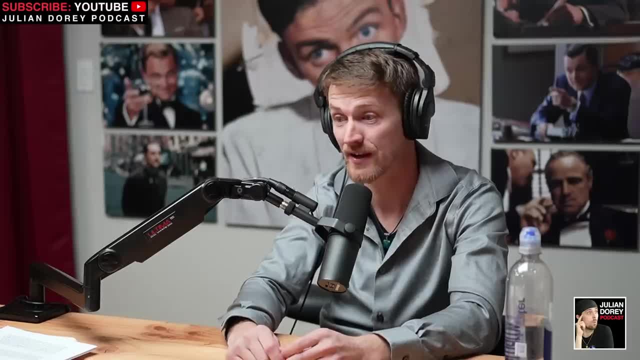 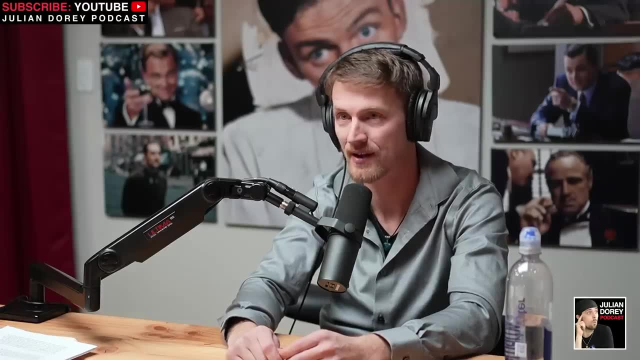 and it's a layer that i'm trying to explain as well- is that my life has gotten um somewhat strange since these discoveries. it's kind of weird dreams, things that i've, things that have been happening that are um hard to explain, like the- let me just put it this way, and paul was trying. 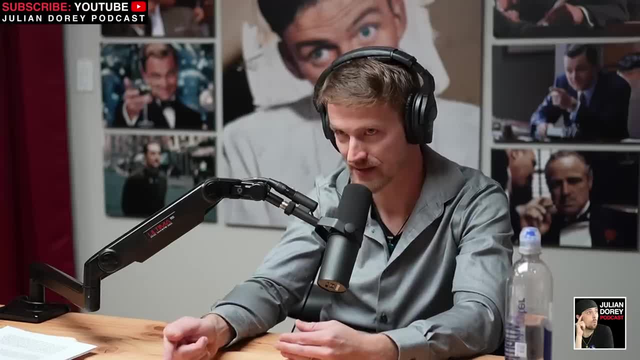 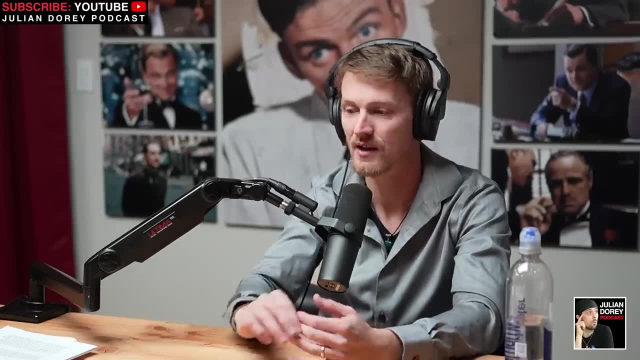 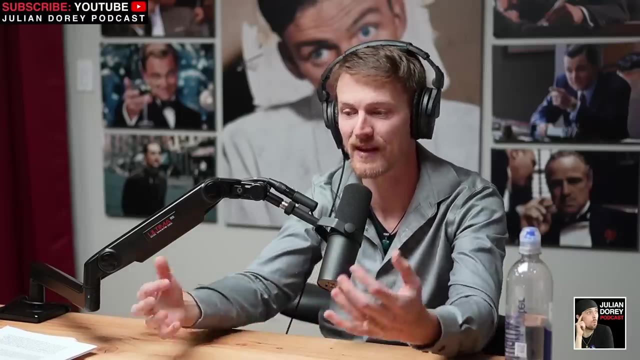 to hint at that. what if this is what i say? it is just for a minute. let's just pretend that i am saying it is accurate. it's the first cross your origins of, like the lost civilizations and these teachings to spare on the world. that then we forgot and we tried to re-remember, and then religions took some of. 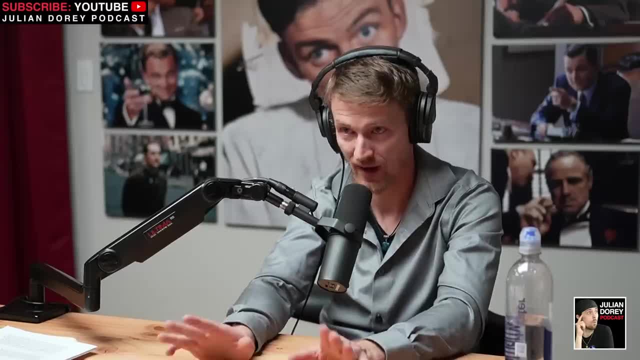 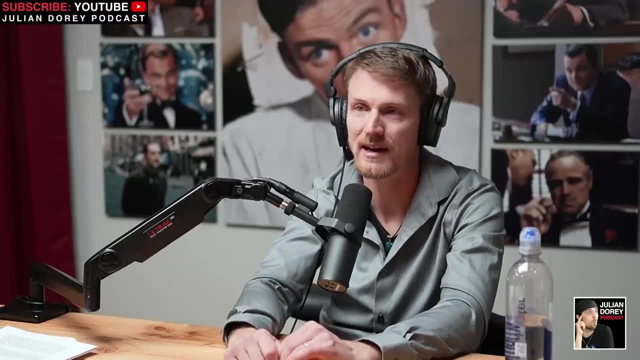 the teachings and wove them together with others. what if that is true for a minute? okay, what kind of implications would that have for humanity? imagine finding the very first cross that has a different meaning than it ever became, the very first chalice cup that has a different meaning. 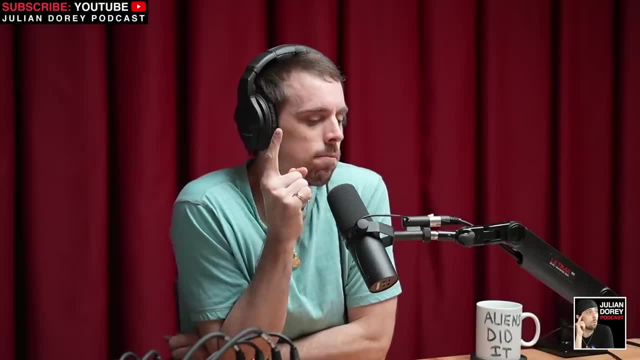 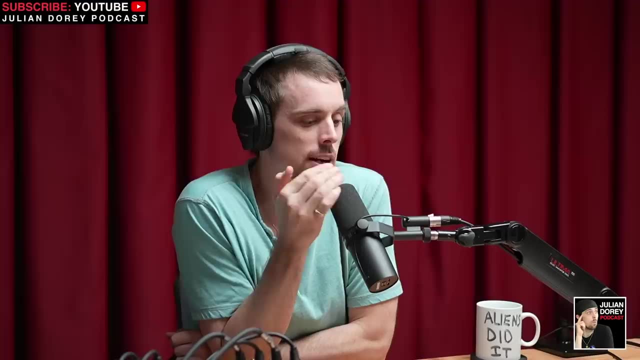 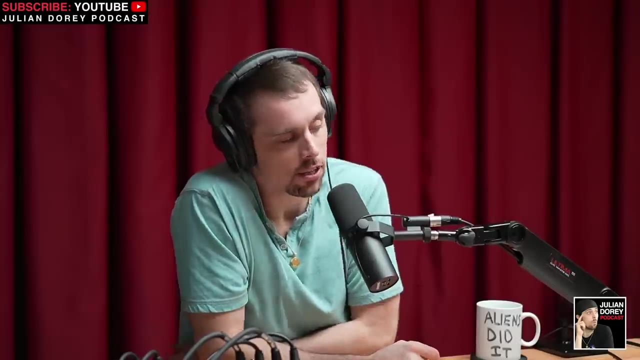 yeah, yeah, i mean it might be what humanity needs, yeah, but it's an incred, it would be an incredible, fine, but it might be less consequential than you think because, like i'm just going to cherry pick one right, you look at the cross, the cross became, and it's interesting to look at all the images you pulled up of people. 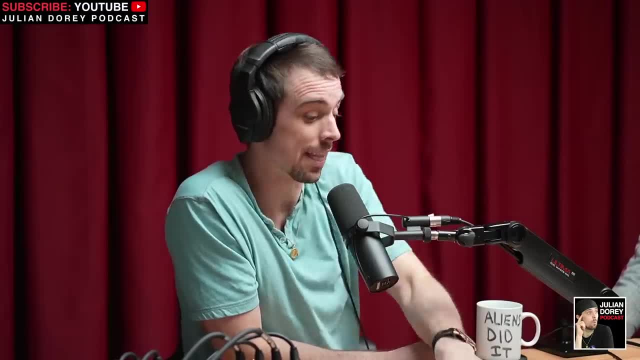 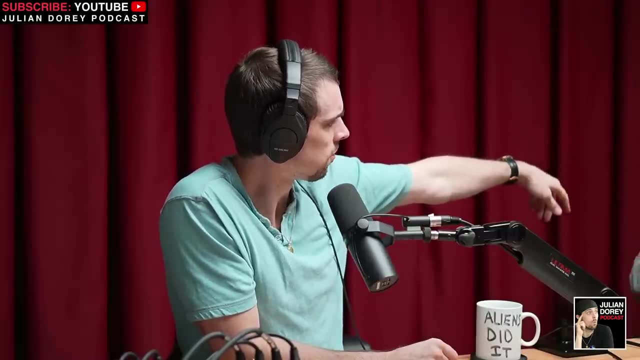 in pop culture, including in religious circles, by the way, who happen to be using this type of cross right here? yeah, the ancient knights, templar cross, but like the cross as we know it, like, do you wear a cross medallion? that's the christian cross. yeah, that's a christian cross, because that was this, and 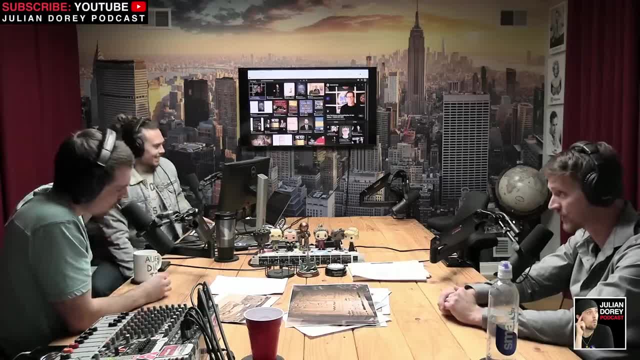 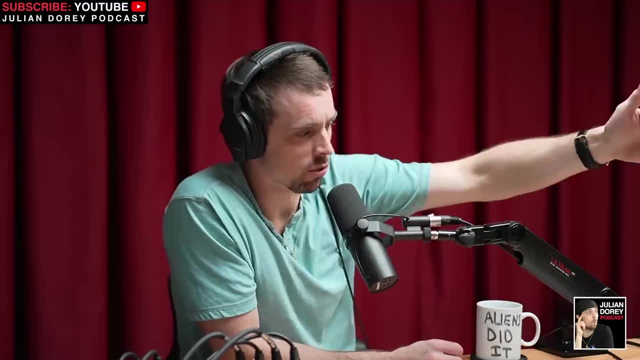 it's a different shape, it's totally. it's different lanes. there's actually more than 20 different crosses in the world and it's, and it's a- i'll bet there's a lot more than that actually- um, but it's, it's the thing that jesus was executed, right, it's the sacrifice, so right, so there, so it became its. 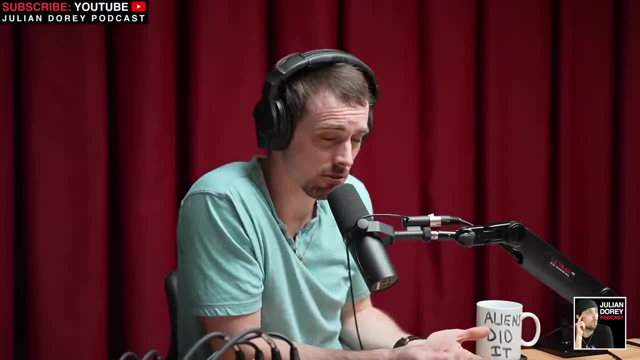 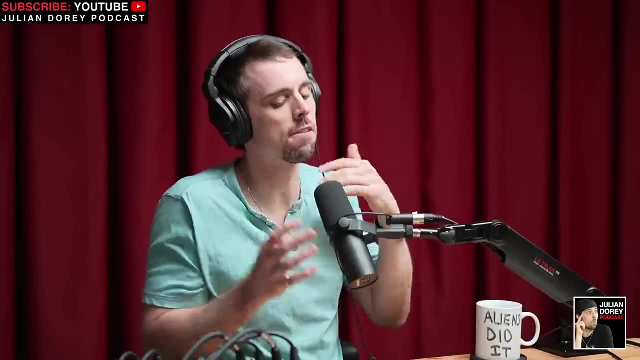 own symbol, again, not that long ago. this we're talking just over 2 000 years ago, right? yeah, this as as like potentially the first type of cross we've seen. it's similar the feeling i get when i look at this as a layman. yeah. 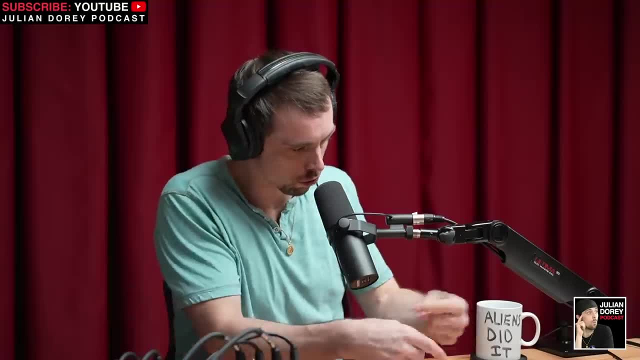 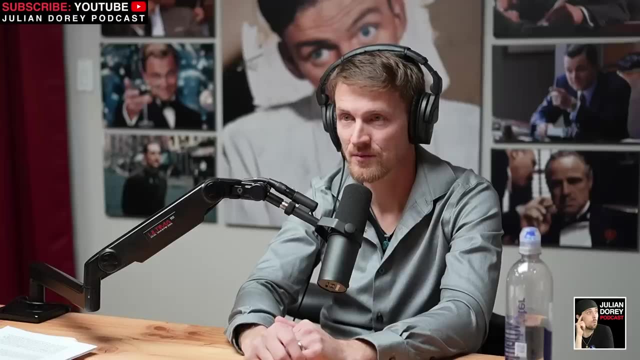 like we all joke about the first time caveman figured out the wheel, like, oh shit, it rolls. it's almost like this is the first time they took a. they took a scrape and they realized they can cross to make a shape. you know what i mean. i don't mean to oversimplify it, but that's what would make. 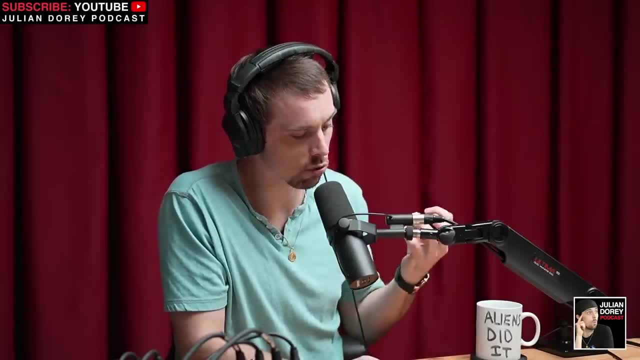 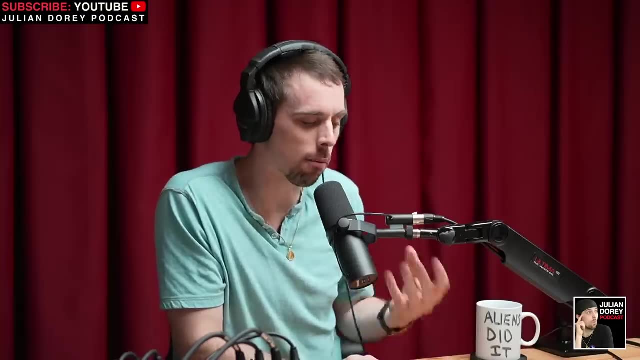 this extremely cool. it's like it's the first time they were using some sort of carving to to get across a point that's not in a word but it's in a shape that would become almost numerical or alphabetical. does that make sense? it does, but what if they're not? it's what if it's not based on? 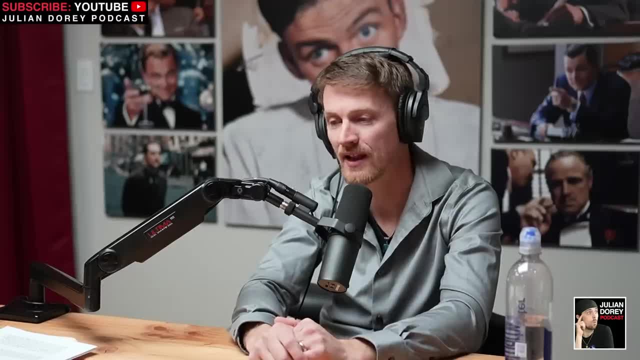 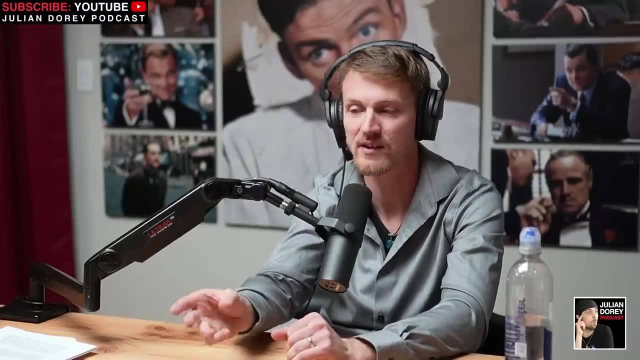 it might not be like. if you look at the associated symbols on in in ionis, you see that it's a sun temple. they're they're worshiping the sun and the sun symbol looks actually a lot. it looks very similar to the shape of the cross symbol in terms of being a circle. okay, it's creating this. this. 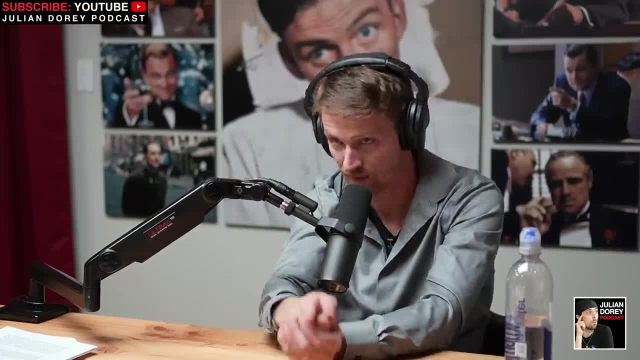 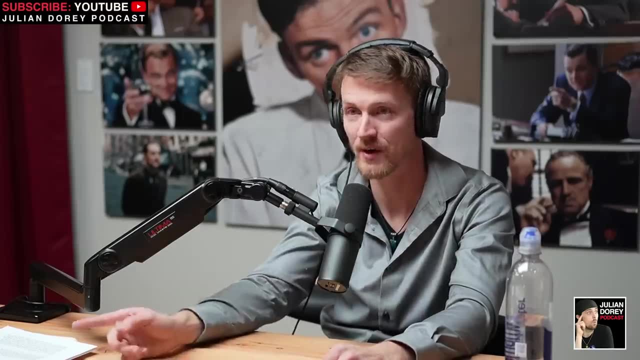 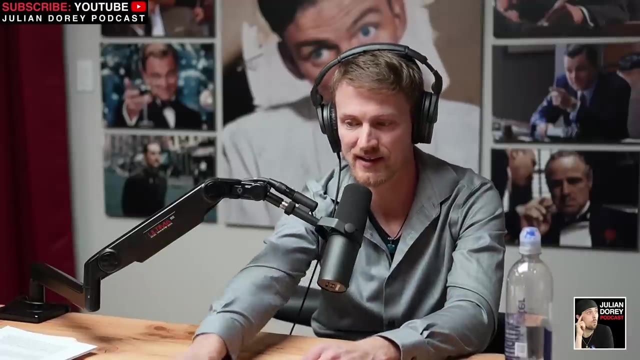 circular type of of symbol, and i think that is part of the meaning behind it. okay, and this gets into: what does a cross mean? what it used to mean? how about not? what does it mean in christianity in terms of a sacrifice type of? yeah, way before that, okay, well, the interesting thing is that, again, let's get back. 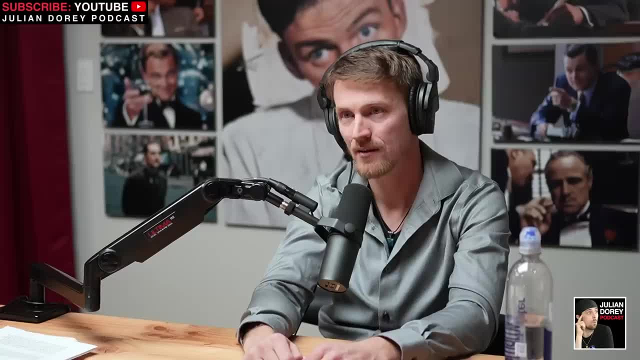 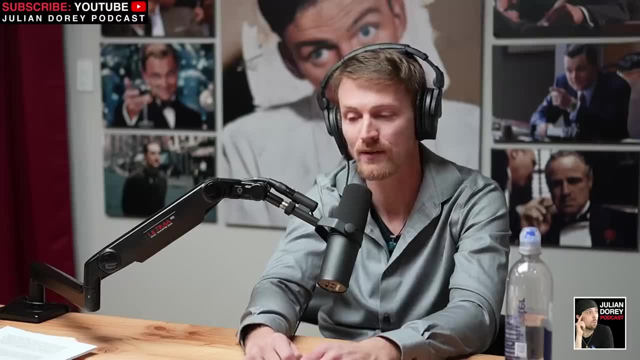 to the the box relief at kef. it doesn't have any crosses on it, right, but it's got a lot of associated symbols that are similar in terms of, like, the triptych doorway in reaching higher states of consciousness and the tree of life. you see that well if you take those associated symbols. 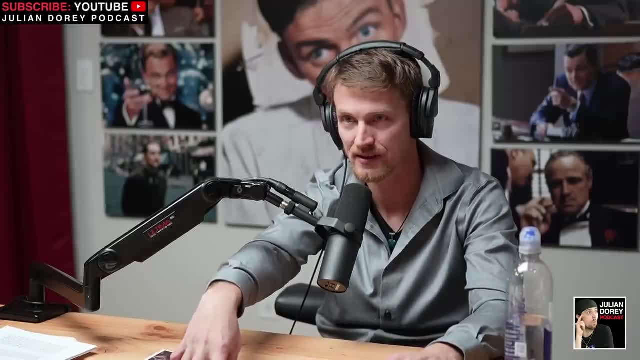 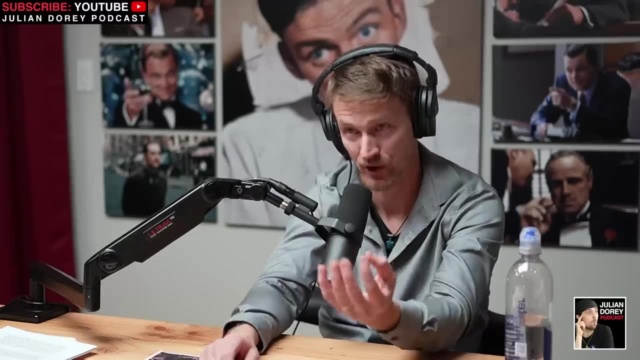 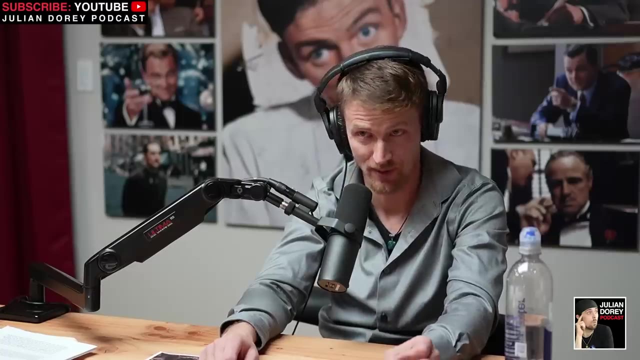 you can figure out what they're trying to say in this and what i believe they're trying to say. if you look at the original cup, or chalice signifies a? um, a significant religious or spiritual doctrine being passed. so if you look at the original cup, it had nothing to do with sacrifice or blood, that's. 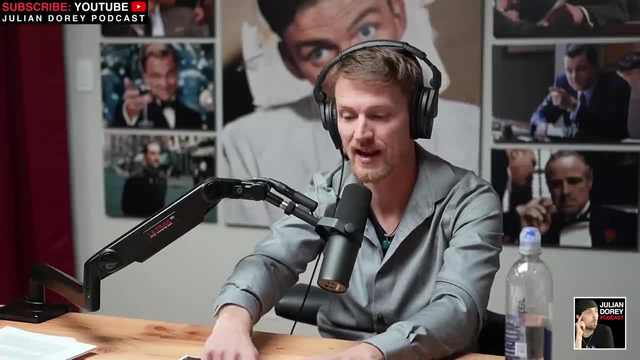 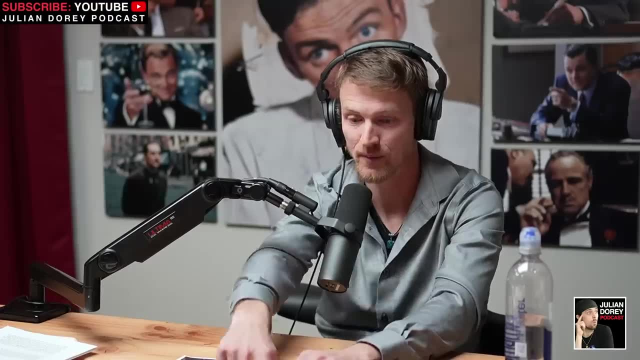 what it originally meant. it was like a doctrine. and here he is taking what's not a lance or a spear- that's what remember, like we talked about. he's taking the seeds from the tree of life and he's passing the knowledge of that. what does that mean? like well, the tree of life has been shown. 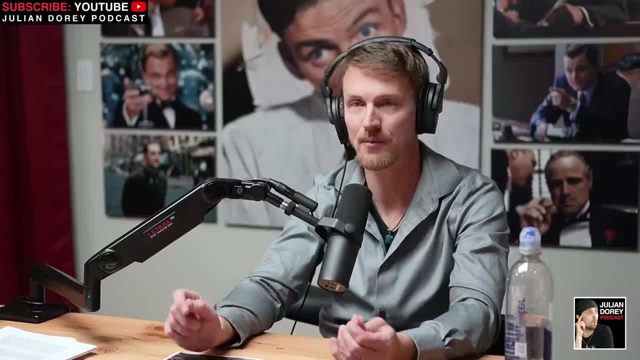 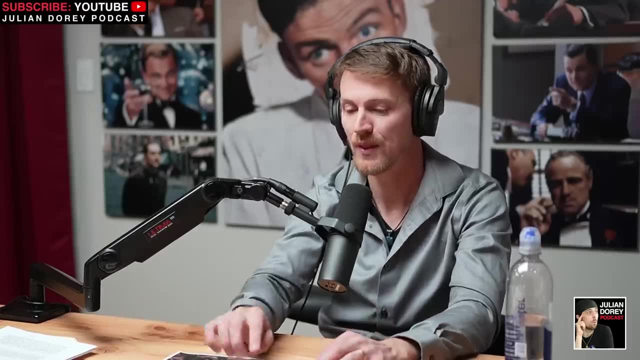 in mesmerism and he's passing the knowledge of that, and he's passing the knowledge of that and and here in other parts of the world, as a symbol for balance, balance with everything, because nature is perfectly balanced. we're just not. they're trying to say: look, you are not separated from. 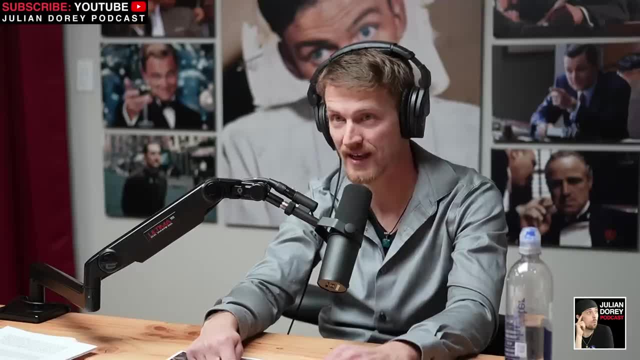 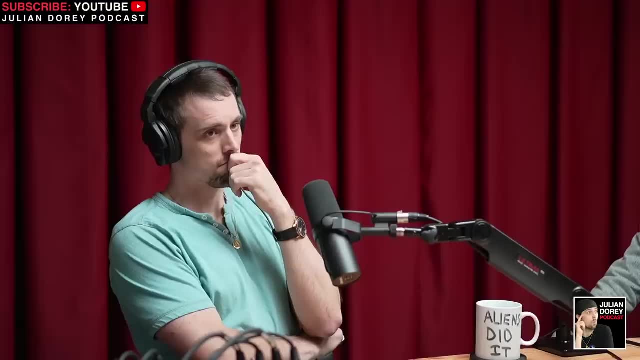 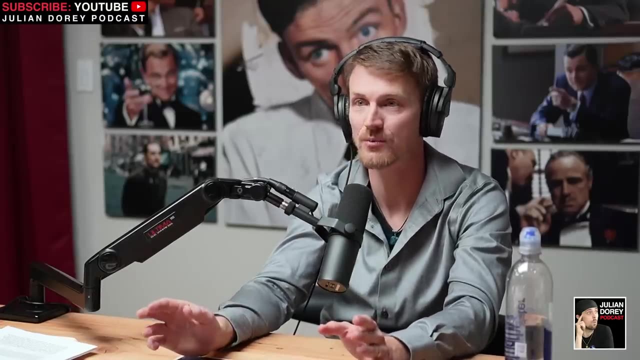 nature. if you want to reach higher states, just like nature, you need to find balance. and if you find balance, see how they're on either side of the tree of life. it's a focus because they're in charge. according a at the tablets, they state that these deities of sumer, they call the anuna, are in charge of 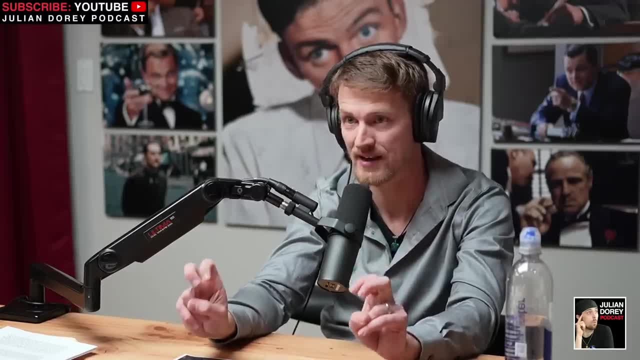 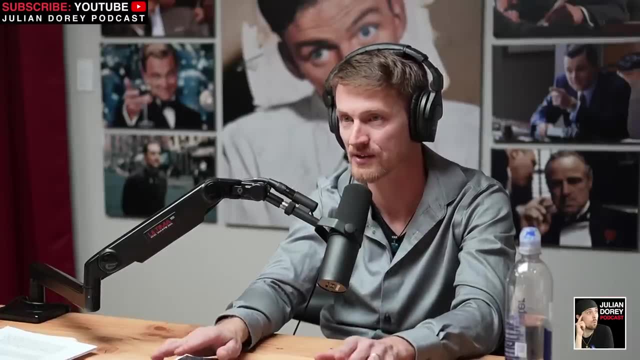 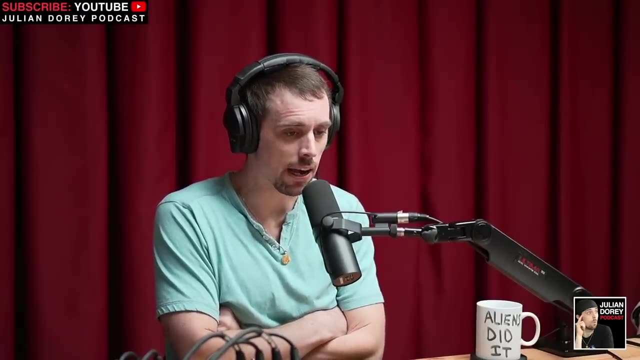 holding- and i put in quotes, that's a direct quote- holding and maintaining the balance. maintain the balance here. that's like their job. they're like in charge of that, supposedly in the tablets. okay, can i ask you a hypothetical here? i want you to pretend i am. 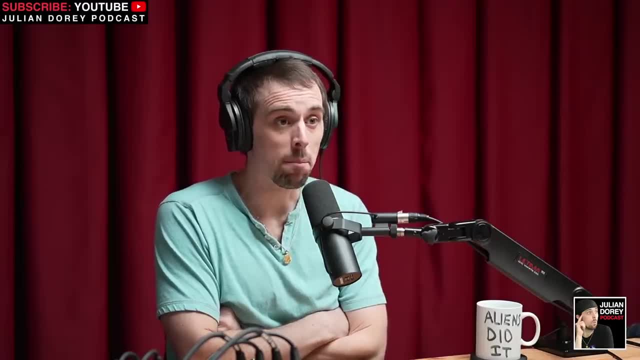 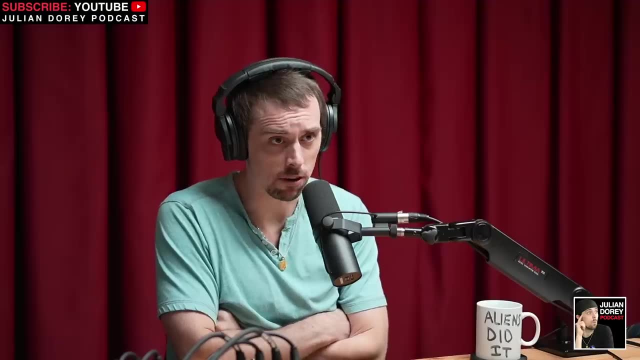 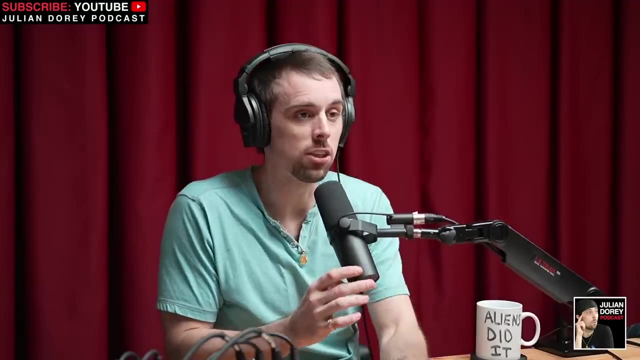 or no. you are a mainstream archaeologist- okay, but you're not a piece of shit. you're not like a zahi hawass? okay, you like. you're not an embarrassment to mankind- how else? and- and let me remove the word mainstream, let's say i am a dissenting on your opinion, okay. 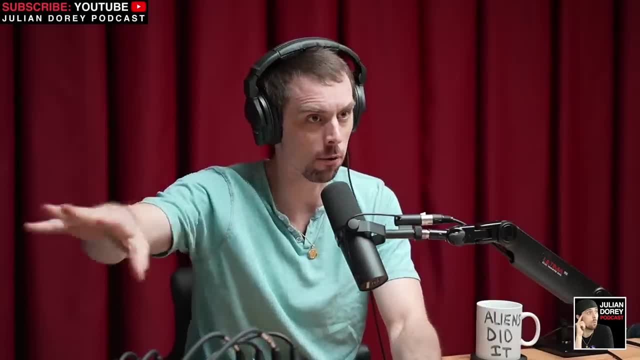 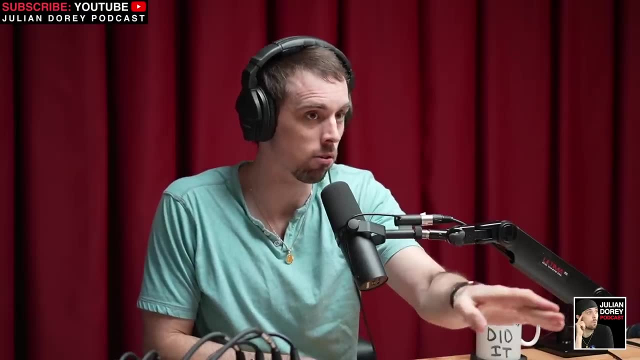 archaeologists, and i have no allegiances whatsoever to other people. i'm just looking for the truth. don't give a fuck if no one ever hears about it. right, you're not a piece of shit. what are the other ways that you could, or the main other way, if we're going to keep it simple? 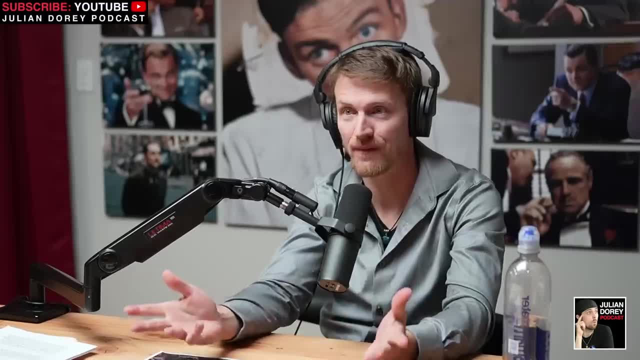 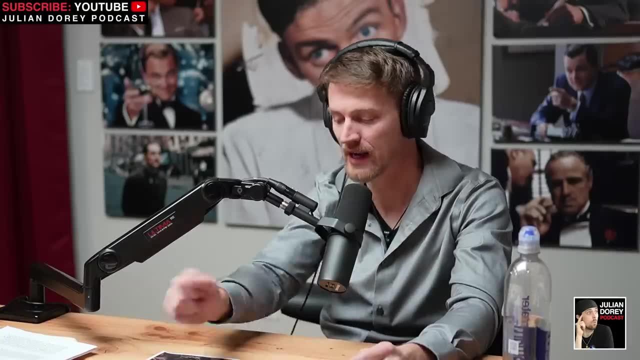 that you could interpret this. that is not how you interpret it. that's the funny thing is, i was explaining those archaeological papers and they did just that. i mean, i i printed them all off and i highlighted sections because the film we're making we might actually use that with an. 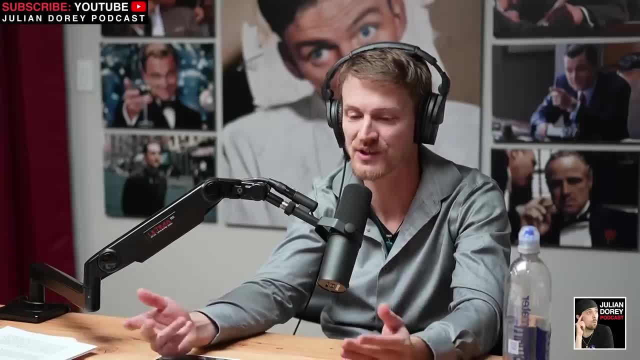 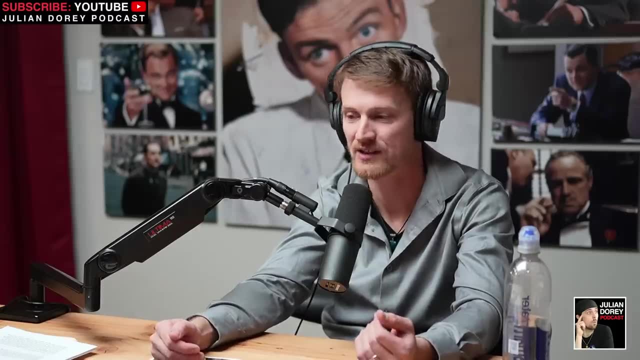 interesting way to. i mean, for instance, our idea with this film to be experts is that we're going to get attacked for not being accredited archaeologists. so i got smart and i realized i just took every single piece of paper and i just printed them all off and i highlighted. 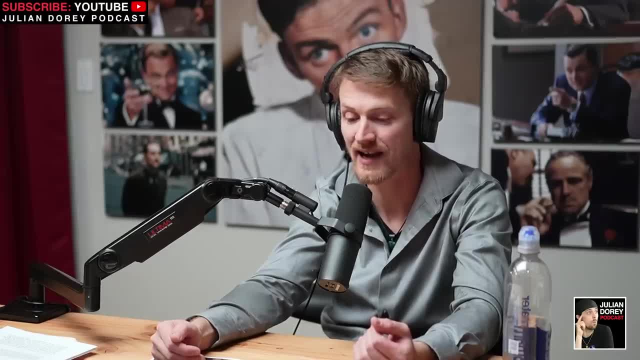 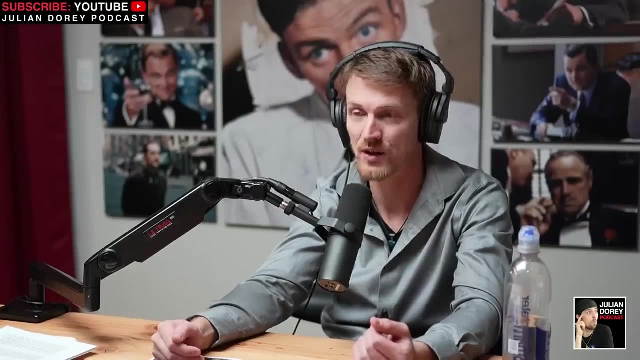 paper from all the archaeologists that wrote about the excavations on site and then just use their own words against them, their own quotes, them coming out and saying something doesn't fit or doesn't match or doesn't align to that, even not coming out and saying it's not the urartian. 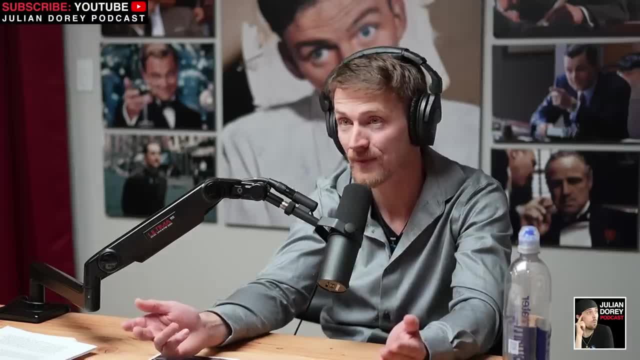 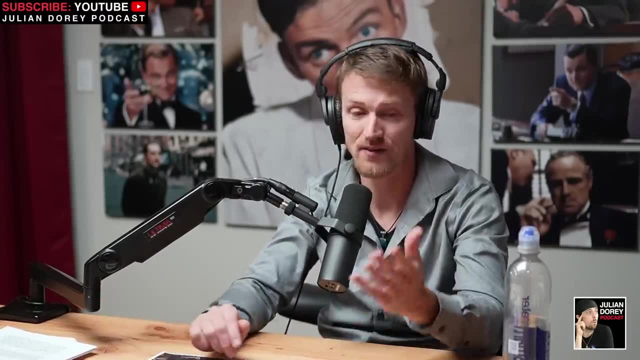 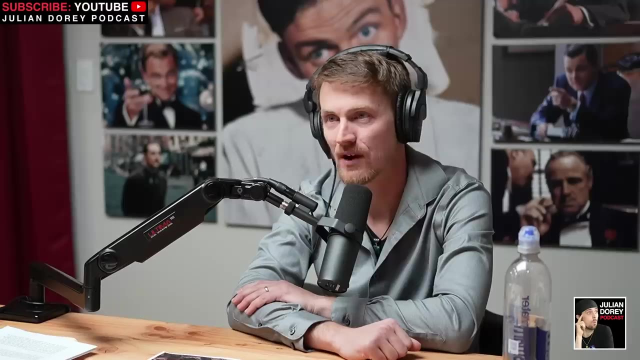 civilization. we can still read between the lines of what's very obvious in what they're saying. okay, and so i, i simply will. i will fall back on their papers and i'll say, look, it's almost laughable that they're trying to mold around their previous expectations of the archaeologists that came to. 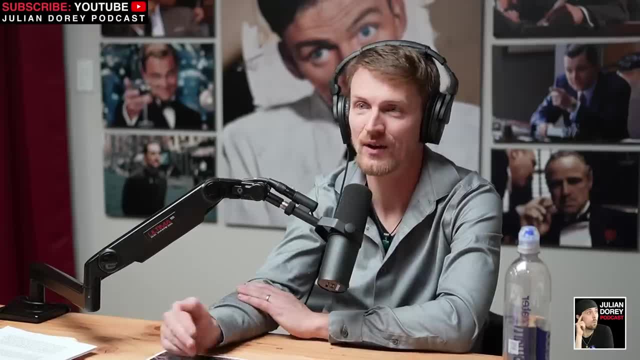 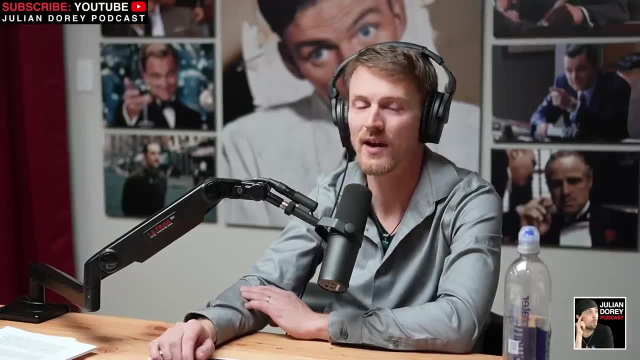 try to define those right. even they, even a child, could read some of those papers and know what they're trying to say. they could. it's like you know, when you want to say something so bad but you can't, so you literally like put so much emphasis on saying it but you don't, and everybody. 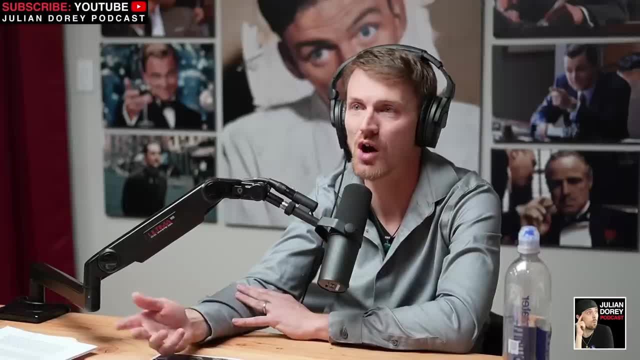 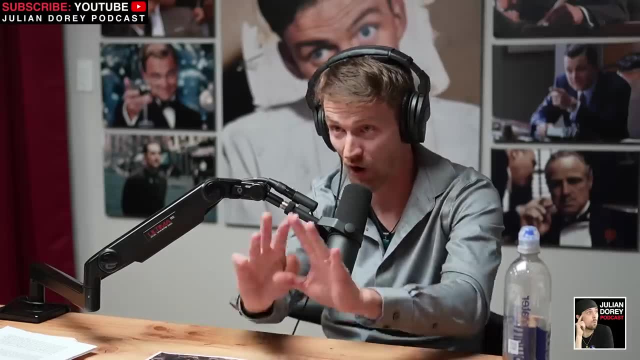 knows exactly what you're saying. yeah, if you're trying to hint so strongly about something, right like people know what you're trying to say, even if you don't say it. that's exactly what's happening here. is that the old narrative that archaeologists are kind of defending makes no sense. is like graham hancock. 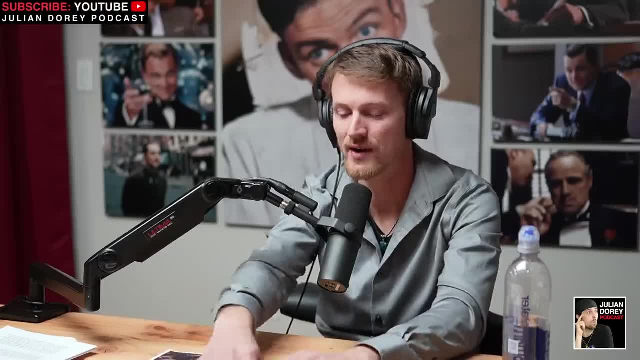 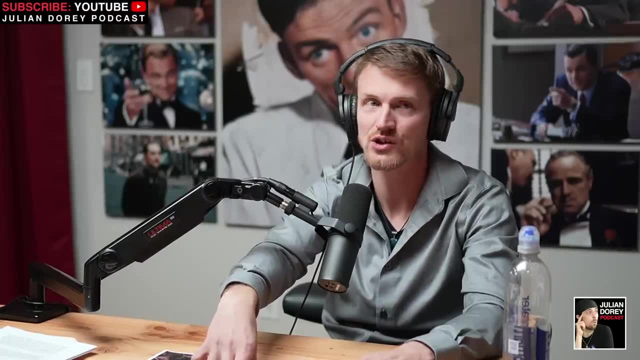 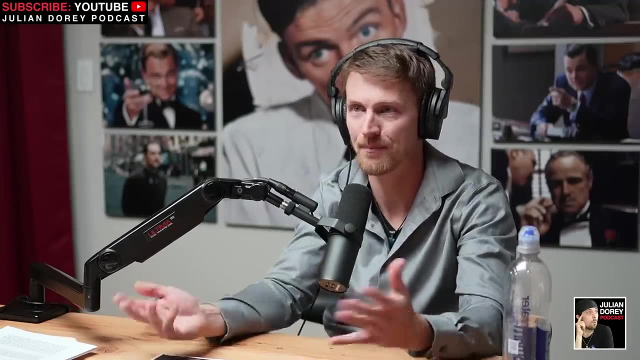 says it's a foundation of sand. trying to trying to associate these symbols in the in the kef box with a war like urartian empire is like trying to associate um, maybe like a mozart play with like a rapper. it doesn't make any sense. you're like not even the same place, right? i don't know if that's. 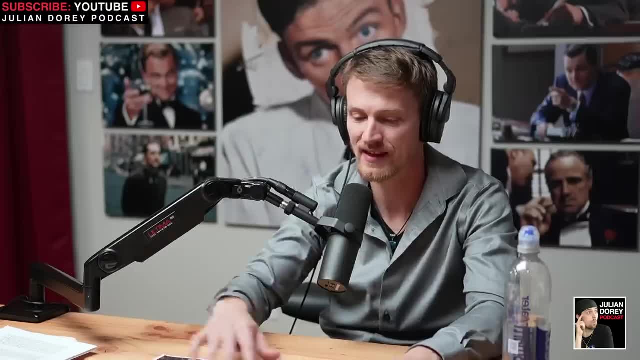 a good analogy, but that's what i'm trying to say. is that i think that's fine? yeah, is that? this is because we're talking about the ancient civilizations and the other way around? right, the depictions here, once you start figuring out what they mean and to know that you'd have to. 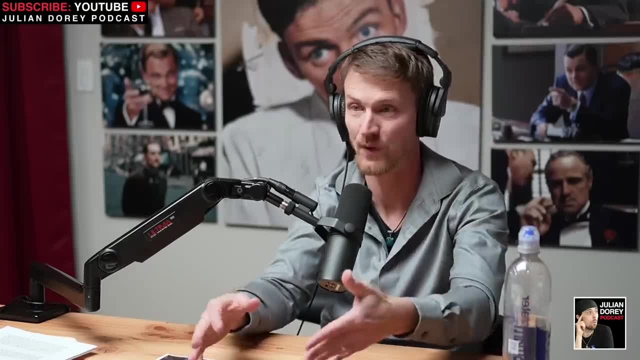 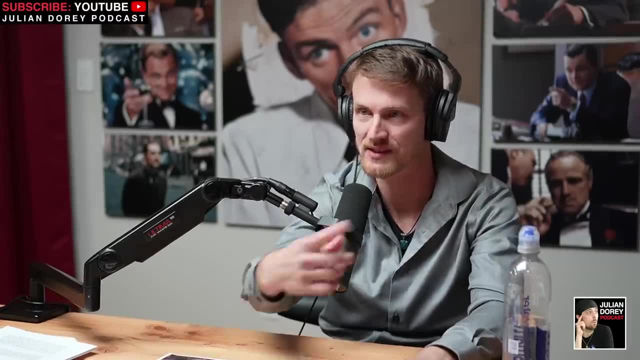 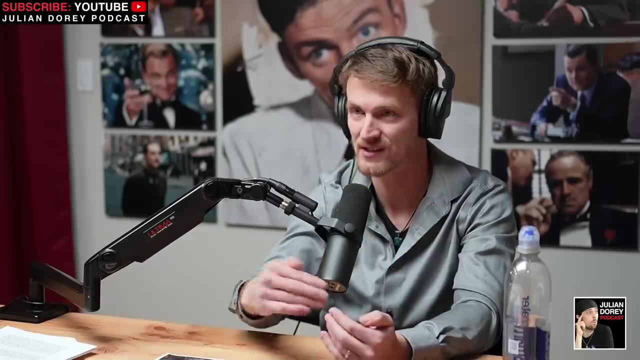 study ancient civilizations and symbols and try to carry them over, and that's what these are. is that these symbols are directly from sumer: the lion, the eagle, the griffin, um, the holiday symbols, the same as the anuna gods, um. it's all there. it's just a carrying over in another iteration of that. 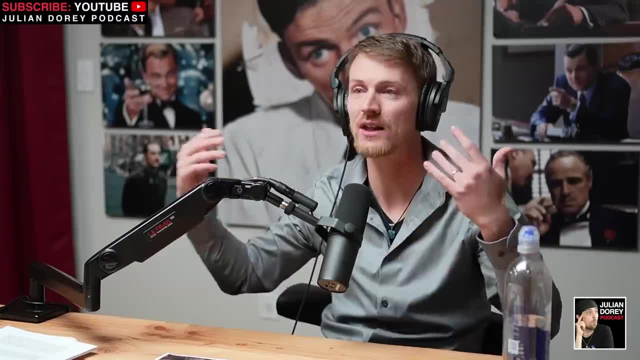 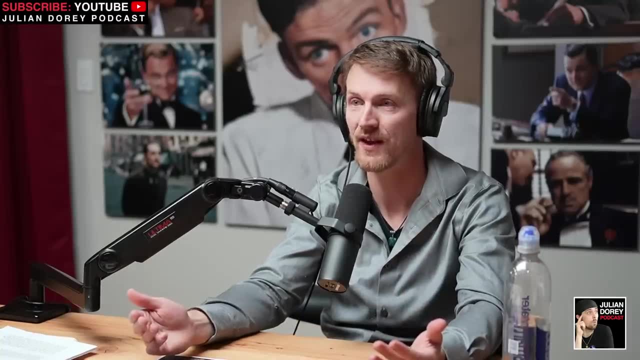 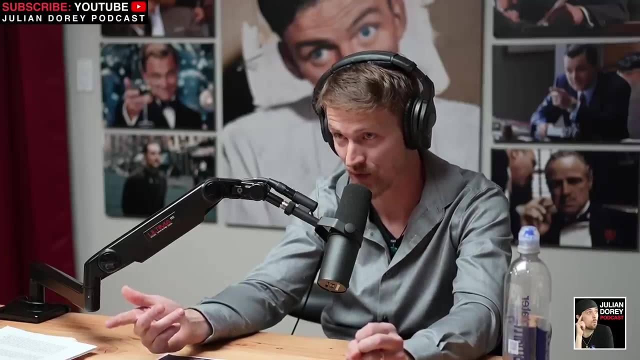 sumerian civilization after disaster occurred and it's like they re-lowered and tried to do it again, but this time they tried to do it in a way where i think the goal was that was what created what they call the golden age. you know, the yuga cycles out of out of the vedic text and hindu. hindu understanding is 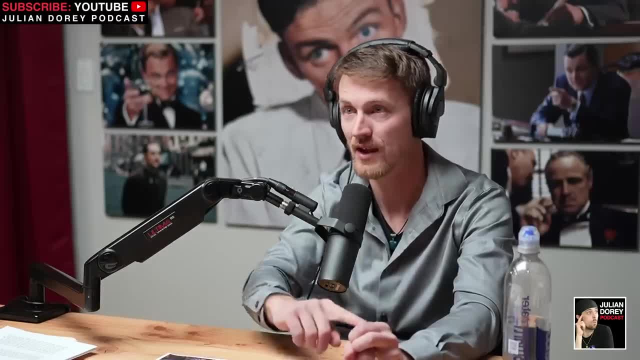 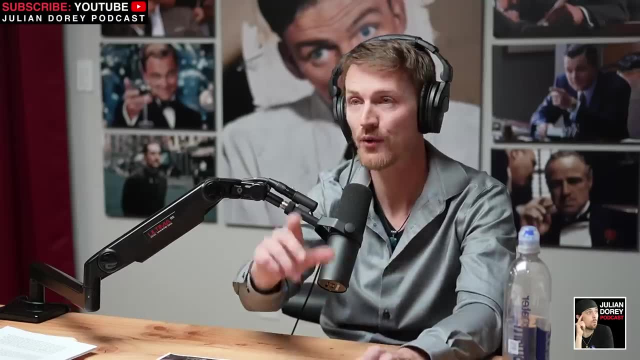 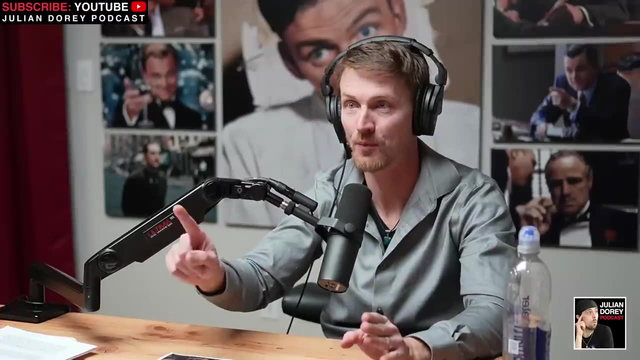 that the human beings, humanity, goes through cycles of like a 20 000, 27 000 year cycle, like the procession of the equinox, excuse me- and that we go through periods of what's called golden age, bronze age, silver age and gold age. golden age, right, and it wobbles back and forth on that. 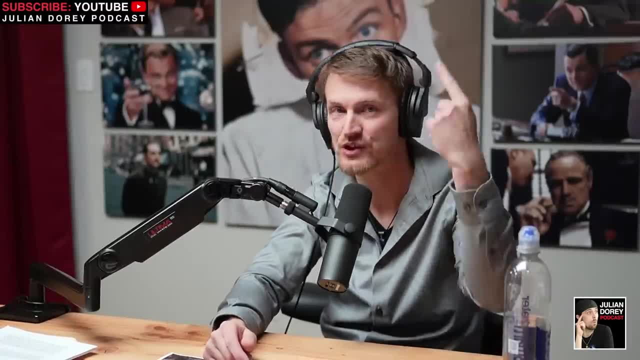 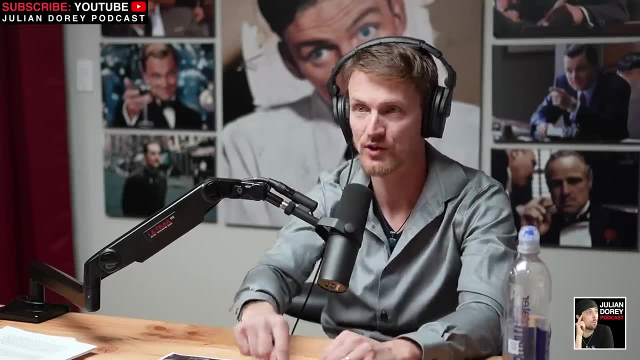 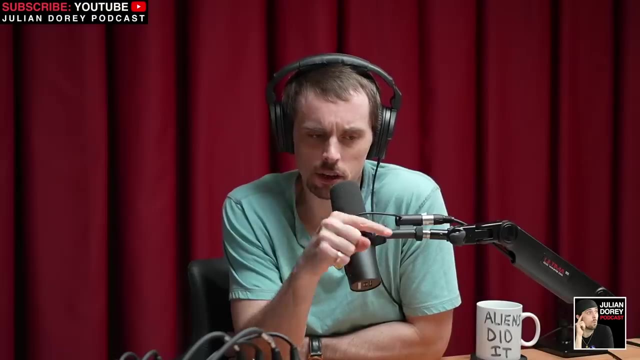 between cycles of energy. having to do the zodiac constellations in our unconsciousness and how that seems to be, they understood more what determines this rise and fall rather than random, just random- events. back that up a second. you said it goes back and forth between cycles. 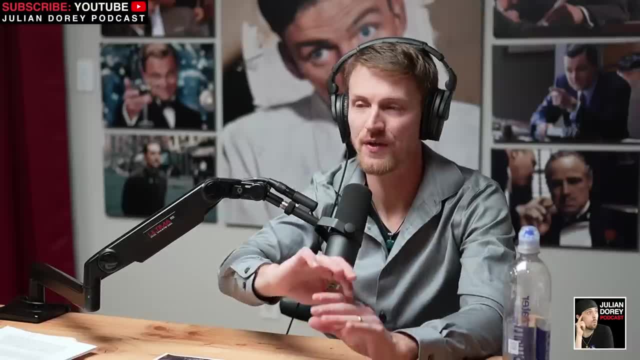 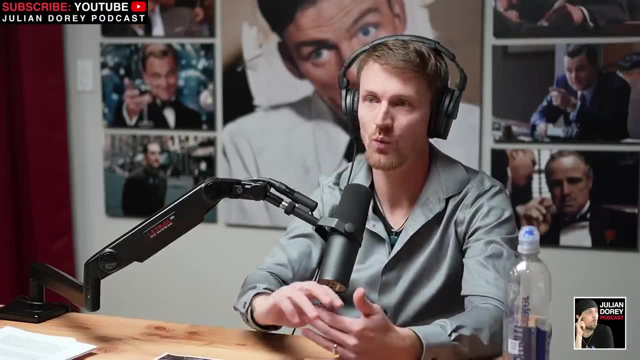 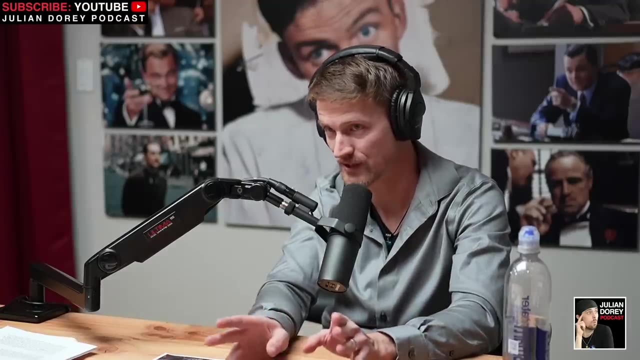 of energy and consciousness, or did i cycles of energy with you in time periods? so give me an example. like um, there are 12 zodiacs, and what it means truly beyond a birthday is that the earth faces different constellations every 2100 years. 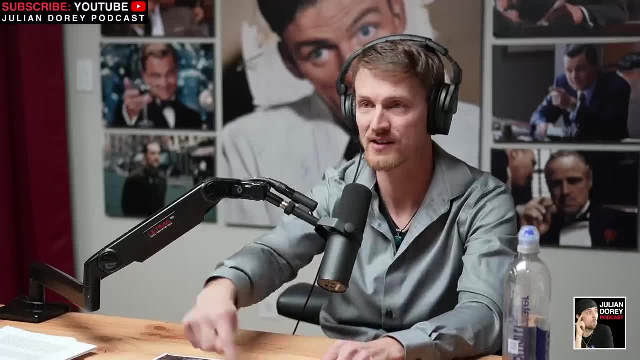 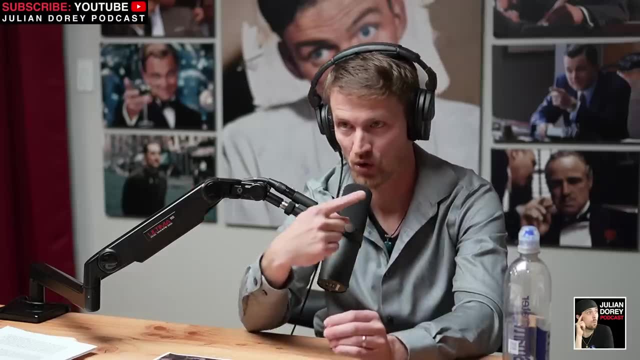 it's called the procession of the equinox, okay, okay. and that if you add up 2100 years by 12, you get 25 700 years. it's called the great year. it has to do with the earth doing a full, entire rotation of its viewpoint of the energy of the sky. 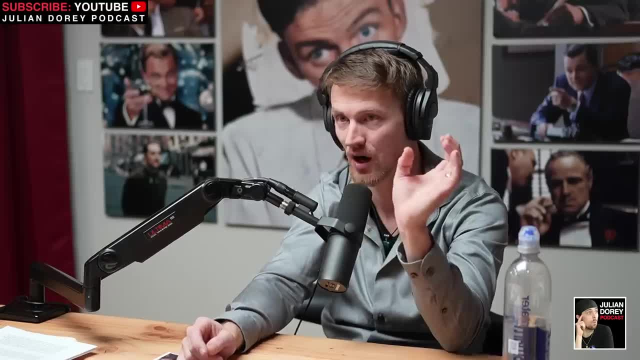 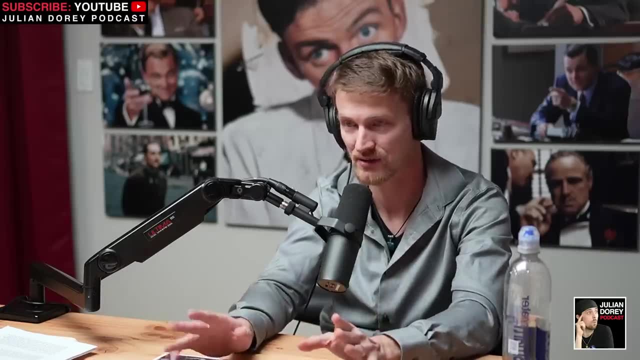 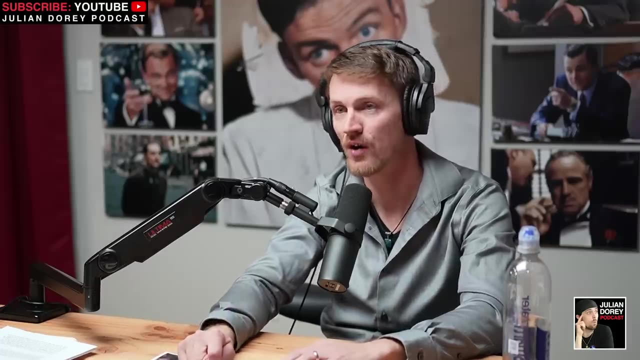 remember the hermetic laws. as above so below, the energy of the stars is actually a lot more significant in how it impacts here than we understand. it's all energy in cycles. all of this is okay. now imagine this civilization, this mysterious era. civilization falls into a time period of that rise, like the. 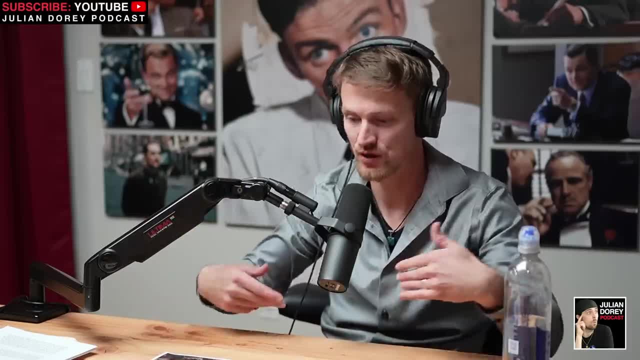 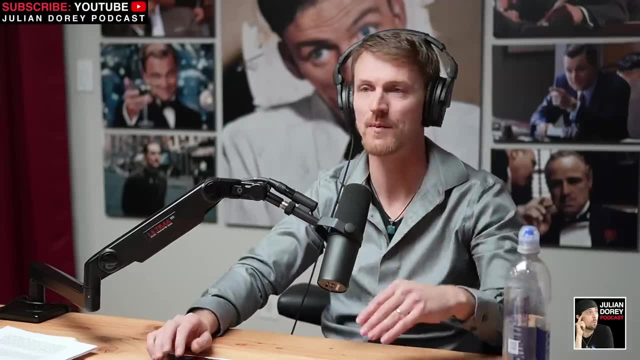 yugas, where it's supposed to be a golden age and they, like, they're the ordainers of cycles and destinies, and they're supposed to be a golden age. and they're supposed to be a golden age, and they're. they then lower the ultimate knowledge on how to build and do all those things everywhere around. 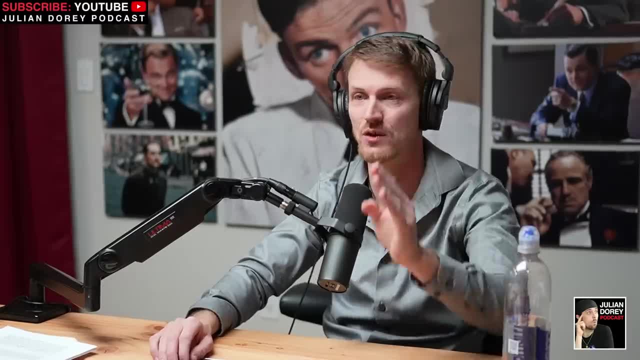 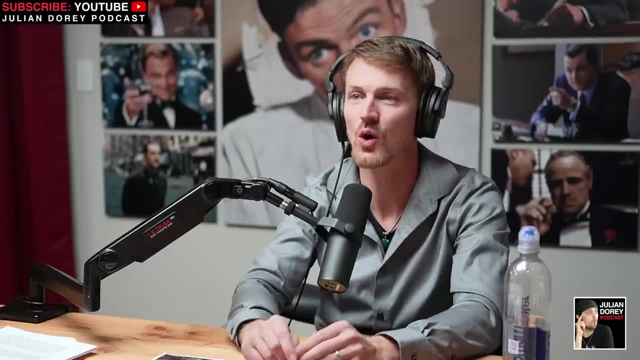 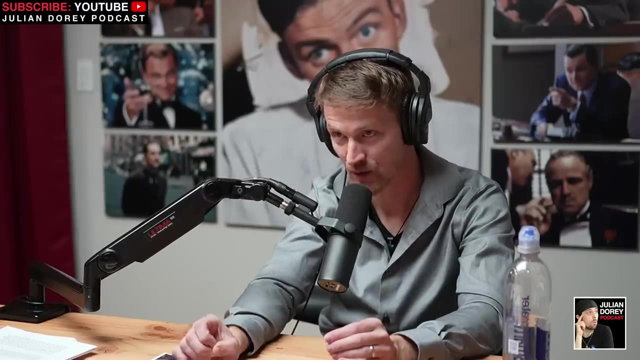 the world and the knowledge, the ultimate knowledge of how to reach buddha-like states. right, but then the cycle. what does the cycle do in the yugas? it doesn't go from a golden age to a silver age. it goes from a golden age to a bronze age, which means that you have to. it's inherently. 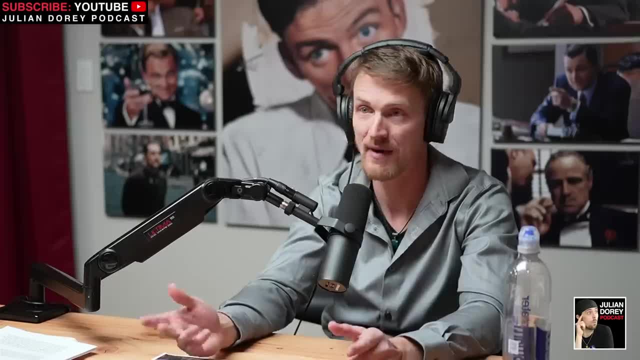 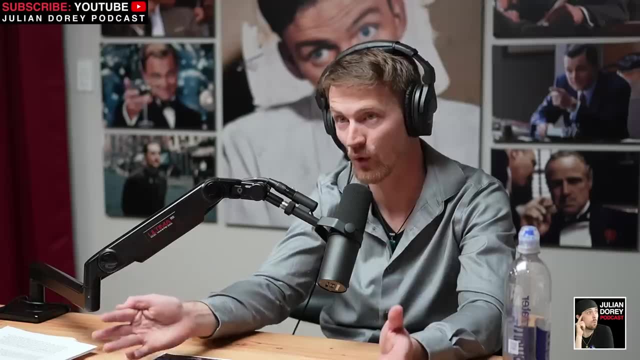 built into. whatever this system that we're part of is where humanity is, is brokenrado. It's like supposed to rise up, be almost wiped out and then have to rise up again, and that's happened over and over and over again, right. 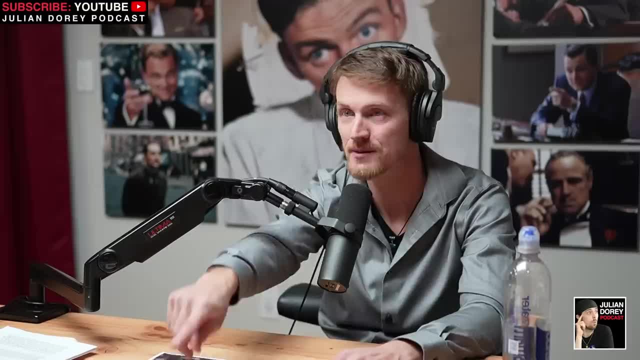 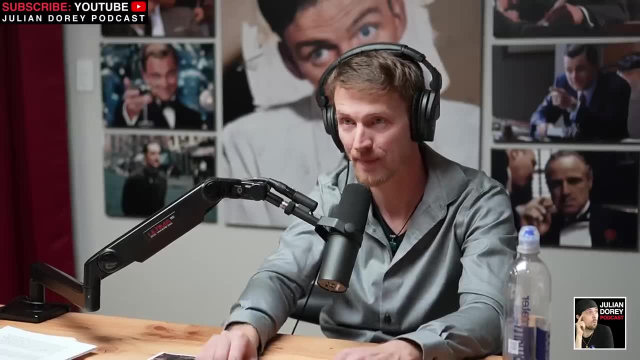 So, then, the point I'm trying to make about this civilization is: I think this may be the origin of the Golden Age that spread around the world, and that's why we're seeing the cross and the cup and the chalice and the pine cone, which we see all over the world. 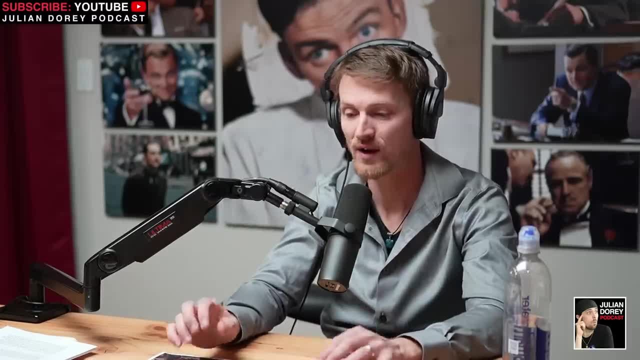 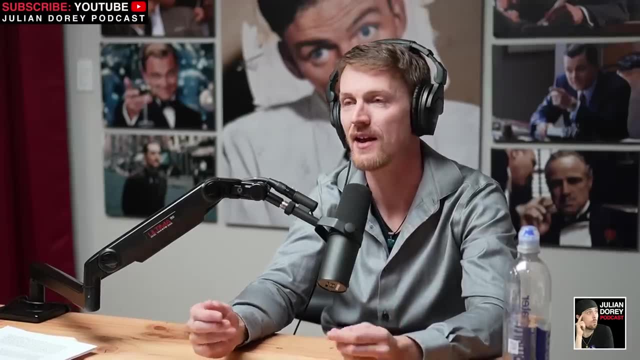 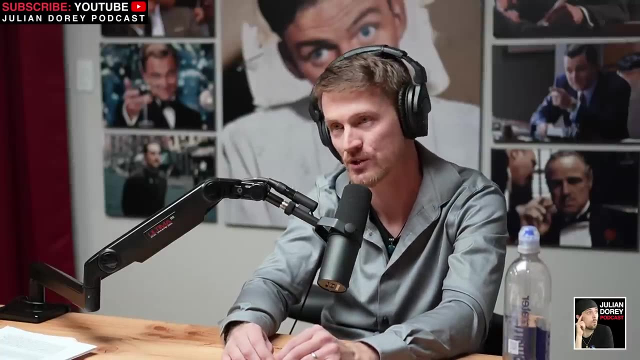 And this step pyramid doorway system, where it seems to be – it's almost like if you had – let's say, you had your own school, Julian's school of higher knowledge, right, And Julian taught – I feel bad for the students, Let's say, he taught those students there and then those students were supposed to go around the world and then teach what Julian taught them, right. 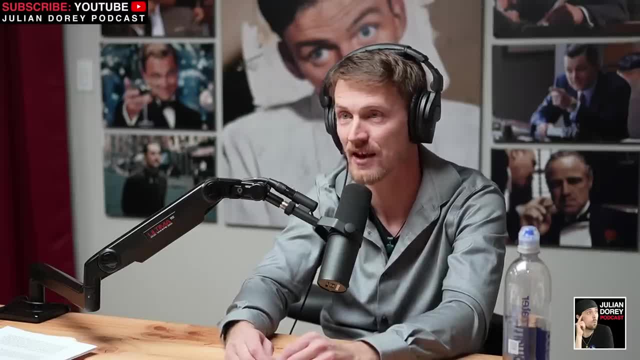 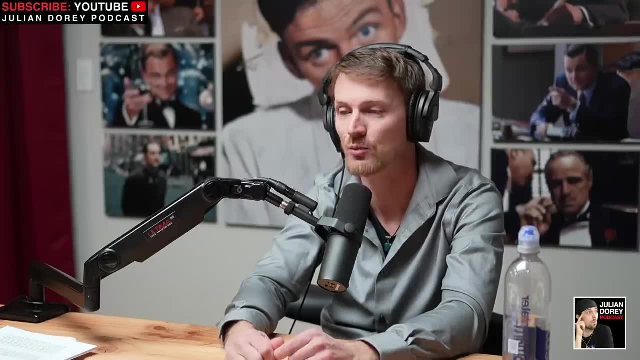 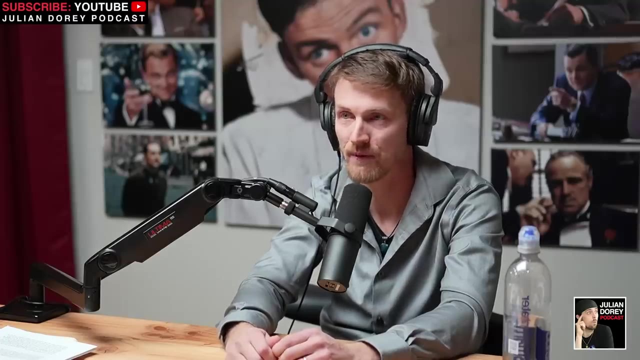 And then they go around and they teach it, and then they create civilizations as they go. That is what I think happened here, and it's why it's been – there's a term out of ancient Sumer called the Apkallu, and it's a term referring to a series of great sages that are supposed to be very wise. 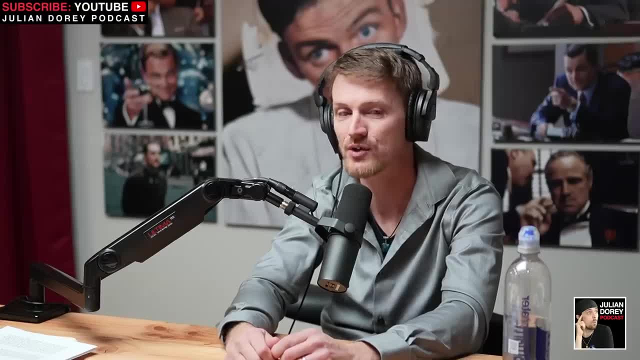 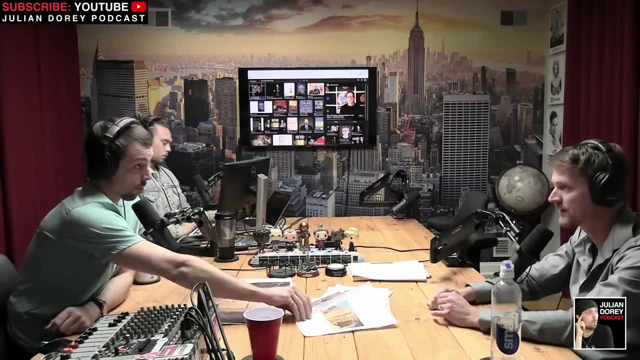 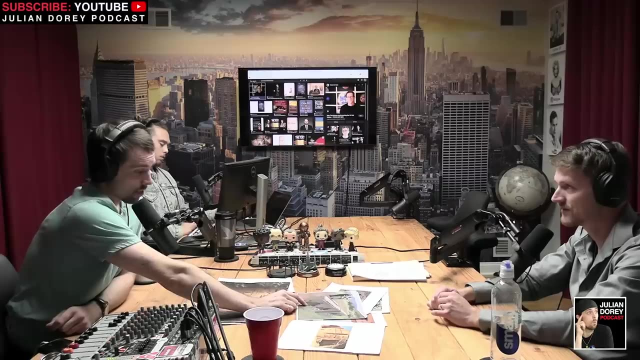 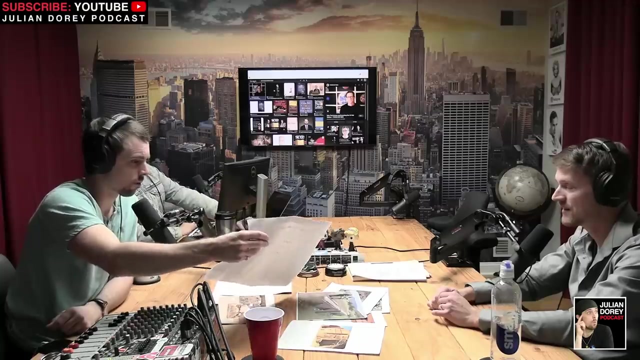 And very powerful individuals, who then travel around the world and create civilizations everywhere. And you were showing me – and this – now I'm going back to before we were on camera. Go ahead, Go ahead. You're showing me all the different places around the world where these step pyramid type carvings, which is what we're looking at again. unless you could probably put this back in the corner of the screen, this original – what do you call it? 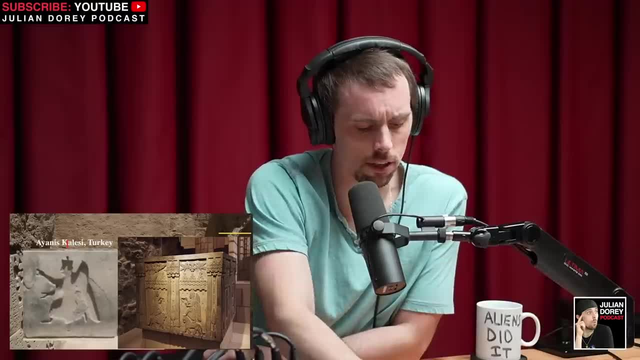 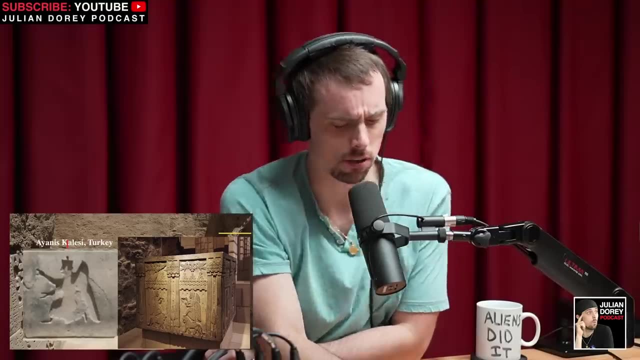 Box. It's Kef, Temple Box Relief Box Relief, That's it. That's the word I was looking for. We see the upside down – Yep, Inverted and non-inverted step pyramid. As you were describing them off camera, you were saying pyramids. I was like wait a minute, but that's – and you're like it's a step pyramid. 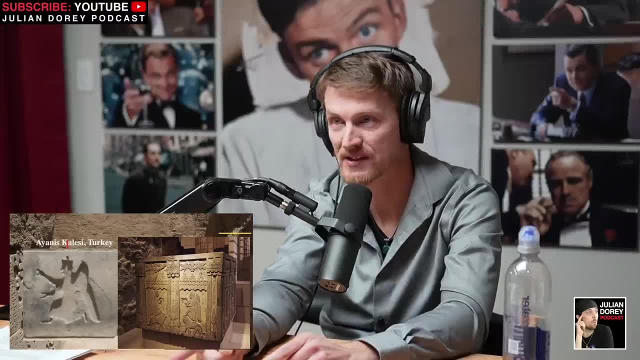 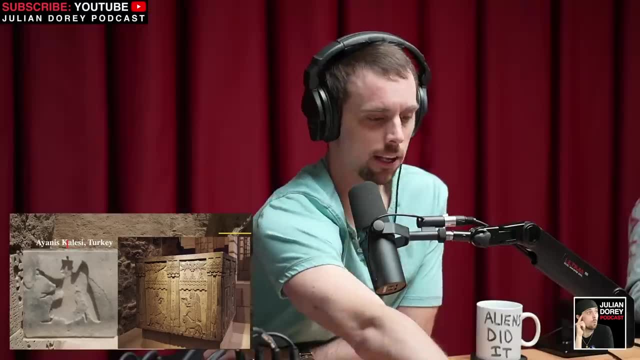 You ever see what a ziggurat looks like, Right, Exactly, It's exactly a manifestation of that. Yes, So now we see it in different forms around the world, but the same pattern, Slightly differently. Exactly Like: it's either in a diamond, like both, or it's facing upward or it's just facing downward. 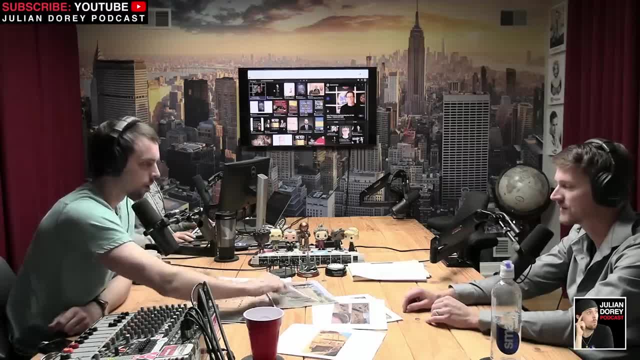 Like right now, I'm looking at Saudi Arabia, I'm looking at Tiwanaku- Yes, Where am I looking right here? That's all. That's Pumapuku, Tiwanaku, by Lake Titicaca, both of those. 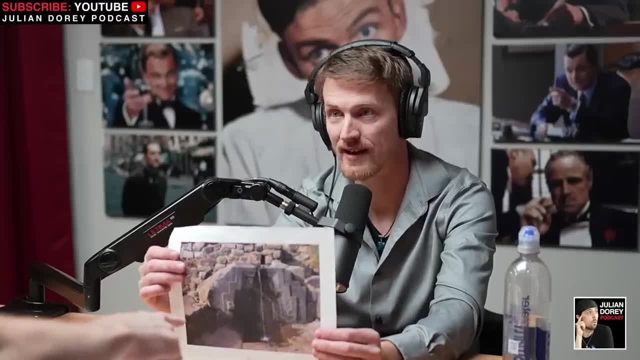 Okay, So these are all different. Now this is Oyetitambo, That's in Peru. This is Oyetitambo, not Machu Picchu. So now what you're seeing is – right, And look at this one. 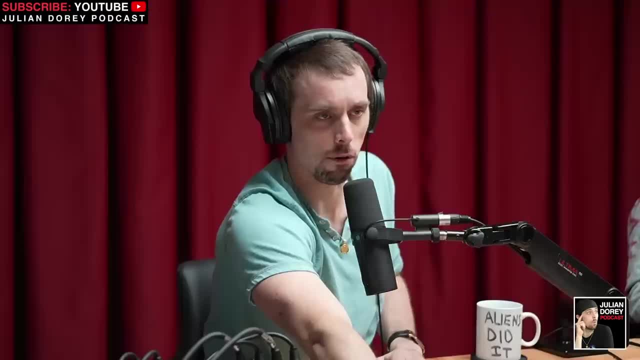 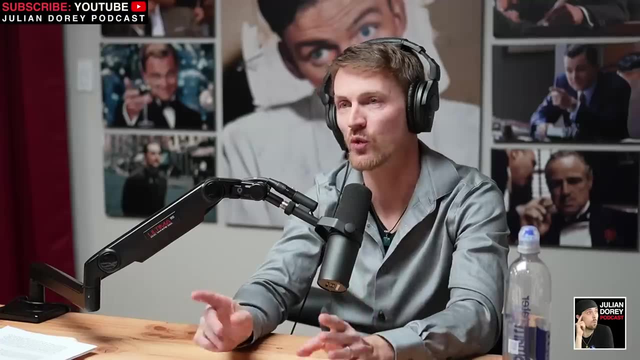 Wait, That's not Machu Picchu. Yeah, It's right next to it, though, But it's in Peru. It's Oyetitambo. Yeah, Yeah, yeah, yeah. But I mean, what you're seeing is that that step pyramid is not really like a physical representation. 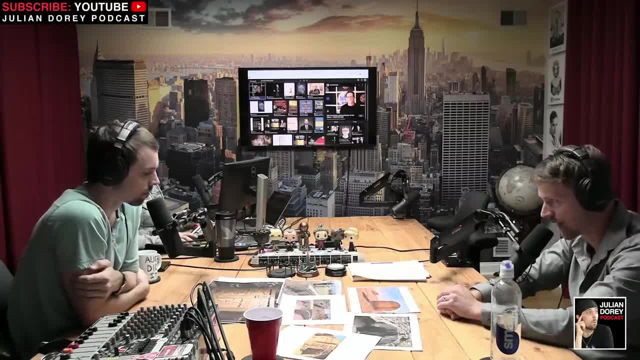 It's the – you see the levels. How many levels are on that step pyramid? Go up, up, up up. Which one am I looking at? No, The one there on the box is three. See this Look. Show me where you're looking. 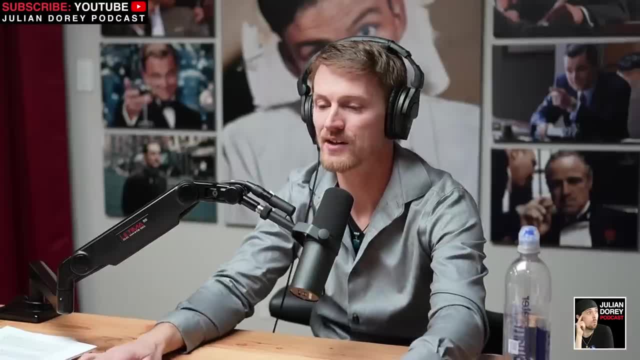 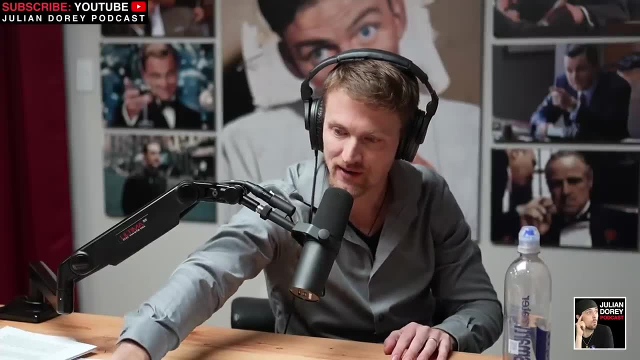 One, two, three. You see that, Okay, Yeah, yeah, yeah. Now that totality of three is everywhere in this civilization. Yes, And you can see it. Not great, but you see how there's a T-shaped pillar and then there's three indentations on that – the central pillar right there. 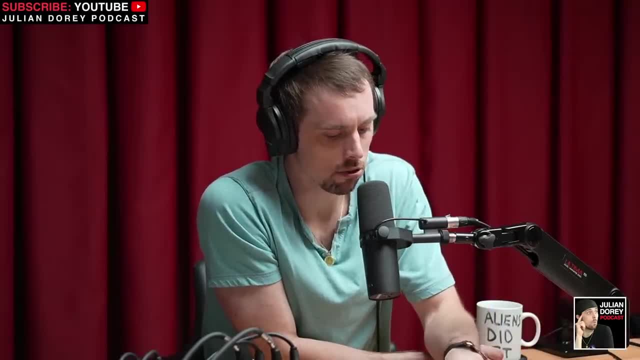 So for people following along, when they're looking in the corner of the screen, we're looking at the box relief and you are looking on the right side, Above the tree of life, Above the tree of life. Okay, There's three little –. 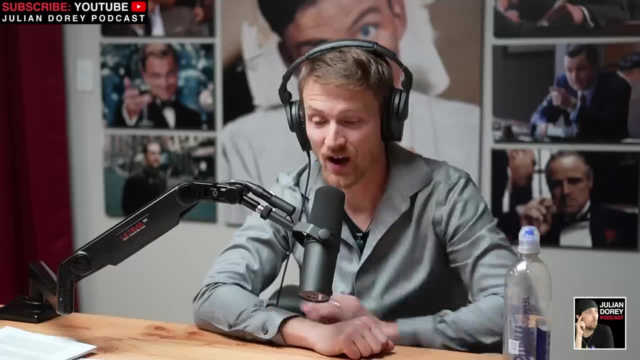 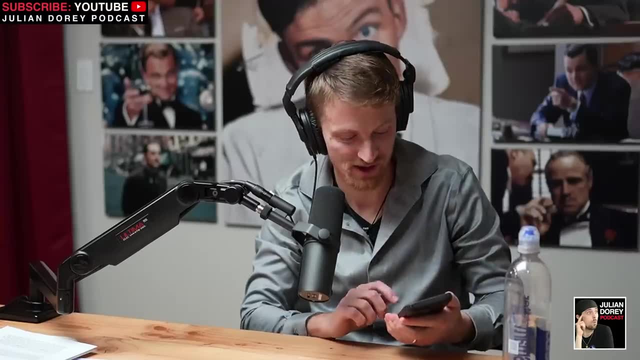 There's three little things we see carved into the stone within that pathway. Now you want to get really exciting here. I always want to get really exciting here. Come on, Matt, Let's go. Okay, I'm going to show you a picture, because I don't have it on – my phone's not on. 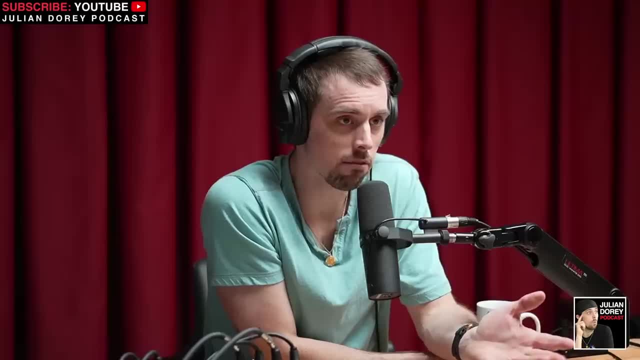 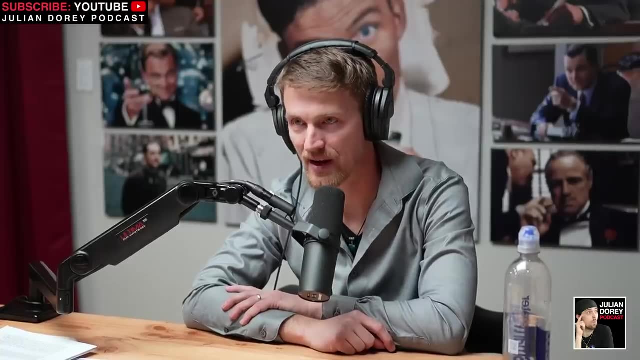 I'll show you it later, but I found – You just got me excited for nothing. I'll get you images. I'll get you images of it up later. Go ahead. I was at Cavistepi. There's people that do some tours like limited, not much, and someone had taken –. 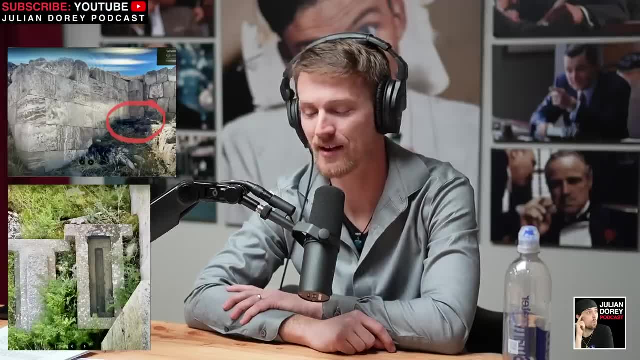 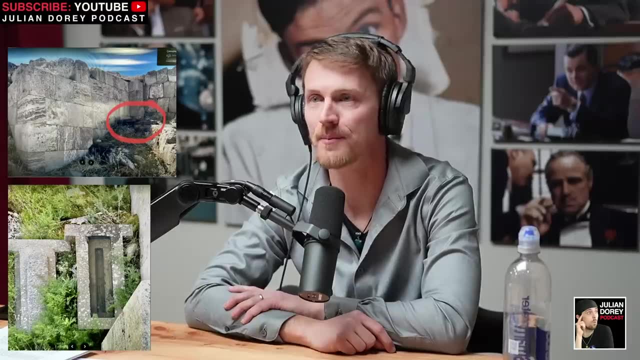 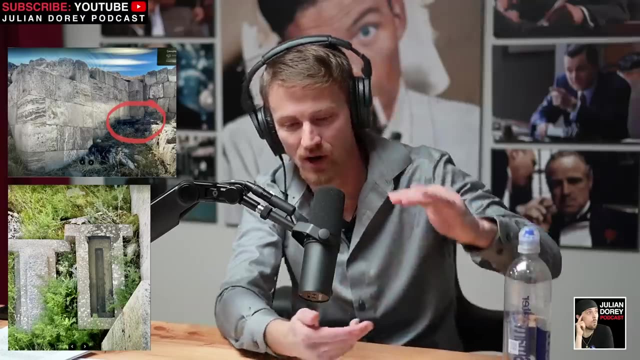 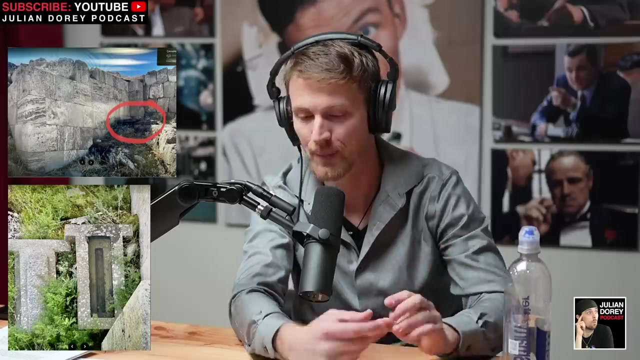 And I'll get an image for him to put up on this. okay, It's wild. Someone had taken pictures of the site and I'm looking around to learn as much as I can. every angle everything. right In the corner of one of the walls, of these megalithic walls at Cavus, there was this artifact- two of them maybe, like a foot and a half tall somewhere in there- made out of basalt. okay. 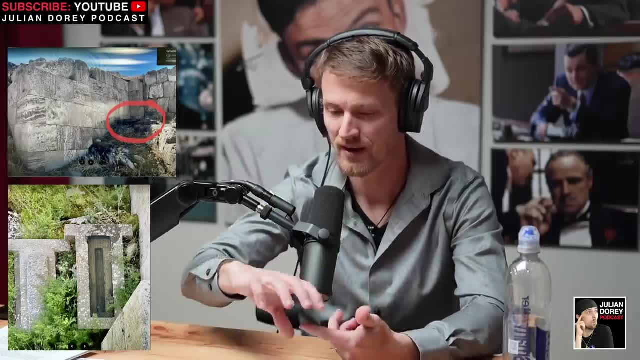 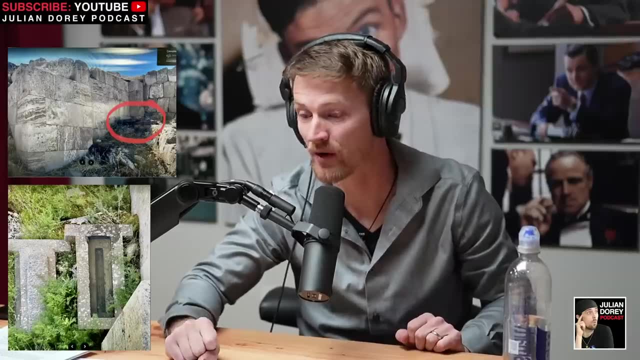 Beautifully, like perfectly sharp edges, like cut your finger on them. still Okay, These two artifacts sitting on the ground, like in the dirt, like nothing around them, just sitting there, You could like walk up in there. You could probably like pick them up and bring them home. 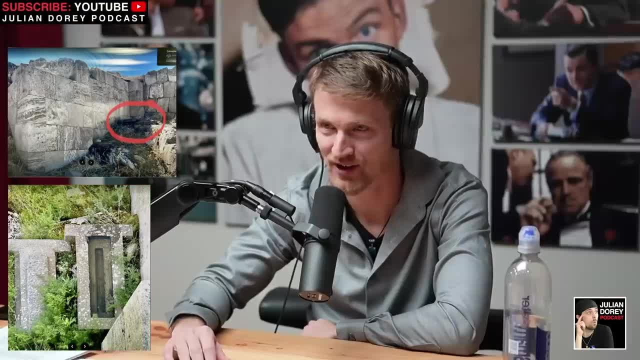 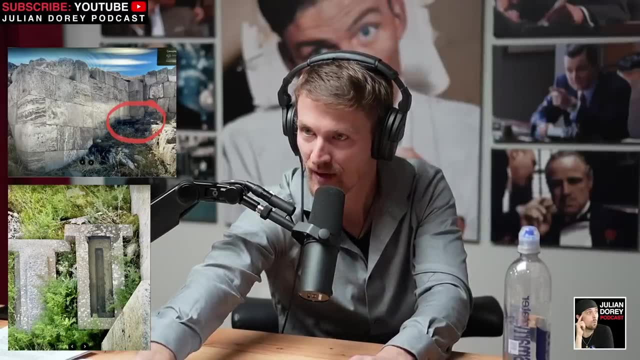 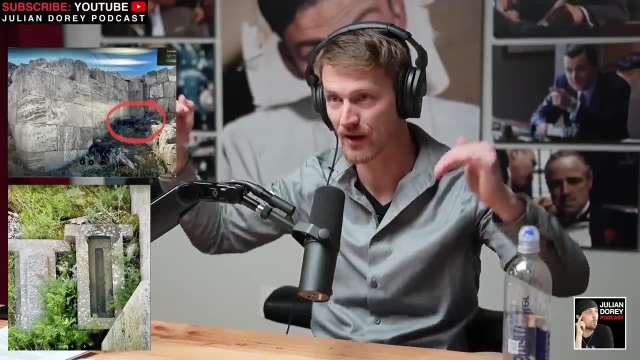 Not that I want anyone to do that. That's illegal, by the way, And I will find you if you take those out. That's pillar. I found the exact artifact for it. The exact artifact with the same indentation. three, with the top pillar that looks exactly like Gobekli Tepe. and when you go to Menorca, Spain, 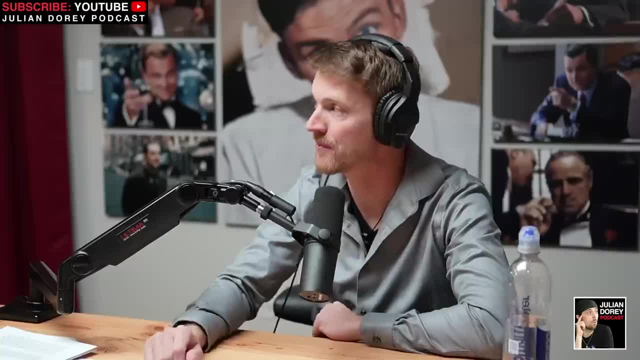 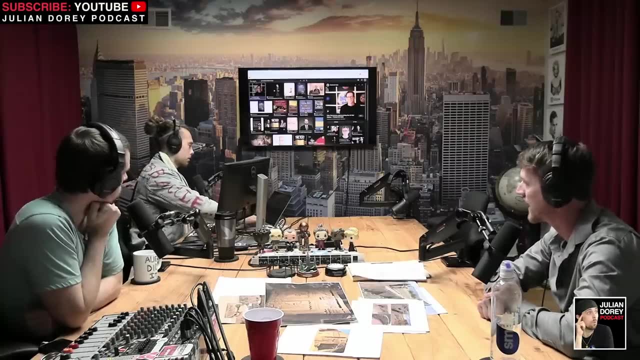 Do you get the exact same shape? Can we pull up Menorca, Pull up type in Menorca, Spain, for a second? and I want you to compare to that symbol for a second. You ready? Menorca- M-E-N-O-R-C-A. 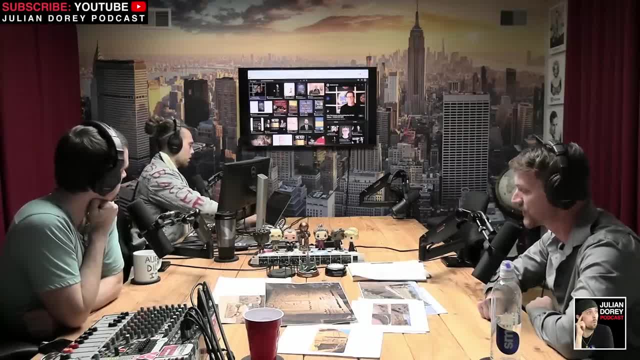 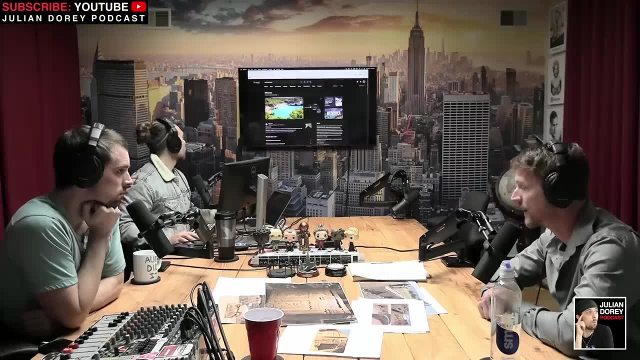 Good question, I was thinking that myself. So it's in the Mediterranean, It's an island. It's not really like Spain as we think of it, It's just owned by Spain, but it's an island in the Mediterranean, okay. 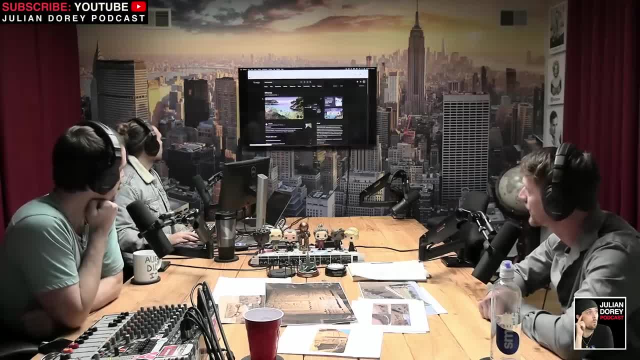 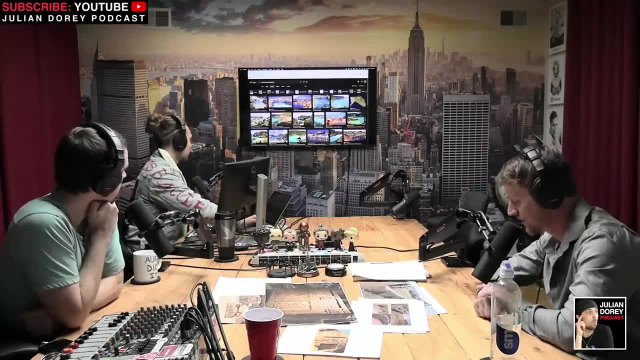 Why are there so many islands like this? They're actually the closest to something else I know. Go to images really quick. Type in: Menorca: T-shaped pillars, T-shaped pillars, Yep, Okay, Okay. so That looks beautiful, by the way, Holy shit. 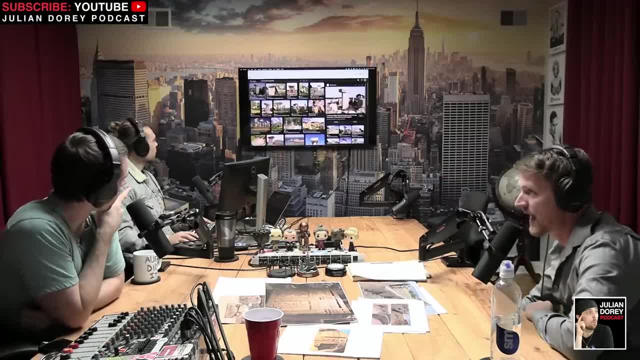 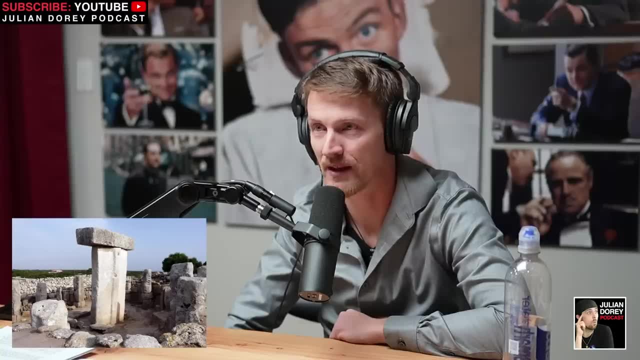 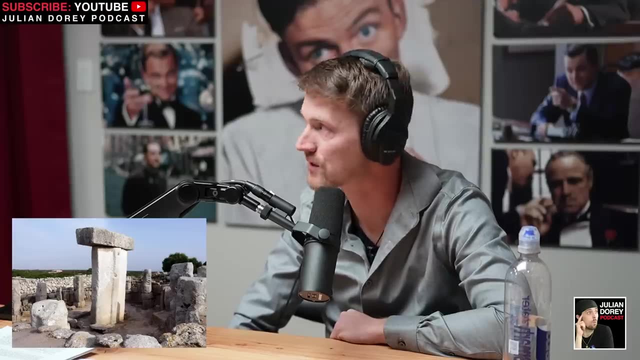 Okay, now click that first one. That pillar That's Stonehenge. looking right there, That pillar is more advanced than Stonehenge. That pillar is 20 feet tall. 20 feet, You literally would be like a little tiny person next to that. okay, 20 feet is the tallest T-shaped pillar of Menorca, Spain. 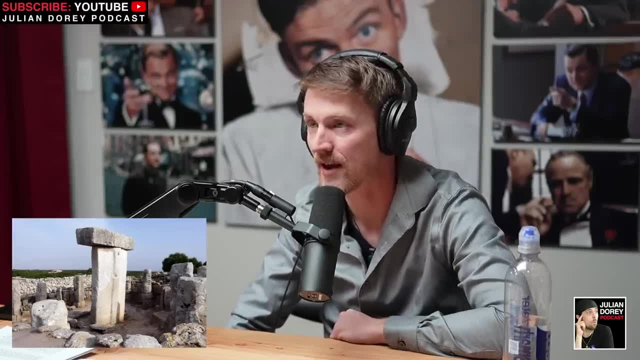 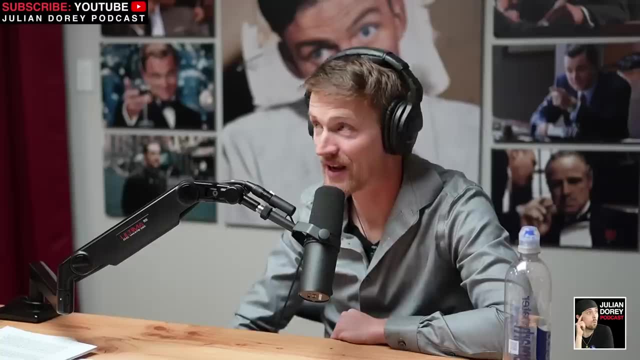 Nobody talks about Menorca. People all talk about Gobekli Tepe And the reason is that they're archaeologists. Okay, The archaeologists. and the mainstream is convinced that that's a lot younger, but I don't agree. Why not? 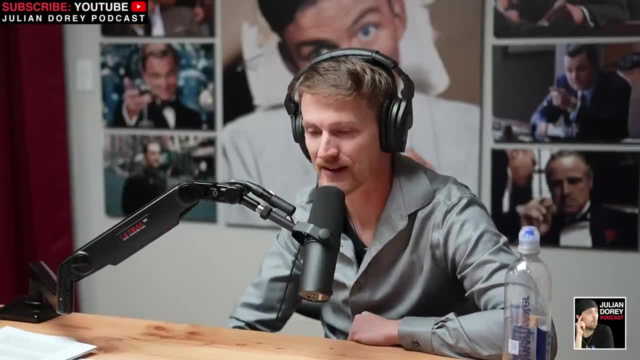 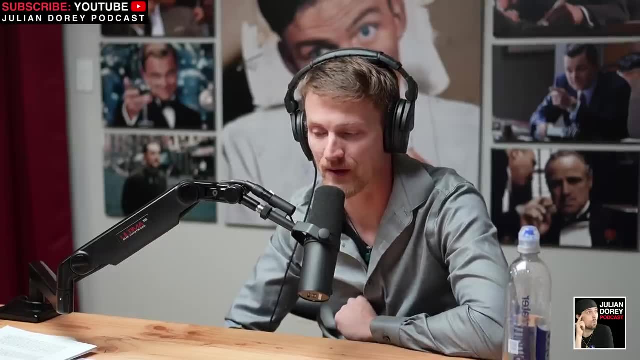 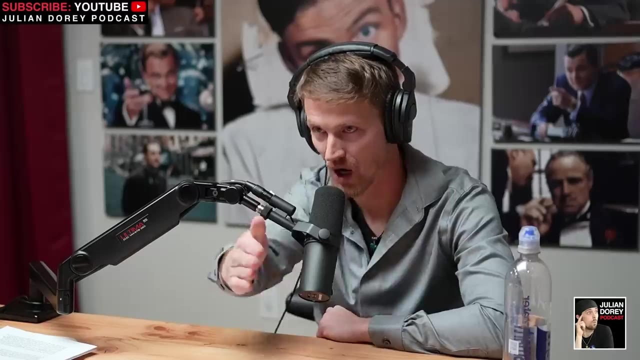 Because that is the exact shape and the same type of highly sophisticated megalithic design, with these enormous stones, that we see in other parts of the world. And I what I'm- the theories that I'm putting forth- is that this civilization, with its sages, moved to different parts of the world and taught different things as they went along. okay, How big do you think this civilization was? Or is there no way for you to really know? You do kind of know, because you can't have a civilization that's small. if they're making very elaborate cultural things, They have to be somewhat of an advance. 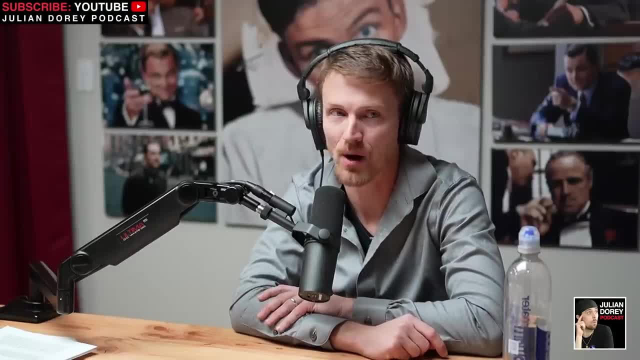 Yeah, but what's big, what's small? Big would big back in this time period would be probably anything over 20,000 people. Okay, All right, Sizable. yeah, I'm not saying there were only 20,000 people in this civilization. 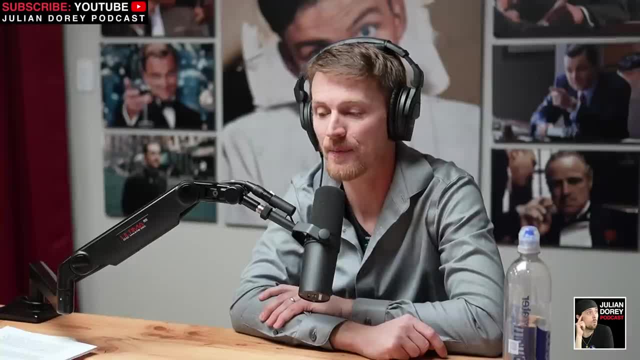 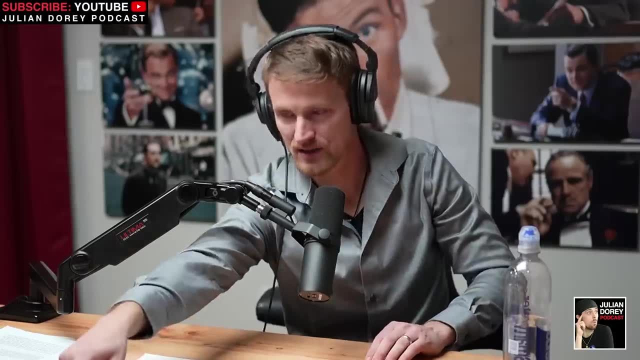 But it was at least 20.. At least 20,000 people, Okay, And It's like the bottom half of Hoboken, Bottom third of Hoboken, Right Give or take. Now Crunch fitness. Going back to that for a second, look at Ionis for a second. You see how I've circled, what's called the hourglass. 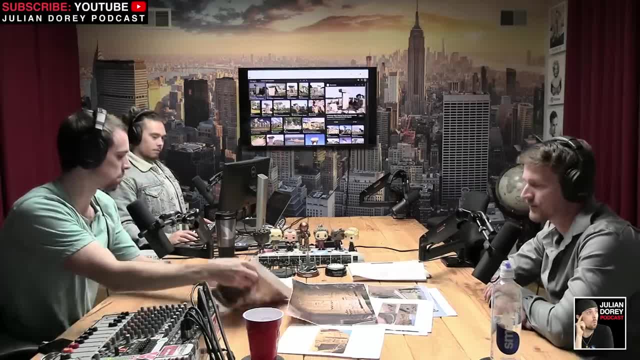 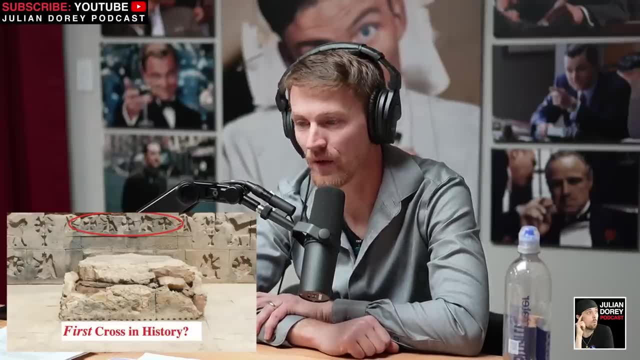 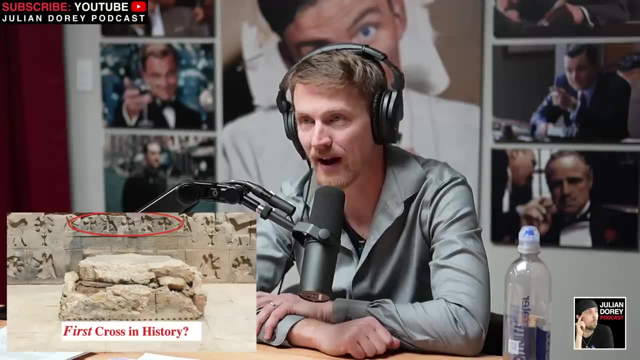 Yes, Okay, Right here on the left, again the left of this picture. Now take all those symbols for a second and put them together. What does that mean? Well, you have a sun symbol, you have an hourglass symbol, you have the cross symbol right, And then you have this Haldi, which became my company logo. 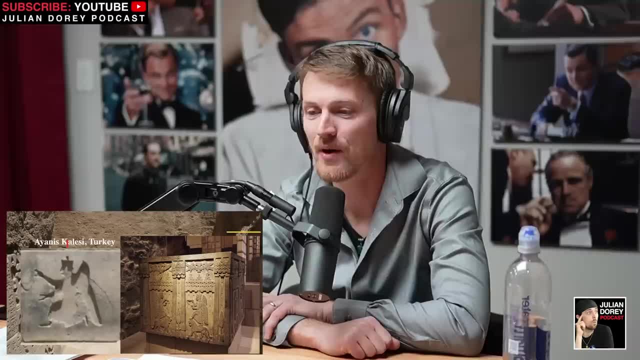 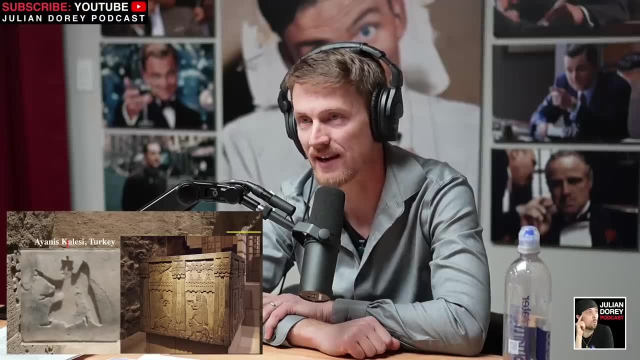 Yeah, Which, yeah, right, Passing all of those things or showing that he's protecting them. And you notice he's kneeling on one knee. Okay, Kneeling. Notice that he's kneeling on a knee. What's he doing with his hands? 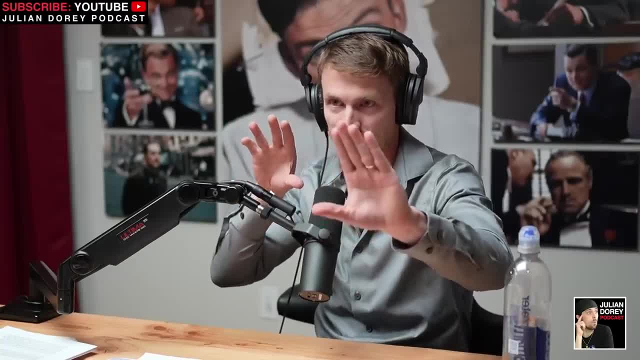 He's like this: Am I fucked up right now? Isn't like the devil symbol, like that or something? He's not doing that. He's going like this. He's not doing that. He's doing like this. No, no, He's like passing, like passing something, Okay. 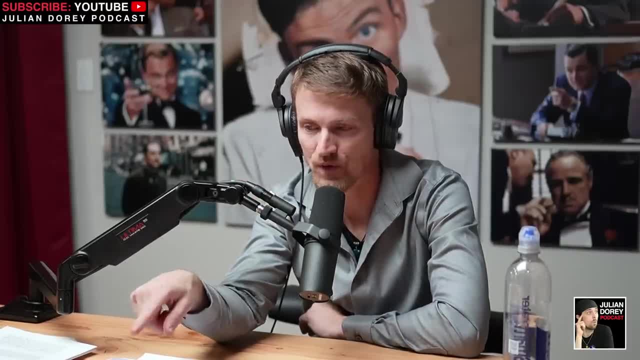 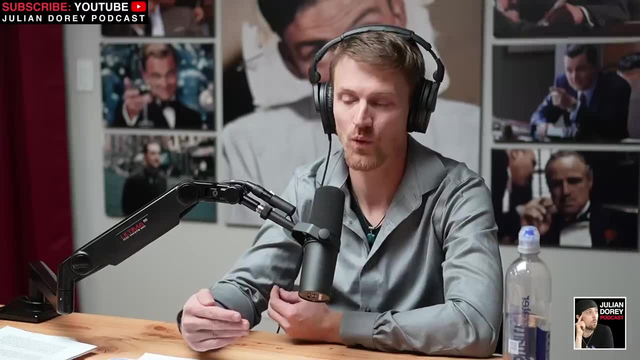 Okay, Now Let's put it all together for a second. It's telling you something, Okay, The sun: we know it's a sun temple, so they're aligning it to the different equinoxes and different, you know, different things with the movements of the sun. So for them, the most sacred, there's two time periods that was most sacred of all the ancient civilizations. Take away our holidays For them, the summer and the fall equinox. spring and the fall equinox were basically the most important two times for them. 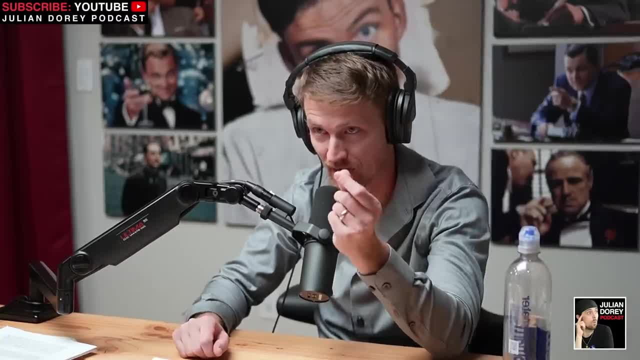 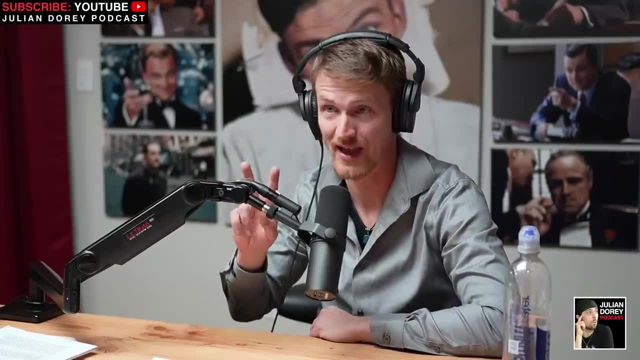 Okay, The time period when the sun comes directly vertically over your head. Okay, That's the equinox. that's what it means. An equinox simply means that the sun it's only two times the entire year. this happens, Right? That's why they're called that. The sun passes directly overhead. Yes, So for them, because they're worshiping the sun, because they believed the sun was God, Okay, They called the sun anu or utu, depending on how they want to use it. You're going to take my next question right out of my mouth. Keep going. 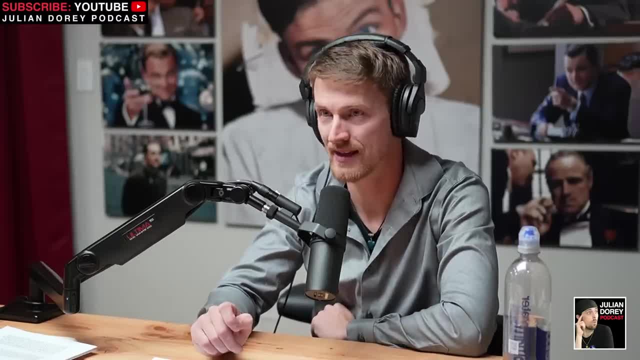 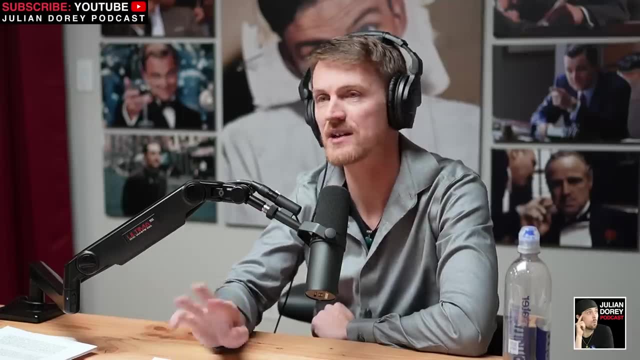 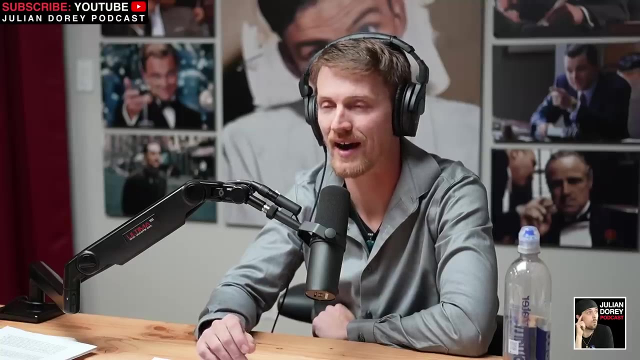 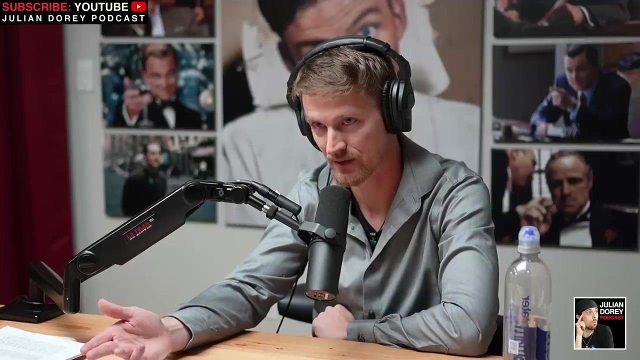 So they believed that the sun was a divine intelligence of God, okay, And that they believed that stars, the sun, are very different than we perceive them today. They're not just plasma gases that float around, whatever That they are actually like, have a lot of intelligence in that the cycles of consciousness on Earth may be related to the sun cycles- okay. 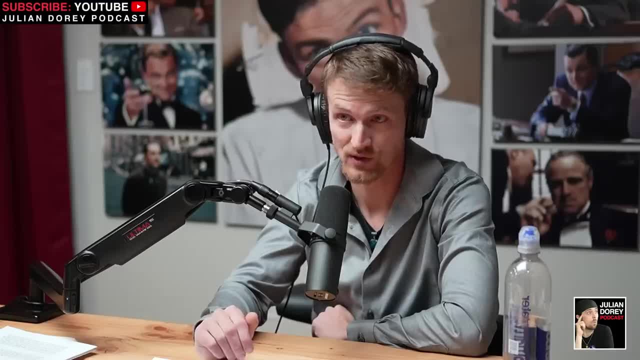 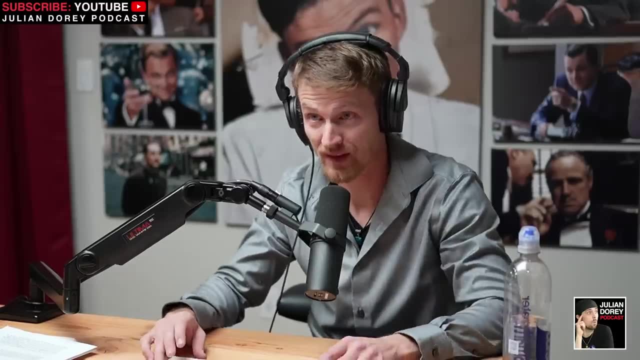 The cycles of consciousness, Yes, Those yuga cycles of us reaching higher states and then going back down to lower states. they seem to be based on things that have nothing to do with us at all And we seem to be just along for the ride. 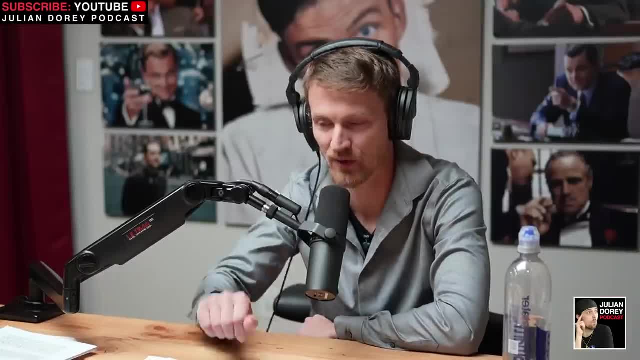 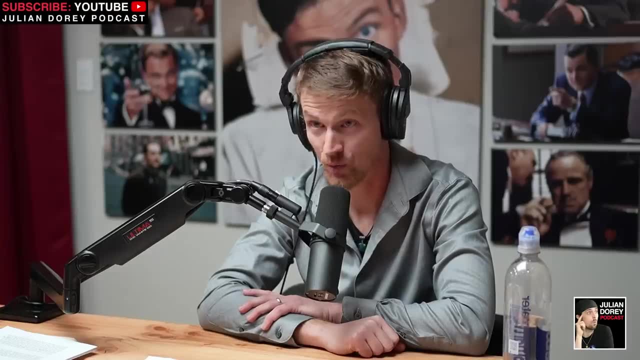 That's what it seems more like. okay, Now go back to the temple again. So it's a sun temple, just like Tiwanaku is a sun temple, with focusing and mapping the sun- Same two things exactly. That's the famous sun gate, you've seen. 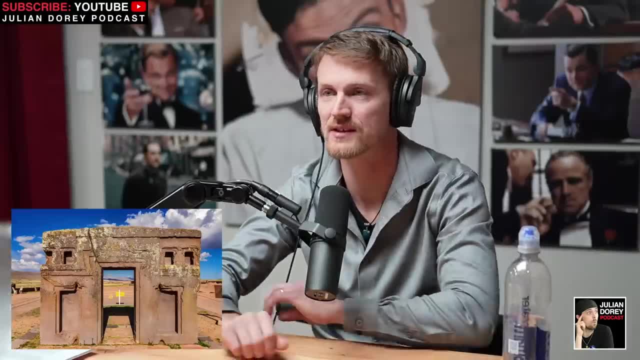 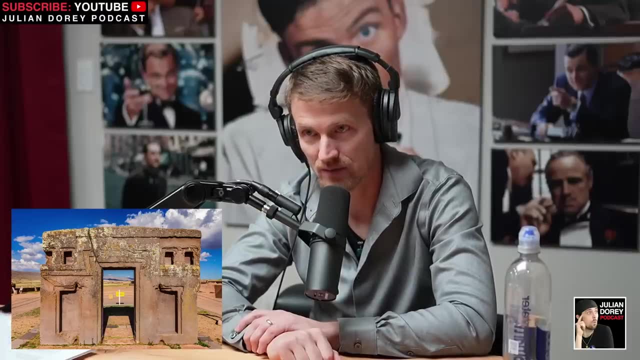 I don't have the sun gate picture on here, but everyone's seen the famous Gate of the sun right At Tiwanaku. But also they have the hourglass. What does an hourglass mean to you? Time Right. 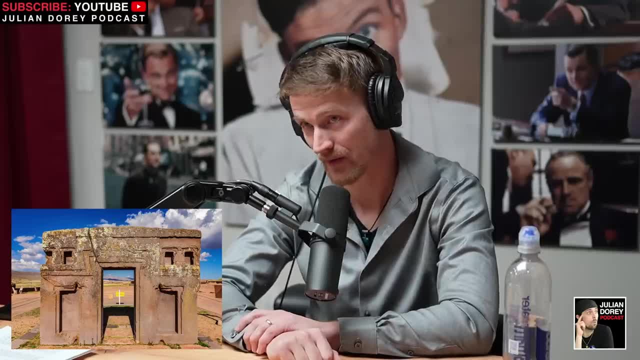 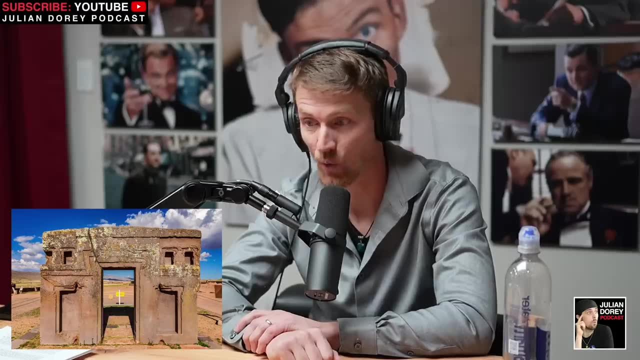 So if you had an hourglass and you had a symbol of the sun above it and you use the sun to measure time, you're referring to being a keeper or like a protector of time, Because look at what's next to the hourglass. 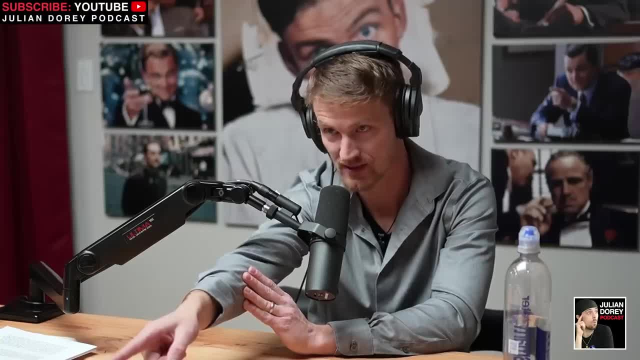 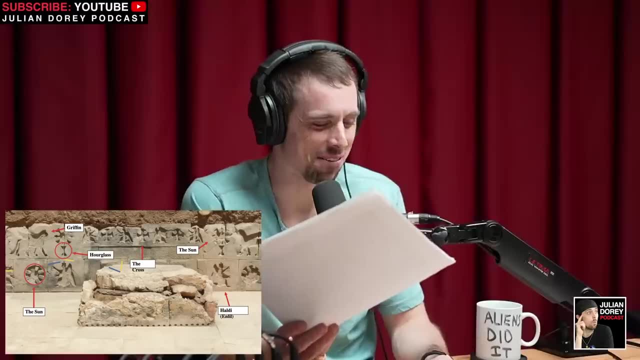 Why do you say a protector? Because what's the symbol that's next to the hourglass? Hourglass. look, What is that On the right? Gryffindor Gryffin, Don't use Harry Potter. I don't fucking want to do that. 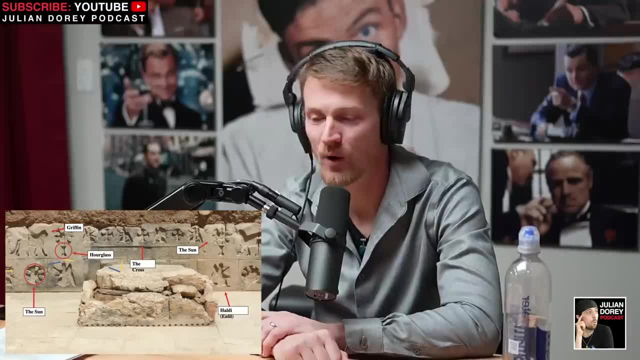 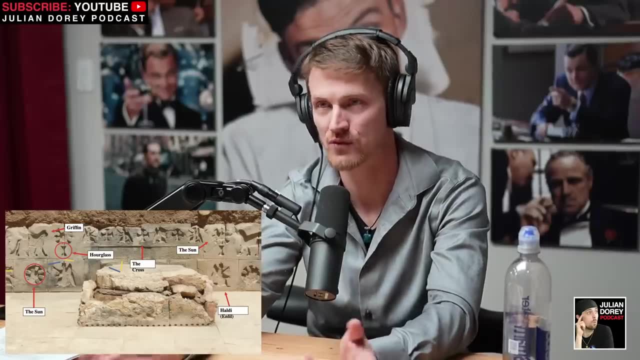 See, I'm just trying to keep you honest. So that is a Gryffin. What is a Gryffin? A Gryffin is simply a lion and eagle together. These are Gryffins. It's a symbol for strength. 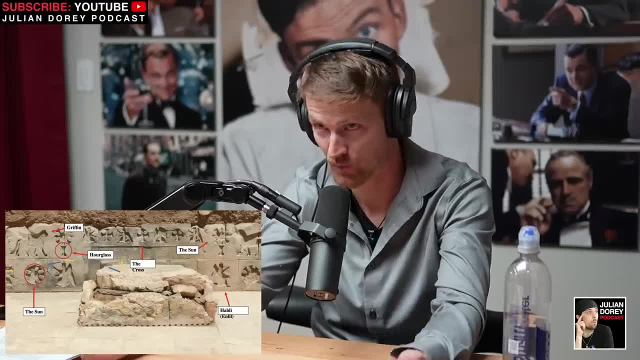 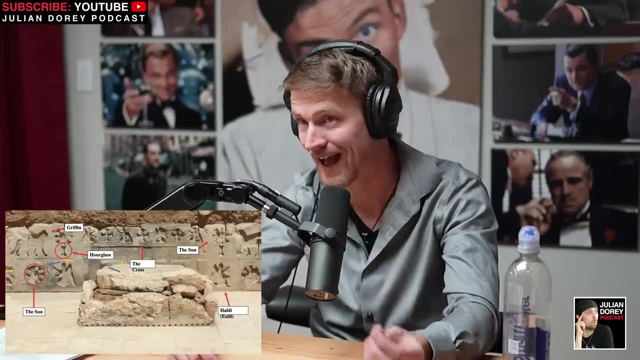 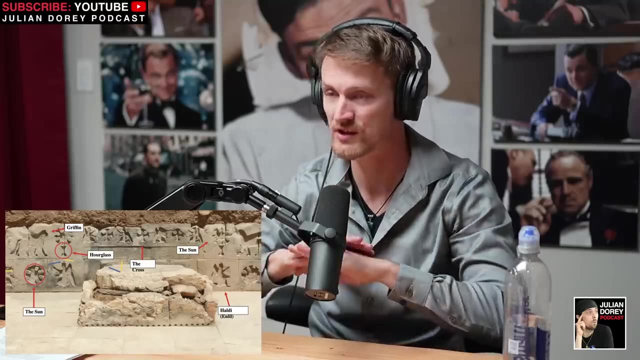 In the ancient world, they believed that you invoked a powerful strength, that you could use it as like a protector, Which is why the great Ed Giza, the great Sphinx, used to be a lion, Not a pharaoh, because a lion who was facing the constellation of Leo and a lion, to the ancient Egyptians, was the most powerful symbol for strength to protect something that they had. 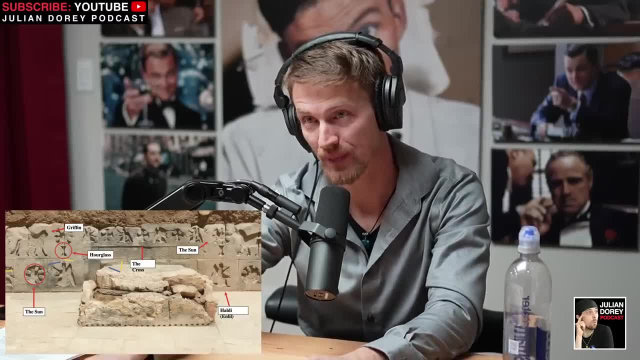 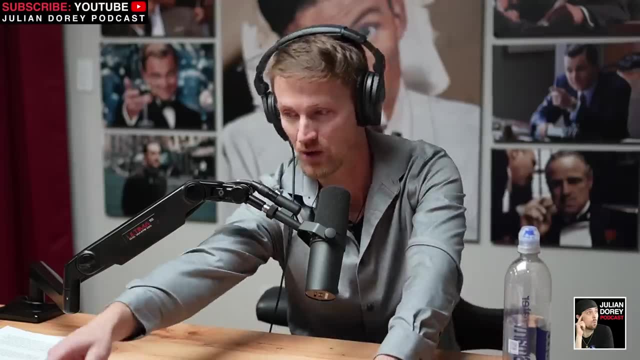 So the lion there? and look, the lion is here too. Bravo, The lion and the eagle, which we see all over the world. they're symbols for strength And that's why. so go back, Go back to your chart. 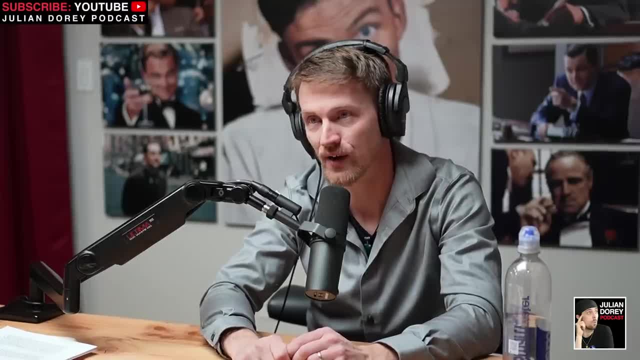 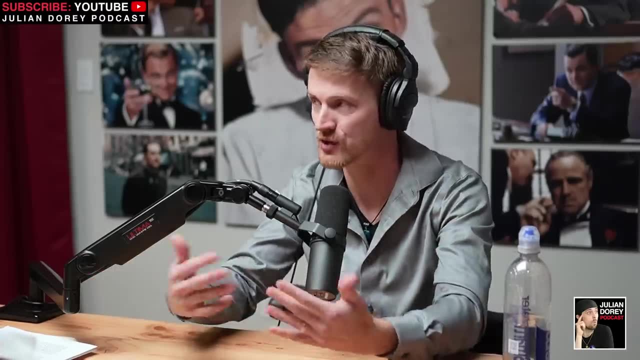 So in this case, the Gryffin is a protector. Does that make sense? Because it's a lion and eagle together. The eagle is like the totality of all above and the lion is like the strength of like down in our realm. 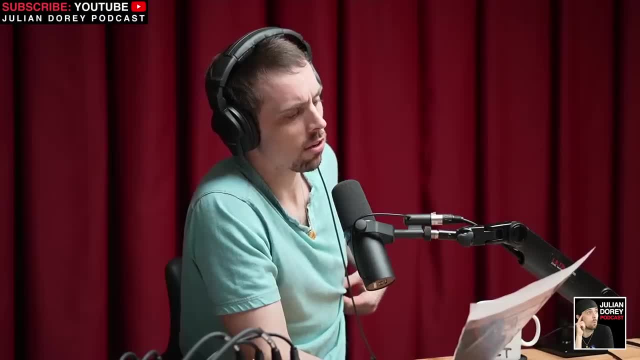 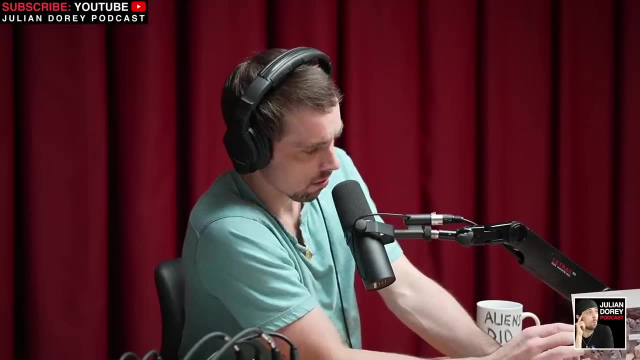 So it's like the strength from above and below. Question on that: Yeah, Because this is so disintegrated. are we making a very highly educated, reasonable guess in saying that's what it is? No, there's that. 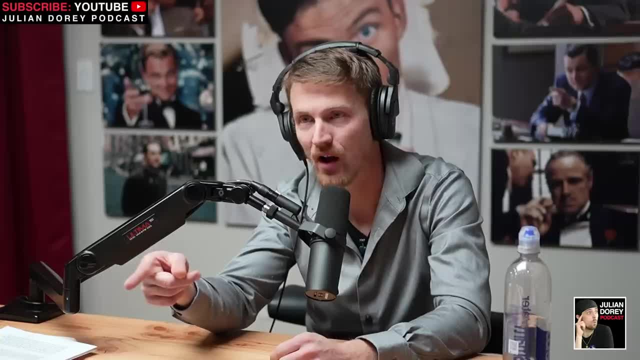 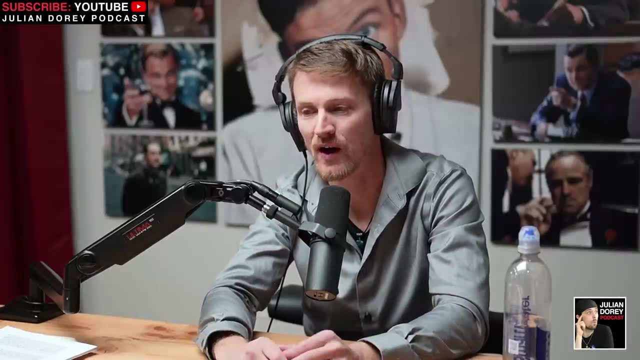 So that temple has that icon like 10,, 15 times. Okay, So turn it over for a second. See It goes. all the symbols go all around the whole site, So there's better images of it that are more preserved. 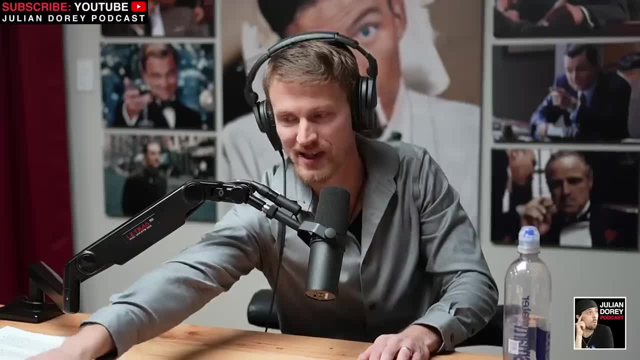 The circle is just. Oh, yeah, Look right there. Yeah, see So the circle. it just happens to be in front of the altar, where the cross is, where the main symbols are. That actually looks like a fucking unicorn. Whoa, It's a Gryffin. Yeah, I know, It just looks like a unicorn. So the Gryffin became one of the main protector symbols of the ancient Greek civilization. Okay, What years are we talking on that ballpark? 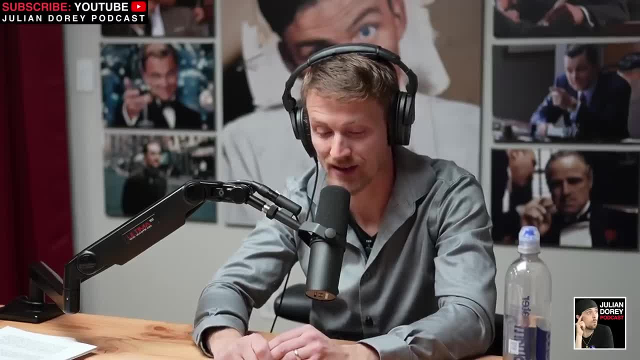 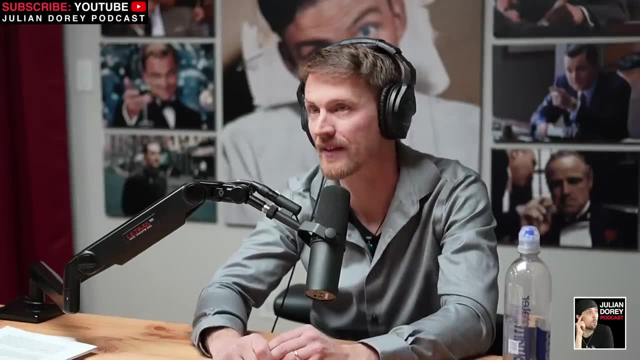 Well, according According to Plato like remember we talked about last time. I love Plato, Plato Diodorus and the Temple Priests of Sais- is that there was another civilization that existed at the same time as Atlantis? Yes, The ancient proto-Athenian civilization, And they're the ones that became the Greeks as we know it. Well, How much longer before did you think that was? Well, it would have been thousands of years after this. And the thing that's fascinating, though, is that Gryffin, that's the main symbol of Ionis and of this civilization, became one of the main symbols of the Greeks. And the bloodline charts of the son that was supposed to. according to biblical charts, that was supposed to be in that region was Japheth, And Japheth is the one that's mentioned in the king's list at Cavistepi, showing that it's true. 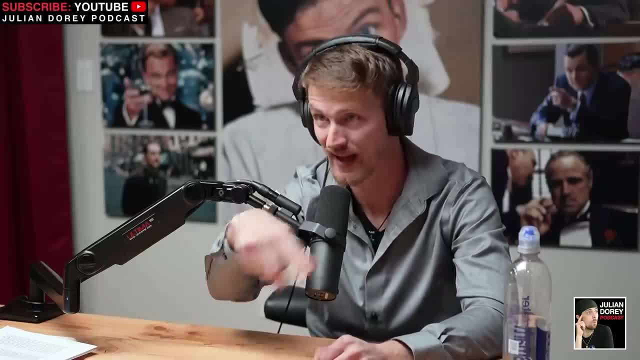 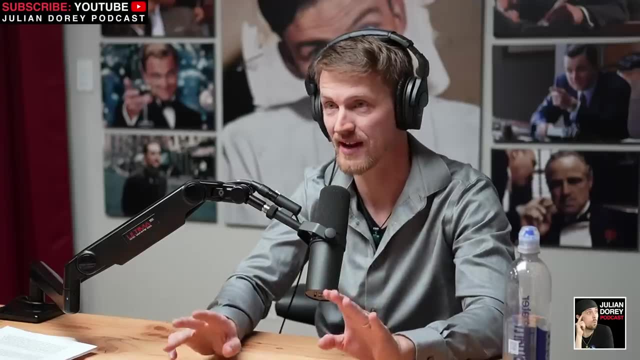 He truly was the descendant that was in charge of that civilization. And who was he descended from? again, Noah. But what I'm trying to say- But he was one of the sons, Right? But here's what I'm trying to say- is: 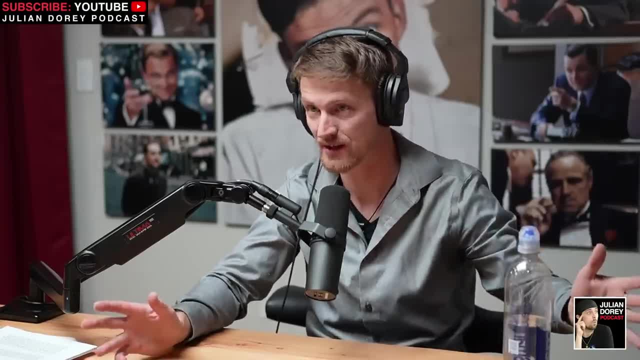 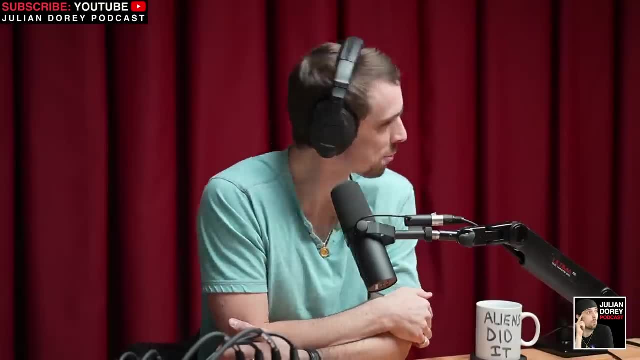 He's assigned And, according to these regions, there are three sons. There is Japheth Thoth- No, that's part of Egypt After that, God damn it. So you have Japheth Ham and Shem. 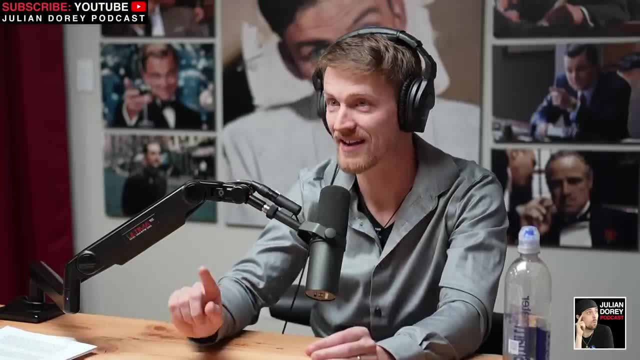 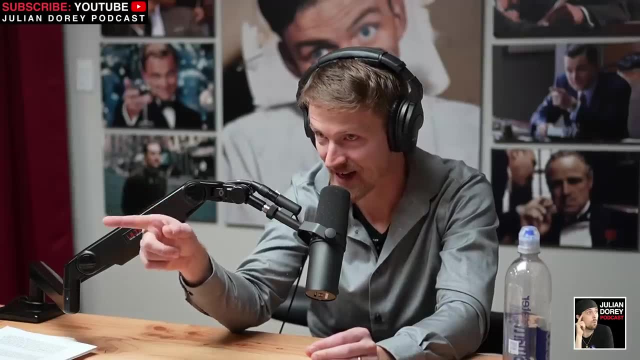 Okay Now do you remember what the name of that Ashurbanipal-like figure I said at the first cross? His name was Shemsi, Shemsi From ancient Sumerian. he had the cross on him, likely a descendant of Shem. 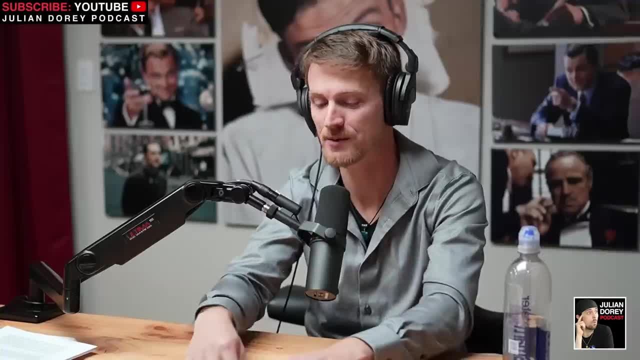 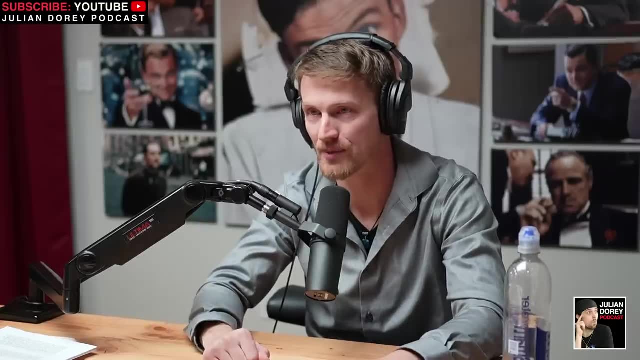 Right, Because that's the thing is. you look at these Biblical, Like his Italian cousin. You look at these Biblical charts. they describe these brothers as going to different parts of the world. Now what we're doing is we're using archeological evidence to prove that that actually happened. 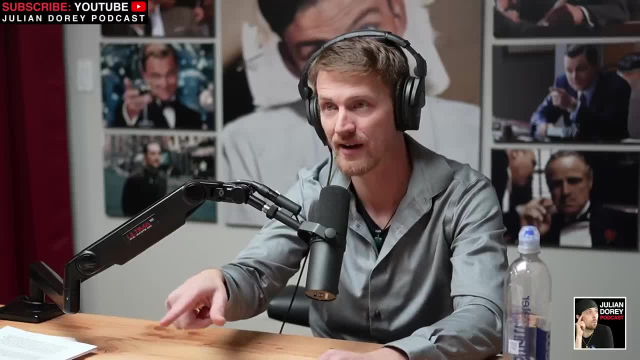 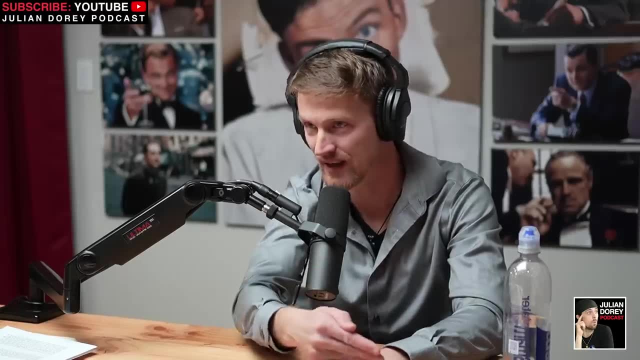 And what I'm trying to build up to say is that griffon that's there at Ionis, if it's Japheth that's in charge of that region, and then he goes west and creates the Athenians. that's why you see the ancient griffon as the protector in the ancient Athenians. 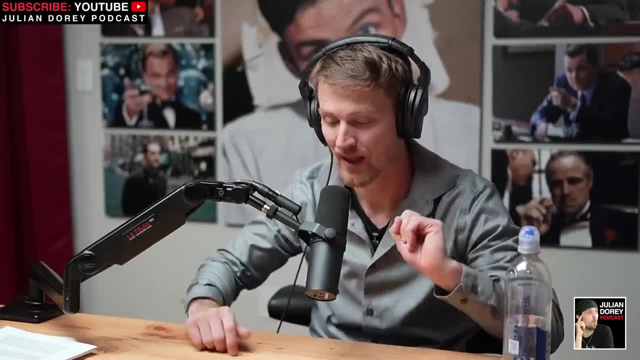 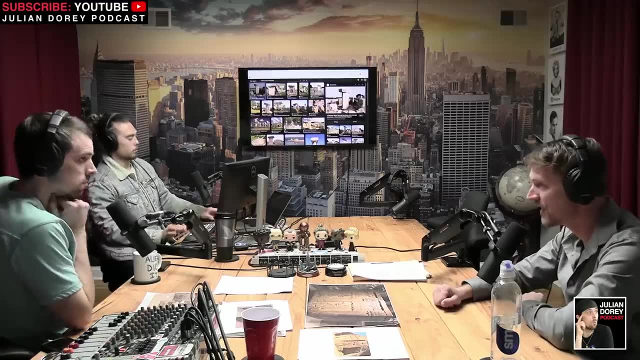 And the same gigantic people don't know about this. I'll say it. Outside of Athens is one of the most incredible megalithic walls in the world, called the Pink's Wall. okay, And that wall- and I have an image of it I can probably get to you- 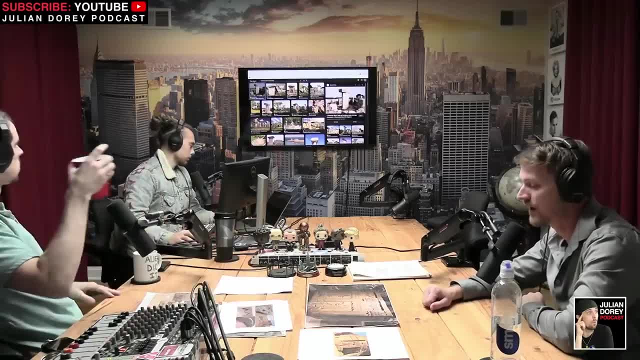 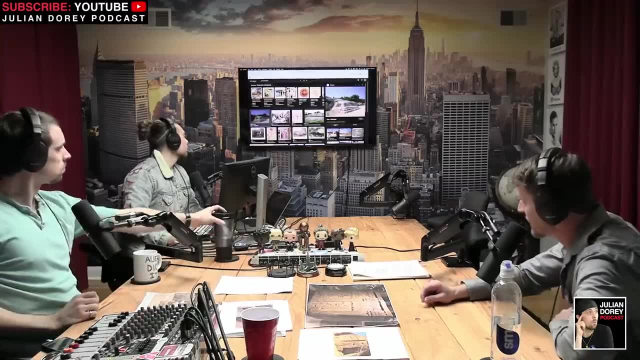 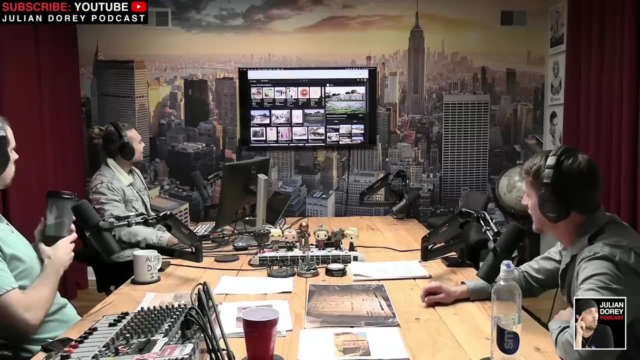 You can pull it up too. That wall is the only thing, one of the only things left of anywhere that exists from the ancient Athenian civilization. okay, Not that section of it, though. Can you keep what you had up there and type in: Richard? 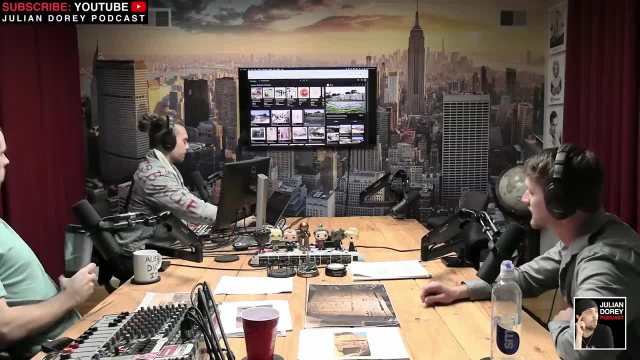 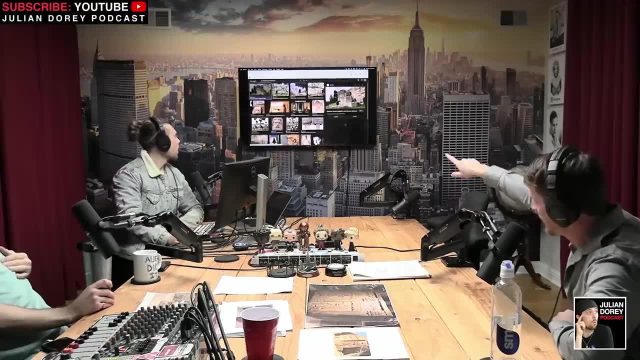 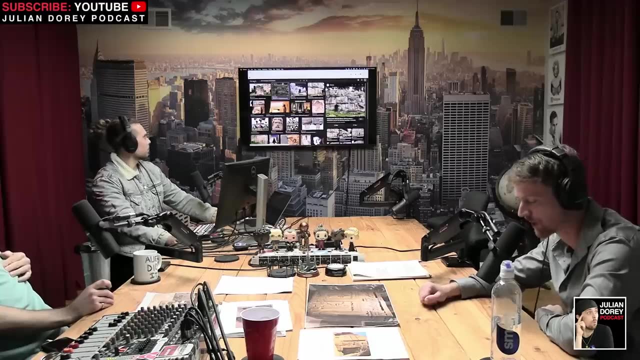 Okay, Richard Cassaro, Richard Cassaro. Yes, Yeah, you'll find it just like it sounds. Thank you. Second picture. second one: There you go right there, Pull that up really quick. I love that that man is great. 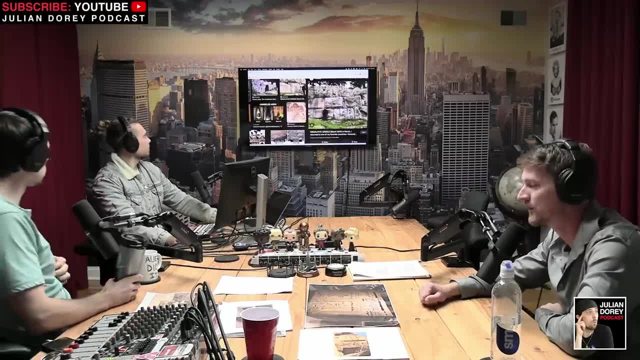 Thank you, Richard. You do great work. He is the one who pioneered the fleur-de-lis symbol with the triptych doorways around the world, and I do want to give him credit for that. So thank you, Richard. 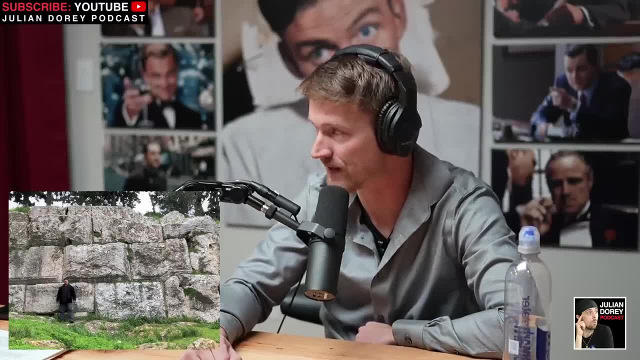 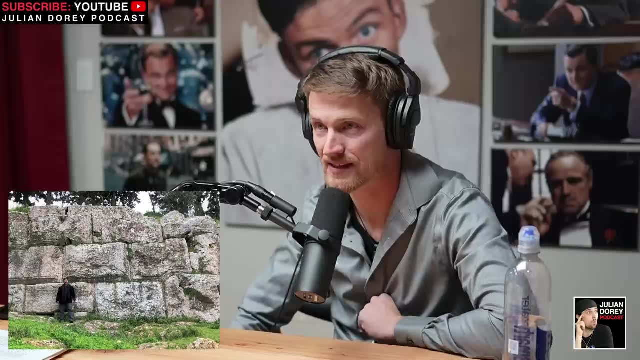 Because I've definitely built off a lot of his work with these civilizations. Thank you, Richard. Thank you, And I've done a lot of work with these civilizations and these discoveries. Now look at these blocks. Not only do you get the polygonal type of building like we see in South America, but remember this idea of this stepped level. 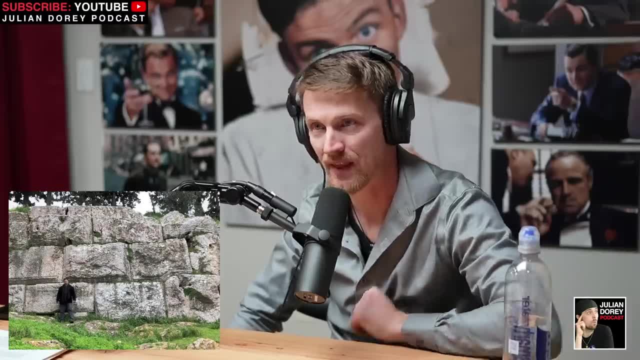 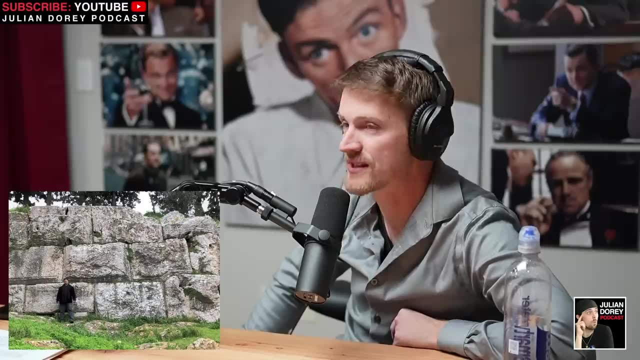 Yeah, It's part of, like a teaching aspect, these steps and levels that we can take. If you look at those stones carefully, like to the left of Richard's head, you'll see that there are steps and levels carved into those gigantic blocks. 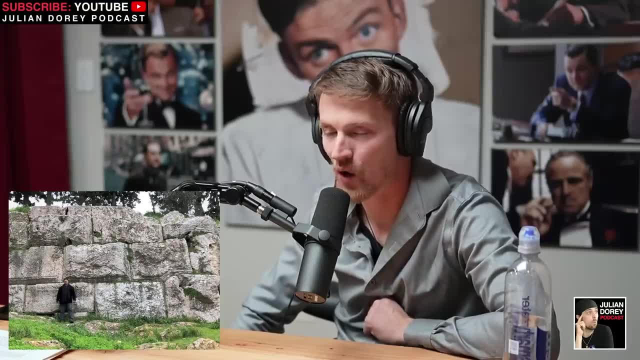 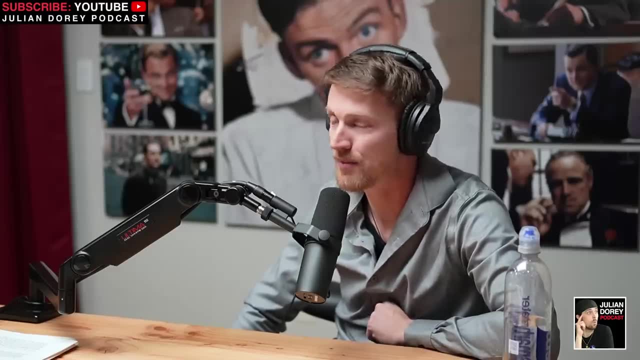 Now for some context. some of those blocks are over 10,000 feet long. Some of those blocks are over 20 tons. That's a lot. Nobody talks about the ancient proto-Athenian civilization, but I believe they came out of the Ararat civilization and became the Greeks as we know it. 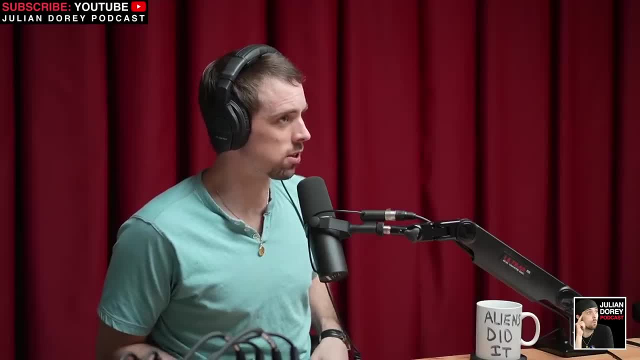 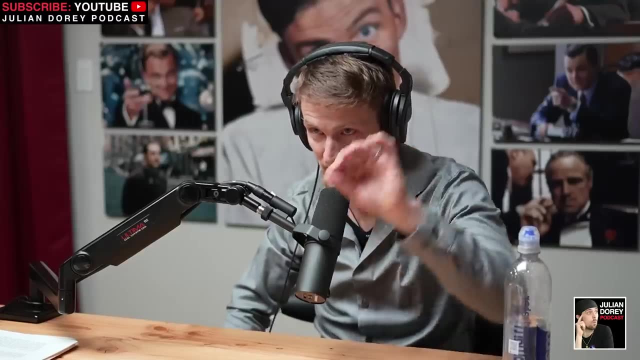 And that's why the Greeks, I think, were… You believe they came out of the Ararat. What's the archaeological research to back that? All of these megalithic sites that mimic this site with the same symbols that came from it, and also that the Greeks were the most sophisticated democracy in the world, hands down. 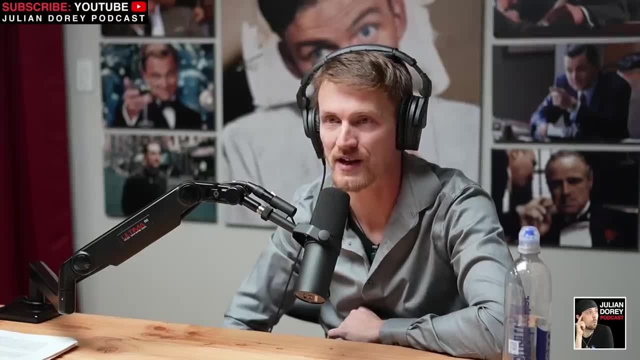 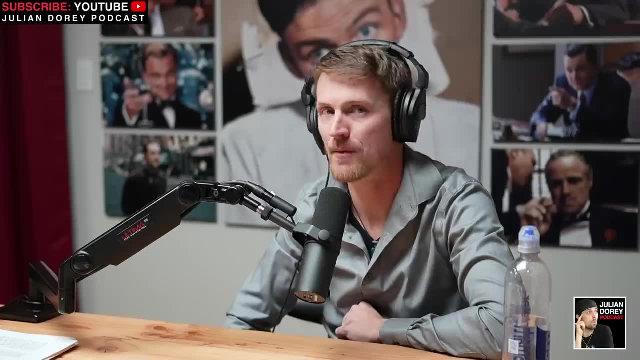 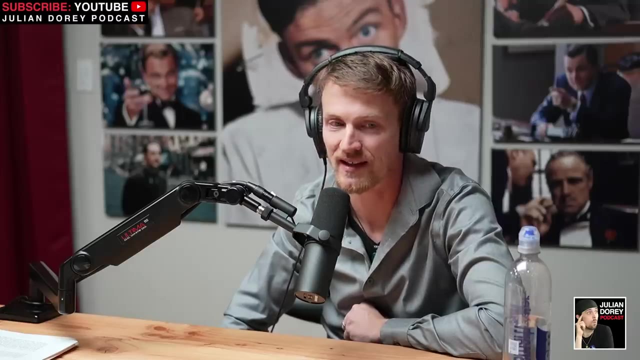 Hands down way that they laid down the foundations for where we are now is is is just like it's uncanny. it's like they seem to have the model for like the perfect civilization, and Plato even talked about that. he actually refers to them as the perfect civilization, versus the Atlanteans who became an. 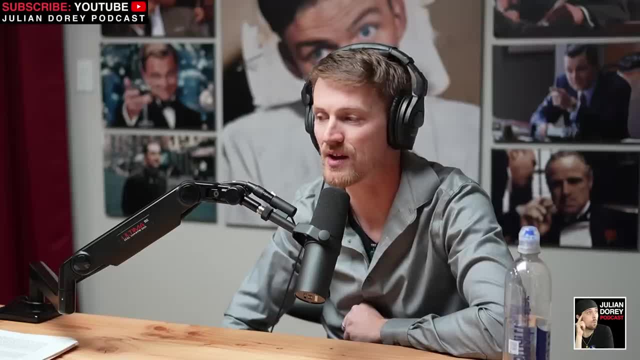 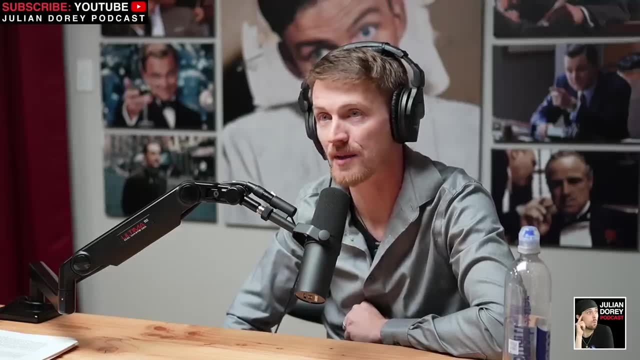 empire, and he talked about how the, the Greeks, were the most. this like perfected society. that's what he called that. he talked about them as being perfected society, with like a perfect democracy, until they were wiped out by a tsunami in the Mediterranean that literally made them disappear. around what time? during the Younger Dryas. okay, now you have to keep in mind: the reason why I don't think Ionis in the era civilization was destroyed during Younger Dryas is because they have the lineage of an older time period in the same technological sophistication as all the other lost civilizations around the world, but we don't see any of those iterations around the world. but we don't see any of those iterations around the world. but we don't see of those lost civilizations after the Younger Dryas, meaning that after 13,000 years ago. 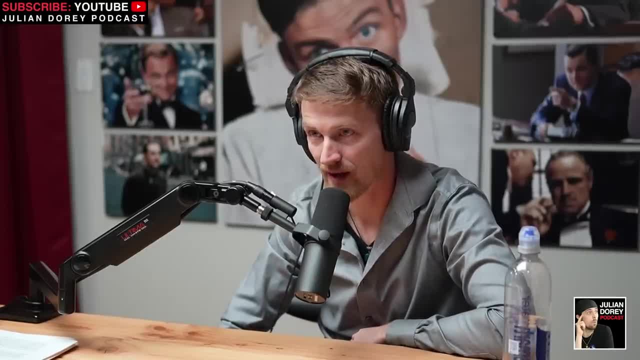 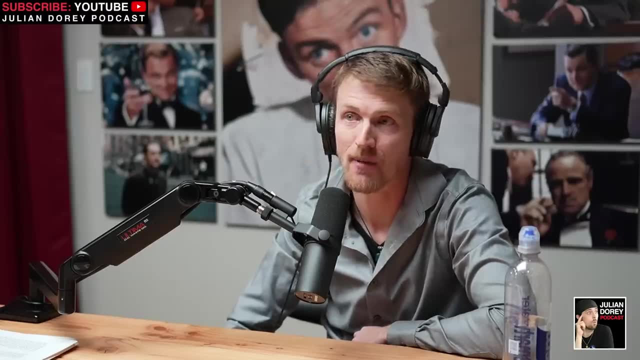 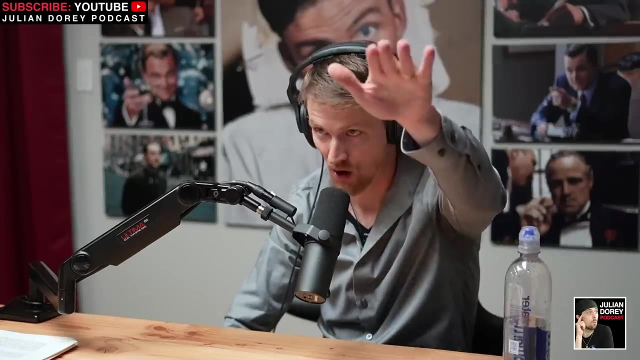 these cultures, the majority of them were destroyed and the majority of the knowledge was lost and they were never able to build what they could ever again. and we know that because of sites like Machu Picchu- and Machu Picchu, next to the Torreon, is a wall there, okay, and in that wall gives shows. 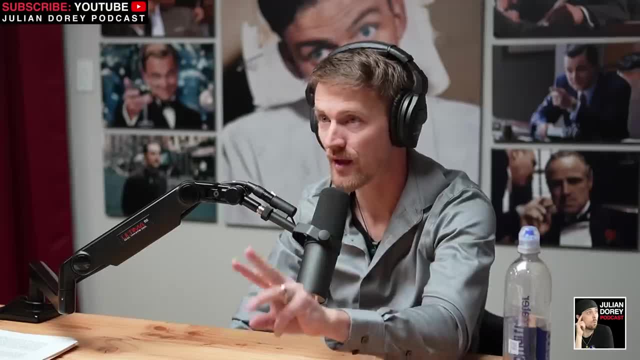 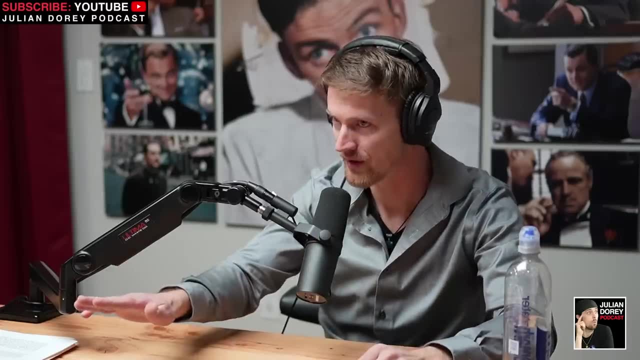 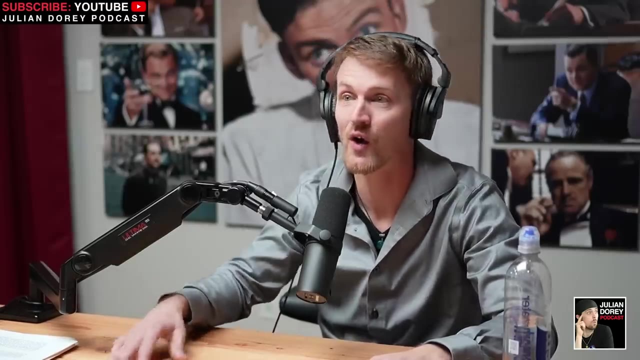 three different levels of construction, not two but three, showing you: imagine you had a, you had a proto-civilization that built it all in perfection. imagine they get wiped out. then there's like survivors of it, just some right, and they maybe grew up, grew up with some of the indigenous and they try to rebuild. because at Machu Picchu we 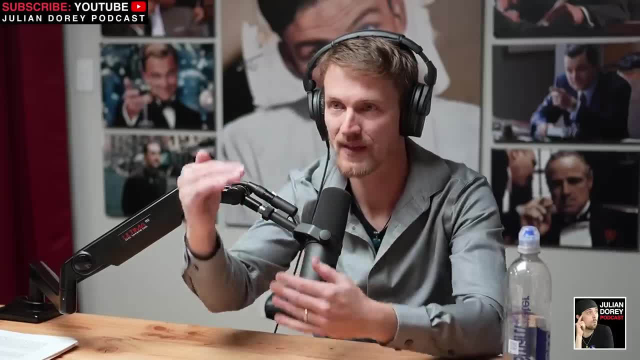 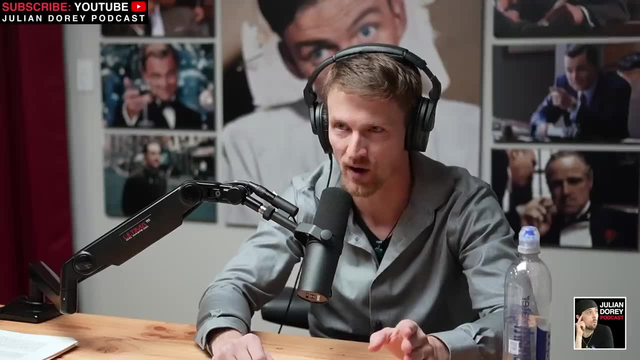 see this second level, that's second level, building on top of it. that's not as, not as advanced and as big, but it's still pretty good. but then on top of that is like really primitive work- brick and mortar and really really simple work from the Inca. so in Machu Picchu, in an urban setting, you have a massive building that's built off the top of it. so it's really huge. that's not as advanced and as big, but it's still pretty good. but then on top of that is like really primitive work- brick and mortar and really really simple work from the Inca. so it's a very modest. все "すぎたい。 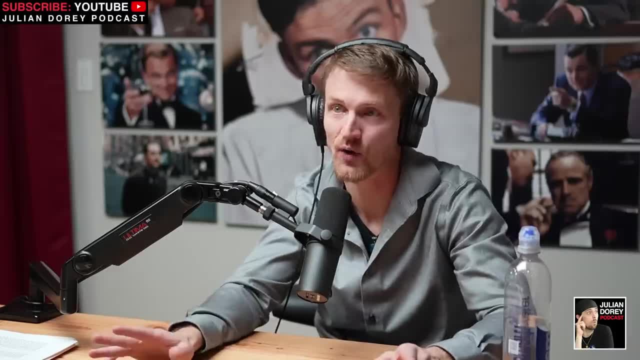 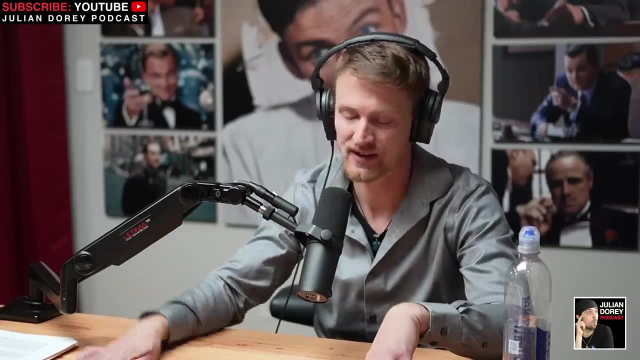 so it's like: imagine this is. this is how i think it played out on earth. i was to a guess based on everything i've studied. imagine a civilization emerges- the sumerians. they get destroyed in a great catastrophe like more than 50 000 years ago. so we can put a time frame on all. 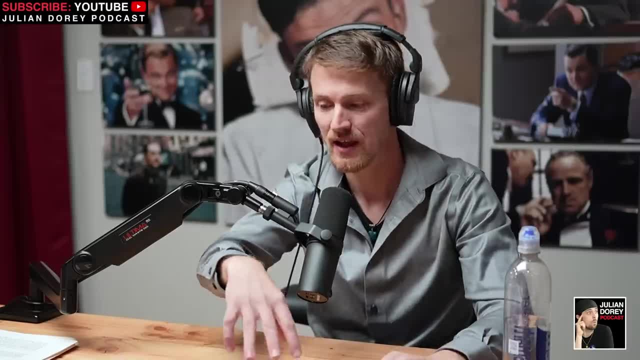 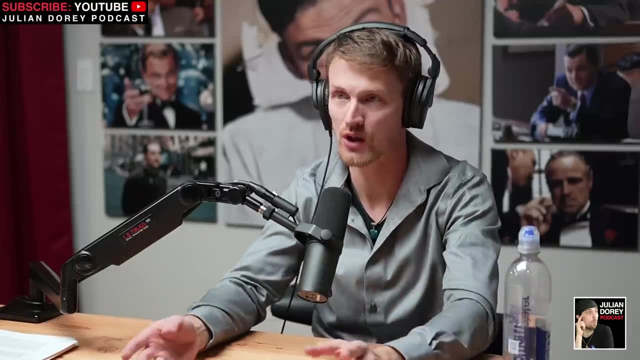 this and i say more then. imagine. the stories are that this era civilization literally comes out of the survivors of that and but something new is lowered and they literally get all this knowledge and all these ancient techniques and then they go around the world and they create all these. 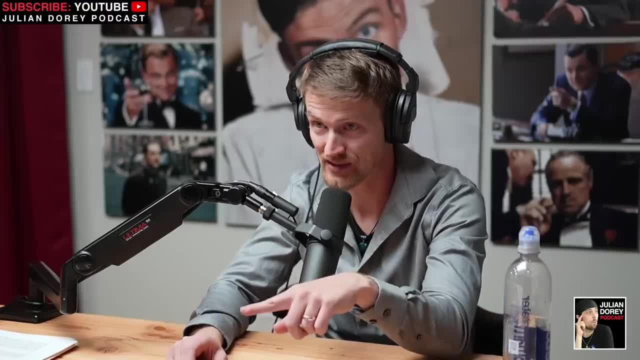 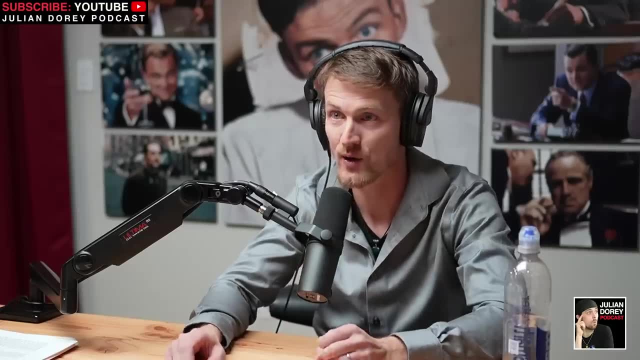 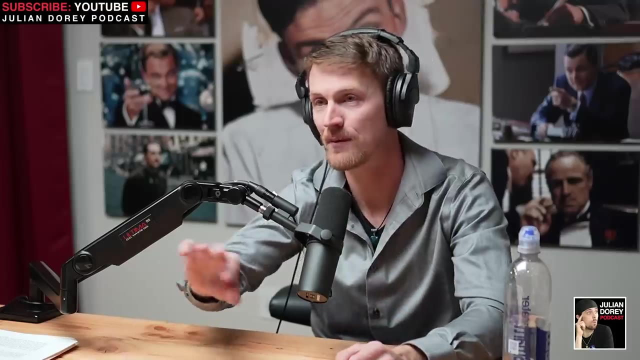 civilizations right now. imagine the younger dryas from 13 000 years ago. is what then destroyed them? so it's like you have these iterations right: you have the first one, that's gone, it gets destroyed, then another one comes. it gets even more advanced because something was handed down. but then when 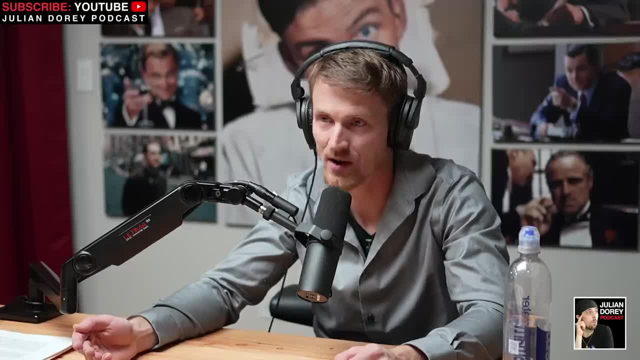 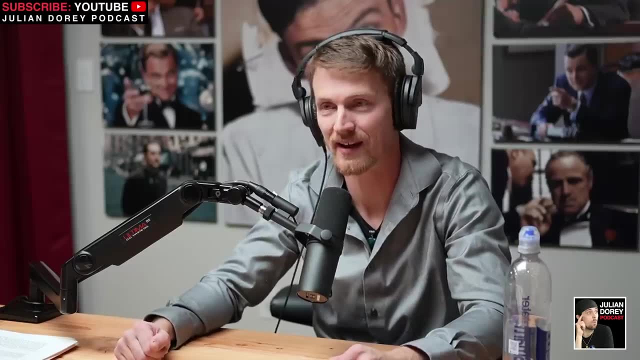 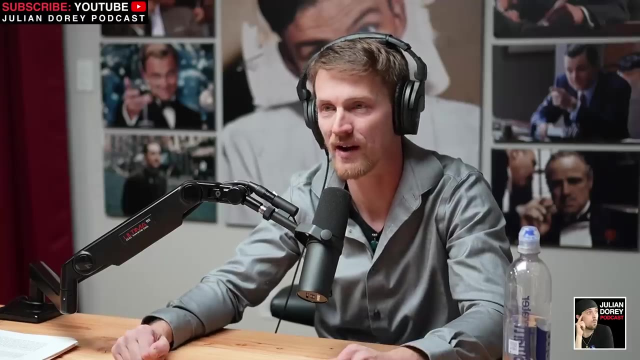 that one gets destroyed. all of those things are not re-lowered again like um, it wasn't supposed to be. it's like: okay, well, you guys find your way. now we're not doing that again, you know. it's like almost like kids finding a bunch of toys in someone's tool in like their garage and they have no idea how. 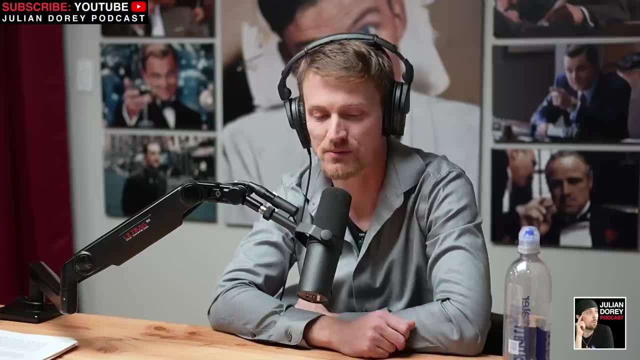 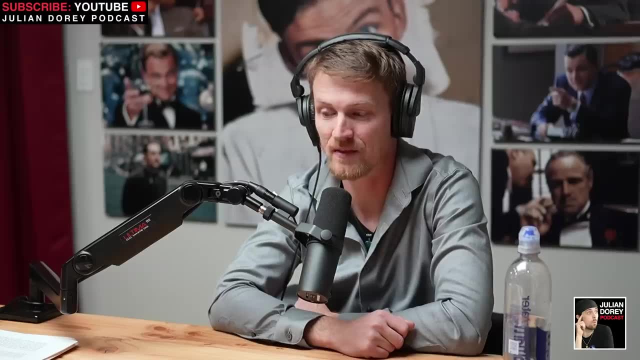 to use them or what they're for. it feels if it looks more like: uh, there was an interest in our story and helping it and giving us all these advancements. and then there was like: now we're just going to be hands off and let you guys do do your thing on your own, see if you can figure it. 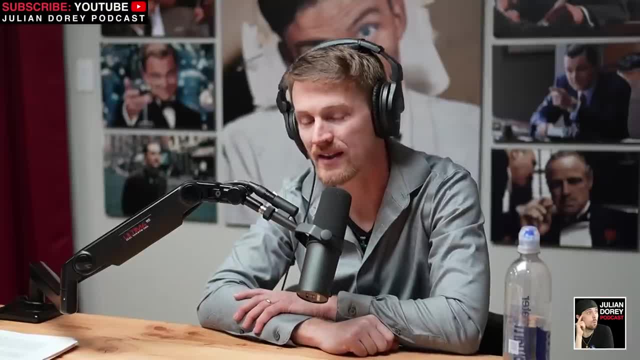 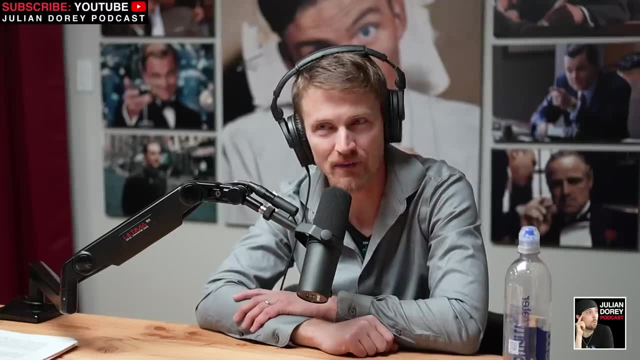 out. that's what it seems more like, and that's where we are right. now is here. we are thousands later. we're becoming technologically advanced. we got more time on our hands. we're starting to like wonder about ancient stuff again. right, things are starting to push the narrative towards that. 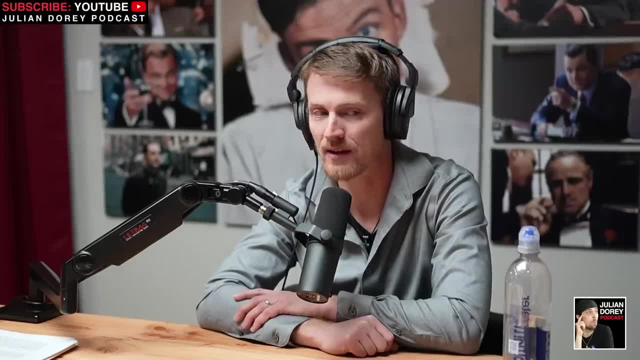 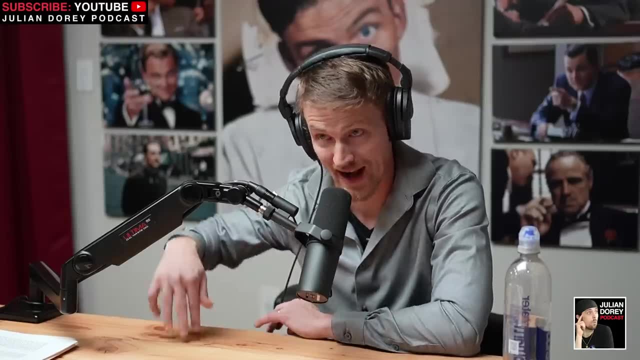 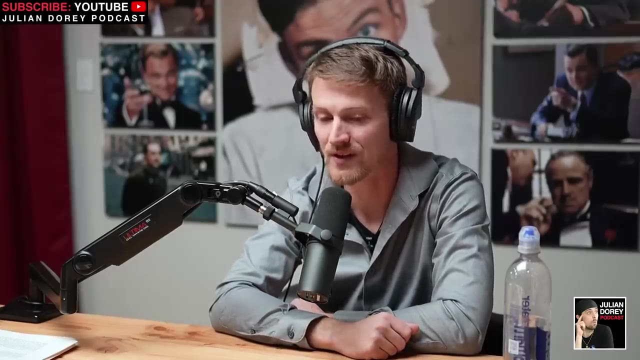 and here we are, we're we're finally looking back and be like: wait, what if that's true? what if they really did exist? and i think that's where we're at right now is we're at that pivotal point where we are going to have a collective shift in our consciousness, where there's going to be so much. 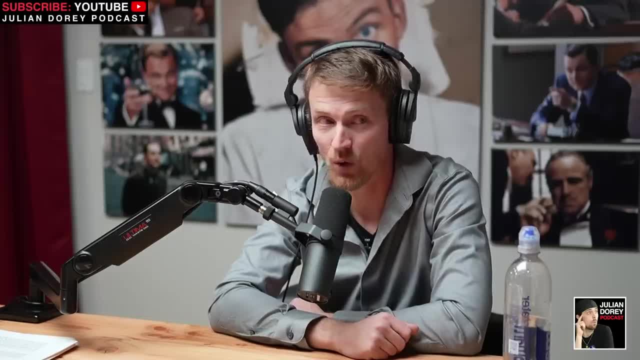 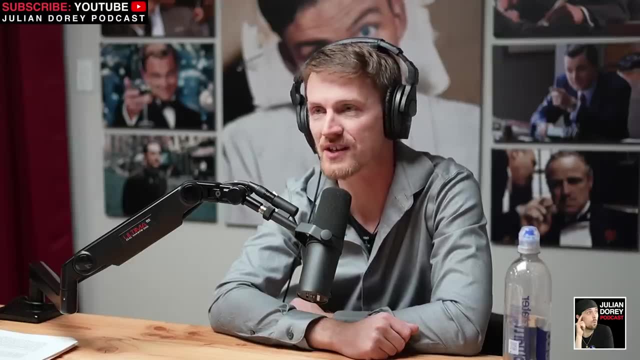 evidence that comes from different avenues, that eventually we're going to have a collective shift, that eventually the old narrative will crumble and i think it's going to come along with the same time period of probably rewriting um education systems and a lot of things. why are you calling? 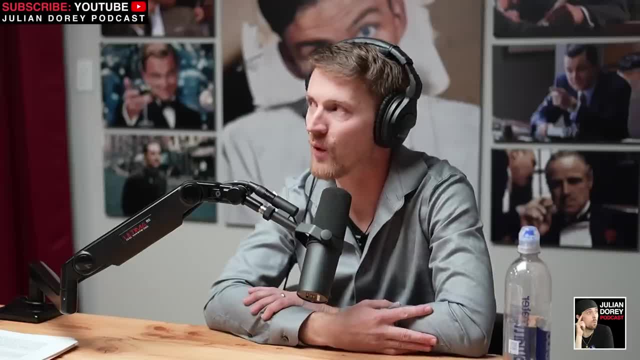 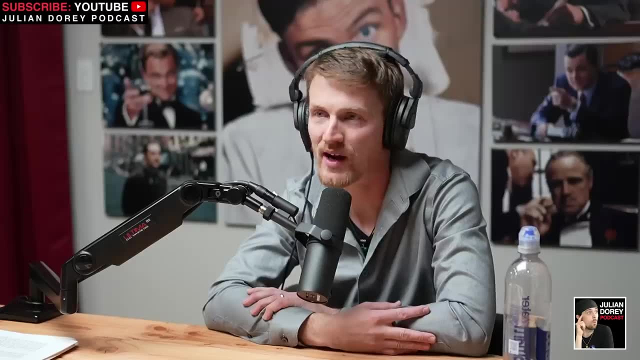 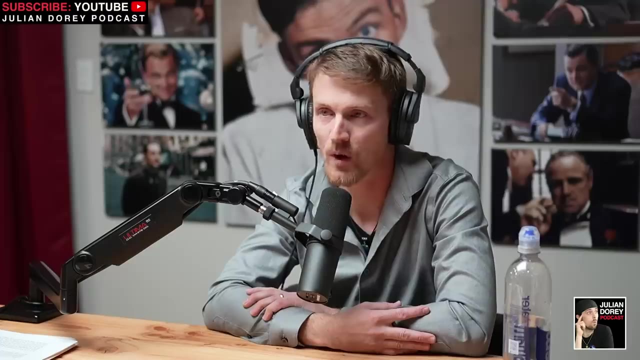 it a shift in our consciousness? well, because i feel like the way that we've been portrayed and taught is almost like being kept in a prison. if you're taught that the brain creates consciousness, then you live in. you live in existence where the life you have right now is a fearful one, because 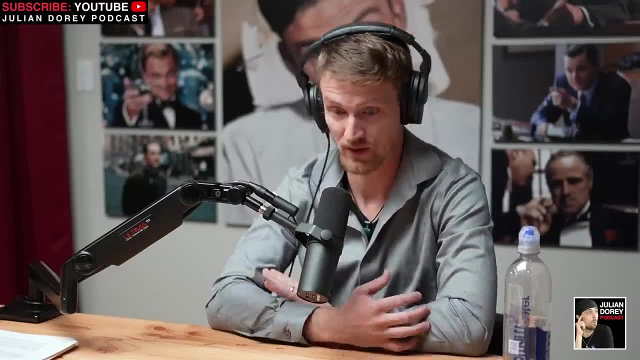 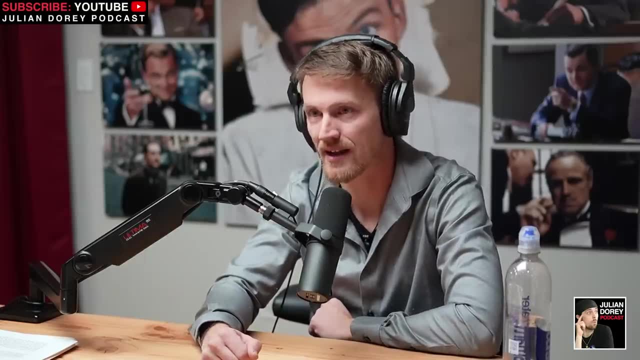 like you, so you feel thankful for what you have and you feel like, oh god, i'm glad i can eat, right, i'm glad i can blow that. but that whole mindset is based on this survival, the fittest mindset that treats us like another animal on earth, just like anything else. right, except that we're not. 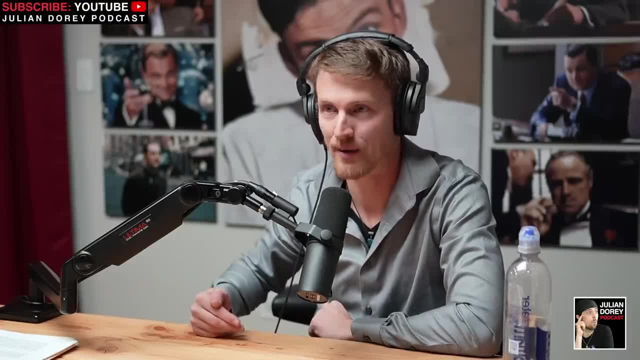 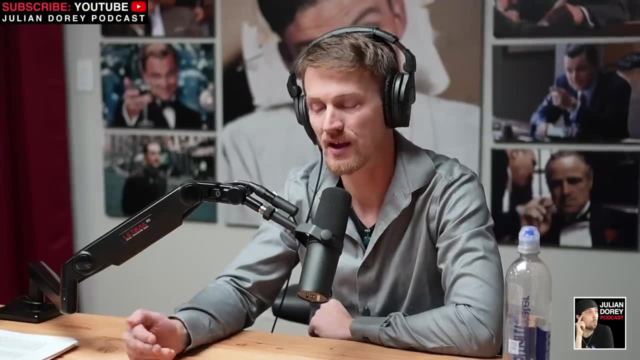 strong. we're not super agile. we can pretty much be outrun by most animals on earth- but we're really smart and i think that, and we have this divine spiritual nature to us, i think that we need to separate ourselves from the world and we need to separate ourselves from the world and we need to. 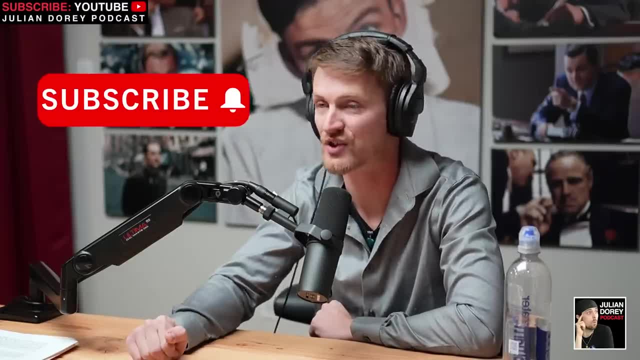 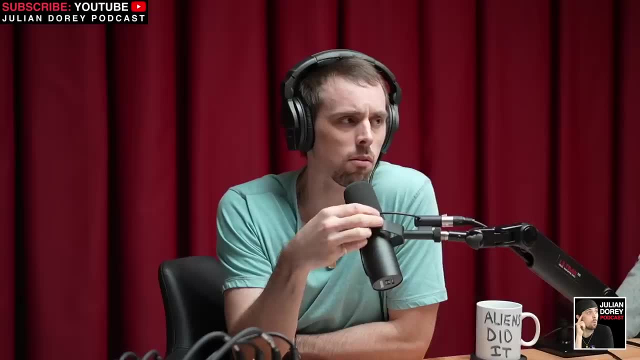 from the animal kingdom. we need to stop thinking about ourselves as just an animal. we need to think of ourselves. we need to start redefining what it's, what it is to be human. we need to start looking at all of the echoes of what the ancient civilizations were trying to tell us, but that's. 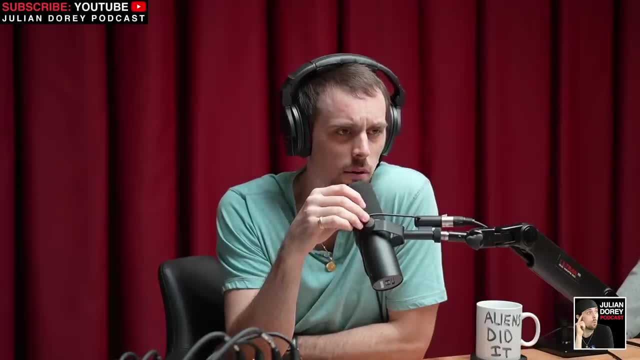 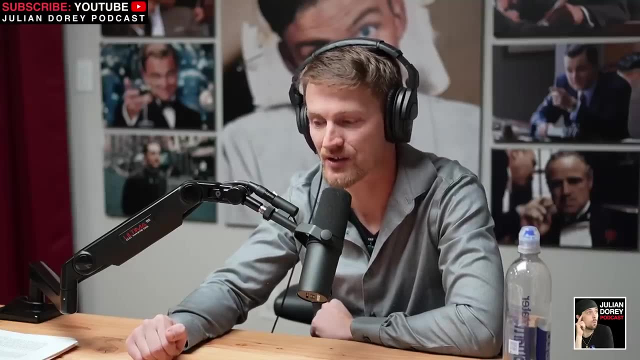 who we are. go against biologics, though, because we are an animal. well, we're an animal, but again it comes back to: how do you measure consciousness? what is consciousness? is consciousness what defines us, and we're just in this body to experience something physical. i'm telling you. 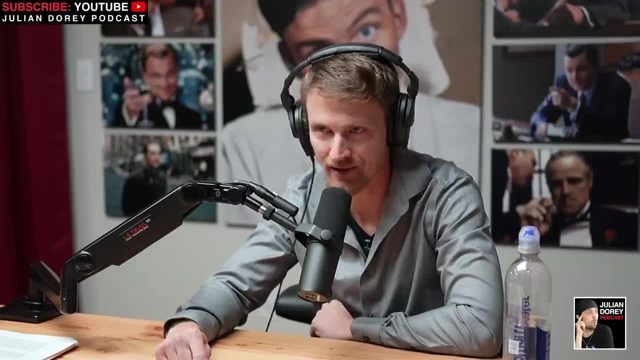 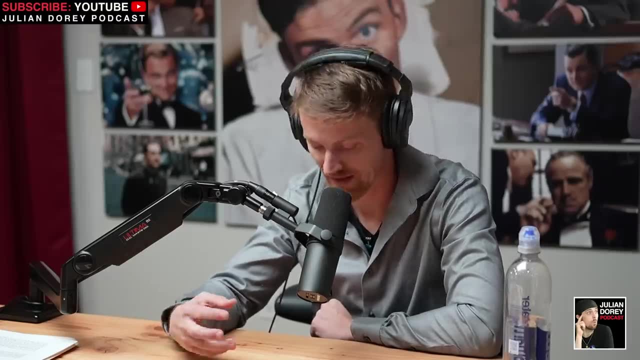 when you redefine something like that, you change the entire human experience. it's almost like if you had an animal in a zoo. okay, let's say you like an animal there's never been anywhere else his whole life. he's like it's just in a cage and it's with other other lions in a zoo and it's like 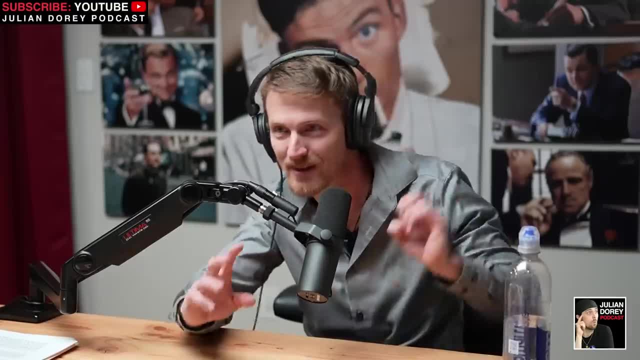 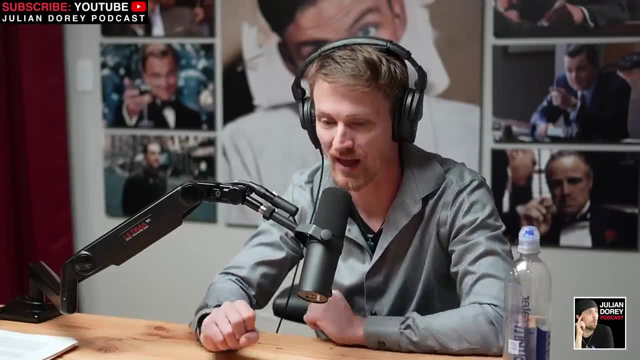 oh, this is my existence, right. i'm like walking around in here and there's people looking at me taking pictures, but then you take that animal and, as stressful as it is, and you bring it to africa, right, that lion, and you let it out and all of a sudden it's like 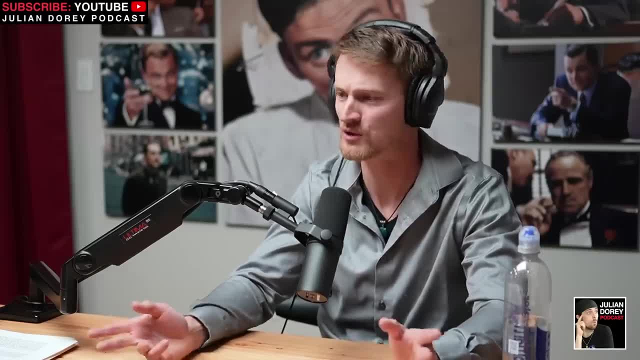 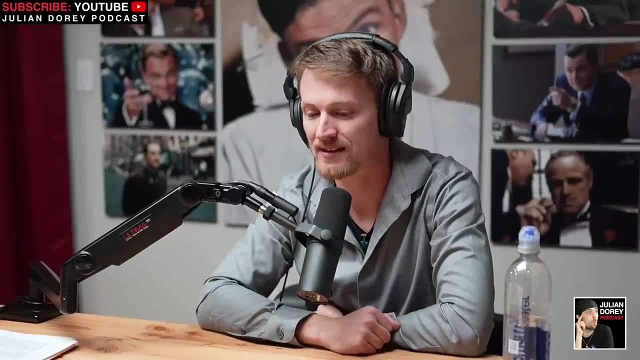 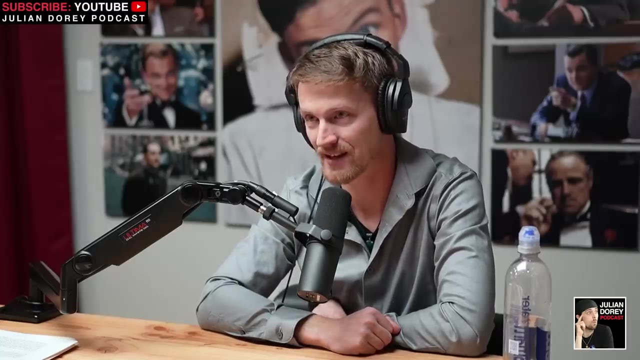 whoa, where am i? this isn't what i. what am i supposed to do? there's no food being brought to me. i'm not eating out of a bowl anymore. yep, what i'm trying to say is: i think that we've been conditioned into a controlling type of mindset on what we are and who we are, to keep us complacent. 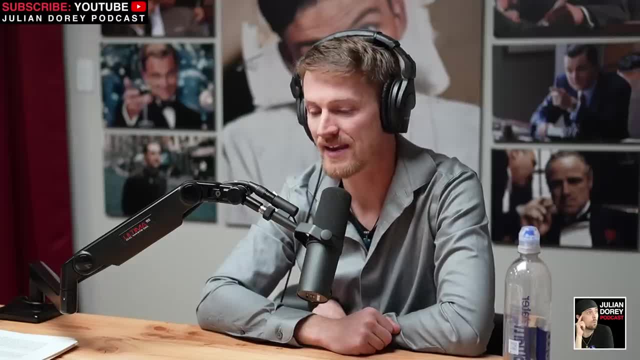 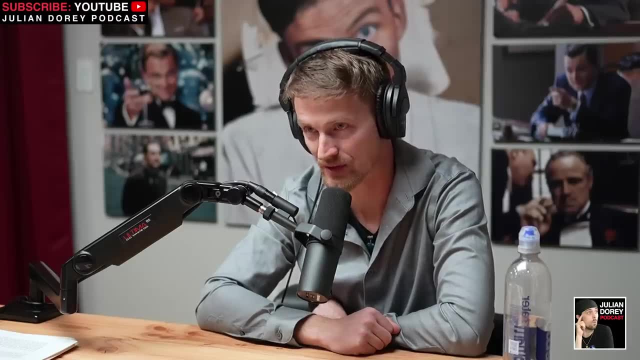 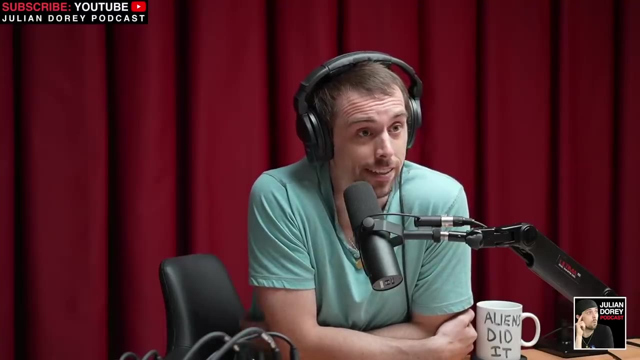 and keep us focused entirely on giving away the creative potential and the divinity of who we truly are to someone else. okay, let me ask this question, and i think you make a lot of fair points about some of the, let's say, organization of society. that happens no matter what, even when. 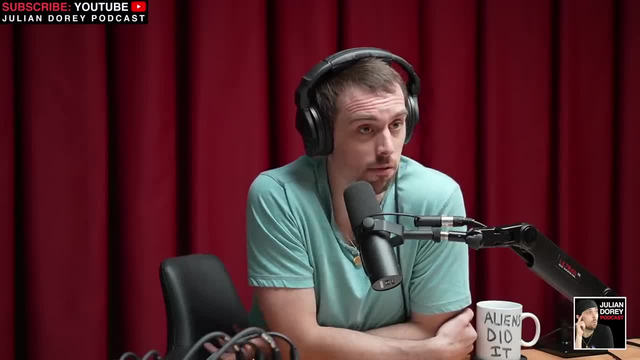 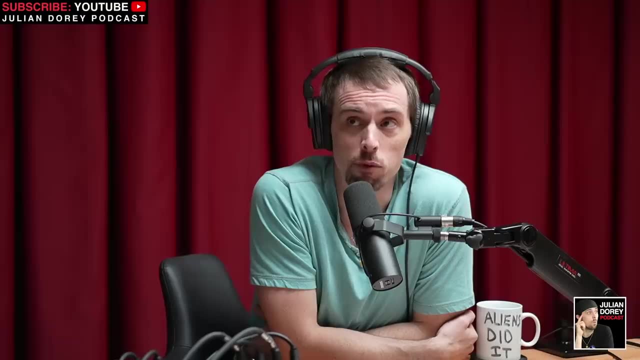 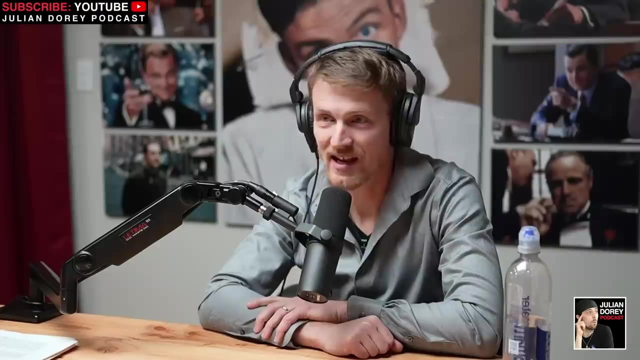 there's better logic sometimes. i i don't disagree. let's play devil's advocate, though. do you think some of your thoughts on this could be biased by your experience? because, like some of the thoughts i have on it, i could admit, are probably biased on mine. i'll say yes, but not in the way you think i'm going to say yes. okay, i'll say yes because i have. 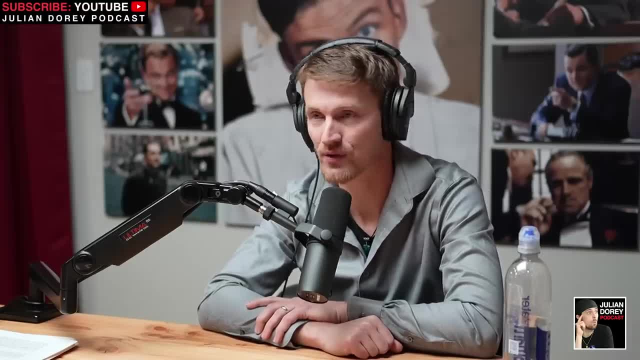 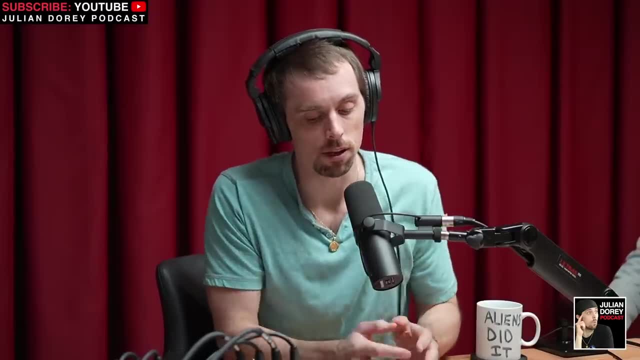 lived and breathed what the ancient teachings that they've been trying to tell us are, and experienced firsthand what they said and what we are. that's not what i mean. let me go back. i wasn't clear enough. i'm saying before you did any of this, yes, before you even got curious about this stuff. 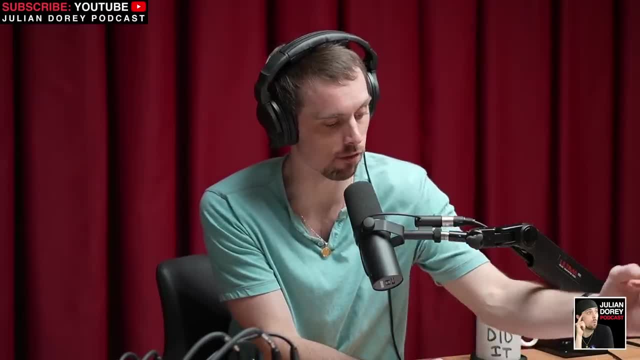 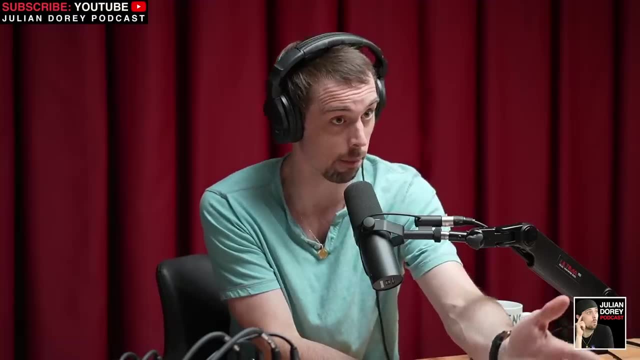 you. there was an impetus, right, and the impetus was: you were pissed off, and you were pissed off at what. you were pissed off at how things were taught or how things were organized, because you believed it to be wrong, which you're right. be right about a lot of that. by the way, i'm not saying i disagree. it's fair, yeah, but then do. 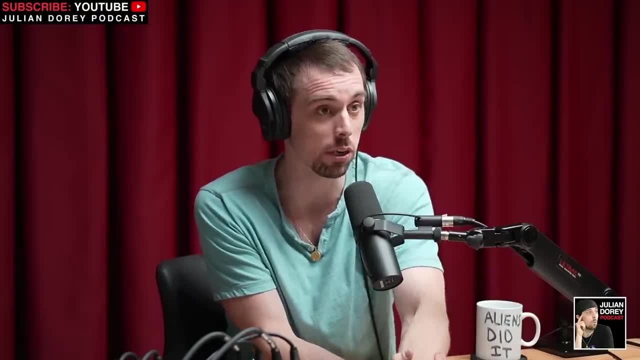 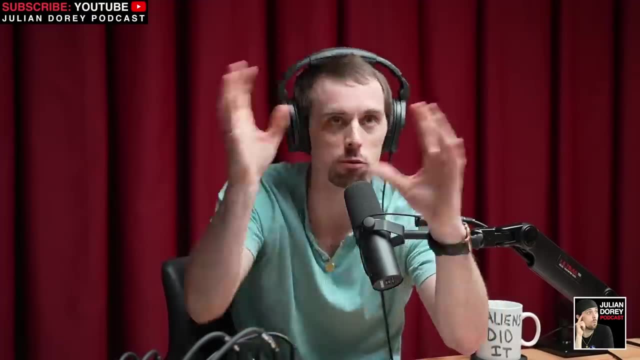 you think it's possible that you could have some form of- in your research itself- confirmation bias to want to find something that could replace this in a better, higher spirit consciousness way that's going to improve the whole systems that you think totally made you upset as a kid. let me give you a 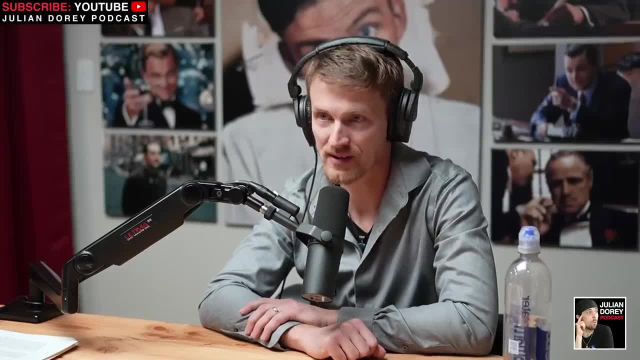 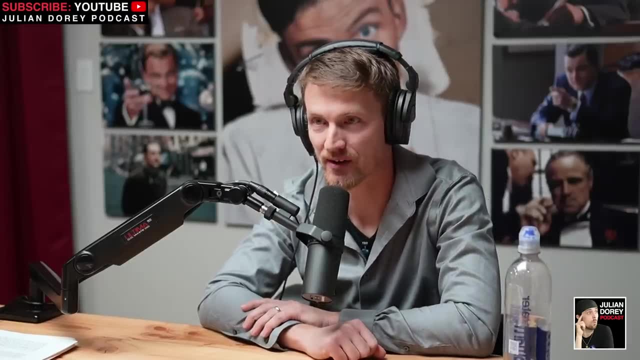 good answer on that. i didn't plan on doing any of this. i wasn't like that. that kid that at 12 years old, years old, is like: i want to be a teacher, i want to be a teacher, i want to be a teacher, i want to be an agent history writer and i'm gonna like. this is people need to know about this. 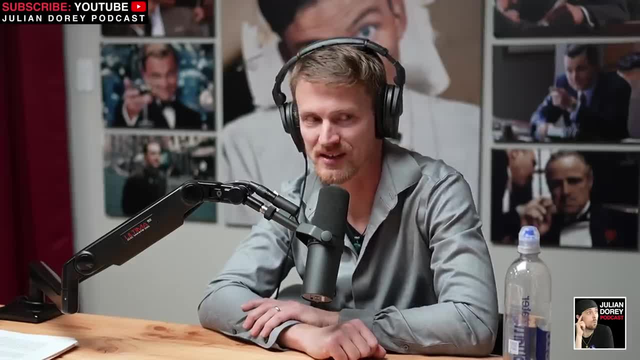 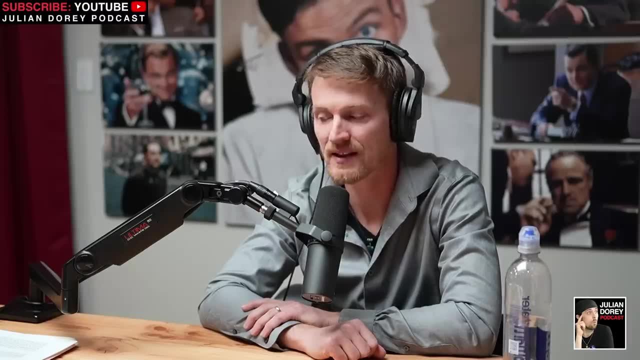 i didn't. i mean i was interested in it, but i wasn't anything like that was driving me to do anything. i was just going along in life like everybody else was, and i think this is important because i came to this from someone who didn't have any expectations or was looking for anything. 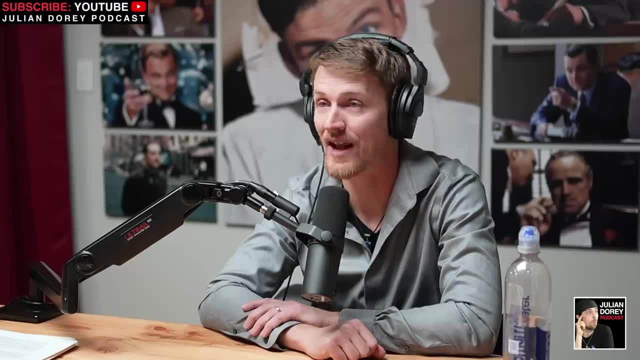 so imagine if you were like looking into something and like you already have a predetermined expectation of what you're looking for. so you're kind of worried about what you're looking for and you're worried right like it's the problem. i'm kind of worried that, yeah, that if i look into this, 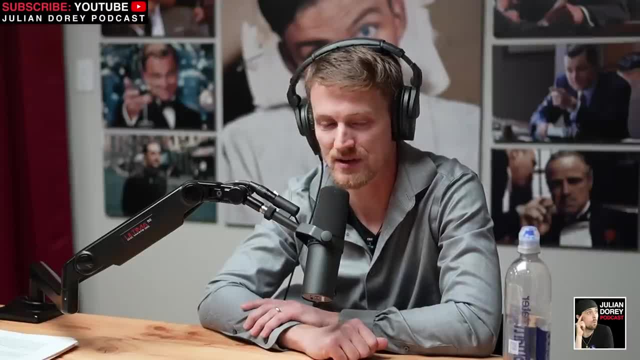 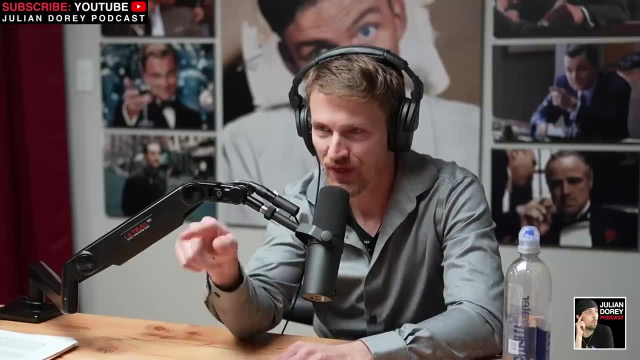 too much. it's gonna- um, it's gonna- provide pieces of information that like make me not believe what i did before, or something right, right, well, something we're all guilty of at some point or another. this like era civilization. anything i've done in this, it's been more like the complete. 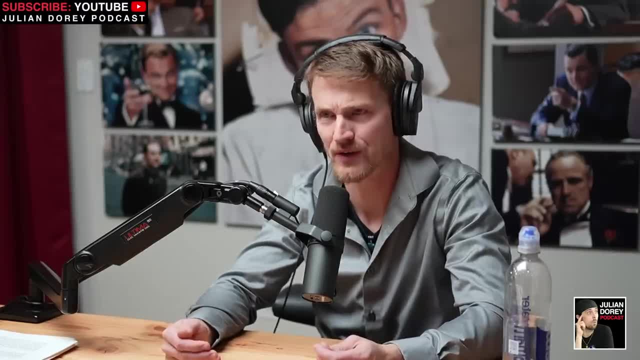 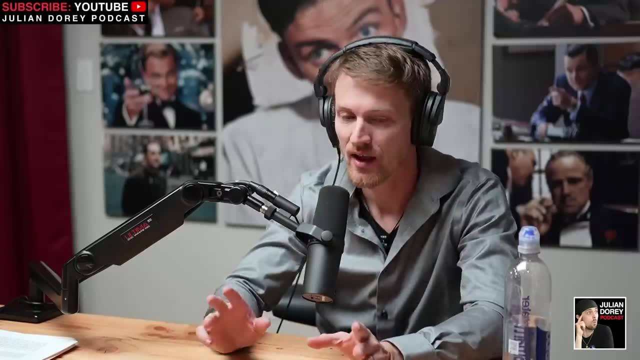 opposite where, like, you go into it and you're like this is kind of interesting, right, my wow, like how do they do that, i don't know, but this is kind of wild- and you start, you start reading, you look at it and you start, you start delving into it without any predetermined expectations, because i didn't 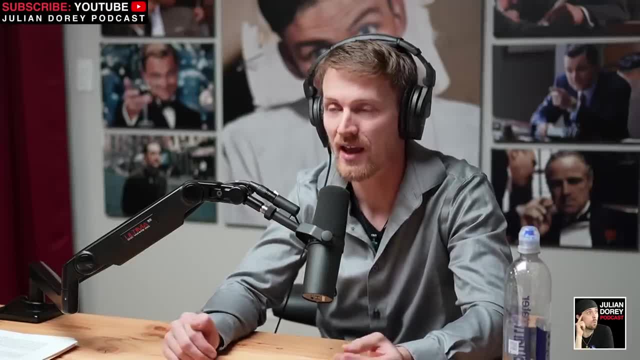 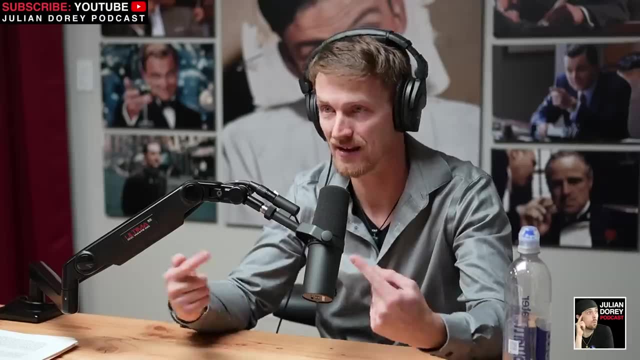 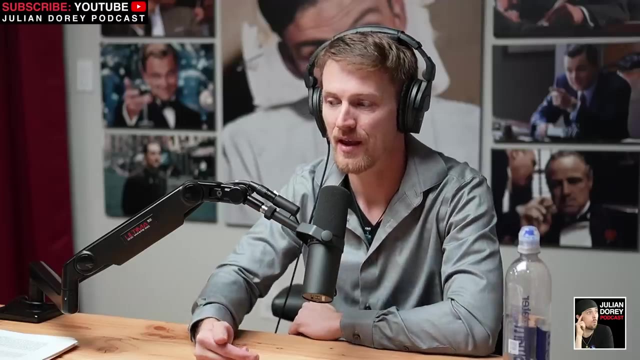 i just was curious, right, just curious and interested. and as you look more and more into it and you, you read what they left behind and you embody it, you almost you take in, you take in the teachings and what they were saying and you almost take it into your life and you, um, you try to live. 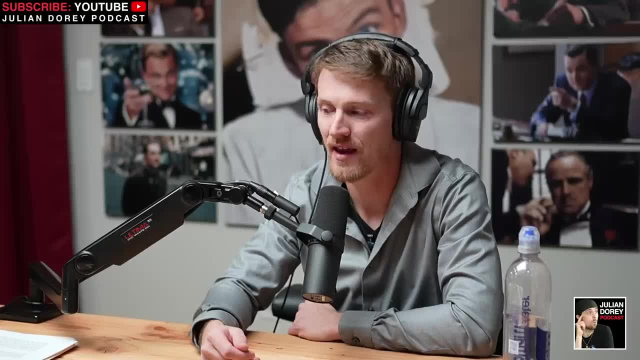 what it'd be like with their mindset, or at least entertain the idea of it. and it's what i can say is. the point is that i'm not going to go into it and i'm not going to go into it and i'm not going to. 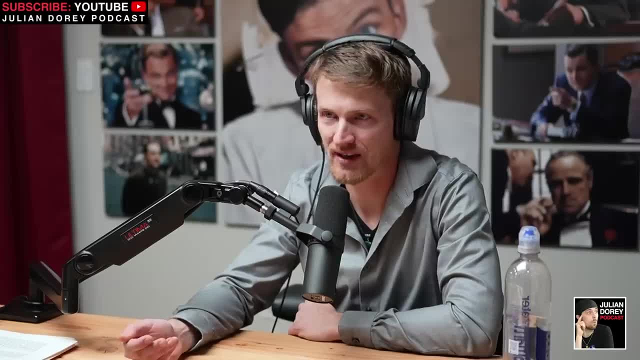 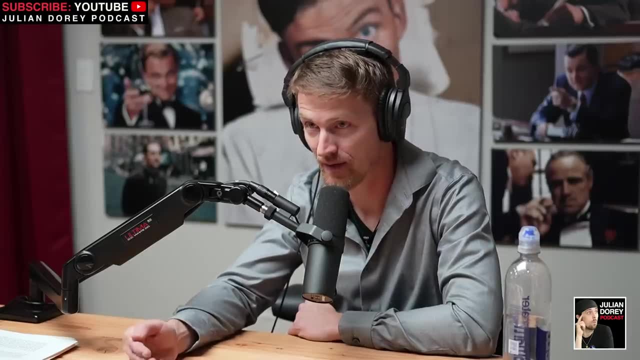 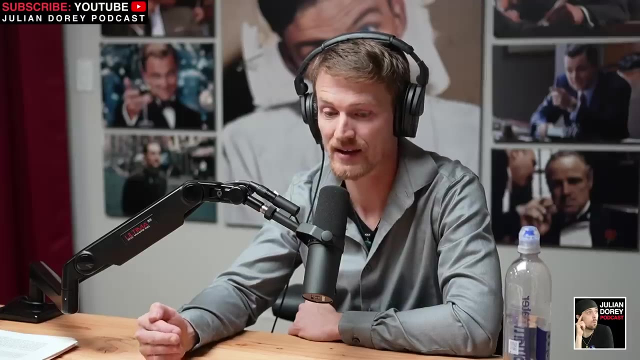 the point i'm trying to say is that i wasn't looking for any expectations or i had no predetermined things of what i was going to find or anything. it was more like the more i looked, the more i couldn't believe what i was finding, the more that it became so powerful that it changed, like my 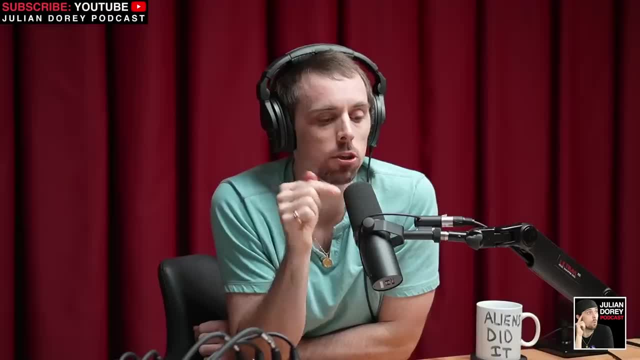 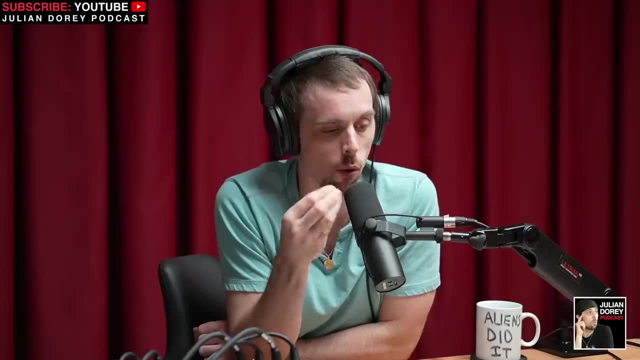 entire career, everything i thought, everything i was doing. that might be true, but also- and again, it doesn't discredit what you're finding either- that's not what i'm getting at here. i'm still. i'm trying to get at the core of like making sure we don't go too far or any situation like that, because i think that happens across. 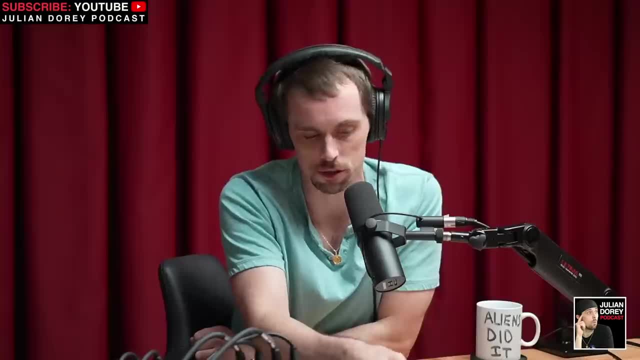 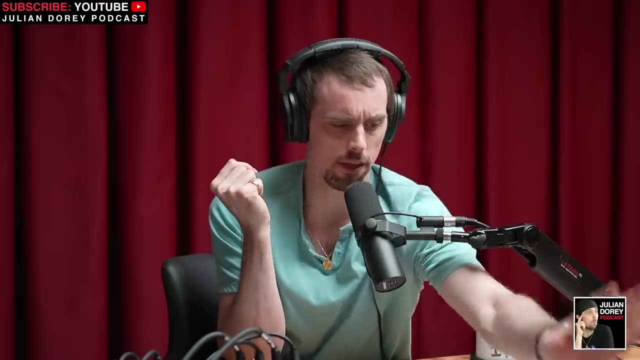 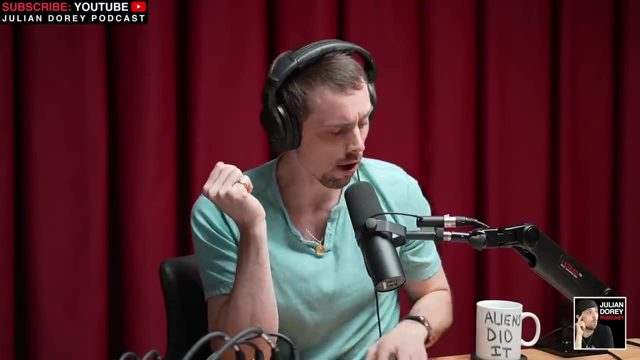 anything in society where we have one side and another side. right, there's mainstream versus not mainstream, perfectly fair. but you may not know. oh, i was going to find this box relief right here. oh, i was going to find this exact temple of the sun right here. i didn't know any of that, it fell. 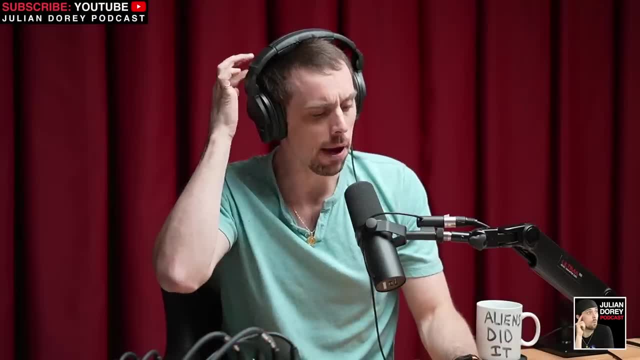 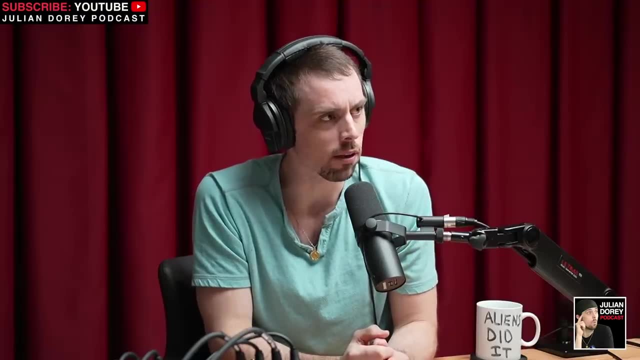 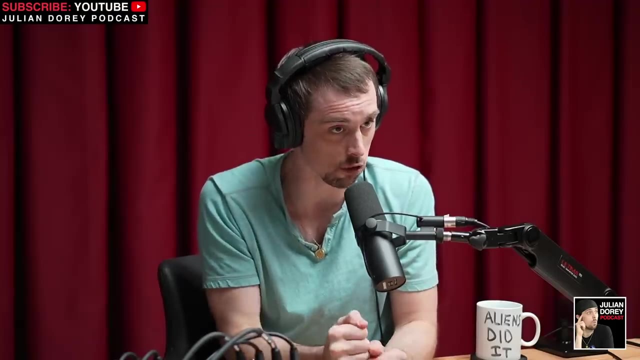 into your lap. but you, it might be fair to say- and this doesn't discredit you, but it might be fair to say you already are pissed off at all the base teachings that happen because you believe so much of history is covered up that you want to find the things that are covered up. so sometimes 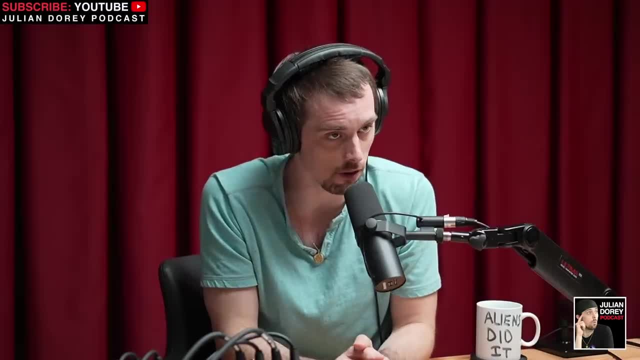 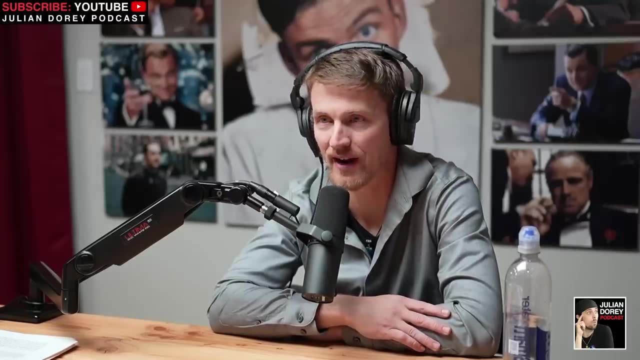 and it might not be this one. yeah, you may find the things that you think are covered up that maybe aren't, because you want to believe that it's covered, totally true, i mean it's that's. there's always conformational bias, like built into someone, which i do as well. i, i understand. 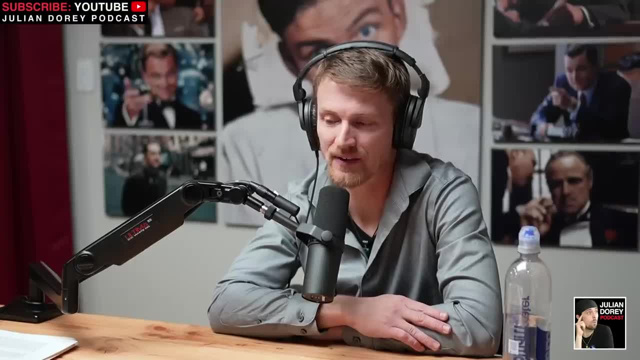 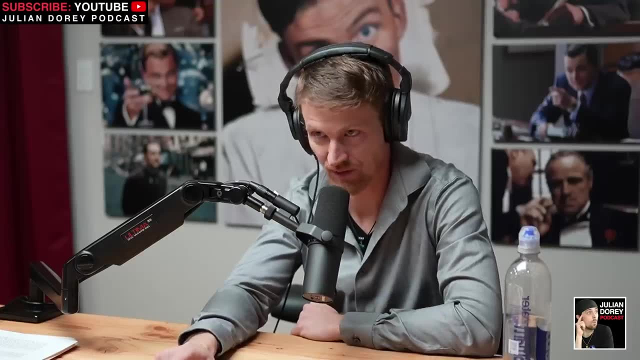 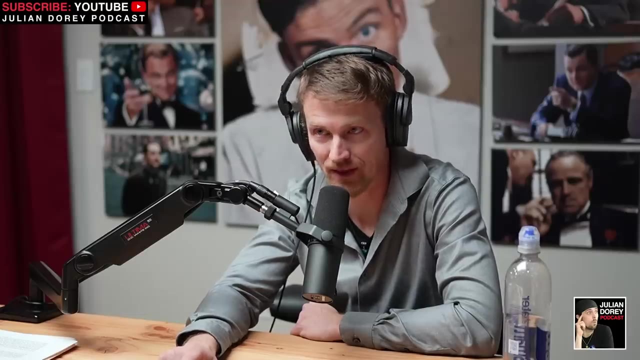 that and that's a glass house. that's a fair, that's a fair point to make and i think that that's something to consider. but i'll just say that i wasn't looking for the civilization. i wasn't, and even when i started to find pieces of it, i wasn't hoping for anything. i wasn't like: oh my god, i hope this turns into. 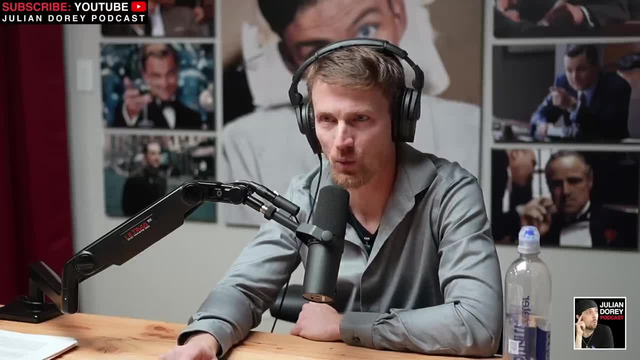 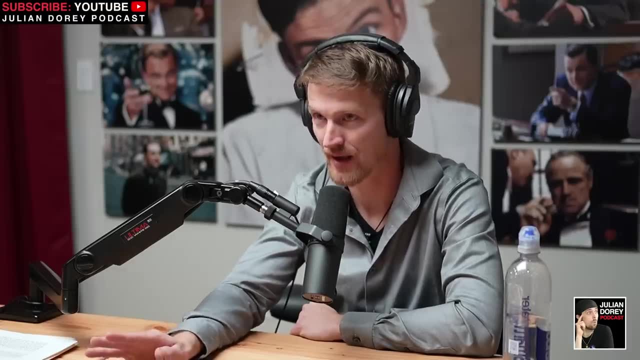 something bigger than it is. it was more like boy. that's really weird. what is that? that has similarities around the world. i want to know more. and then the next one has like even bigger stuff. and then you're like: and then i saw ionis and i was like holy, you know, i could not right. 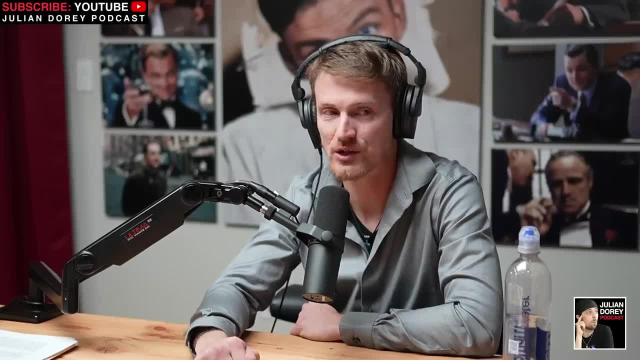 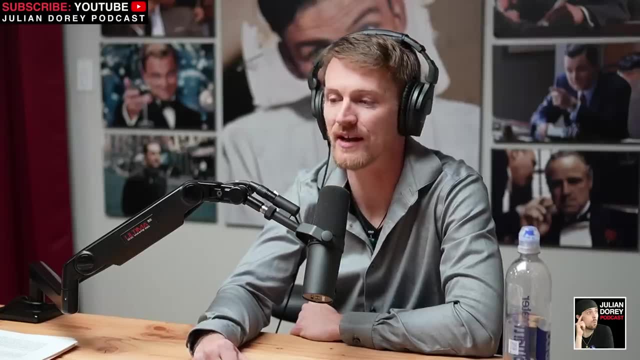 it was, for me it. that's why i said it was a george smith moment, like i wasn't expecting it at all, and i think that's what you're trying to get at is: yeah, i wasn't. i wasn't like hoping that something would bend around. what i was looking for to become something like: oh, i hope this. 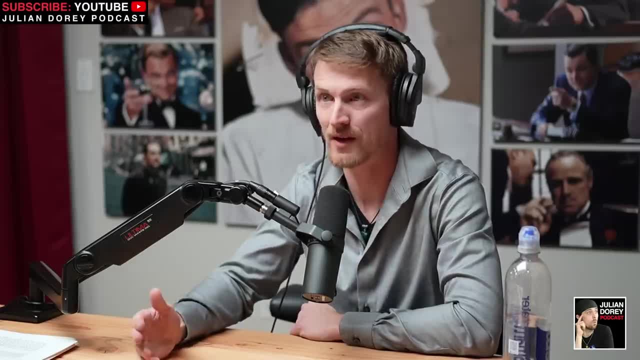 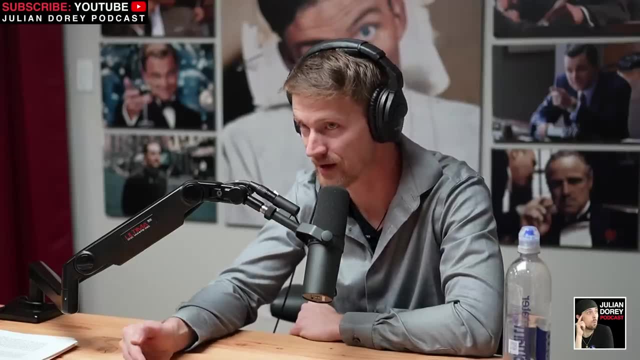 civilization exists, to finally prove everything. it literally just fell into my lap and the more it unfolded, the bigger and bigger and bigger it got, until i realized the implications of what it really was. from someone who's an obsessed, i can look at any megalithic wall and i can look at any 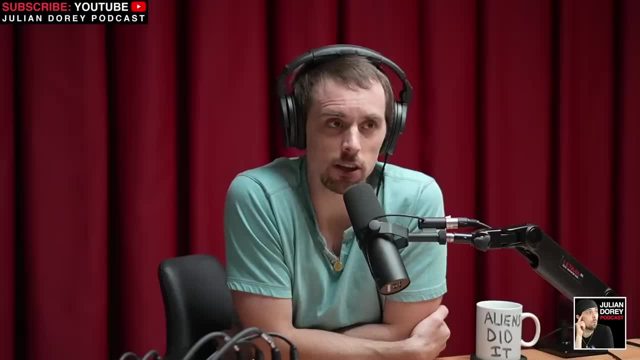 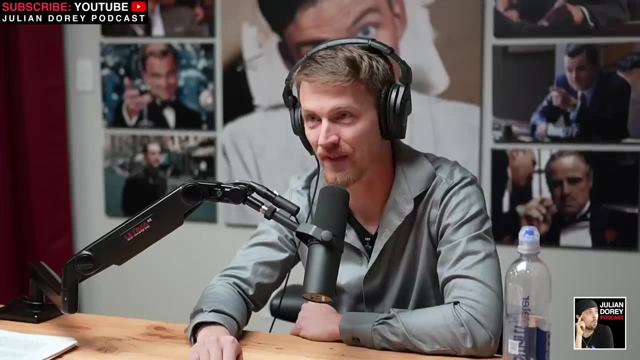 megalithic wall in the world. i, i do, i, i do. i will hang my head on jerk off to megalithic i. i can look at any megalithic wall in the world and tell you where it is. so i hope someone can challenge me. 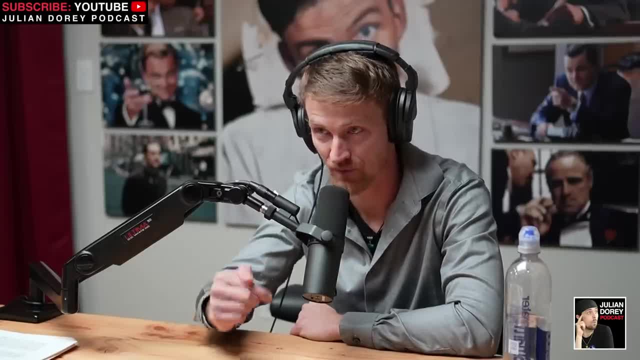 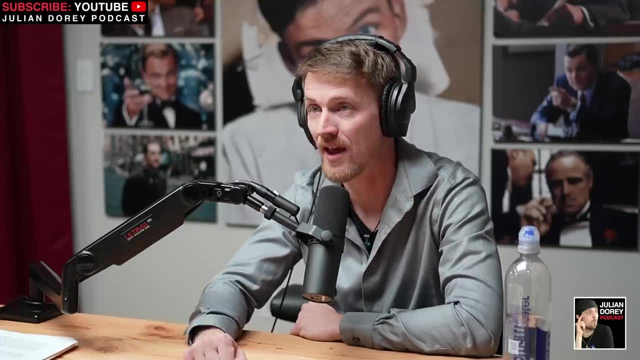 on that? yeah, um. so when i saw these, it got my attention very quickly because i had never seen those walls before and that's what led to these discoveries. but your point is fair to make. i had no expectations or anything going into this, or even knew what to expect. it fell into my lap and 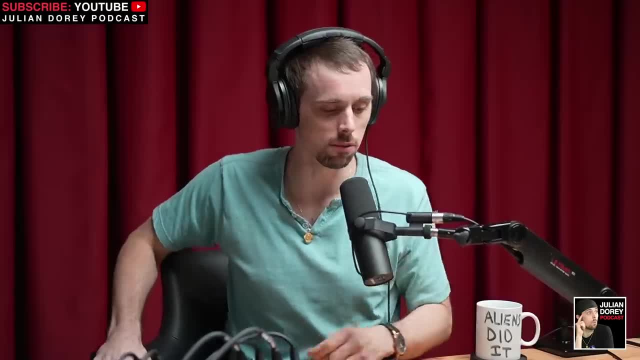 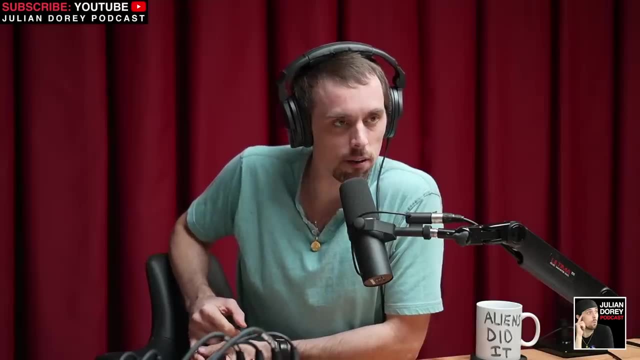 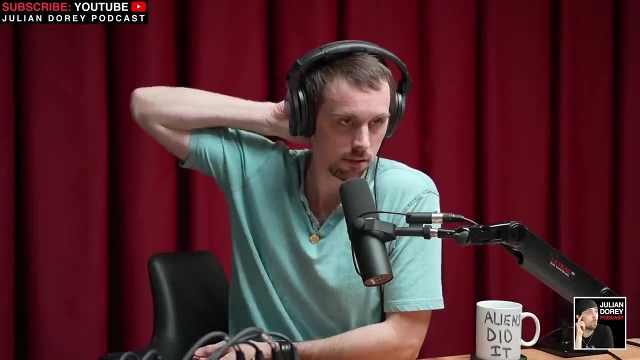 then changed my life forever. recently too, only well about a year ago, this all started, yeah, oh, so you knew about some of this when you were in here but weren't talking. you wouldn't know. well, you and i were talking, i had found cavus, just not discovered, but had it connected. i'll say connected cavus and kef. 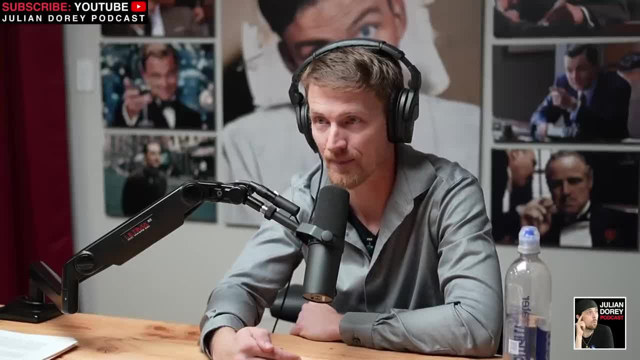 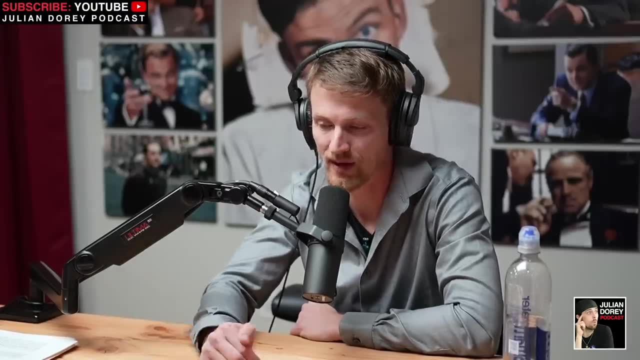 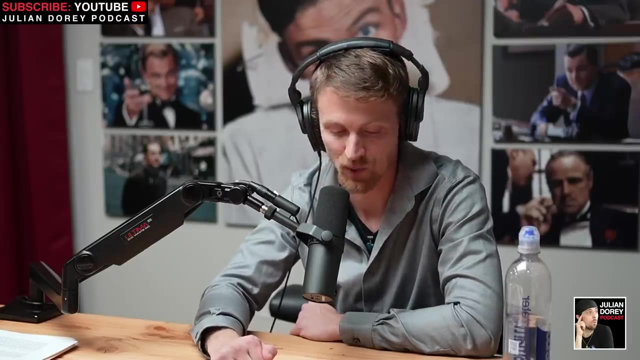 but i hadn't even known about honest yet, or the connections with south america. so a lot of this grew and got bigger and bigger and bigger, and i think i think the whole point of this is that we're going to try to tackle this film and i and i- i do want to just want to mention this to people- so what we're doing is 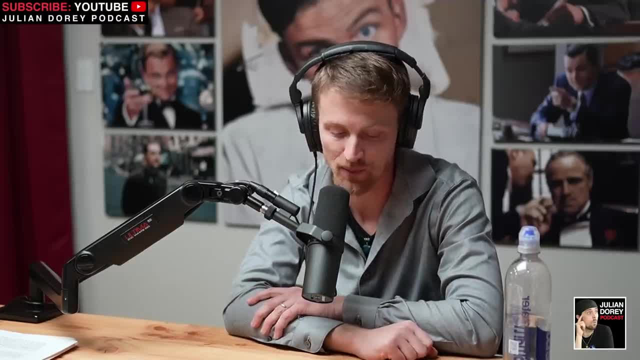 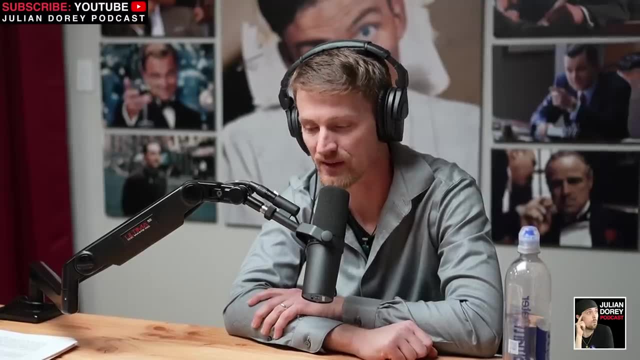 we're. we have an incredible director and producer- i won't mention um who they are yet, but they've done some amazing things- and we have a team of four experts from around the world and we're going to be traveling to lake vaughan, to these sites and bolivia, and we're going to go and and. 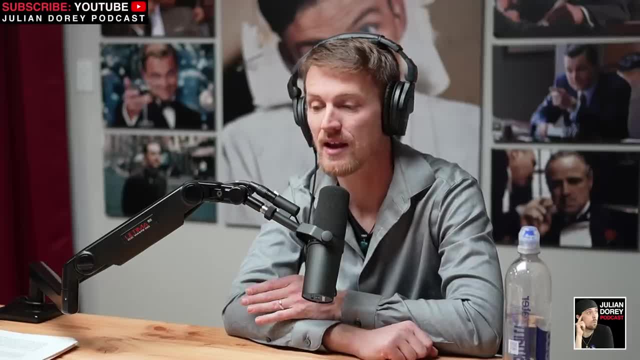 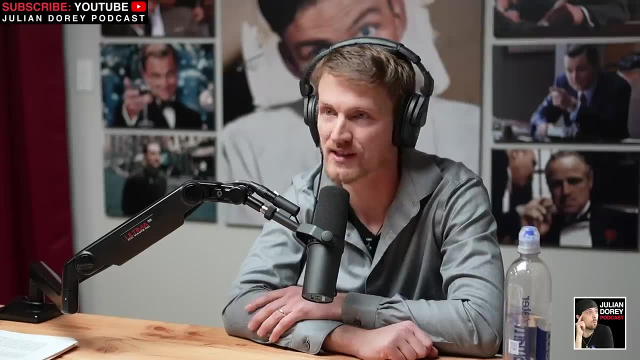 capture all of these incredible sites, these discoveries, bring them all together in a like, in a film that is powerful, and then go and do it. and i think that's what we're doing, and i think we're going to go all the way to bolivia and show the same symbols and we're hoping we can build off. 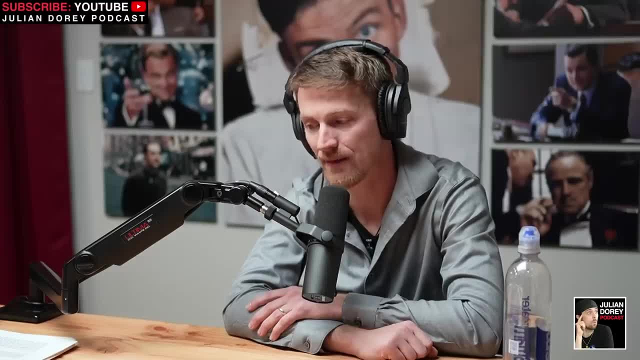 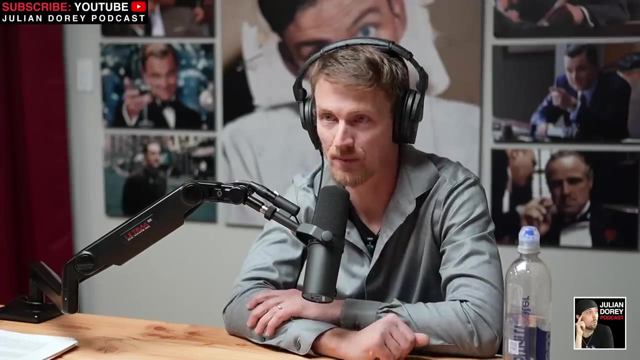 of all the amazing work, like graham hancock did on netflix with ancient apocalypse. i don't think people are understanding the significance of that. it's all about pushing a narrative for it forward. in order to do that, it takes a lot of time. moments like precisely time for when people are ready. 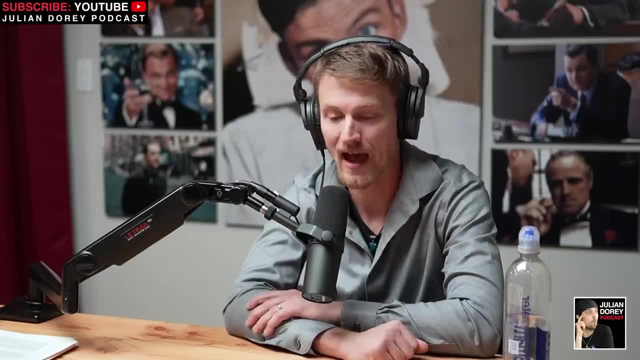 and graham getting that on netflix just opened up the avenue for this to be talked about in a way that we're never going to be able to do in the future. so i think that's what we're doing, and i think that's what we're doing, and i think that's what we're doing, and i think that's what we're doing. 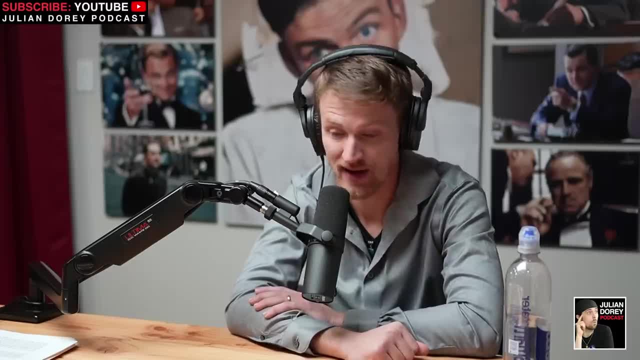 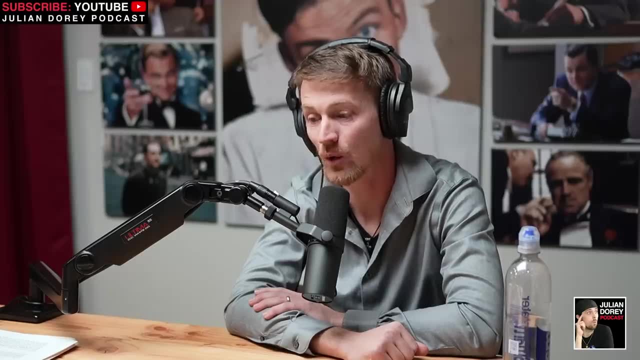 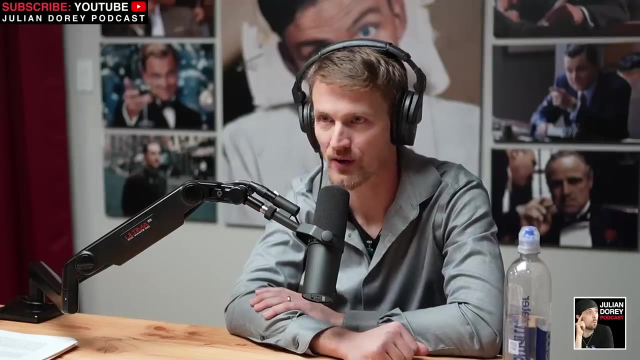 has, and so what we're hoping to do with this- to get on netflix or something like that- is to make a film that encompasses this in a way where it, like, touches people's hearts. you know, like, imagine- touches people's hearts in a way where- look, here we have potentially the oldest cross on earth, that. 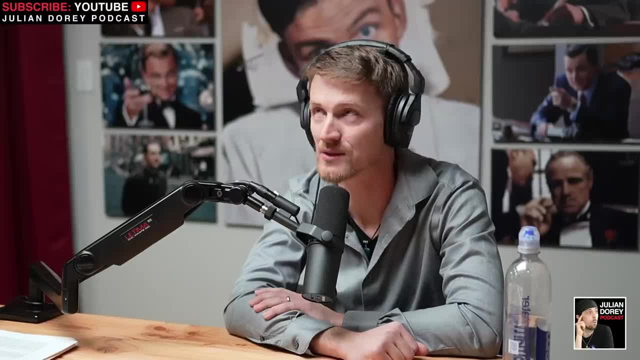 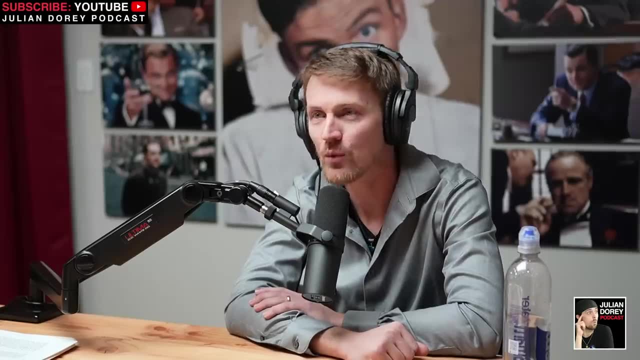 was supposed to be about this totality of harmony and balance with the universe and reaching these higher states of consciousness. who's going to fight that? in terms of like i don't like that, like what do you mean? like these are, as long as you back it with real evidence, right? these are the core teachings. 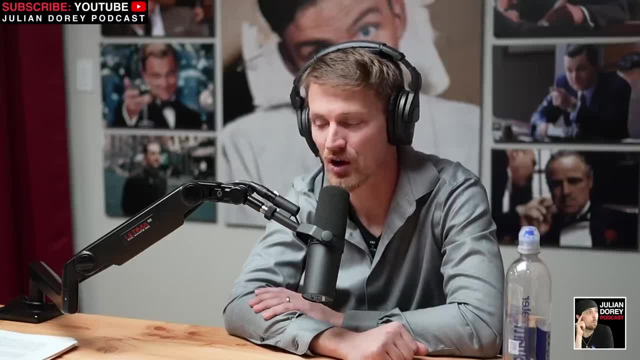 that went around to whether or not it's the ancient hindu civilization cultures or it's the ancient maya, or it's the ancient peruvians or the egyptians. they understood a lot of this. they understood it. people, you the thing about this stuff, and this is why i don't envy the. 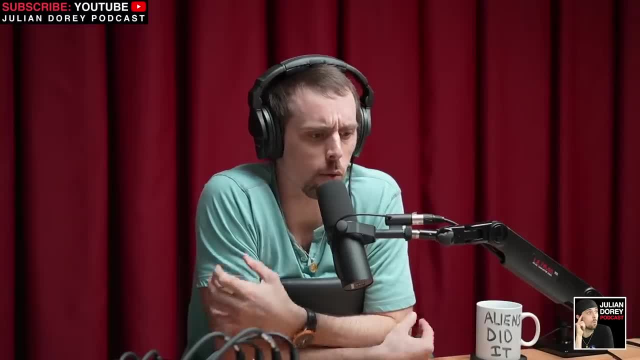 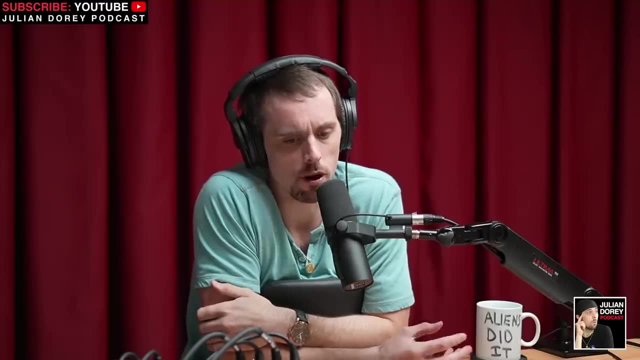 position you're in in this way. i i'd love the type of work you do and like the research, but when it comes to the messaging of it, the reason i don't envy being in your position is because you're not. you're not like: oh look, there's groups always and everything, but you don't really get there. 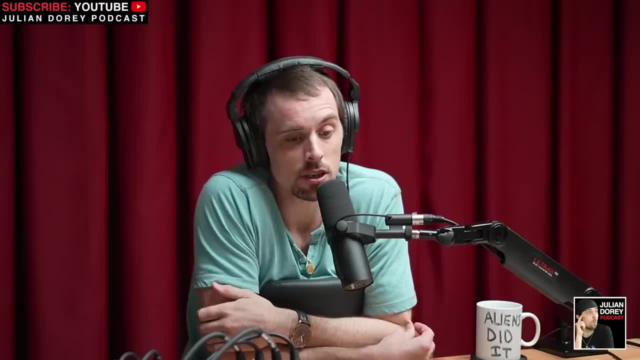 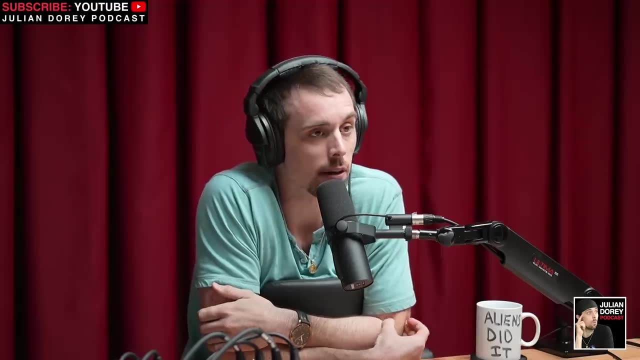 and why is that not being an issue? i really don't those groups are that eager to give you to begin. really, thank you. it's really interesting this question. but like yeah, right, um, so when you come about repetition in a way like perhaps society thinks that everything denken every. 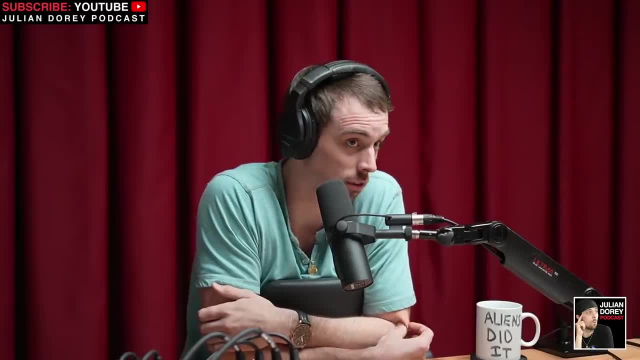 person and you kind of talk about it with the same sense that an active ITAL GENETICAL PASSAGE ly города. that's how we get to its real culpability: Paracletic Vertical Sygusal, package it in a great way and say, oh, we're gonna look at our consciousness and excitement and you 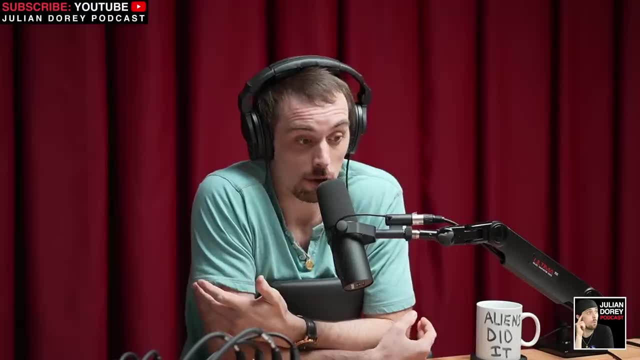 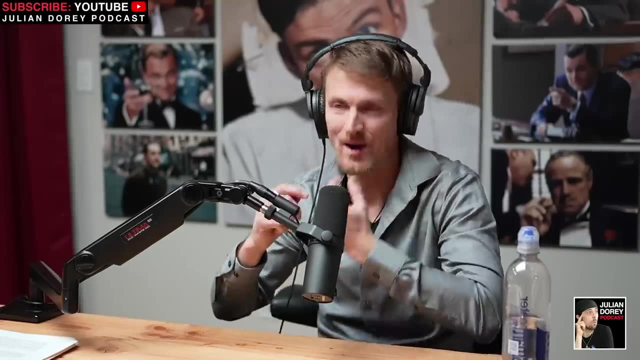 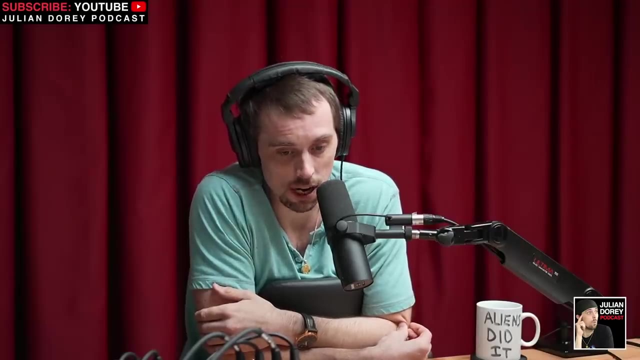 said like: oh, who's not gonna buy into that? a lot of people are gonna buy into it, for sure. a lot of people aren't though, too, and that's okay. no, i think that's normal. there's nothing wrong with that. it just is a shame that you know we have trouble in parts of society talking about these. 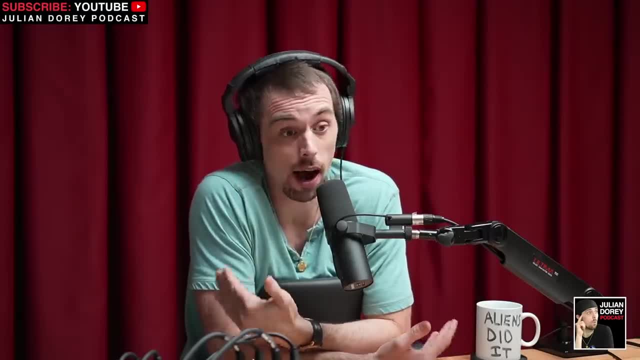 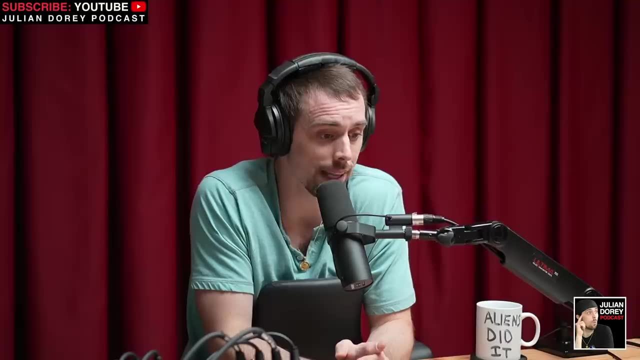 things. i mean, look, that's why i do what i do. i believe in talking things out. you know, i love, i love this stuff, i lean into it. it's just it's a very difficult, like like i agree what, what graham did doing that show and getting another, a way different perspective on there, literally on the 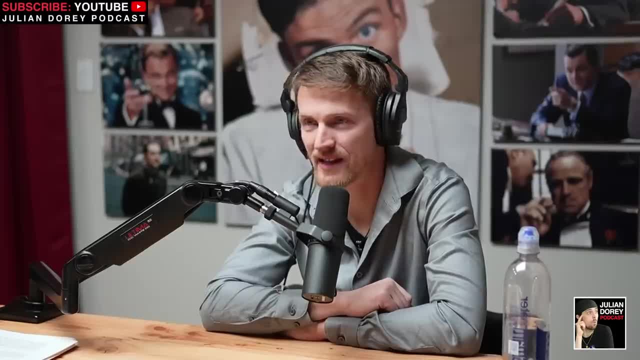 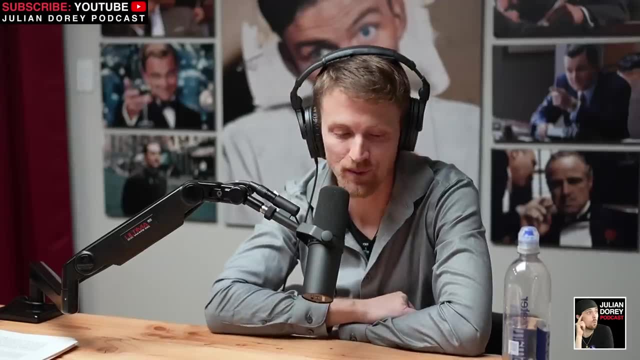 mainstream, right, yes, like grant went mainstream, let's fucking go. well, that's what i mean is that it's the time for this. it never has been until now. yeah, and, and that's why we're gonna- we're gonna make this film. we truly want to touch and capture the hearts of not only people, but to try. 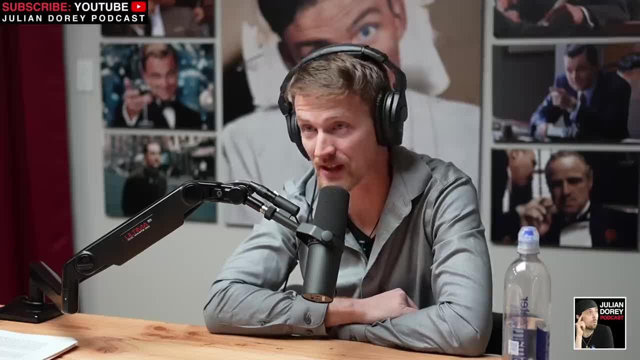 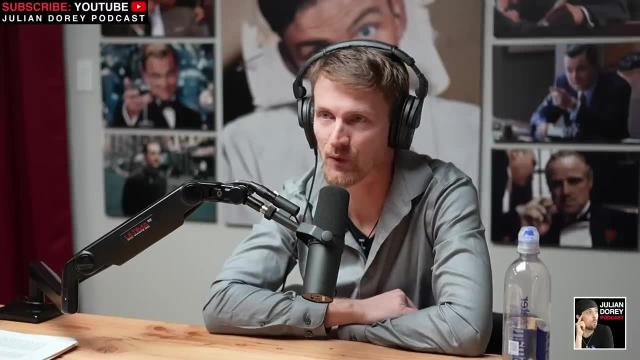 to change the narrative of ancient civilizations and how far back we go and sophistication, all those things right. so we're trying to do this for a position to do something good we really, we really want. this story needs to be known by the world. it's waited long enough. 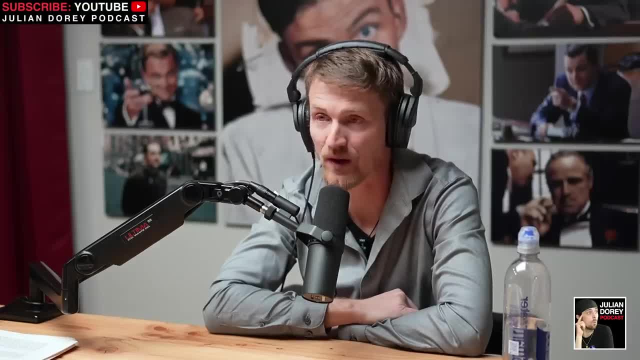 and so, if, if people want to be part of this, to contribute to the, to the film or at any point, please go to the stage of timecom and just check out everything we're trying to do because, um, you know it takes a lot to change history and i know that's a loaded statement, but it's not just. 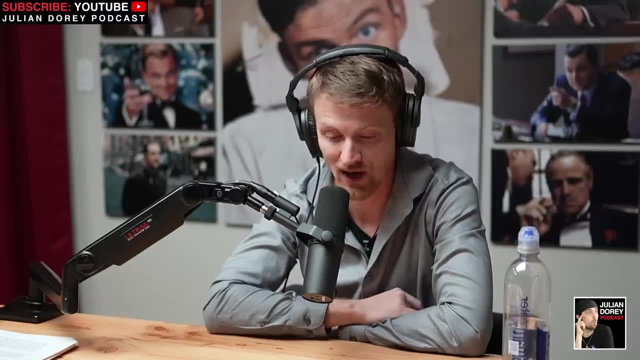 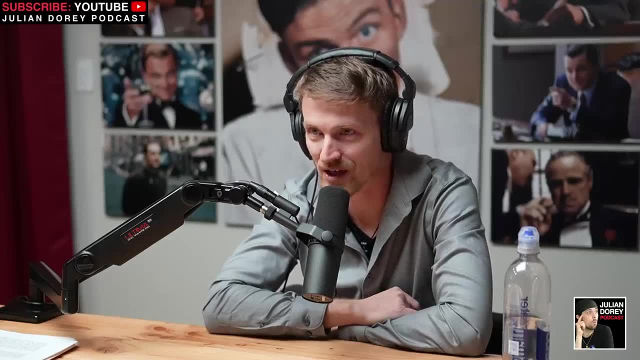 one person like graham and, and like you, you want to know who changes history. how about, like the, the start of what unveiled with robert bravall and john anthony west in egypt? that's called changing history. you know what i like that. i just thought of this on the spot right now. i'm surprised i haven't thought of this yet. 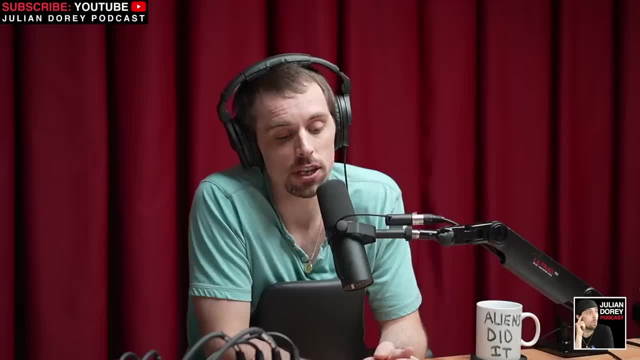 i like the idea of discovering history right, because changing it doesn't. actually, we could discover things that go beyond what we already have known or have been taught. yeah, i like that because look at- i mean shit- how much of the ocean has been unexplored. do you know? at the top of your 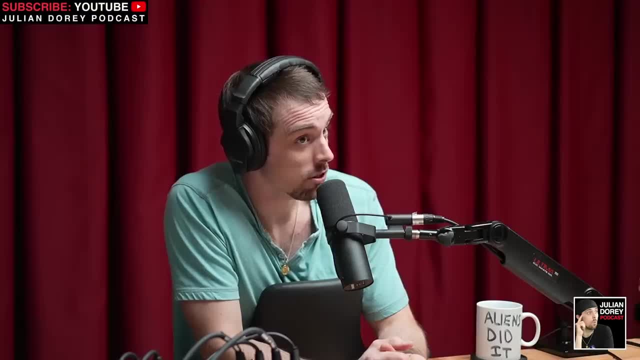 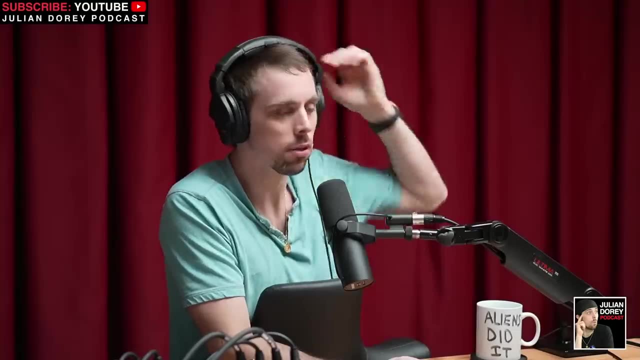 head. five percent. five percent's been explored. five to seven percent right. so just the ocean itself, which is a physical thing right here that we could all go to, and our planet's 70 per 70 percent water, roughly so, right. so you think about that now, think about how much our history is. 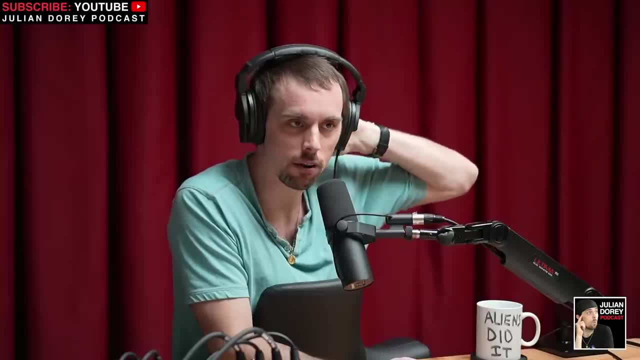 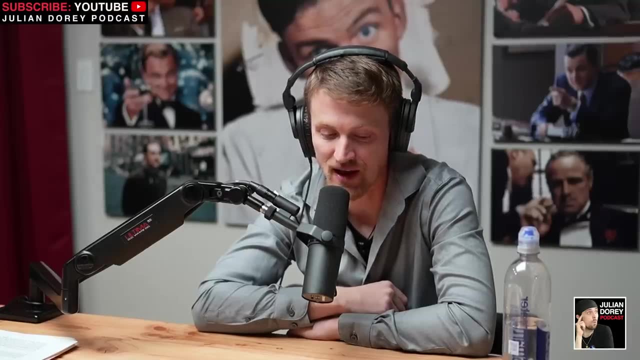 unexplored totally. we're constantly discovering. we're using our past to create prologue in a way. i don't know if i'm using that correctly there, but no, that's, that's good and you're right. it's like, instead of saying that the era, civilization and its implications are going to change history. 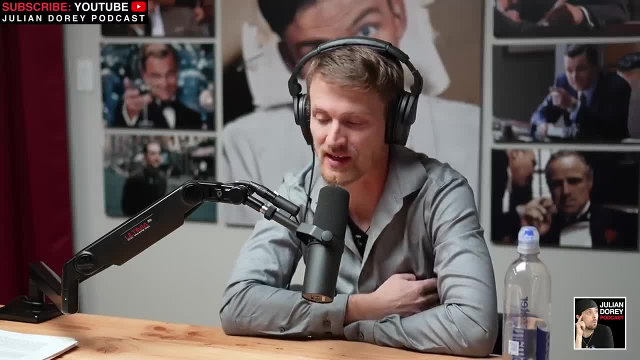 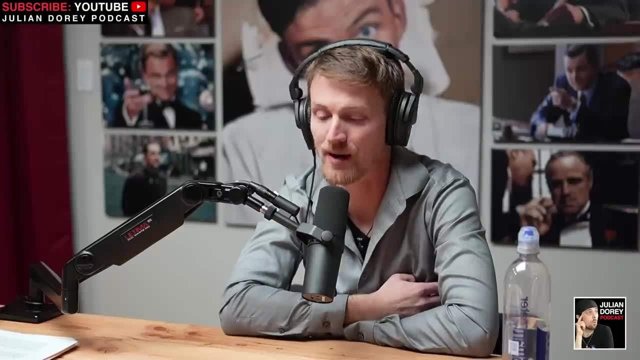 maybe this film and what we're doing. i'm writing my new book on this and i'm going to be taking at least two trips to turkey next year. i have two already planned- yeah, that's exciting- in egypt and bolivia. yeah, yeah, we're going to be on site doing all this. 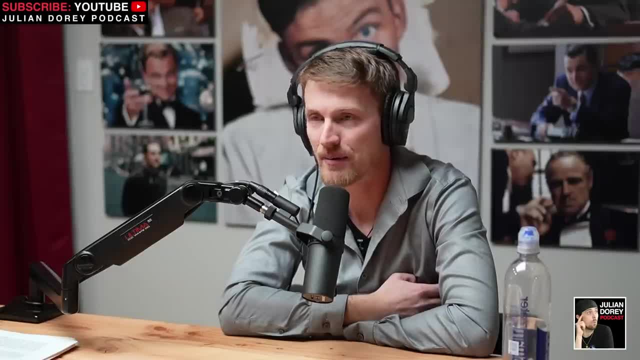 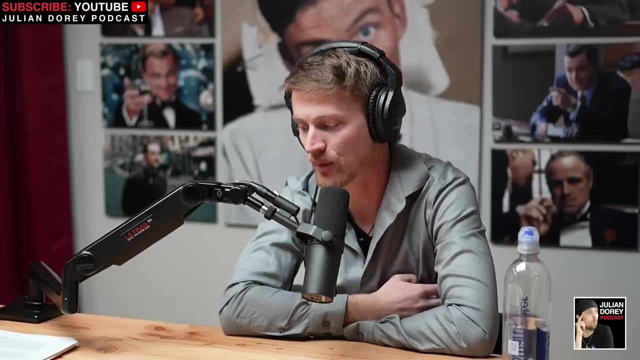 that's awesome, um, is that maybe you're right? is that we're really we're discovering history here? we're discovering it and maybe that's a good point. is we need to stop saying that we're going to change it? is that maybe we need to discover and then just rewrite it in the right? 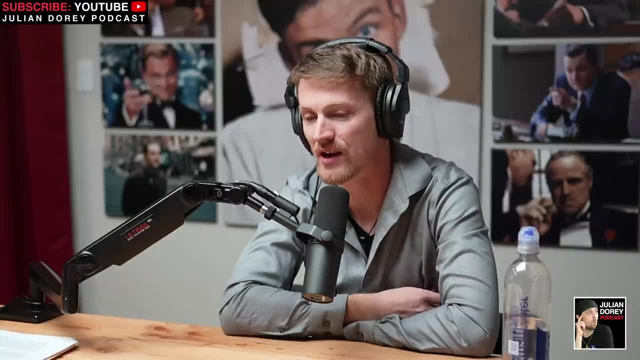 way. i hope that someday that i hope that someday that archaeologists can completely get out of that mindset of not being able to step on anyone's toes and not being objective. i want archaeology in the future to be like: this is what the evidence is. yeah, let's try to figure. 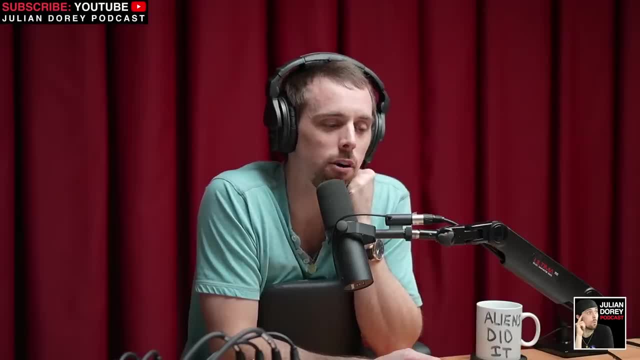 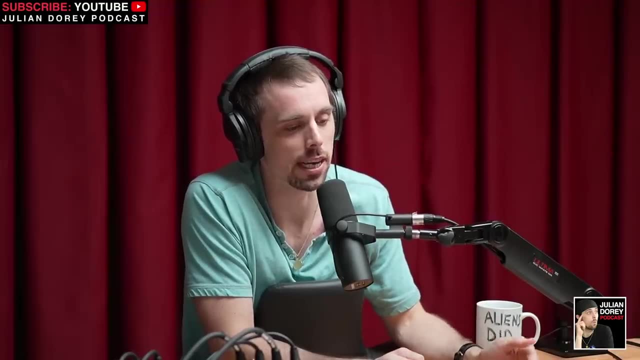 it out and let's try to constantly disprove it by finding something farther there. this is where science and history meet. the farther back you go in time with history, the more you need science to actually get to where it is and not- and science is, by the way- is, in a way, finding, using science. 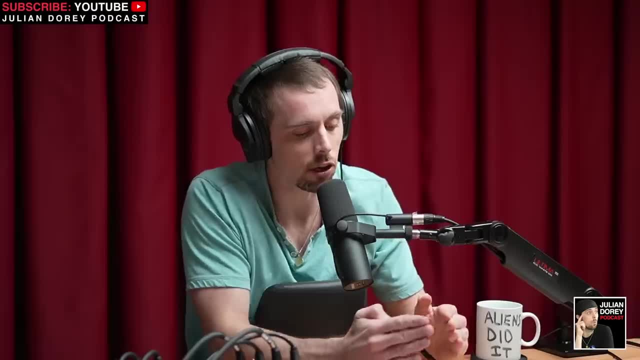 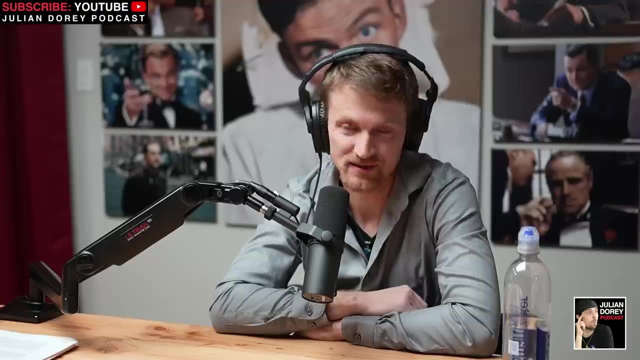 to find stuff like this right, absolutely. it's amazing. the cross pattern there is there, and that's the beauty of it. a guy like albert einstein is one of the greatest to ever live- greatest minds. yeah, the beauty of his work is that one day, maybe not even that far down the 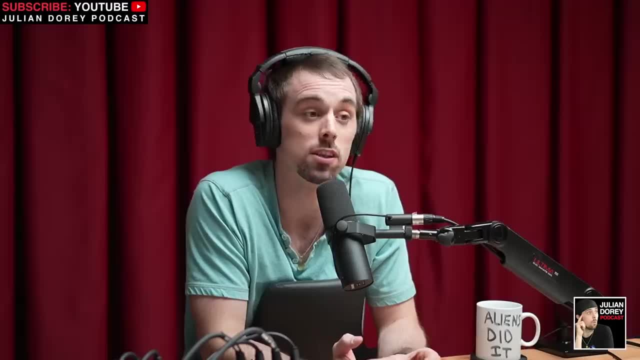 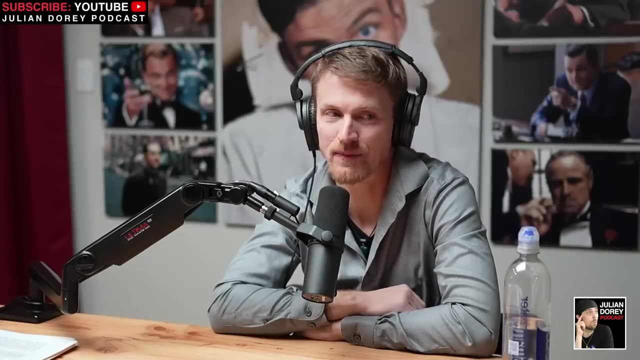 road. almost everything he worked on will have been able to be disproven in some way. well, it's incredible, but it's also sad when someone like someone like, maybe like nikola tesla, dies before they ever know that any other discoveries were ever found. i mean very sad, i i mean i guess it. 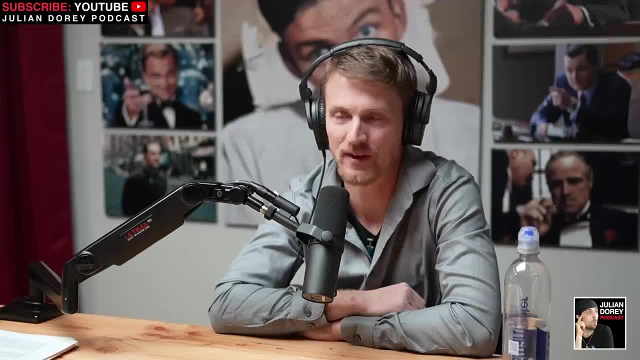 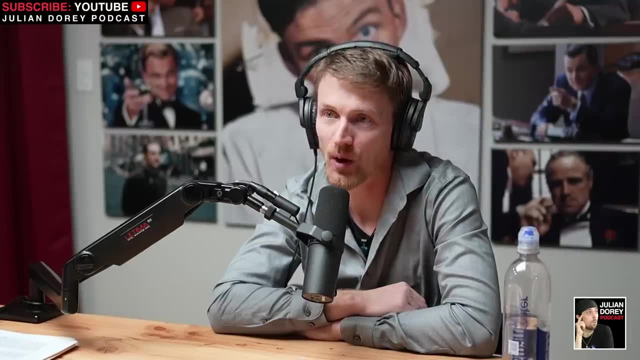 gets back to the idea that we're energy and we're eternal. it's not like we're. we're in some fiery pit somewhere, like waiting forever in damnation. obviously that's not the purpose of this life. the purpose, i think, is to try to take it as far as we can. you know what can you like you're doing, having all kinds of people? 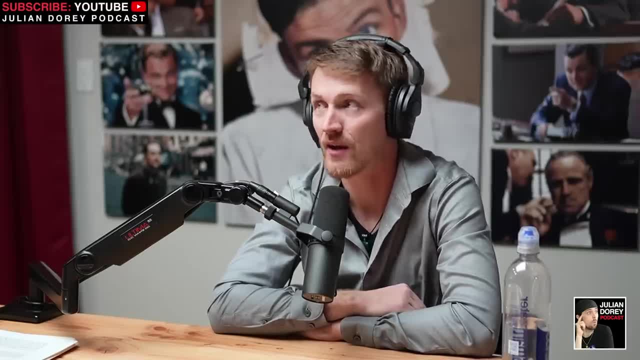 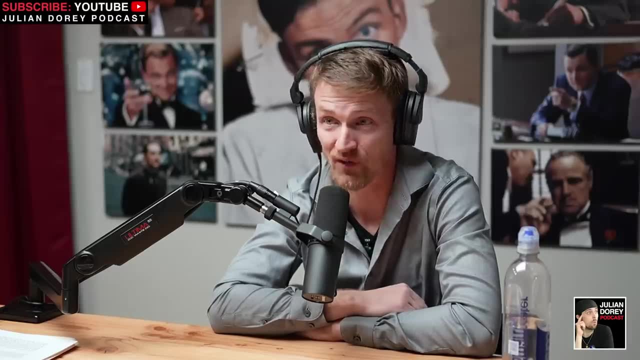 come talk and try to change. change things, give different perspectives, open our minds up to different things. that's what we need to do, going forward as humanity, and it doesn't matter what it is in right, ancient civilizations, consciousness, or even just like what good food to eat. yes, we. 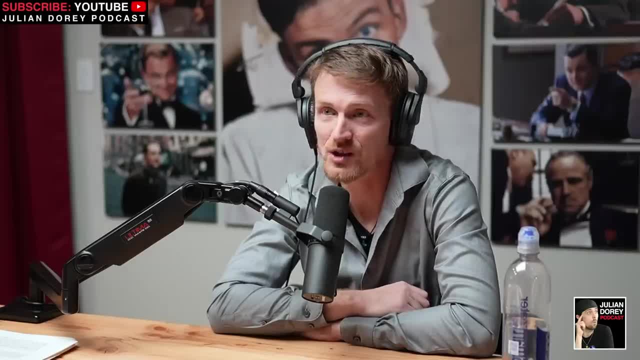 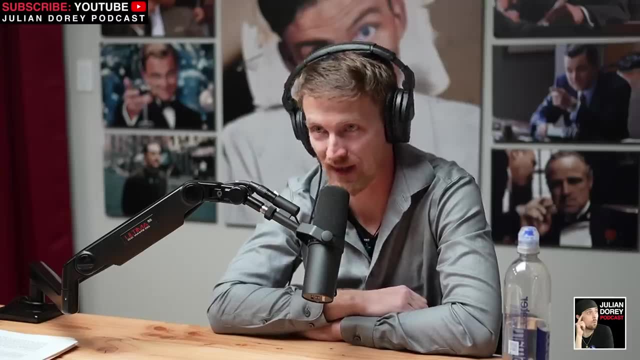 need to stop being afraid of what someone else thinks and just be open to like to talk about things, and i think that that's where we're gonna eventually go, and i know it's like blasphemy to say this might be the first, might be the first cross in history. 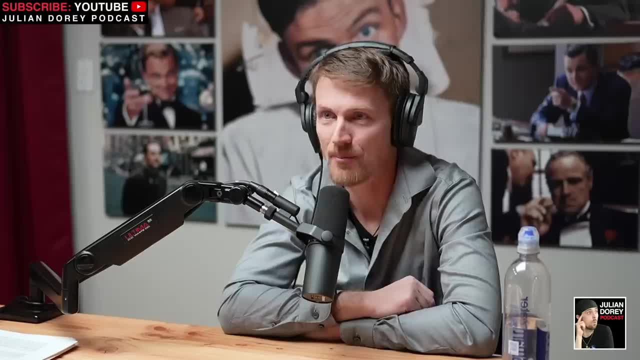 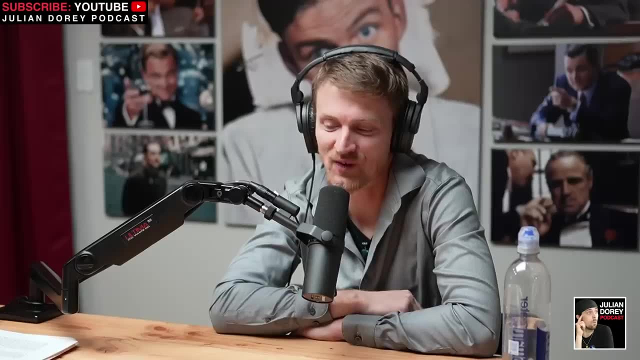 and the first cup chalice, right, and all those blasphemy, but to some it is, to some, but it's how you say it. yeah, that's that's why i was talking about earlier. there's different types, don't worry about right, right, but it's again. i just um, i cannot be more excited for where some of these 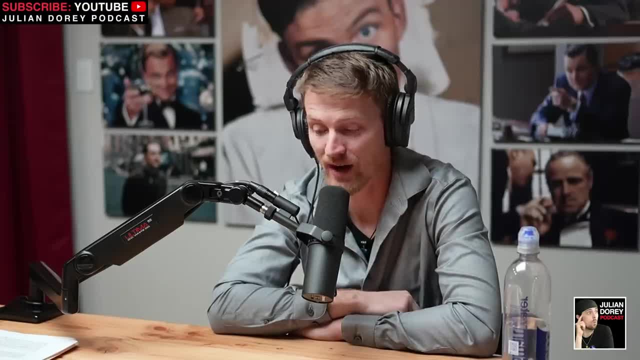 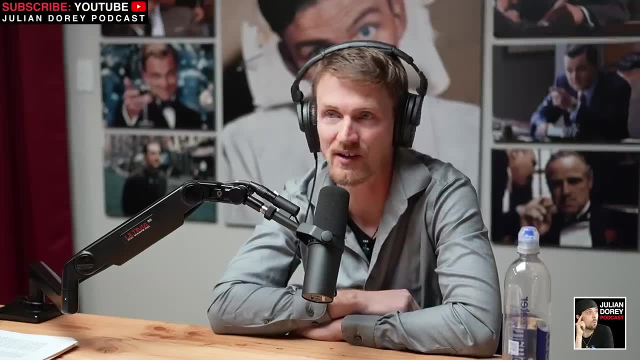 are going to potentially go um, and now when i get there we're gonna, i'm taking two trips, probably april and again may or june, and we're doing measurements, uh, complete photographs and analysis of the sites. we're going to try to go as archaeology, archaeological as we can without 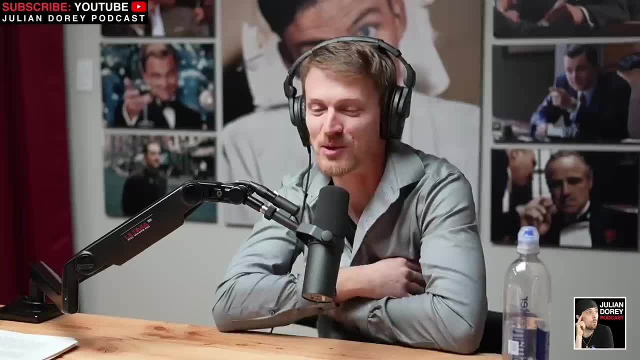 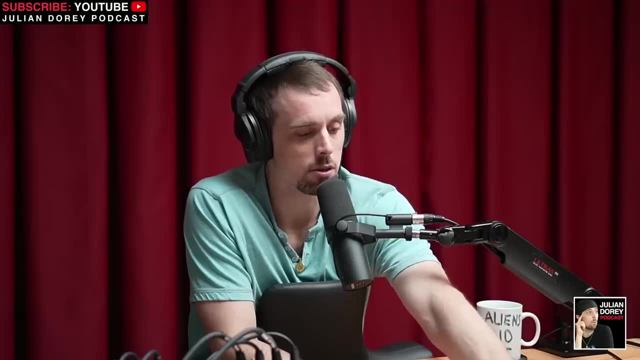 disturbing them and getting arrested or in trouble. yeah, right, let's not do that. um, so we're gonna, we're gonna toe the line with that, with with total respect on these, but yeah, i want to. i want to go back to this, though, because there was something that in my head. i put a bookmark in. 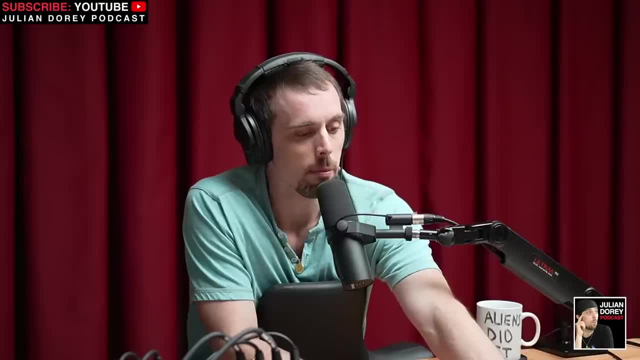 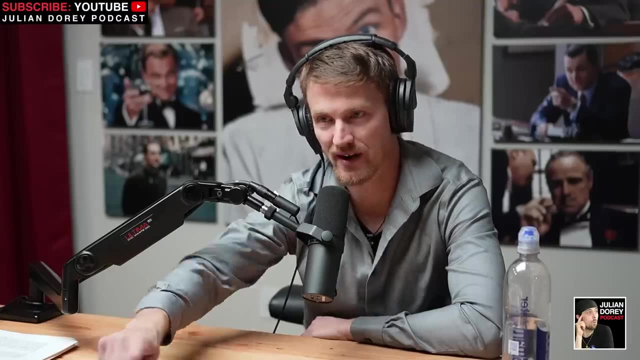 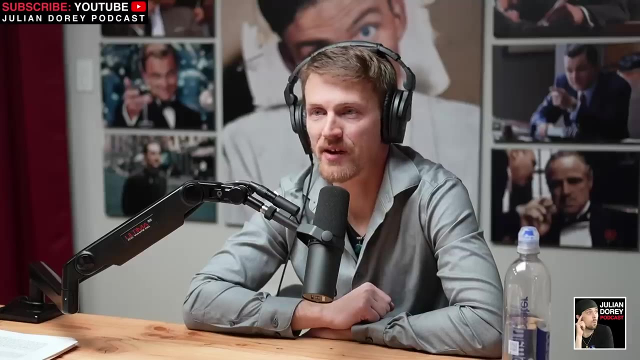 maybe was it 20, 25 minutes ago. okay, no, you mentioned the anuna, sure, in relation to what we were looking, which is what this is basically right here. yes, so we had talked a bit about the anunnaki, which is the same thing. the anuna is the sumerian version. we had talked a 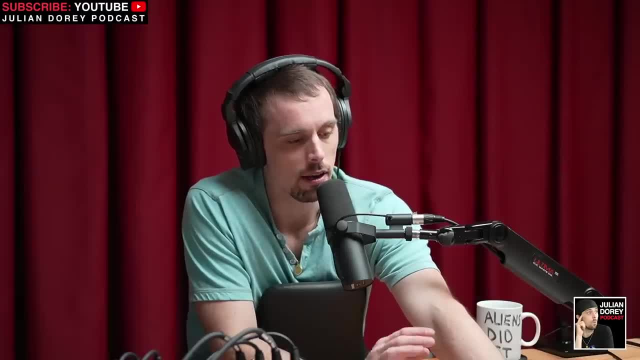 bit about the anunnaki last time and we hadn't really gone all the way down into it. so if you don't mind, what i'd like you to do is give some people a refresher on what we think we know about them, where the origins are, etc. 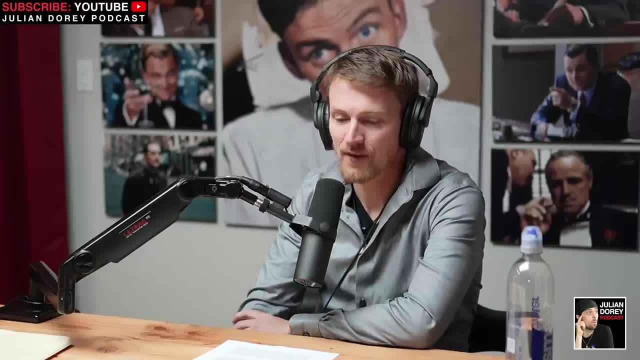 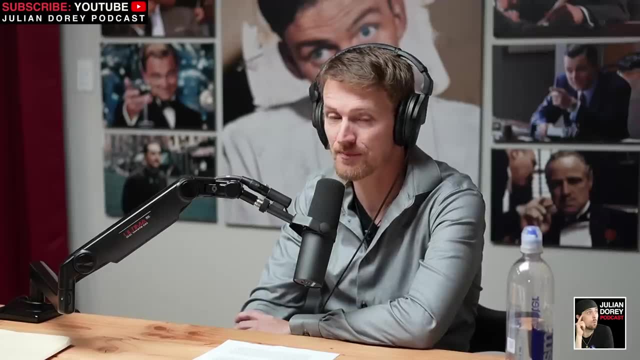 so the anunnaki or anuna, is a very mysterious area to explore. it's one that has a lot of opinions from a lot of different people, and it's perhaps one of the most enigmatic of all concepts to think about. and i really mean that, because then, when you read the tablets, about what, just how they- 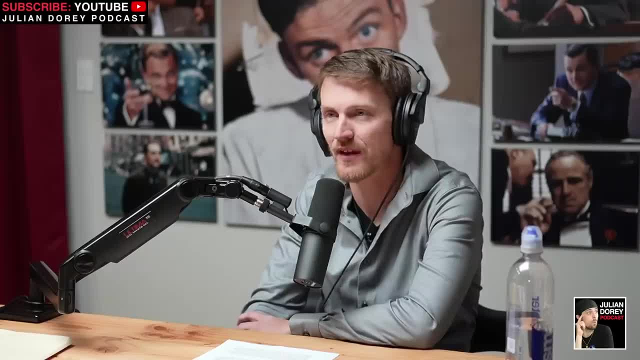 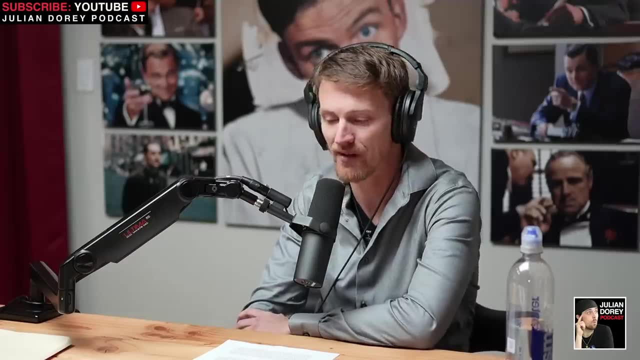 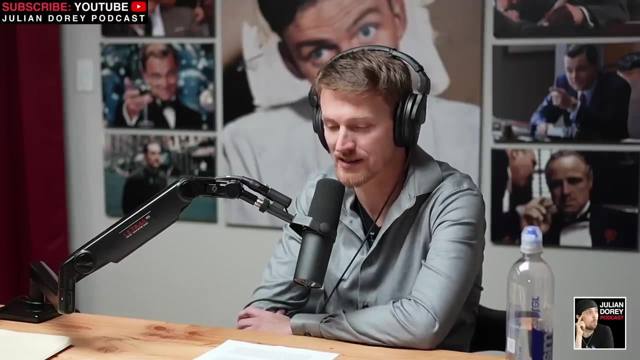 described, it almost comes across as supernatural and fantastical. it's something where we have to look at in a lens we're like. so what are they then? to give people a little background before i read a little bit here, just to fill in the gaps: is that what we find before the ararat civilization? 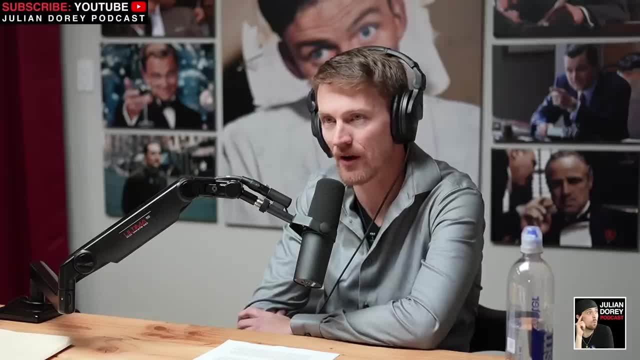 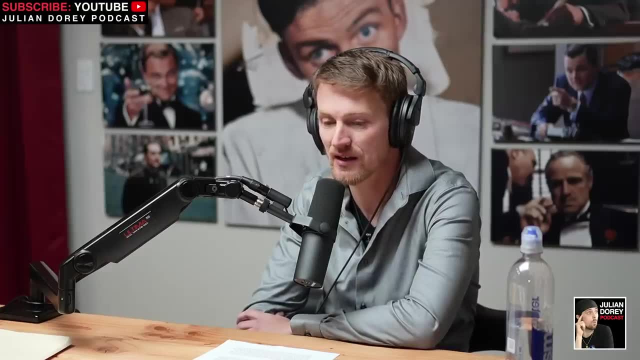 is that the original sumerian civilization that came out of the iraq area that i talk about, with aradu and then shurupak is the last city they discuss very extensively in the tablets, this group of sumerian deities, these beings, they call them that, they call them the anuna and sumer, and 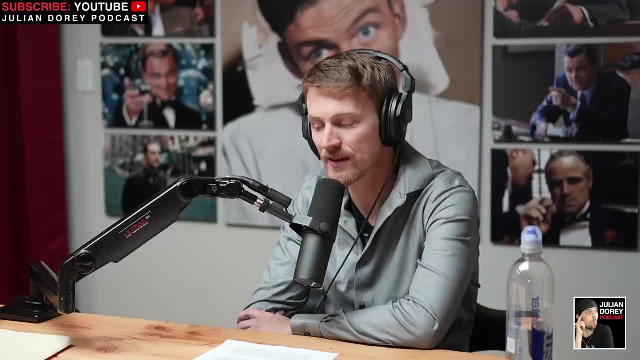 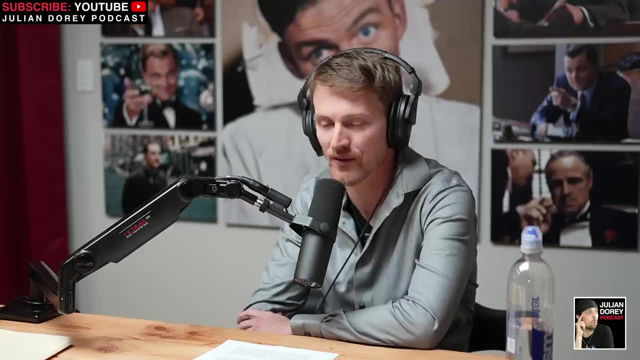 anunnaki uh in assyrian and akkadian, and they call them the sumerian deities and they call them the, and what that word translates to mean is those from above, those from heaven to earth came, or those from above to earth came, it just basically those that those who from were from this realm, or 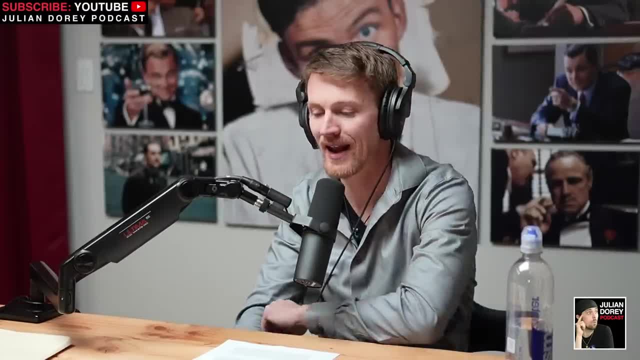 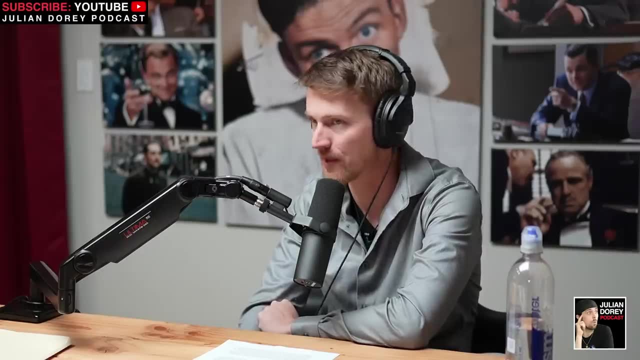 us came here, they stayed okay and i- i don't want to label that as what a lot of people will jump on right now- like some people be like, oh well, they come here to spaceship, are they like flying around space? and then they come to earth. i don't think this is that way at all now. 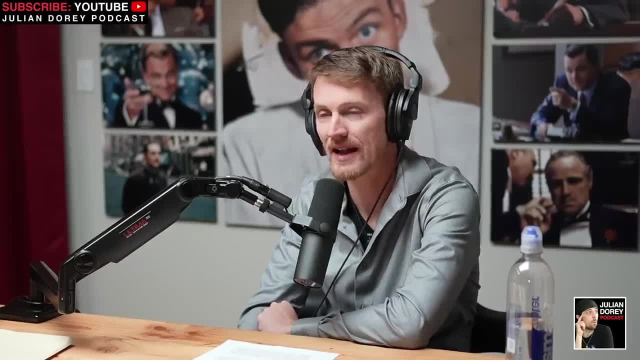 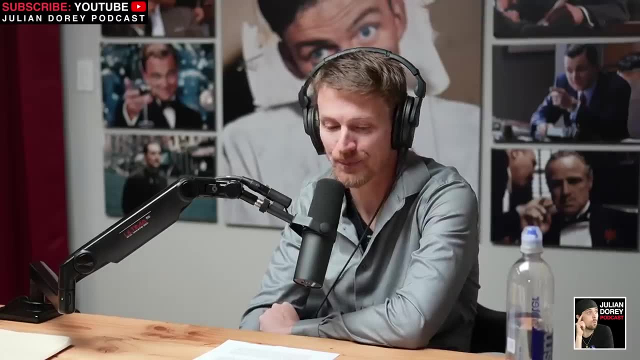 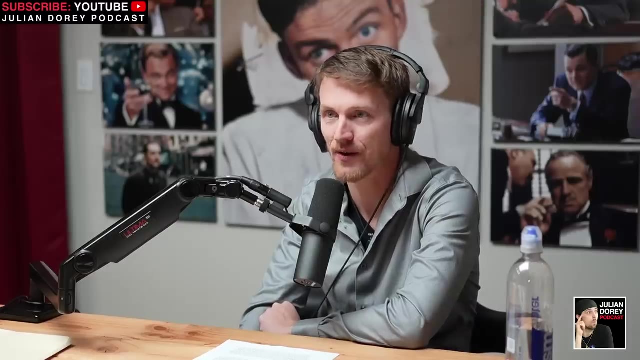 i am probably one of the only researchers that has that opinion. i fall, i fall in a bit of a crack. well, i fall in a bit of a crack because you either have you either have researchers who are like all in and like all their physical beings and all these like technical tools and they came here. 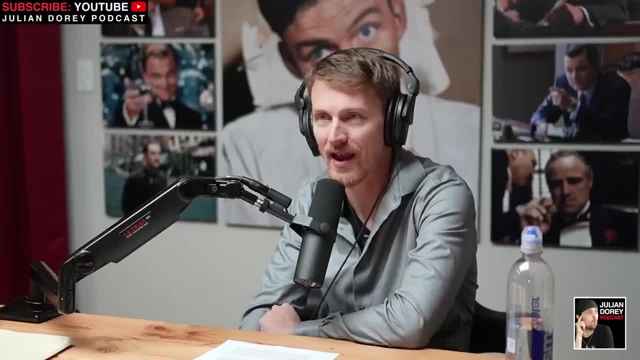 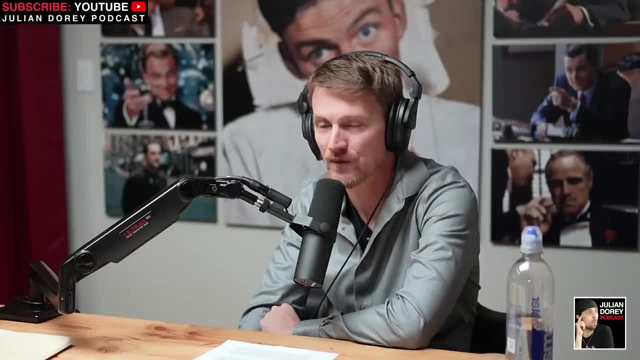 and like space suits and right people, people either go all in or you get academics so like well, they're not actually real, they're forces of nature and the planets and they're not actually anything tangible. so you get the idea of the universe and you get the idea of the universe. 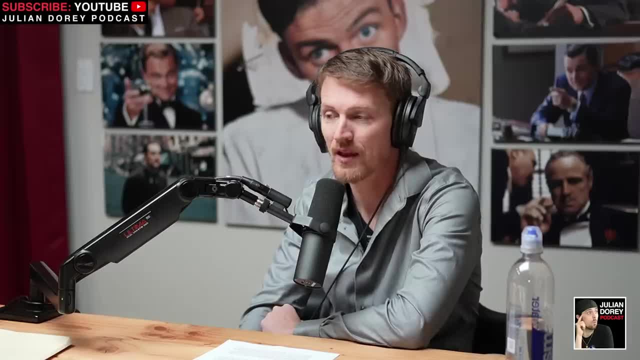 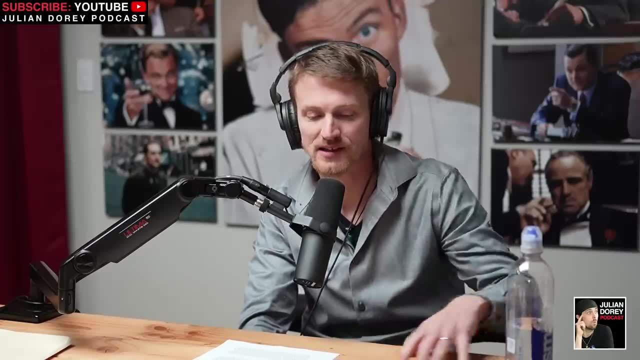 you get the extremes of both ends. okay, that's what you get. you get the extremes of both ends because it's interesting that if you learn about ancient sumerian and the gods that are associated in stories, you find out that there are two very distinctive things. there are the forces of nature. 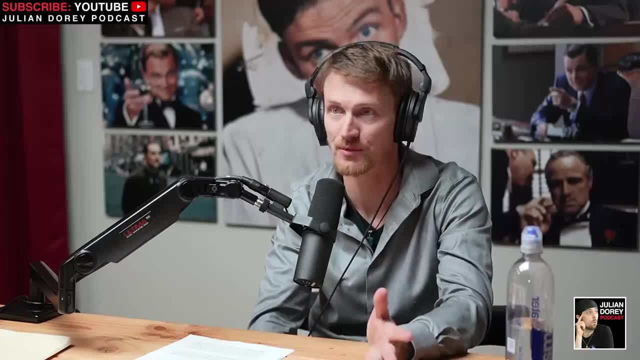 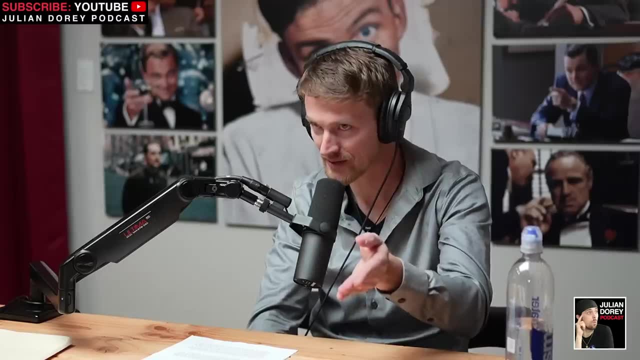 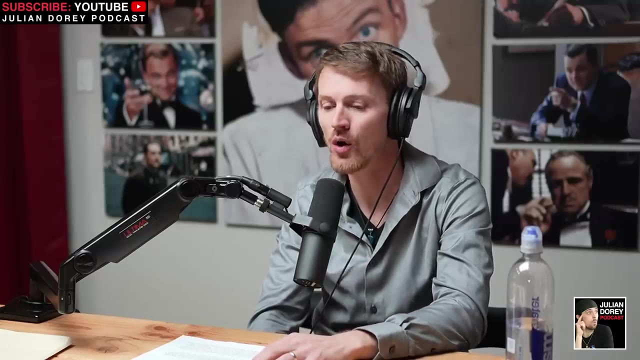 and they're represented by like things like fire and storms, right storm gods, and adad is one of them, right so, and. but they're depicted like beings, storms, forces of nature, and it's really easy to be like: oh, so, they're all that. oh, they're all just like. 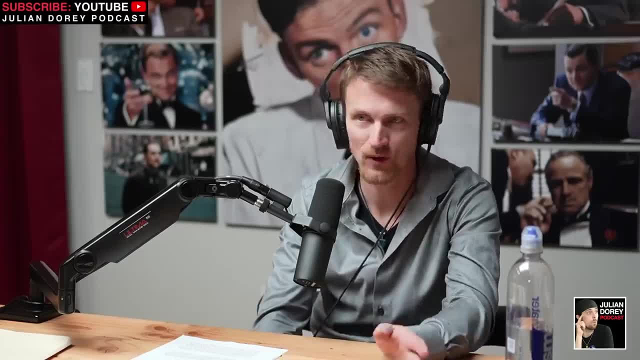 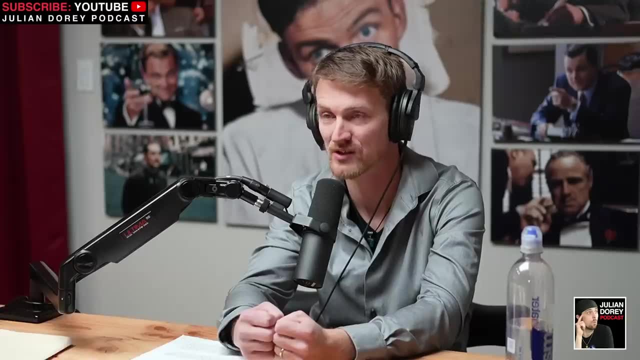 forces of nature and things like that, so that they're not real. but then you get this whole other problem, and this is where you get very few people like me that actually academically look at this in an open mind and study it, saying, well, there are forces of nature mentioned, but there's. 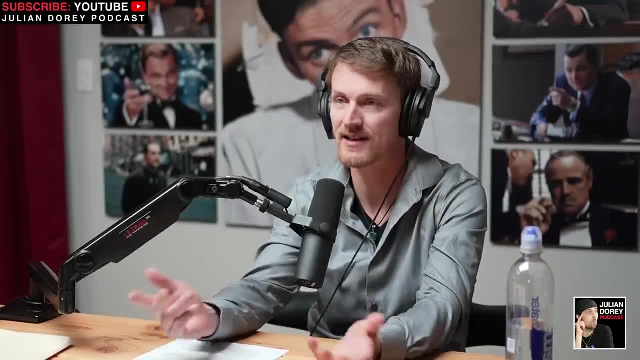 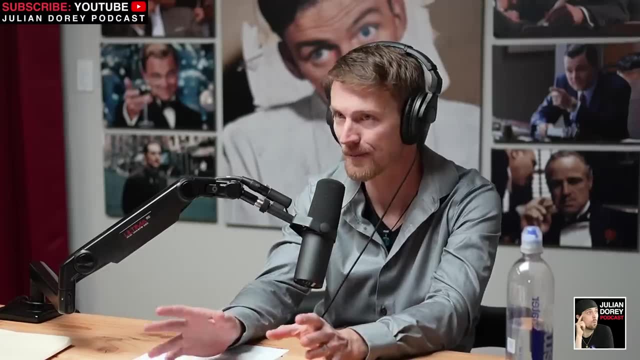 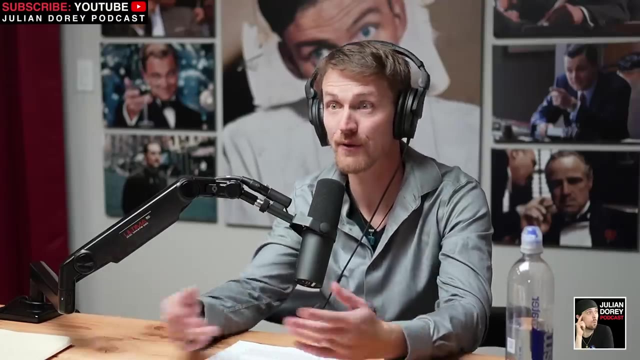 also ones that have complete conversations and have identities and have roles and do these physical things and have all these things happen here. so what's going on right now? well, in the ancient world, they believed that everything had consciousness: everything, the sun, um, you know the earth. they believe that the earth is a living being. they. 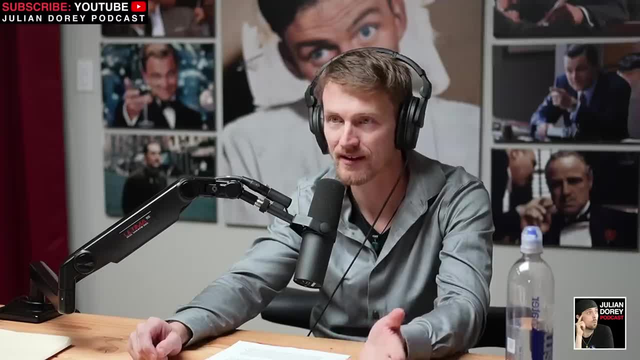 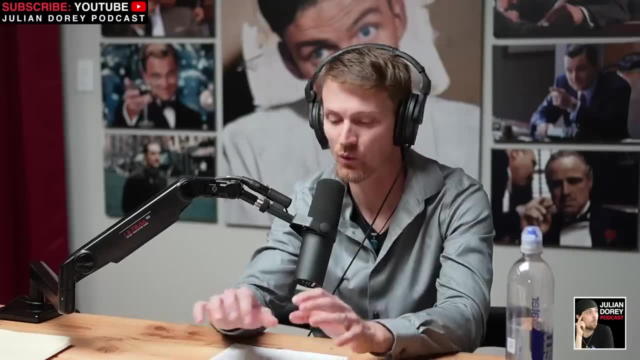 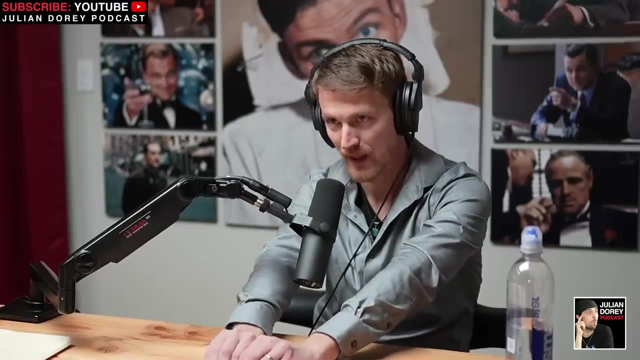 called it gaia. they called it um. there's different names. they call the key. ki was actually one of the original names for earth, believe it or not. ki who was calling it? this? the the original, like some of the oldest tablets we have, like the numa elish, um they. they talk about it like that, but they say, in this very mysterious way, where. 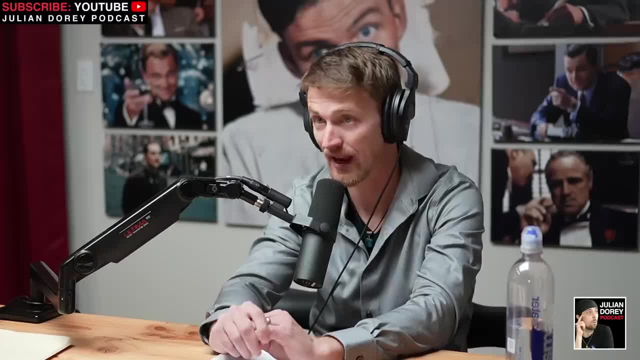 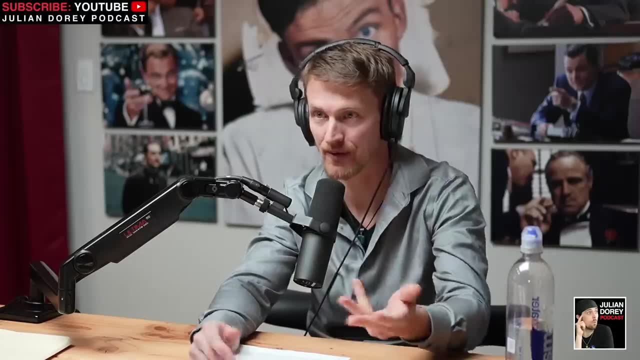 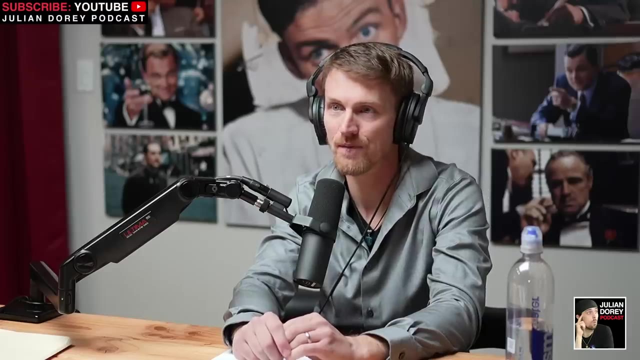 they talk about it in an ancient, ancient, ancient way where it's mysterious because it doesn't seem at all in even the time period of humanity. for instance, they talk about um like planets colliding and things, um astronomical things occurring that they're like part of, to like creating. 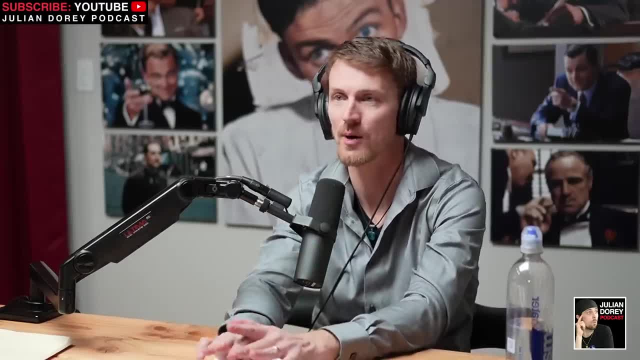 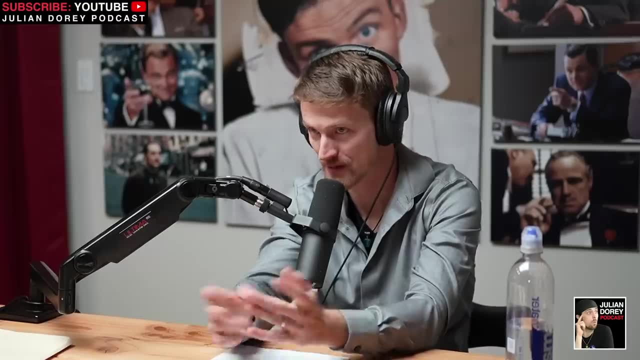 an environment that's like they have all these, they have all these terms they talk about, where they seem to be fighting against the natural elements to almost conquer them, is what it is, what it comes down as and it describes it as okay and it's very bizarre and i and i want to read. 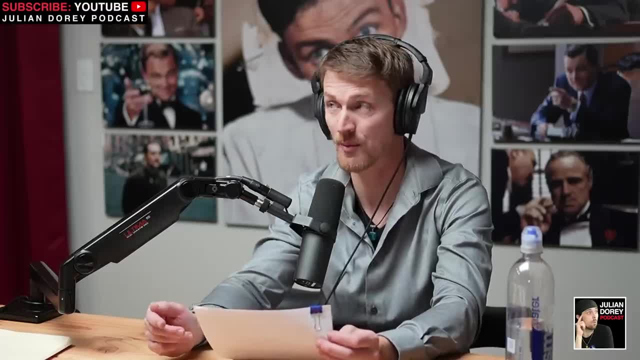 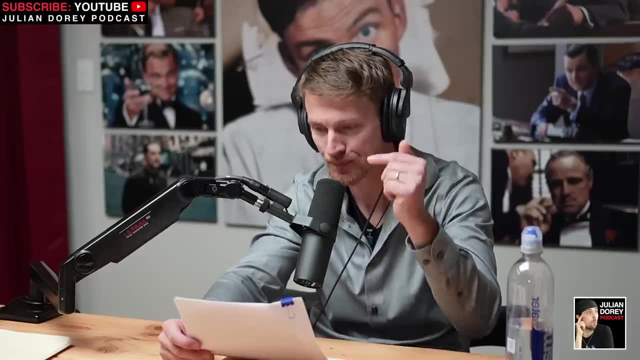 two little passages here before i discuss any more, so people don't think i'm totally crazy. okay, because this is. and again, this is what it's. it states. and now the myth of adapa that came from, translated in 1912, and it's a myth of adapa and it's a myth of adapa that came from the. 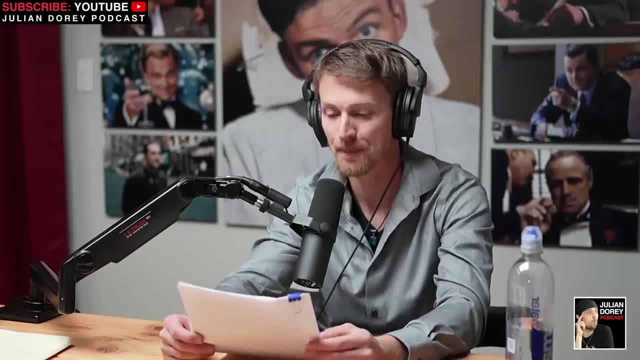 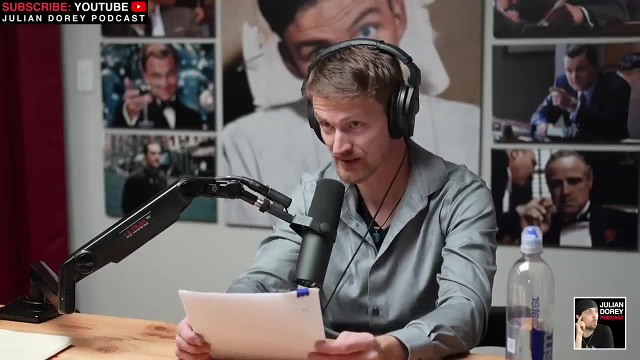 from rw rogers, who originally came out of the ashurbanipal library. i want to read this tiny little piece of the front because i think it's going to blow your mind and anyone listening to try me. are you ready for this? okay, it's called the myth of adapa. okay, now, adapa- a lot of people. 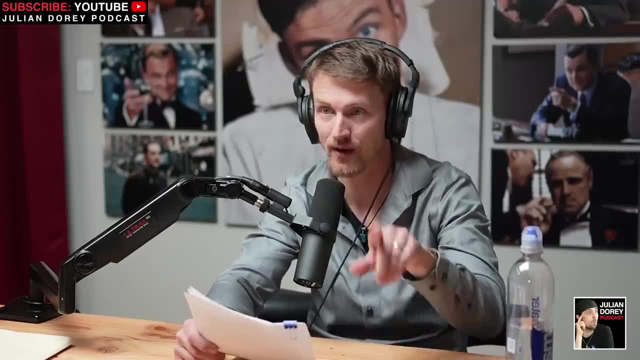 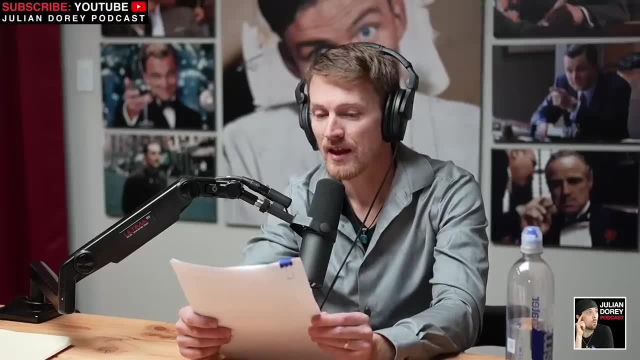 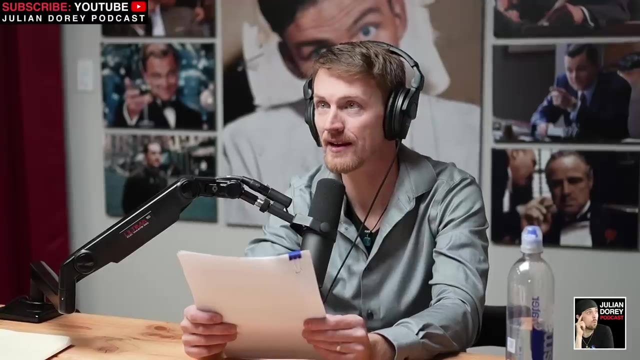 believe as well, including me, that adapa is the original name for adam. what? on what basis? listen you ready? okay, i'm reading direct quotes from the myth of adapa. this is tablet one. he possessed intelligence, his command, like the command of anu god, he ia who's who is a sumerian? 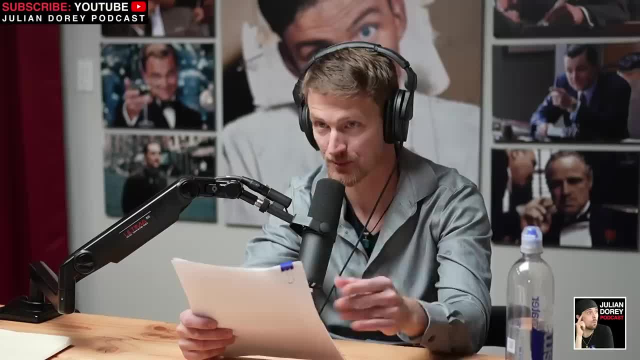 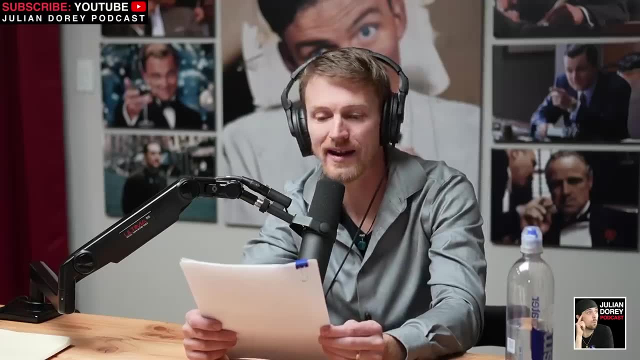 god named enki or ia, who's one of the patron sumerian gods. he's supposed to be the creator of humanity, of mankind. according to the tablets says he, ia, granted him a wide ear to reveal the destiny of the land. everything's cryptic. think about everything for a minute like a cryptic. 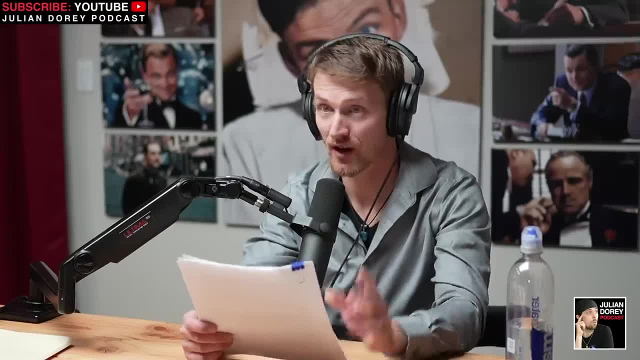 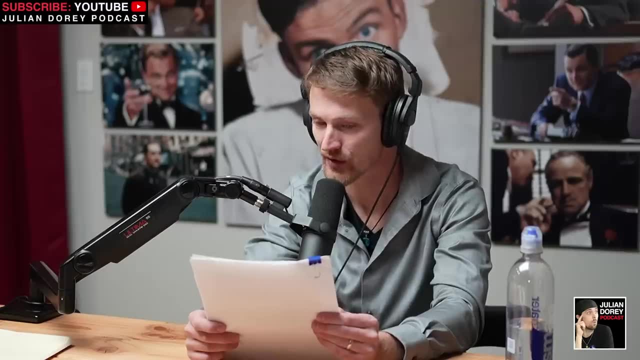 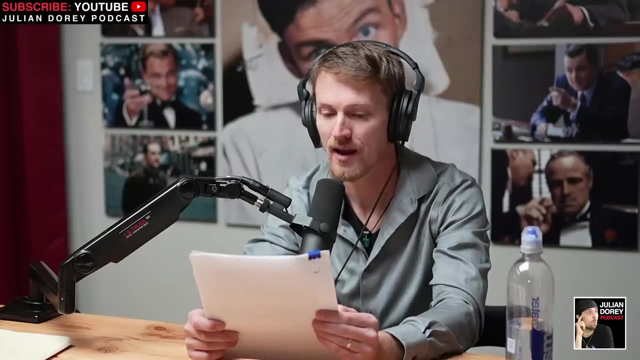 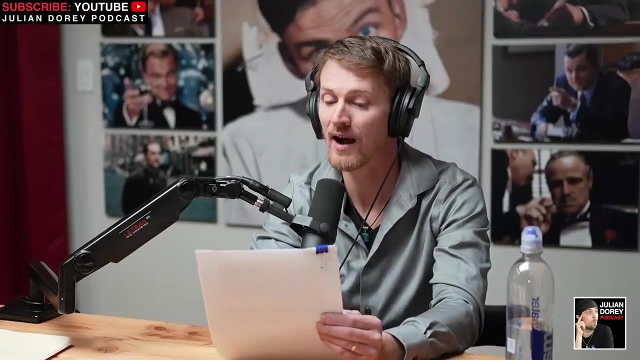 symbolic way. he granted him vision, adapa. he granted him vision, but he did not grant him eternal life. in those days, in those years, the wise man of eridu ia had created him as chief among men, a wise man whose command none shall oppose. the prudent, the most wise among the anunnaki, he was. 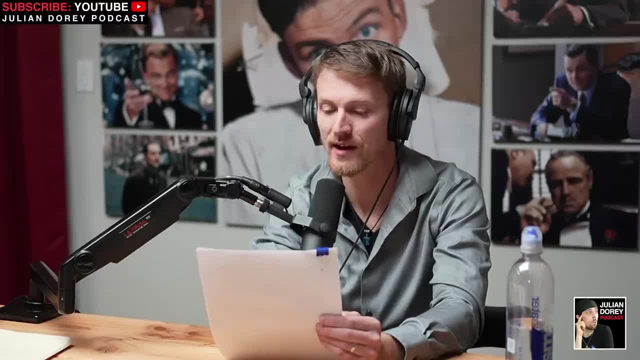 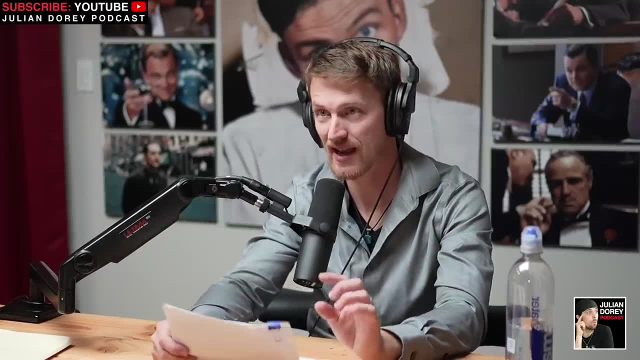 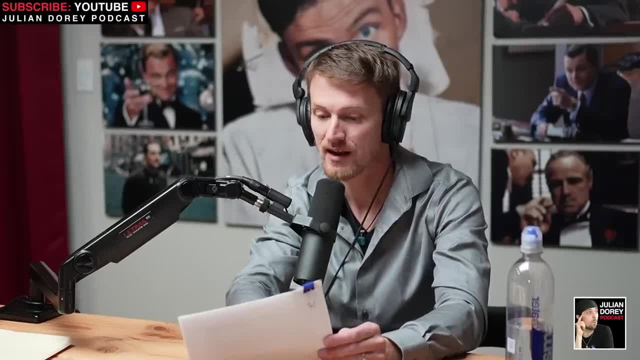 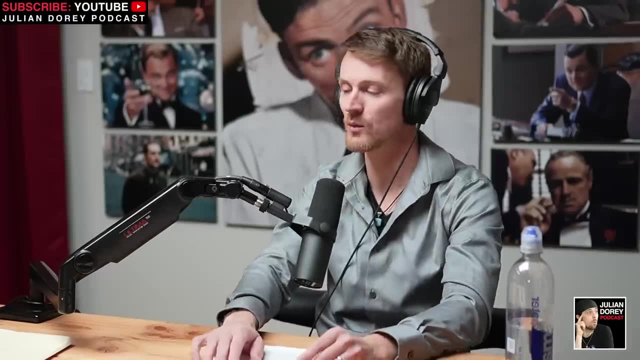 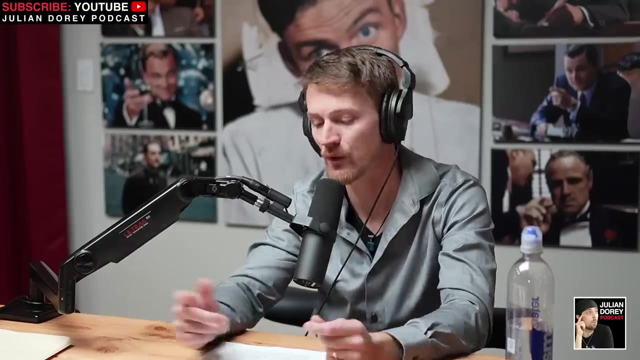 created perfect and that he was even more wise than the anunnaki. it says the prudent, the most wise among the anunnaki he was. so wait a minute, think about that for a second. it's saying that adapa, who's a human, is great. he's considered a great sage. if you read other tablets, it talks. 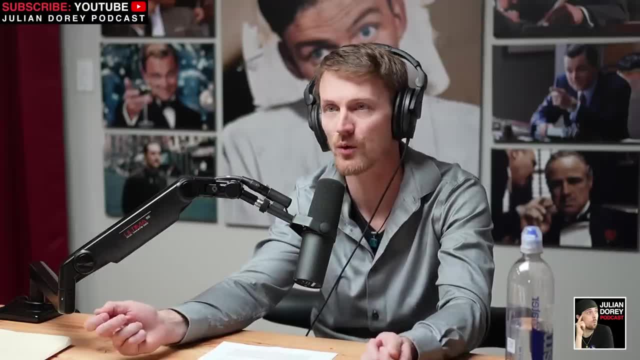 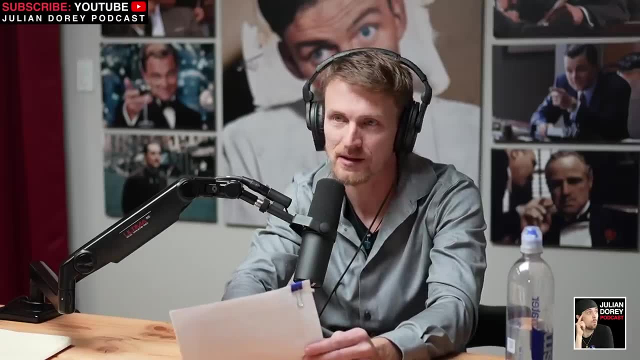 about how he's considered a sage who was part of the up college and he's considered a sage who was, who traveled around the world to teach. okay, that's what he was. he wasn't a king, he was a sage. and it says here that he's the most wise among the anunnaki. wait a minute. so he's an anunnaki. 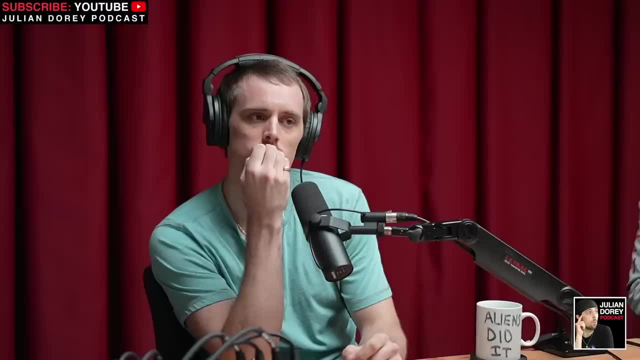 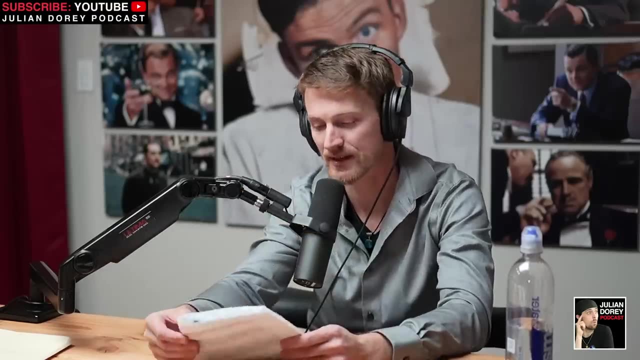 so what does that make us? it starts to unveil layers. to try to understand this now let me read one more little piece to to even expand this further. this comes from the legend of atana, which is another set of tablets after the flood, when they re-lowered kingship again during the 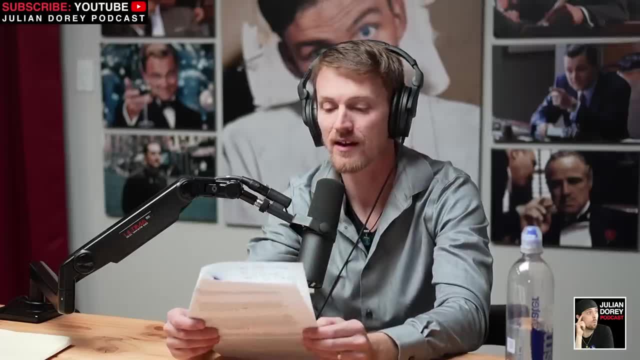 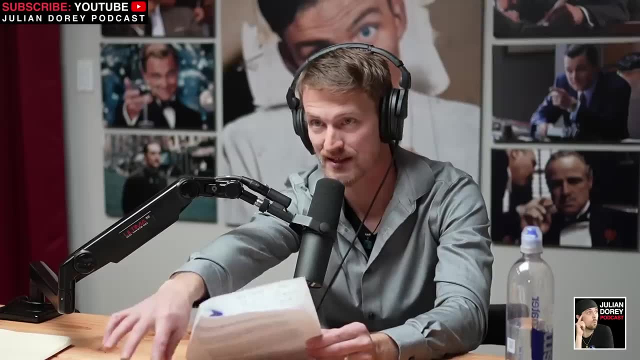 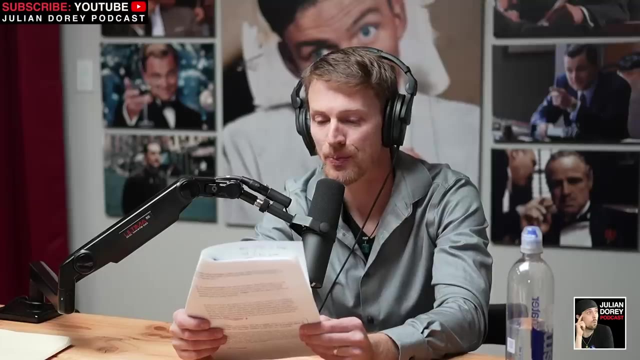 same time as the iraq civilization, i believe it says here. they planned a city. the gods laid its foundations. they planned the city of kish, the first city after this deluge in iraq. same time period though, okay, the ajiji founded its brickwork. let him atana, be the people's shepherd. 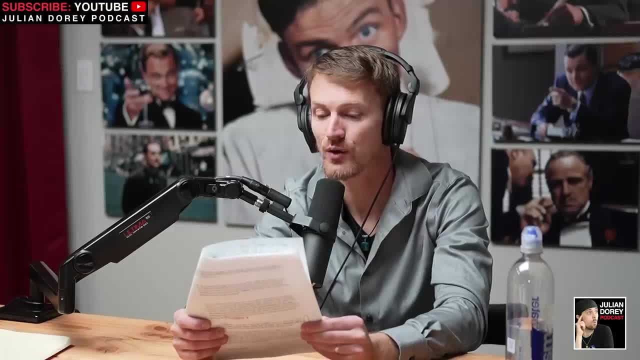 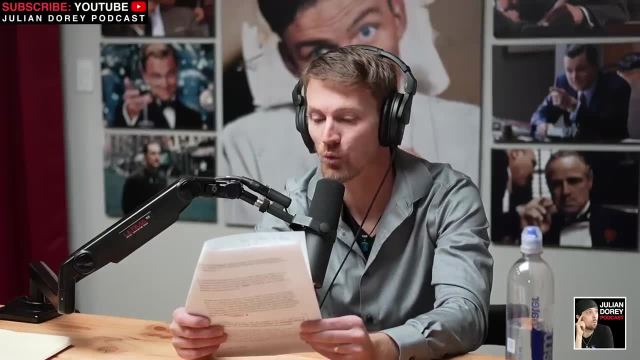 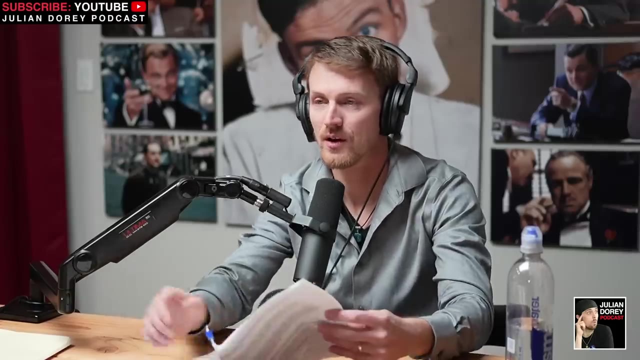 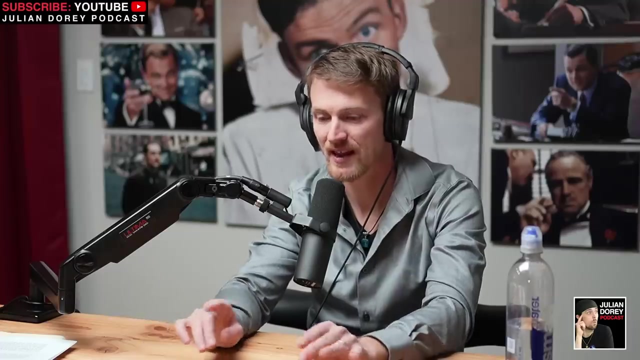 let atana be their architect. the great anuna, gods, ordainers of destinies, sat taking their counsel concerning the land, the creators of the four world regions, establishers of all physical form. so those are two completely different tablets that discuss the anunnaki in mysterious ways. 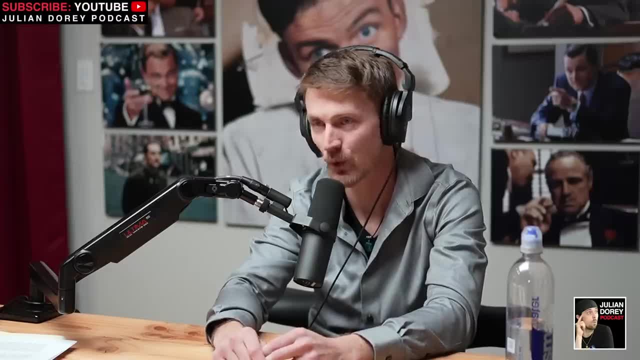 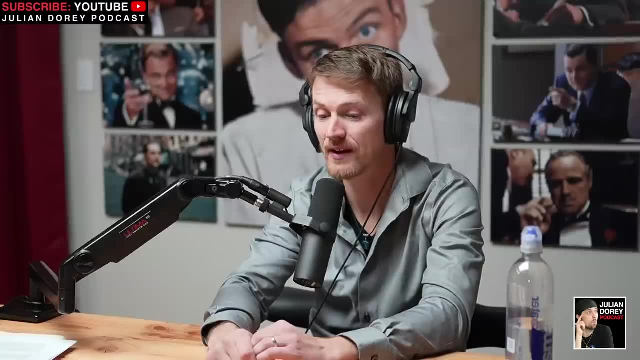 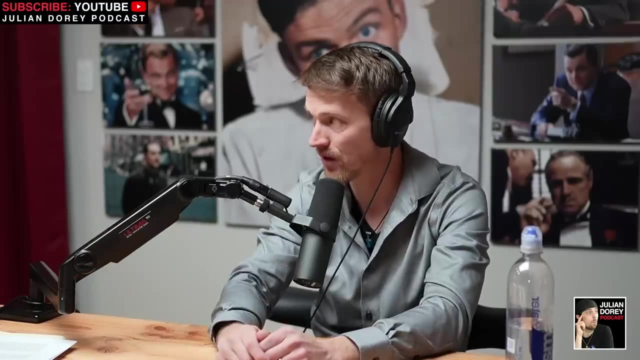 and also that we are basically them. so what does that mean? for a minute right? do we have any archaeological evidence of anunnaki? we have more than you could ever imagine. i mean literally, of right, the, the, the ashurbanipal mural of none of us, i don't know. 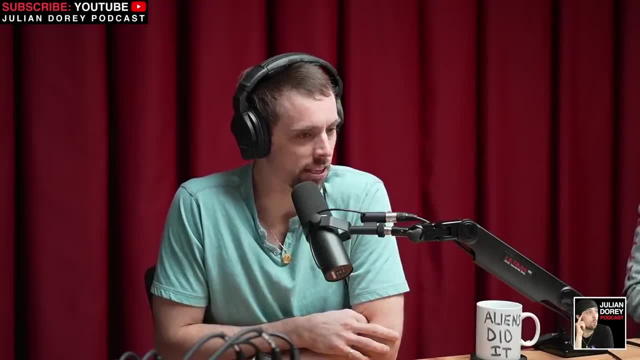 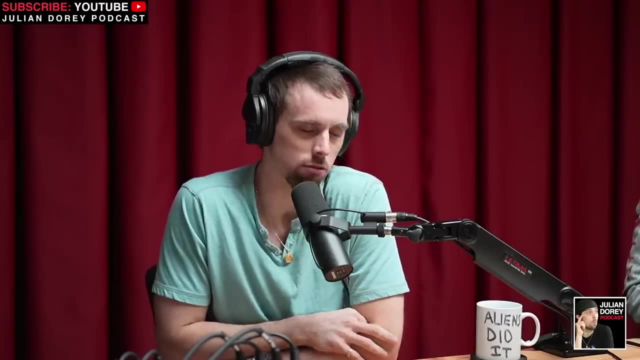 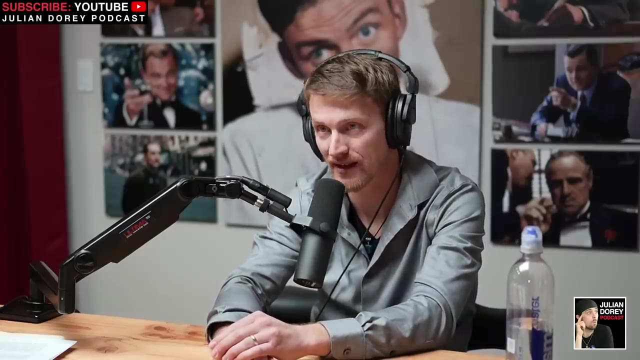 is there any? are there any weird remains found that could point to them being anunnaki remains, for example? well, human remains don't last very long. first of all, and secondly, they were looking in the wrong place. i think this is scary. this is a sad 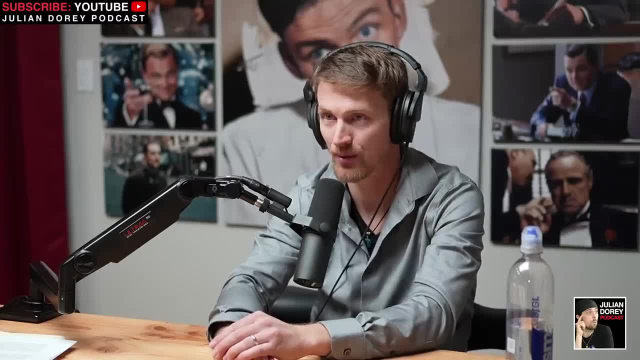 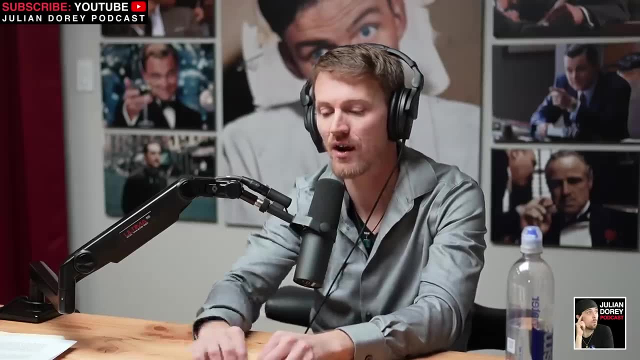 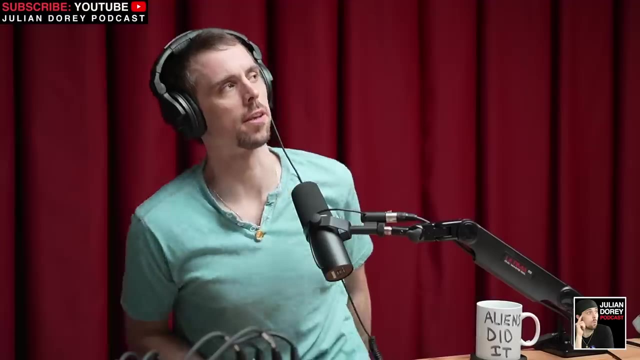 we need to look at the ancient lineages of some of these kings and why they lived for so long, it rules for so long and why so many mysterious people like matthews, chakra, book of enoch and an uh enough himself there. he just constantly describe it as them living like six, seven, eight, hundred years. 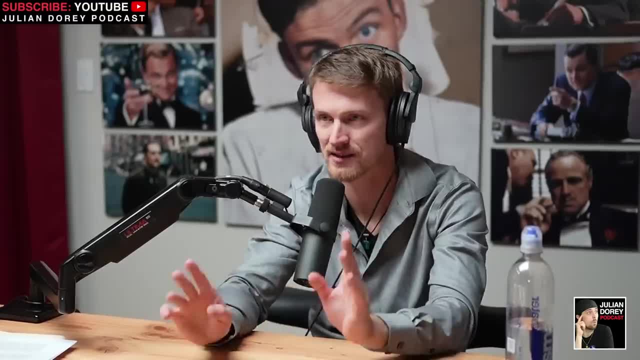 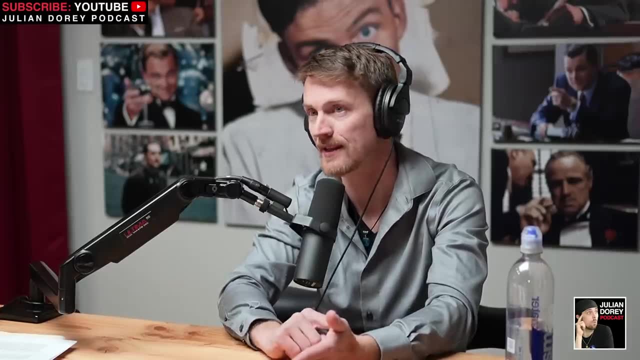 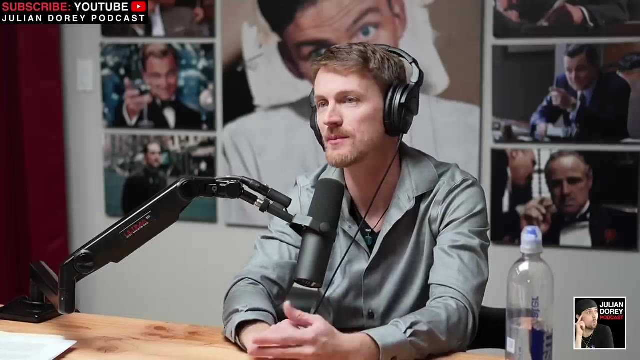 or more. that can end so many different places. it not cannot. not just like this smerian stuff, right, babylonian text, egyptian. it echoes this concept that we used to be something that were different now. we used to be taller, we used to live a lot longer, we used to have connections that we don't. 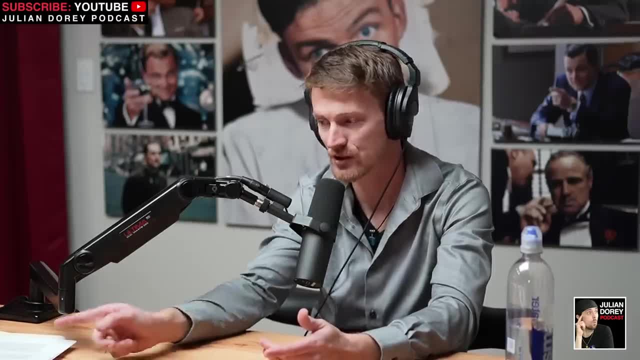 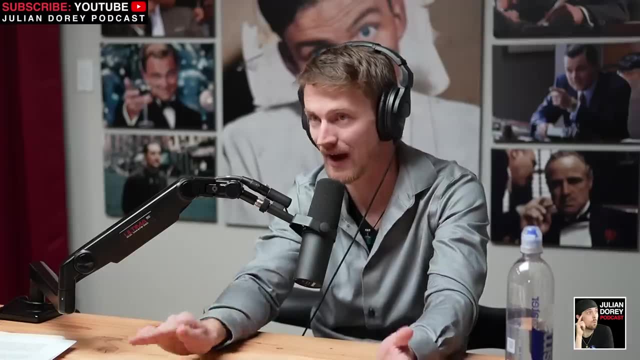 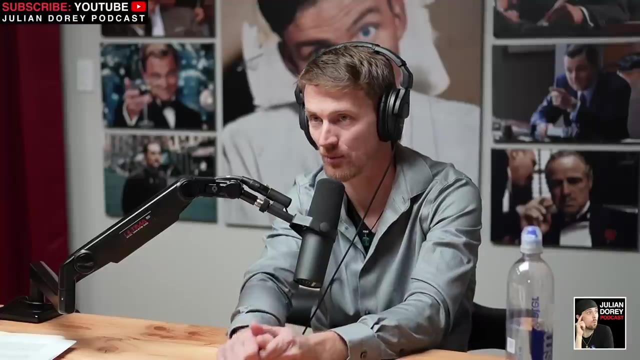 seem to have any longer, and that's, i think, the whole point of the stories i read you: the flood on how the noah figure was preserving some kind of a seed of mankind, because i think it's what divided us from being more animal-like. so, if we think of what means to be homo sapien sapien, 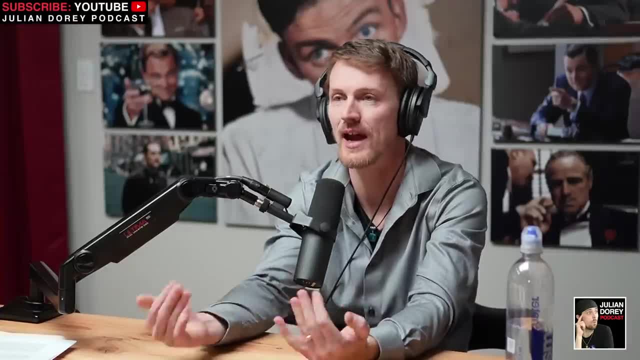 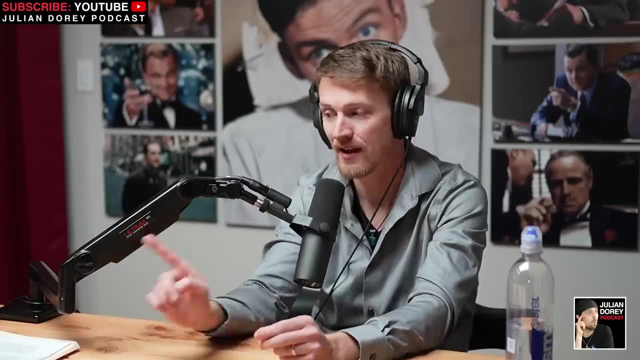 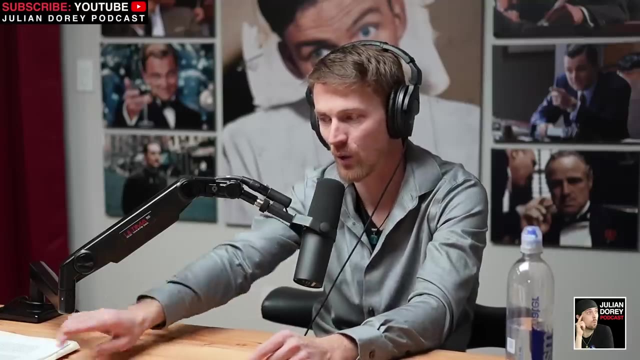 and these, this, these connections we have and who we are. i it it has come to the attention of a lot of people and it's the possibility that that bloodline is what disseminated to create the gifts in what we are today, but what it gets back to what we originally read, because it says that 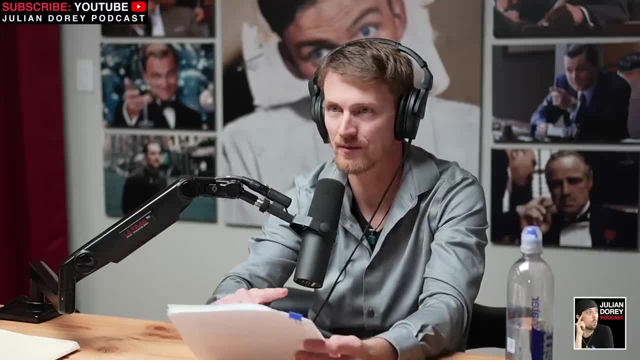 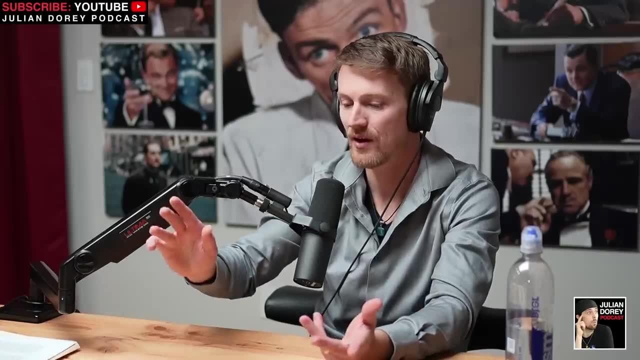 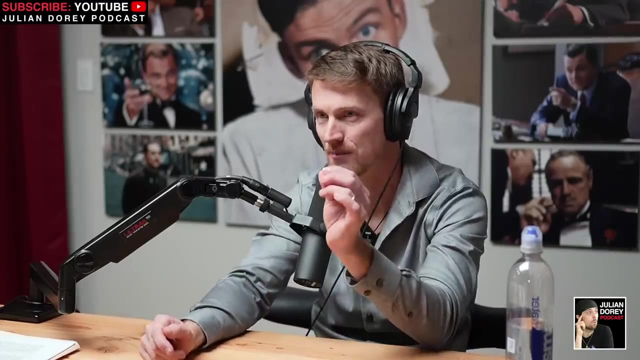 adopt was the wisest among the anunnaki, which means that we are the anunnaki, and what? what's interesting about that, though, is that we are mysterious and we have all these gifts and we're powerful, but we, it seems like we don't remember any of it, and we have only bits and pieces, like if i'm gonna. 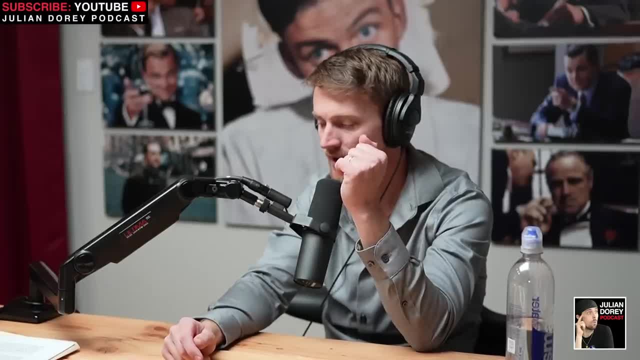 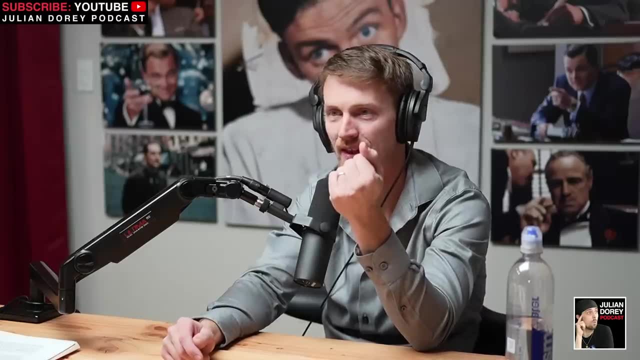 go give an example. this is really easy. everybody knows this. if i'm gonna go call you and i pick up the phone, i'm like god, i gotta call julian door. i gotta set up another podcast, right. and i'm like about to call and i put the intention out there: i'm gonna call julian. but you're really gonna do it. you can't. 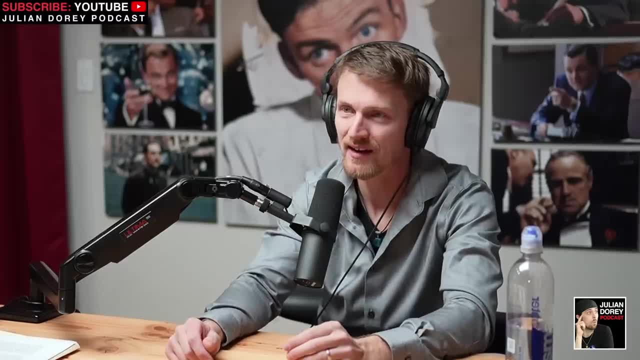 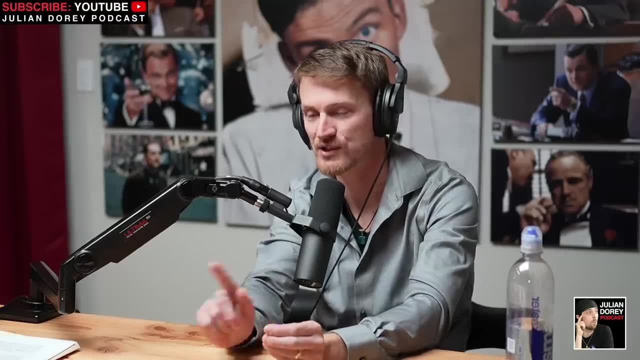 play with it. this is how it works. you can't be like i might do that. if you set your intention on something like i'm gonna do this and you pick up the phone, you're gonna do it a lot of times. the person on the other end- and i know this happens to a lot of people- they'll be like whoa. 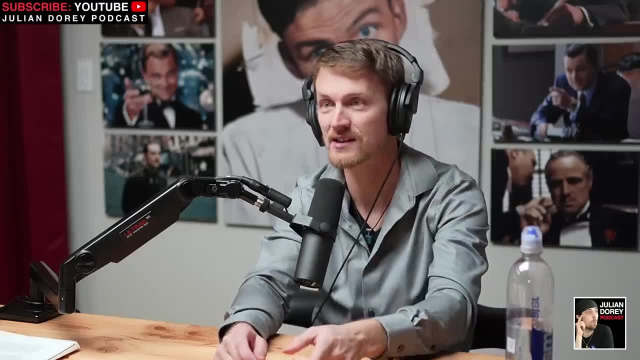 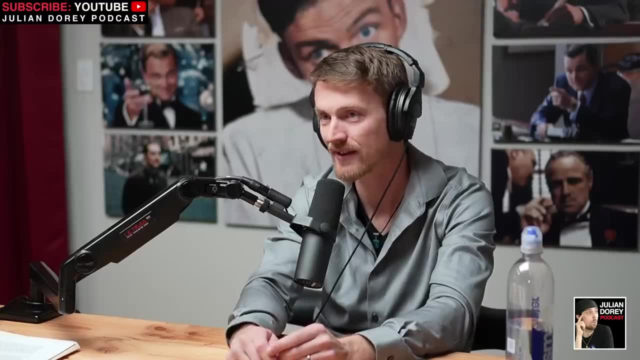 why did i just get a thought of julian dory in my head. and then the phone rings and then it's you calling, or me calling, vice versa, right, yeah, the weird subliminal messaging. what are you doing there? what's happening there? break that down for me. 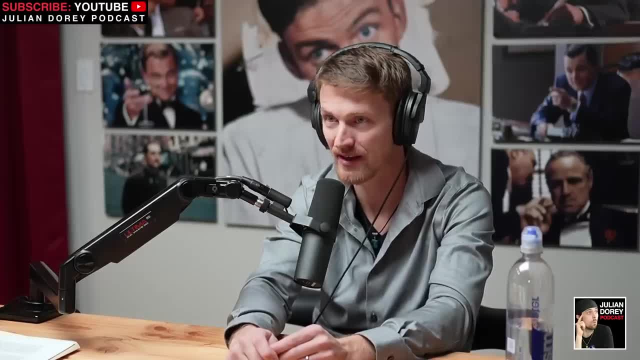 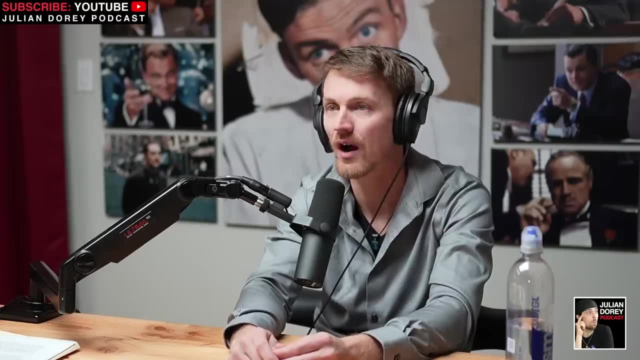 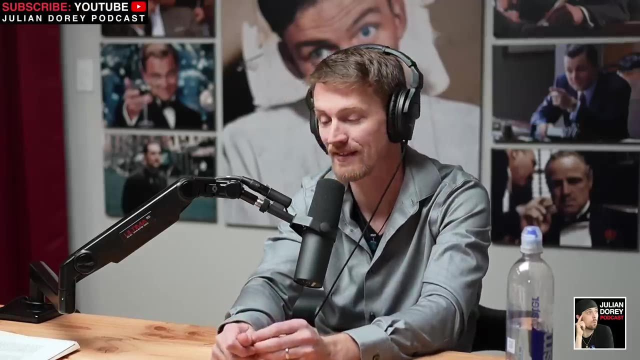 about that a lot. it's because we have telekinesis, we have gifts within our mind and energy, we within our consciousness, that are not fully unlocked and understood. it's like we forgot all those things and then we're trying to remember them and unlock them again, like 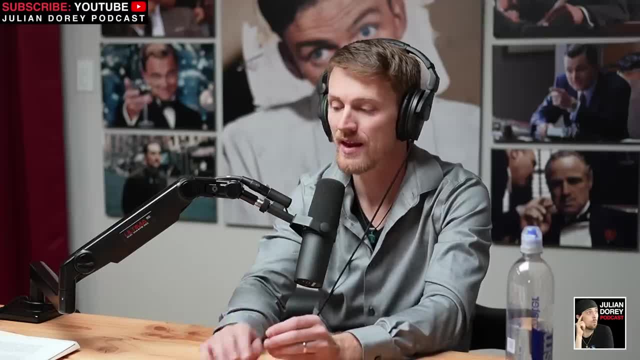 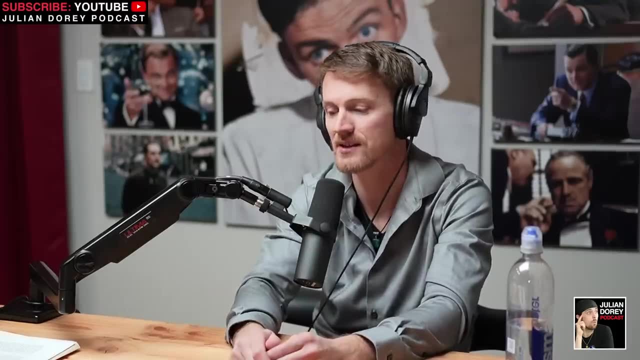 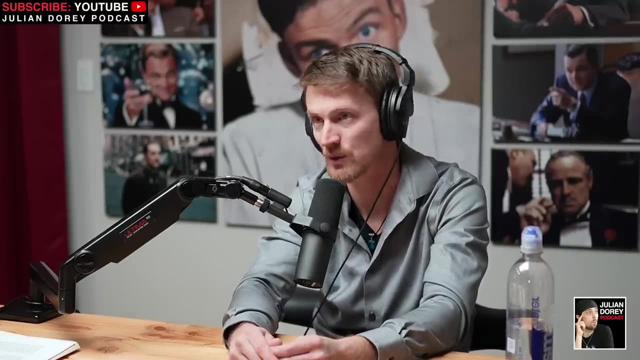 they're dormant within us. all right, bring this back to anunnaki now. well, we seem to have had all these divine gifts and and we were the certain type of individual- and it's discussed how it was- some, some texts like the book of enoch, consider like the nephilim, like the cross between them, and 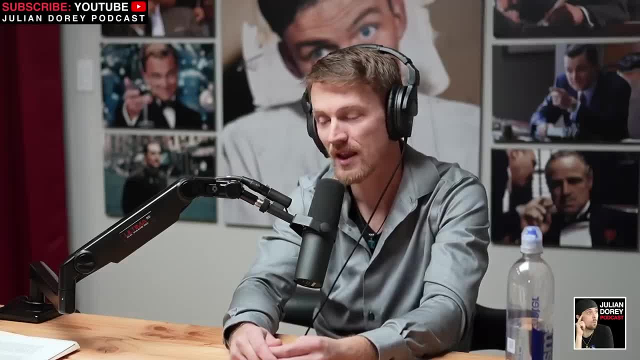 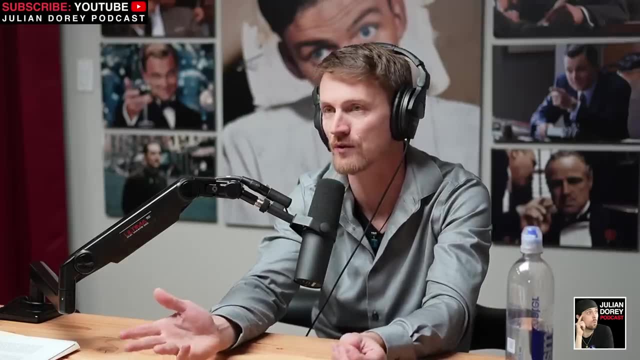 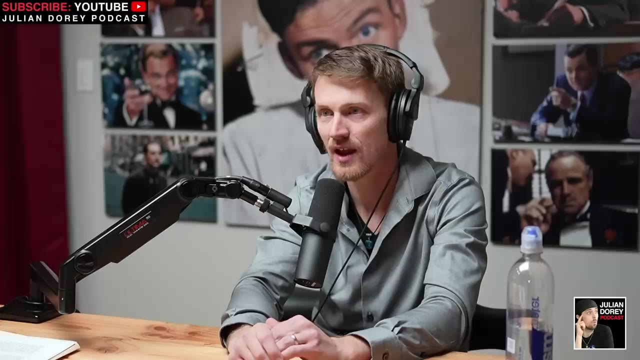 giants. they call them like an abomination. it gets into this concept and idea that we were created based on, like the noxic texts, like the nakamadi scriptures, if you want to reset the secret book of john. it describes how this creator, being in there is, is jealous of us and uh discusses how it. 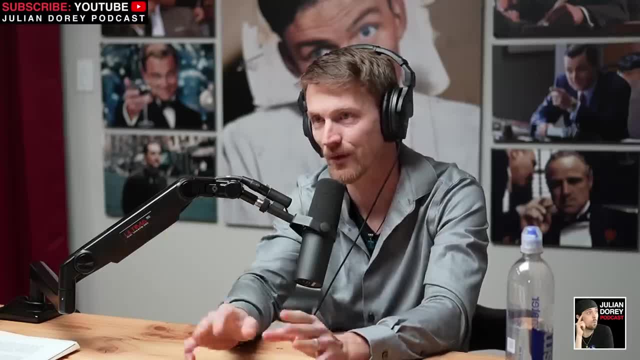 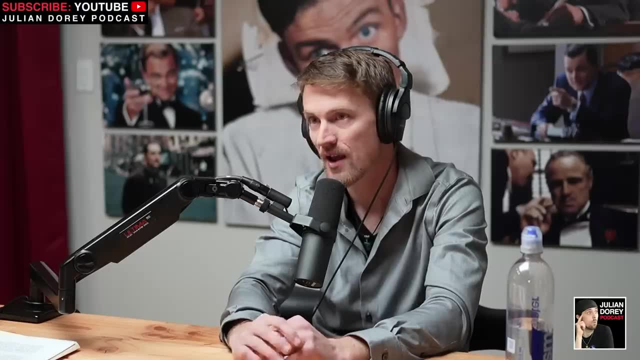 it wants to throw us his powerful being, which i think is one of the anuna he wants to throw us into like the. it says the lowest form of matter as like a punishment for us. um, because there's a jealousy in inherently in who we are. but go back to that. i just read: 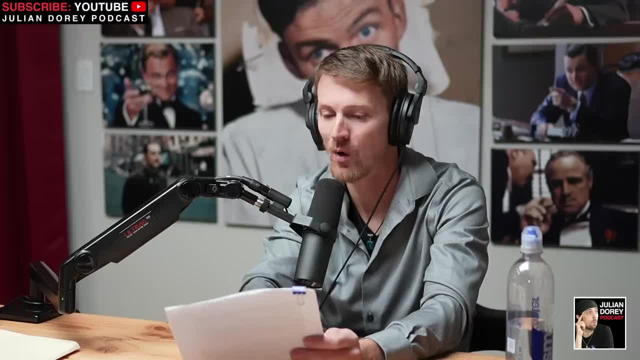 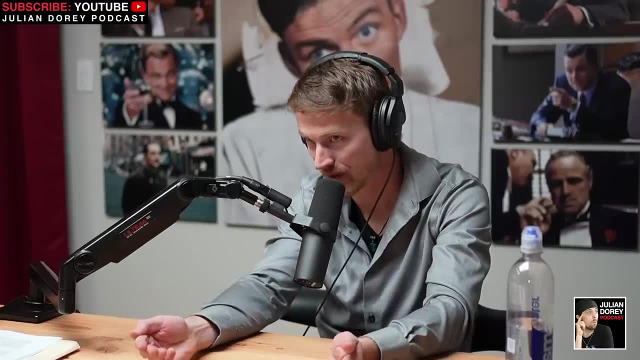 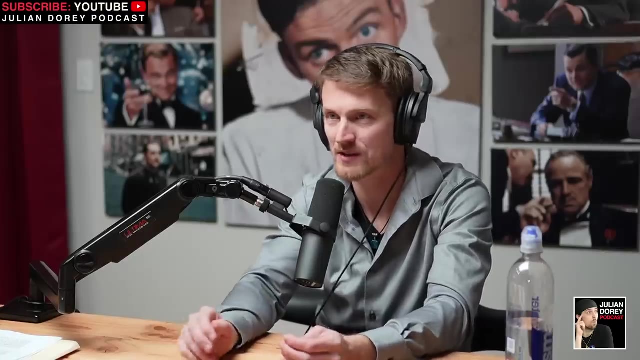 remember i just said, a wise man, the prudent, the most wise among the anunnaki he was. what that means is that we were created to potentially be greater than them. i think we are them. i think there's even a possibility they're somehow related to us in the future and we're not. 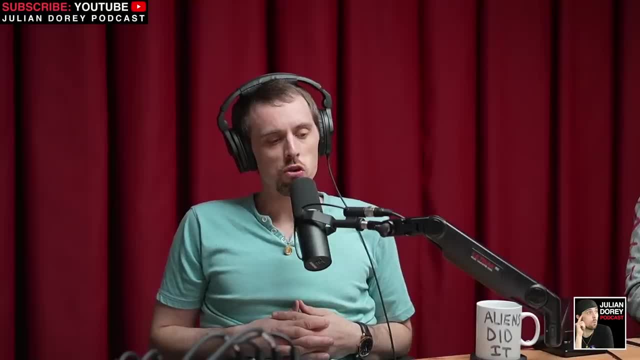 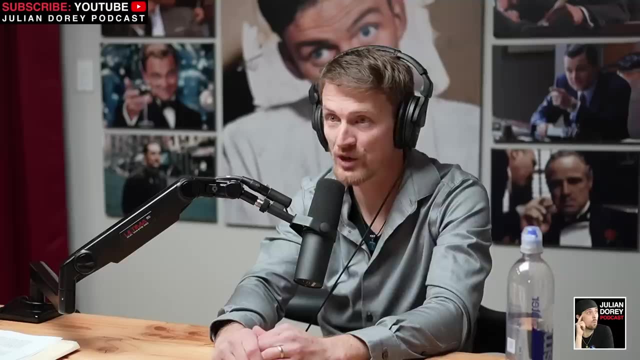 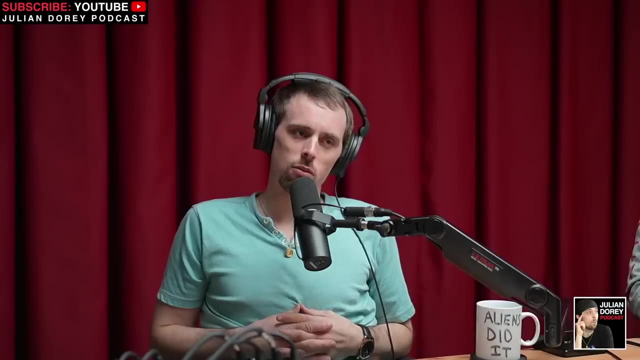 future. but you're saying adapa is human, but more the connotation there is that he's more perfect than the anunnaki, which is where the jealousy came in originally, because it's saying that we were created, which is the adam and eve story, which would mean they're human though too. no, we mean which. 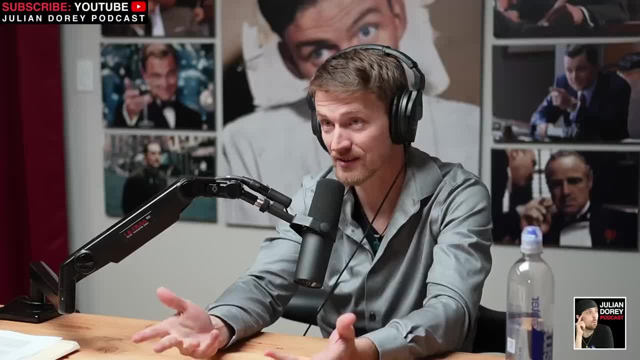 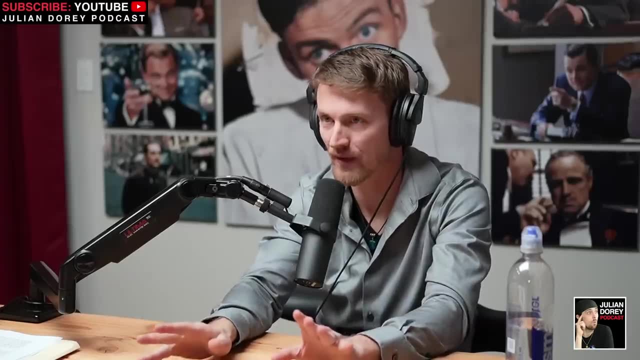 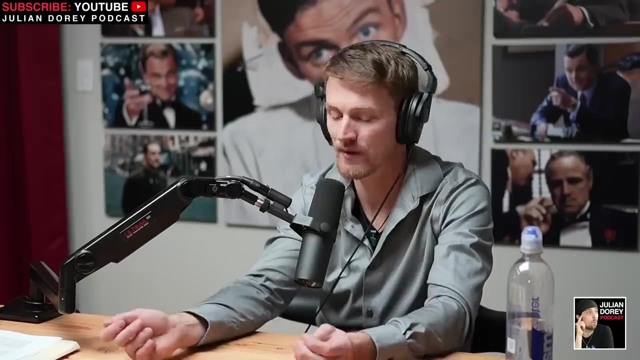 means we're them. yes, right, yes, exactly yes, but i don't. so there's no separate. that's what i was trying to get. so what are they? let's get, let's get down to the core of what they are. then, okay, i think they're us, but like a million times more advanced, i don't what you like. for instance, let me give an. 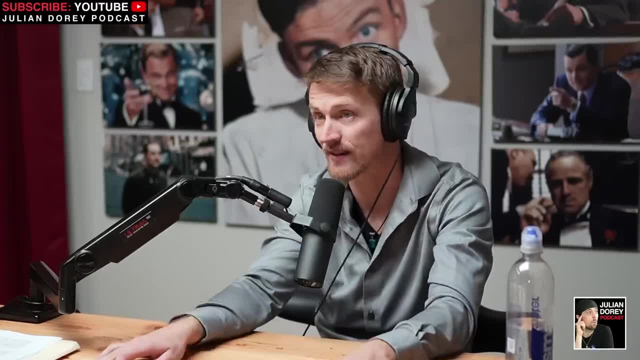 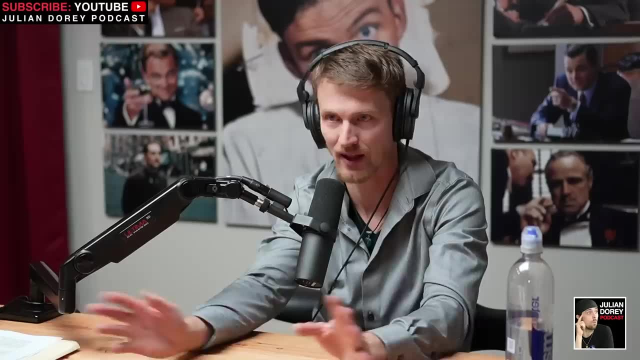 example, george smith, the greatest translator in history, that literally cracked the sumerian code. he wrote a book called the chaldean account of genesis and in that book he summarized his entire life study. it's literally his life's work and he- and at the end of the book he has a conclusion- 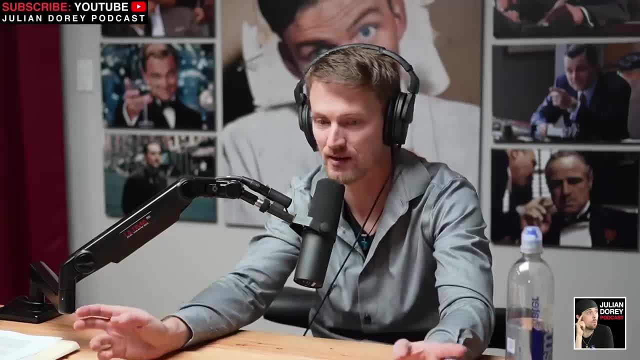 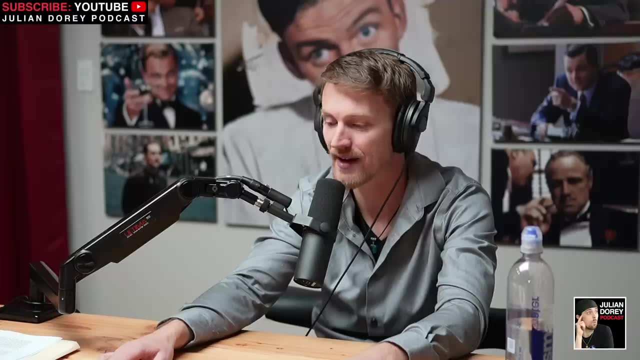 where he summarizes as someone who's read more tablets and studied more than anyone else in the world, and he summarizes on his thoughts about the anunnaki. it's really wild, actually, at a time when academics would never even touch it or talk about it, and this is the 1800s. maybe that's why he was able to do it. 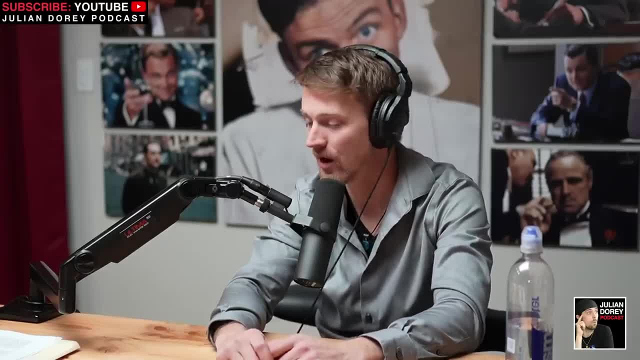 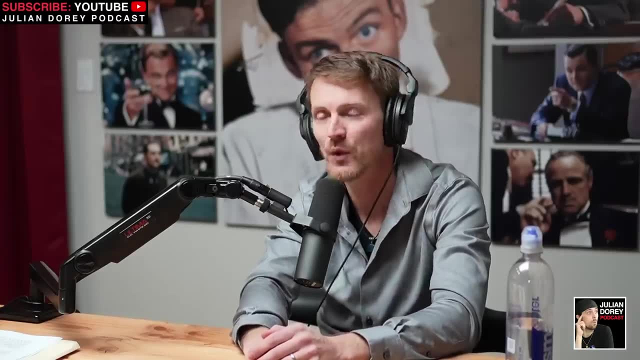 i'd encourage anyone to read the very end of the chaldean account of genesis- and i've saved and highlighted all my in my book. but- and i read it all the time- but he basically says that the only thing that makes sense to him about the anunnaki is that they come back backwards. he says this: 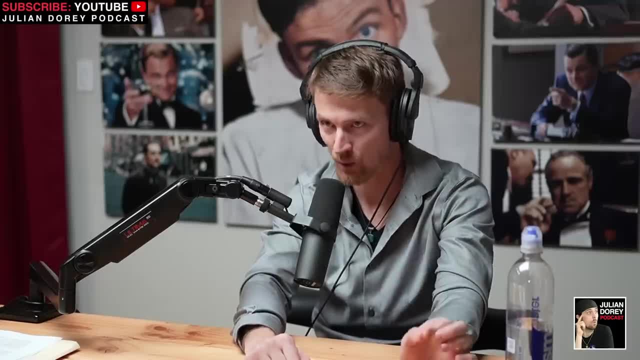 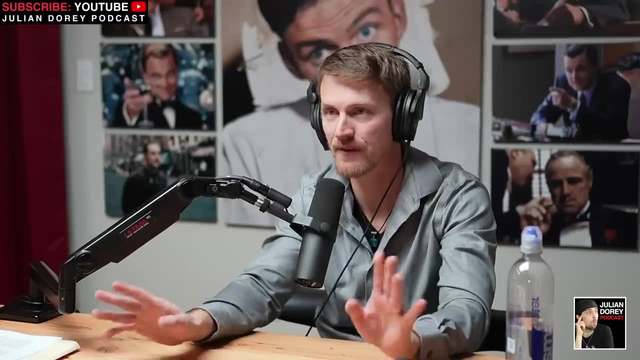 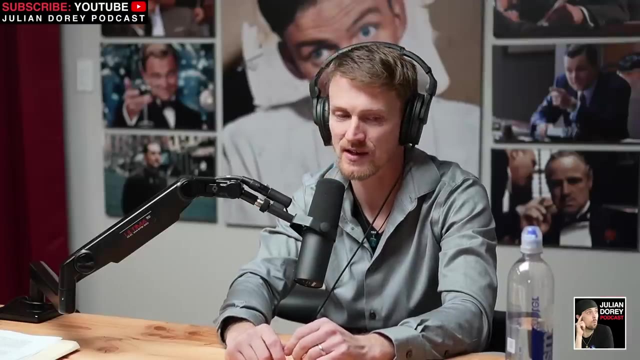 exactly. he says they seem to come backwards and forwards in time in our, in our, in in earth's time for specific reasons. what did he mean by that? that's all he says. and he goes on to say that he doesn't necessarily believe the king's list. 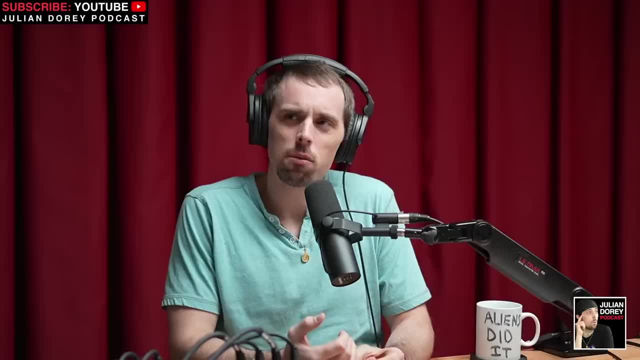 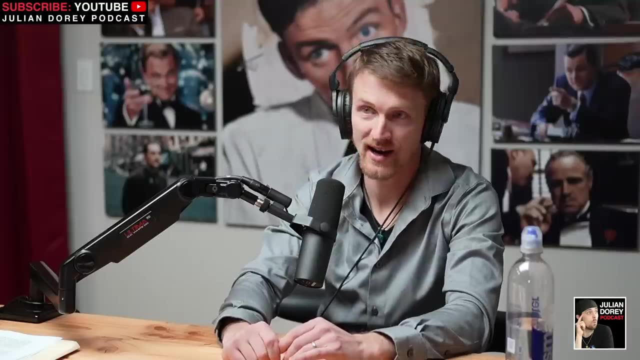 because they're too long and it's like beyond our comprehension to add it up backwards and forwards, unless they were time traversing the multi. yeah, yes, okay, so now we're getting into where i really think we need to go, because we need to stop thinking about what like alien ships and 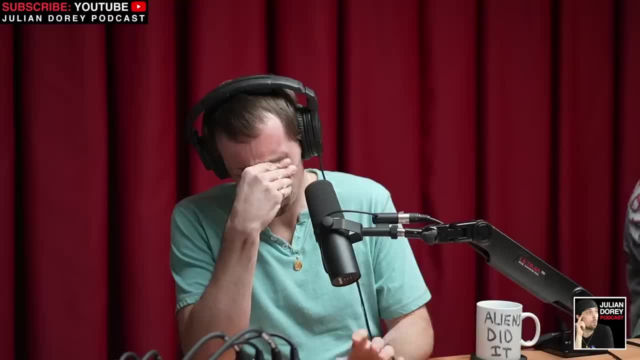 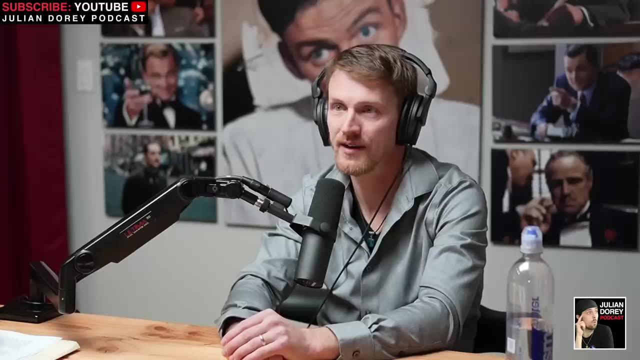 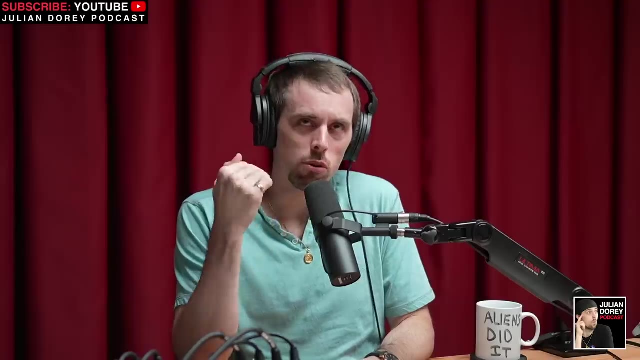 gray aliens and stuff. let's stop doing that. let's, yeah, but yeah, but hold on back up, okay. this and time travel is all a hypothetical. i know radical physics, i know that, right, yeah, i know. but when i listen to some of the greats who look at this, i i try to relate their concepts. 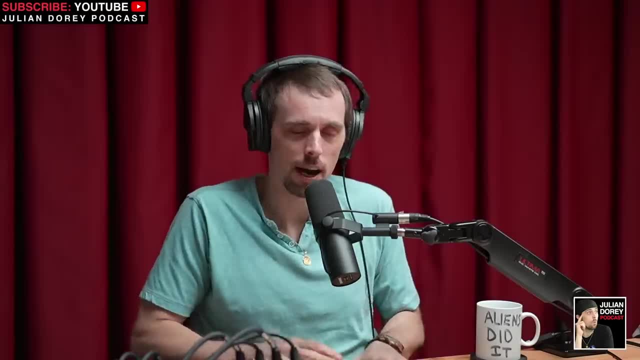 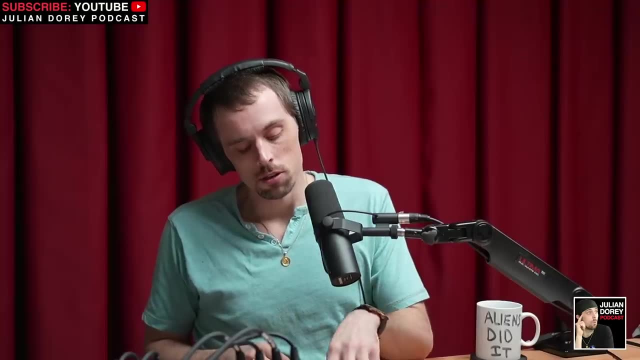 and make sure that i'm going off of some of that, because i'm not a physicist, so like i'm not, let's use a guy. we both like michu kaku. i love michu. michu talks about like the rivers of time, right, so meaning the best example. i've used this a ton. 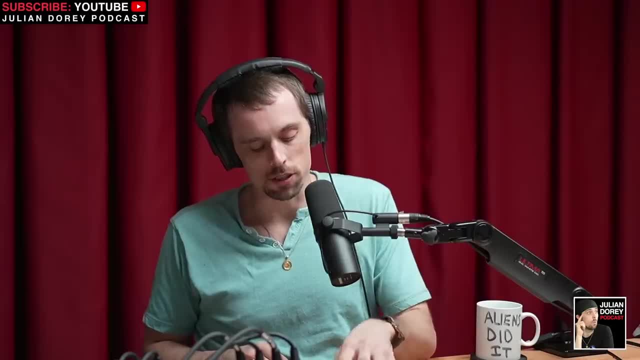 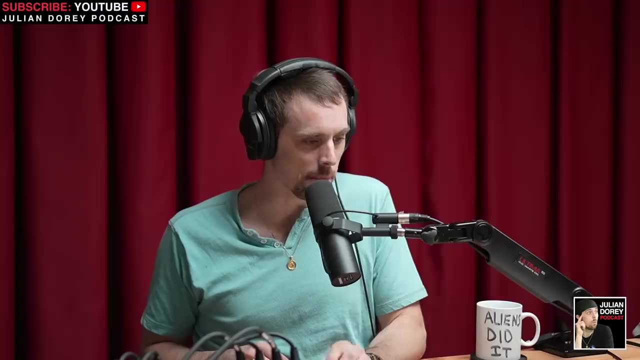 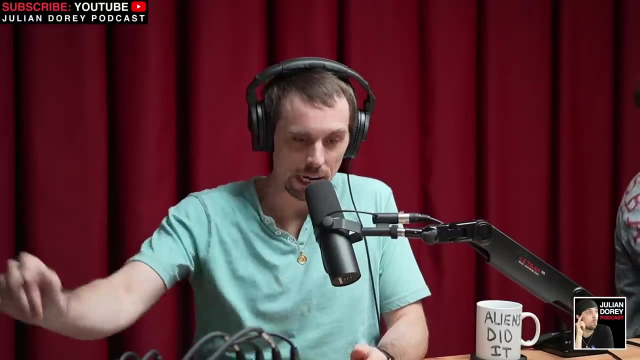 on the podcast, so apologies for repeating, but he says, for example, if you went back to april 19 or 1865 to try to stop the assassination of lincoln and you stopped john wilkes booth from doing it, you are not changing the multiverse reality that you came from, you are creating another. yes, that. 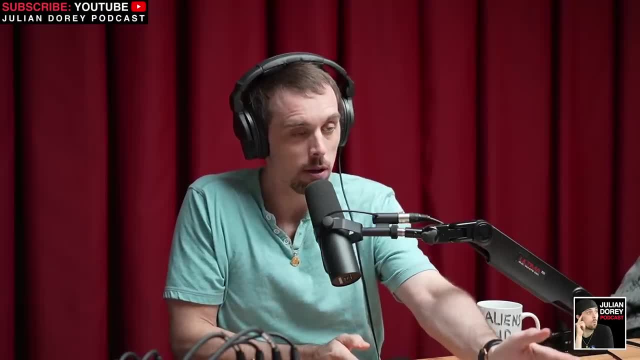 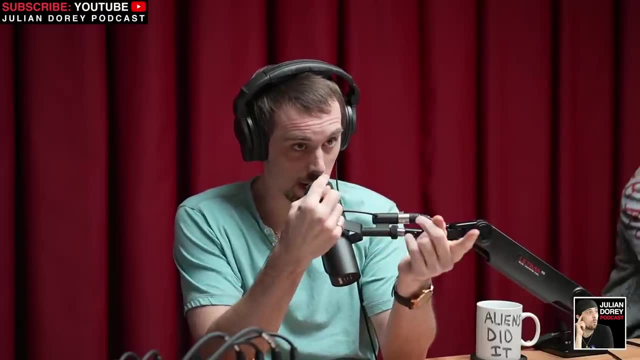 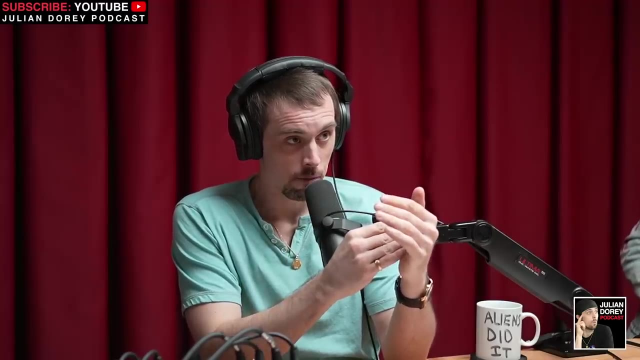 is, that is, a, an actuary from that river, if you will. right for a different reality. so when we talk about within this reality, you and i are allegedly sitting in together right now. right, if the anunnaki are traveling forwards and backwards, when they're traveling backwards they're affecting other realities that we're not in right now. they 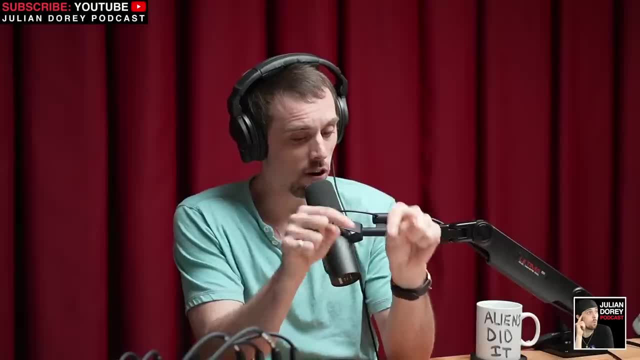 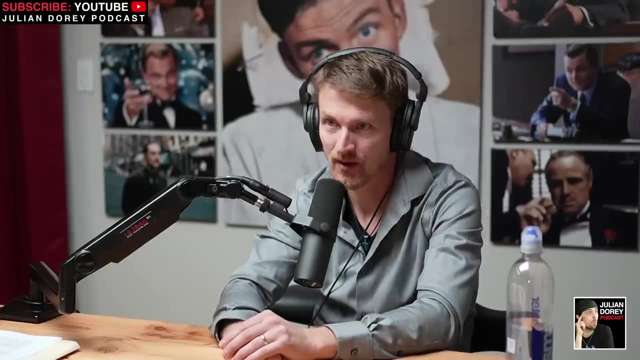 talk about it too. they talk about how would? why would we be talking about it in this reality if we didn't? you see what i'm saying? well, i i totally understand. i think it comes to karma because, loops right back to our discussion earlier about karma, in the atrahasis, there's this bizarre. 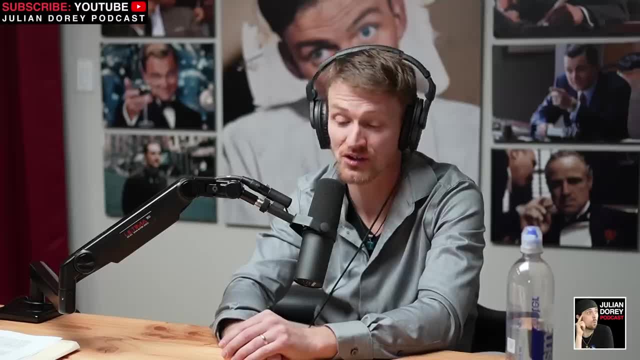 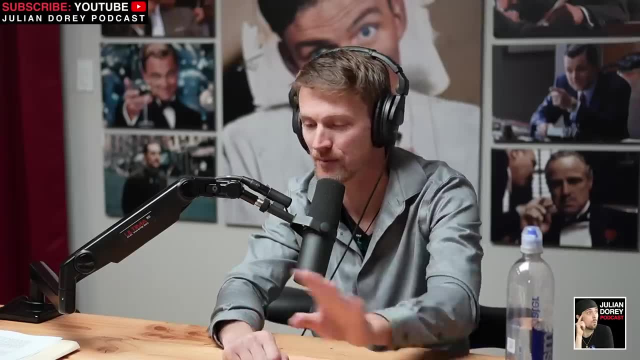 line. the atrahasis is that is the, the noah figure. who actually that's? he's he. it's his set of tablets. he has his own set of tablets called the atrahasis, my favorite set of tablets of any of them and i would consider them the most important of all the tablets, the atrahasis in that is the most peculiar. 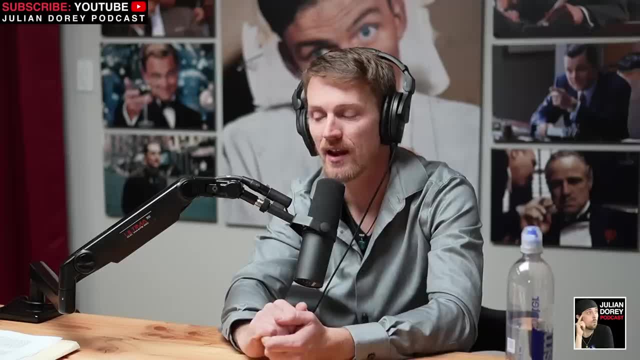 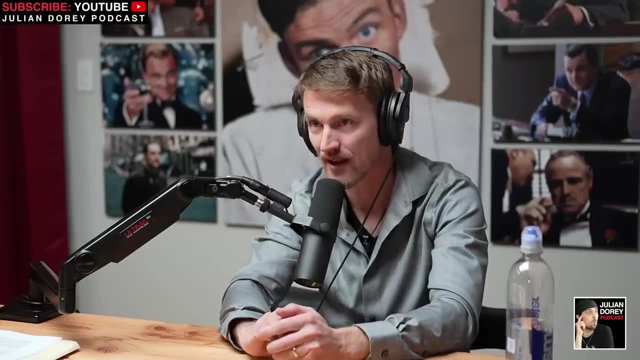 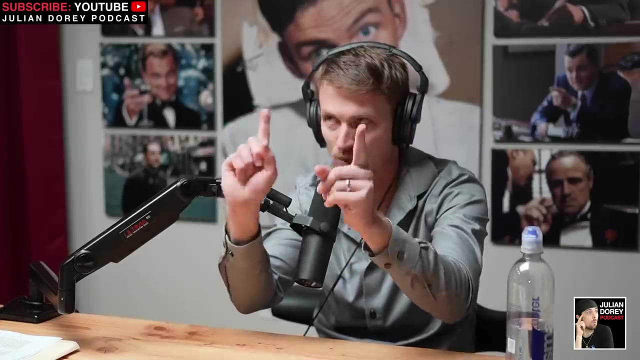 line and i can say it off my head because i know i don't have to read it: there's the most peculiar line of anything ever said in any tablet like peculiar and it ties in exactly what you just said. it says in there: enki and lo's talking to enki, they're both sumerian, they're both these powerful two uh deities that. 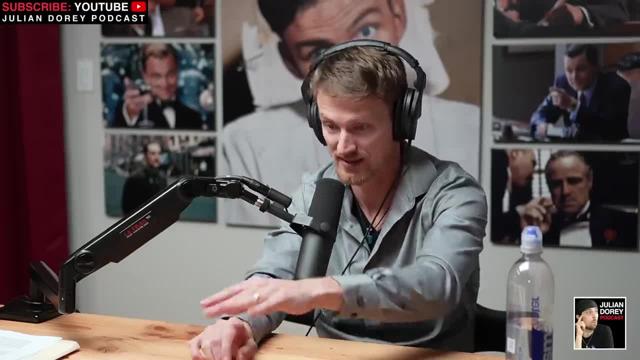 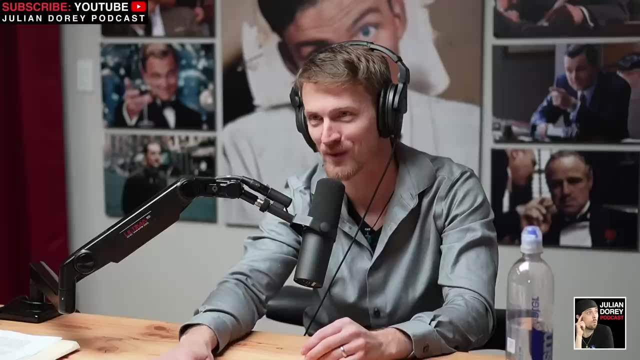 seem to be very much in charge in part of our reality, in our history. they seem to be like: this is enlo right here, his name is haldi or haldi. i can't say i can't, i'm not gonna say that's gonna hurt my throat every time. but um, we'll use a soft h. um, it's the same thing and what he says in that. 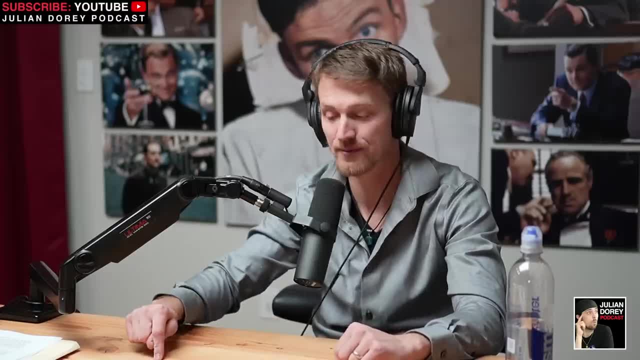 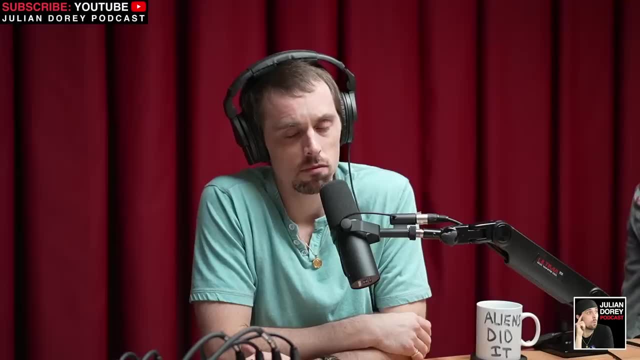 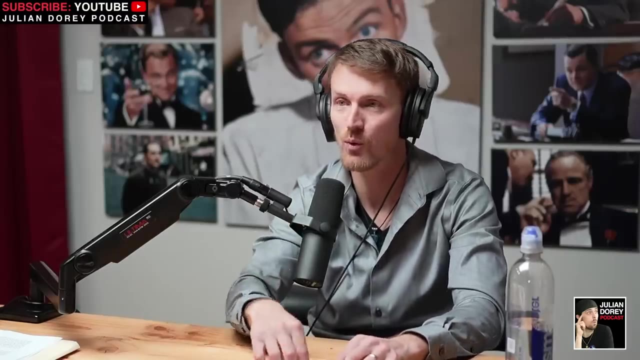 is. he says enki, where you went and you can find out where he went through the legend of atana. he went in the underworld. remember saudi arabia with all those inverted step pyramids, the doorways. he said where you went. i want you to think about this for a second before you say anything. it said enki, where. 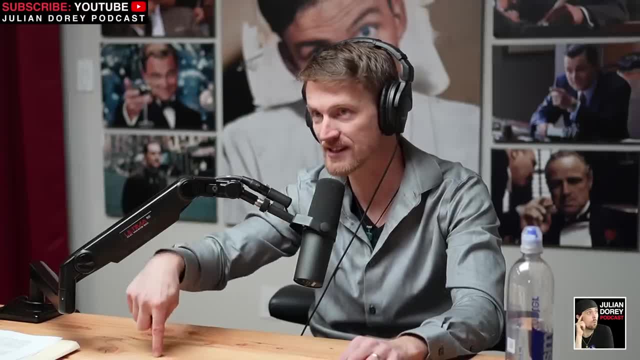 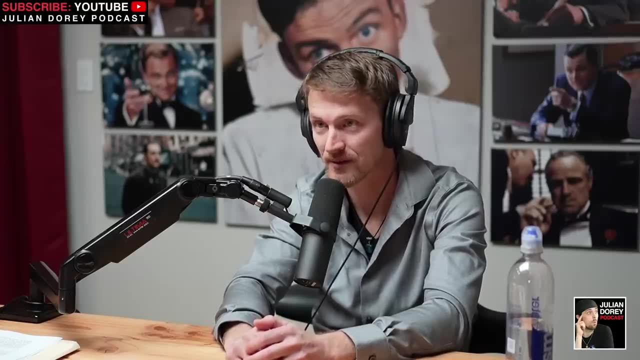 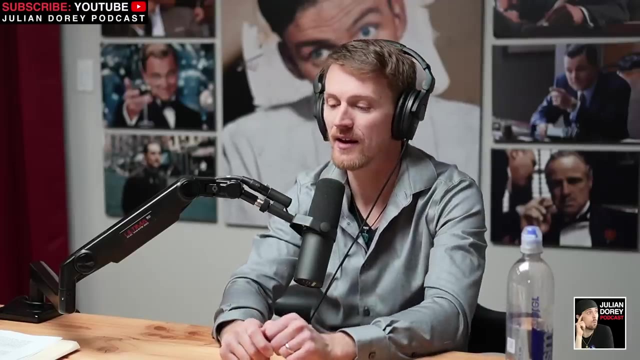 you went, you were to undo the chain and set us free. i kid you not. it says that word for word. and what's your connotation with that? well, why would you be? what's a chain like? okay? so a chain is like you're stuck to something, right, yes, right, okay, uh, why, what would you need to? 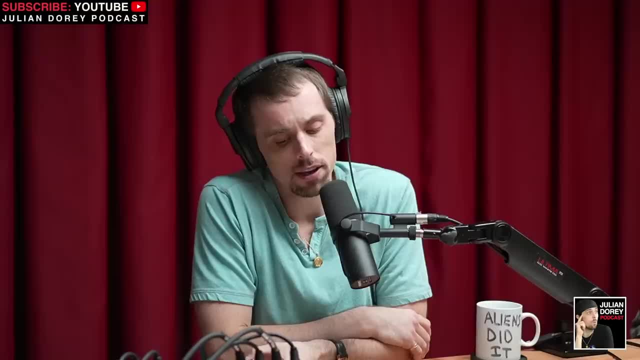 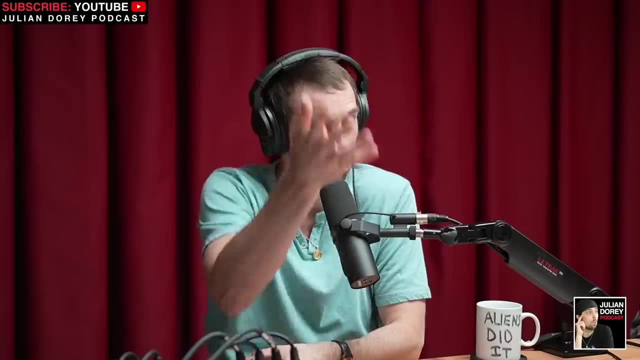 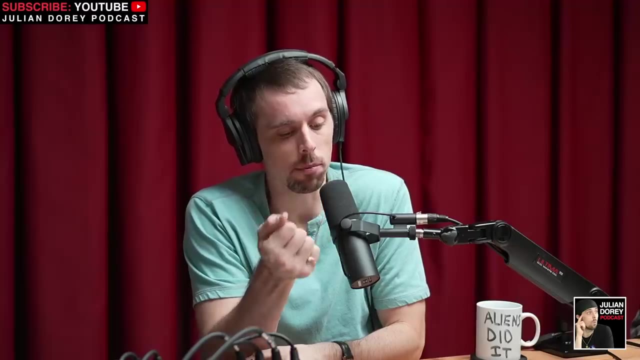 undo it. for why are you chained in the first place? well, i think i mean i'm drawing the parallel to what we see in all kinds of religious texts, like let's look at the bible with adam, because we were just talking about a minute ago with with adapa. the chain is is the unknowing right. but then 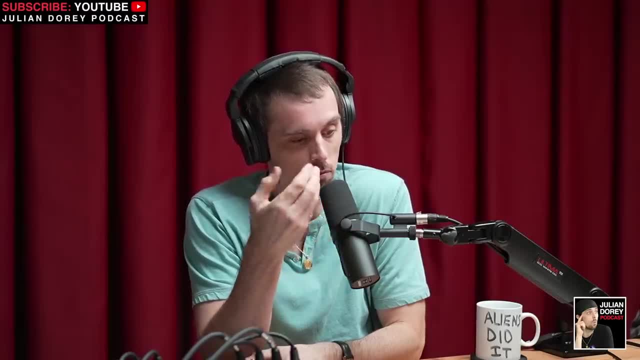 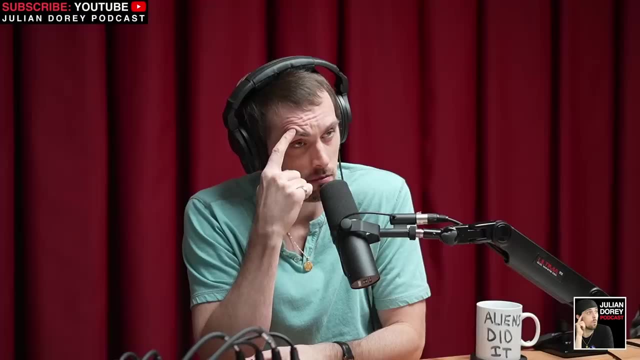 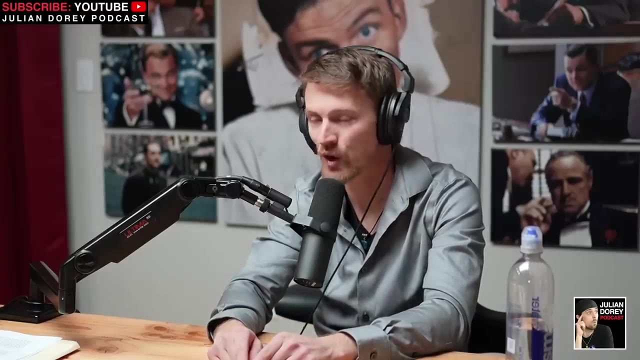 he gets unchained when he eats the apple but then pays for it. and now he's imperfect as well as a sinner, right? what if the chain's time? what? stay with me for a second here. what if the chain represents time? okay, now what if george was? george smith was spot on, he was right. i mean the human. numa illich speaks. 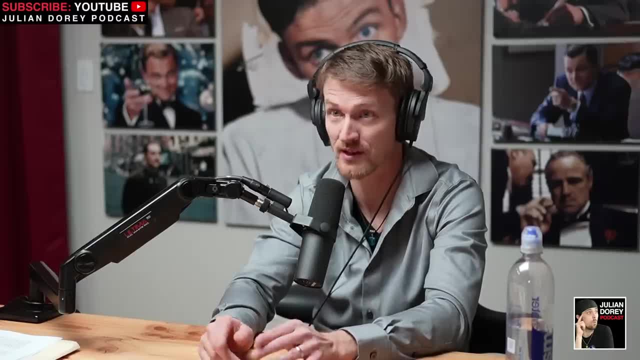 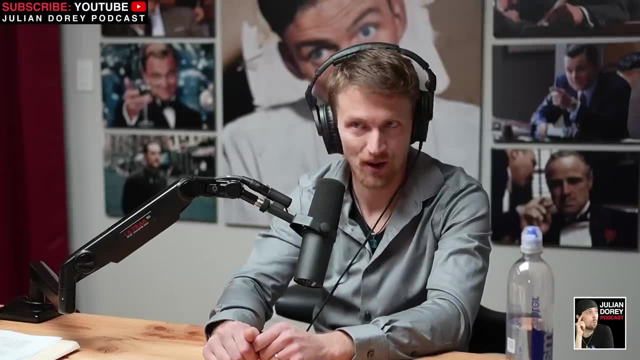 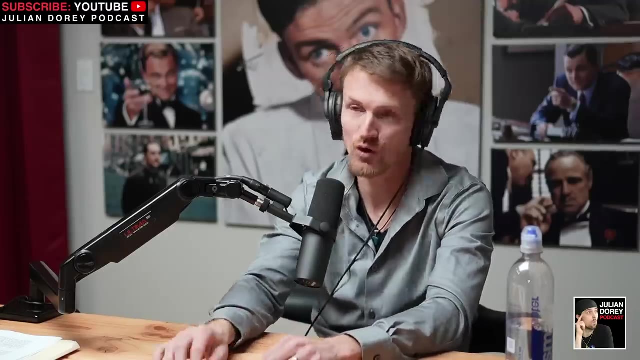 to them. being here before we were ever here is something about like proto-earth. seriously, read it. um, it's called the seven tables of creation. if what? if he's right, what if they did come backwards and they did things? what you just said is beautiful. if you go back, think about what you just said. if you go back and you alter, 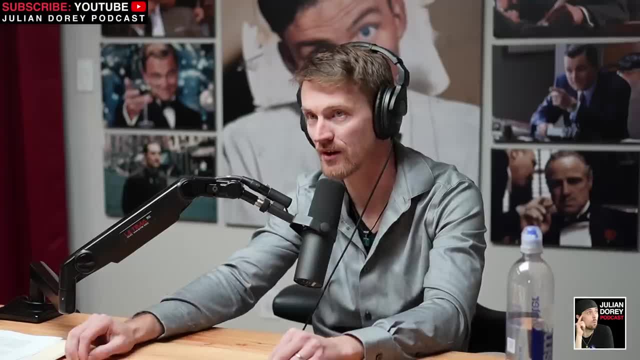 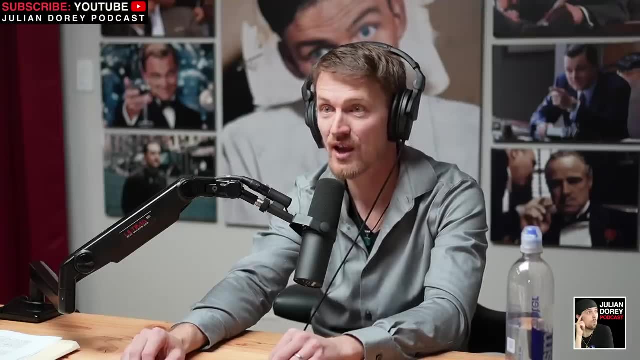 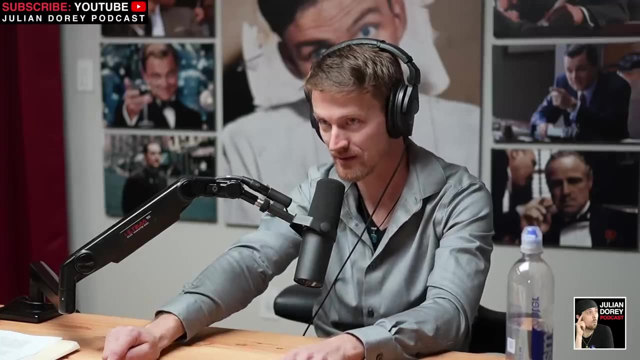 something in the past, it doesn't change the future. you create an all alternate timeline, yes, which means you screw around with karma, because you are then altering what was supposed to happen. you then be bound, you then become bound to it, unless now we're getting real metaphysical here. 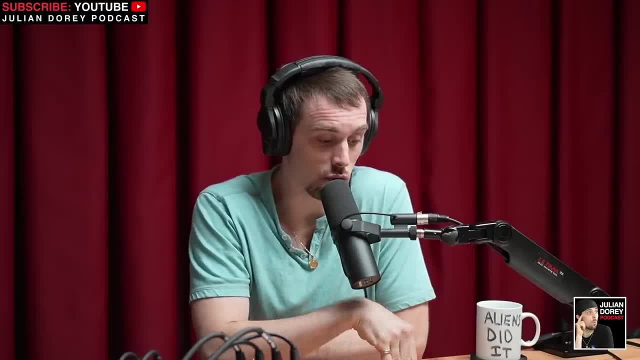 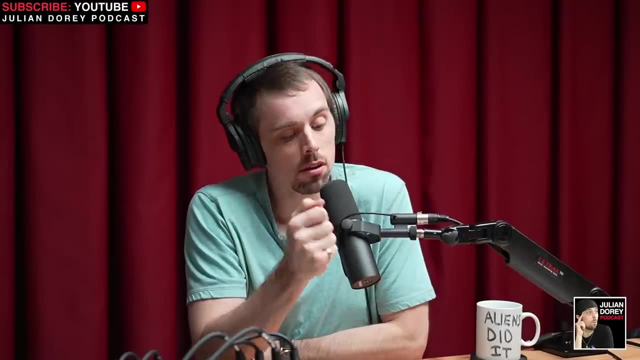 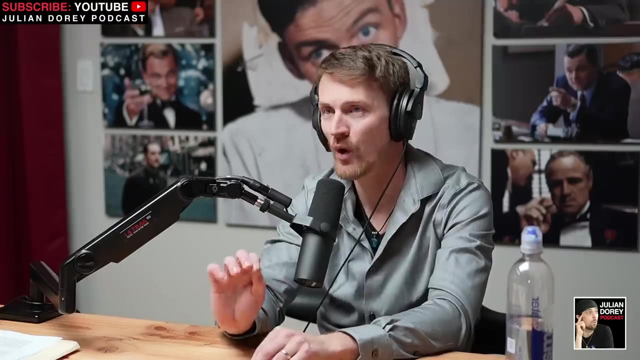 right, unless each of those new creations creates the other ends of the multiverse that your karma will take you to as yourself or maybe someone else in the next life. that's happening simultaneously. you see what i'm saying. but why would he say where you went? because we know where did i could go. legend of tana tana. 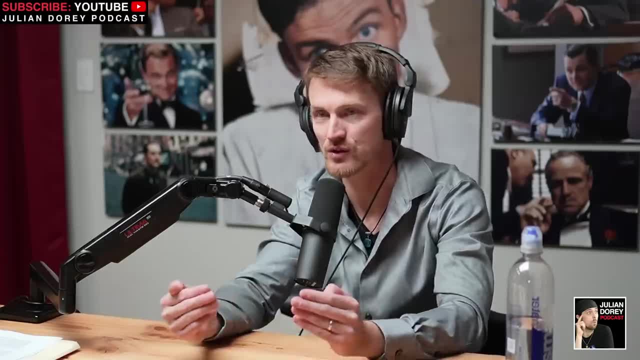 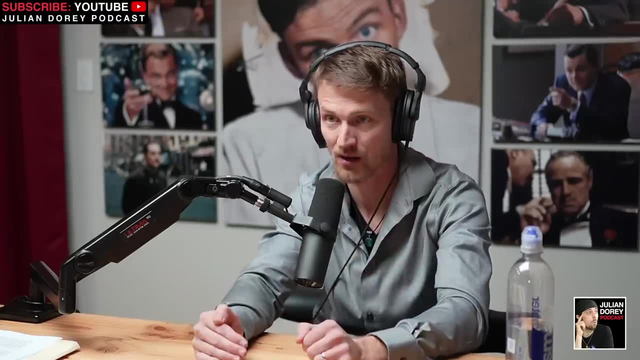 very clearly states, he goes in the underworld. he becomes one of these rulers in the underworld as a positive counterpart. so you have a positive and a negative, and a negative and a positive. it's like that. this is a hermetic law you have there's. that's the way everything seems to be. 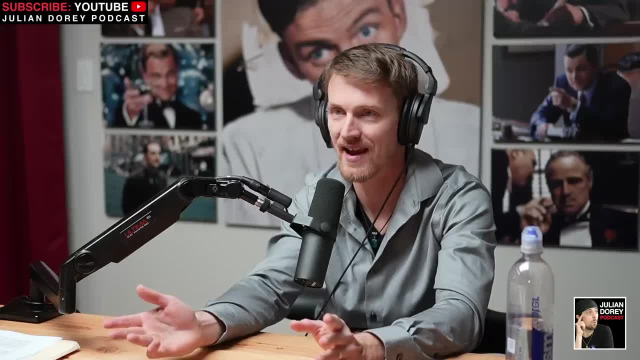 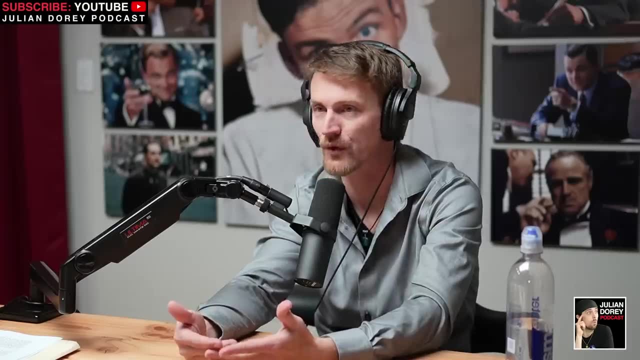 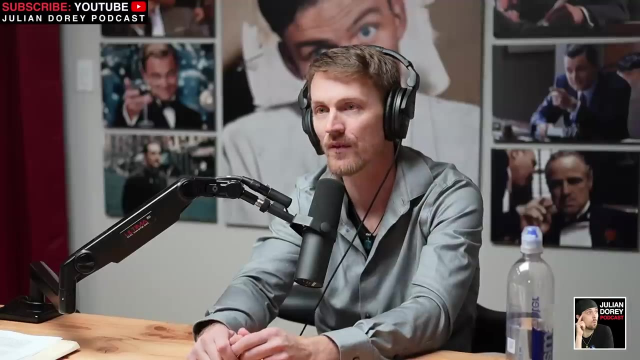 just so you know, is there seems to be like the underworld is not just a negative evil. there's a, there's a war, there's a. there's a demon like being in the underworld that is called nergal and it is playing the role of death and destruction and war. nergal- his name is nergal. 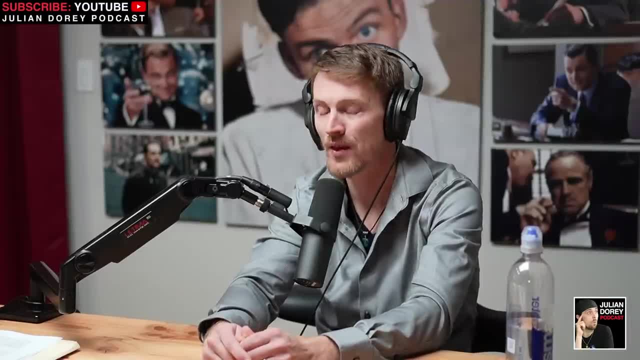 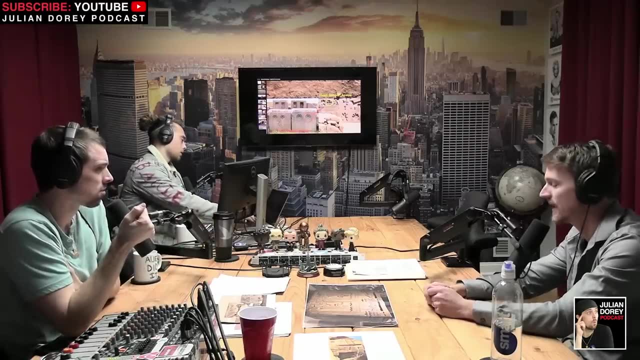 n-e-r-g-a-l. yeah, okay, he's a demon like. yeah, he plays the role of like a demon here. where is he first seen in what we know? like what? what you see is that nergal? yeah, you find on the tablets that there were four anuna, four again. 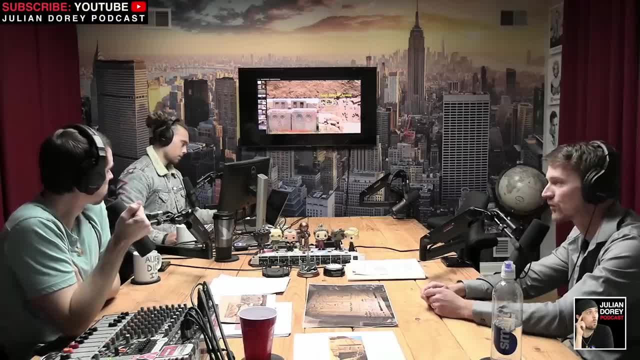 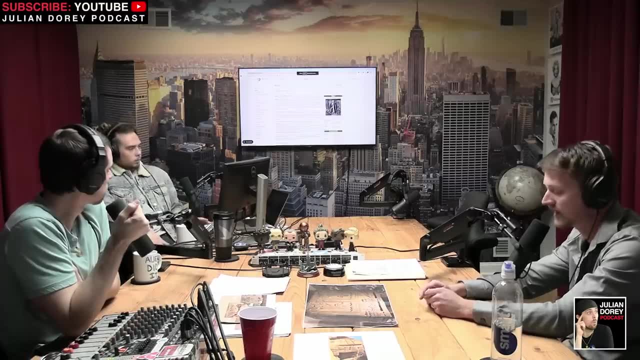 there's a totality of two and two above and below that assume different roles within our reality. that's what they describe them as, and so when there he is right there. so when, and i believe nergal was known as was, god is no- was known as god el and the maya, which was like a corrupted 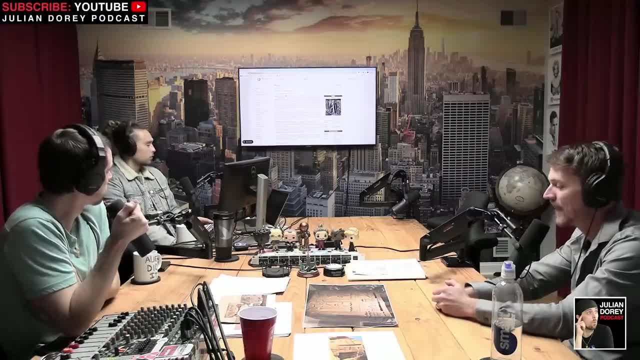 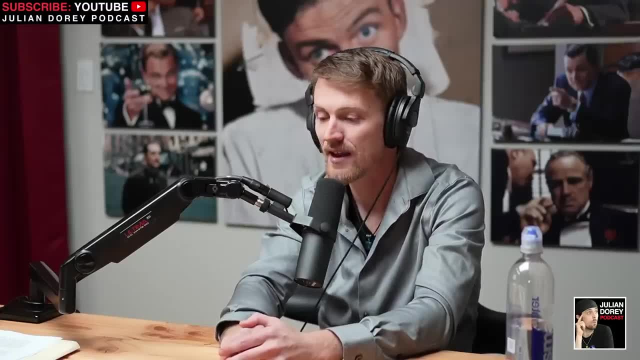 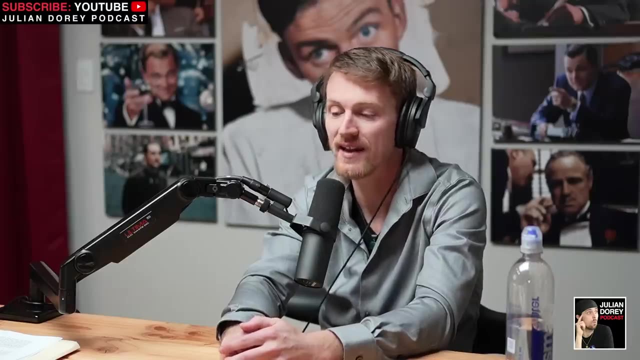 blood sacrifice type influencer. that's nice, well, no, but imagine they're all playing roles, just distinctive roles within the duality of existence. okay, and imagine that that that being is playing extremely like these: playing the negative, the bads, the bad guy, right? well, enki was supposed to go in the underworld to play the positive. 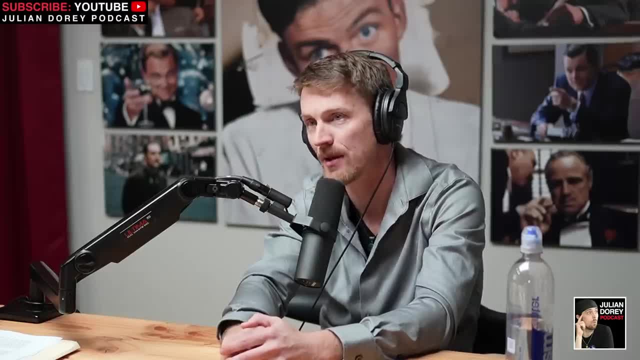 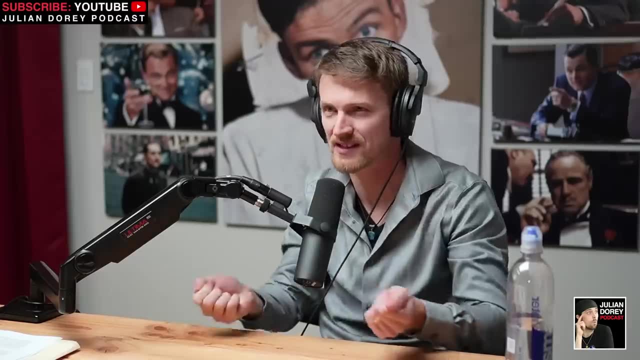 counterpart to him- that's what the tablets describe him as is playing a positive, positive counterpart to nergal in the underworld. so it's like. it's like. there's like a balance that exists that we don't understand. okay, with with these concepts. now that's where enki went, the reason. 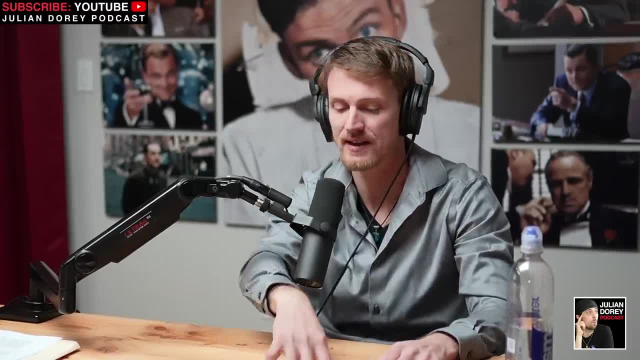 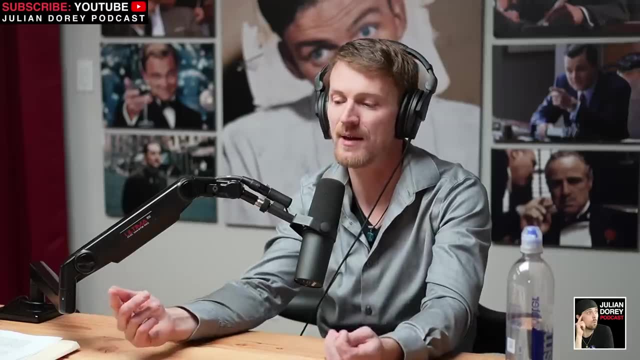 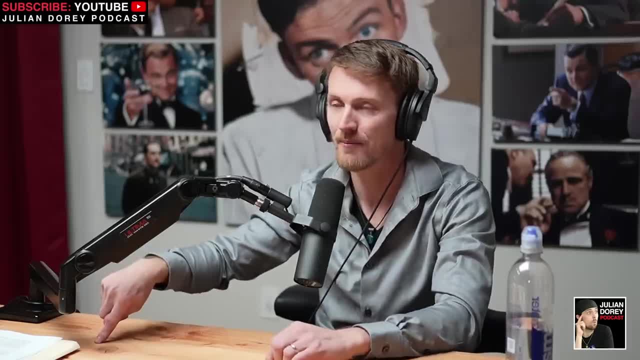 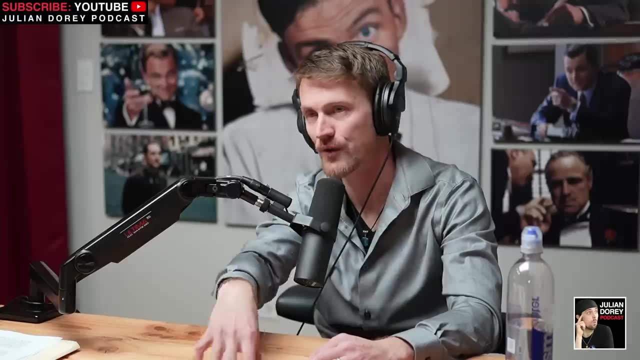 enki where you went. you were supposed to undo the chain and set us free. my theory on that, based on everything i've looked at, is that the anuna came back in time and altered our future and screwed up their karma and became bound to it. they got stuck here. 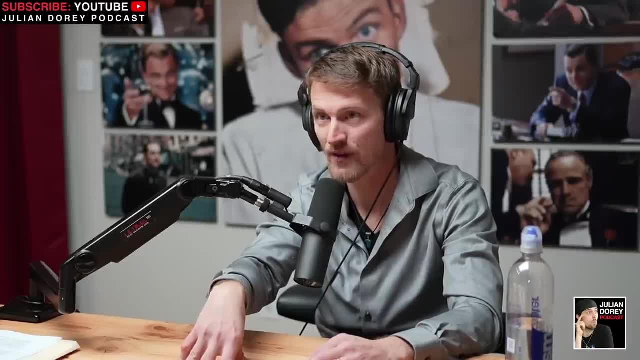 they couldn't leave. that's why they're all throughout history and they and they're and they're so involved is that they got stuck in our realm and they literally. there's cosmic laws that, i think, prevent certain things. wait, how do we, all right, are we making too big of a stretch there? 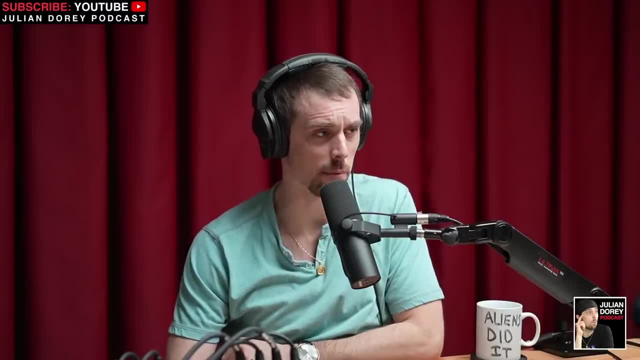 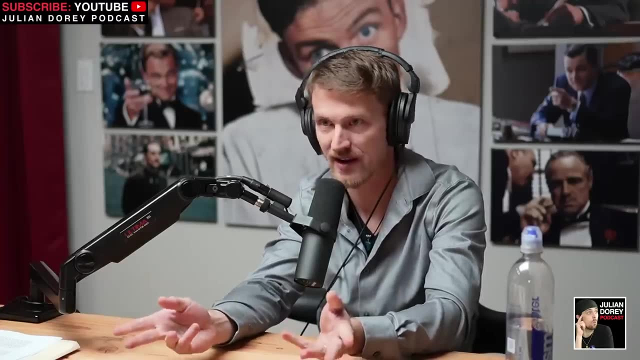 like, how do we even know these cosmic laws if we're limited by our own understanding of physics, which is still extremely limited? we there's, you know sherlock holmes right, the famous fake, fake character that's based on- oh shit, sherlock obviously right, um, that famous. 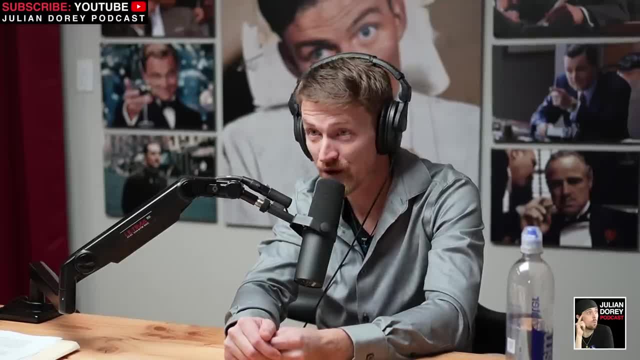 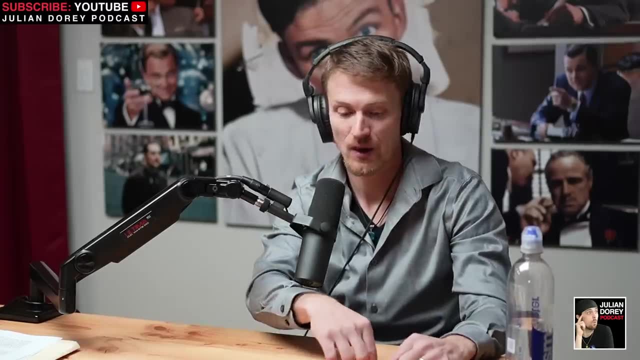 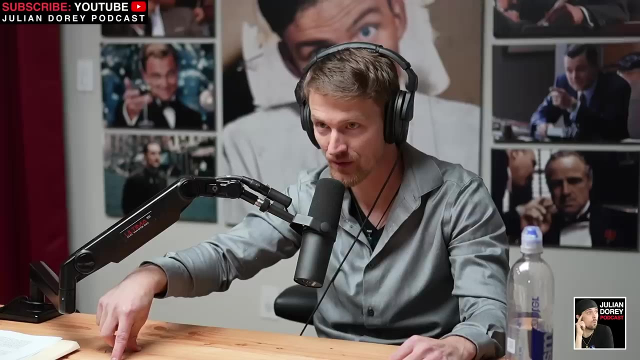 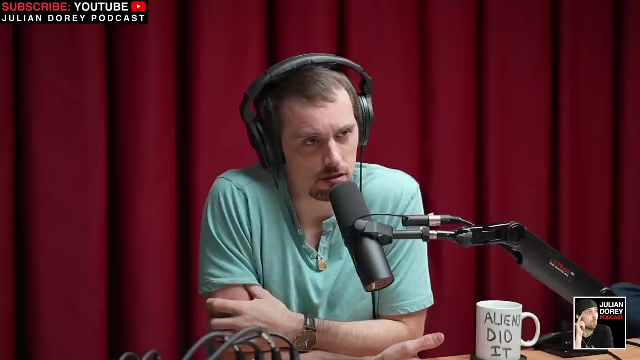 quote from that: right when you're trying to figure something out, no matter. this is a blanket statement and i think anyone should use this: no matter what in life, once you eliminate the impossible, whatever remains- no matter how improbable must be the truth- well, there could be a lot that remains, well, but what? but what do you? what are we knocking out? we? 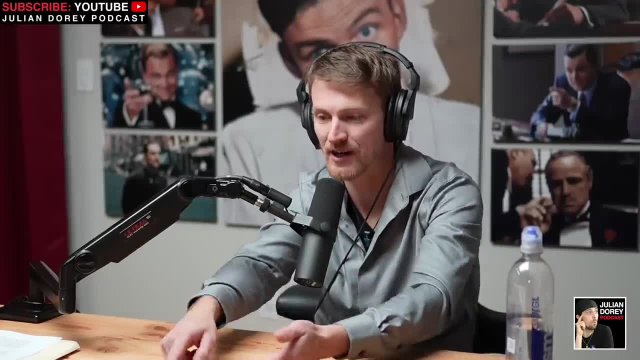 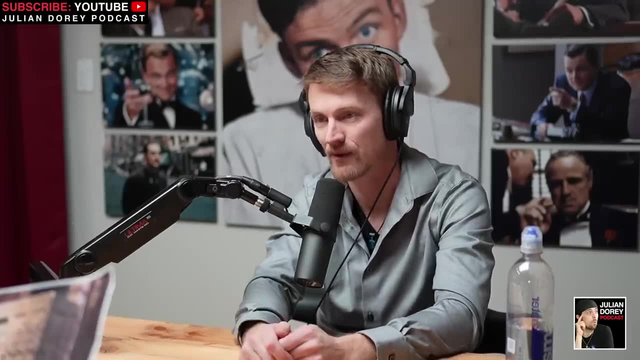 know they're not here in spaceships. we know that because we look at the depictions: they're us, they look exactly like us. we know we know a lot of things actually, but we just need to put them together like look at that being right there. that doesn't. 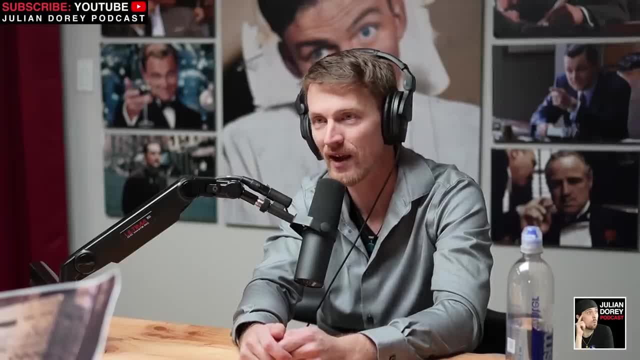 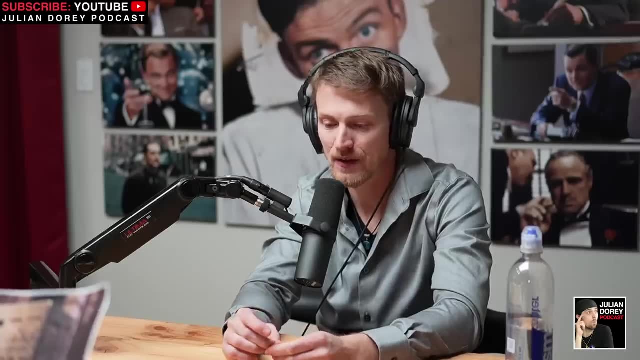 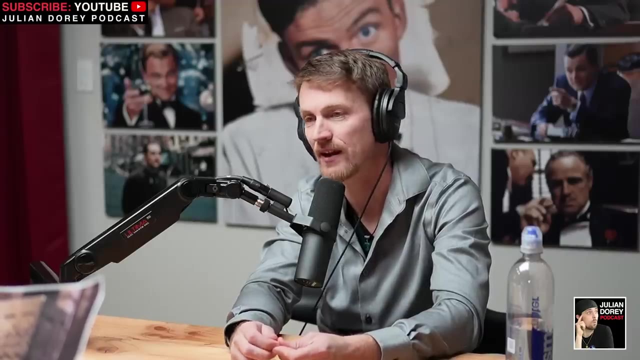 look like some gray alien. it's us. she's got a hat on and wings, and it's the same thing: eyes, nose, mouth, right, but but they. it's a nice hat, though, but they seem to be integrally connected to our future and and our destiny, which is why they call themselves the ordainers of destinies. 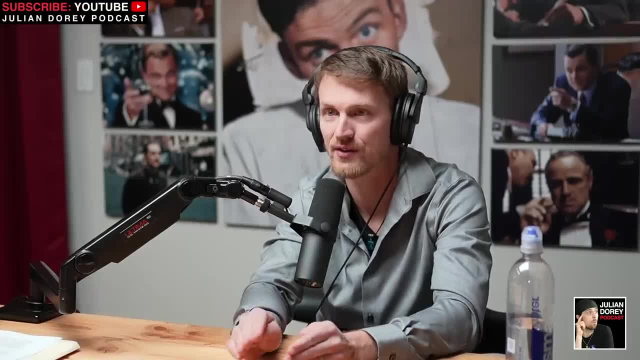 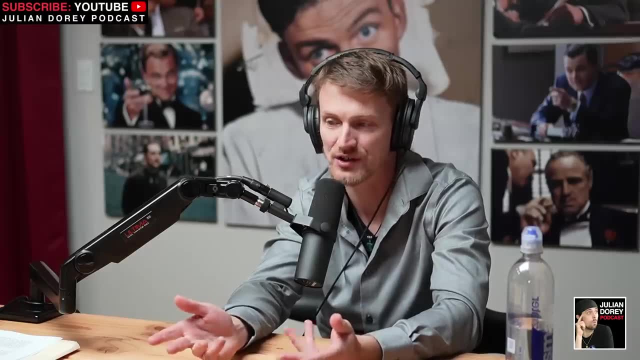 and they seem to be in in a deeply integrated into, in the path that certain individuals take here, and they- and like, for instance, the epical gilgamesh is a great one to identify- is that he goes on this, this journey to find immortality, and they talk about how he's. 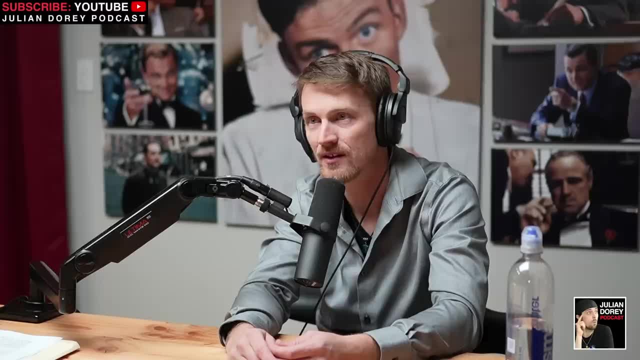 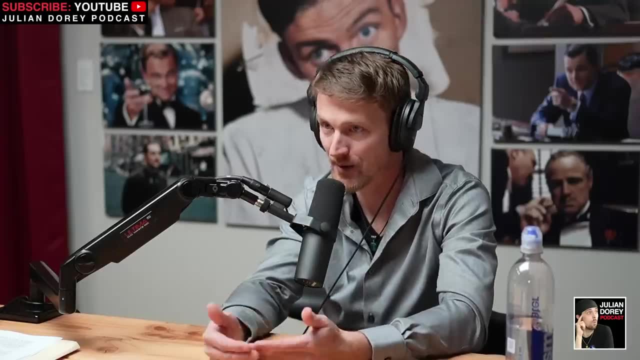 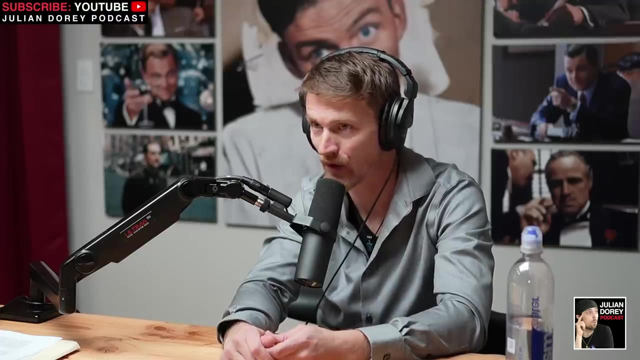 um, they get his attention and then they start like assisting him on his journey. so there's a lot of things going on here, but the ramifications are that i think our reality is complicated, and i think that it's. we're part of something far greater than we understand. 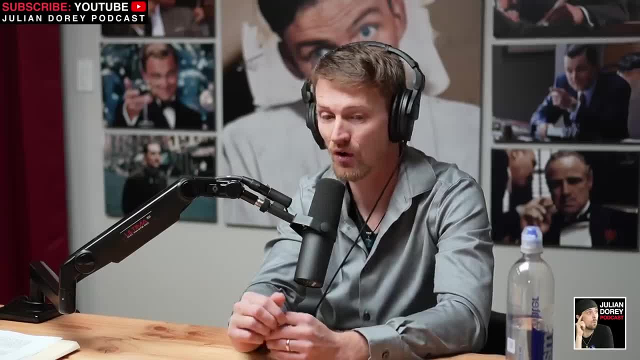 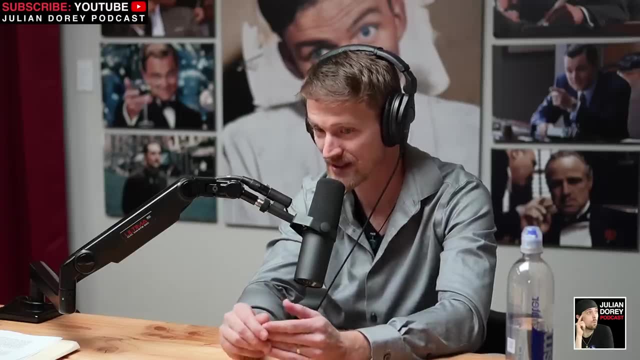 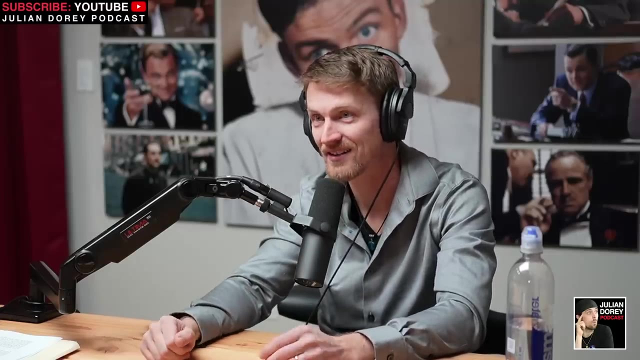 and that these ancient sites and these depictions are all trying to tell us about that mysterious origin, about who we truly are and about how far our past goes. and this entire game here is so that we can try to forget it and then find our way back. why would 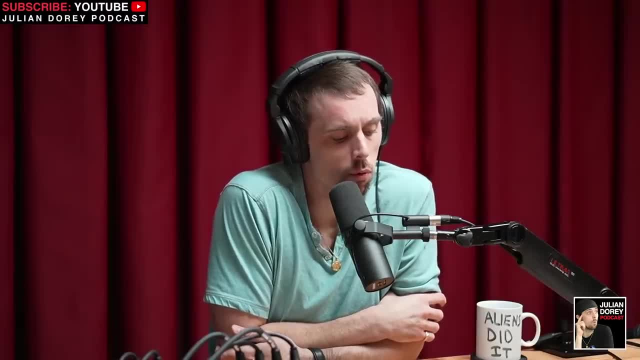 why would the anunnaki not want us to know about them? is it a part of the game to you to find our way back? so they? so they place humans in our way who just question stuff like this and say no, it must be bullshit, and therefore make everyone else accept that as mainstream is. am i going too far down the 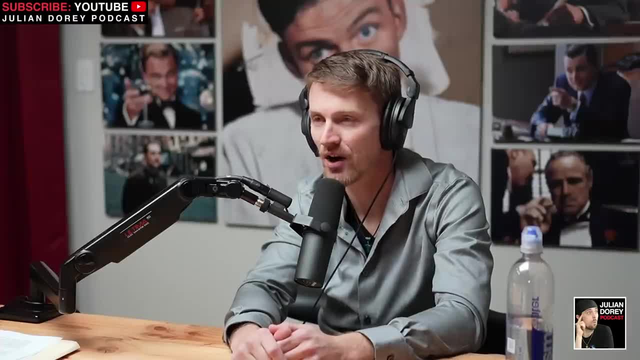 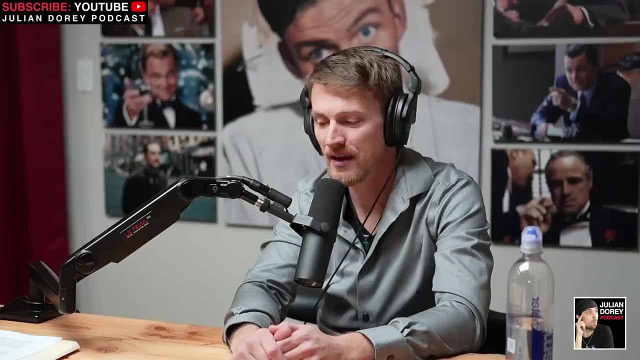 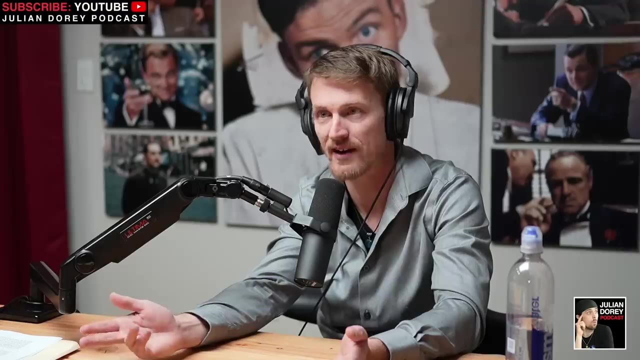 conspiracy rabbit hole here. it may be more that the earth is an important incarnation place for souls. a what incarnation place for souls? all right, in english, not japanese. meaning that let's say based on energy, that energy never, never be, never destroyed, right, it can never be created it. 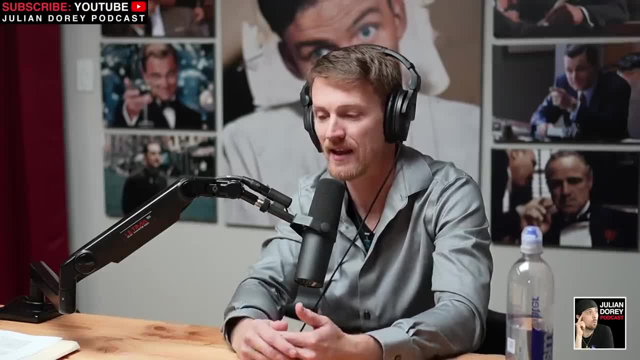 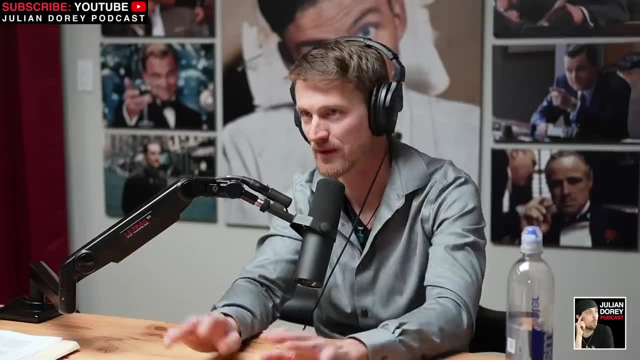 can only change shape, right. so energy is eternal forever, meaning that if our consciousness is just purely energy, then we were to our eternal beings. but that doesn't mean that the soul is the same level of development as another soul. when you get in you really get into looking at it and like 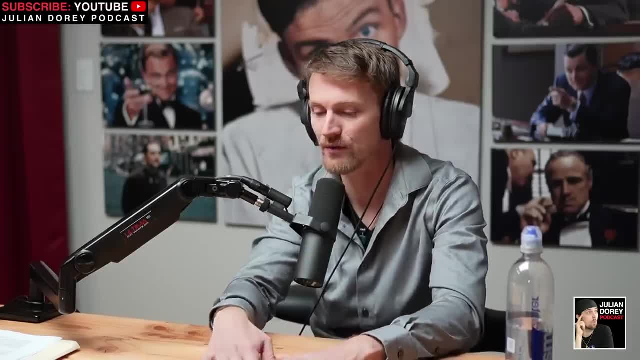 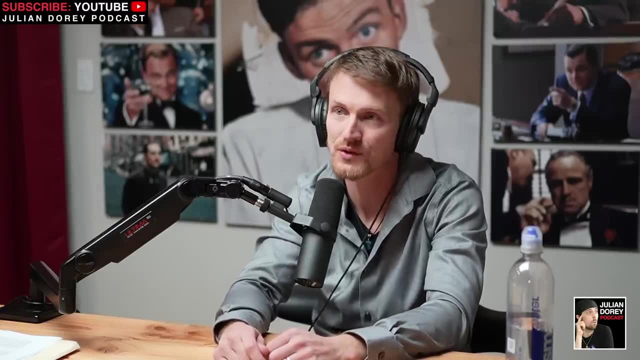 especially like hindu texts. you learn that there are levels of souls here. some are kind of new, figuring things out like, and others are old, like old souls that have been and done this many, many, many, many times right, and we're all here for different reasons. how do you determine what's? 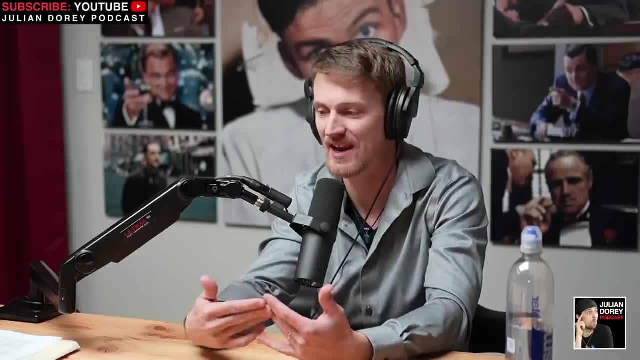 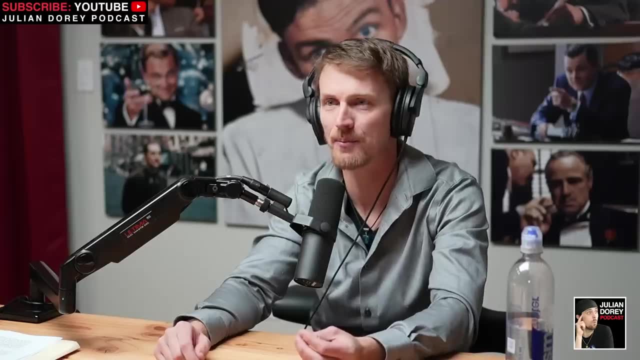 new, what's old? well, i mean, you'll have someone who's just inherently wise, very mature for their age, very like balanced. they seem they're like really different than other people. they seem like they have knowledge that's really profound and there's something. but what if they? what if? 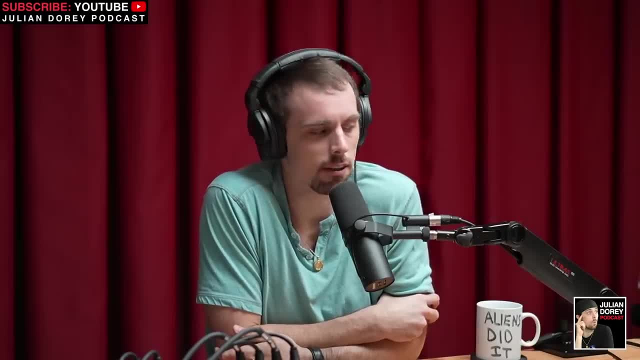 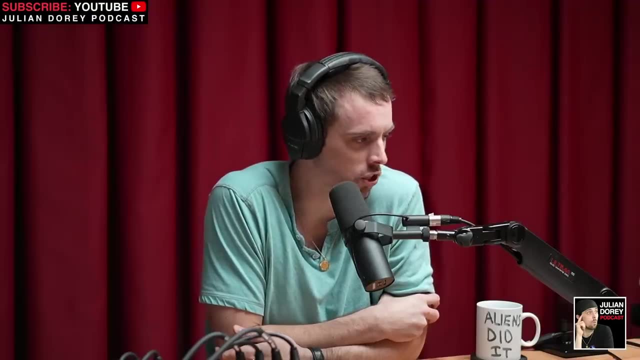 they were born into a broken household. their dad was an alcoholic. they had to take care of their totally. they were self-educated. they had 140 iq and then suddenly they learned all these lessons at age 10 that no one else had to, and by the time they were 18 they'd already been a father to their 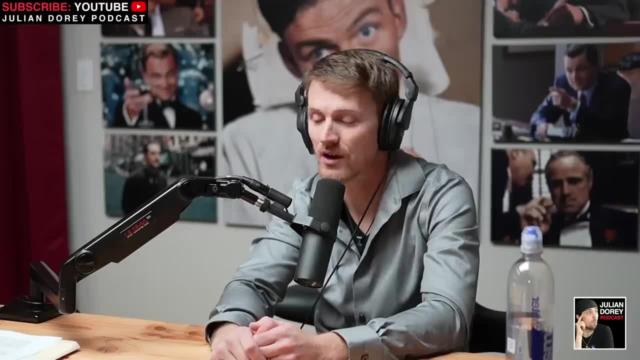 younger siblings, and so they're wise at 25. oh, that's obviously a factor, but what about like what we carry from other lifetimes? there wouldn't be a purpose of us to be doing over and over again if we didn't bring something back. what's the point? what's the point? the point is it's like a game. 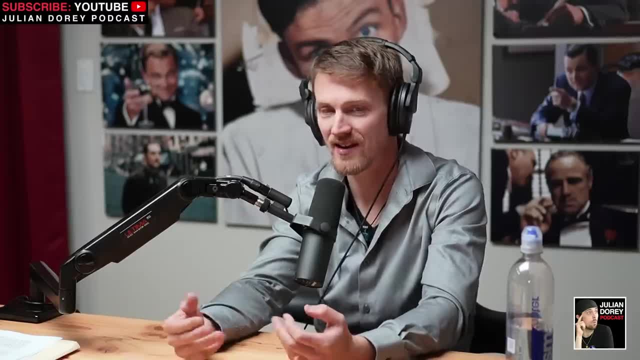 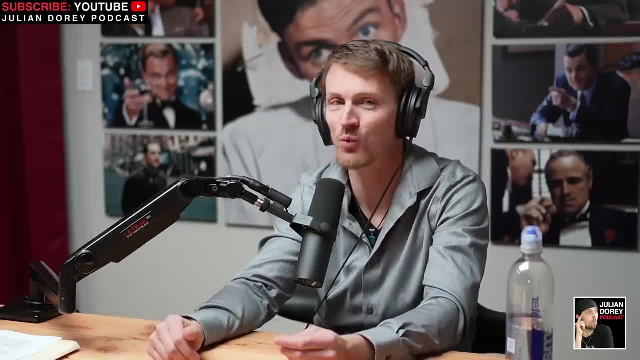 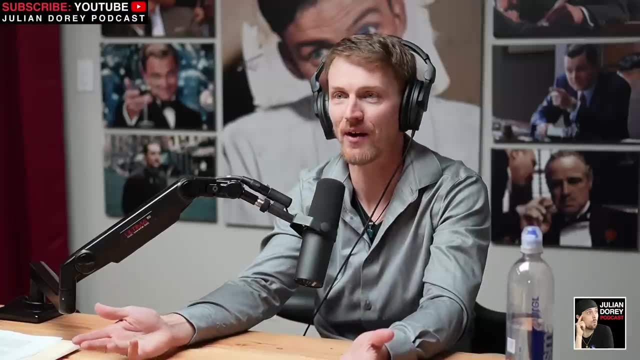 here and forget everything and don't know anything. and then look, we're in this world where it's like the truman show, where it's like kind of fake and we're like this is kind of weird, right, but that's what's so beautiful about it. it's like can you take this divine being that? 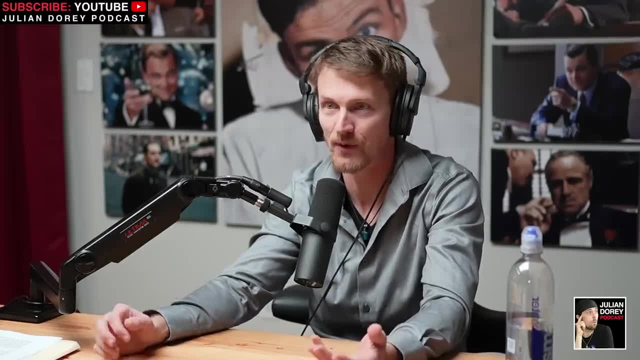 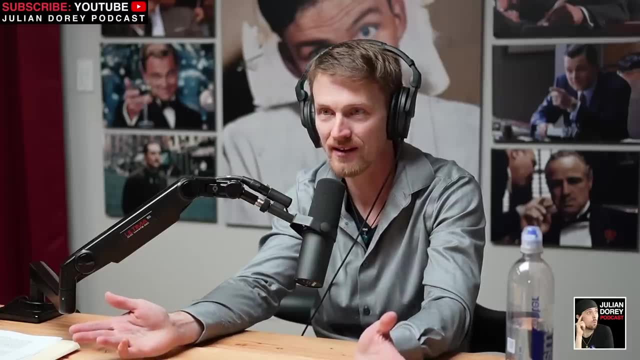 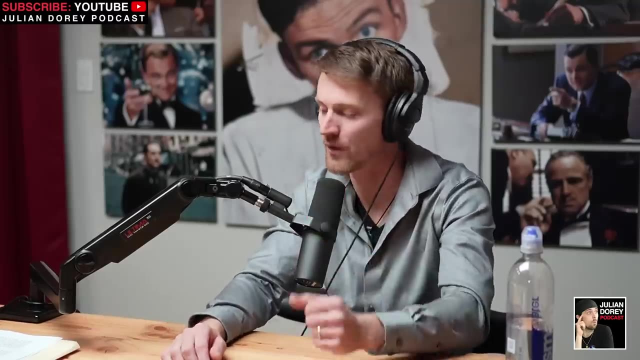 doesn't know anything about who it is anymore and has been controlled through war and other mechanisms, can it somehow, through the unexpected, somehow make it like it's? it seems like an amazing movie, that's the only way i can describe it is. if so, for instance, if you're like a, if you're powerful, if you're like omnipotent, you can do. 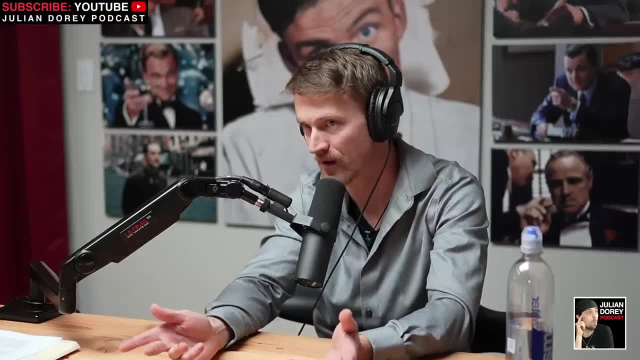 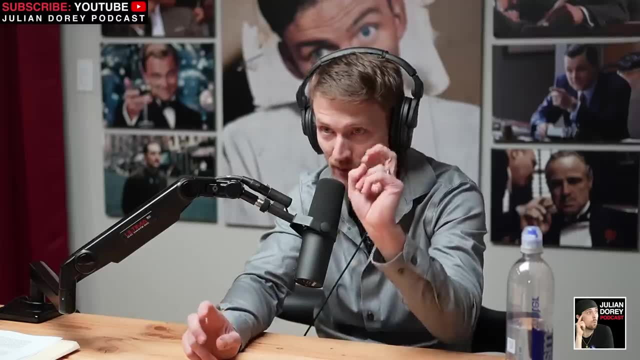 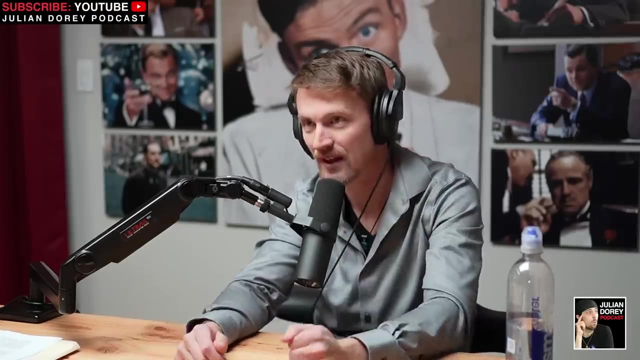 anything you want you're, the greatest thing you would be afraid of would be being bored. being bored is literally like the most horrible thing you could ever imagine for anything, because it would be like being in hell, like religious term: hell, right. so what you would have to do is you would have to create entertainment, like we do, and the entertainment though you would 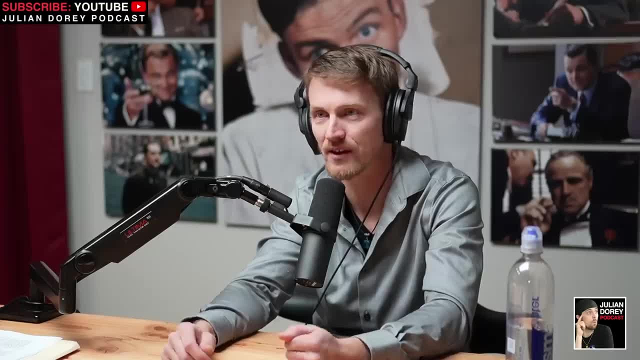 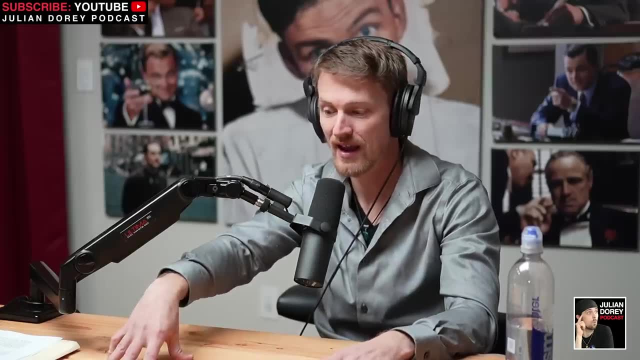 not be able to know the outcome, because what's the point of watching a movie if you already know what's going to go right? the point of a movie is that you watch it and you get grabbed into the story and then a lot of times, something unexpected will happen. at the end you're like, oh my god, i can't believe that happened. that's. 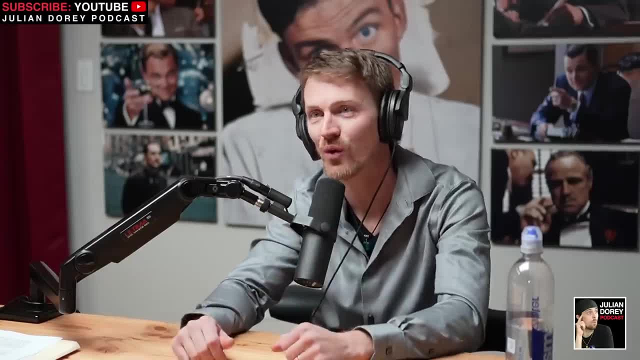 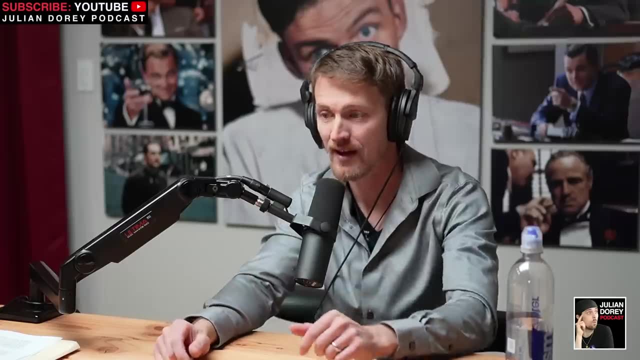 that's amazing, right? i didn't expect that to happen. i think that's our story. i think it's playing out like it's it's supposed to. right, think about our story for a minute. what is our story? well, if we take the ancients and all the evidence we have, we were somehow divinely created in the 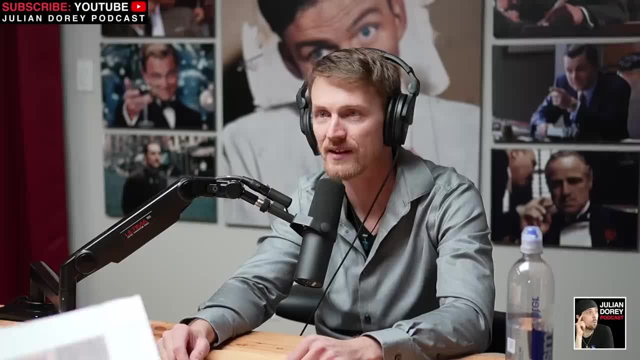 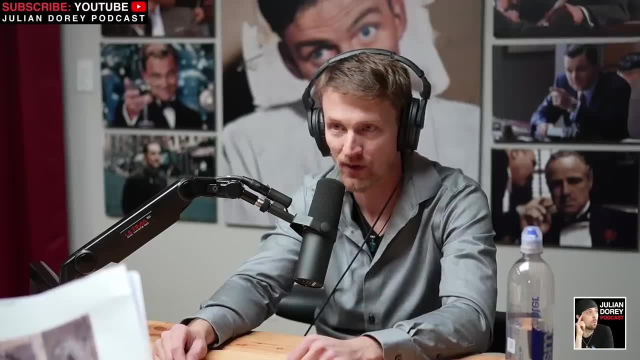 universe as some kind of powerful being and we're like, oh my god, i can't believe that happened. that's a powerful being. there was jealousy then that arose over it, and then we were almost destroyed in some catastrophe that was created only for us to barely survive and then the seed of us to carry. 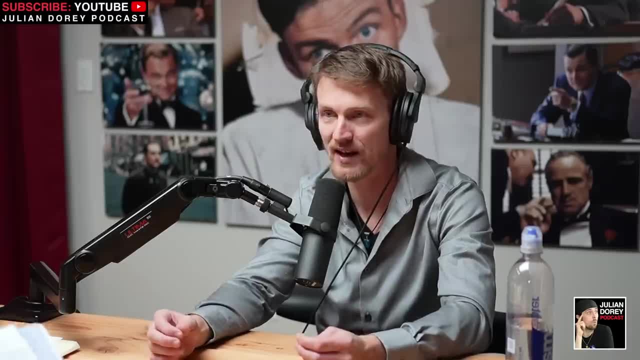 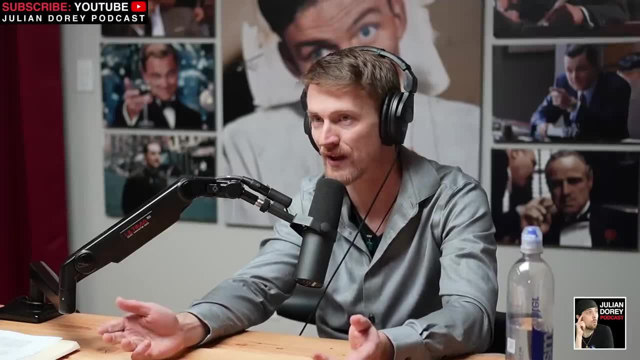 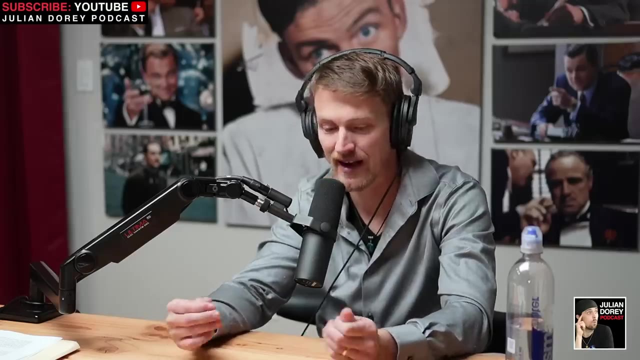 on and we rise up to become this powerful golden age civilizations. they're creating temples and pyramids, only to be destroyed by a catastrophe and to forget nearly everything and have to start over again. god damn, every time you need humans who survive too, and then all of a sudden at all. 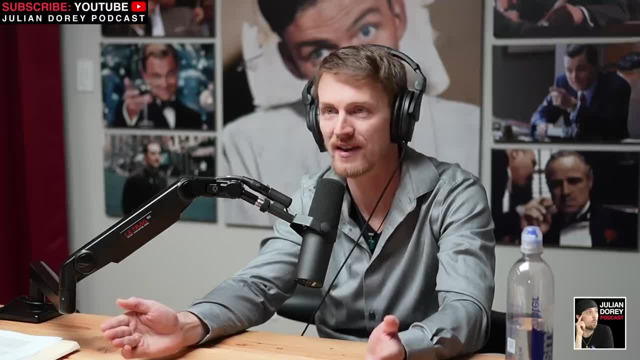 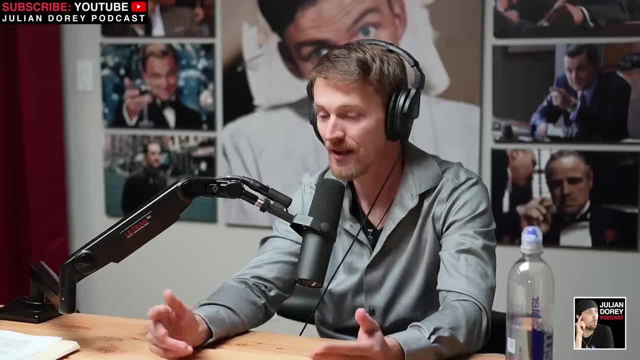 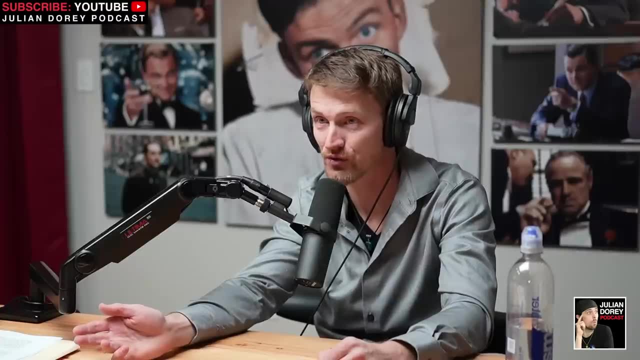 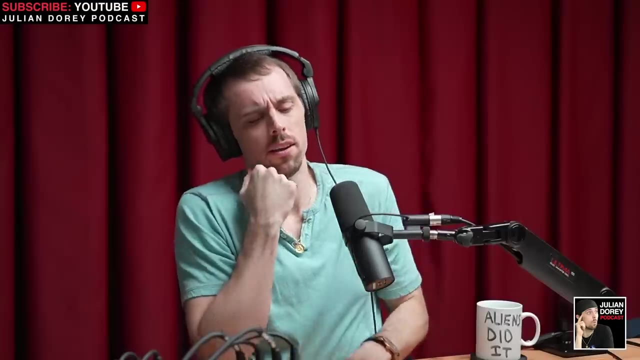 and then the cold war with nuclear weapons that can just annihilate all of us. what happens? we somehow make it. what a beautiful story it is, and i think that our story truly is the greatest story ever told, and maybe that's the point, maybe, i mean, that's where it gets weird, for me too, because 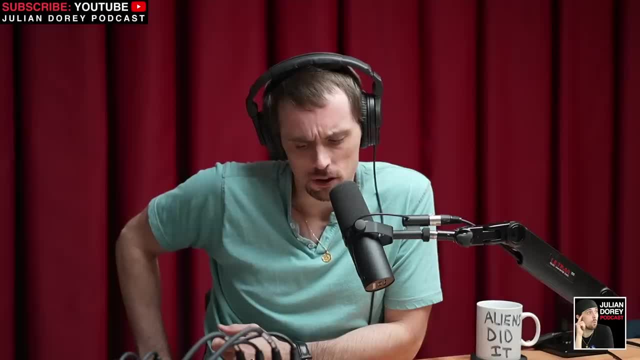 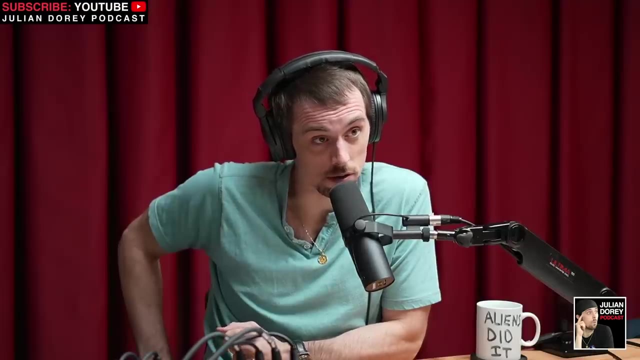 we had talked last time about the underground system. what, what civilization was that in turkey? derrick kuyu, derrick kuyu, yeah, where they had the shafts, basically, yeah, and you said this could be living underground. yeah, this could be catastrophe proof. they could have lived down here for hundreds of years, exactly right, so every time, 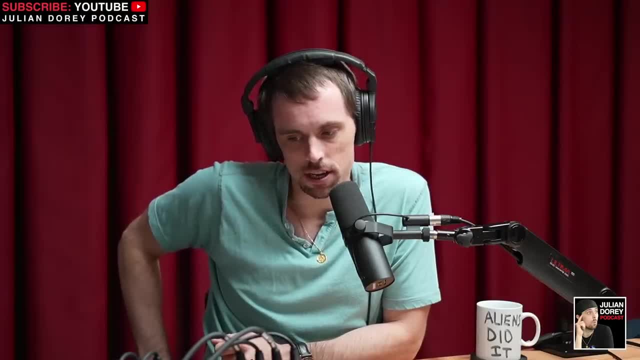 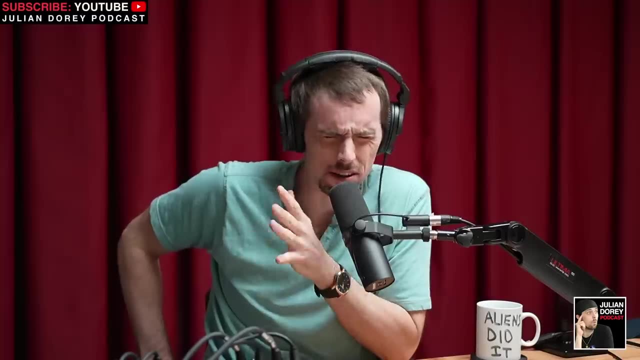 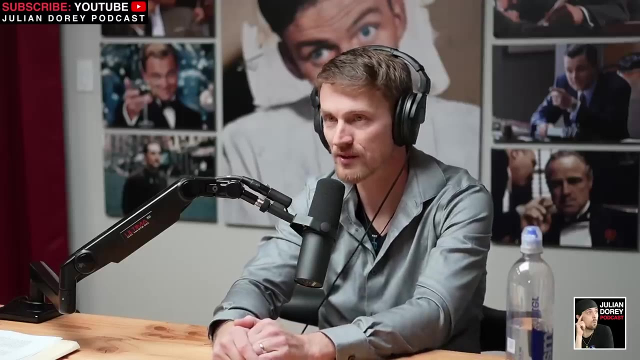 we've had these catastrophes if, if, let's say, lawrence krauss is in the ballpark when he says somewhere in the neighborhood of a hundred thousand years ago, something like that is when we separated from the ape gene- and i would say he's more on track than most right for sure. so either. 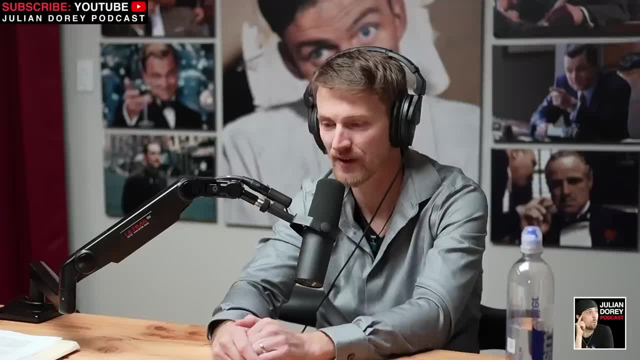 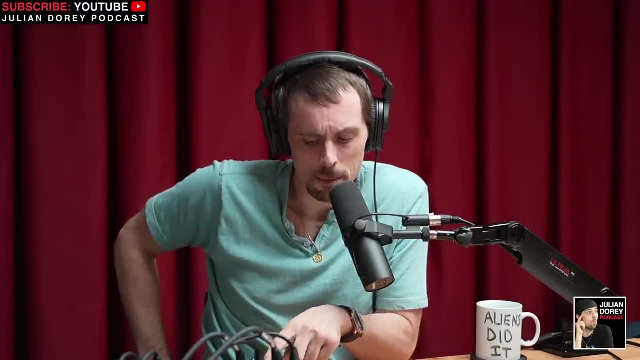 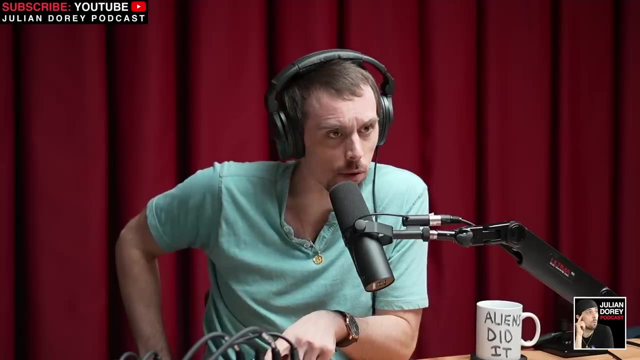 way. a hundred thousand hundred fifty. who the fuck? yeah, whatever, same one. two somewhere in there, right, somewhere in there. all the, all the catastrophes that have happened since then. humanity as a species, as an organism, needed to survive. i couldn't be like the tasmanian devil, where the last one was. 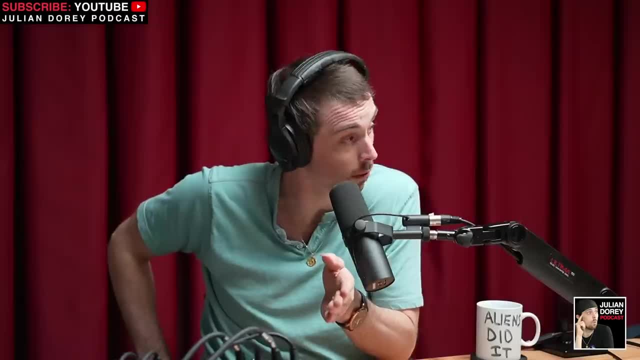 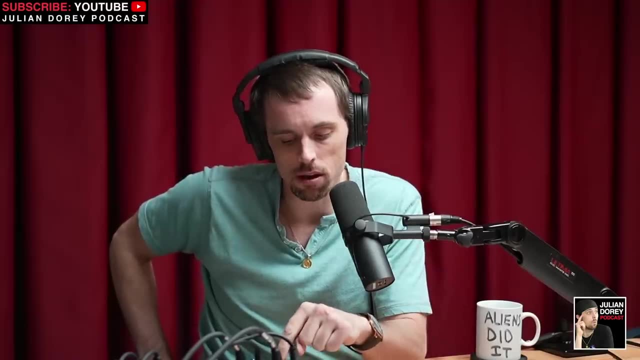 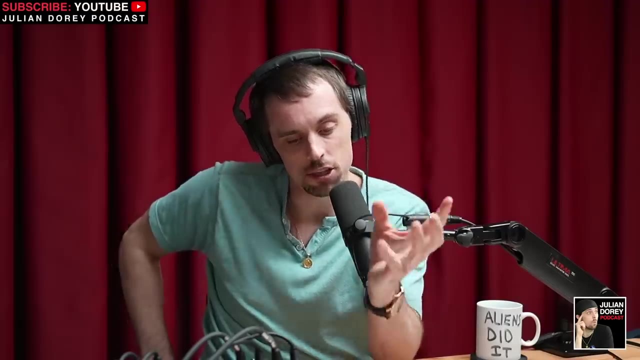 in whatever it was, 1933 or something like. they're gone, you know. hopefully we're able to recreate that with some science here, but assuming poor dodo, right right, poor dodo, poor dodo. but you know, if we, each one of those times people survived, think about how advanced civilization got, yes, and then these few, whether 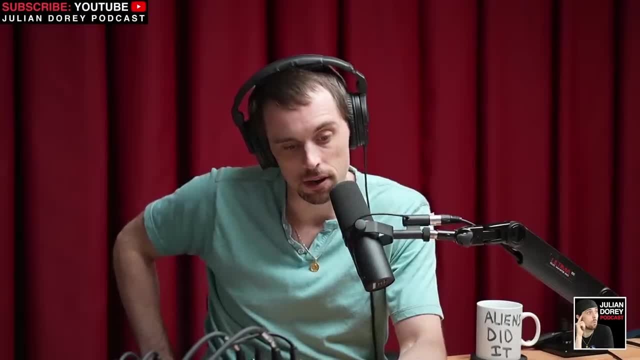 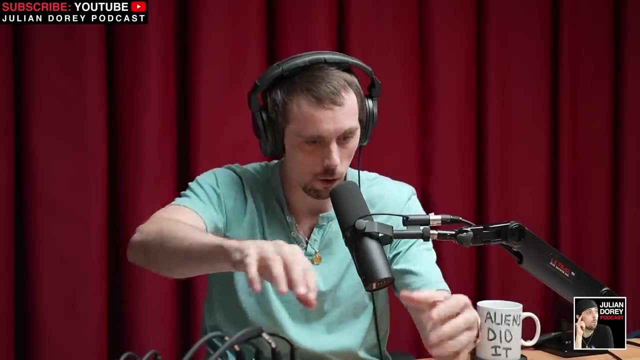 it's, i mean, if it's 10, you know well, there was definitely indigenous they were. they were surviving too. so it's not just them right? yes, but and again, and based on where they are in the world and the lack of, or the communication that may have been able to occur, based on whatever technology was. 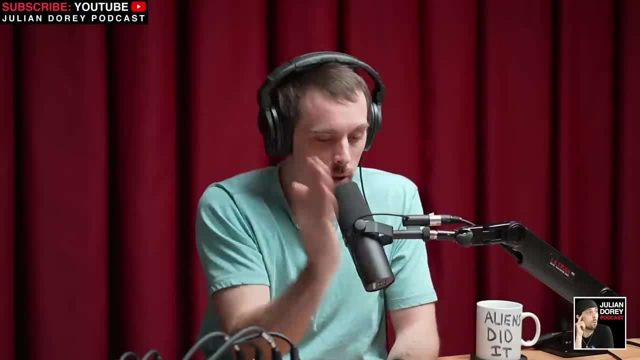 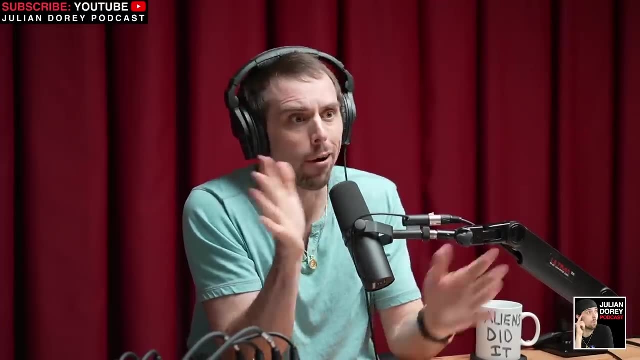 that maybe we don't know about. let's say like right now- here's the best way to put it- right now, the world ended and the three of us, along with 10 other people like us from america, maybe we'll keep it on the same country, okay. 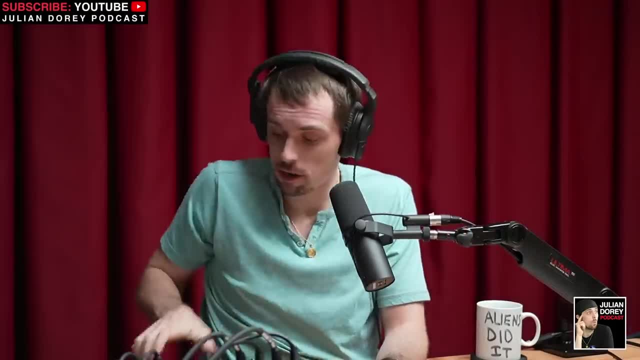 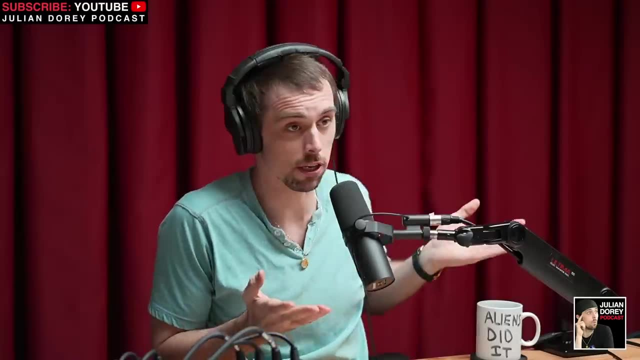 survived. think about all the stuff we know, all the stuff sitting in here right now, the technology we're aware of, yeah, compared to them not knowing anything right- and none of us are engineers, right, in this case, we can't recreate it, we only know about it. so we only know about exactly. how would 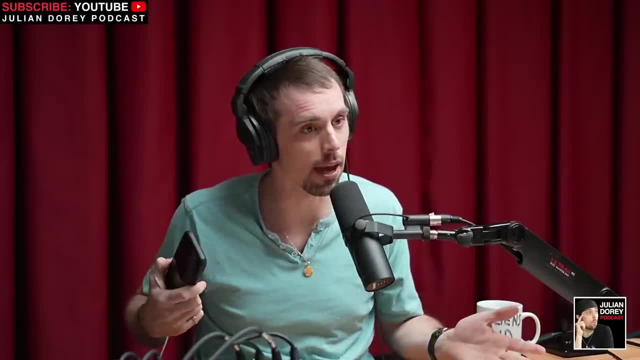 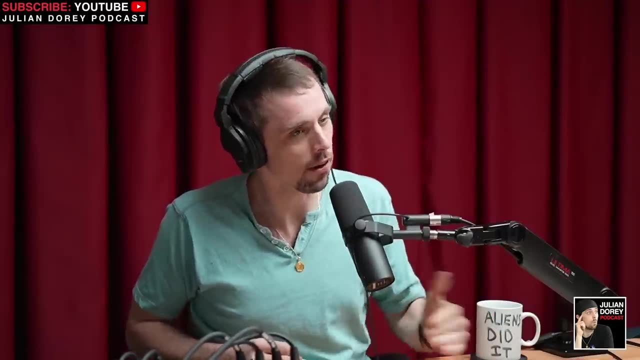 we teach our kids and make them understand. if we can't turn it on, we can't turn it on. we can't turn it on, we probably can't. so once a generation gets maybe two generations away, they're at there. maybe they're not at zero. right, they're not at zero because there's some sort of human understanding that's. 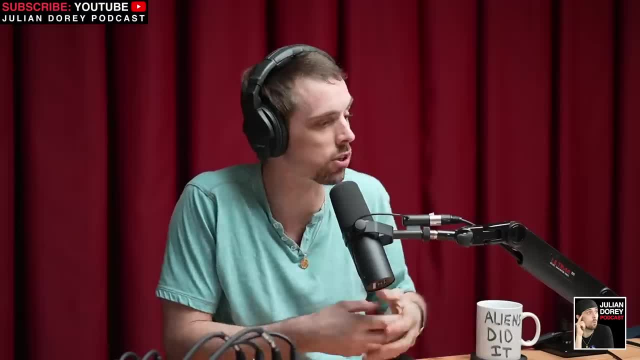 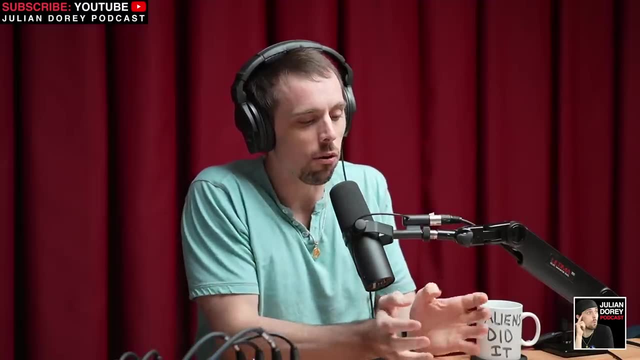 been passed on, that they're not going to create and create new texts and new stories, like their own bible, if you will, or their own ancient sumerian tablets, if you will. they're still at a, at a birthplace point, right? how many times might that have happened? i think it's happened. two to three times, and i think that is why, and what's the difference between two to three times? what's crazy about it, though, is that our story could have ended just like that, um, and every time it doesn't. i don't think we're supposed to disappear. 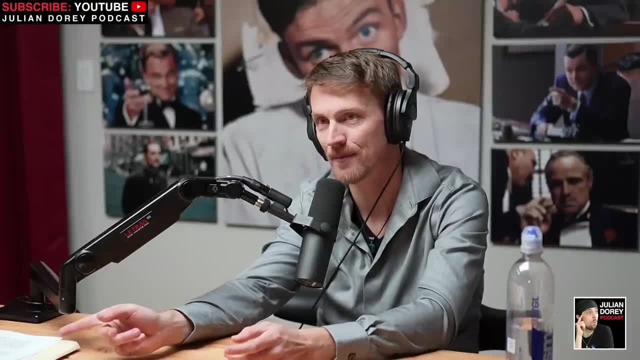 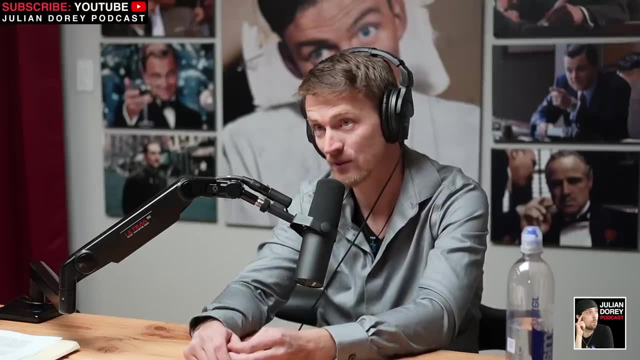 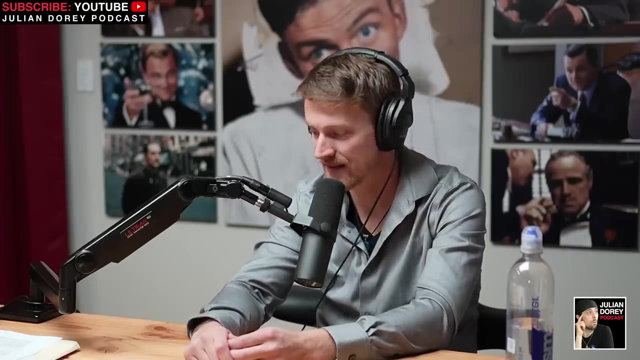 why? well, because we're connected to them. our, our looks like our karma, that chain, remember. i think our future is intertwined with theirs. we are them, they are us, we are part of. where are, where were they from? that's the question. that, and you start when you start trying to figure that out. 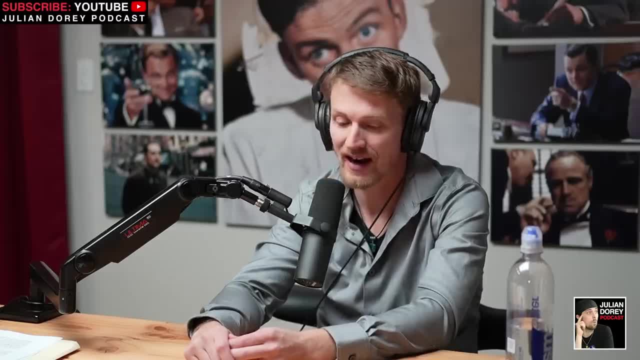 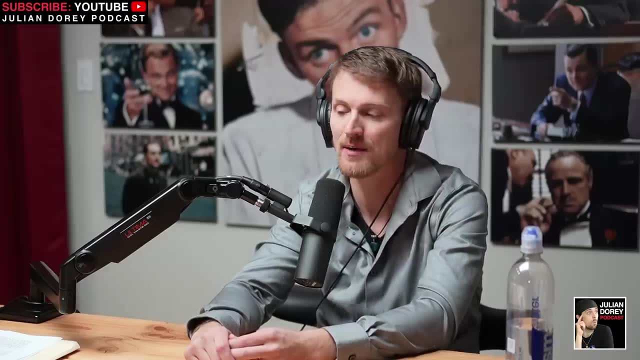 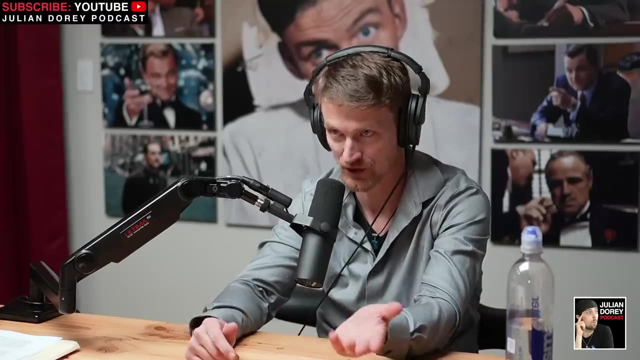 it gets really, really deep because i don't think we or they are what most people even that study it are. and now let me give you my conclusion that i've had to come to, and it's really difficult to come to this, but again, like that quote i just told you from the sherlock's home home quote. 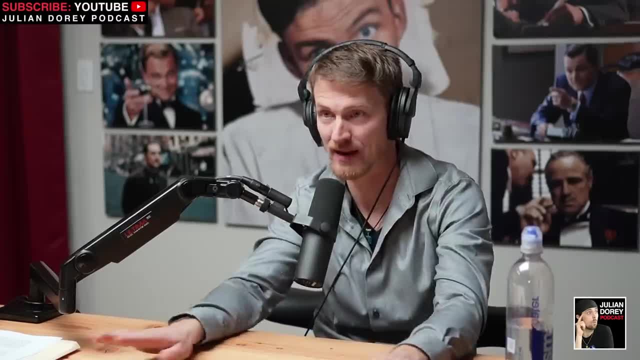 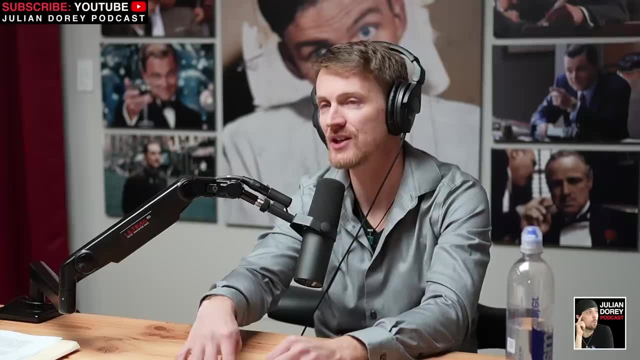 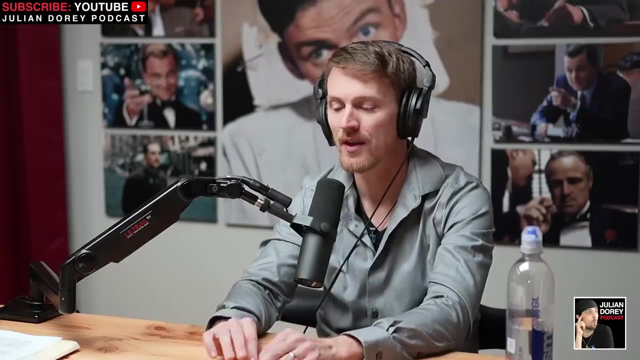 the only thing that makes sense when you eliminate all the other ones that don't, is that. look at, look at how angels and demons are described in later religions. okay, right, they're sort of like helping some are bad. whatever we see that context throughout the world, this idea of like angels and demons, 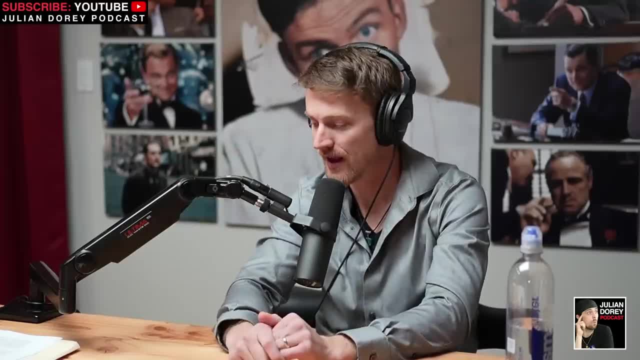 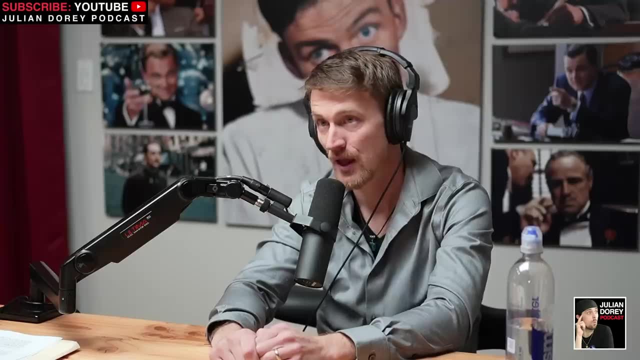 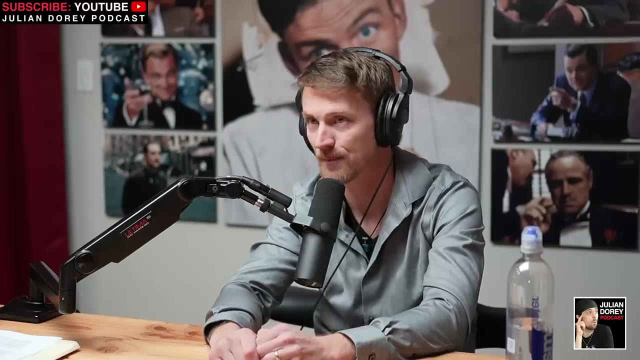 influencing our, our reality. right, they describe in all the tablets as coming here and creating everything they don't. they don't say they came and found like earth, like a, like a beautiful place. no, actually the complete opposite. they talk about coming here and fighting. it's a natural, the natural forces that were like out of control, like imagine an earth. 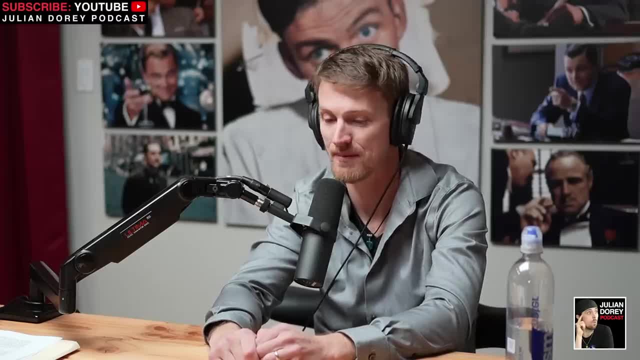 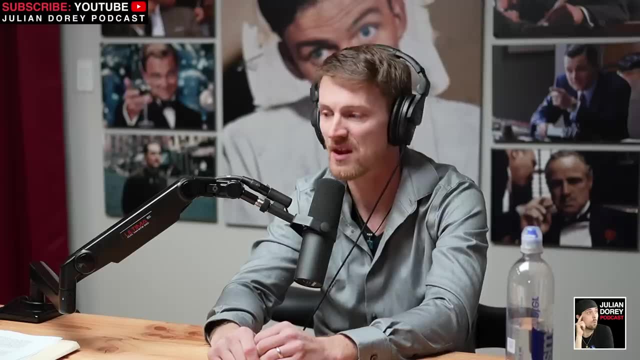 that had gone through different events and for, like maybe a, you know, thousands and thousands of years, hundreds of thousands of years, whatever it was. imagine a planet that was like no life: volcanoes going off everywhere, just like a, like a, and they tamed it. um, yeah, imagine. 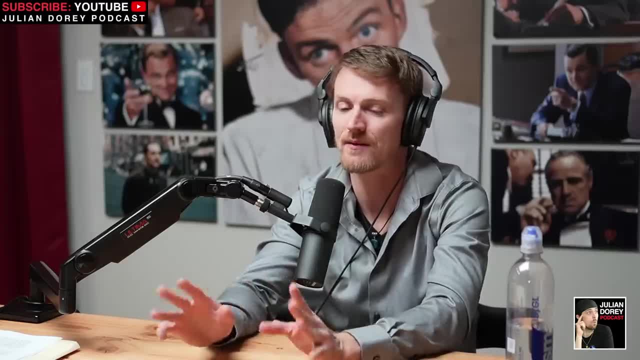 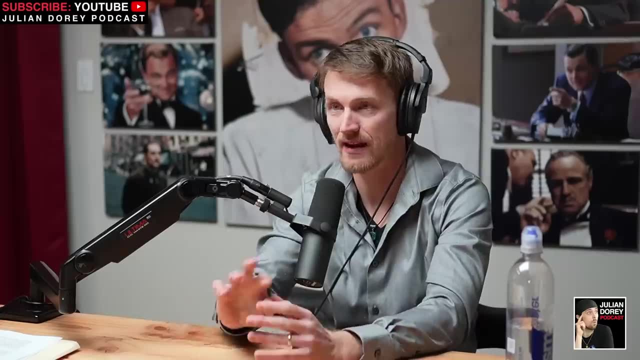 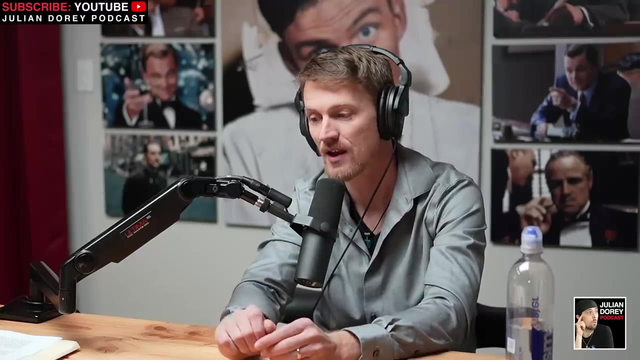 a planet like venus or something, or you know, not having a physical, a terrestrial planet though, but that's the only thing that makes sense, like if you read the enumeration and others, like with george's clip chaldina, count of genesis. i told you backwards and forwards, um, george smith, it's like they're. 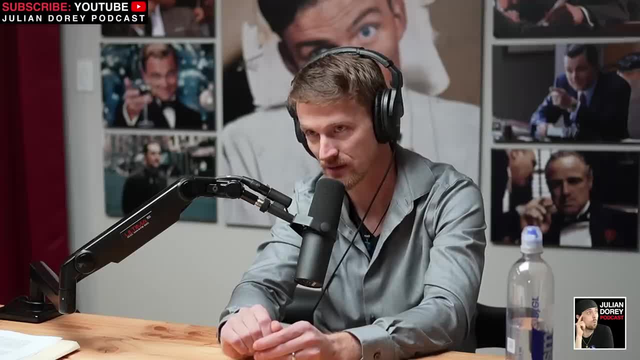 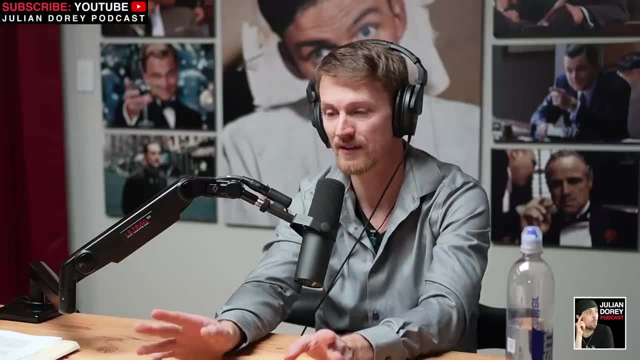 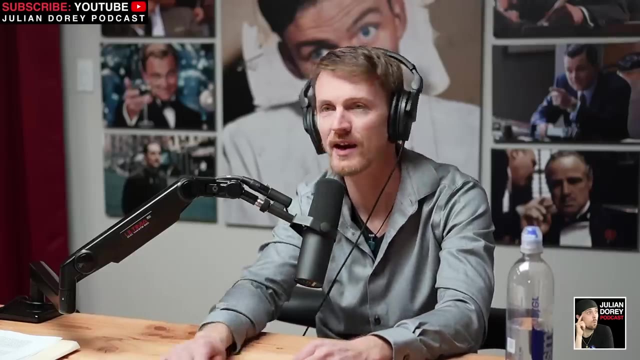 somehow related to creation in the universe. let that sit with you for a second. imagine there's a- there's a prime creator. okay, this is how they describe it in in the tablets. imagine there's a prime creator that it's like the underbelly of everything, the. the golden ring is the golden ring. 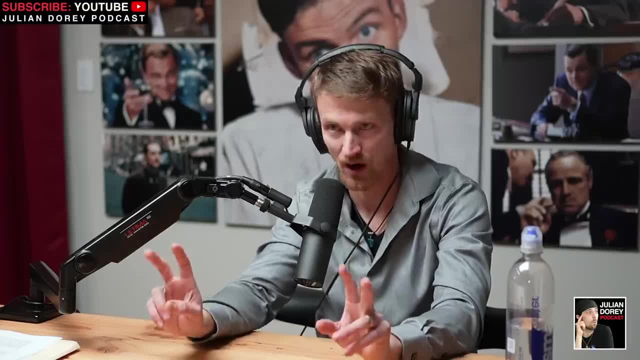 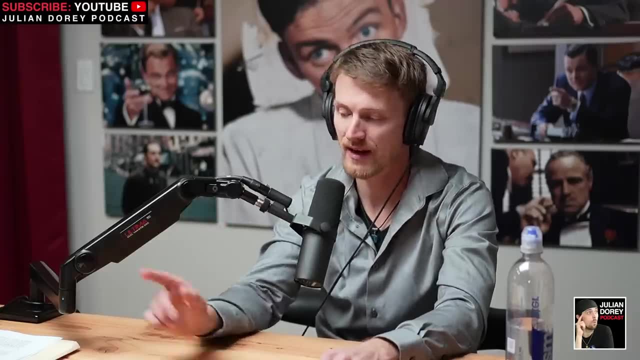 ratio, the balance of nature and harmony, and they describe that as being God. That's what God is to them. is nature and the balance in everything right? Well, in the Christian text and other ones, they just: they talk a lot about creation, though right, And people are like: 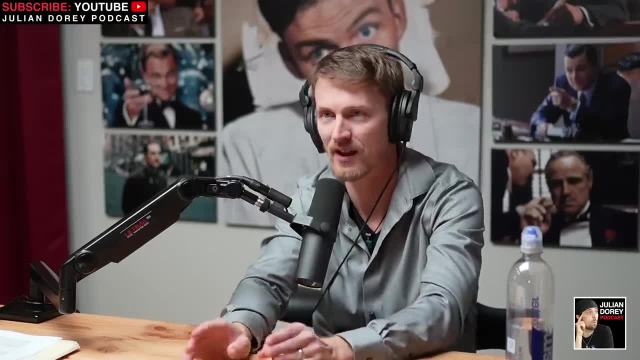 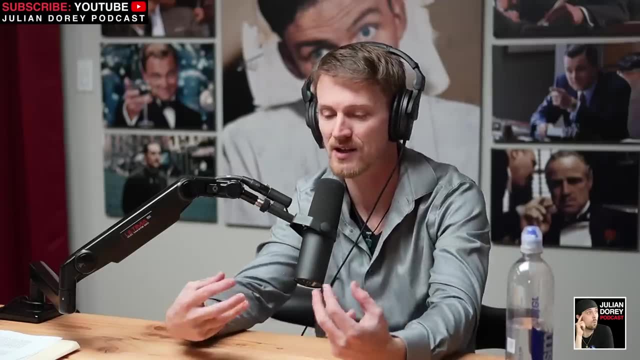 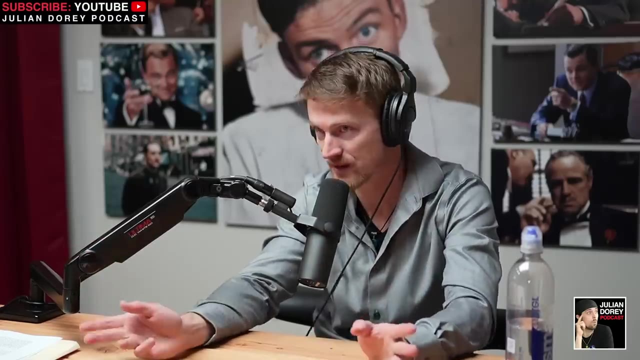 oh, my God, you're a creationist. That's insane, right? I'm not a creationist. I'm trying to explain something, though The way that they say it in every time. there's only one way they say it is. they describe it as more like manifesting things here. right, That's what they describe. 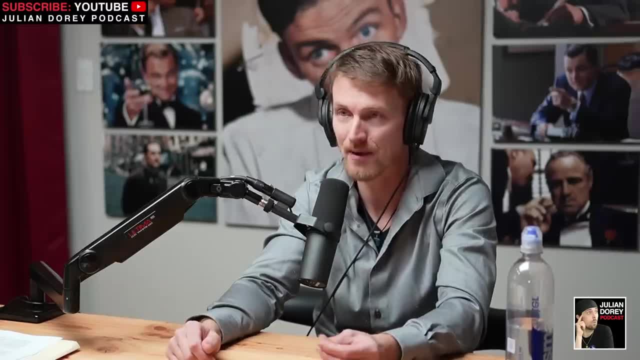 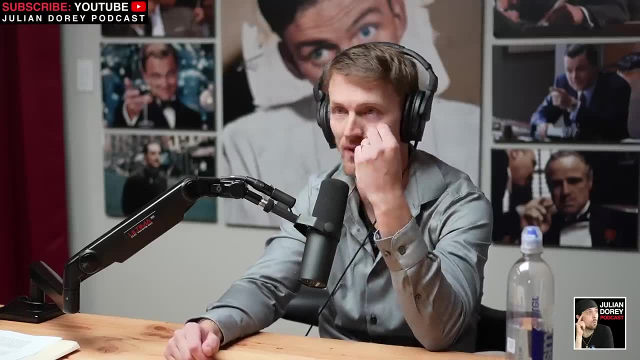 it as like they can just create whatever they want, And that maybe the reason why we're so powerful and why I can have a thought to call Julian Dory, and why Julian Dory all of a sudden has that thought in his head, is because we are creators too. We just don't know it and we don't. 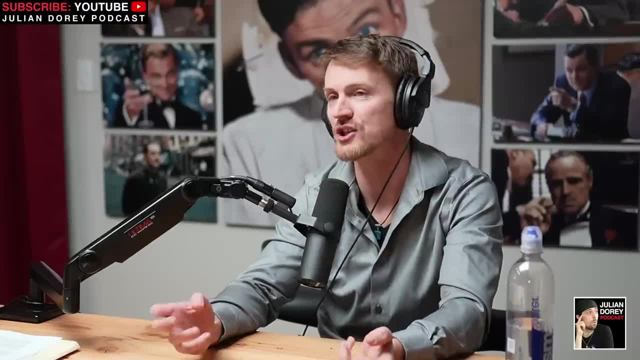 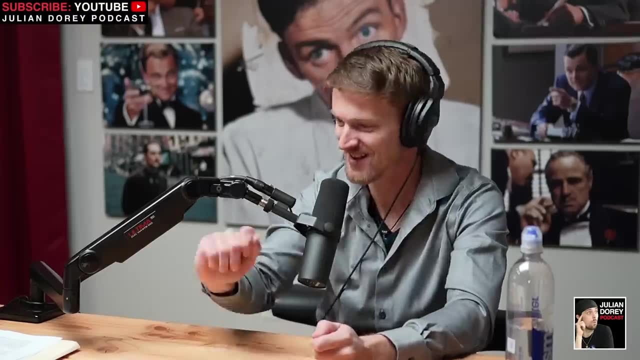 understand it, And we're like children Creators. how Well. I think we're like children right now. I think we're like children, Like you just said, we're like banging on stuff As a civilization- Yeah, As humanity. 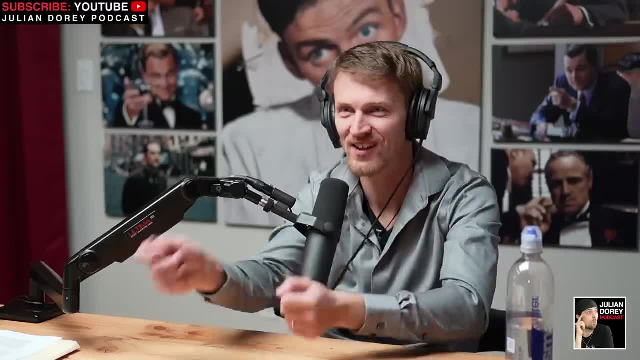 We're like children And we're like: what does this do? And we're like: you know, I don't care if we have technology or not, We don't know anything about the universe. We're like whatever, Like we're kids with big guns. 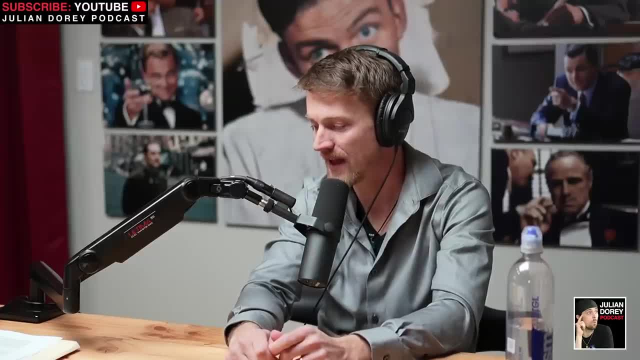 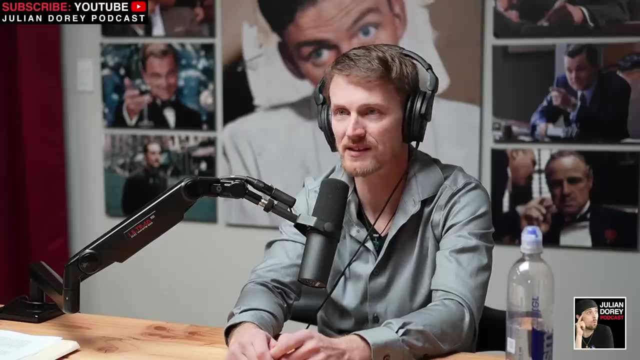 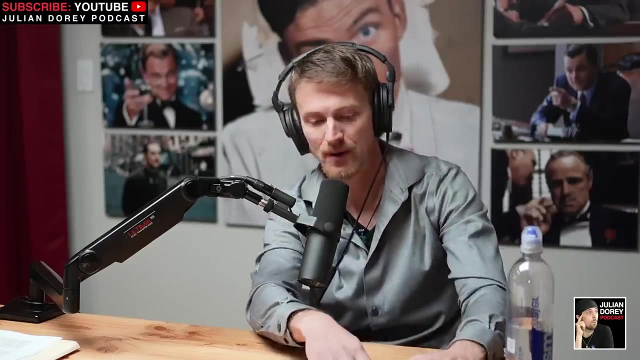 Big nukes, Right, But imagine, though, is that we have a lot of things dormant within us- our DNA and within us- that we don't remember and that has been lost long ago. If you have a number of like, let me give you an example. If you are someone who practices a skill like, 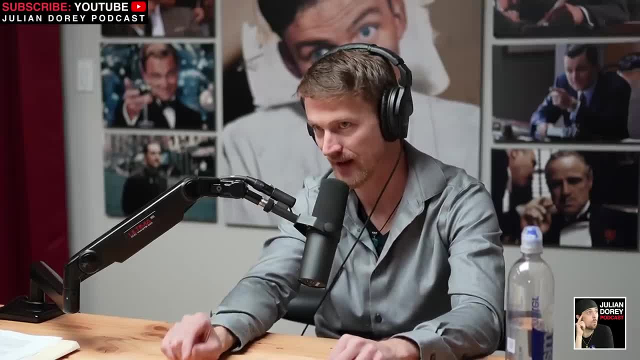 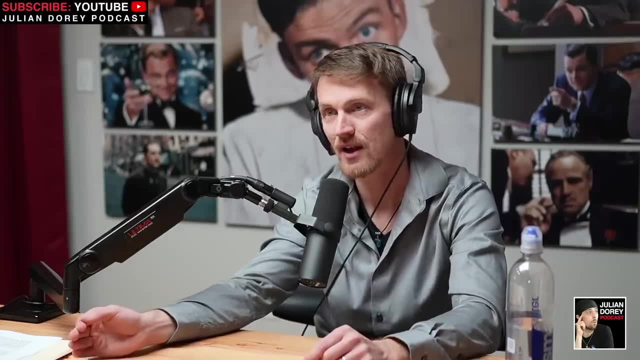 your whole life. you can actually pass that genetically. Athletes have often been shown to pass some genetic skills to children in ways where, like they're just really good at baseball, like their dad is right. Maybe that's a purely genetic thing, but 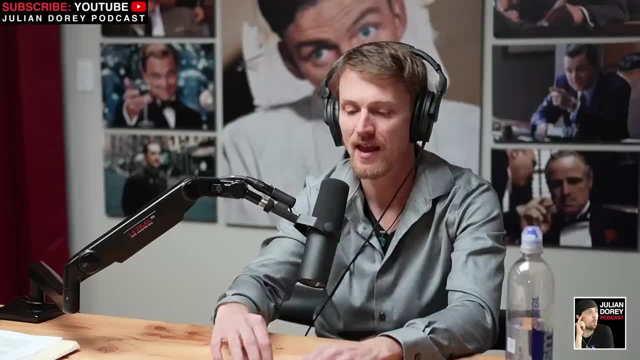 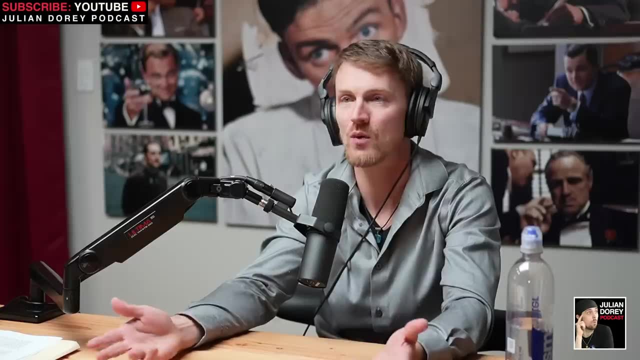 Has to do with their hand-eye coordination, Exactly, But what if there's a whole nother side of it, though. What if there are all these things that we don't remember how to do? Like you said, we're those kids that haven't learned how to do any of. 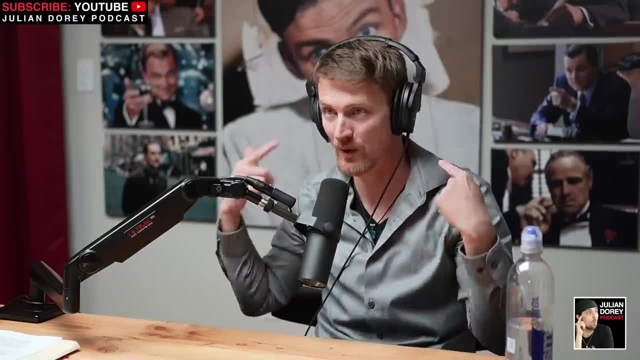 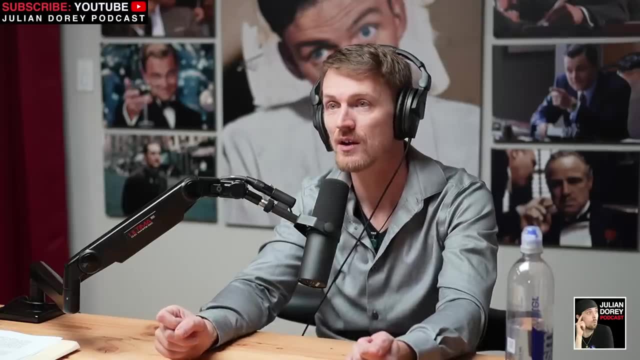 those things yet, And that all these things that are happening are so that we can grow up, And then part of us living in these lives and being here is to grow up as a soul, because you know that phrase where with great power comes great responsibility. 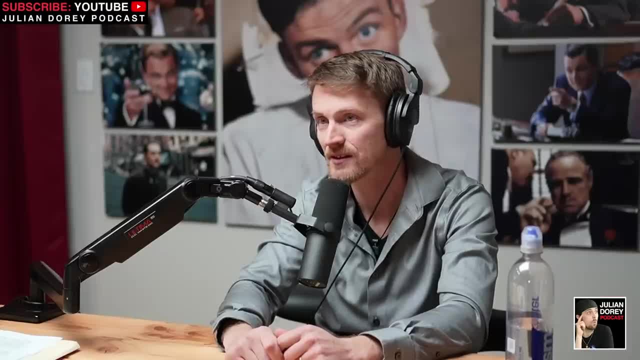 Yeah, Peter Parker's uncle. I think that's us. I think that we're not allowed to achieve what we can until we're ready. I think we're too immature, I think we're too small-minded, I think we're too childlike, And I think that 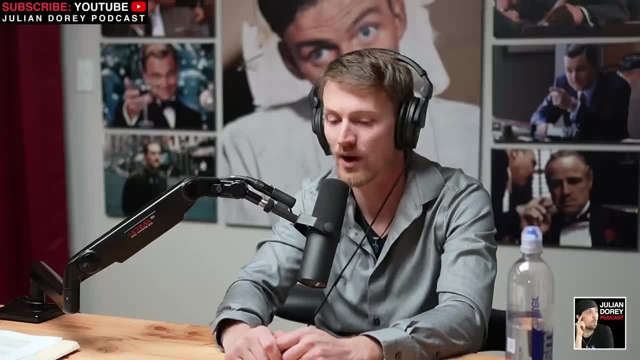 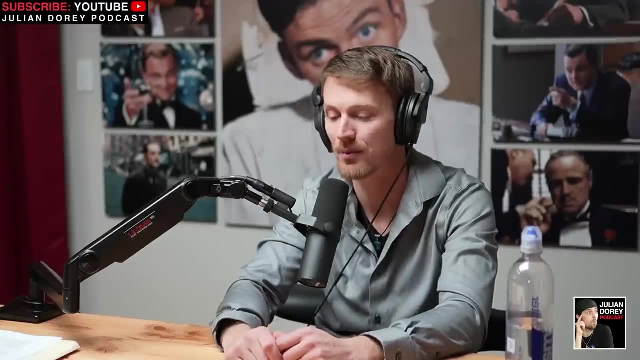 that's a collective understanding of when our consciousness can finally be ready and we can get to a place where we can be. That's your working theory on it Is that once we can get to that place, we're going to see an acceleration in humanity. that's going. 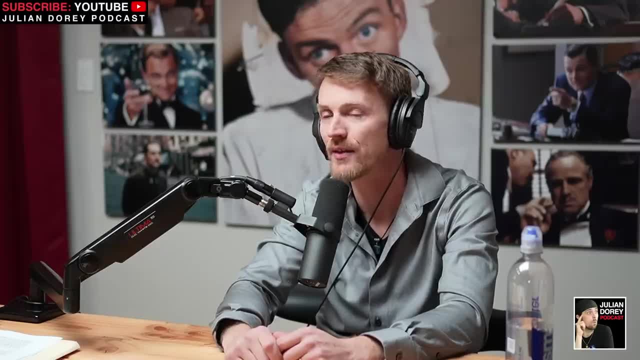 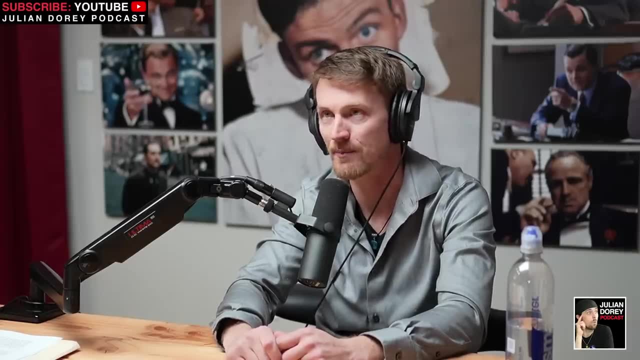 to lead us down a path that maybe we don't necessarily expect. Rather than just getting these high tech spaceships and all this technology, like what if the real journey is about going inward, to these high states of consciousness, And then maybe we can travel like anywhere in? 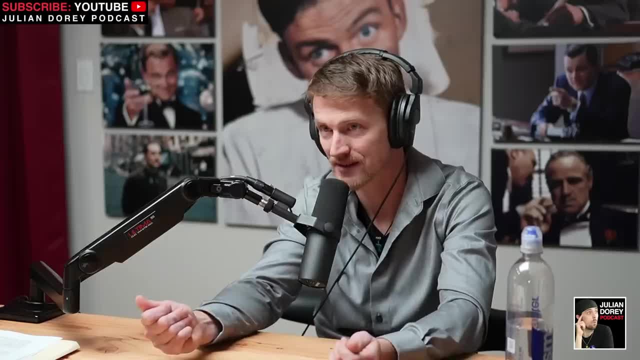 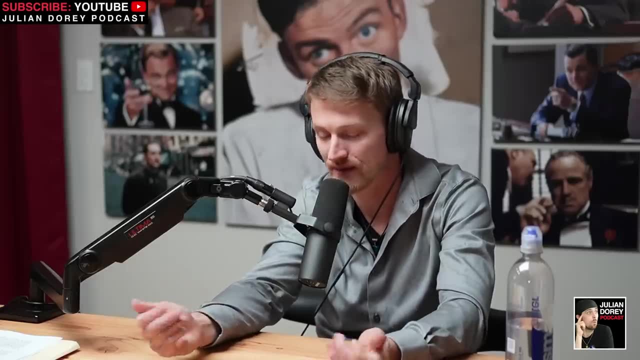 the universe instantly, because consciousness is not localized And then we're looking at It's going to get weird, Like we're going to become. I think we're going to eventually Here. I'll just throw this out there, but I think we're going to eventually become. 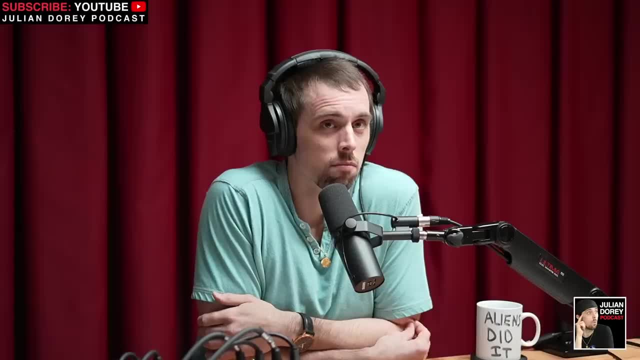 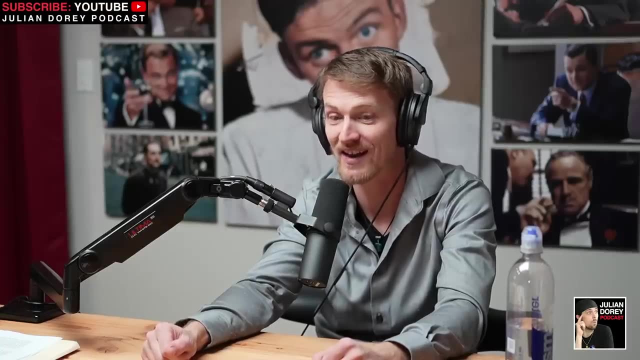 The choice to become non-physical and interdimensional. That's what we are at our core. We are interdimensional, powerful creators. that the game is like: hey, let's just throw them into a war, chaotic place and let's have them forget everything. Let's see if they can make it back. 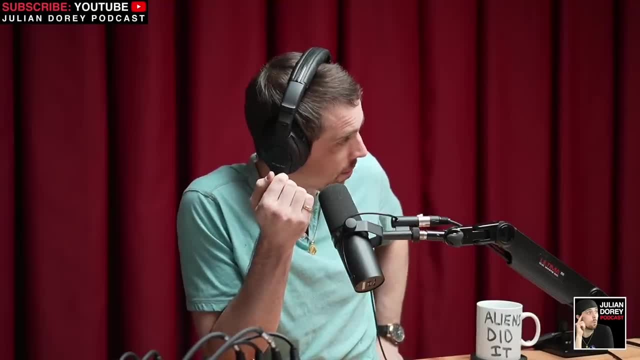 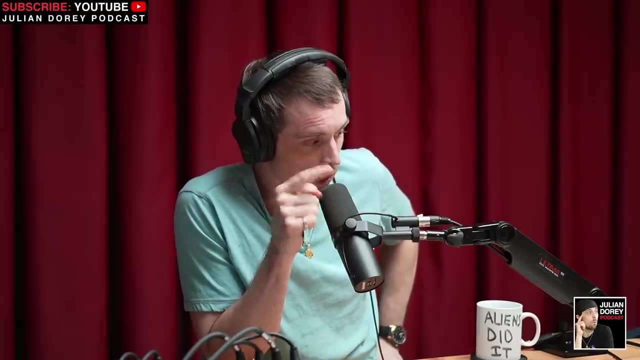 All right, So here's what I'm going to do. I think we got to be just over three hours, Is that about right? Yeah, Okay, I got you here all day tomorrow. Yeah, So we can do another one. Let's stop there. 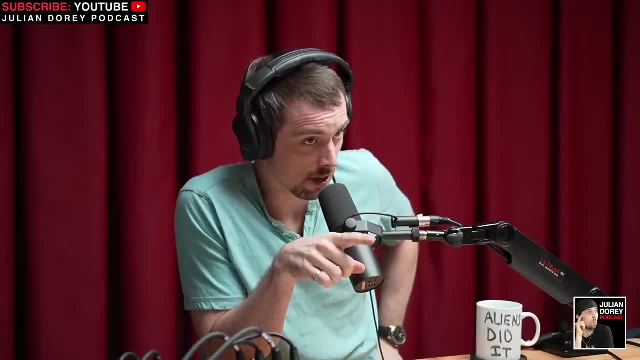 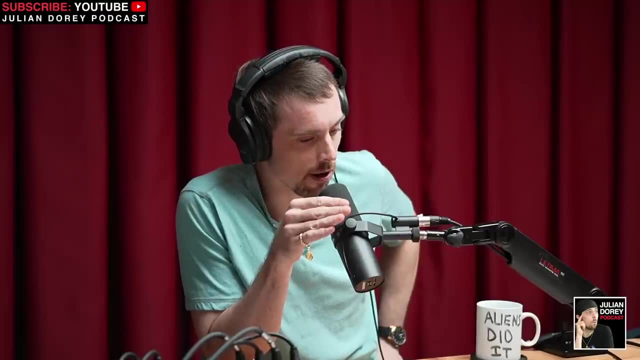 Sure, We'll go get some dinner, We can dig into the interdimensionality argument. That is a whole rabbit hole right there. It's very fascinating to me. People love that stuff, though- They really do. I want to talk all about South America with you, though. 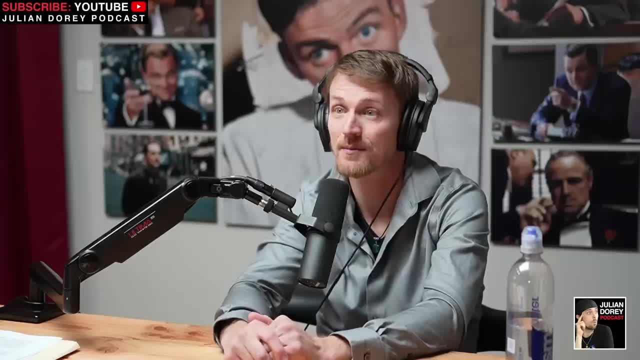 Sure, Yeah, You and I have a lot to unpack with the fucking pyramids. Yeah, Yep, There's a lot that we did not get to today, So let's fuck it. Let's do it again. Let's do another one. 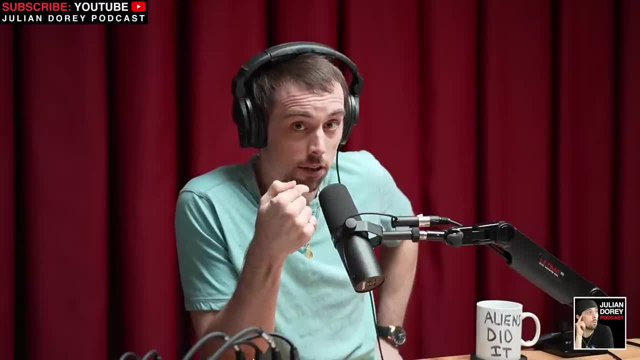 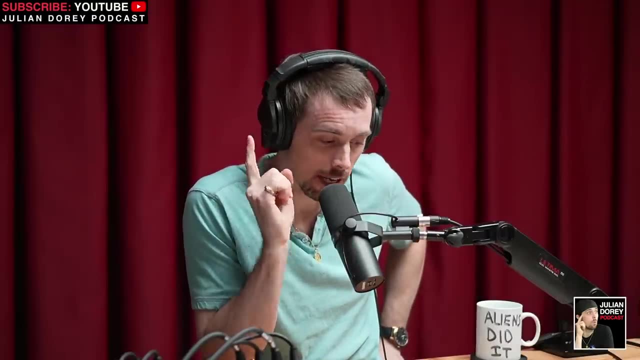 How do we end that one? though? I'm ending it right now. This is me on the fucking mic doing it, So let me end it. This guy directing the fucking show, All right people. So hit that subscribe button, Hit that bell button as well, So you get notified when we. 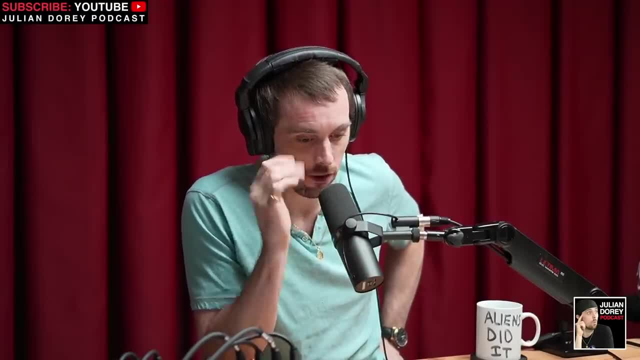 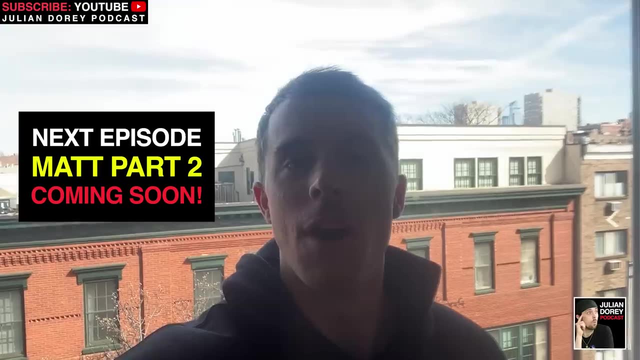 have the next one coming out. We're going to be putting on another episode with Matt after this one, probably within the same week, So keep your eyes out and give it a thought. Get back to me. Peace, All right guys. that takes us to the end of part one of my two part. sit down with Matt. 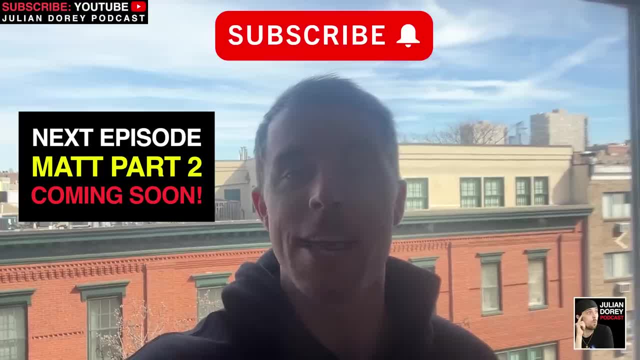 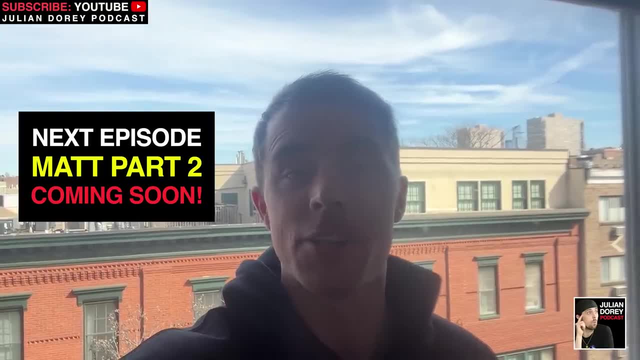 LaCroix. This next episode is going to get deep on Atlantis And Matt is going to take us through a theory that you've seen around the Internet a lot and why he actually disagrees with it. We also talked about categories, The Vatican, much more. It's a loaded episode. I think you're really going to enjoy it. 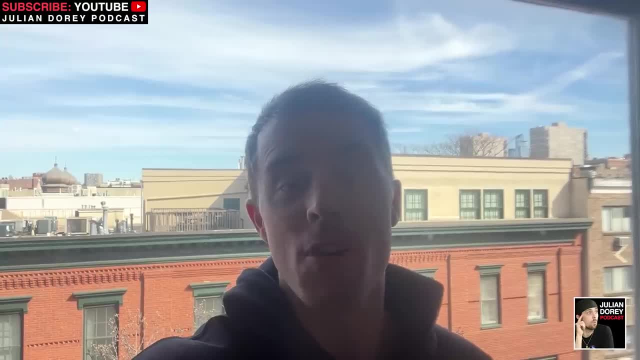 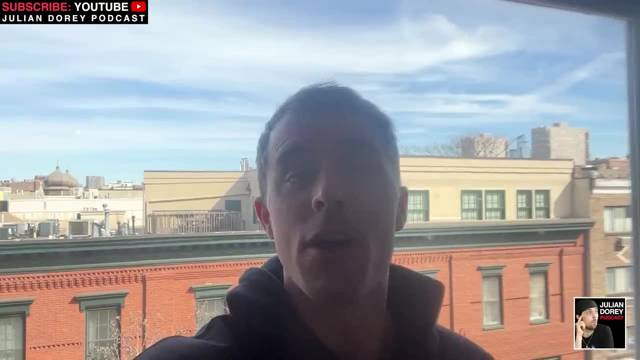 So if you haven't already hit that subscribe button, please smash that subscribe button right now. Hit that like button on the video. Also hit that notifications bell so you find out when the new episode comes out in a few days And also if you're into an episode like this if you enjoyed. 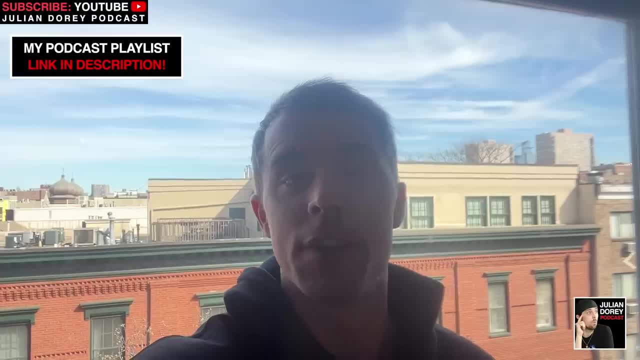 this one. there is a playlist down below, at the top of the description, that takes you to similar episodes we have recorded on the show, So be sure to check that out, And I'll see you guys in a few days.